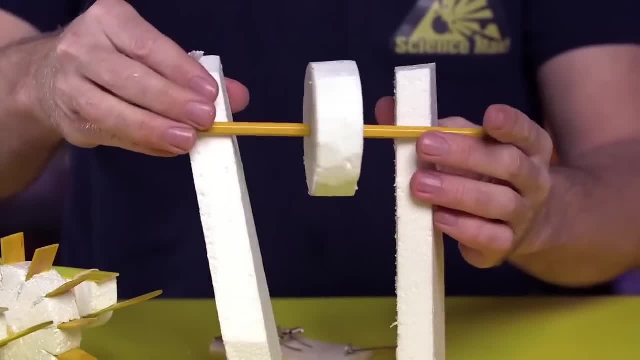 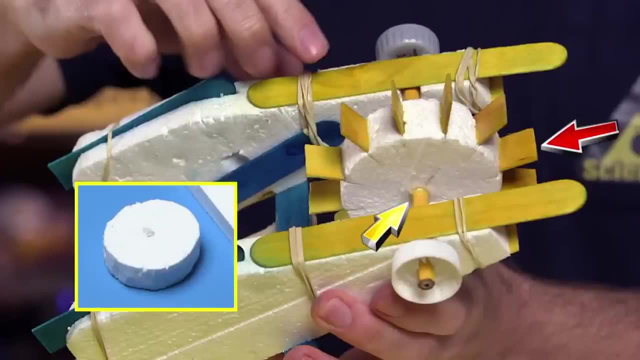 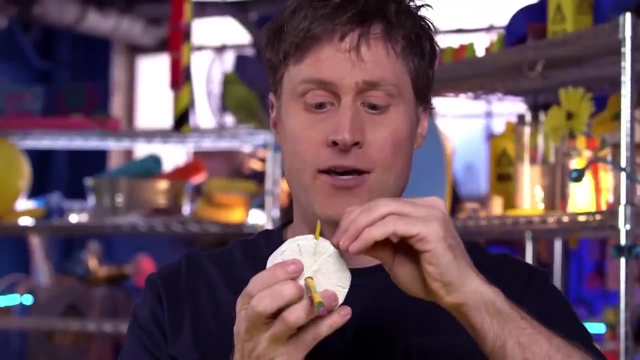 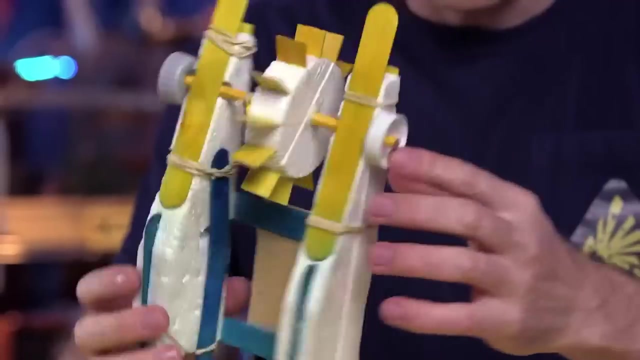 the same size. Your paddle wheel is made from a circle of styrofoam with a pencil through the middle and it will go across like this. To make the paddle wheel I use cut pieces of craft stick- Or they can be plastic- and make some cuts and then put them in like this And that is what will make your paddles on the paddle wheel, Because that's the wheel and that's the paddle Paddle wheel. That's why they call it that Stick drink caps to the ends of the pencil after sticking it through the styrofoam. I like to use a few craft sticks. 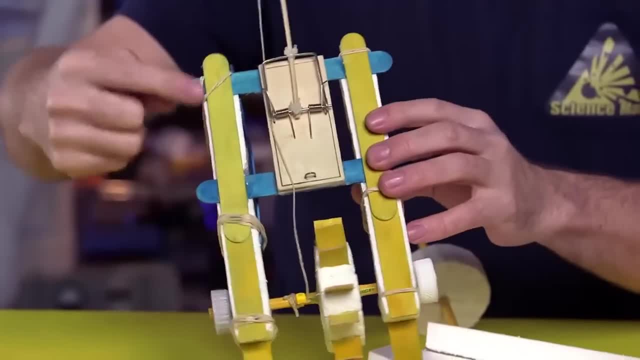 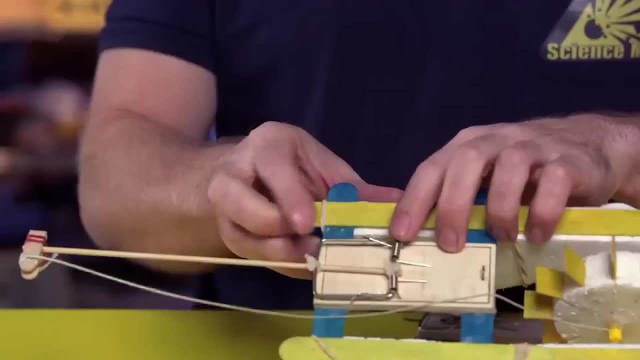 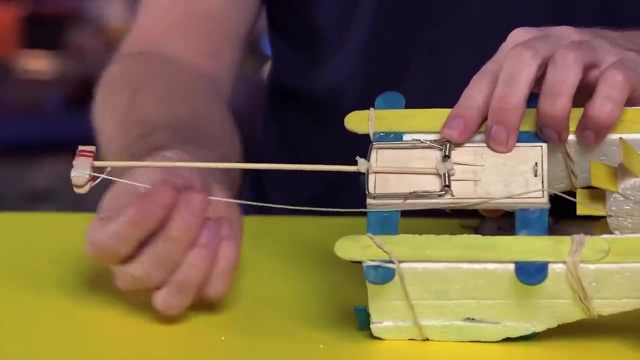 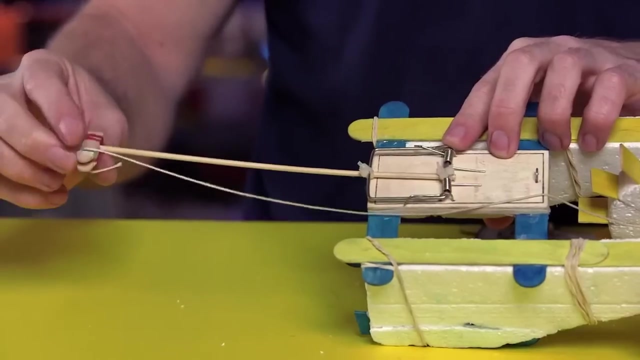 and elastics to help give the styrofoam strength. Next is the mousetrap, which you want to glue down to a frame of four craft sticks. Attach the frame to the boat with elastics, then attach the shish kebab skewer or a pencil to the mousetrap with zip ties. I like to put some craft sticks on the end to make it easier to tie the string to it. Wrap the other end around the paddle wheel pencil and remember you need enough string so that your stick can lie flat. Okay, let's try it out: Wind up the paddle wheel. This will be a little hard. 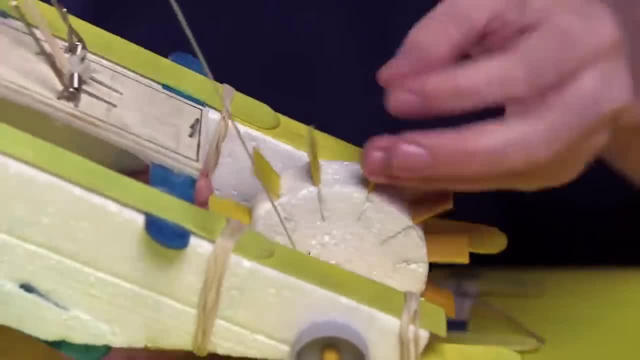 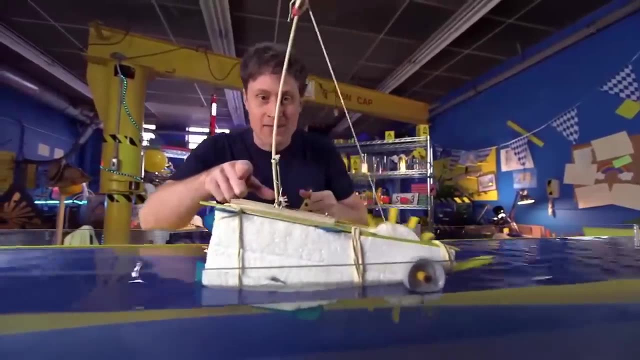 as the spring will pull back. but that's where you're storing the energy And when it's wound up, put it in the water and let it go. The paddle wheel turns because the mousetrap is transferring energy that we put in earlier and it goes all the way. We stored the energy in the tension of 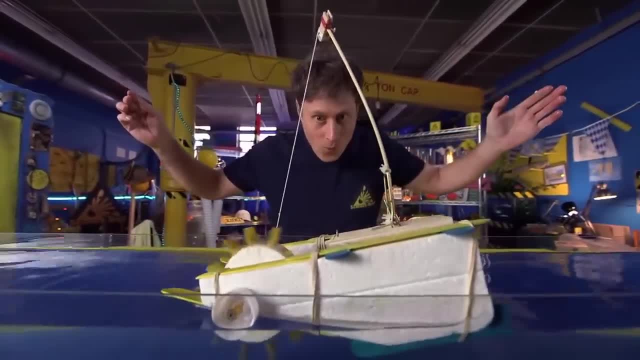 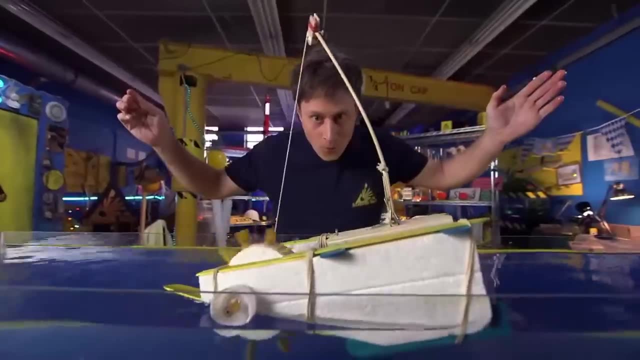 the spring, Now that tension is pulling the mousetrap, the stick and the string which turns the paddle wheel and makes the boat go, Mousetrap powered boat. If you want more detailed instructions or other designs, look up mousetrap boat And there you have it. 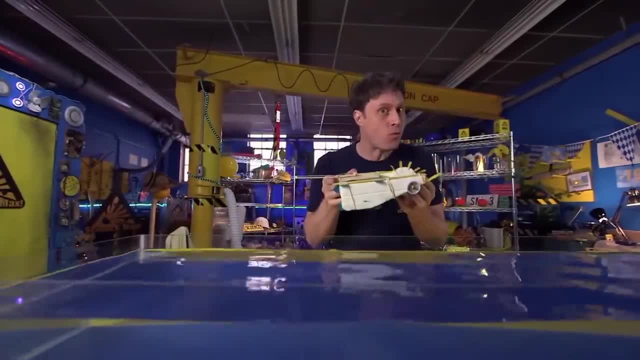 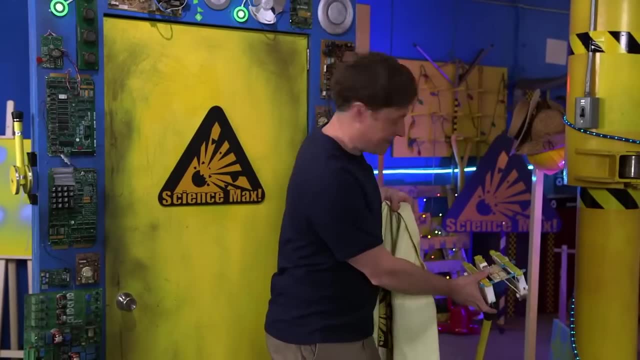 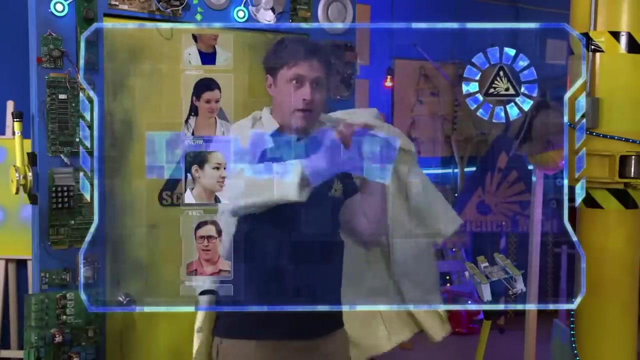 the mousetrap powered paddle wheel boat, And this is what we're going to max out today. Come on, All right time to pick an expert and go off to max it out. Careful, Okay, let's see here. And, uh-huh, Who to pick? Ah, Michaela from the Ontario Science Centre. She'd be perfect, All right. 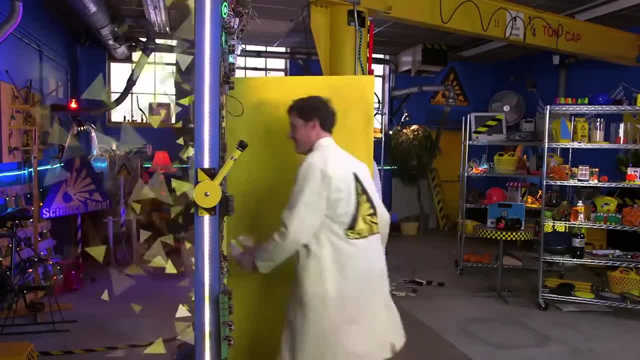 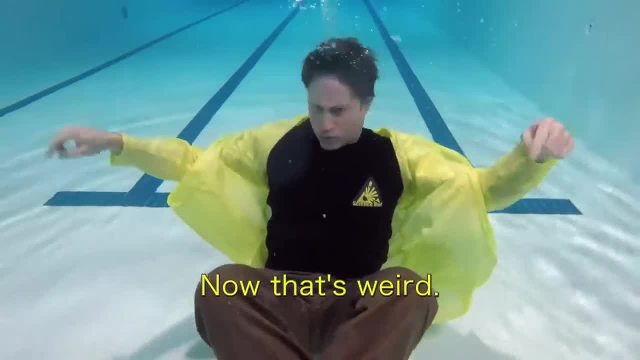 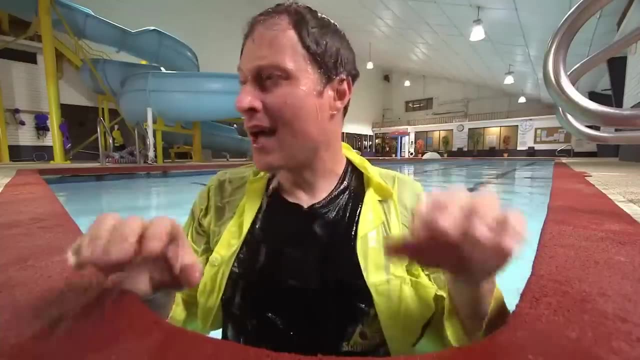 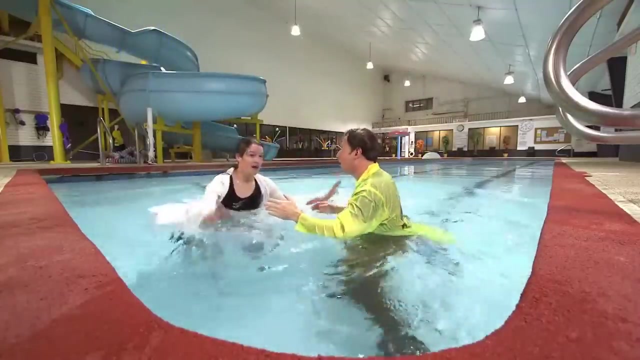 Come on, I ended up in the water again. Oh well, at least maybe Michaela made it. Oh, Michaela. Whoa Phil, Are you okay? Are we still fixing the portal? Yeah, I needed to wait for just a little bit. It was uh, it's a little off again. 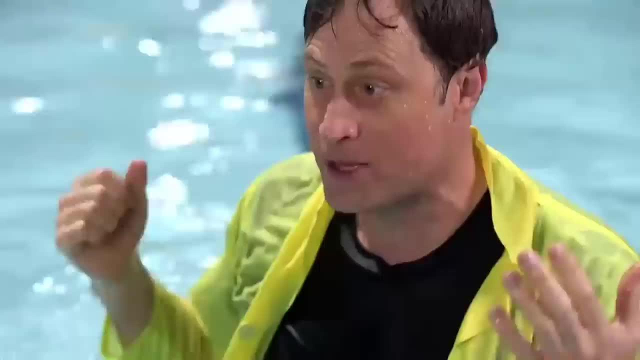 Anyway, great to see you, Michaela from the Ontario Science Centre. You're going to help me max out the mousetrap boat. Awesome, Yeah, Wait, where's the boat? I, yeah, I don't have it It. 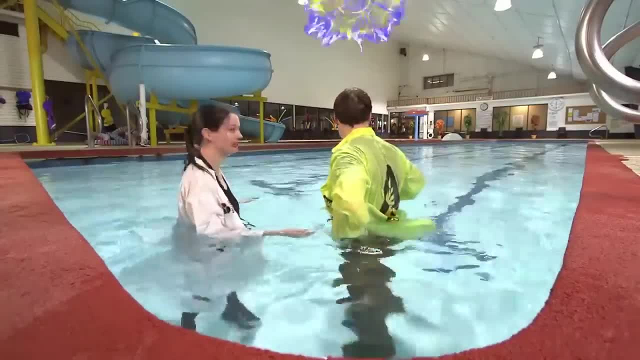 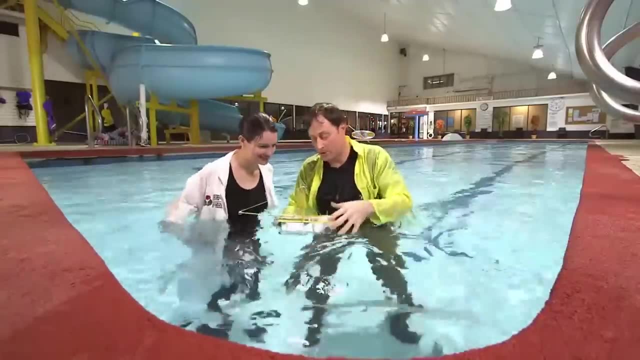 I thought it was going to come through the portal. Um, it could be anywhere, really, What? Oh, here it is, Okay. good, So here is the mousetrap boat, Check it out. So, got a mousetrap here, right, And you wind up the paddle wheel and it goes, Yeah, right on. 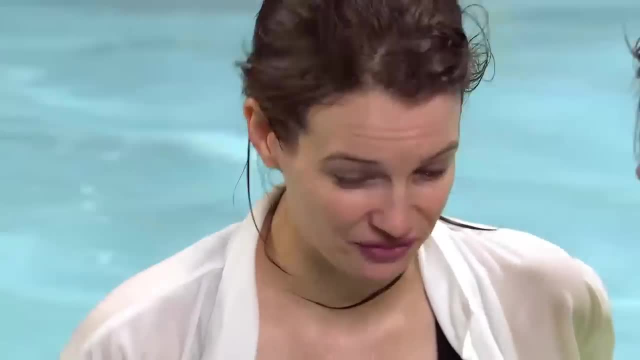 So what do you think we should do in order to max this out? Uh well, first idea: I'm just thinking: more mousetrap, More mousetrap. So we just make a boat and it has like ten mousetraps on it At least. Okay. 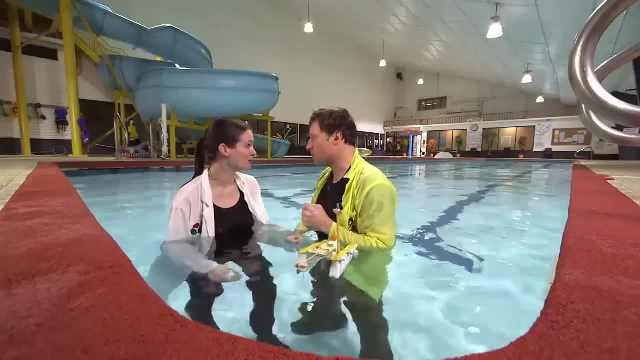 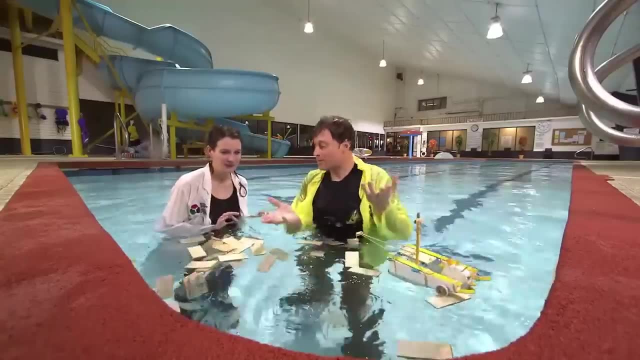 great, Actually, I had mousetraps. I had mousetraps coming through the portal as well. Oh, okay, Okay, Okay, we're all right. Okay, so now we've got the mousetraps, We can start building. 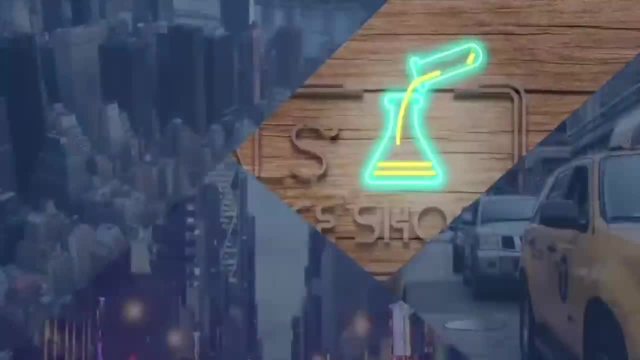 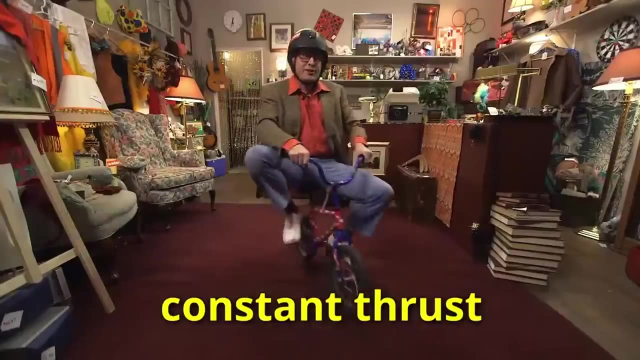 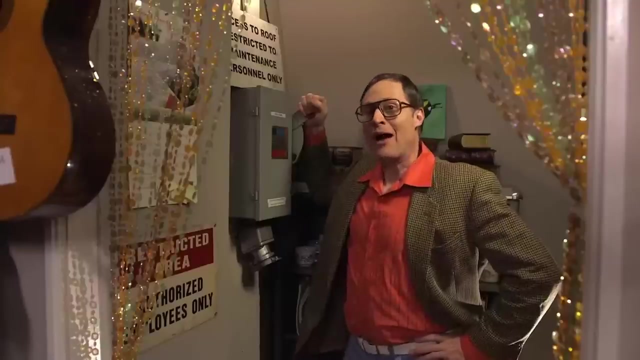 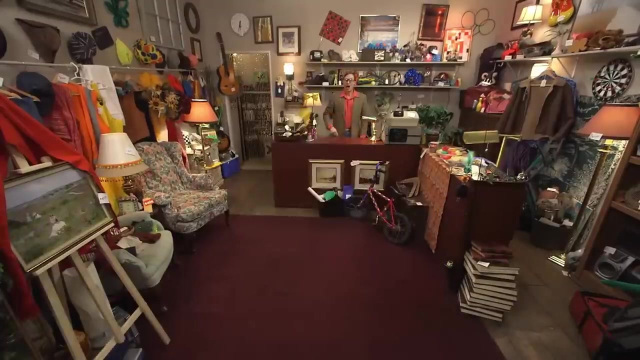 Let's collect them carefully, though. I don't know if they're Initial thrust or constant thrust. What's the difference? It's all about power. Ha-ha, Uh-oh, Paper airplane. initial thrust: It gets all. It gets all of it. It gets all of its thrust from my throw. Ha-ha- Initial thrust. 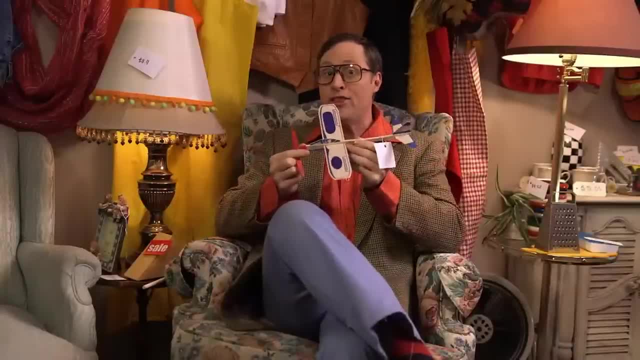 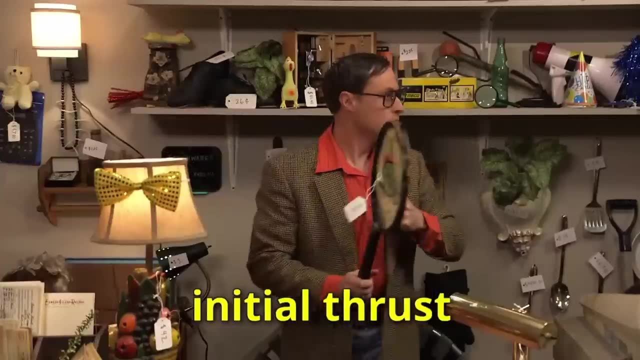 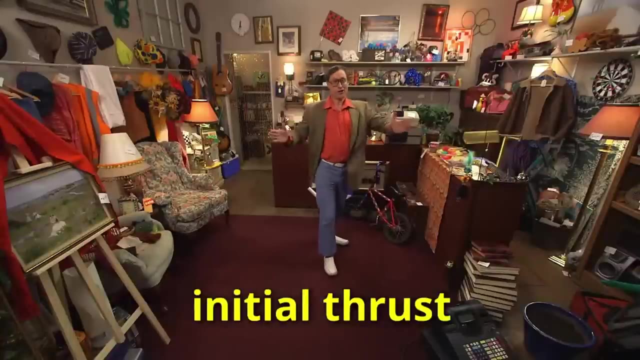 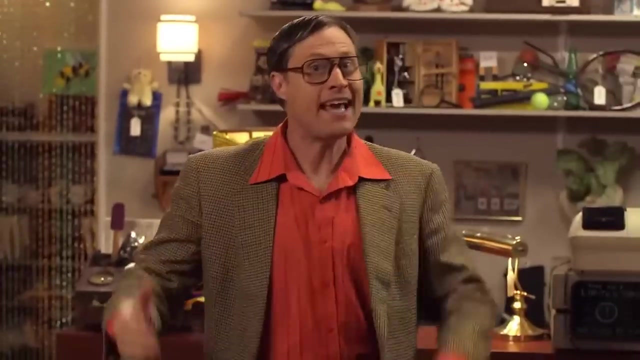 If you want constant thrust, you have to take the thrust with you like this- There's a lot of cats in here- Initial thrust, Initial thrust, Initial thrust, Initiative thrust. All the energy is put into the beginning. All the energy is put into the beginning. 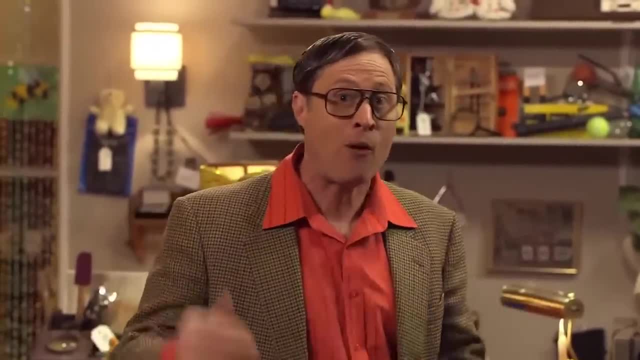 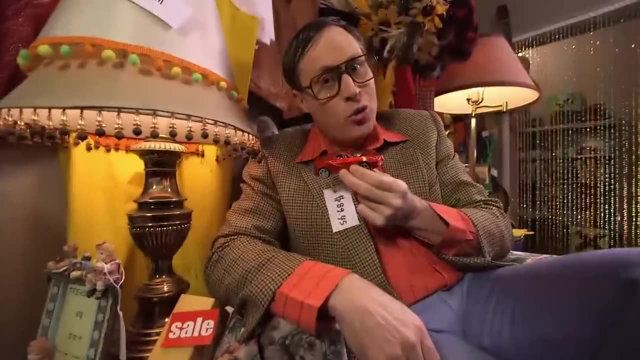 If you want constant thrust, then the thing has to produce power while it's moving. Windup car: Constant thrust, Actual car- Yeah, that's constant thrust because you have an engine. Of course not this car. This is a. 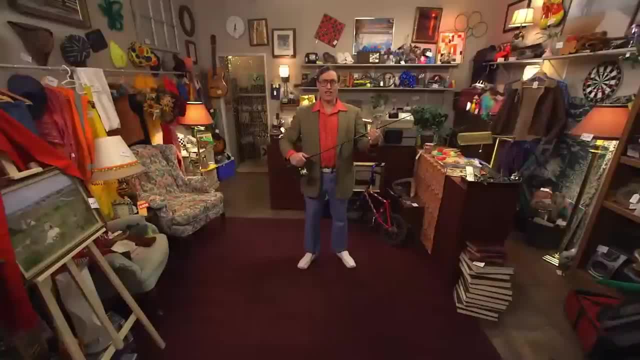 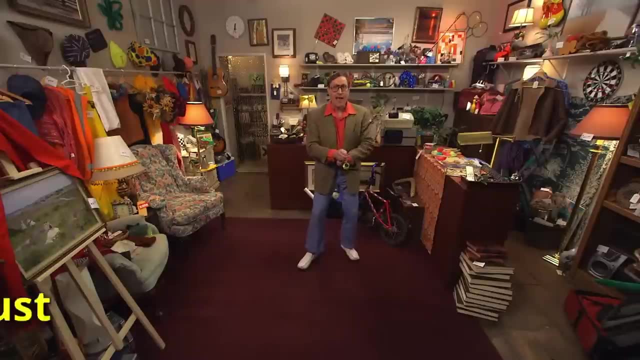 This is a toy car, but you know what I mean. Check out this fishing rod and on it I have a lure with a hook. Now watch this. I cast it out, initial thrust, but then I use the reel and start winding it back in. 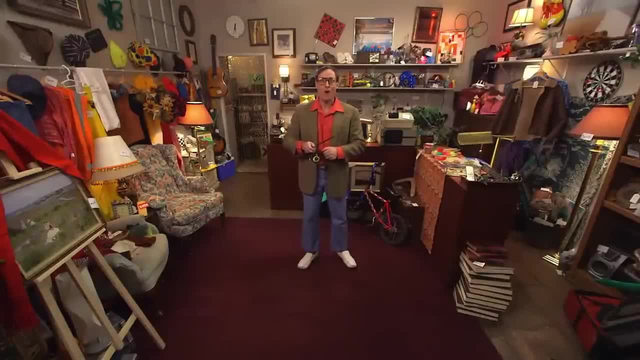 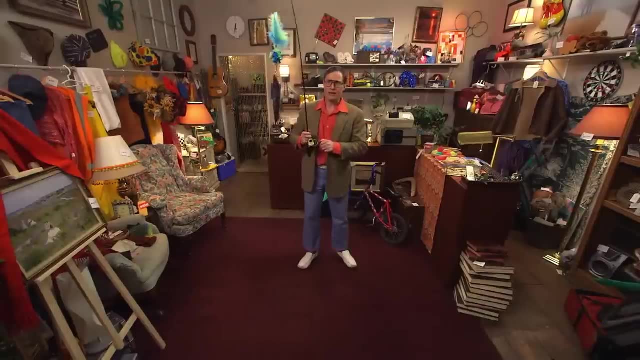 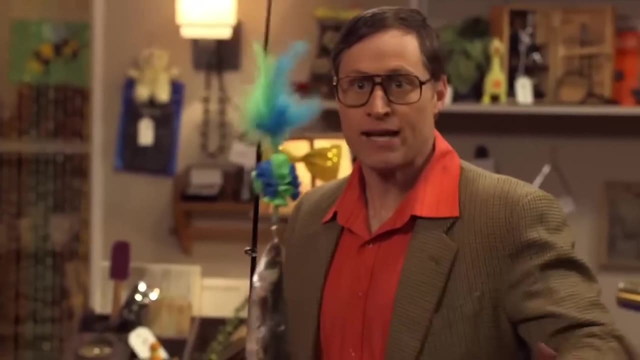 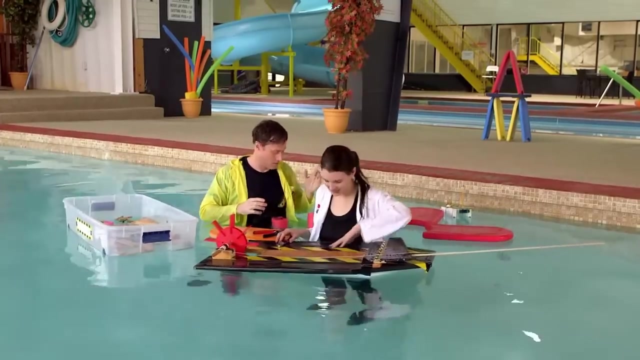 constant thrust. huh, Two thrusts in one. and now you know the difference between initial thrust and constant thrust. Hey, I caught a fish. Hey, hey, hey. Easy kitty, Nice kitties. Easy, Ramona, Michaela and I are maxing out a mousetrap boat. 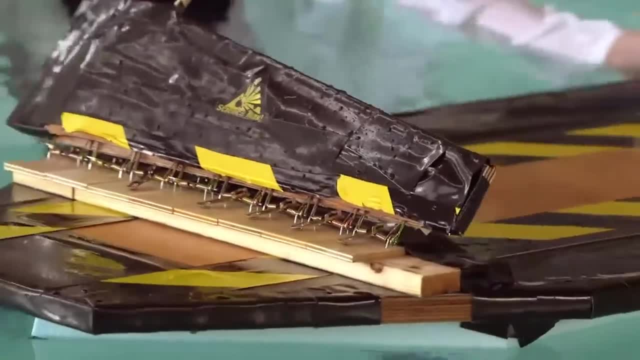 We built a larger version with ten mousetraps all in a line, So it looks pretty good. I think we're ready, right? Yeah, I think so. Got a whole bunch of mousetraps. Should we wind it up and see what happens? 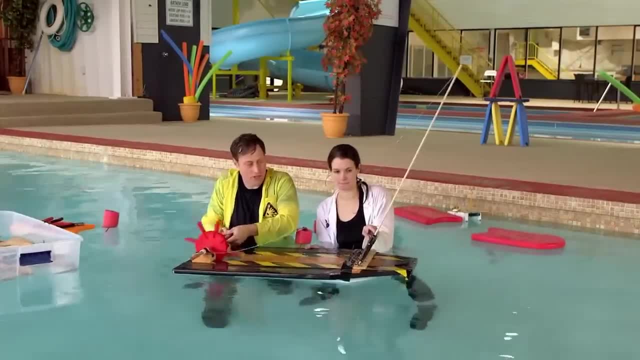 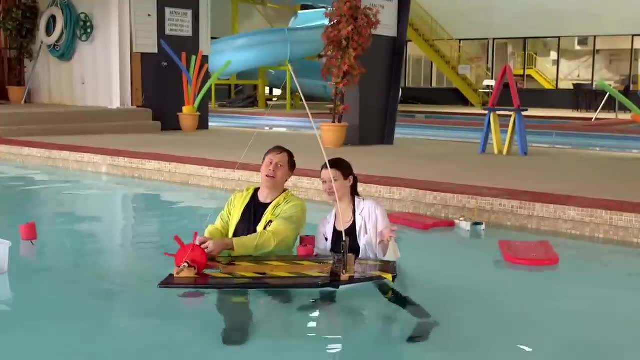 Let's do it. I think this is going to go pretty well. What do you think of that stick? Is that going to bend Too much? Is that going to snap? It looks pretty flexible. I think we're okay. I think we just keep going until it breaks. 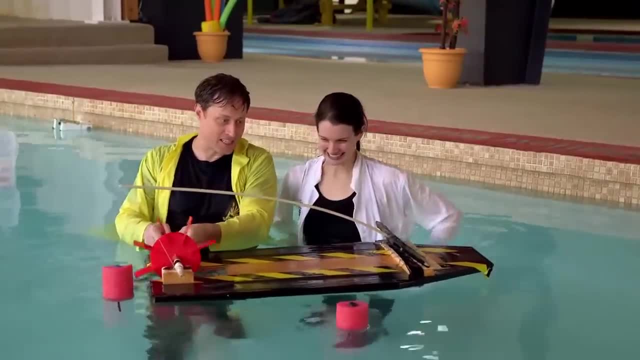 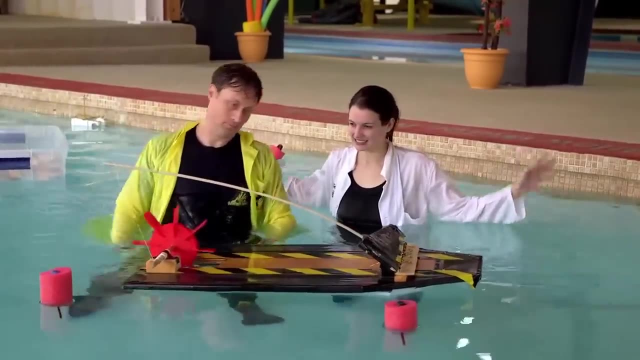 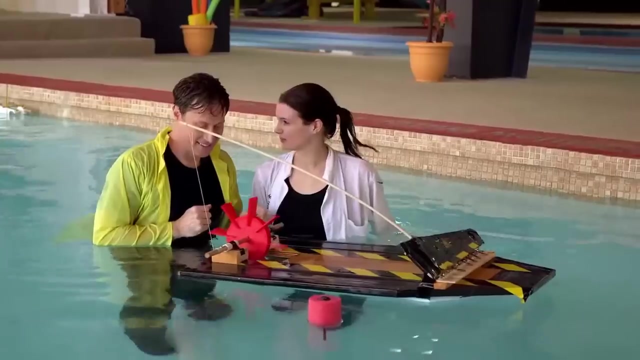 Now it's starting to look very fast. Yeah, like it looks like a speedboat. Okay, ready, Well, positive, It is working. It's not going to win any speedboat races. It is not going to win any races at all. 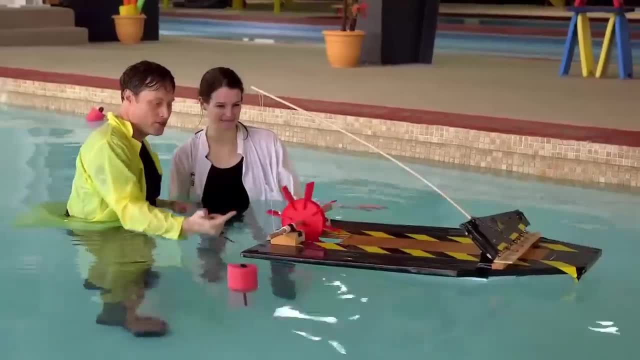 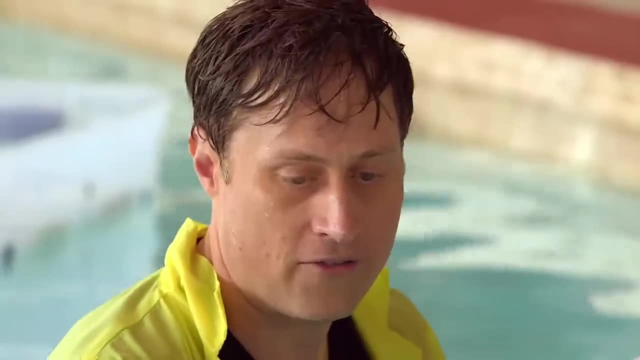 But it's totally working. The mousetraps, they're pulling on the string. The string is making the paddle wheel turn. Just not much. I would have thought this many mousetraps would be a little bit more effective. Yeah, it looks like we're going for distance over power things. 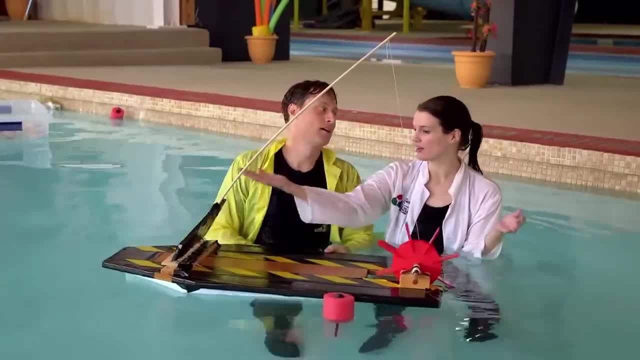 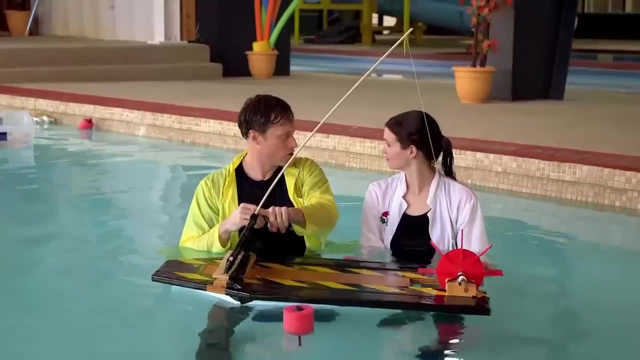 Oh right, That's a lot of distance for this to travel. Small amount of force over a much longer distance. That's how a lever works. So we slide the rope down further on the stick. Then we would get more force and it just wouldn't go as long. 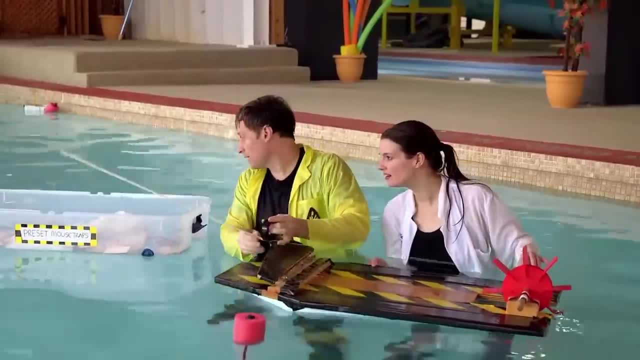 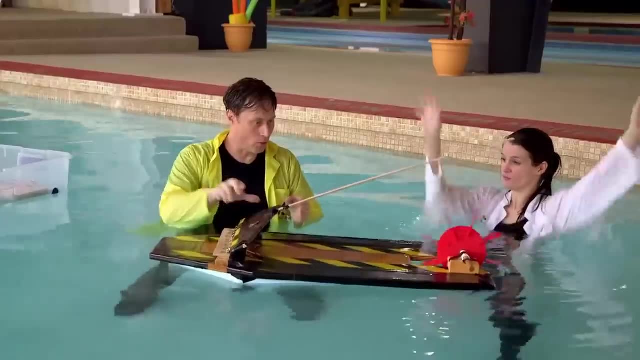 Okay, so why don't we try that Wrapping like that? Nice, All right, Once again. Trial two: Okay, Ready, Ready, Set Go. Oh, Yay, That went better than last. Oh, now it's picking up. 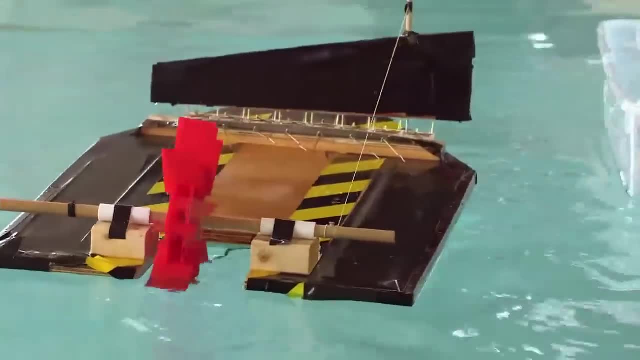 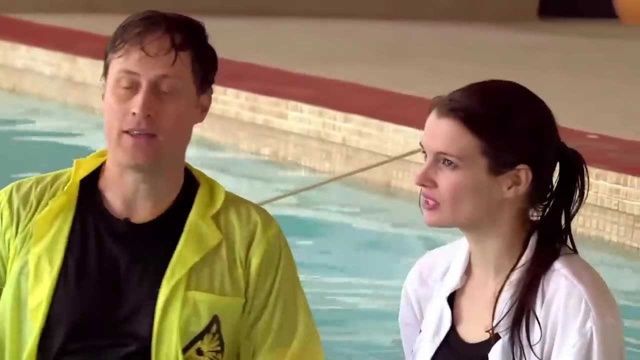 Yeah, that's really working. Whoa Careful. Oh, look out So good. It's good. It's not great, Not yet Right. How do we make it better? What do you think? Well, I was thinking. what if we try to reduce the friction? 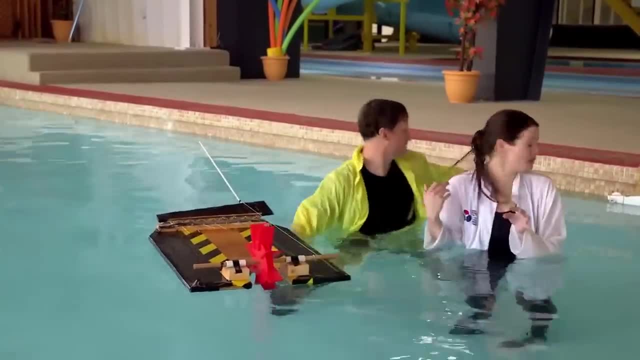 Remember that other boat we tried? Here it is, Oh yeah, The little one. you mean, Yeah, the little one. See, look at this one. It has the pontoon style. Do you see how we have it floating on these two surfaces? 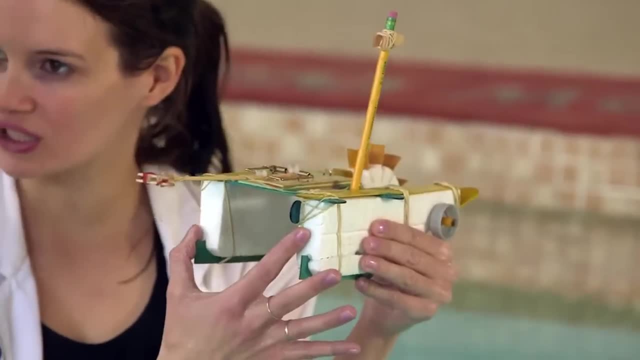 Yeah, So very little is actually touching the water, Oh, Whereas this one we have a giant haul that's going to drag the water and slow our boat down. So it's sort of like the difference between like pushing a whole bunch of water like that. 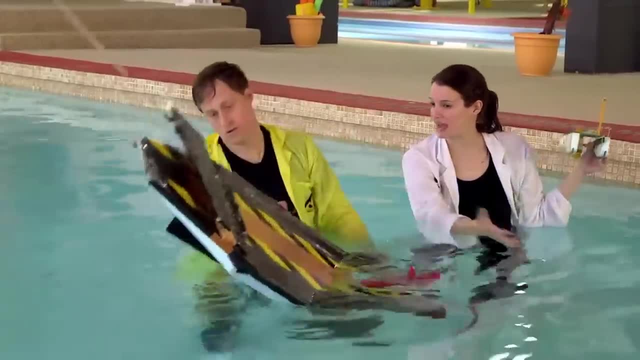 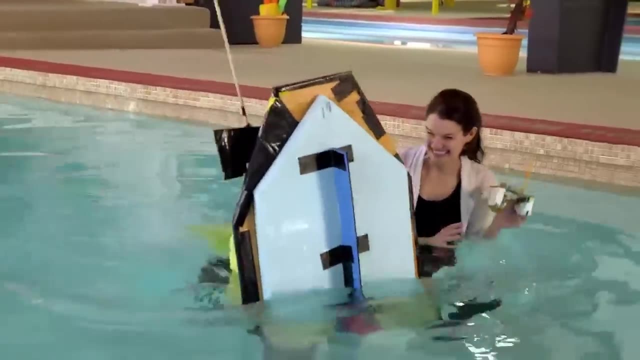 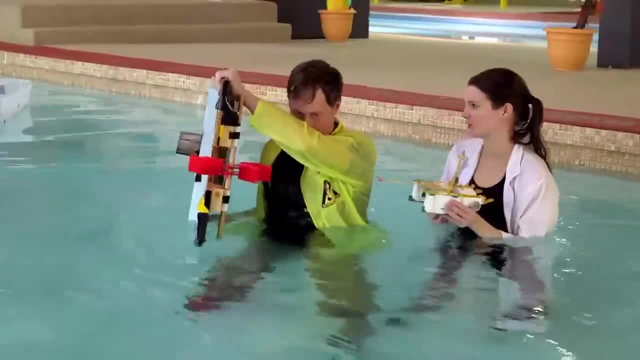 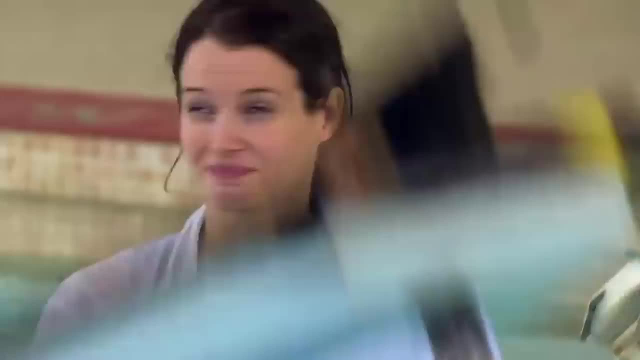 That's right. That's right. Yeah, We want very little resistance for our boat, So little resistance with a couple of things that just stick down like that. A lot of resistance when we have big, flat, big like that. So we completely rebuilt this boat. 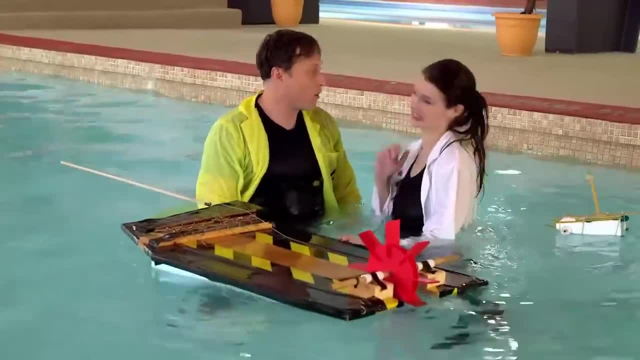 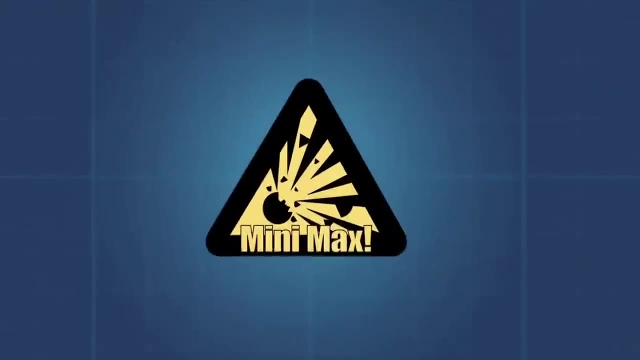 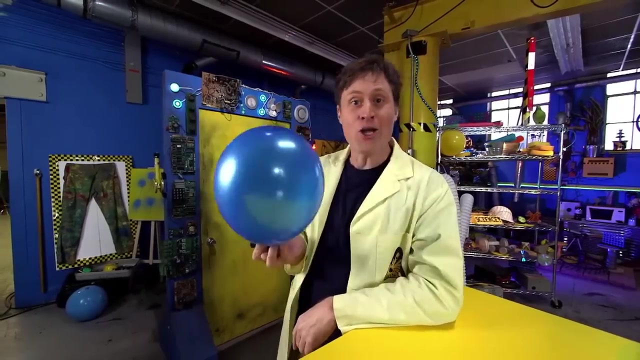 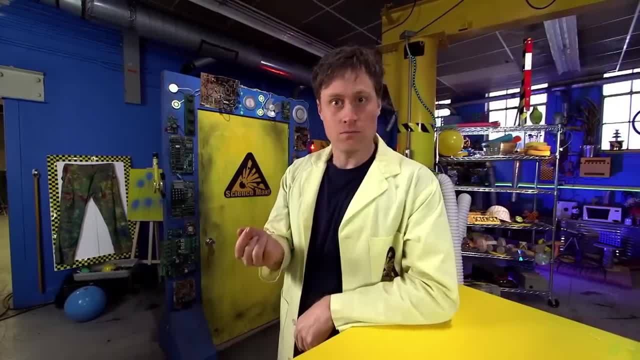 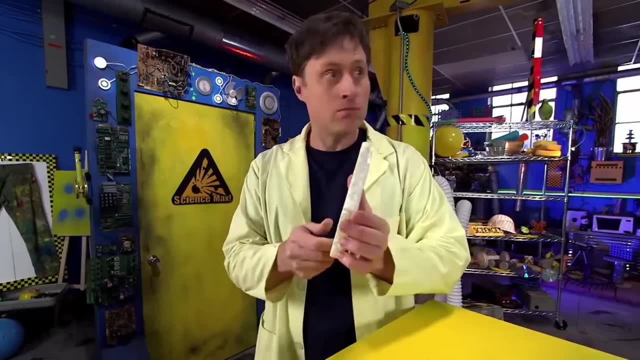 Yeah, And they're going to put this on the boat anyway using a balloon. Let's make a balloon powered boat. All you need for that is something to be your boat and a balloon. Then you attach them together. Actually, the best way to do it is use a straw and attach the balloon to the straw. 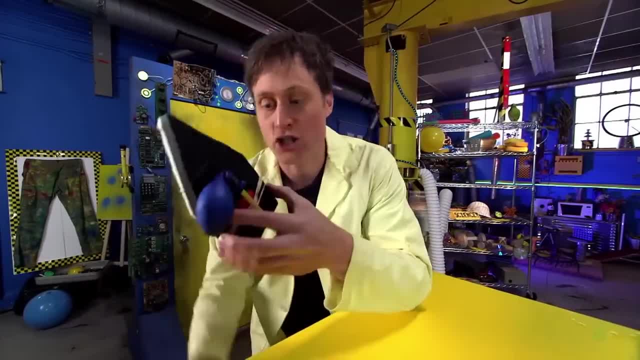 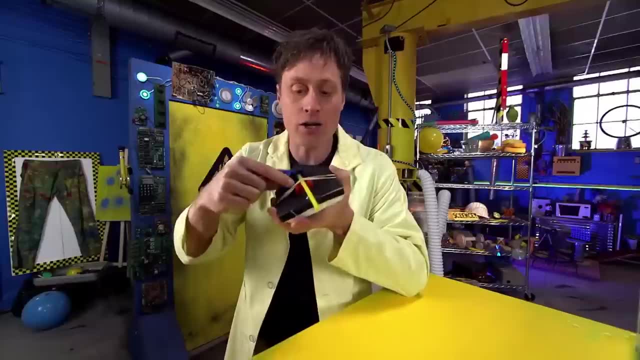 using an elastic band and then you attach it to your boat using more elastic bands, just like this. I've put a nice tape top on the boat to make it look awesome. I also put a little bit of a riser here using just anything plastic to keep the straw nice and straight. 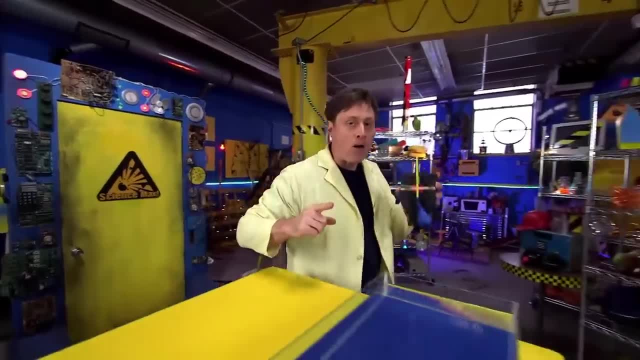 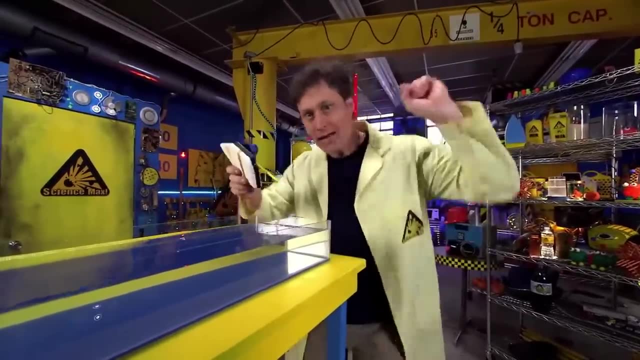 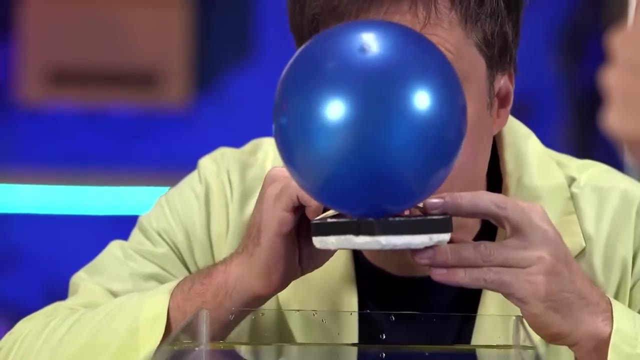 because the question is: will our balloon-powered boat work better if it's pushing in the air or if it's pushing in the water? Well, let's do a science experiment and find out. First version in the air: Oh, almost all the way. 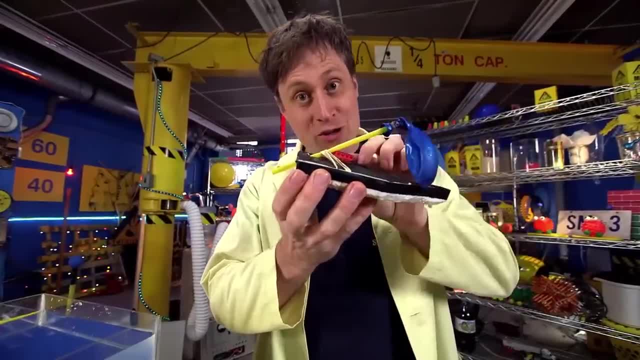 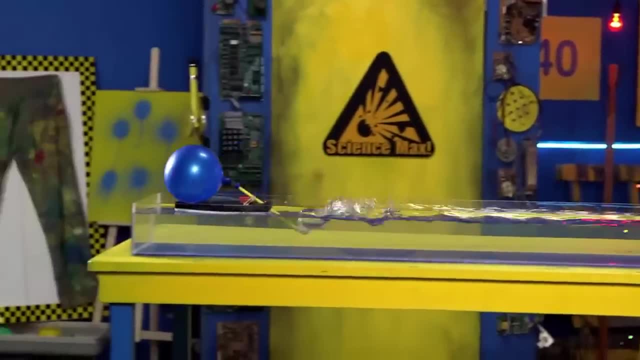 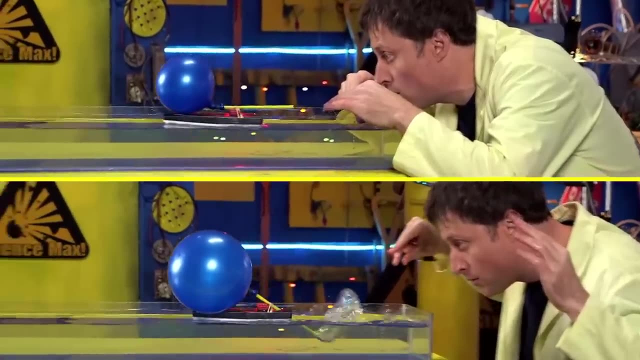 Now let's try it with the straw like this, so it pushes into the water. Whoa, It works so much better. Why? Because water is denser than air. The air coming out of the straw has to push against something to make the boat move. 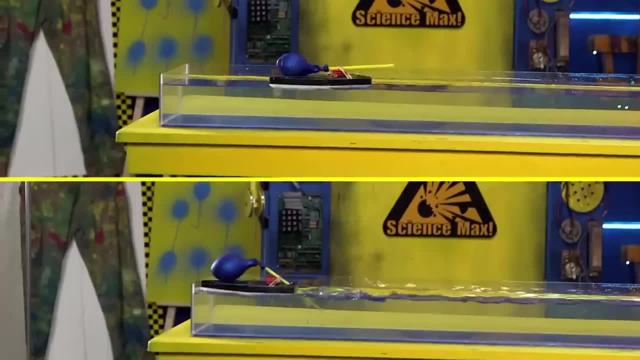 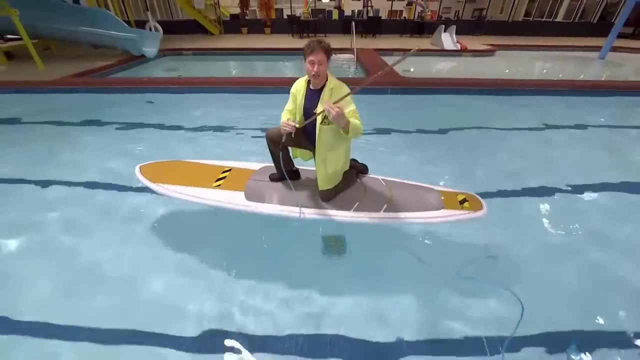 Water has more mass than air, so pushing against water has a better result. Now let's max it out. This is an air compressor. Well, actually That is the air compressor. You see, the engine here pushes air into this tank, which works sort of like the balloon. 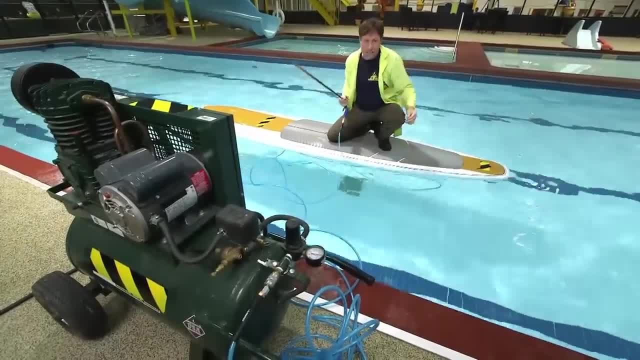 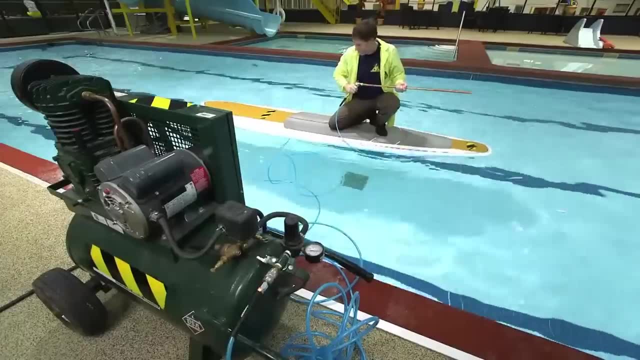 And then it goes out, this long hose which sort of works like a straw. So let's make a maxed-out air-powered boat Ready, Just like the small boat pushing against the air doesn't produce much thrust. Huh, Not so great. 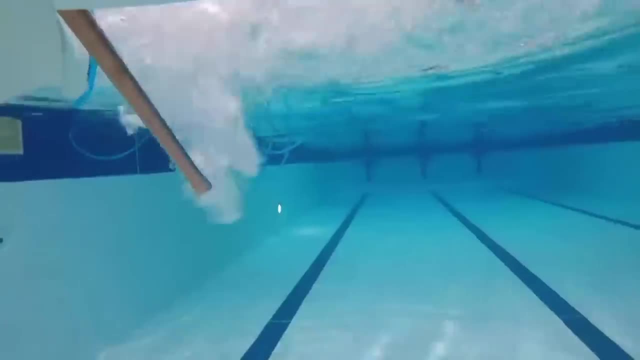 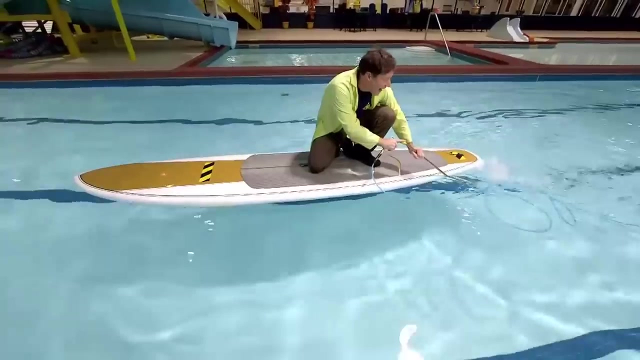 But now let's put it in the water. Pushing against the water gives me much more thrust, because water is more dense than air. Whoa Ha, ha, ha, ha ha. Maxed-out air-powered boat. Maxed-out air-powered boat. 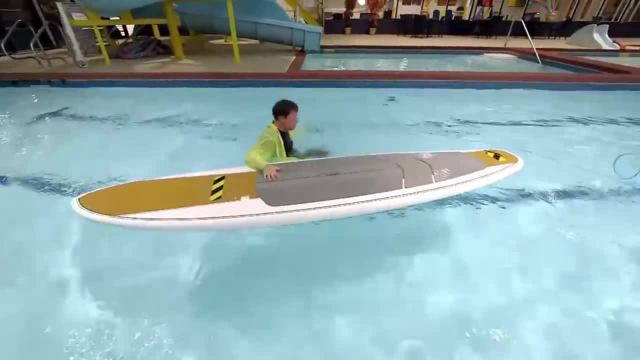 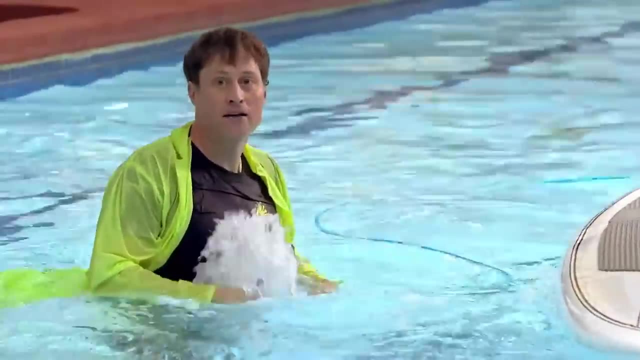 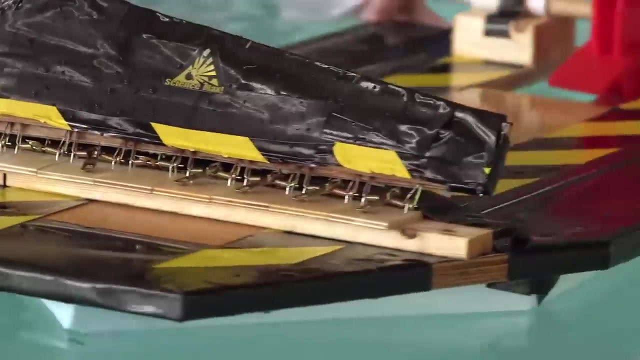 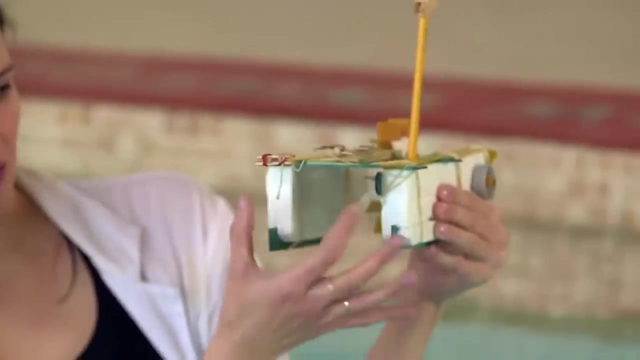 Yeah, Whoa, That's, That's not me. Michaela and I are maxing out the mousetrap boat. Ten mousetraps didn't seem to make our boat go very fast, But moving the string down our lever arm helped, and now we want to redesign the hull so it has less friction with the water. 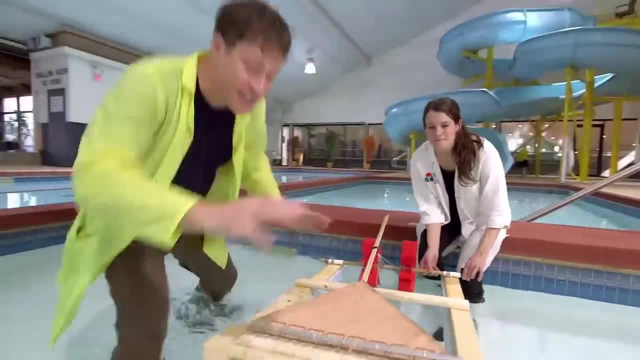 Check it out. This is the ultimate mousetrap boat. We've got ten mousetraps here. We've got our long arm, We have it attached at the right point of the lever, we think. And then we've got two, two paddle wheels at the back and pontoon. 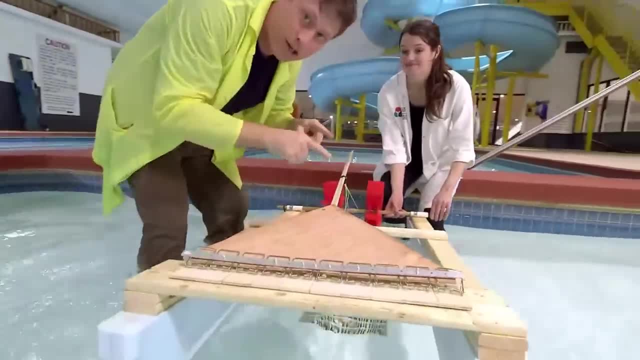 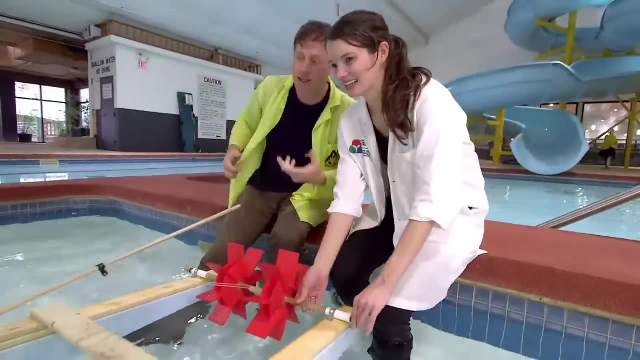 Yes, Yeah. So what do you think, Michaela? I think this thing is set, It's going to be awesome. Yep, Okay, Ready, Ready, Let's test it. Oh, it's working, It's working Hey. 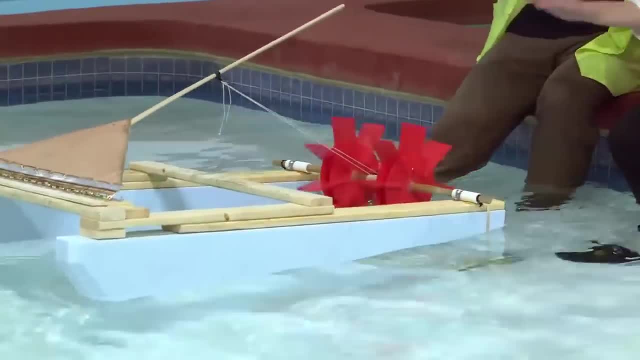 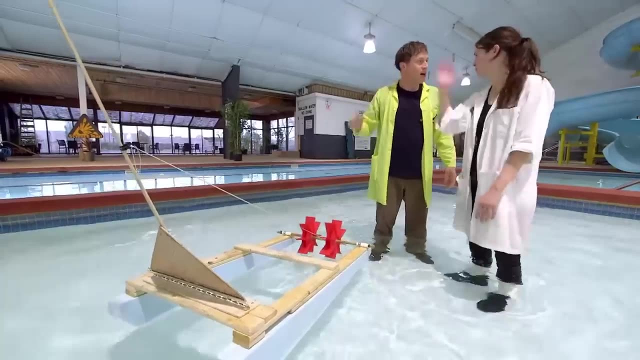 It's picking up speed. Yes, Wow, Whoa Mousetrap boat. I mean it's good. It's good. It's not science, Max, It's good. Yeah, We were hoping it would go faster, Faster, or 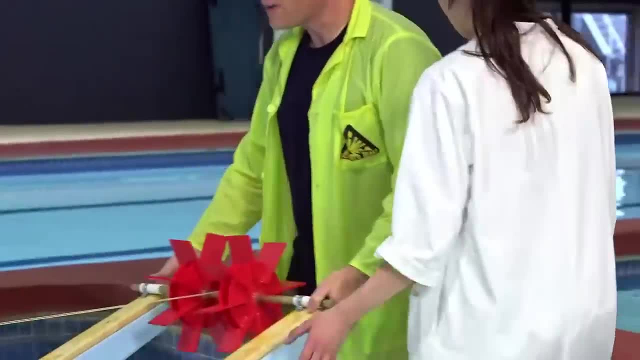 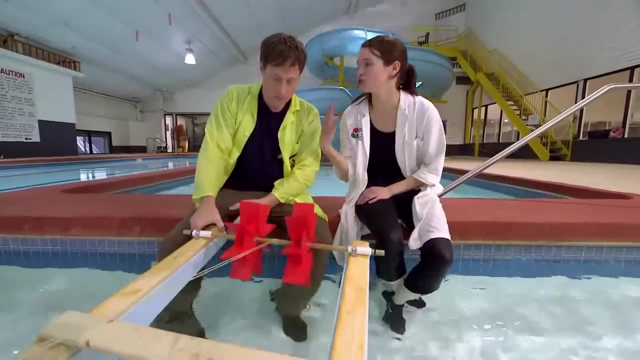 No, Pretty much, just faster, Yeah, Okay, Obviously we need to store more energy that will make the paddle wheels go faster, right, Yeah, So we just have to think about it, right, Like what's stronger than a mousetrap? 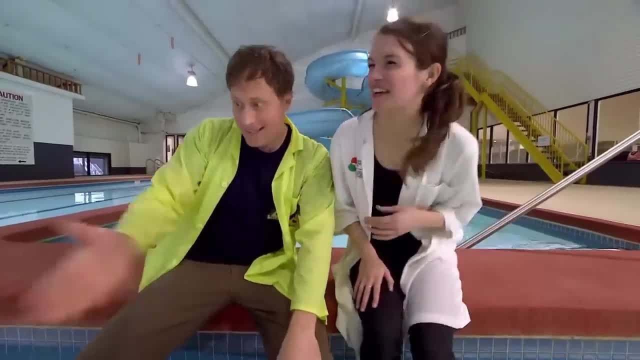 Well, ten mousetraps. That's why we have ten mousetraps, Michaela. Okay, What's stronger than ten mousetraps? Eleven mousetraps? Look, If we just keep going, Okay, Enough with the mousetraps. 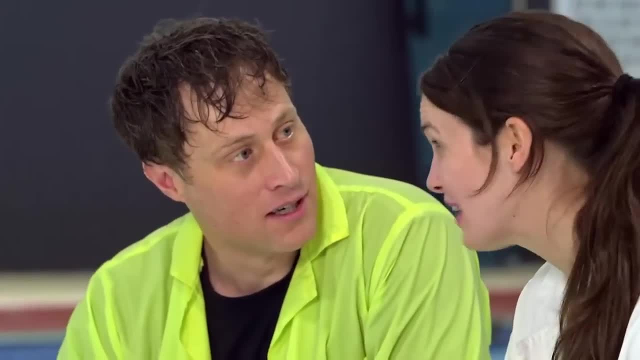 It's going to get super wide. We have a thousand mousetraps wide. Enough with the mousetraps. Have you ever seen like a rat trap? No, It's huge. Well, hold on, I can just get one from the portal. 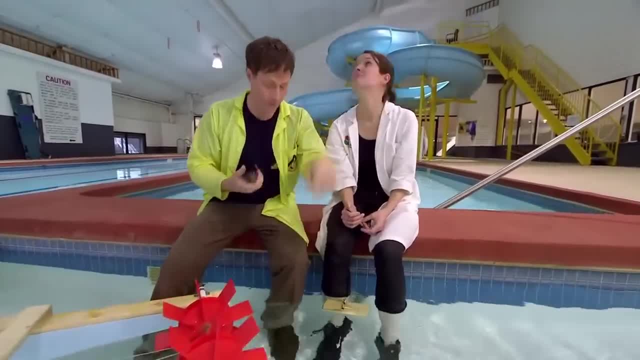 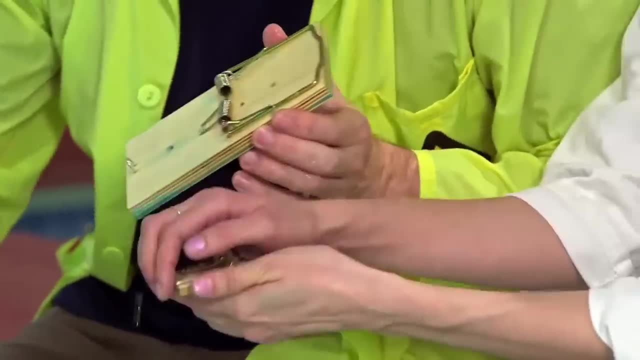 One rat trap coming up. Oh, Okay, Came from All, right, Well, that's fine. And Whoa, Wow, Look at that. Yeah, That is a lot bigger. Okay, So snap yours. All right, Ready. 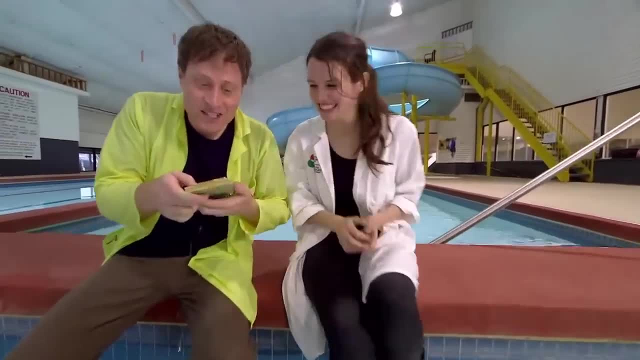 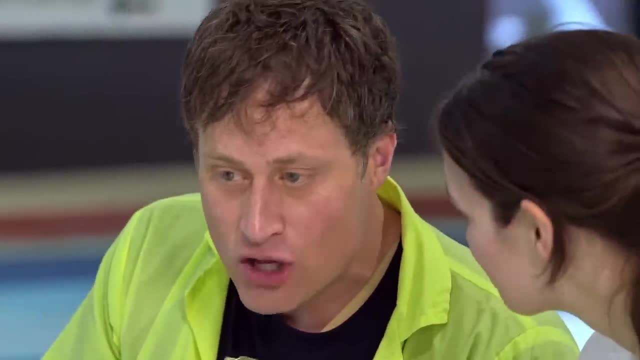 Mousetrap, Okay, Okay, That's terrifying. So that's a lot more power, Yeah, A lot of force. So tell you what? We have a little mousetrap boat. It's a single single rat trap-powered boat and we'll race them and we'll just see the. 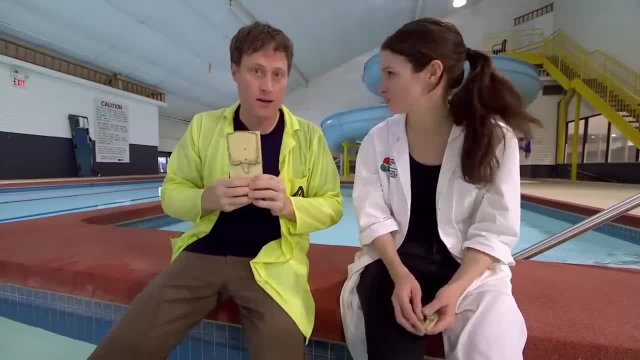 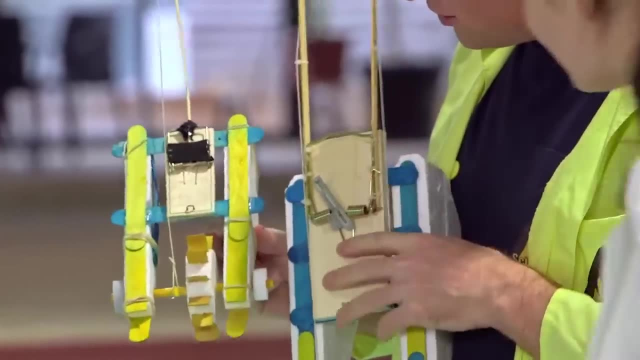 difference in power from one rat trap to one mousetrap. I like that. We'll do a prototype before we make a big one. Yeah, Okay, Come on, Let's go. So we built a rat trap boat to race the mousetrap boat, and then Mikayla and I got a little. 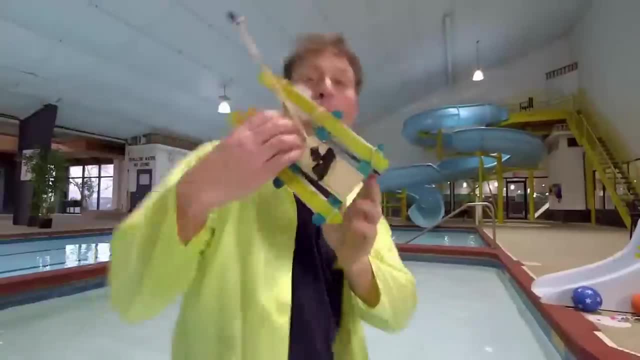 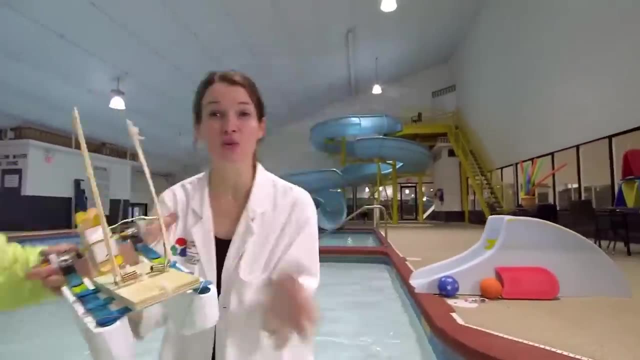 competitive. Check out the rat trap boat. No, Check out the mousetrap boat. Mousetrap boat is better because, Yeah, Rat trap boat is better. It's got bigger springs, more potential energy stored in there And mousetrap boat has less potential energy. 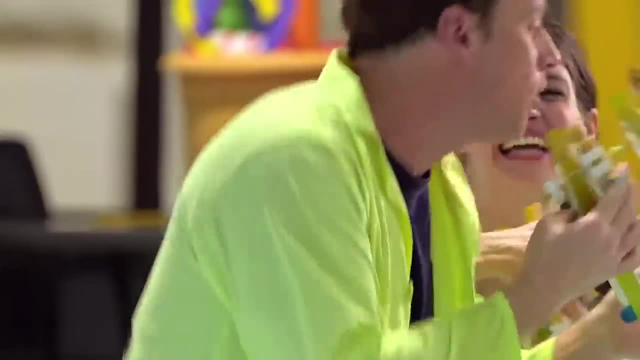 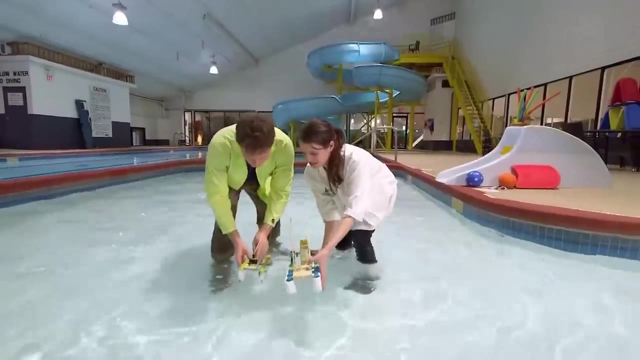 and less springs, but it's got more heart and he really wants to win. Okay, Yeah, Tell you what. Phil Loser jumps in the pool. What? Oh, Okay, Sure, Let's do it. Okay, Ready. 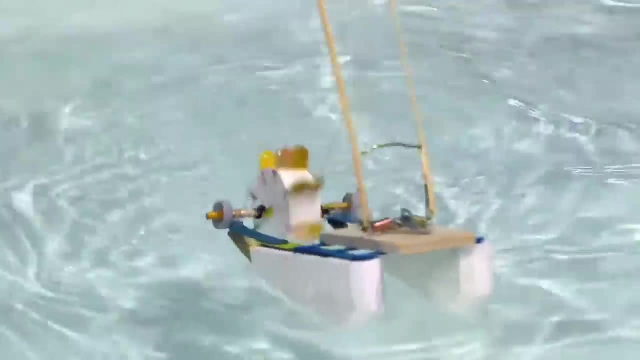 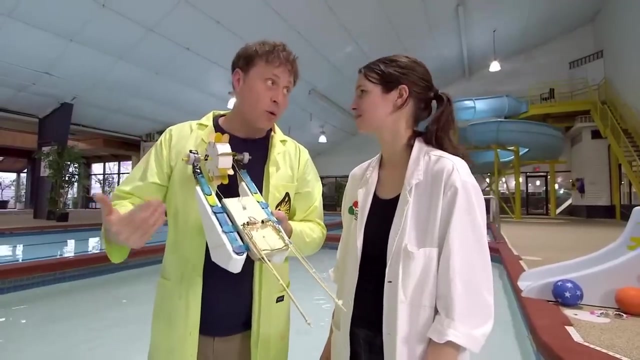 Go. So, as you may have guessed, the rat trap boat has a lot more potential energy that can be stored in the spring. Okay, So rat trap boat is clearly better than the mousetrap boat. We make the boat the same way, but we use rat traps instead of mousetraps. 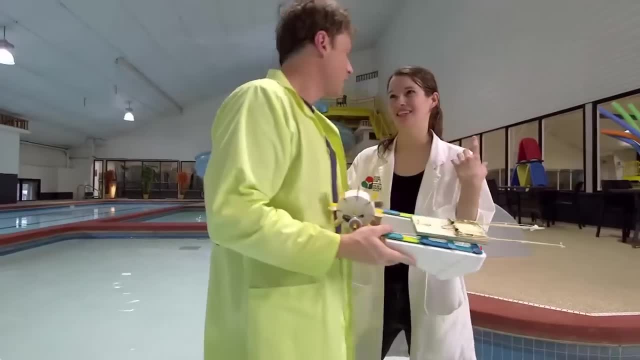 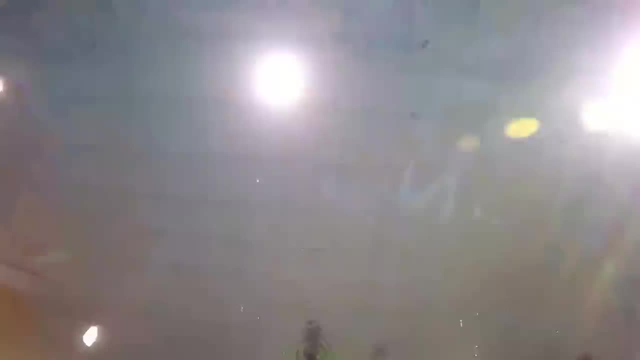 What do you say? Love it? Okay, Wait, a second Phil. What? Ferris, Ferris, You've got to jump in the pool. Okay, Fine, Here you go. Hold this Inertia. What is it? 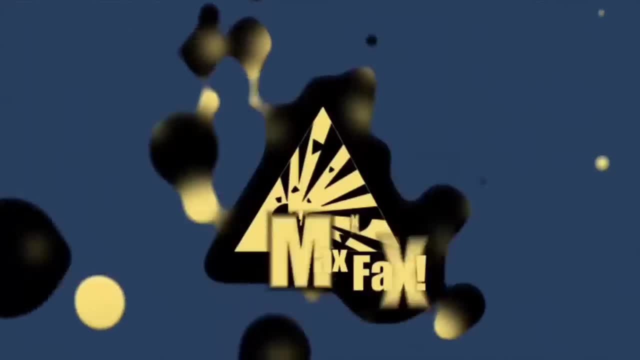 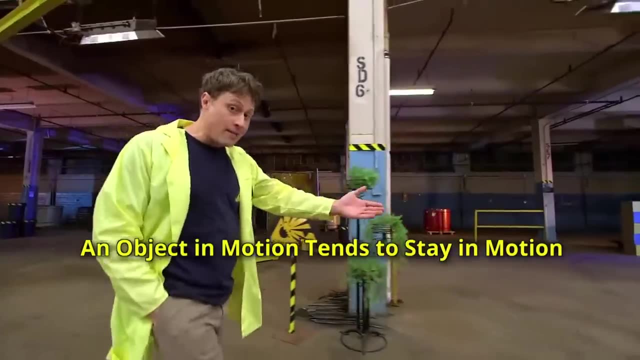 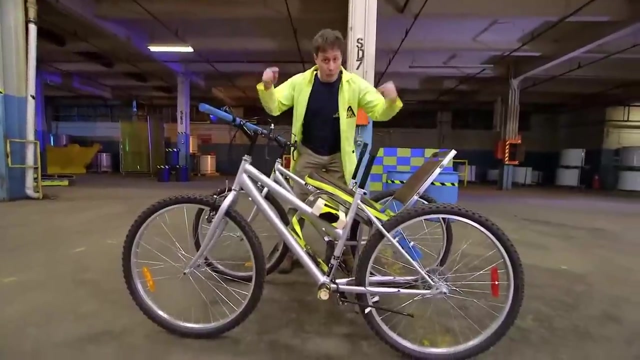 Well, it's directly related to Newton's first law of motion. An object in motion tends to stay in motion. An object at rest tends to stay at rest. Let's do an experiment. Here is an object Right now. it's at rest. 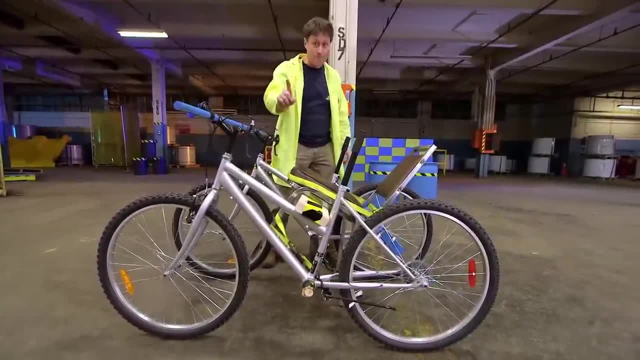 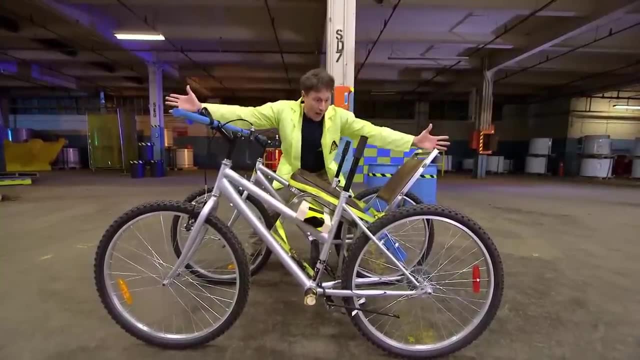 You might think that means it has no inertia, but that's not true. Inertia just means an object's tendency to keep doing what it is doing. Right now it's doing nothing, But if I wanted to overcome its inertia I would have to put energy in. 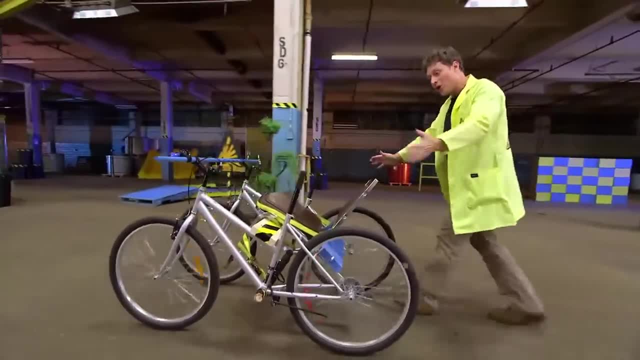 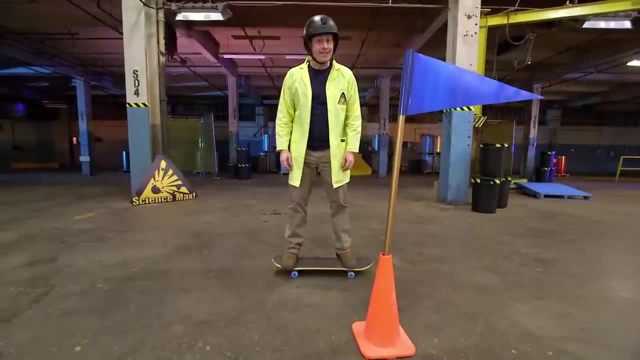 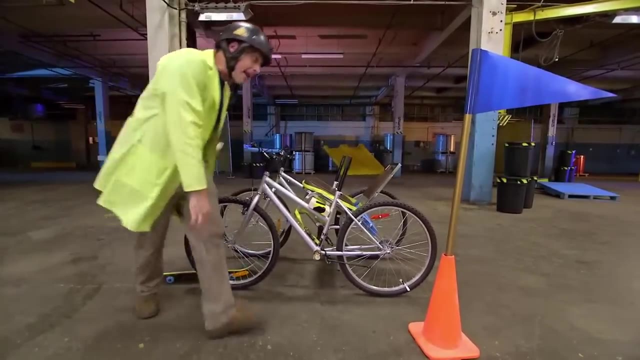 And now that I have it is moving on its own, It has inertia. If I wanted to stop it, I would have to overcome its inertia, its tendency to keep moving. Okay, There, I went exactly that far. Now let's max it out. 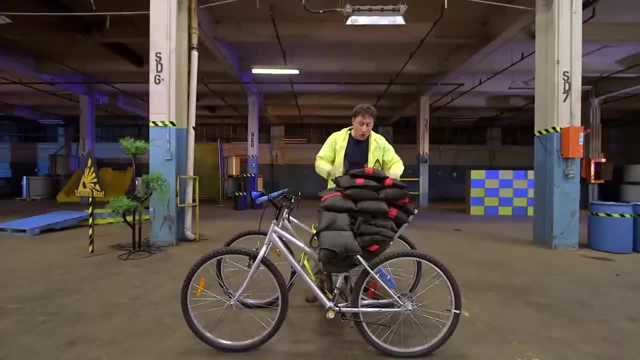 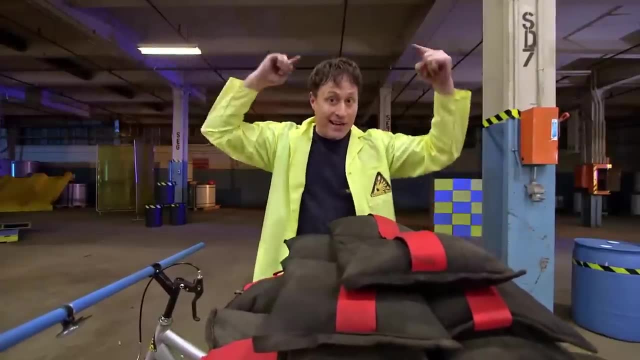 I'm adding these weights to the cart. Now it has a lot more mass, which means it has a lot more inertia and its tendency to do nothing. But this time it has a lot more inertia. If I wanted to get it going the same speed as before, I'd have to put in energy. 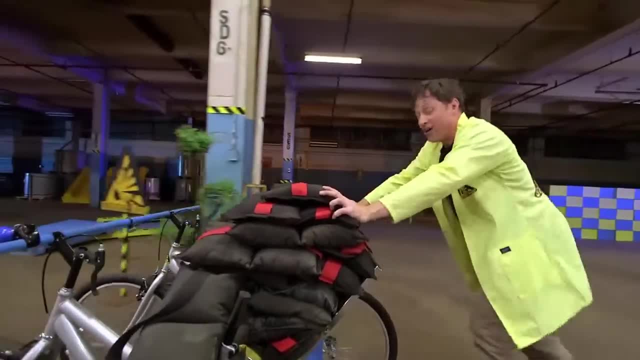 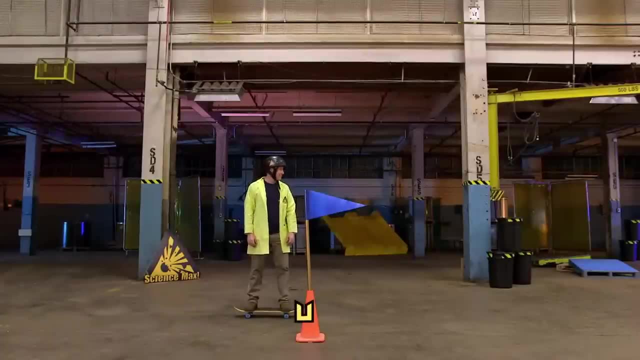 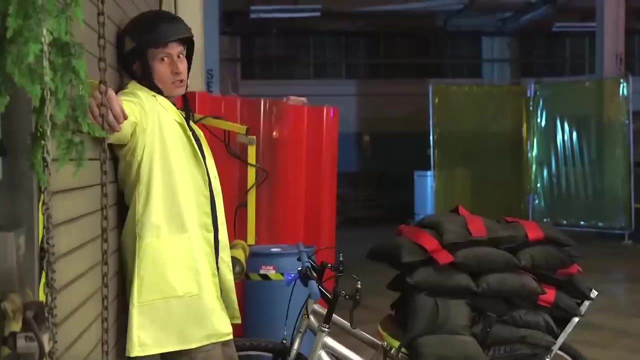 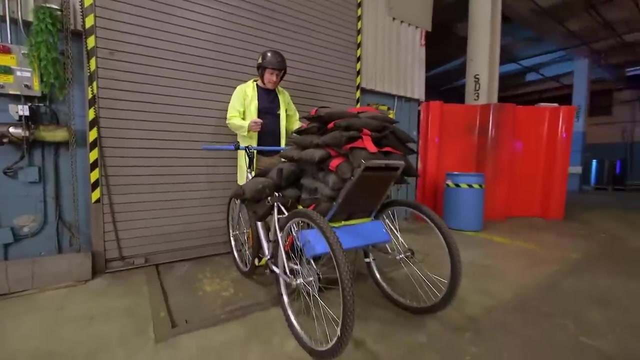 I'd have to put in a lot more effort There. Now it's going the same speed as before, but now it has way more inertia, so stopping it will be harder. So there you go. Inertia: A thing's tendency to stay moving or stay still, and the more mass, the more inertia. 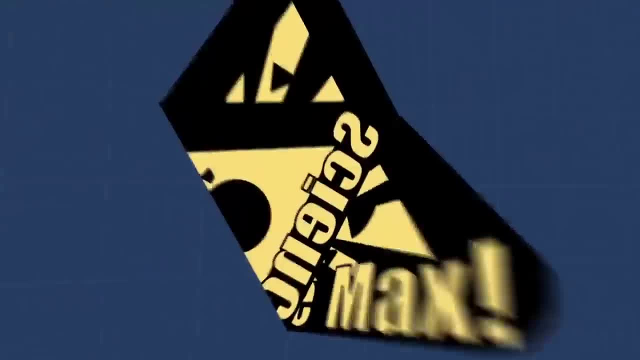 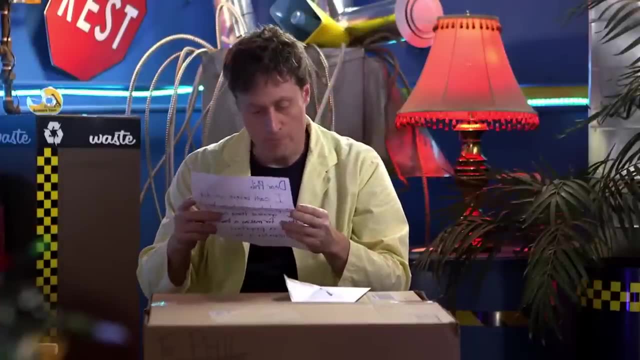 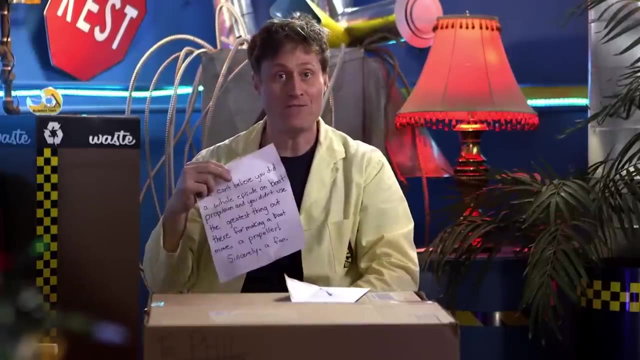 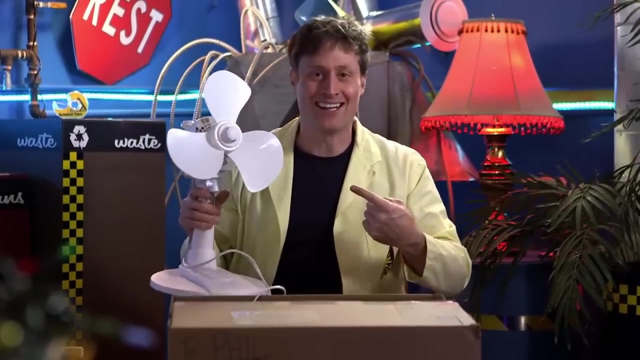 Oh, Oh, Oh, Oh, Oh, Oh Oh. One, two, three Minimax. Dear Phil, I can't believe you did a whole episode on boat propulsion and you didn't use the greatest thing out there for making a boat move: a propeller. 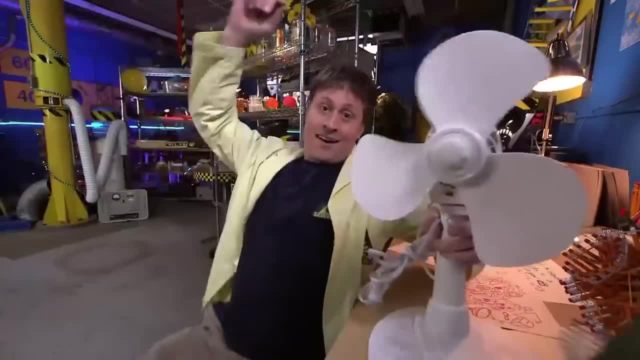 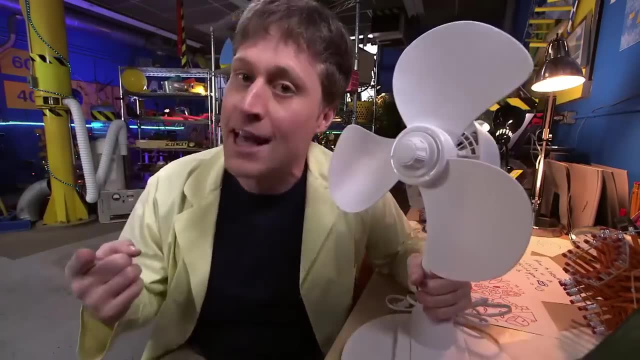 Sincerely a fan. Well, Let's talk about propellers. Oh, A fan pushes air, just like a boat propeller pushes water. They're both fluids and they behave in the same way. Now, if you look closely at a fan, 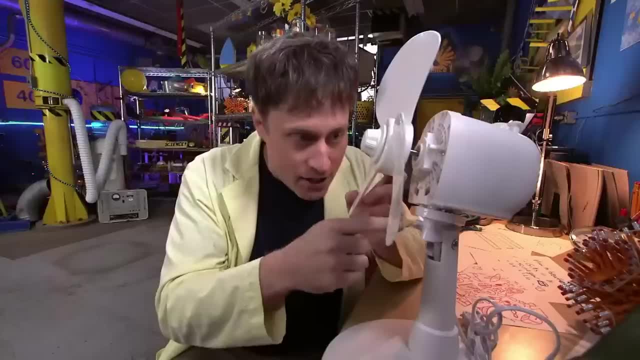 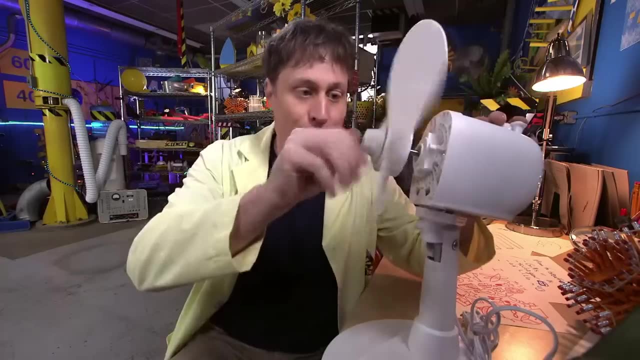 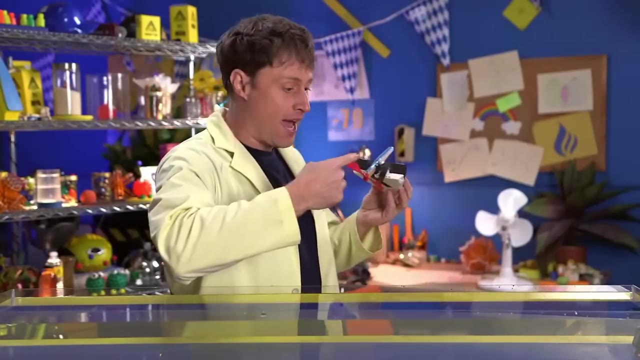 it's curved on the blades, The air or water is caught under at this side, and then it's pushed out on the curve to make it go that way, And the faster it spins, the better it works. Now this is a propeller powered boat. 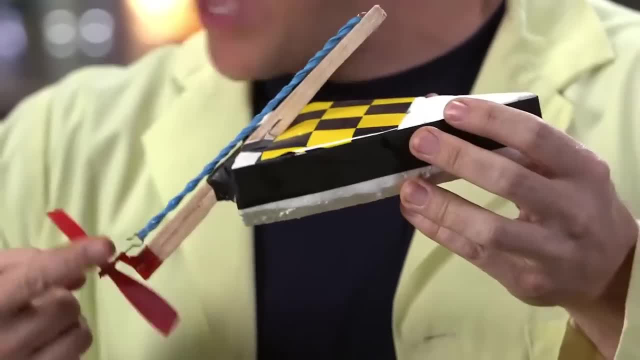 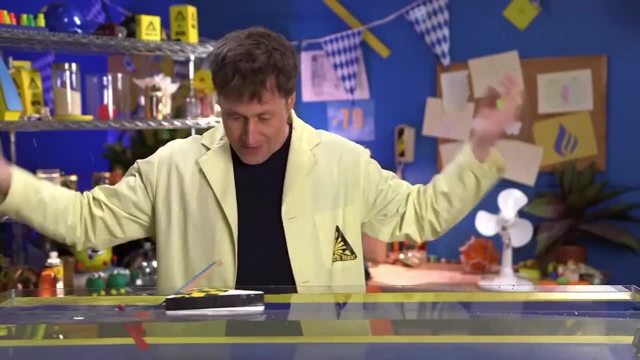 And what you do is wind up the propeller. I have an elastic band here to store the amount of energy I put in, And then you put it in the water. The propeller spins and the boat goes forwards. It's being propelled by the propeller. 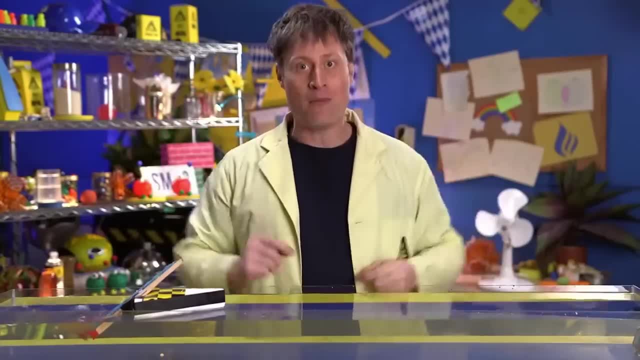 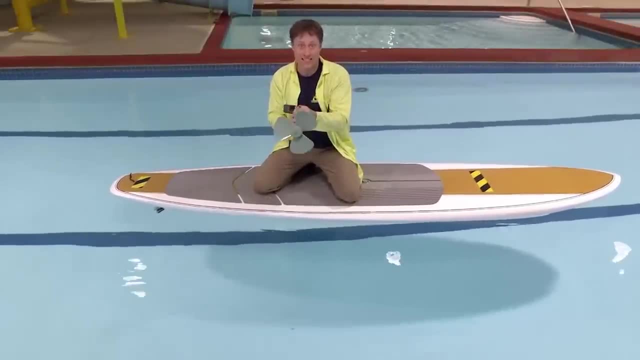 That's why you call it that Awesome right? Well, now we'll max it out. This is a drill, It spins And this is a propeller, And when you put it in the water and spin it, it provides thrust. 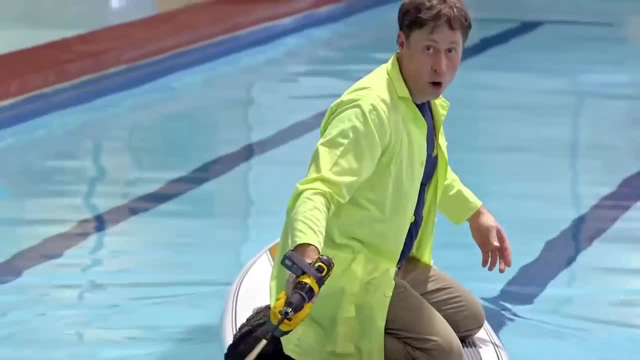 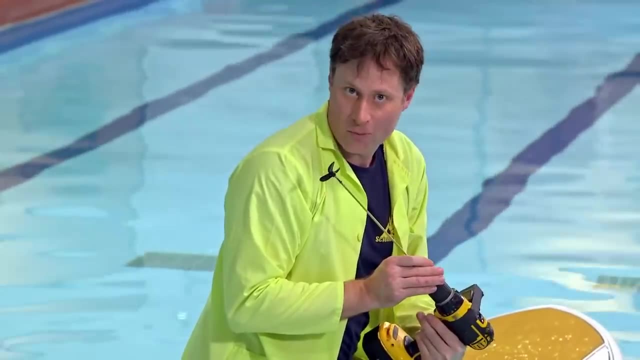 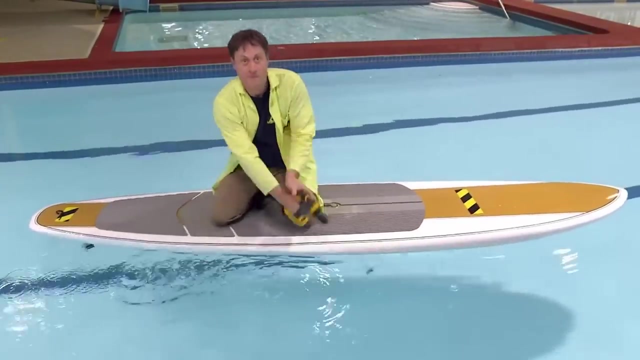 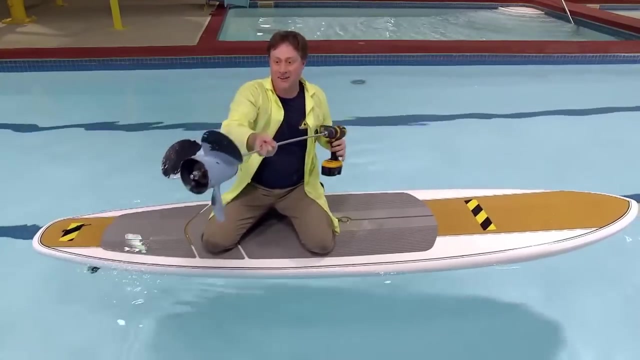 So let's try it out. Whoa, Remember not to try this at home. I am a trained professional. This is a very small propeller. Let's compare This: this is a super maxed out propeller, Whoa. 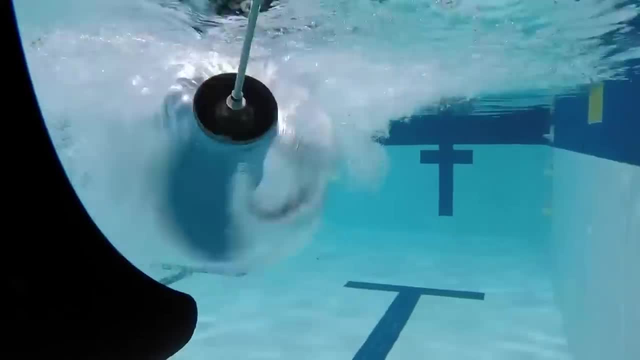 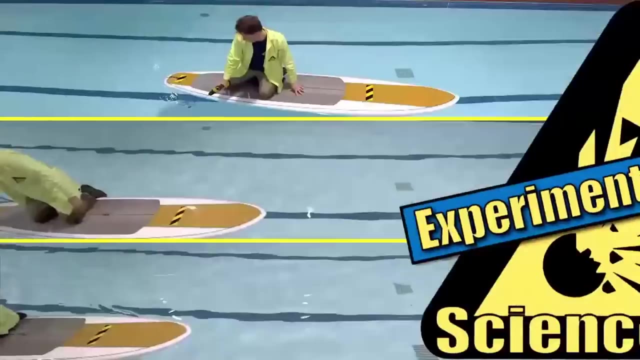 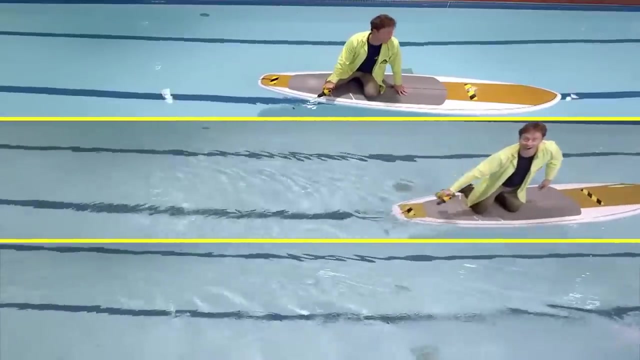 OK, let's try it out. Yeah, Whoa, Whoa. The larger a propeller is, the more energy you need to turn it And the more propulsion you get out. Mikaela and I are maxing out the mousetrap boat. 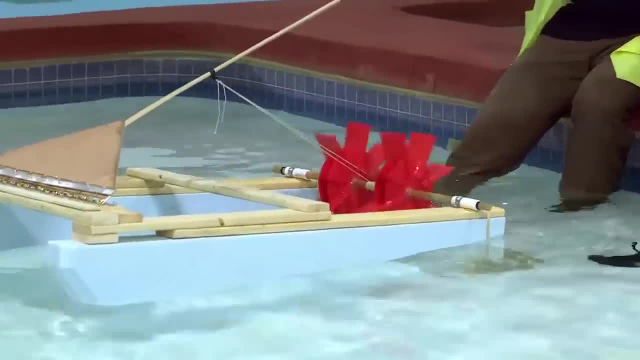 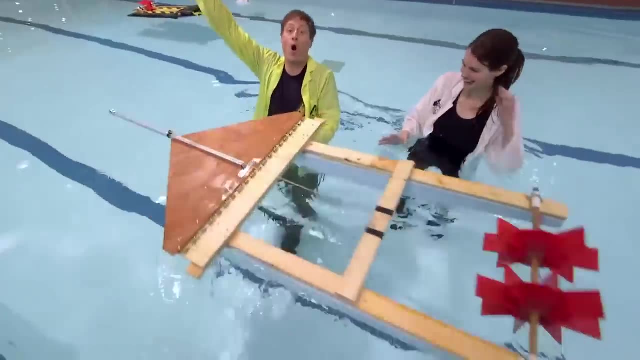 Well, actually we can't call it a mousetrap boat anymore, because now we're using rat traps. The design is the same as our 10 mousetrap boat. Rat trap boat, Rat trap boat, Rat trap boat. It's the super mousetrap boat. 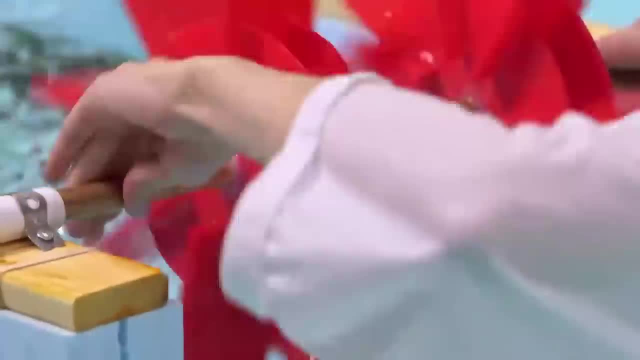 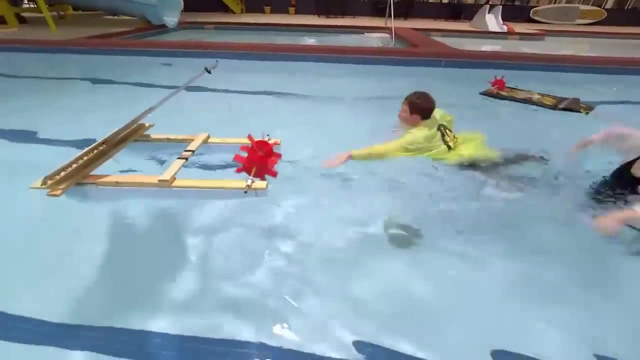 It's the best mousetrap boat ever. We wind it up and try it out. OK, ready Go. It worked great. The reason is because this boat was storing a lot more energy in the spring tension. More energy means more propulsion. 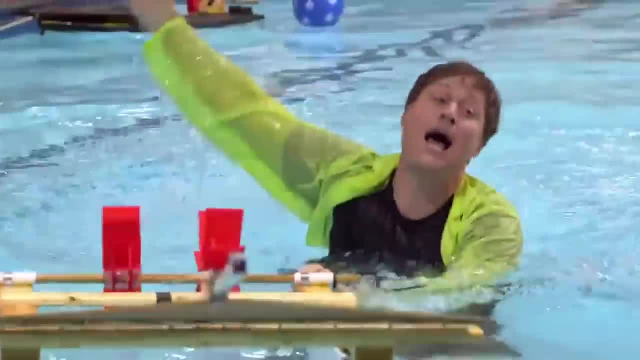 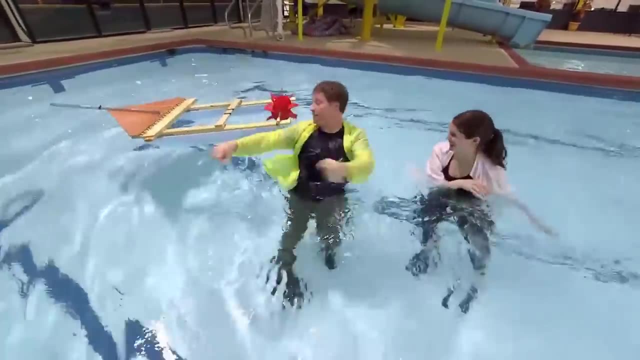 So much we couldn't even catch it. Yeah, That was awesome Rat trap boat. What the Science facts? Experiments at large: Rat trap boat, High five. Let's do it again. Let's do it again, OK. 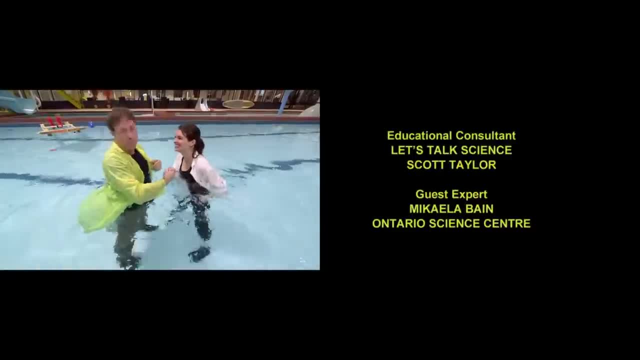 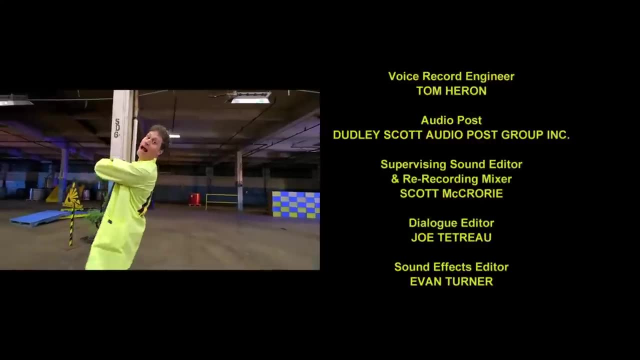 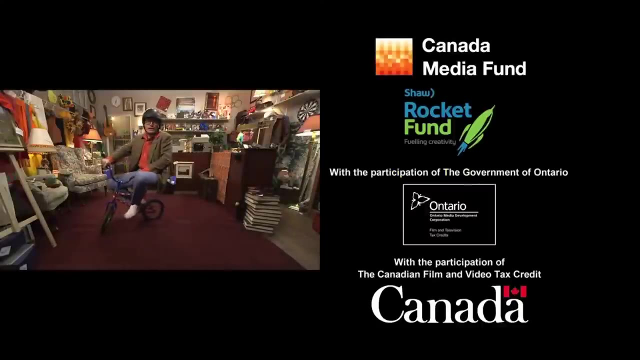 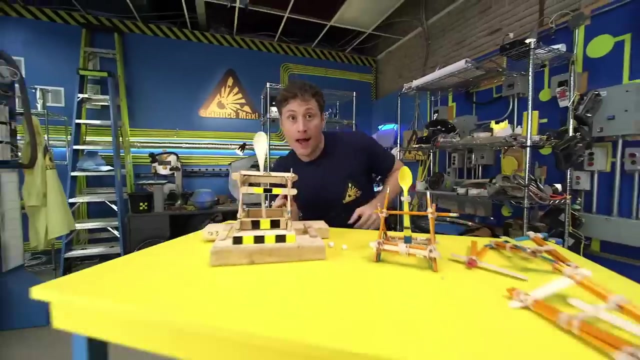 And one, two, three. Oh no, Stand by for a Relayed and directly Now. this, Oh a constant thrust. Have you ever done a science experiment and wondered what it'd be like if you did it big? I have. 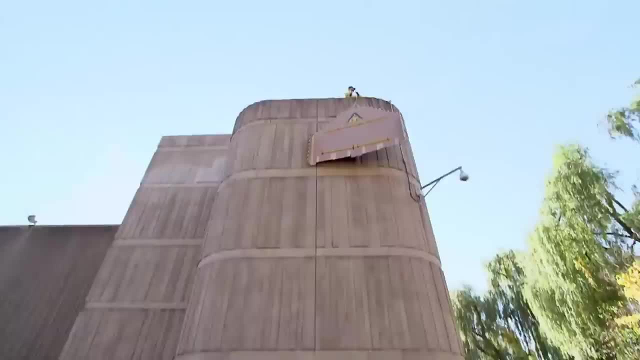 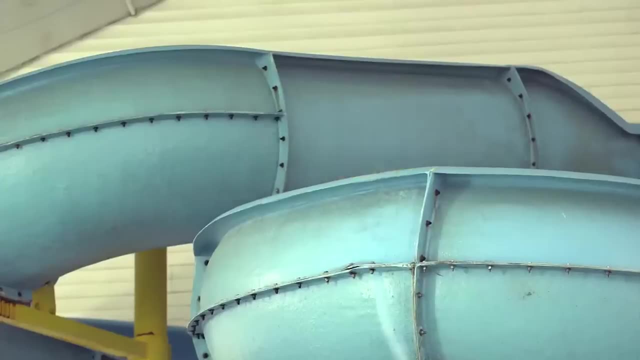 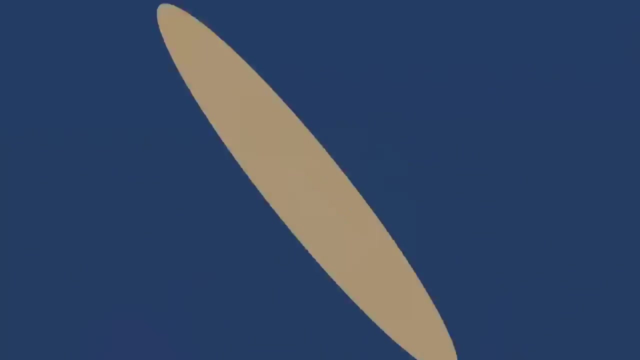 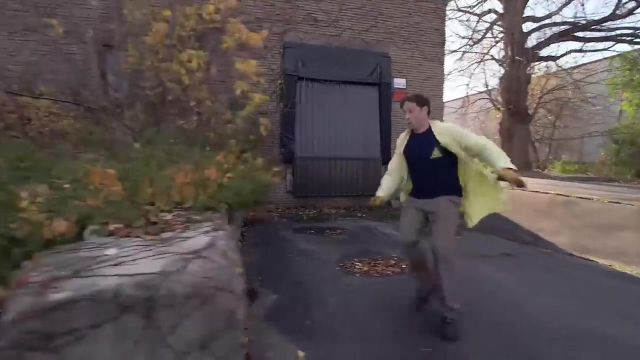 Yeah, My name is Phil and I take your everyday science experiments and do them big. This is Science Facts: Experiments at Large, Science Facts, Science Facts. What good is science if you can't use it to give you super strength? 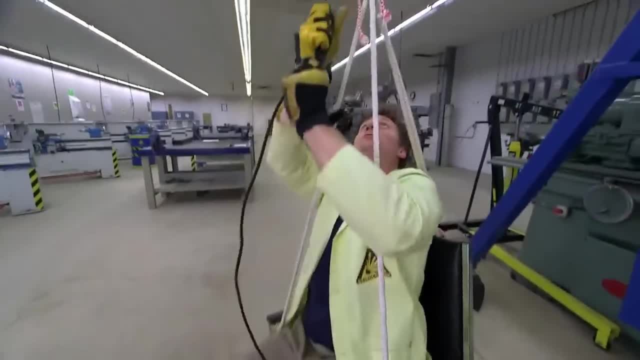 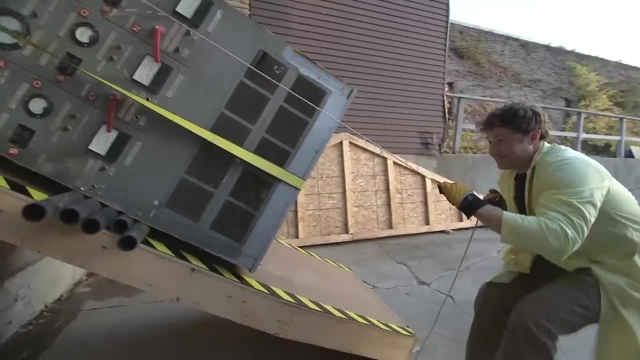 Well, I try to do just that on this episode of Science Facts: Lifting more, rolling more and a whole lot of running. What, What Simple Machines Today on Science Facts: Experiments at Large, Huh, Hm. 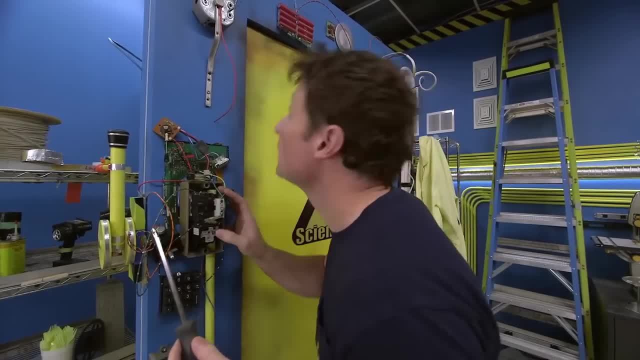 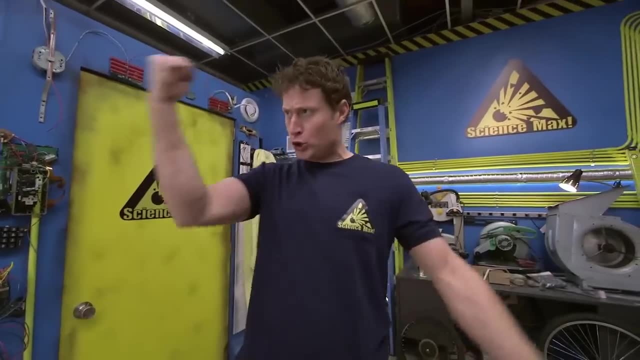 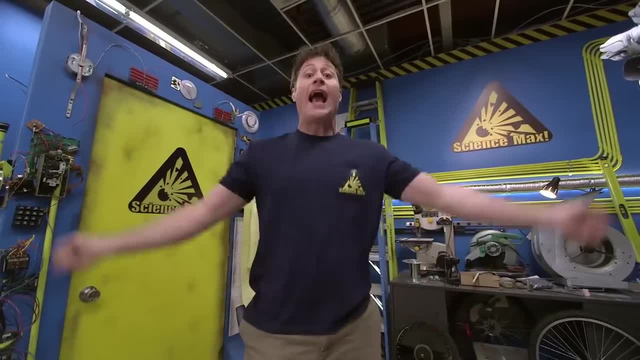 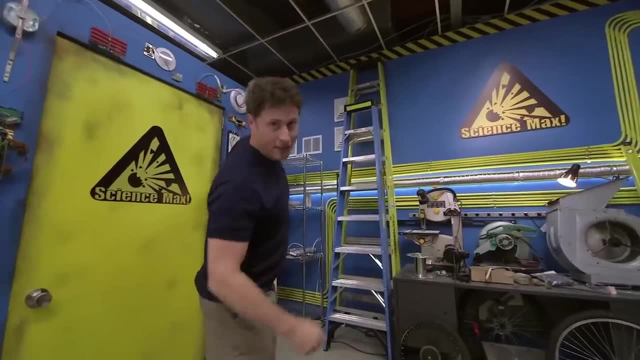 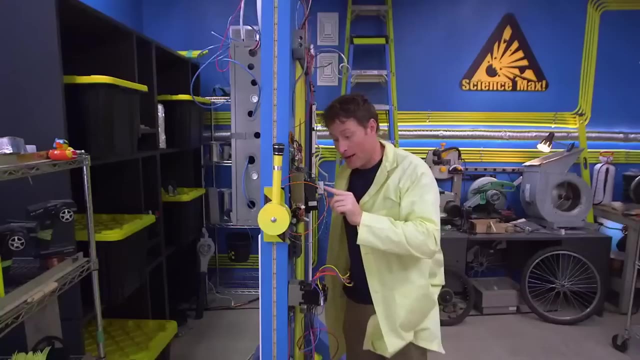 Well, today, on Science Facts, Experiments at Large, I'm gonna give you and myself super strength using the power of science. But we're going to do things a little differently today, You see. well, the portal hasn't been working perfectly since, well, since I built it. but 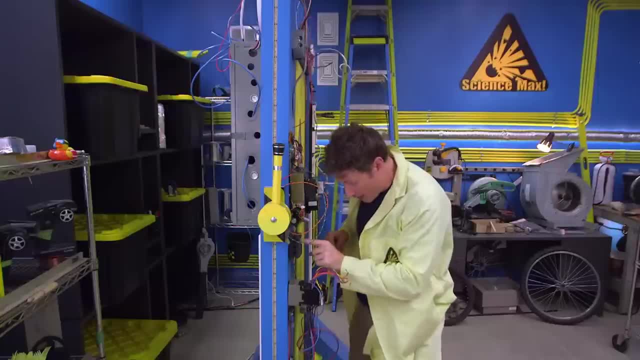 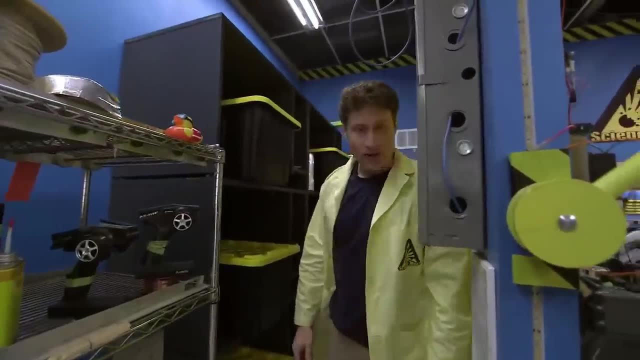 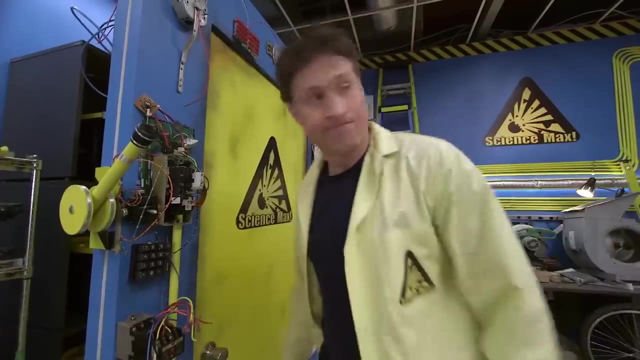 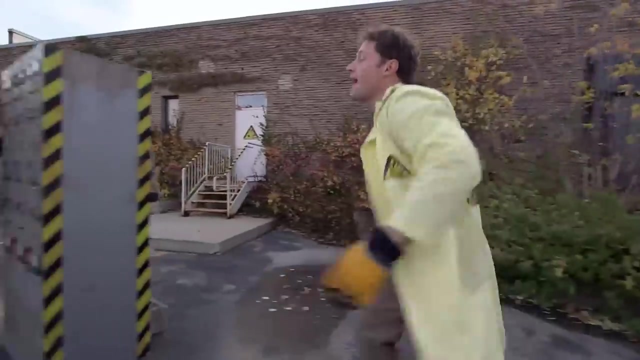 I ordered a new particle impulse controller and all I have to do is get it back to the lab. Perfect timing. it looks like the portal. the portal is broken. Um, okay, well, no problem. Okay, okay, I'm here. I'm here, wow. 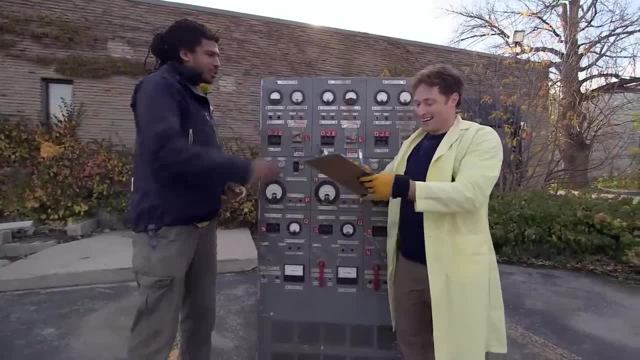 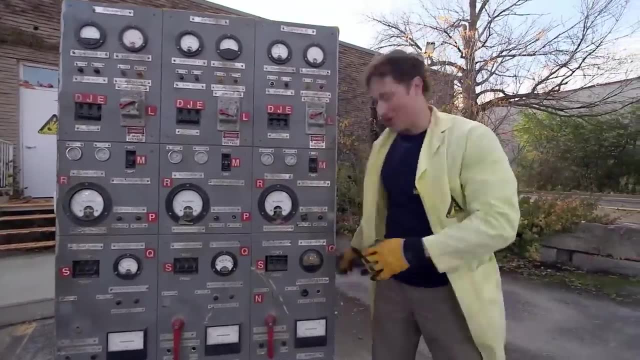 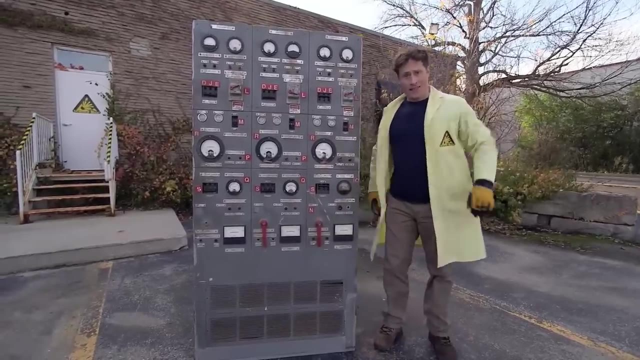 That's perfect: one particle impulse controller for you, Alright, thanks very much, No problem, Appreciate it, Enjoy. Well, my very own particle impulse controller. okay, That's as heavy as I thought I was going to be. Alright, Science Maximites. this episode of Science, Max Experiments at Large- is going to be a little different. 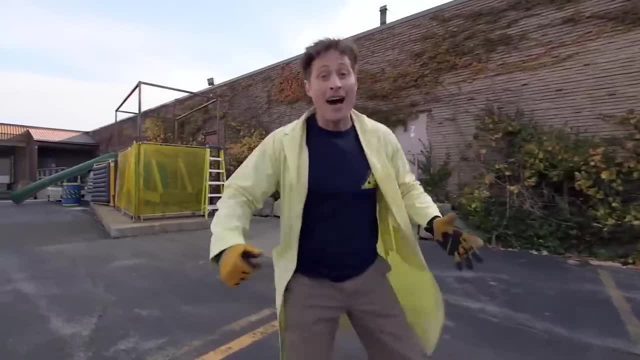 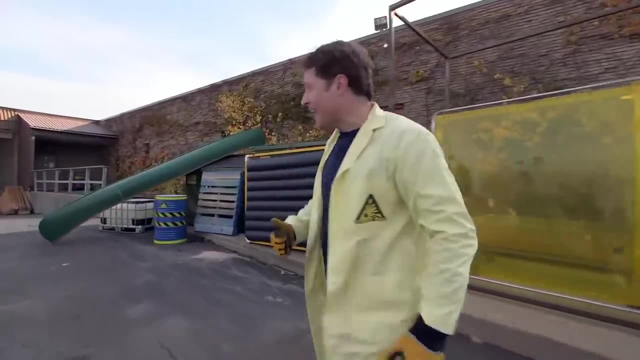 Because today I'm not going to have an expert come and help me, Because I'm going to move that giant heavy particle impulse controller all the way across the parking lot and all the way up that loading ramp by myself, With nobody's help. 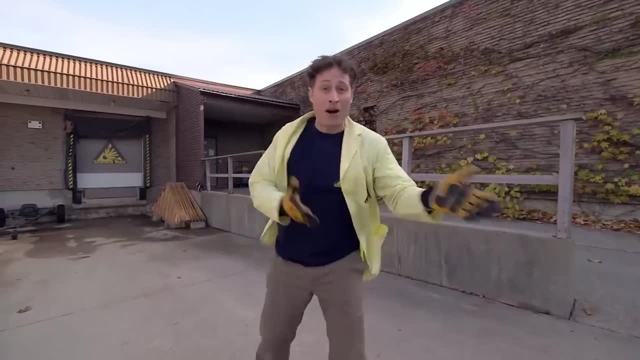 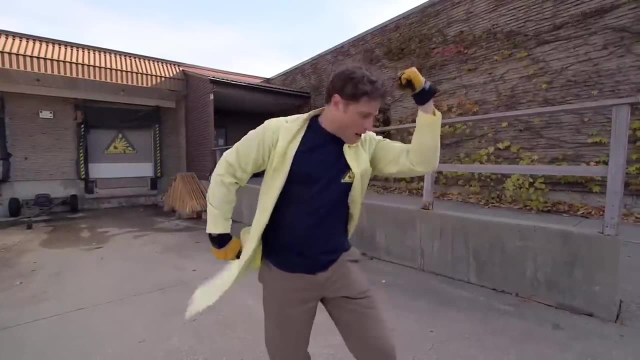 How am I going to move a giant heavy machine all that way if I can barely even budget? Well, I'm going to give myself super powers, super strength, with the power of simple machines, And the first machine we're going to start with is the lever. 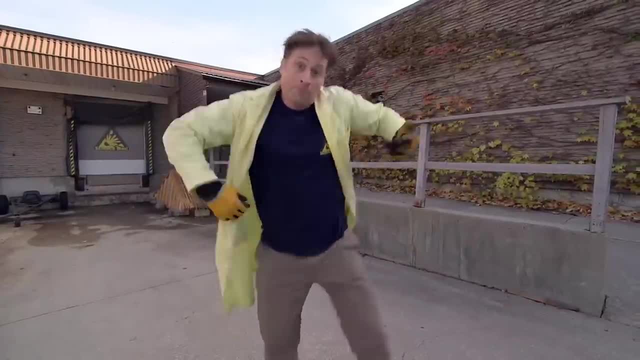 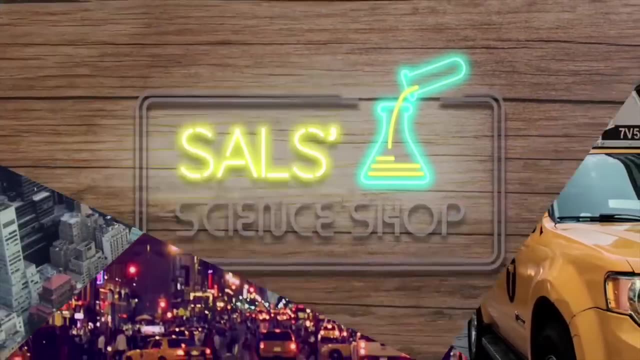 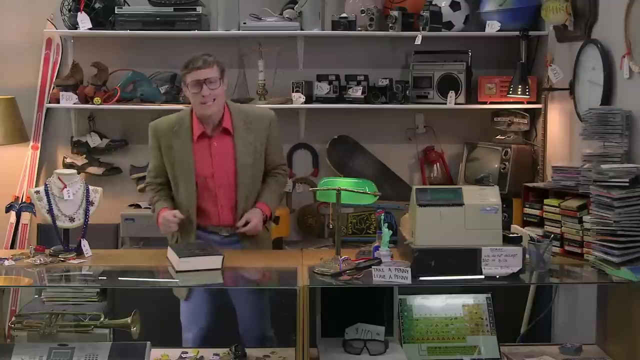 Which I guess I should go back to the lab to tell you about. Alright, Sal, I'll see you next time. Oh hey, how you doing? Let me guess you got some work to do when you need it done. easy, right. 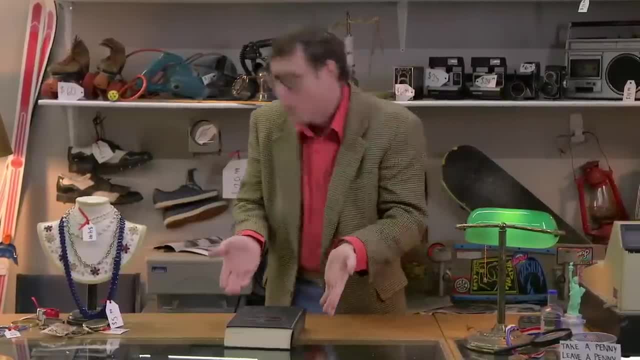 I mean, look at this book. I mean you could pick it up. but what are you going to be some sort of book picker-upper person now? Is that all you're going to do? Is that going to be your life, just picking up books left, right and center? 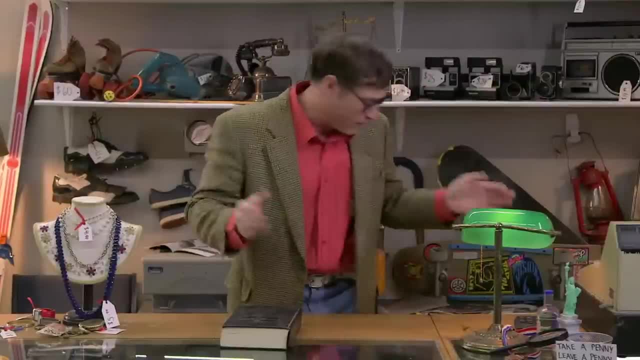 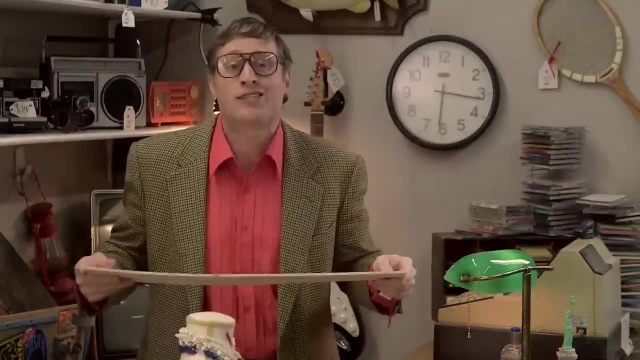 No, you're smarter than that. You know what you need: A lever Like this. Now, I know what you're thinking. I know You're thinking: hey, this is just a plank. You're right, That's because you're smart. 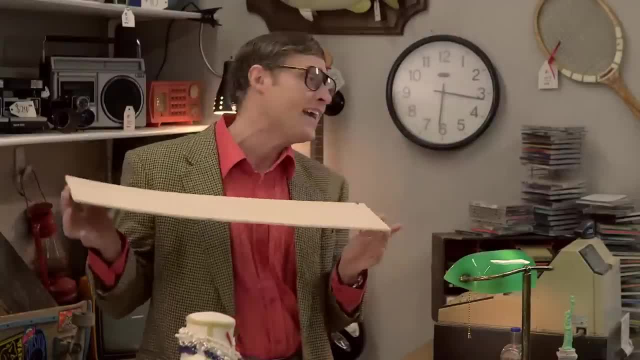 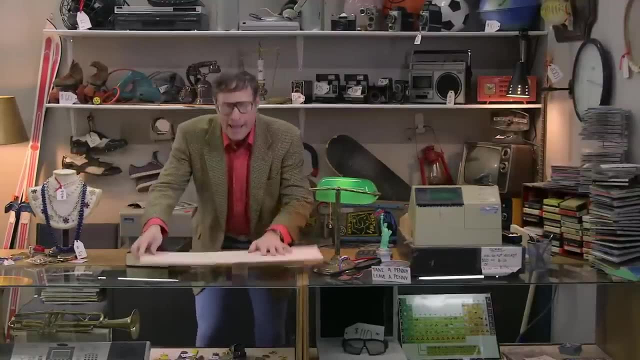 A plank can be a lever. All you need is two sides and a place for it to pivot- A fulcrum. It can be anything. Look at this Bam. Now it's pivoting. I put the book on this side and then I push down on that side. 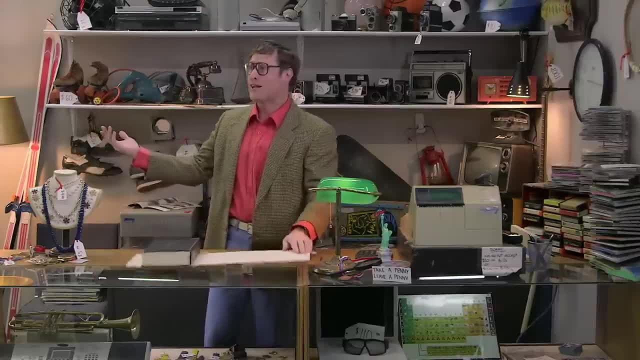 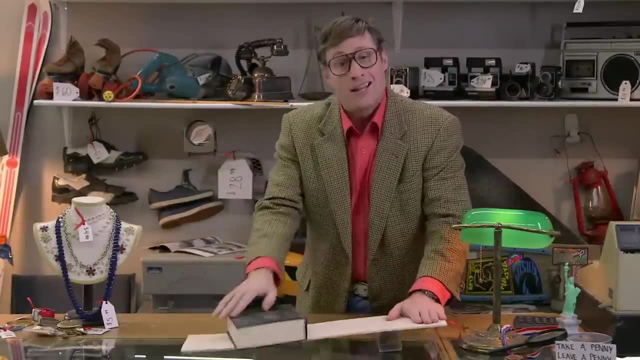 I'm doing work easy. Hey, look at me doing this work over here. If I want to do more work, I could move the fulcrum a little bit further over. Now. I do lots of work, but I lift the book a lot further. 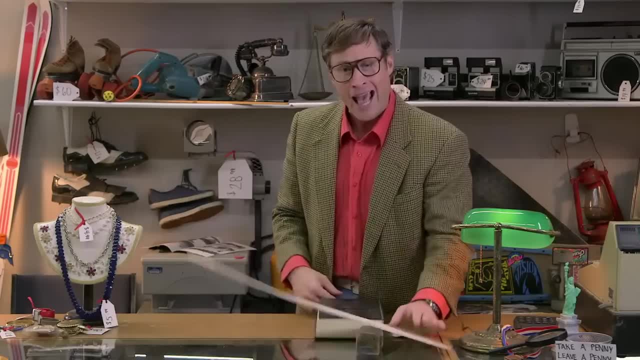 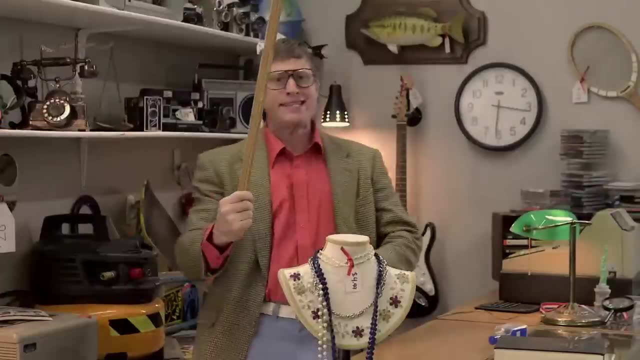 Look at that: Whoa, What, Whoa, Yeah, Huh. What do you say? What do you say? Huh, Huh. You don't like this lever, Don't worry, Hold on, I got another one for you here. 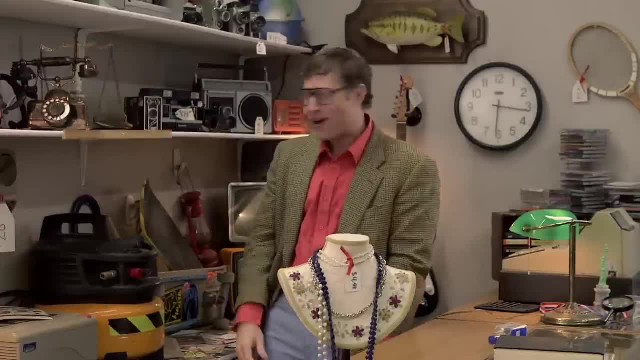 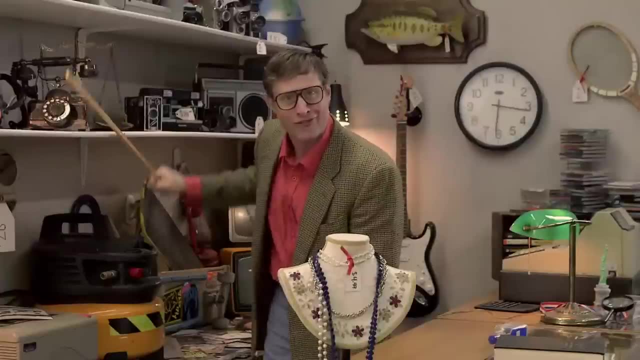 Hey, take this stick. All you need is two ends and a place for it to pivot Like this Bam. Now it's a lever. This side goes down, That side goes up, Down, Up. It's a lever, It's a lever. 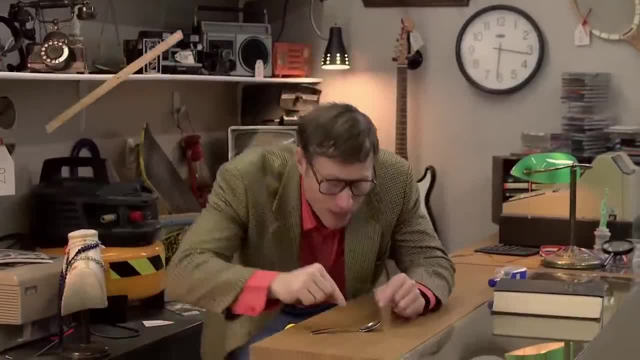 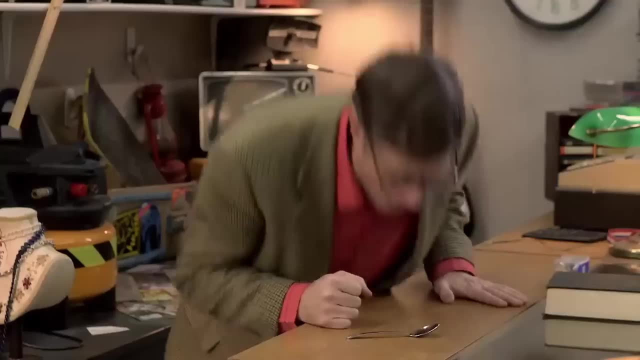 You want to make a catapult, Use a spoon. The place where the spoon pivots is the fulcrum, And now It's a lever. It's a lever, It's a lever. Look at this lamp. Now it's a lever. 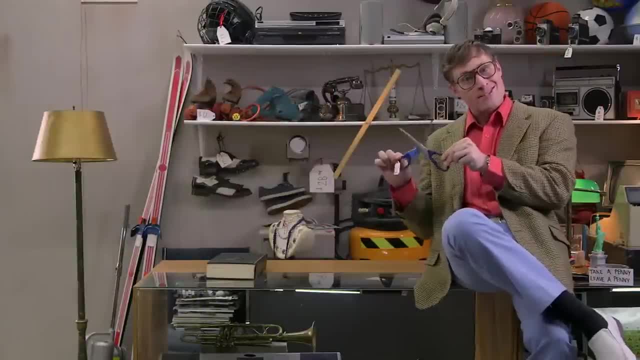 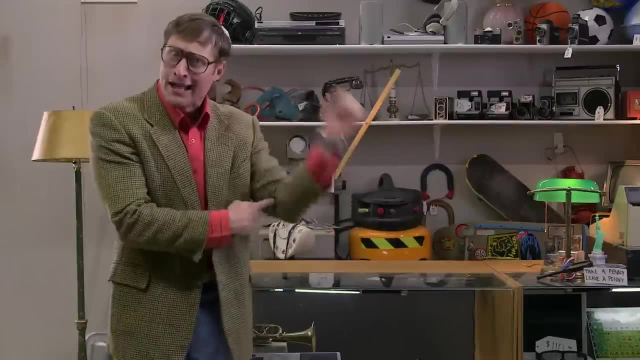 Scissors. Two levers, Your forearm It's a lever, Two ends And the fulcrum where it pivots. Yeah, The fulcrum can be at one end. Crazy, This fish. You guessed it Makes sense. 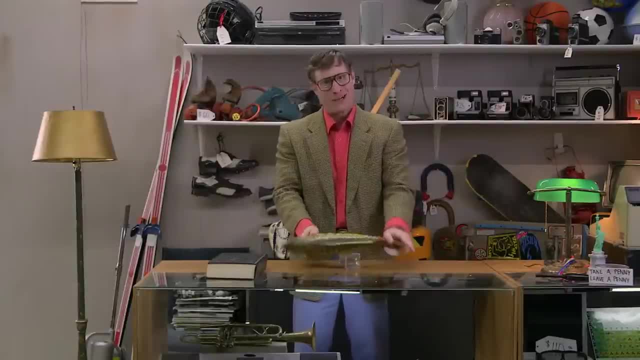 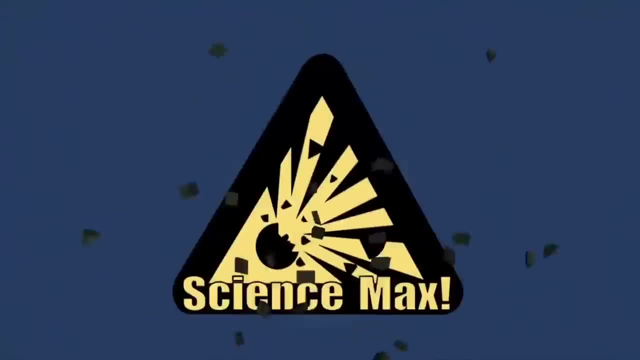 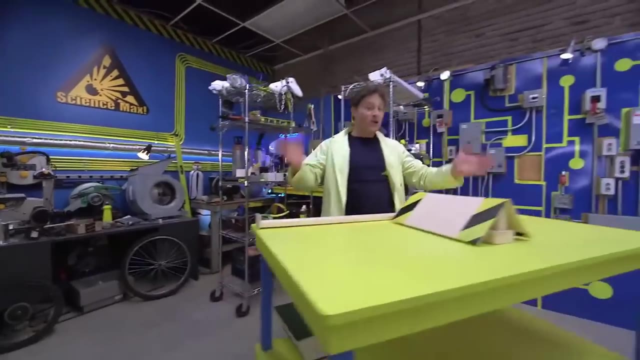 This fish. You guessed it. now it's a lever, and now you know you'll leave us. okay, where were we? oh yeah, levers. so you can use levers to become much stronger or at least lift something you couldn't normally lift. levers are simple machines and they work like this. 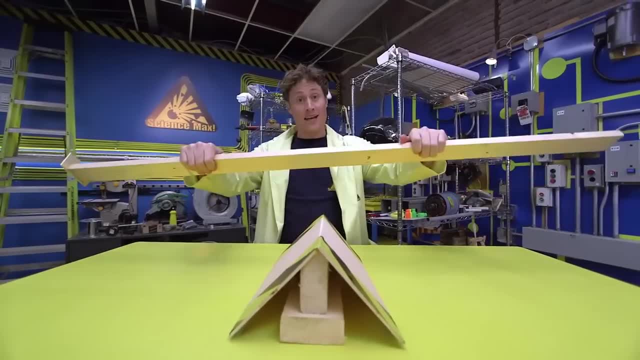 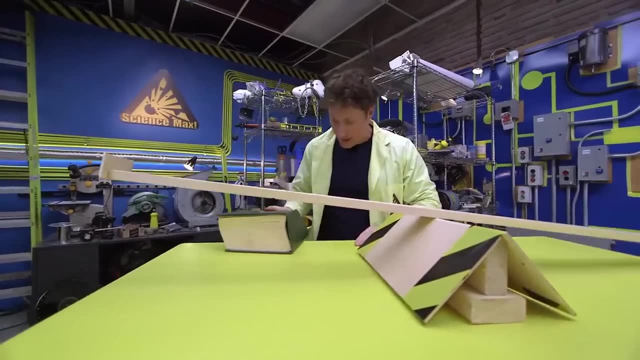 levers are just a long rod or a stick or pole or a piece of wood like I've got here, and something for them to pivot on, a fulcrum. now let's say you have something heavy like this book, sure I can lift it, but what if I told you I can? 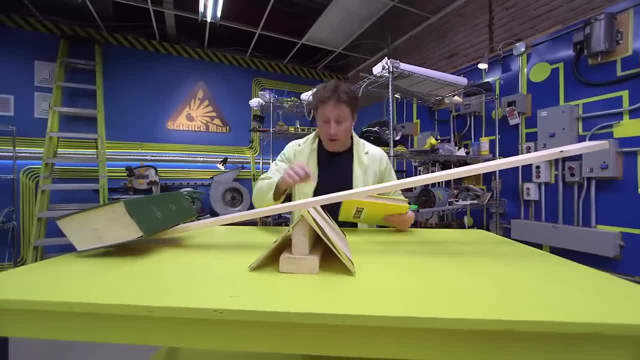 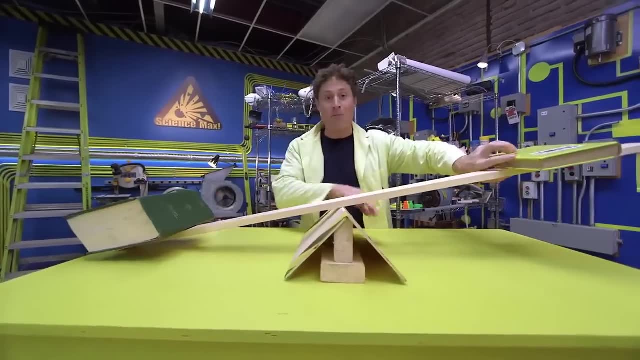 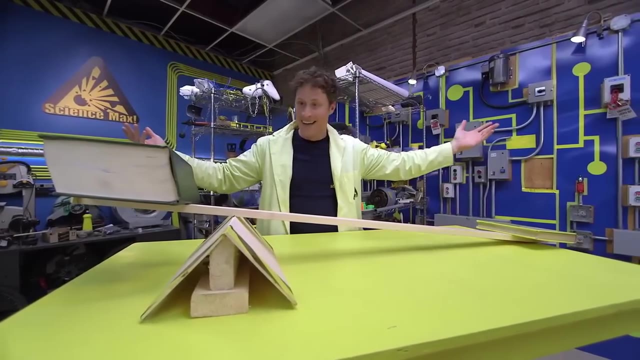 lift this heavy book with this book. now, if the fulcrum is in the middle like a seesaw, you can tell that book is much heavier than the other book. but watch what happens when I move the fulcrum: mm-hmm, mm-hmm, huh, it's like magic. but 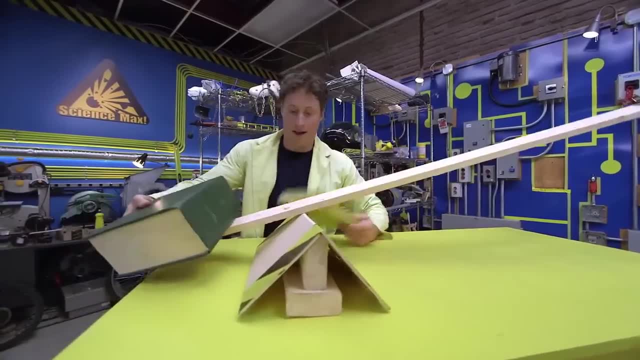 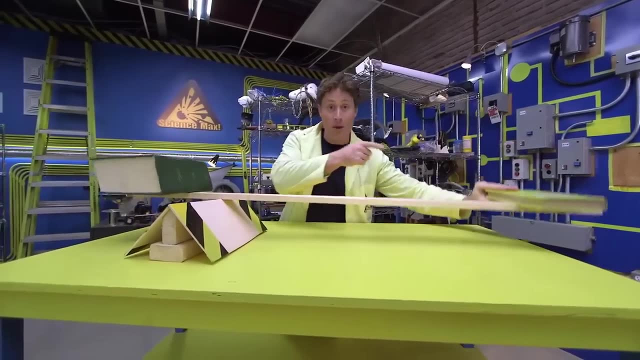 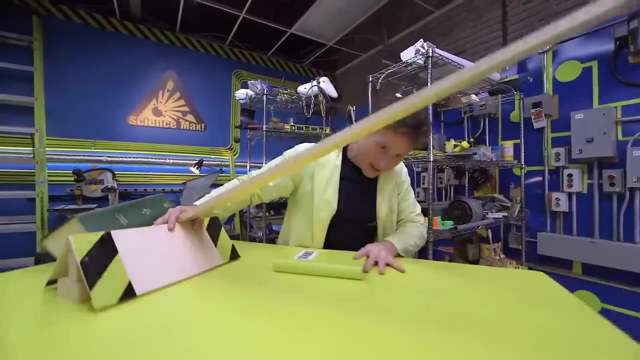 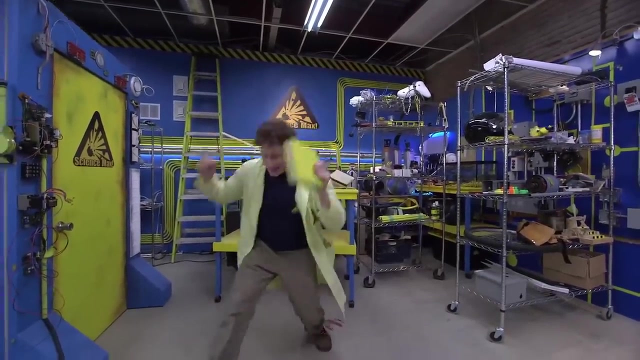 it's not magic, it's not magic science, whoa? it's because the small weight is moving a long distance and the heavy weight is moving a short distance. small weight, long distance, heavy weight, short distance. so everything balances out. but here's where it gets interesting: the longer your lever, the more weight you can lift. these are two heavy cinder. 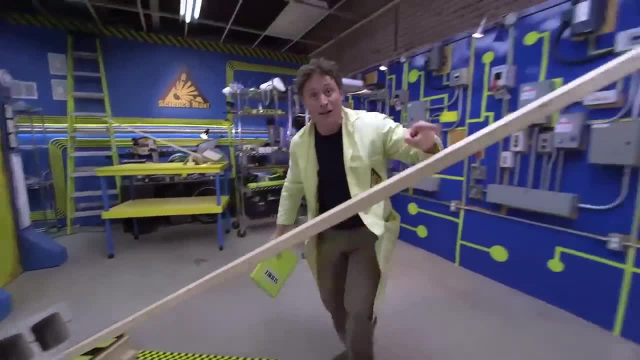 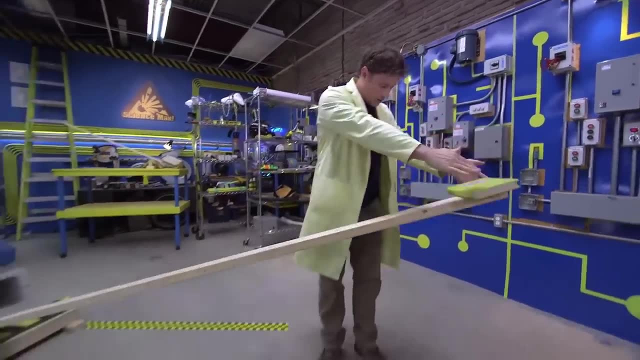 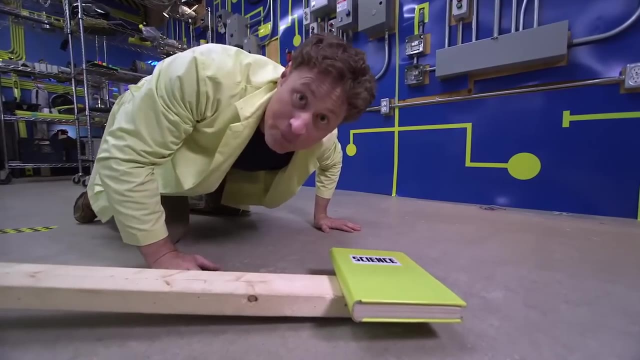 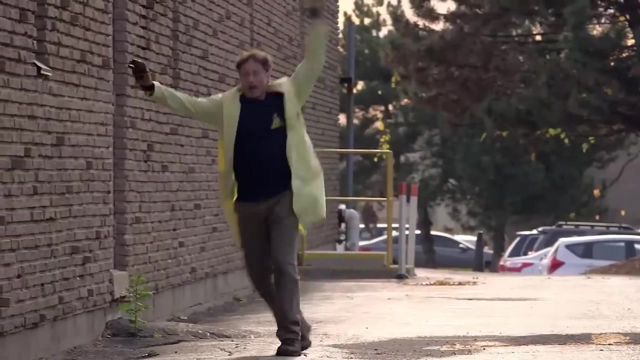 blocks. there's the fulcrum and here is a very long lever with which I am going to lift those cinder blocks with this book. and there you have it. levers now back to the particle impulse controller. oh right, oh haha. lever, lever, lever, lever lever. 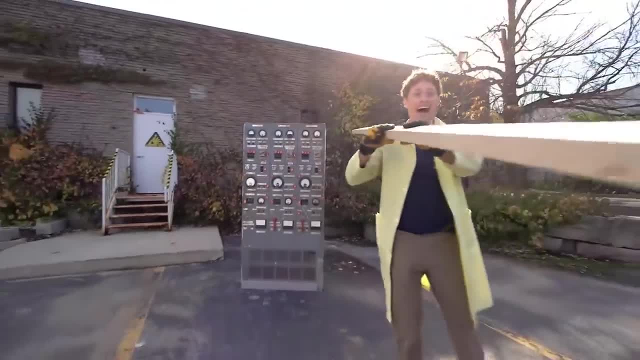 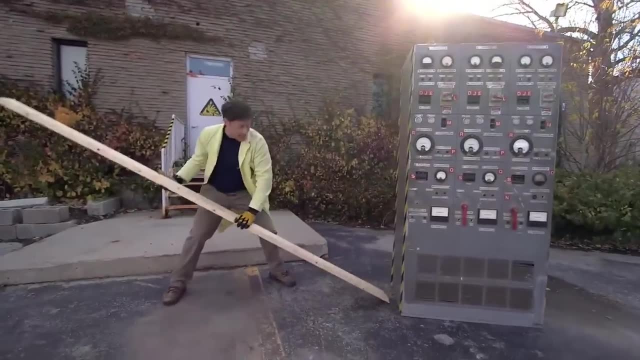 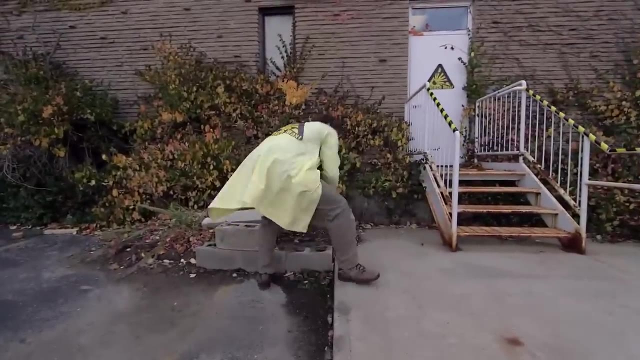 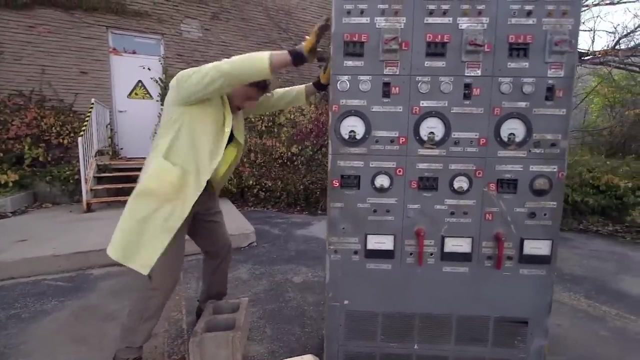 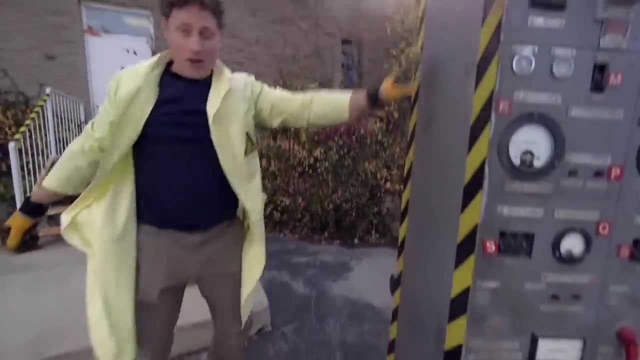 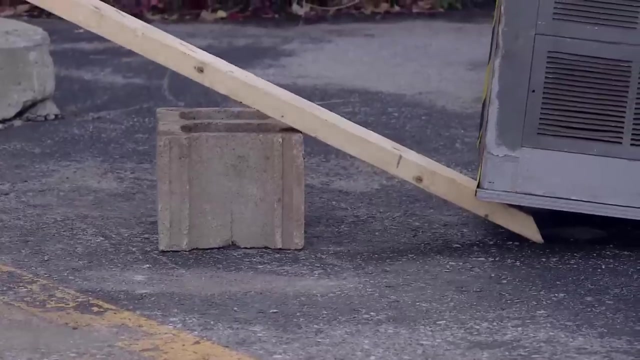 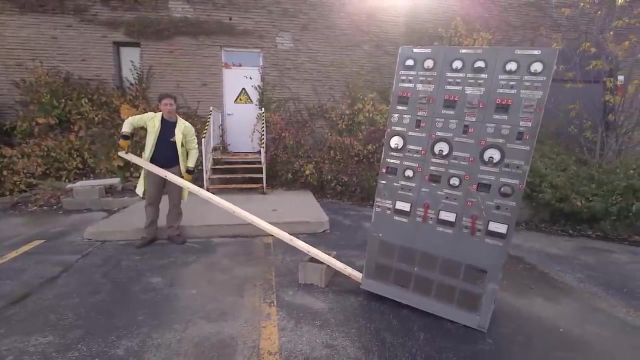 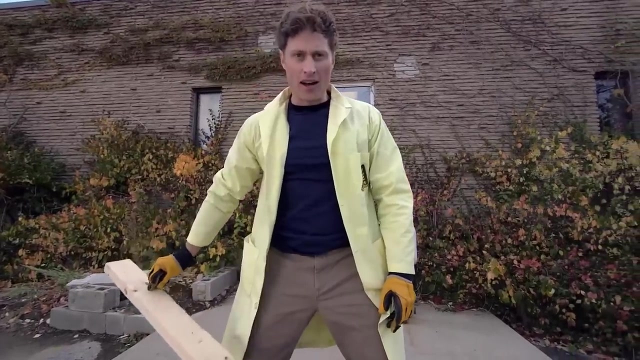 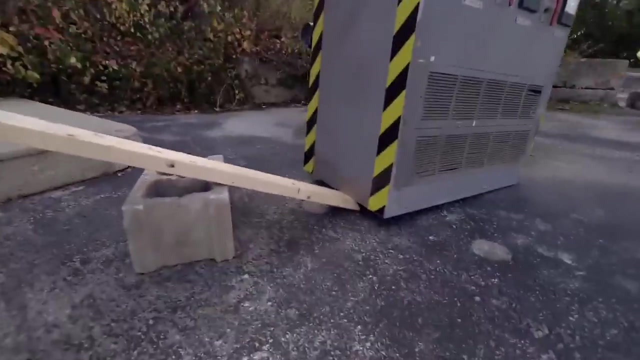 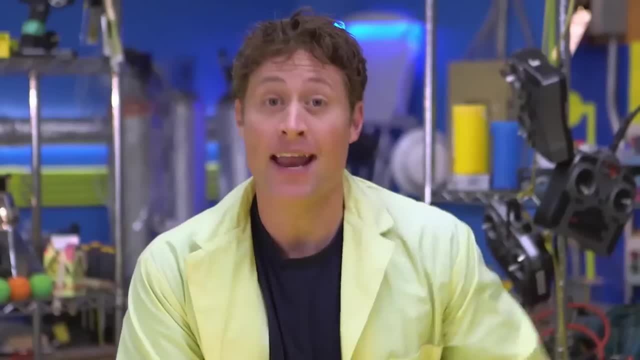 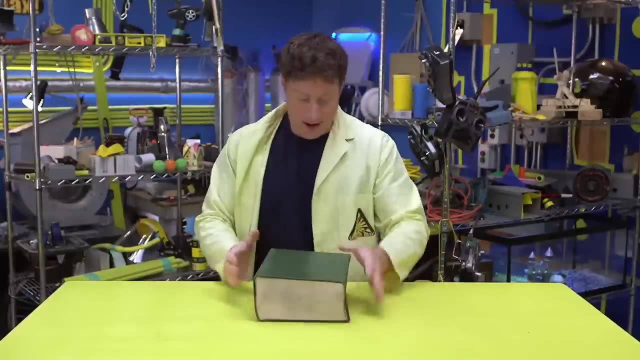 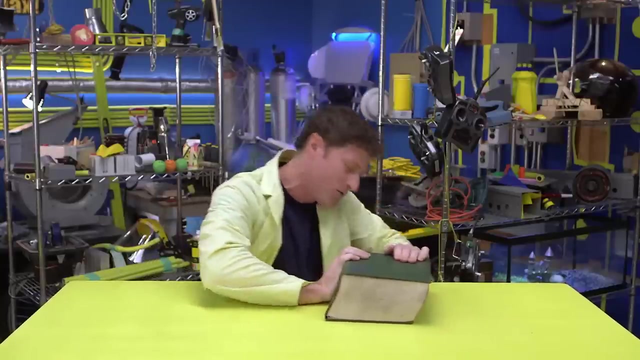 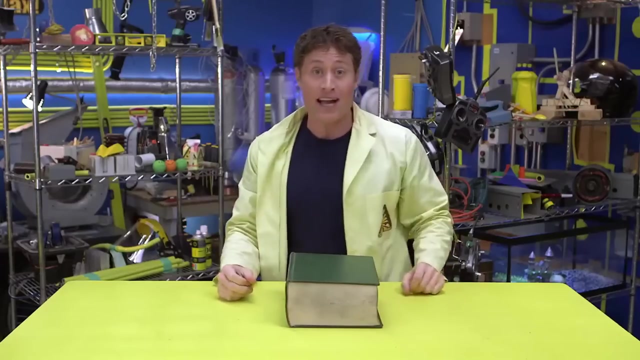 Rollers. Rollers are like wheels, except they're not attached to anything. In ancient times they used to move giant, heavy blocks of stone using rollers. We can demonstrate using a book. Now get a book, put it on a table and try to move it across the table. You'll see that it's very difficult. I can't move this book across the table. I can't. Okay, it's not really that hard, but still it takes effort. But if we get some rollers, I like to use pencil crayons and not pencils, and here's why 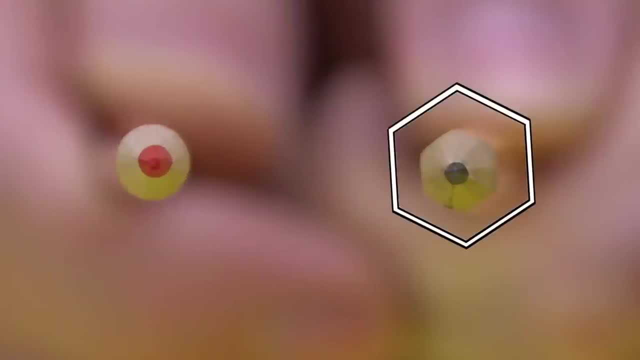 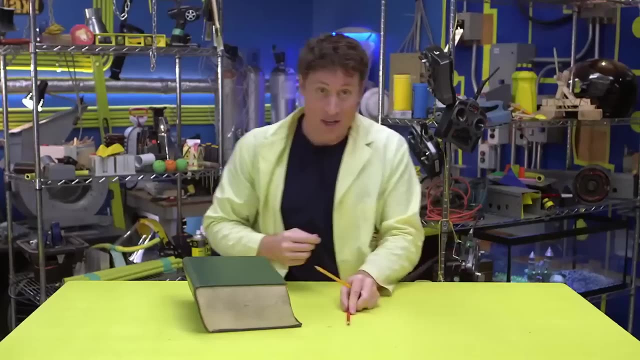 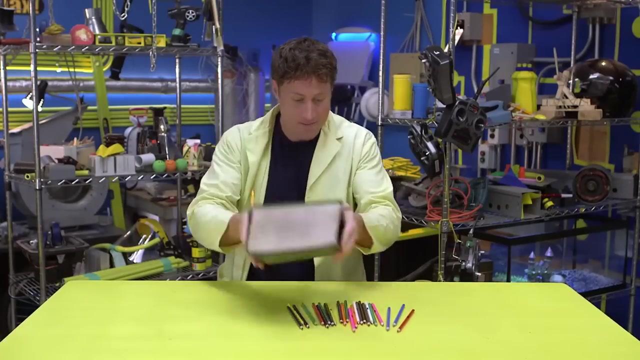 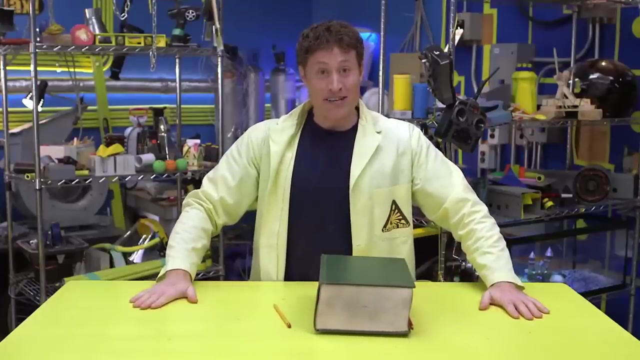 Now take a closer look. You see pencils aren't round, They're hexagonal, They have six sides, whereas pencil crayons are round, and of course, if you want something to roll, you want something round. So get a bunch of pencil crayons and put them on the table, and put the book on the pencil crayons and you'll see that suddenly, moving it is a lot easier. Alright, that's rollers. Back, I go. 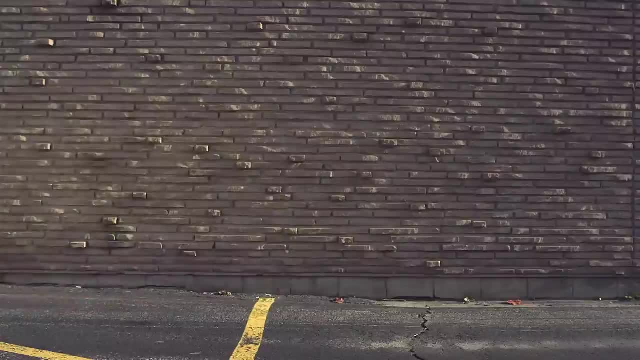 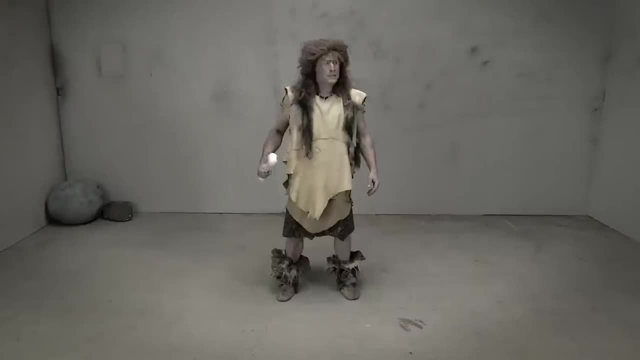 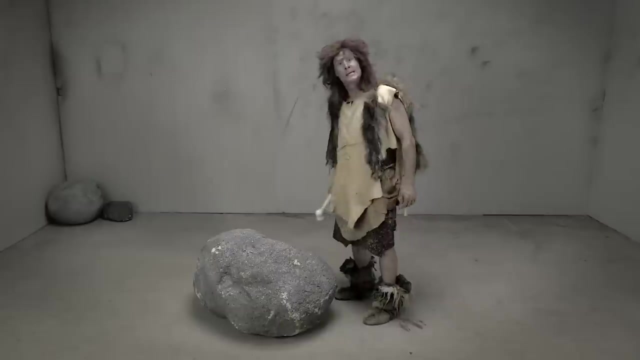 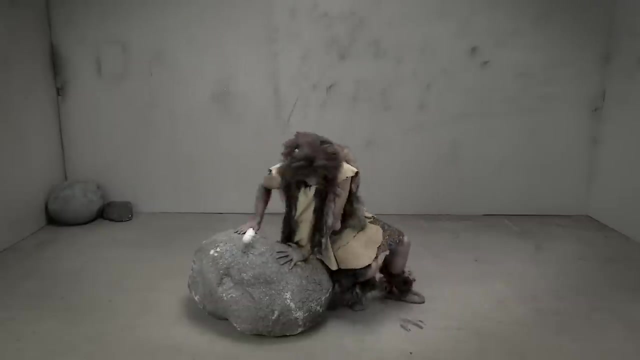 Now it's time for science. so simple a caveman could do it. This is a caveman, This is a rock. It is a well-known scientific fact that if this caveman were to try to move that rock, he would not know how to do it easily. Poor caveman. 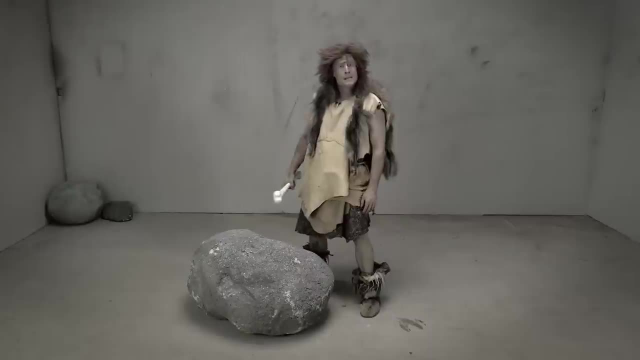 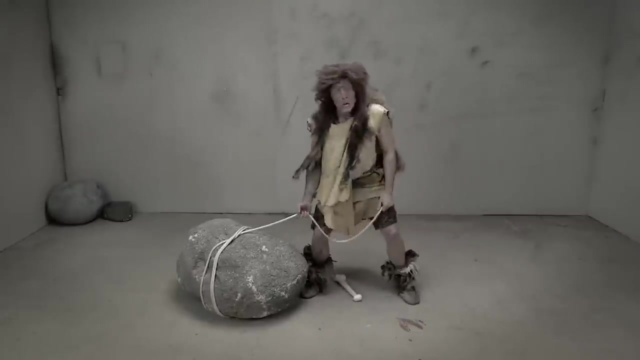 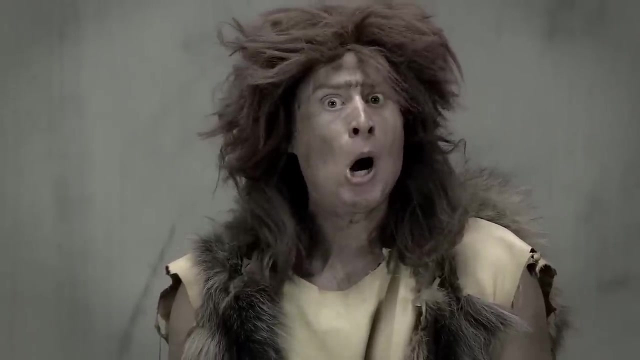 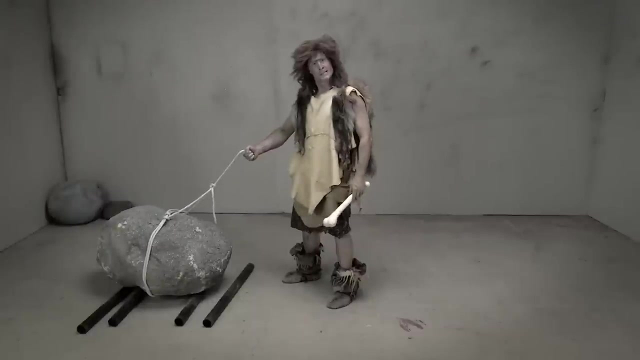 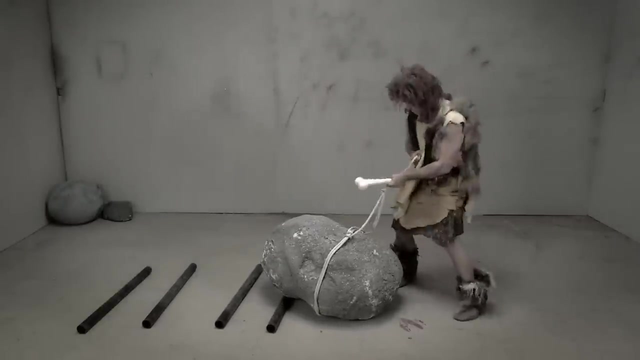 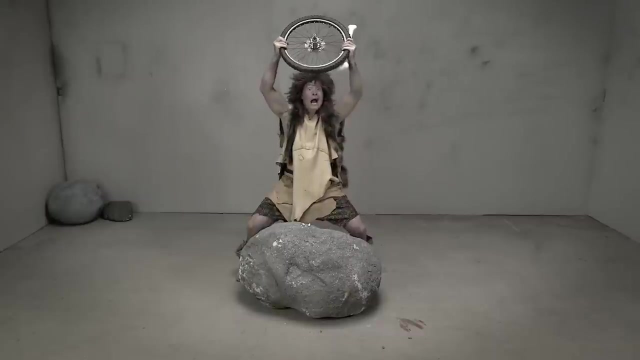 But in ancient times, people learned how to move heavy rocks using ropes and rollers. Oh, Rollers, Yes, rollers, Rollers, Rollers, Rollers, Close enough. Rollers make it much easier to move a heavy object, But they aren't perfect, So the wheel was invented. The wheel is a simple machine and one of mankind's greatest inventions. But no, that's not how it works. 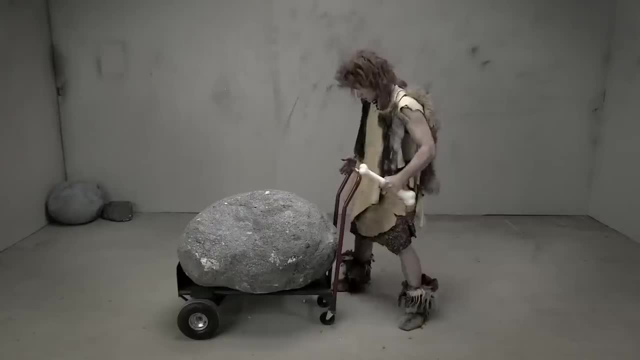 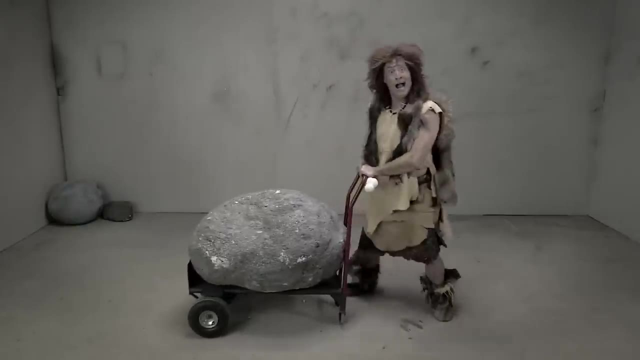 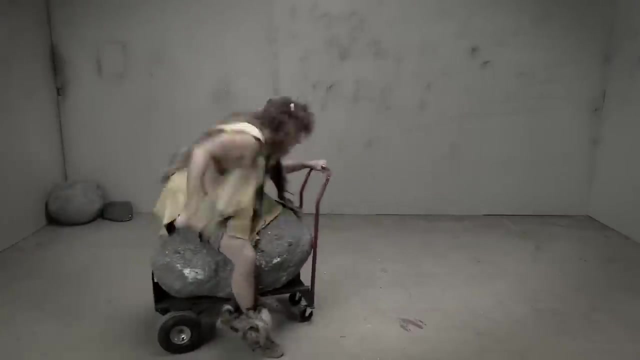 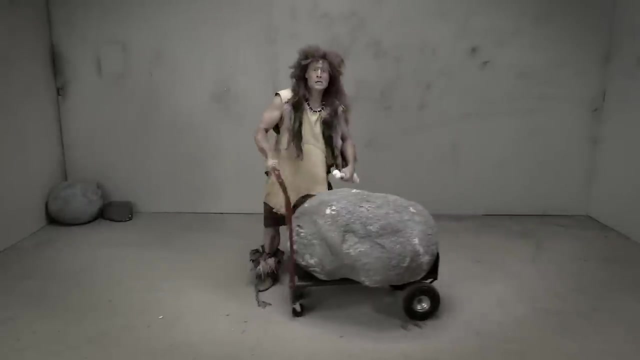 No Wheels go on axles which go under a platform. Now you have something to place that heavy rock on to move it around. But all these great inventions came after the time of the caveman. Caveman had to do everything the hard way. 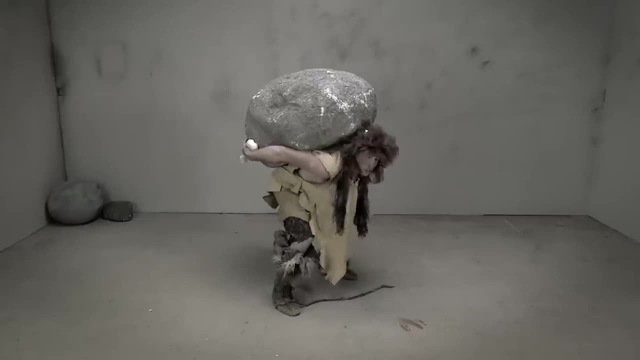 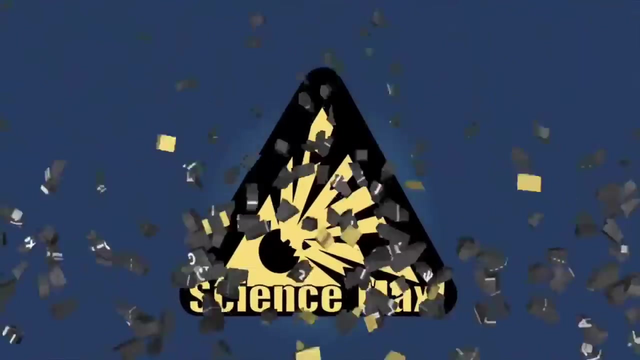 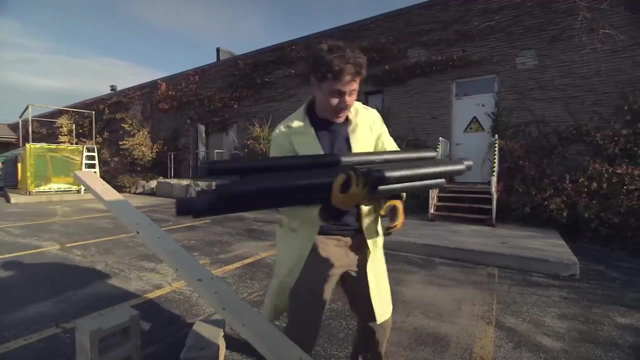 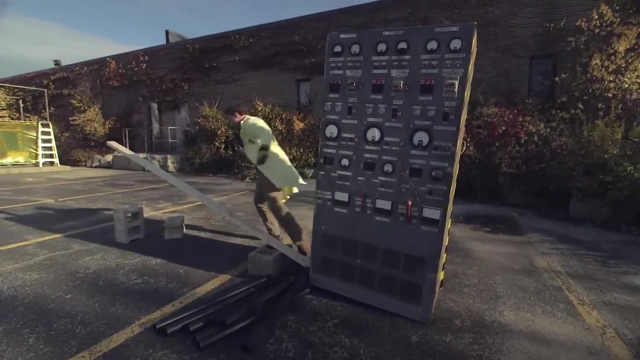 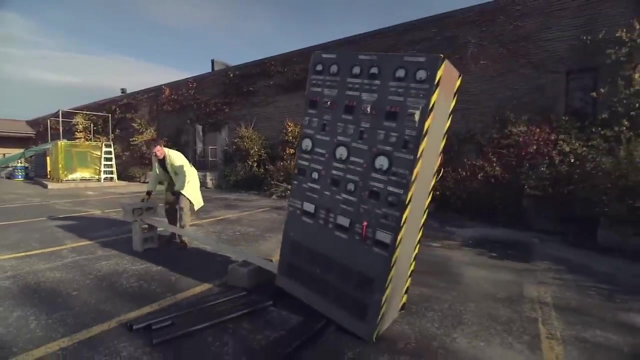 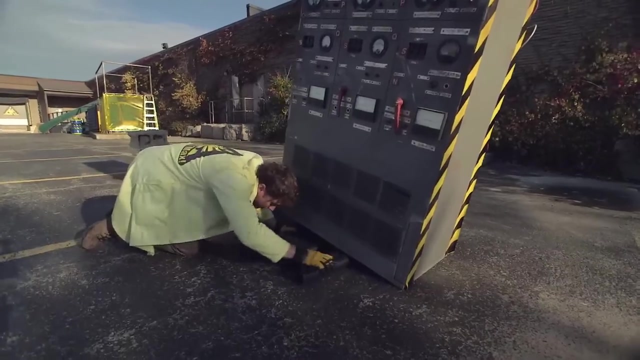 Join us next time for more science. Okay, I've got rollers. They're just plastic, They're just plastic pipes, but they'll work perfectly. I put them here And now to lift up the machine. Okay, Perfect. And so the rollers go underneath like that. 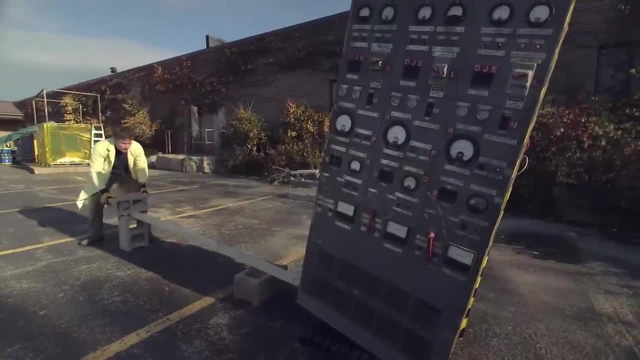 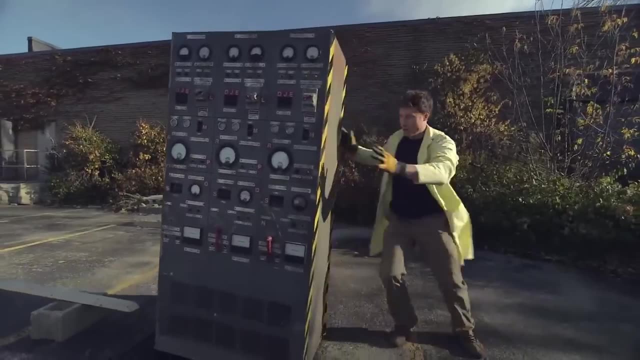 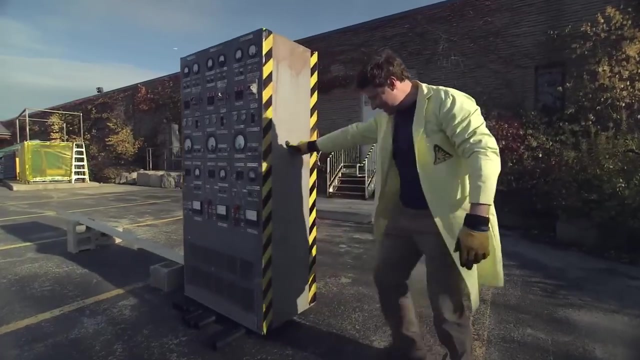 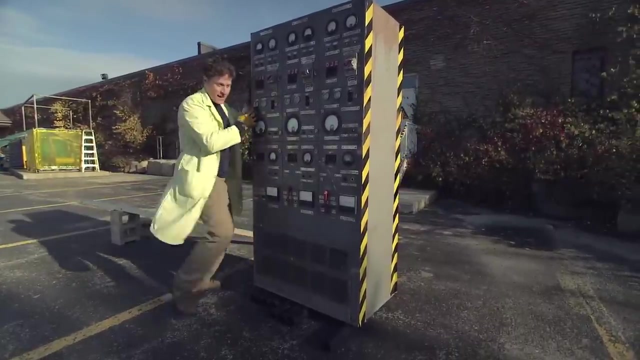 And then Whoa, Whoa, careful, Uh-huh, Look at that, No problem, Wait, I got to get rid of this To get it moving. Now, the trick with rollers is you have to keep taking them out of the back and putting them in the front. but 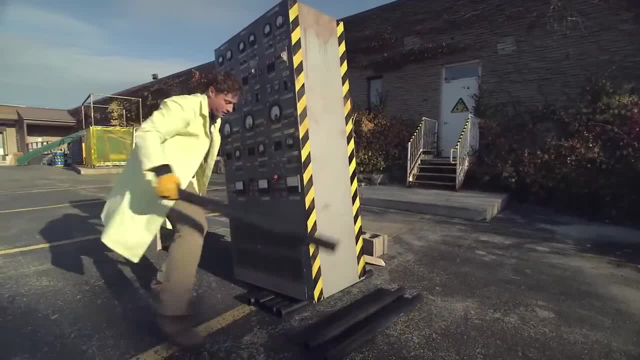 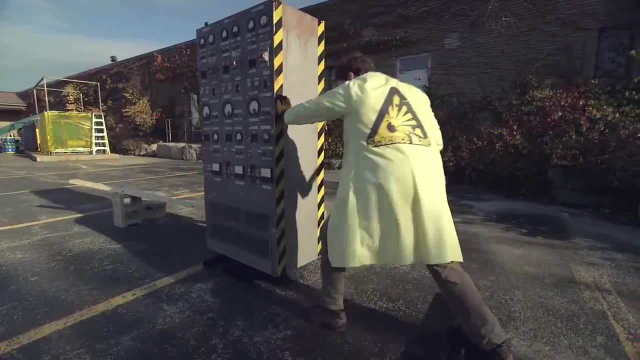 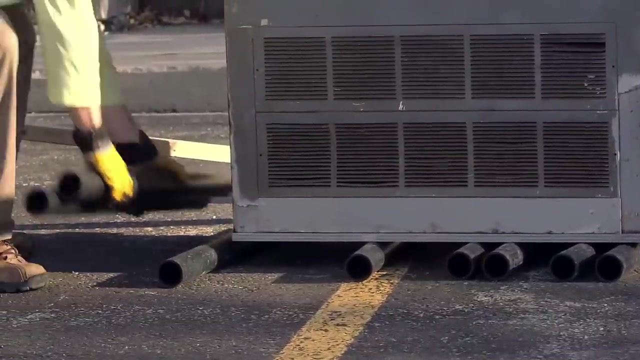 Whoa, Whoa, Whoa, This is bad drawing. Whoa, whoa, stop, rollers, stop. oh no, oh no, okay. okay, whoa rollers, easy, there we go. Okay in the front, roll it forward. 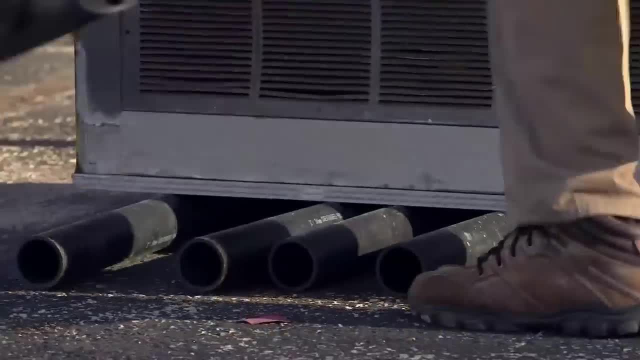 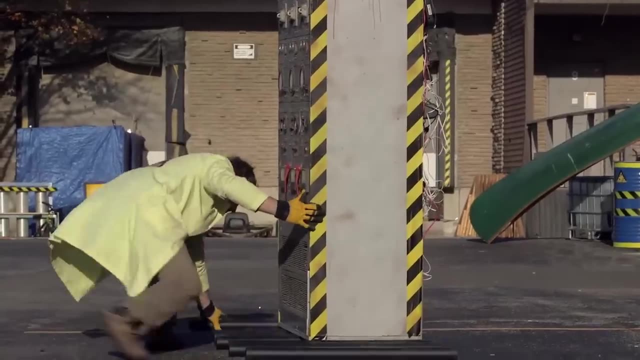 Now I know what you're thinking. you're thinking this seems like a lot of work, and it's true. moving the rollers back and forth and back and forth does take some time. But did you know? this was how the pyramids were built. 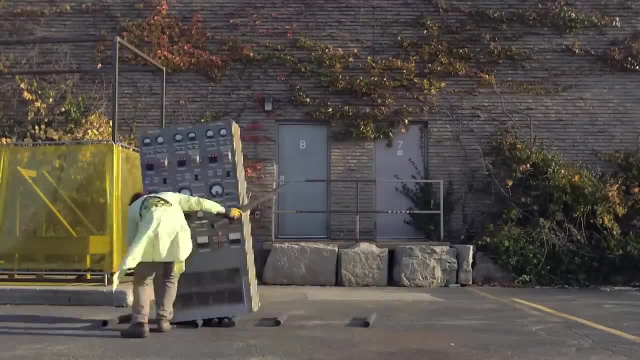 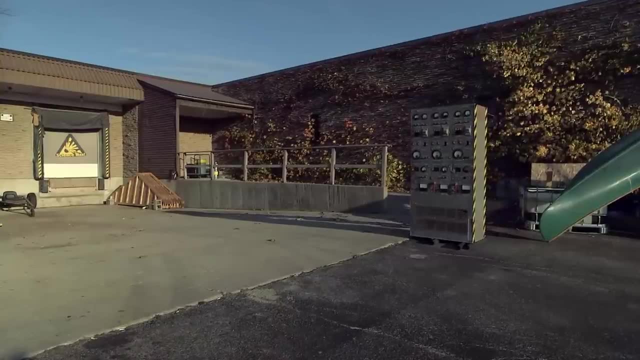 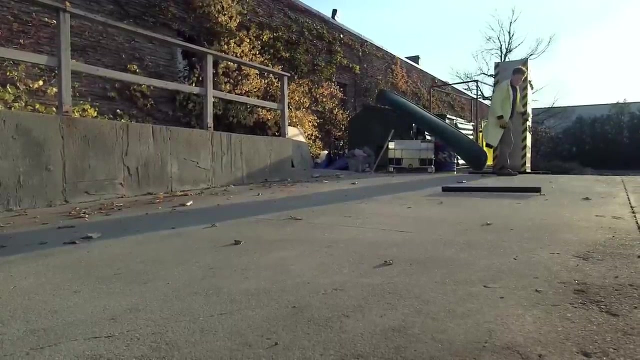 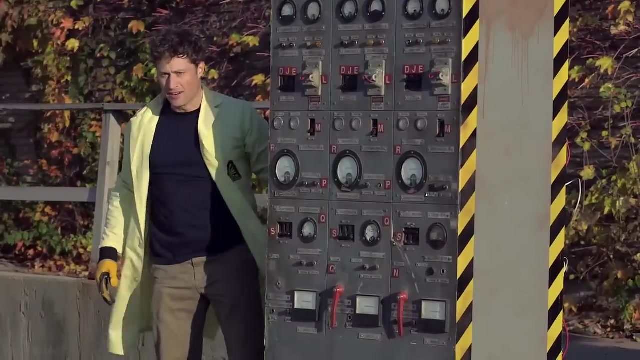 It's true, giant stone blocks were moved on rollers, just like I'm doing here, And, as you can see, what worked for the ancient Egyptians works for me too. Uh-oh, Yeah, there's a hill here. If I go down the hill. 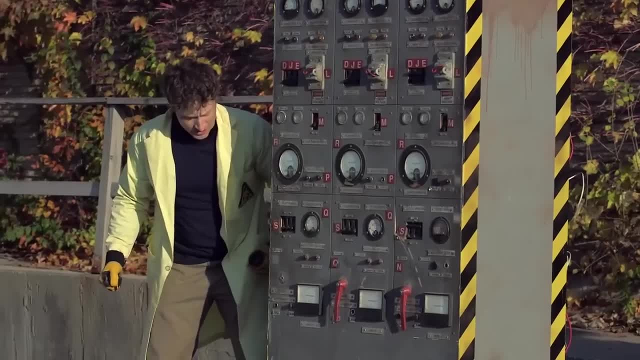 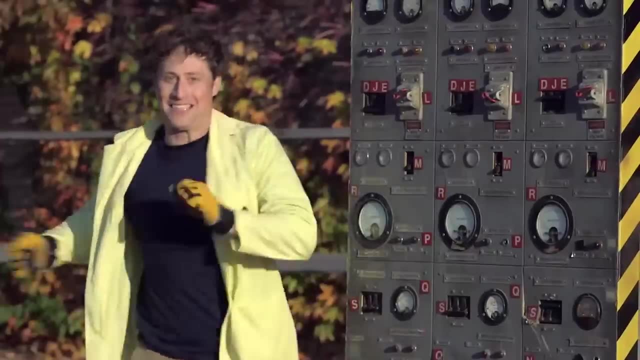 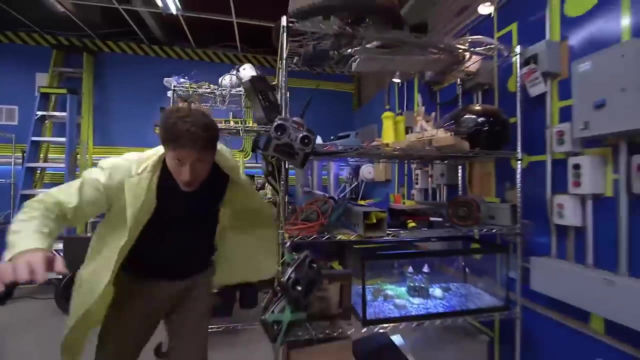 it's going to start rolling faster than I can do the rollers. I'm going to need some help. Um uh oh, I know, pulleys, pulleys, pulleys. Okay, pulleys, pulleys are a great way to change the direction of force. 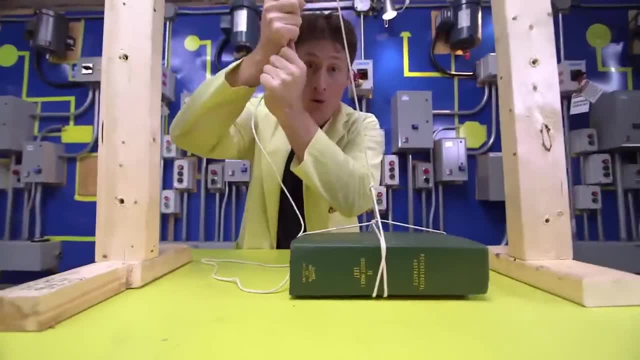 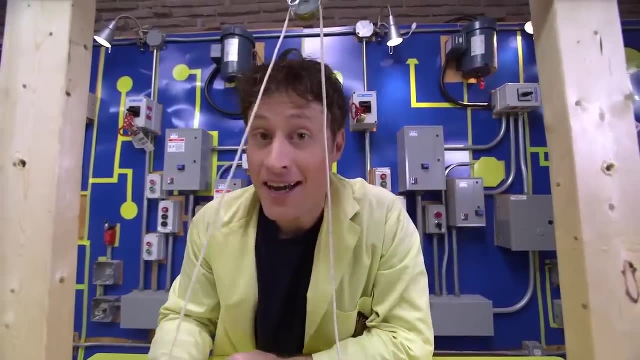 I've got a rope going through this pulley and down to a book, so when I pull the rope down, the book goes up. Changing the direction of force can be very helpful, but pulleys can be helpful in another way. Pulleys can let you lift something that you couldn't normally lift. 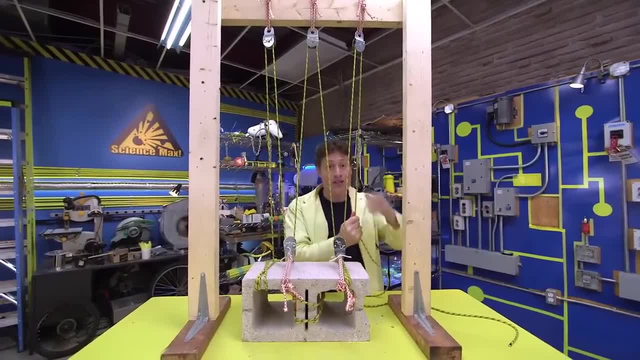 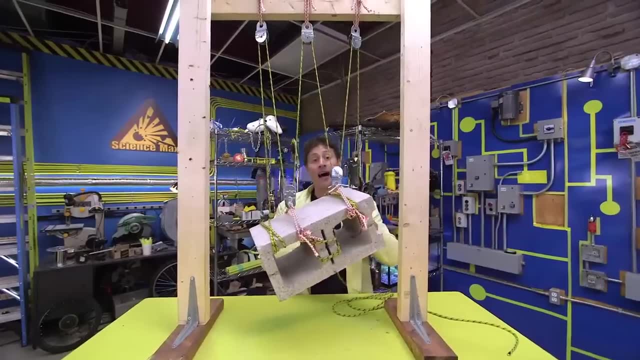 Now the rope goes up and down, and up and down, and up and down, and the force I need to lift this cinder block is a lot less than if I was just lifting it by myself, But I've got to pull a lot more rope. that's called mechanical advantage. 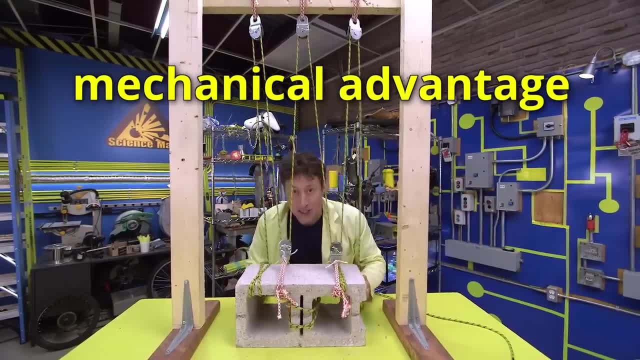 Spreading out the force over a longer pull so you can lift a larger weight. If you use more pulleys, you're going to have to pull a lot more rope. If you use more pulleys, it reduces the amount of force. 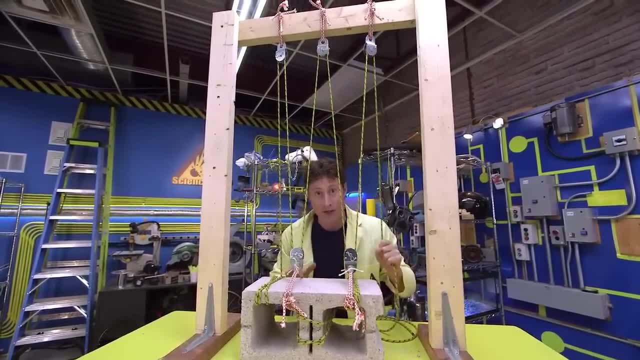 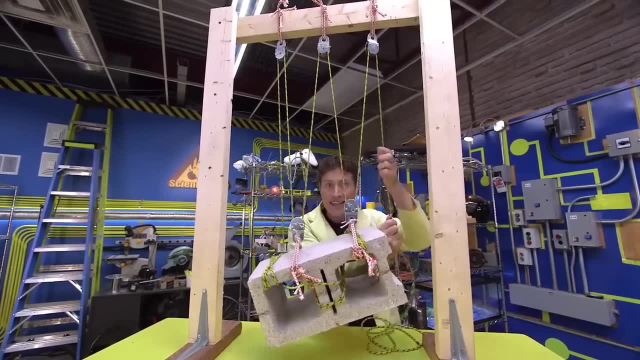 One pulley same amount. Two pulleys half the force, Three pulleys one-third. So I've got five pulleys here, which means I only need one-fifth the force to lift this cinder block. So there you go, pulleys. 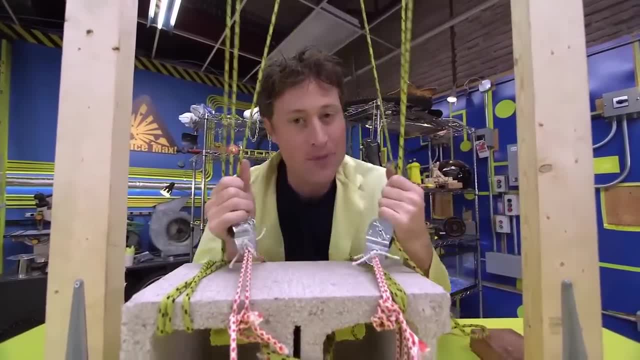 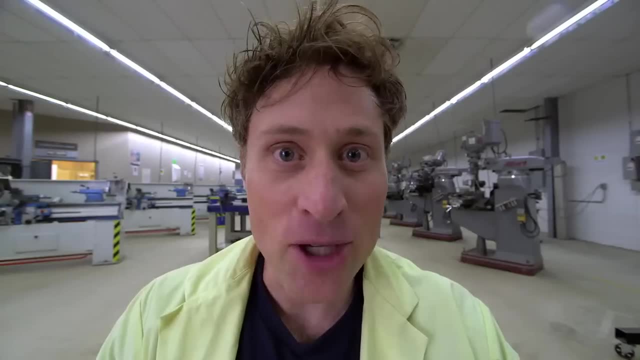 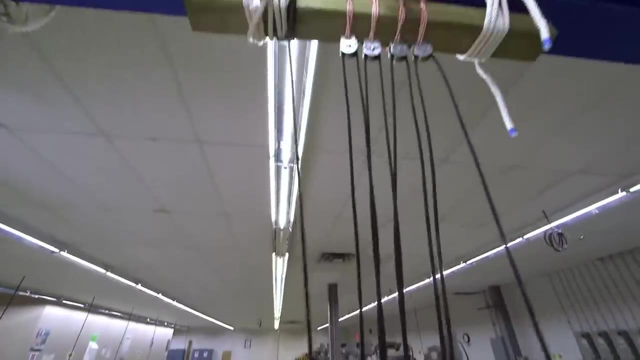 Now back to the Wait a minute, wait a minute. This calls for a mini-max, Mini-max. So how much weight can you lift with pulleys? Well, as much as you want, really. I have four pulleys on the bottom and four pulleys at the top. 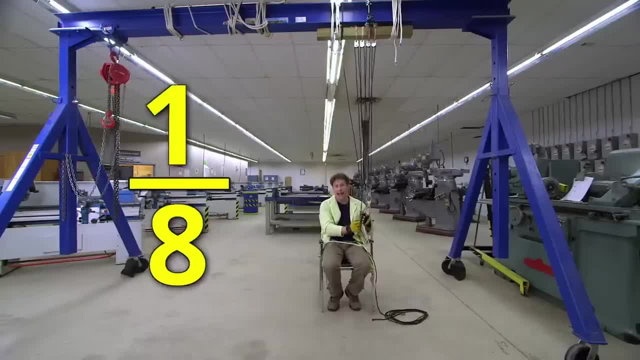 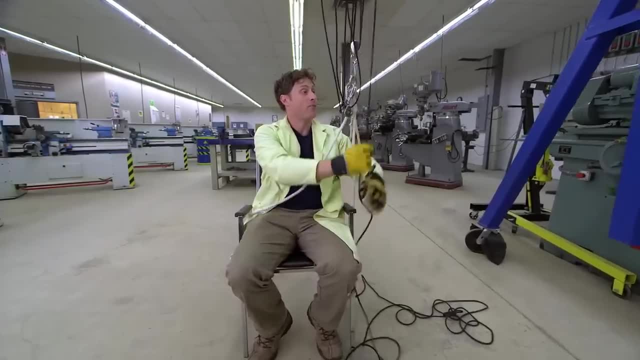 That means with eight pulleys, I only have to lift one-eighth of my weight plus the weight of the chair I'm sitting in, And if I keep pulling, you will see that the chair I'm sitting in is roped to the pulleys. 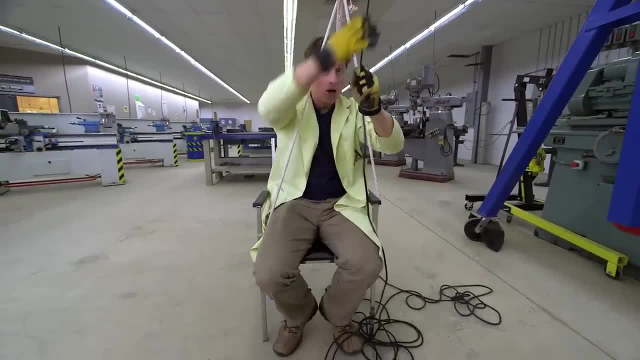 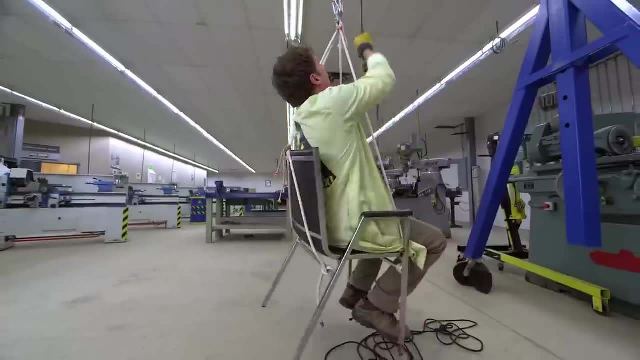 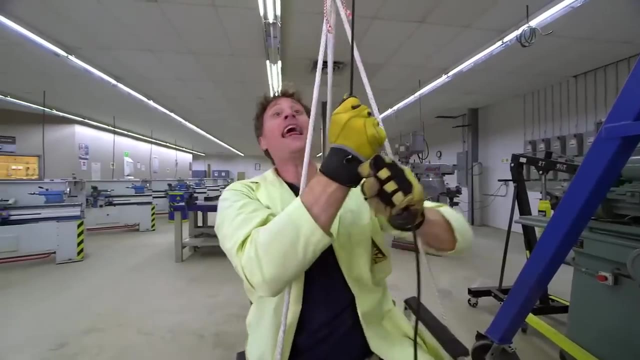 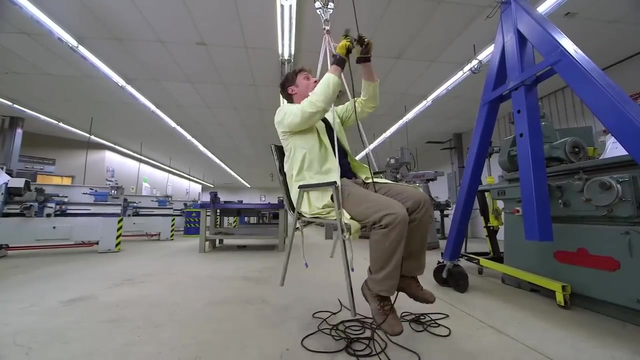 So now we see if I can pull myself up with nothing but pulleys. Look at that. I'm totally lifting myself into the air with the power of pulleys, And I don't need to use two hands. In fact, I only need to use one finger to hold myself up. 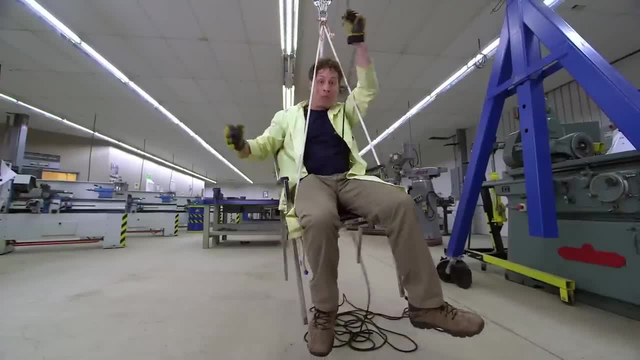 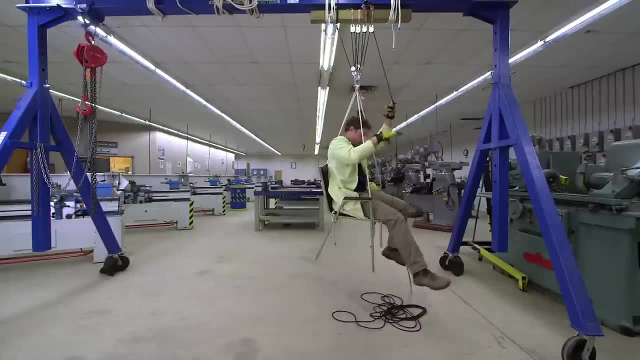 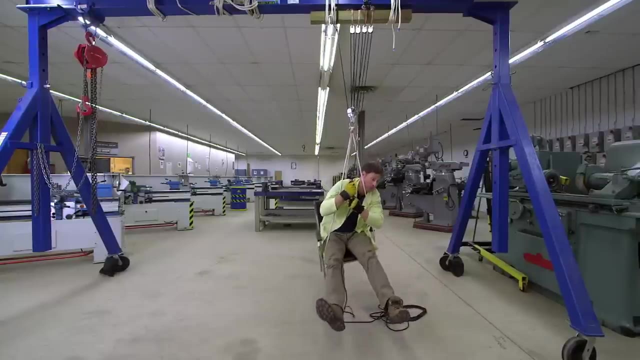 And my thumb, obviously, to hold the rope. That is the power of pulleys. I can almost make myself fly. Well, almost Now back to the particle Particle impulse controller, Letting myself down. Particle impulse controller, Let's go. 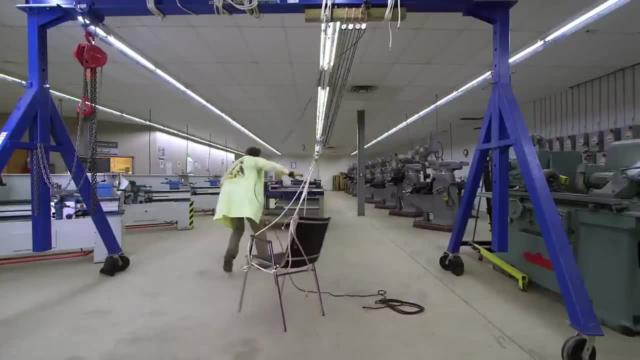 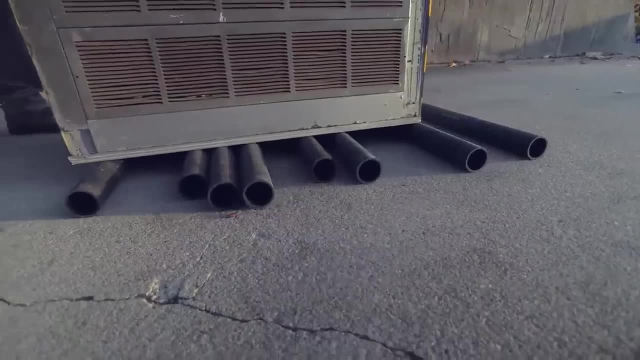 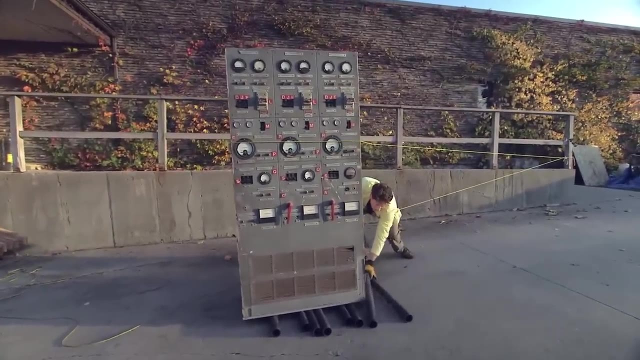 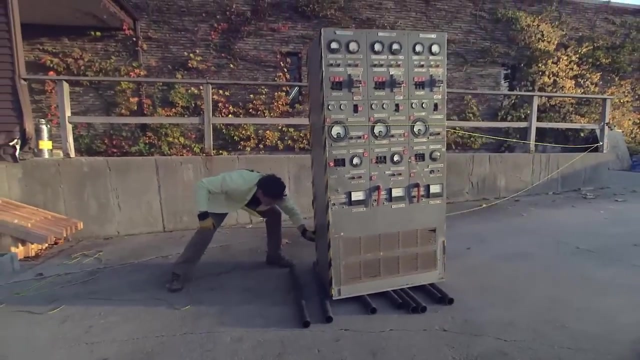 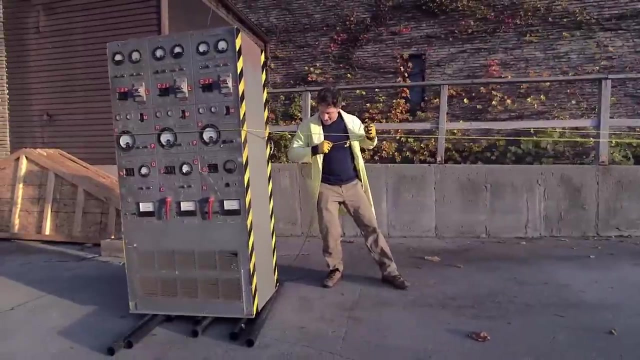 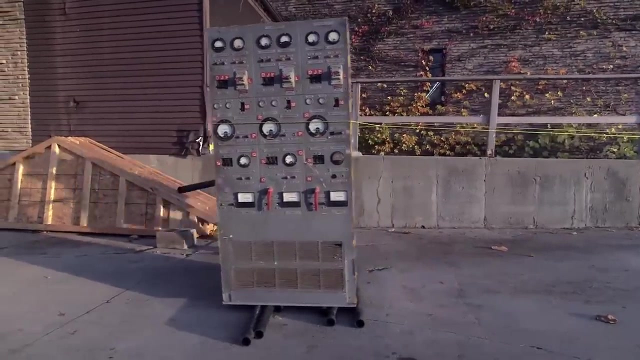 Wait, Let's go. All right, I've been able to use this pulley to lower it down the hill at the speed I want to go. Interestingly, I'm using the pulley not to make it lighter, but to just change the direction of force. 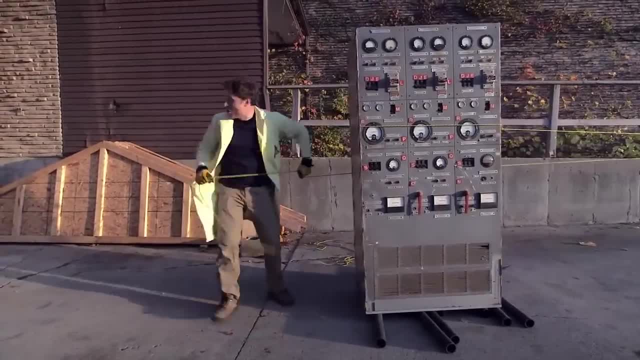 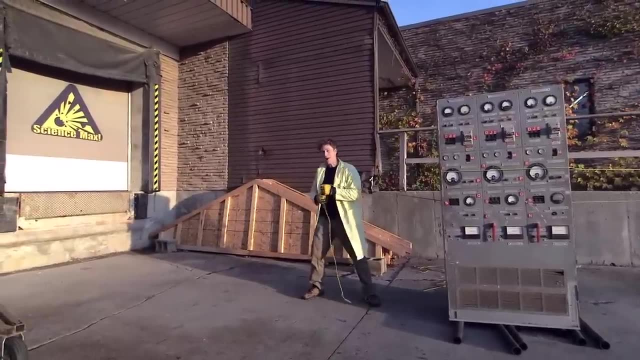 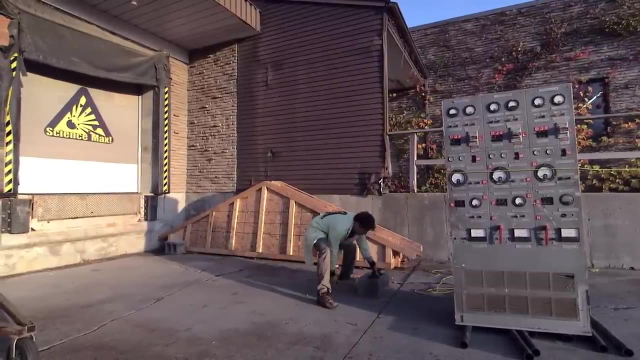 And I managed to get it right here at the bottom. Now I've got to get it up onto the loading dock, so I think this is where I need a ramp. Whoa, Whoa, Oh, Oh, Oh, Oh Oh. 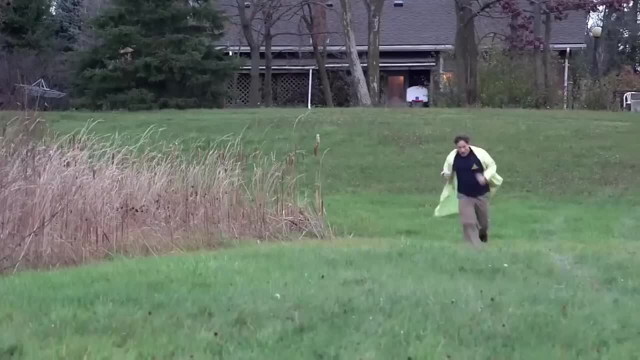 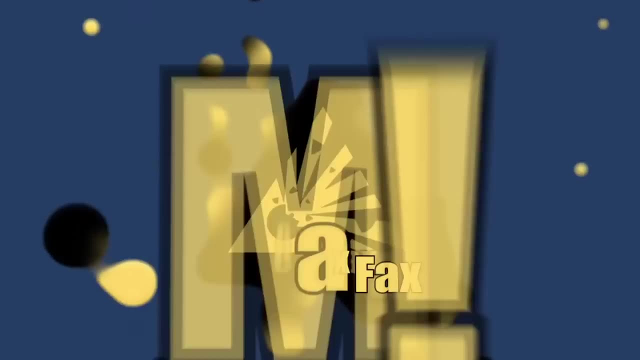 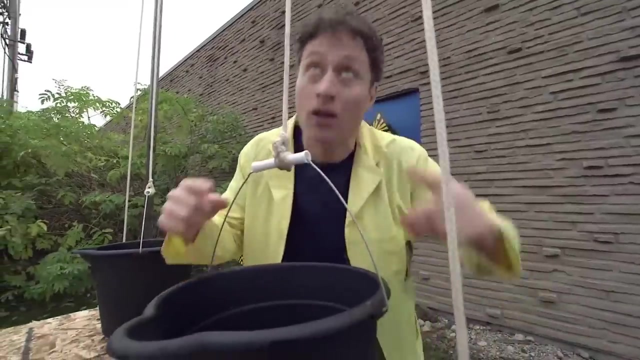 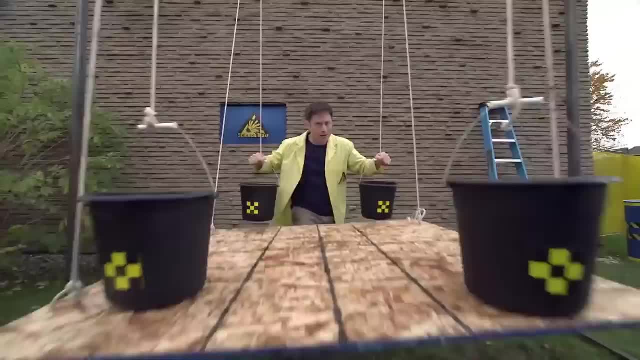 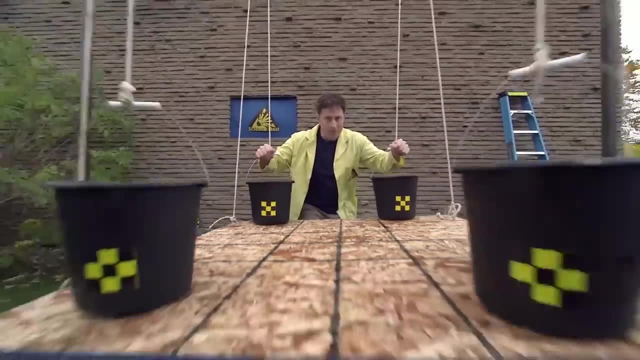 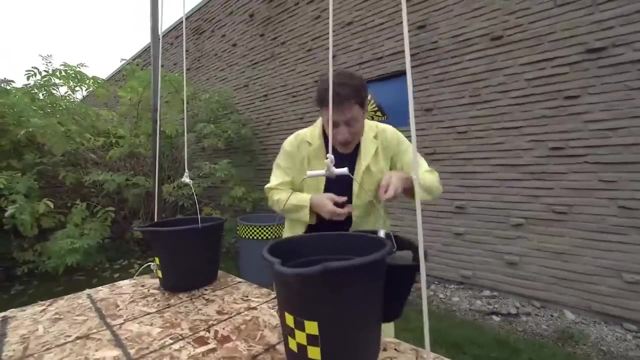 on the table. So if I took the buckets off the table, the weight of the buckets pulls the table up, But because the buckets are on the table, everything is in balance. Mind bending, right. Okay, wait, If I took a weight and I put it on the table? 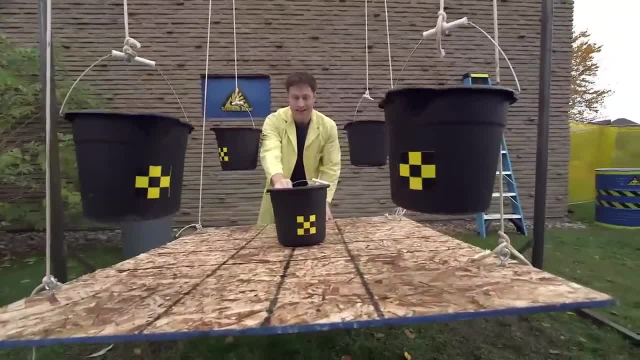 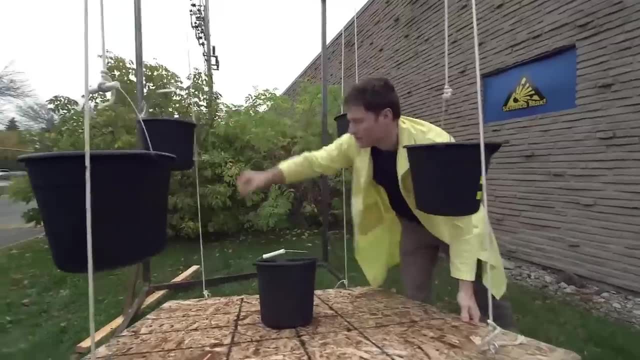 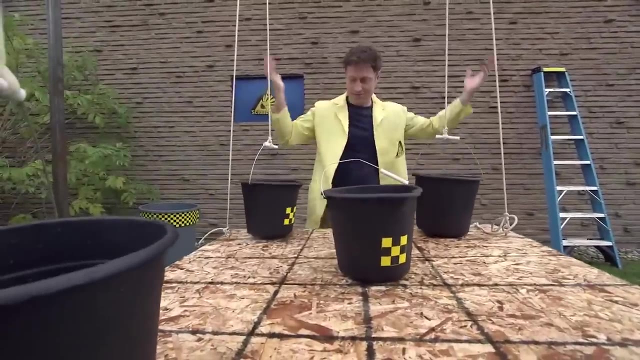 the weight of the buckets isn't enough to keep the table up, So I have to add more weight to the buckets, so the buckets hold the table up. Whoa, And there you have it. It's weird, It's mind-bending. 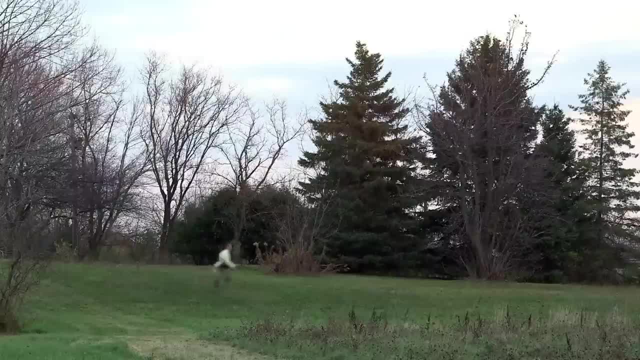 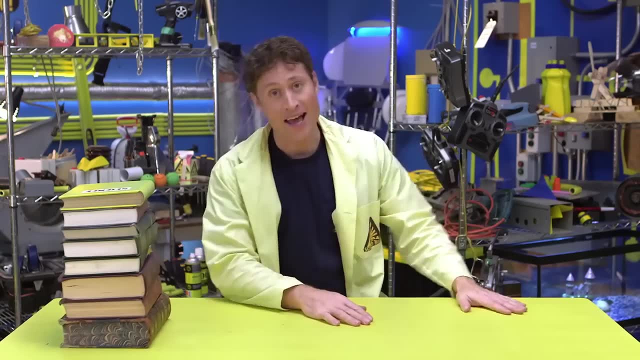 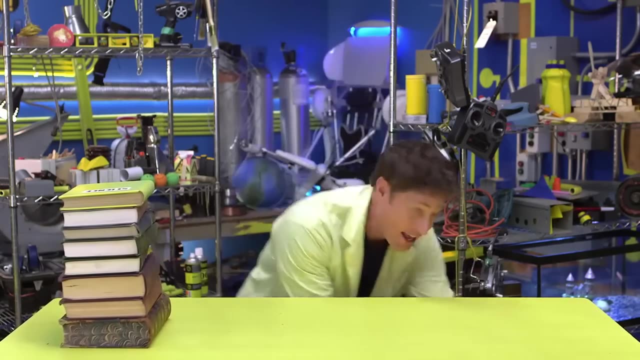 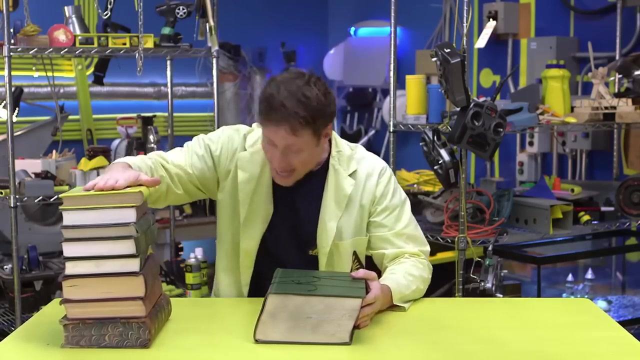 It's science. Oh, OK, OK, Ramps. Ramps are a great way to move something up. I will demonstrate using- you guessed it- a book. Let's say I wanted to move this heavy book on top of this stack of books using just this little string. 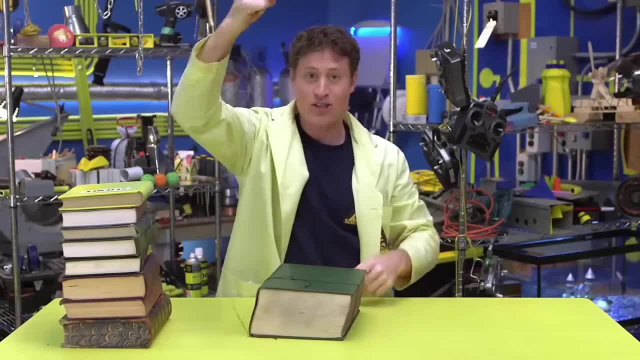 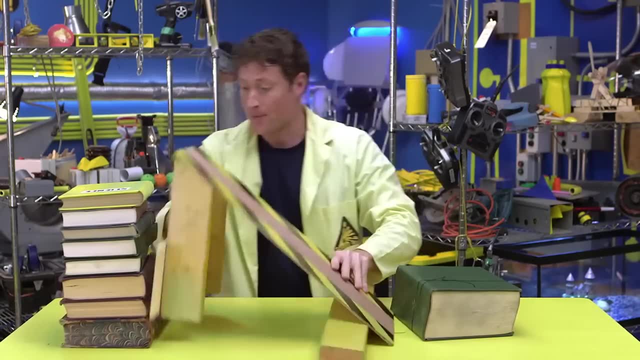 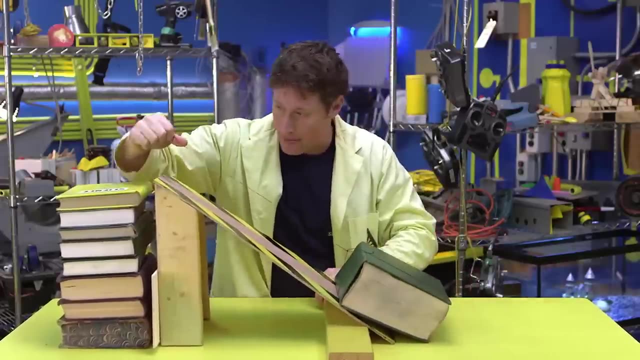 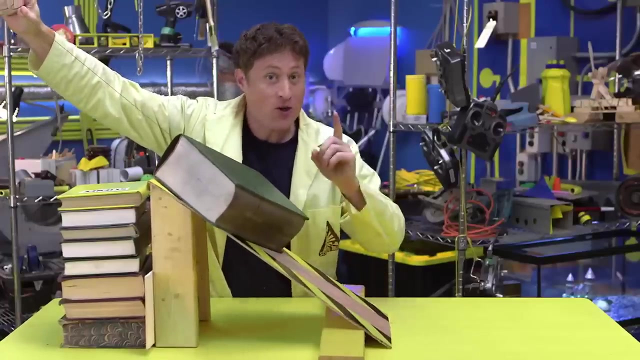 Watch what happens: The string breaks. But If, If I built a ramp to get the book on top of this stack and I use the same kind of string, watch what happens. this time You see, the ramp distributes the force, So you use less force to pull the book over the same amount. 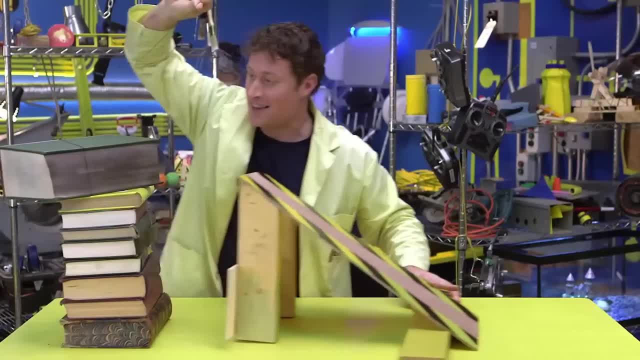 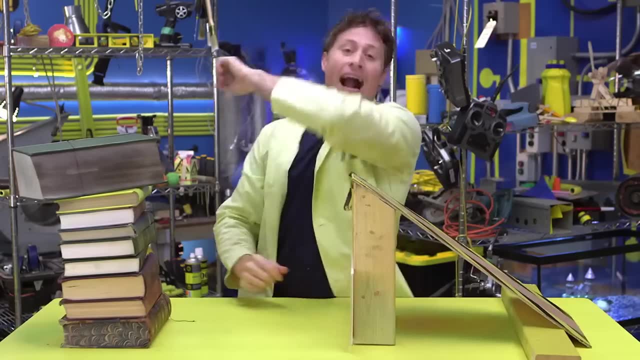 of distance, and I can get it up to the top of the stack of books, and the string doesn't break. So, ramps, Let's put them into action, Let's put them into action, Let's put them into action. Whoo. 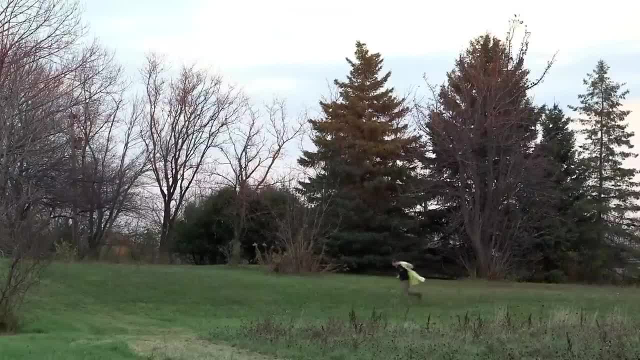 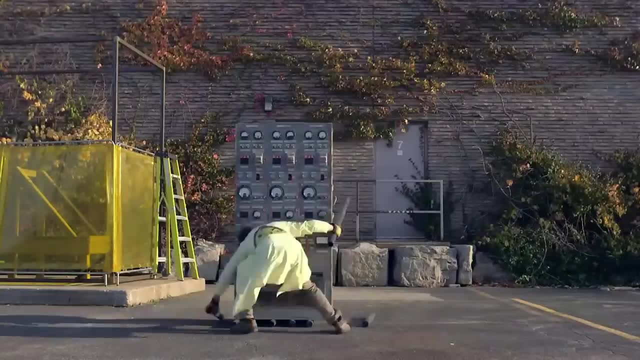 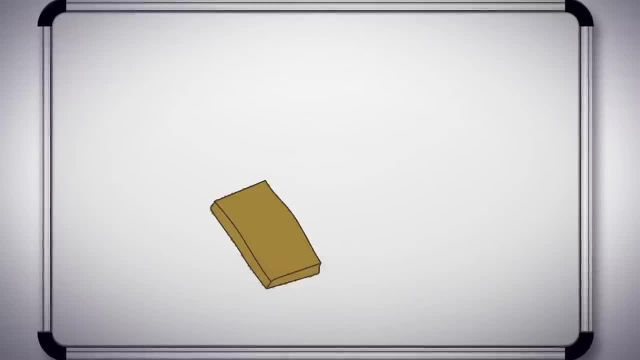 What I need to do is build a ramp that goes from the ground up to the loading dock. Then I need to pull the heavy impulse controller up the ramp. The best way to do that is to use a system of. The best way to do that is to use a system of. 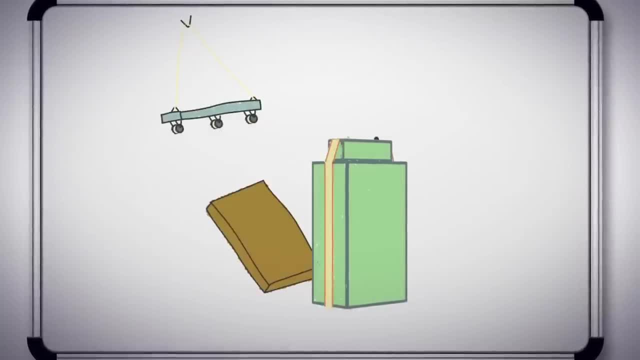 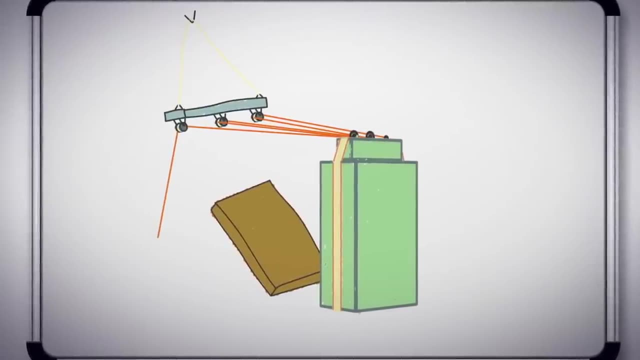 pulleys. I have three pulleys on one end and two pulleys on the controller. Because I have five pulleys working together, I'll only have to lift one-fifth of the weight. The plan is to get it tipped over onto the ramp. 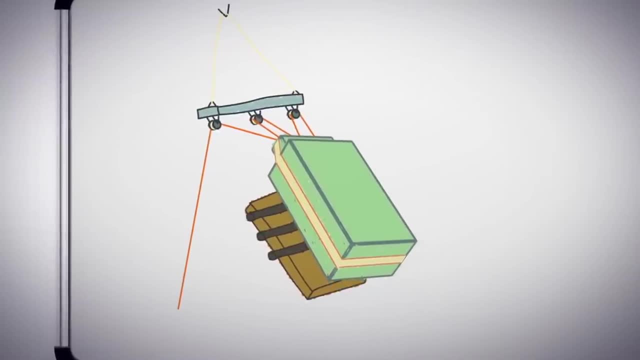 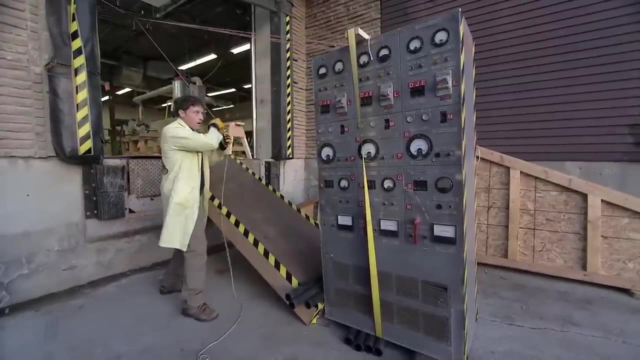 then use rollers to help it roll up as I pull on the rope. There's three pulleys on that piece of wood over there and I got two pulleys on this piece of wood here And now, if I pull and I carefully put the rollers. 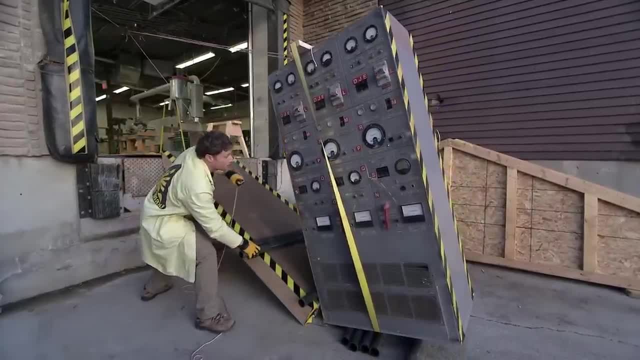 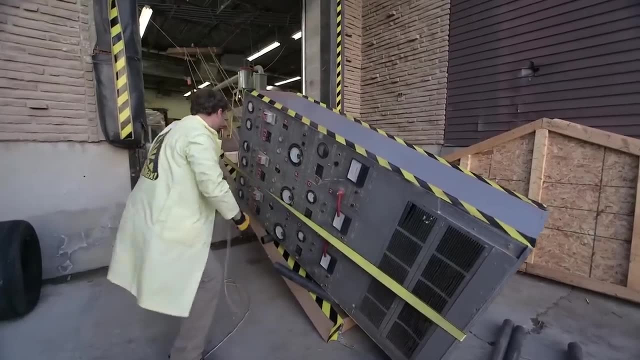 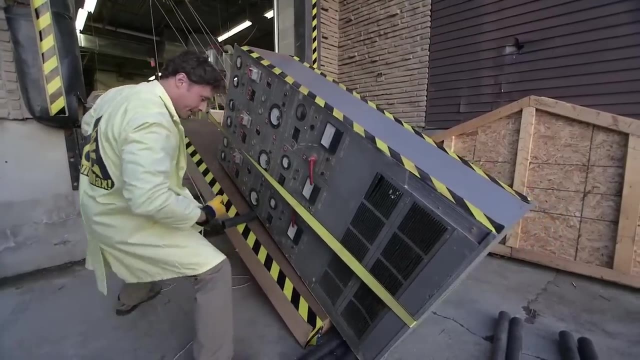 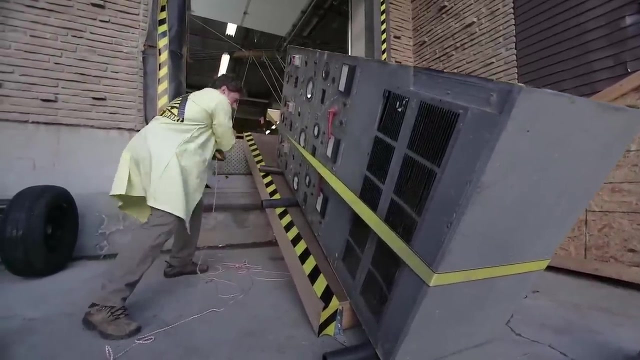 in there Underneath, Careful, Careful, Perfect, OK, Now it's on the rollers And now I can pull it up the ramp. Now I got to carefully put new rollers underneath as I go Pull it up the ramp. 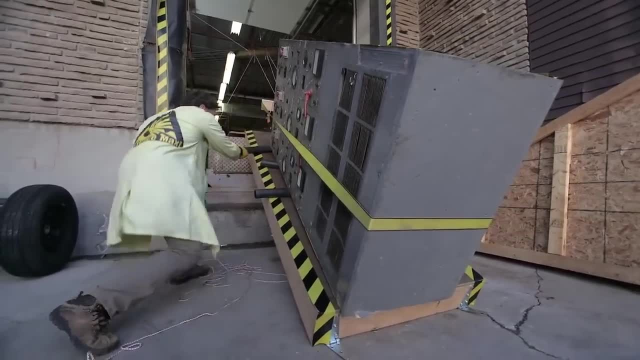 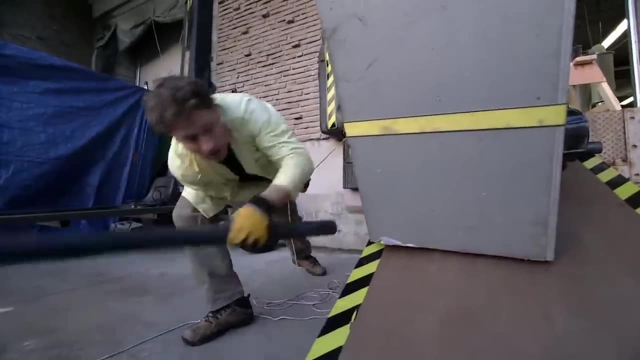 The ramp Roller. I know what you're thinking. It still seems pretty difficult. If only the simple machines could give me longer arms. Well, they can't do that, But what they can do is give me the strength to do this heavy. 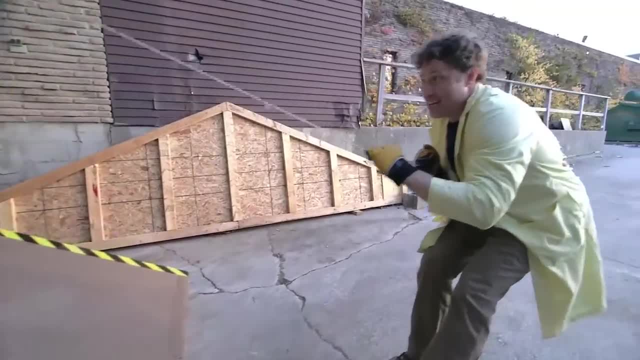 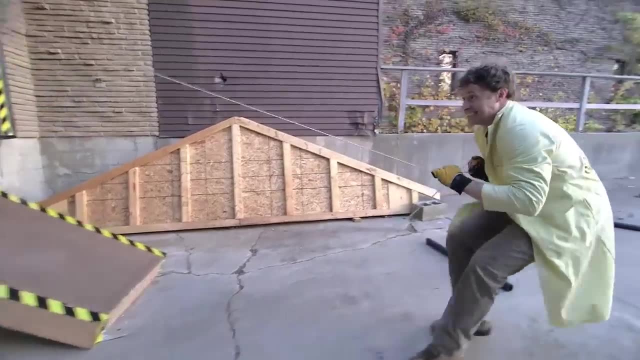 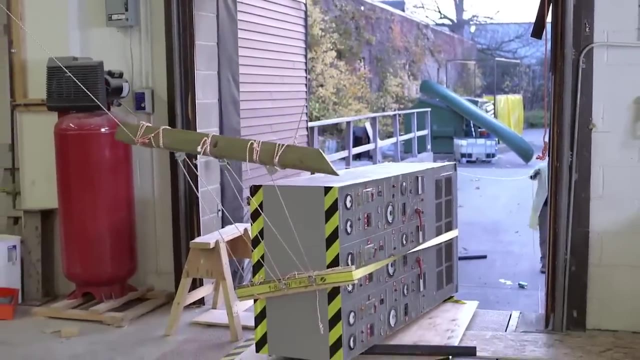 job with no one else around but me. Hopefully that won't be a problem. There we go. I did it All the way across the parking lot and up onto the loading dock with the help of levers, rollers, ramps and pulleys. 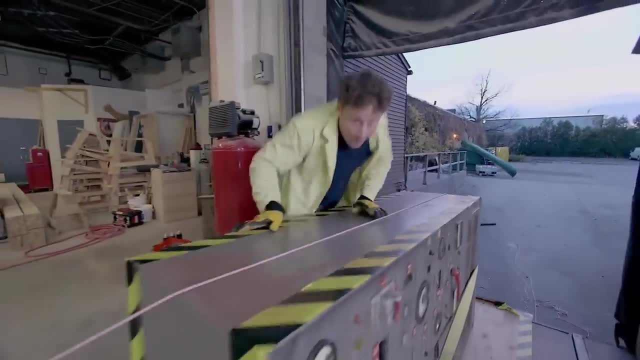 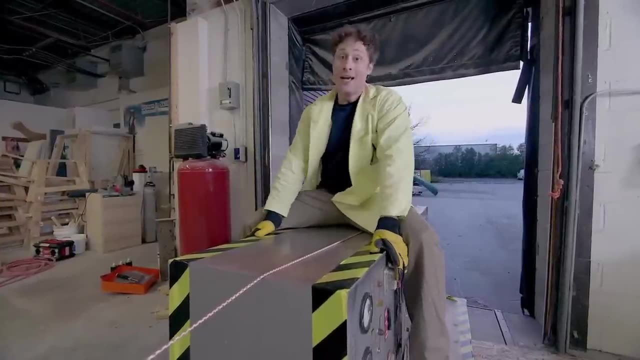 The hard part's done, Now I just have to get it into the lab. All right, Let's see if all that effort was worth the effort. All right, Let's see if all that effort was worth the effort. All right, All right. 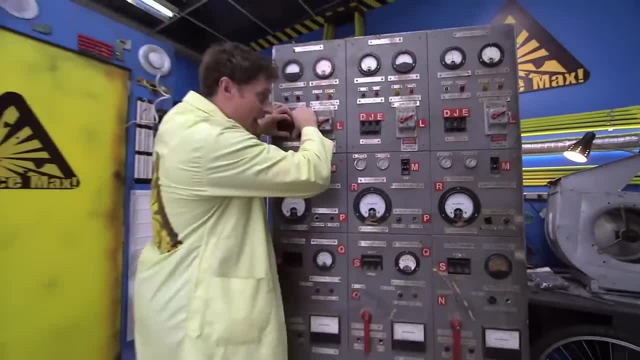 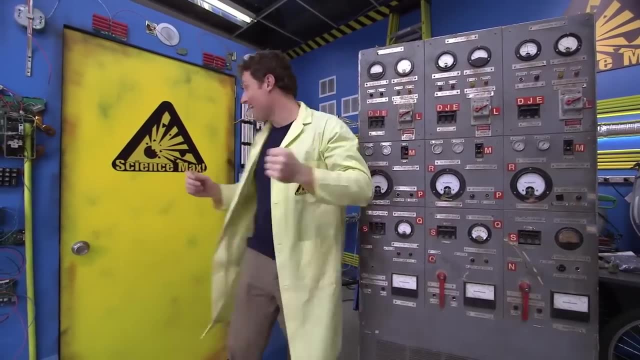 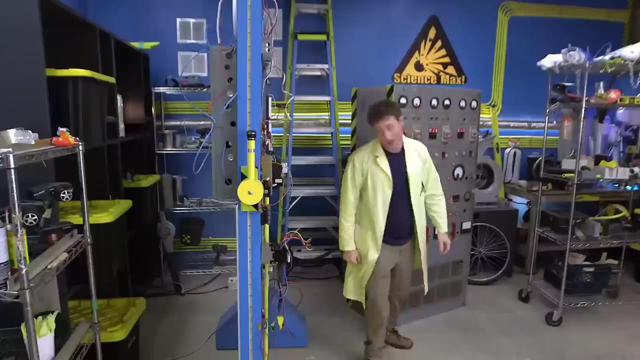 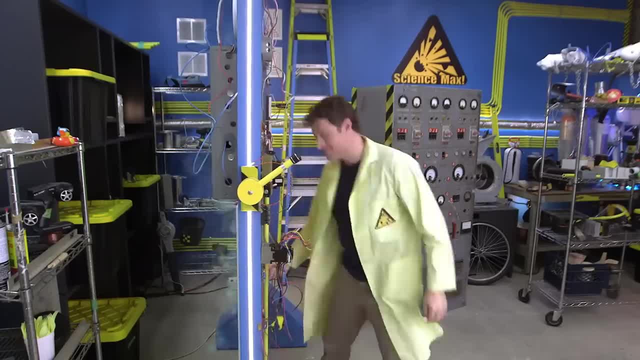 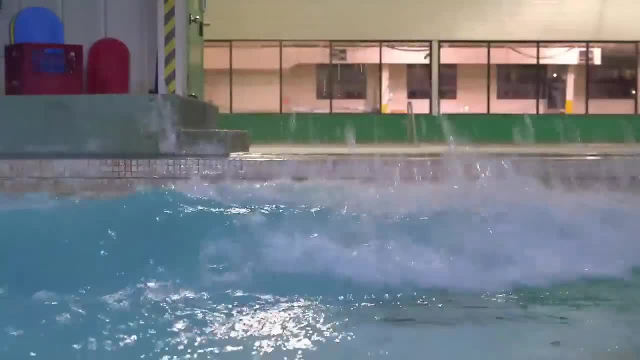 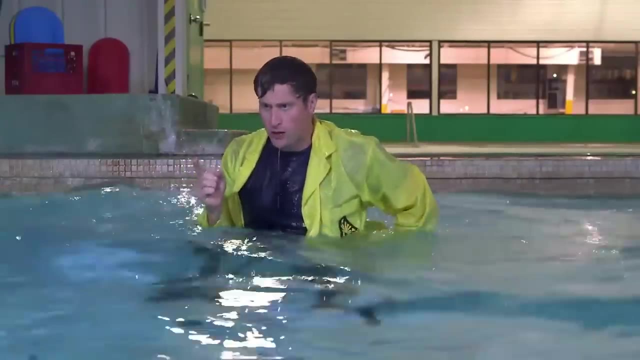 and I could really use the rest. See you next time. Wait, I hit three four one two. I should have hit three four two one. That was my. that was my. that's okay. I'll just go back and um. 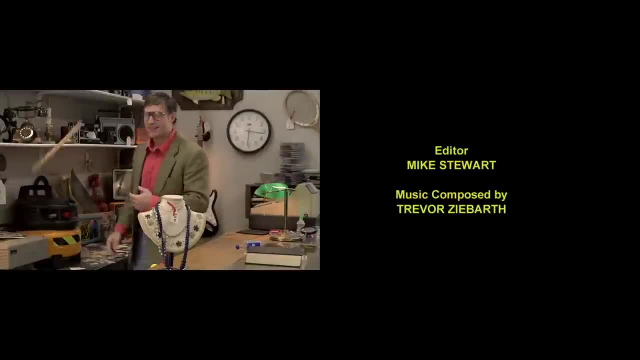 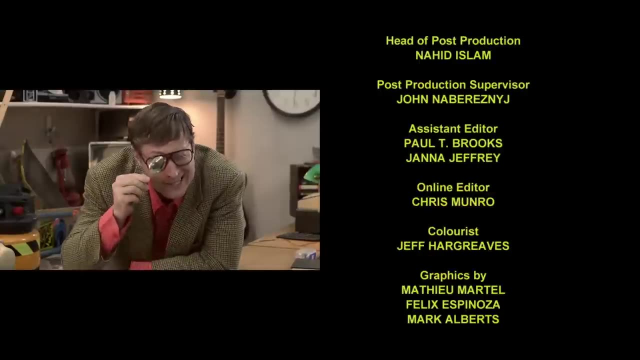 Now, this is a lever. See, it's a catapult and a spoon. It's two things in one. I mean it could also be, you know, it could also be some sort of like. it's like an eye patch. 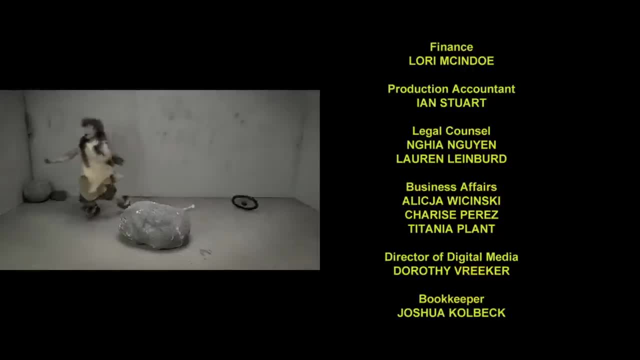 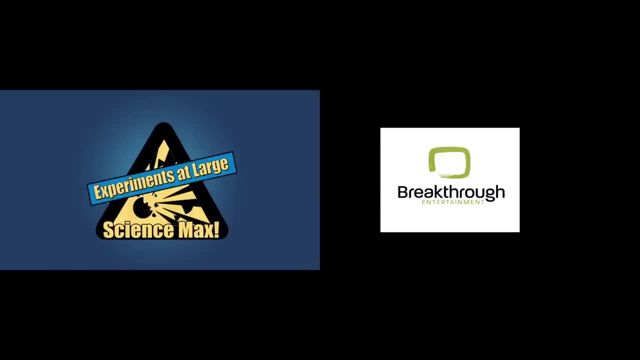 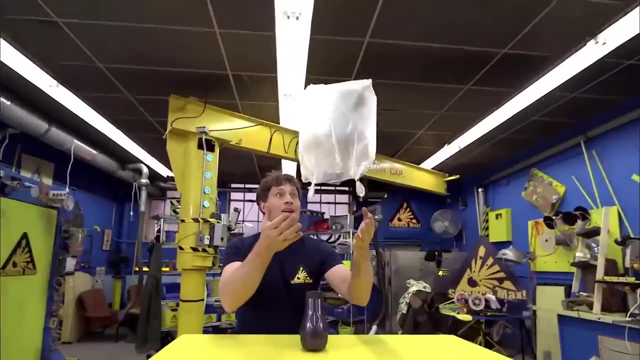 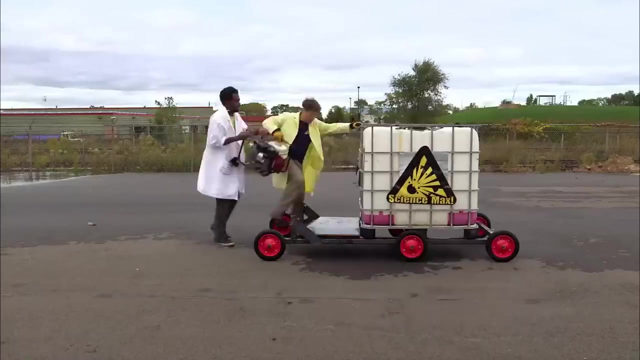 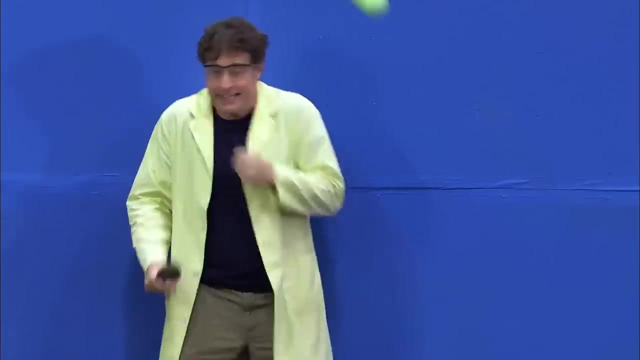 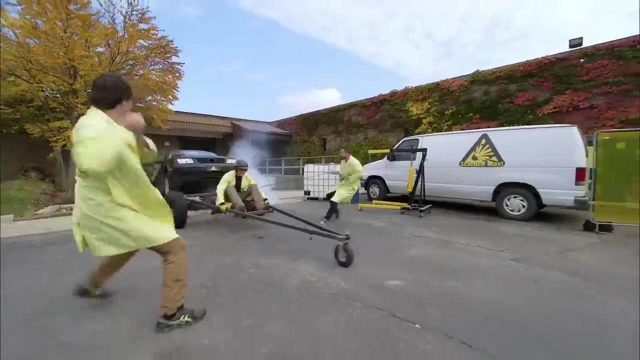 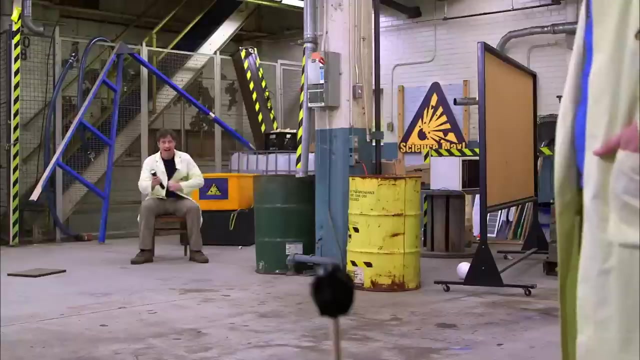 Have you ever done a science experiment and wondered what it'd be like if you did it big? I have. My name is Phil and I take your everyday science experiments and do them big. This is Science Max: Experiments At Large, Science Max. 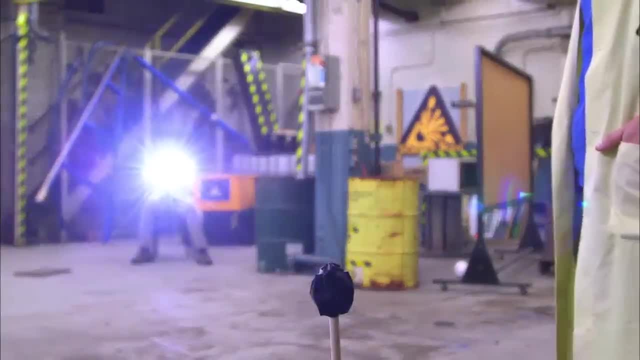 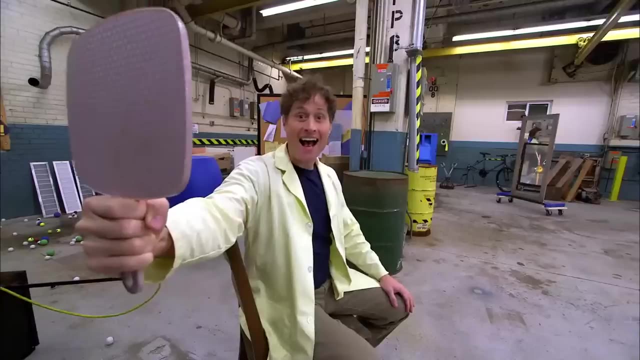 This episode of Science, Max Experiments At Large, is all about light and bending light to your will, Huh huh, right, right, And challenges me to an ever more tricky game of light manipulation Plus lasers, Periscopes- And what does that have to do with light? 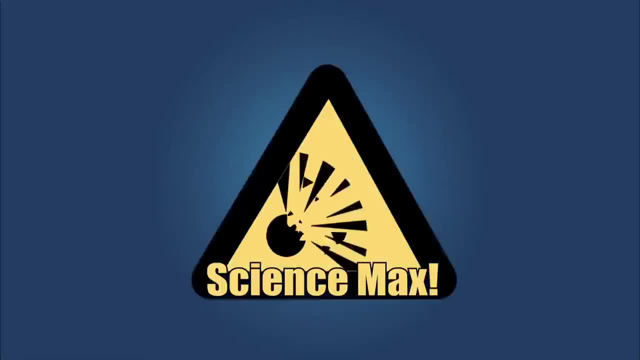 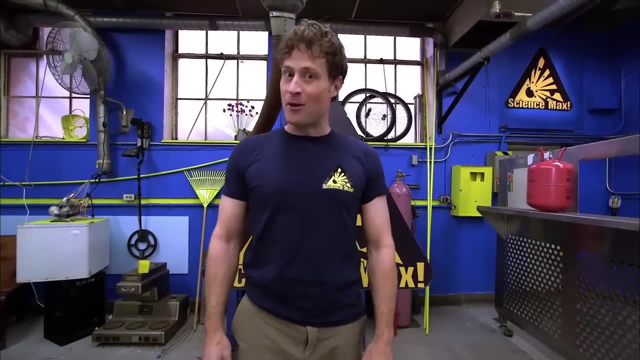 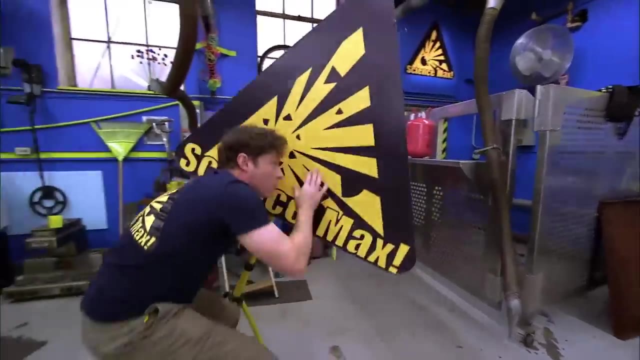 Cut to animation. Find out on Science Max Experiments At Large. Greetings: Science Maximites. I'm Phil, and today, on Science Max Experiments At Large, we're gonna be looking at light. Ah, oh, oh, oh, okay, oh, oh, oh. 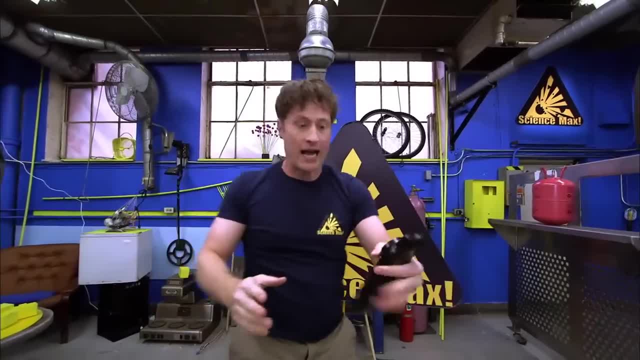 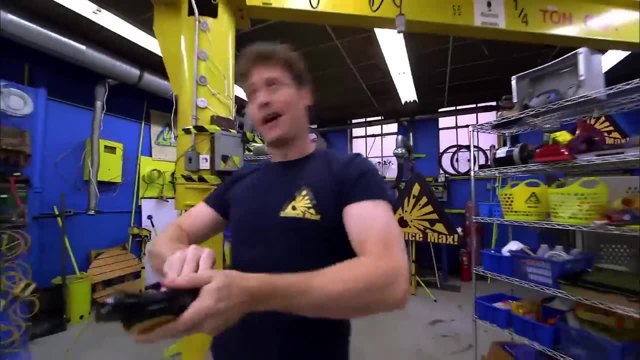 Okay, stay That. that wasn't supposed to happen. I was supposed to press that button and there was supposed to be all these lasers and special effects, But it didn't. Well, today, on Science Max Experiments At Large, we're not gonna be doing one experiment. 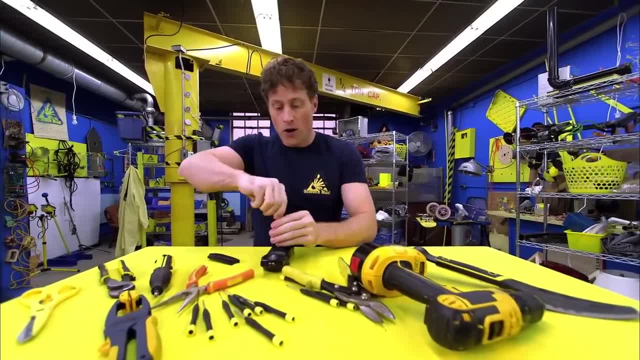 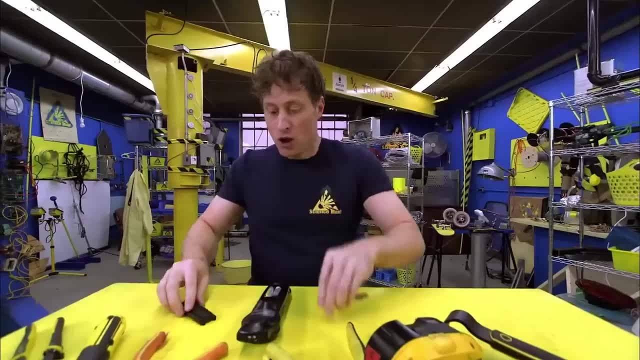 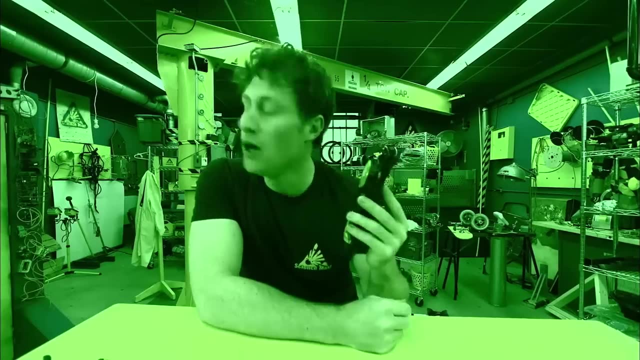 We're gonna be doing a number of small experiments because we are going to do a light manipulation challenge. I'm gonna get an expert and she's going to challenge me to a game of light manipulation, because I am the master of light. Oh. 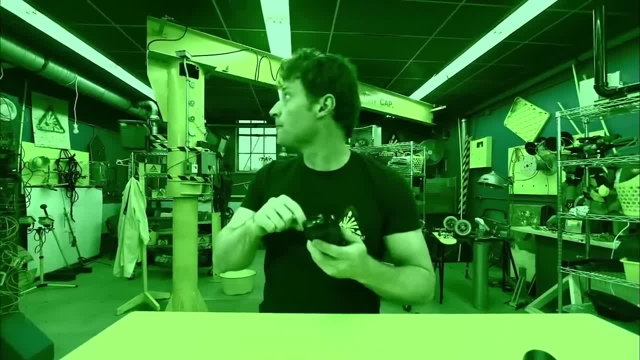 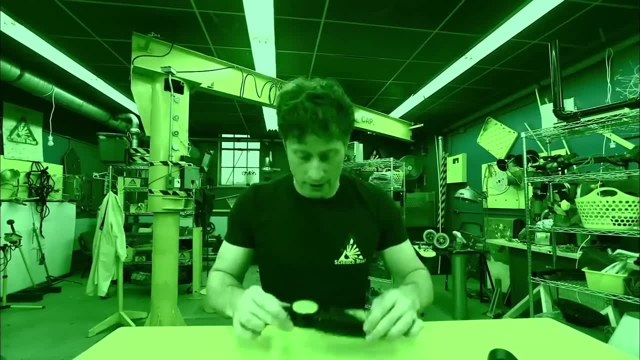 Well, at least the green lights are working And okay, okay, forget it, I'm just gonna turn. I'm just gonna turn it back to normal. Come on, turn back to. I'm gonna work on that. later. I'm gonna need an expert to help me though. 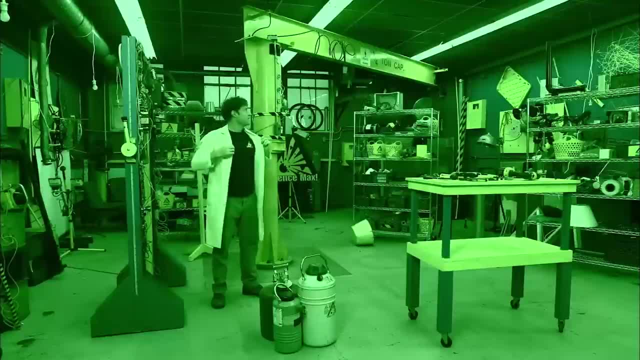 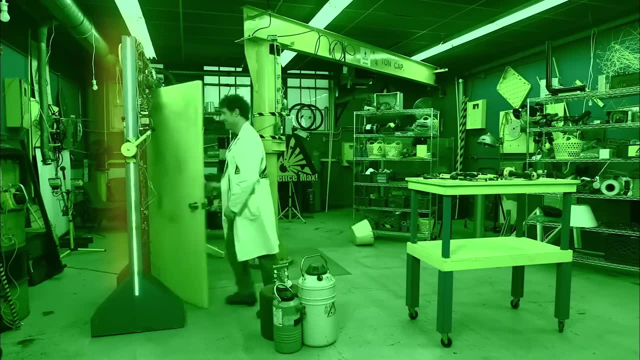 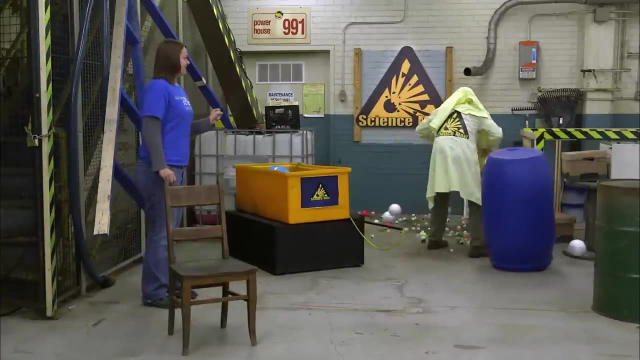 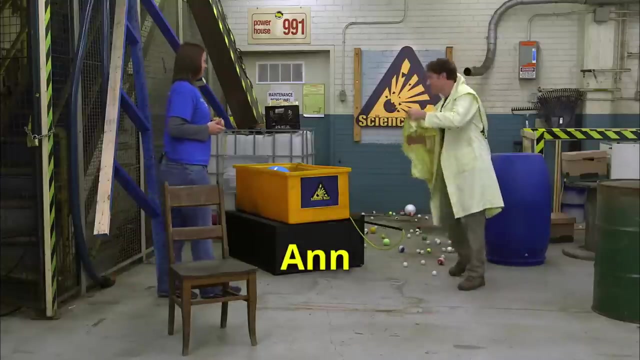 Oh, I know Anne would be really good at this. It really does look kind of weird in here, doesn't it? Oh well, You, okay, Let's go back. Hi Hi Phil. Yeah, I didn't, I couldn't see what I was doing. 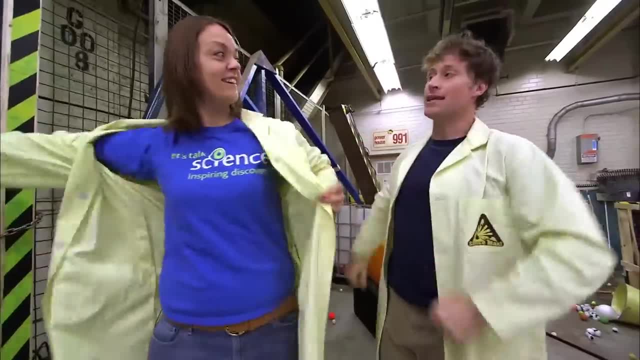 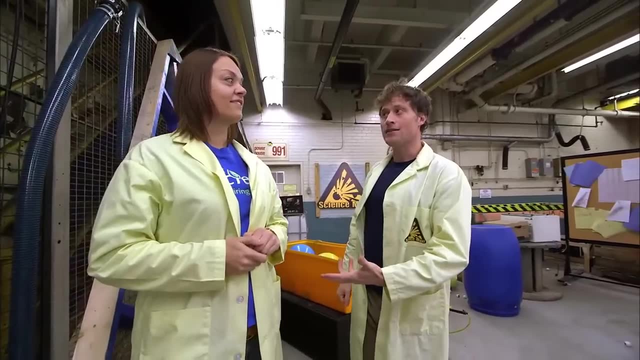 Here's your lab coat. Oh, Thank you for coming. Great, Now you're from. Let's Talk Science, right? Yeah, that's right. All about science, education, just like us. Now you're gonna challenge me to a light manipulation game. 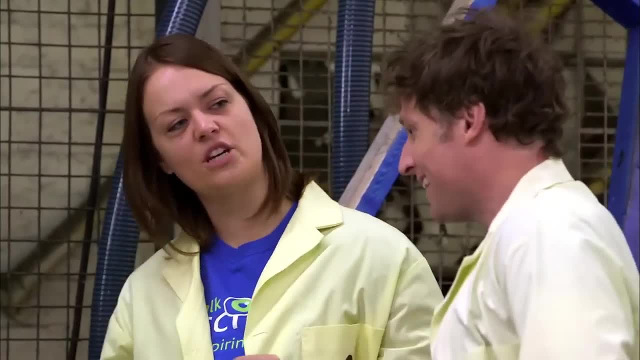 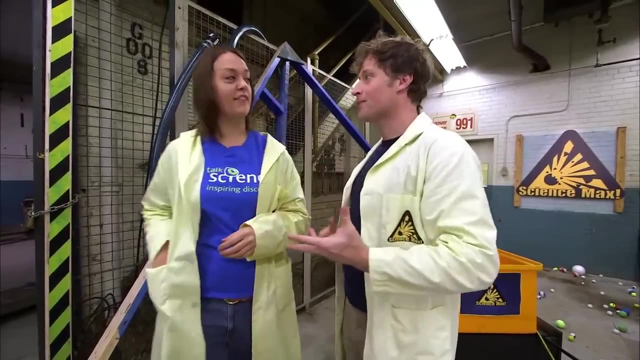 A light manipulation game. I've been working on a series of challenges since last time we talked Awesome, Each a little more difficult than the last. Well, this is gonna be great because I am the light manipulation master. Okay, well, we'll see about that. 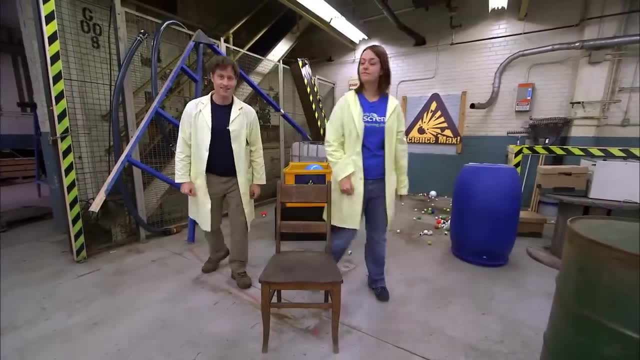 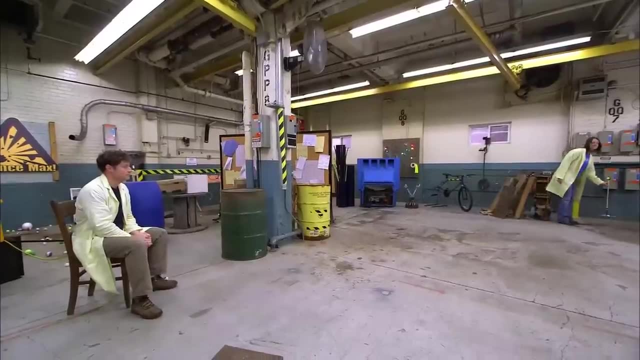 Okay, Number one, Take a seat. Oh, that's easy enough. I have written something on the back side of this ball, Okay, And I'm gonna challenge you to read it. Okay. well, I'm ready. I might be able to read it from here. 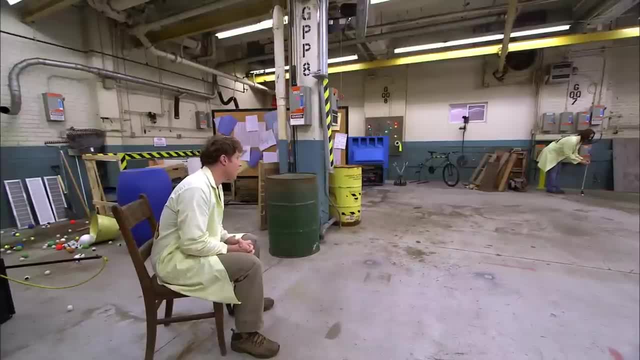 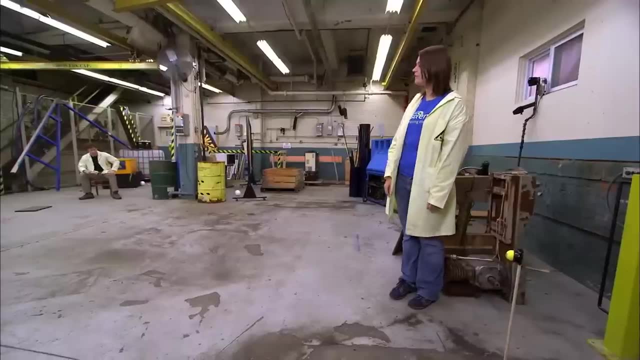 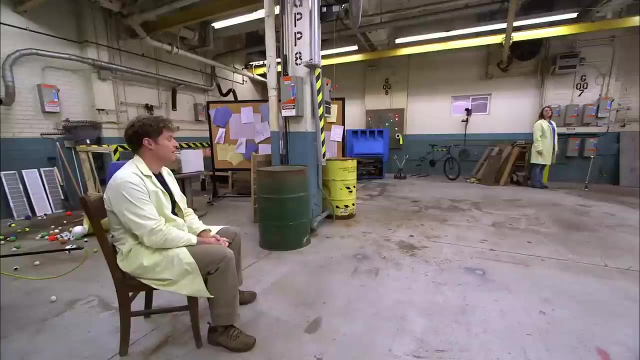 Let's see. All right. Okay, I see something's written on it, but I can't read what it says. What if you squint? It looks like a couple lines, maybe. I can't quite tell Any ideas how to solve this challenge, Phil. 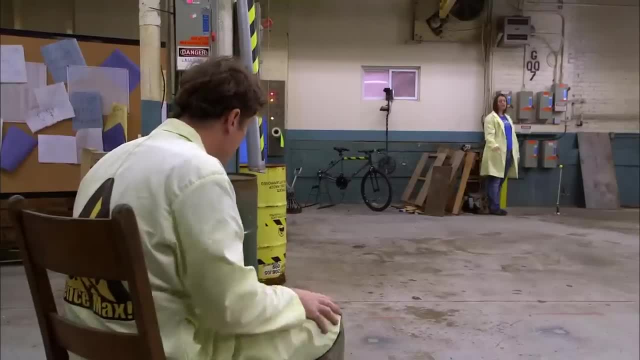 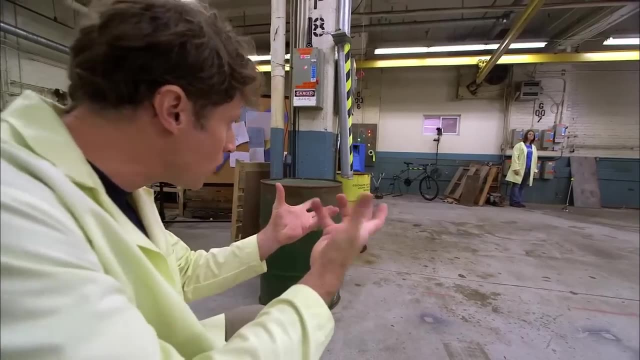 Um, and I have to be in this chair. Well, you can get out of the chair to set up your solution, Okay, But when you read what I've written on the ball, you have to be sitting in the chair. Well, it's light manipulation, right? 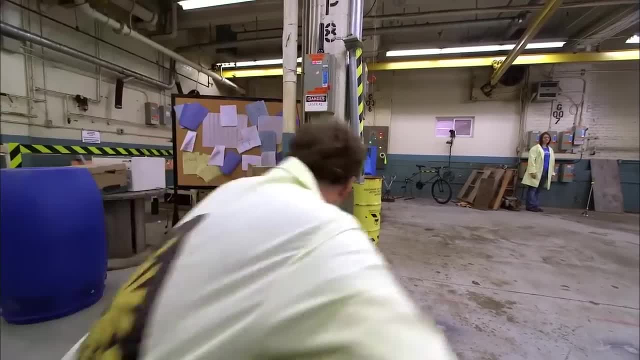 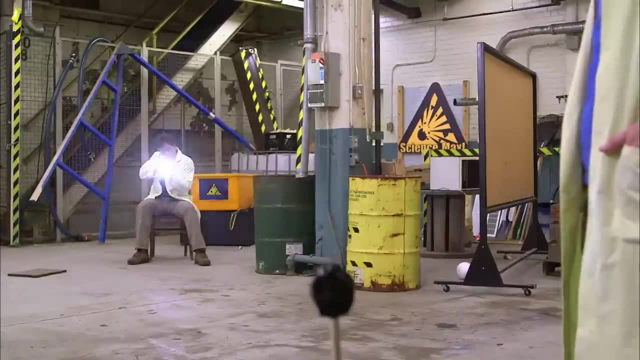 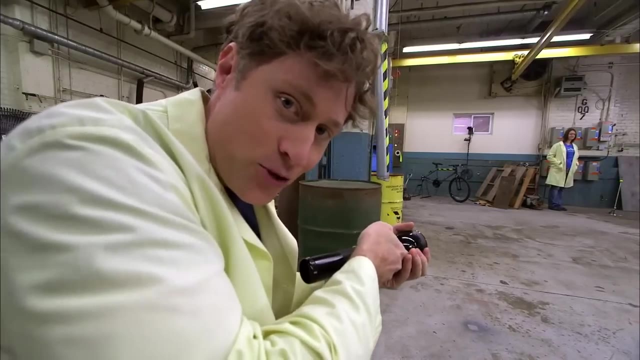 Mm-hmm, So I Wait a minute. I've got flashlights in case the power goes out, so maybe I can use a flashlight. Ha-ha, Okay, ready, Pew. Um Huh, Doesn't seem to make it any easier to read. 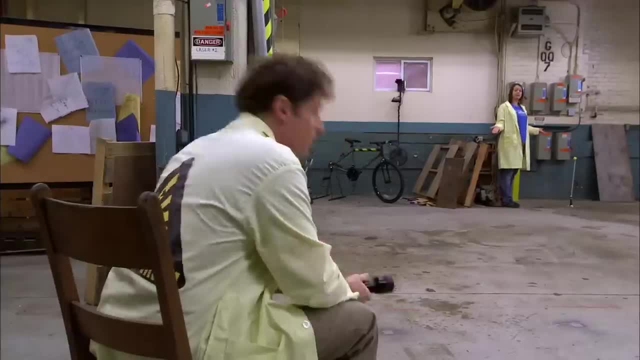 Yeah, I got nothing. Do you give up already? No, Of course I don't give up. I told you these were going to be challenging. This is nothing. I will figure this out. Um, I don't know yet. You're going to have to get creative. 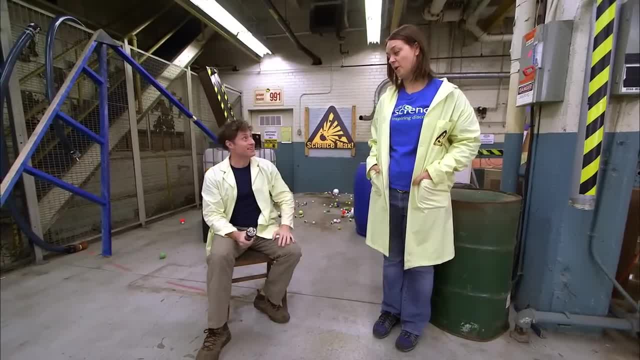 I don't know yet, but I will think of something, Okay. Okay, I will be back Here. hold the flashlight, Not looking, not looking. I'm going to go this way. I'm going to wait right here, Okay. 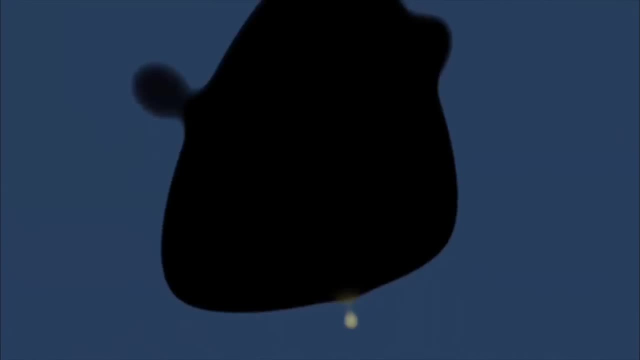 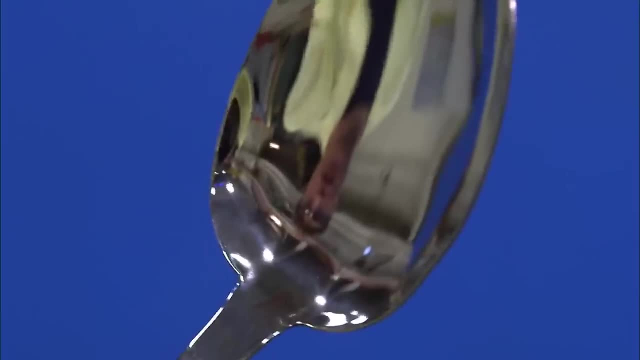 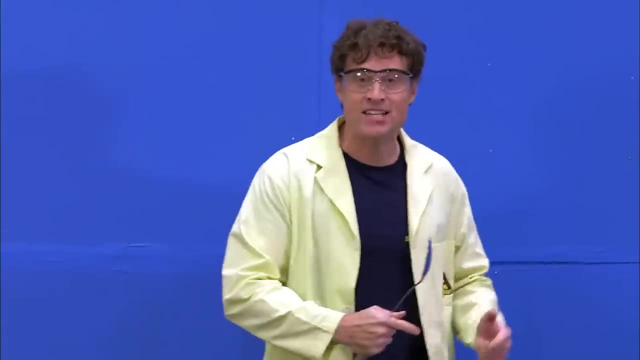 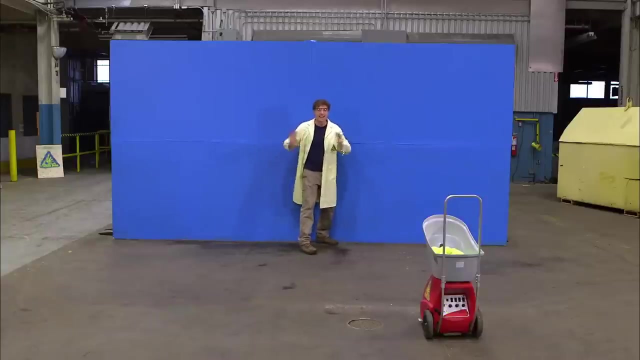 Have you ever wondered why you end up upside down when you look at yourself in a spoon? It's because of light reflection. Light is made of photons. Let's say that these tennis balls bouncing off this wall are photons of light. Now, when the surface is flat like a mirror, 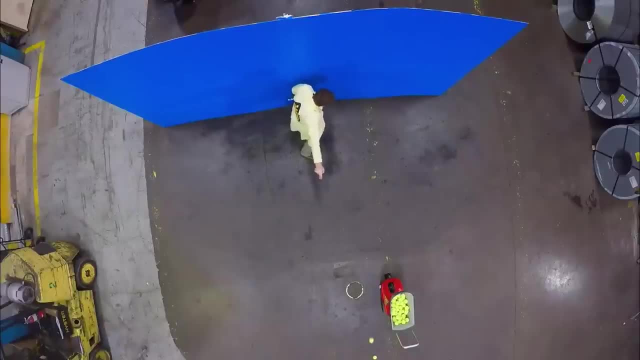 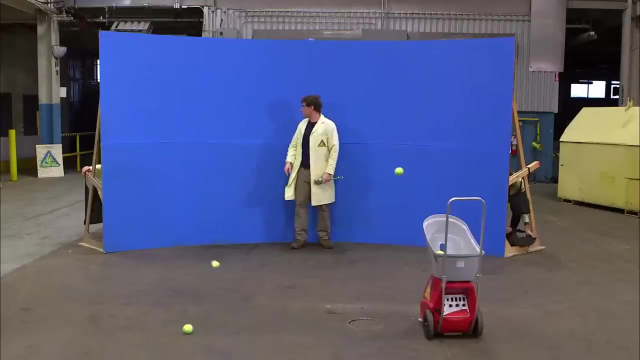 the photons, they bounce in and straight back out again. But when the surface is curved the photons don't go straight out, they get reflected. So now this photon is going over there, and if we had photons on this side they would. 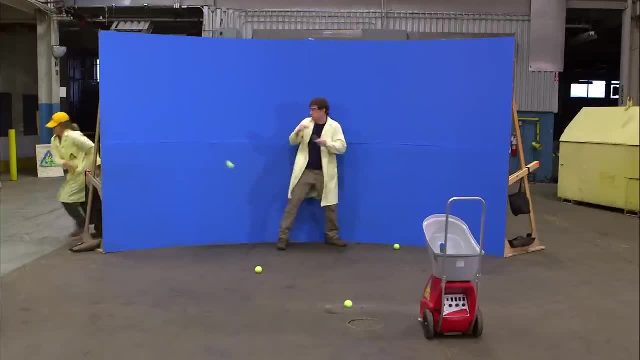 I don't even know where those ones are coming from. Then, okay, so we got. we got photons on this side that are going that way and photons on that side that are going this way. so the top becomes the bottom and the bottom becomes the top, and that's why you look. 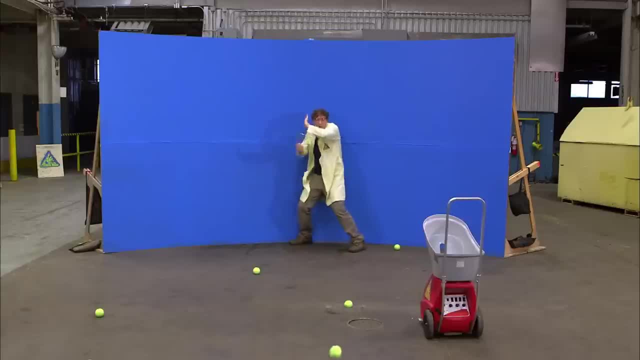 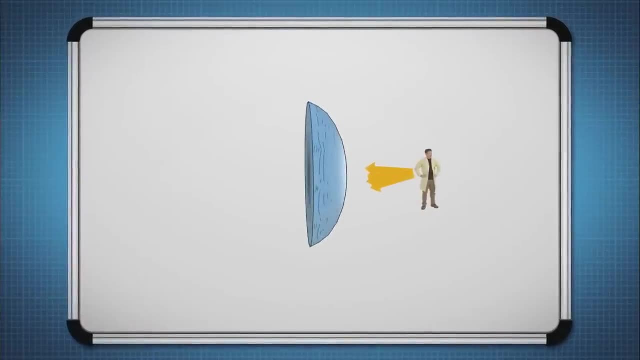 upside down when you look at yourself in a spoon. Okay, cut to animation. cut to animation. A lens works by changing the direction of light too. Lenses are made out of curved pieces of glass. When the photons of light pass through the glass, 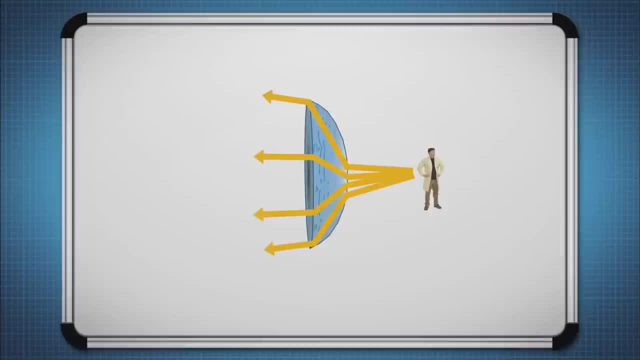 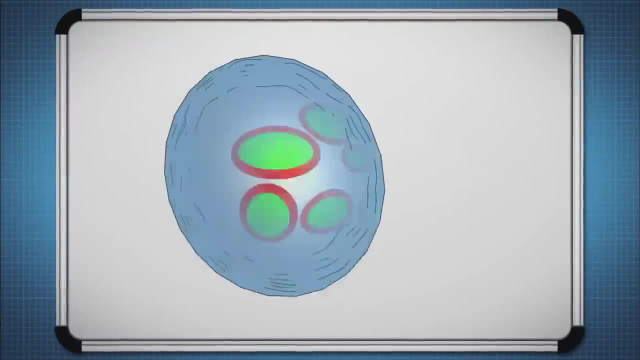 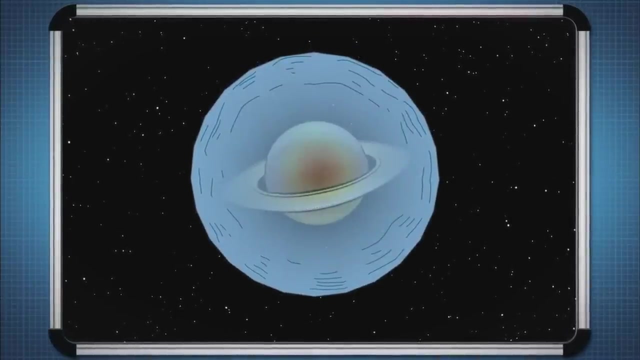 the curved surface makes their paths change. What was only this big before becomes this big when you see it. Lenses are used in microscopes to see things that are really small, or in telescopes to see things that are very far away. Both times, they are making something small appear large. 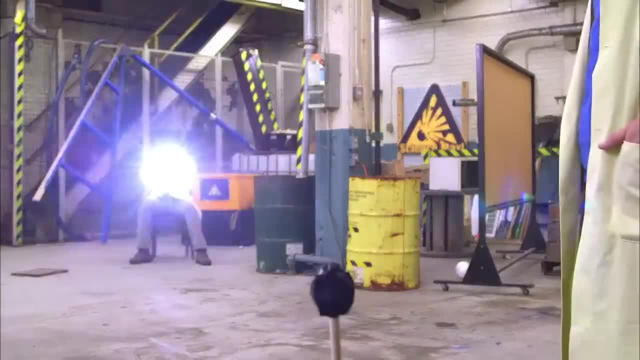 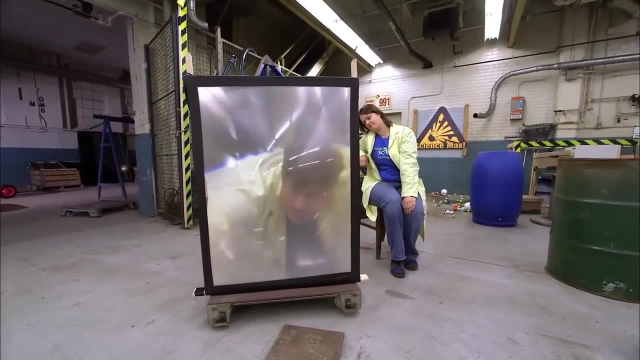 Ann has challenged me to figure out how to see a small object far away, and using a lens is my solution. Check it out: It's a giant magnifying lens and I'm going to use it to magnify the ball so that I can see it. 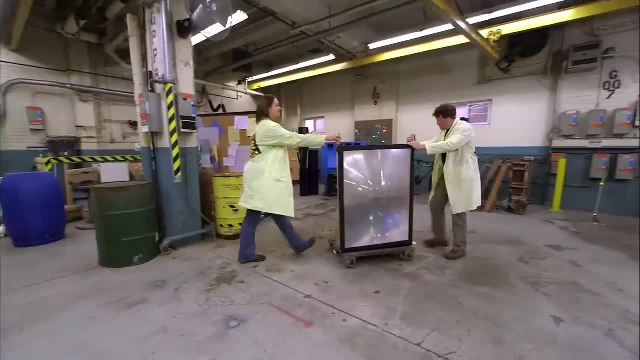 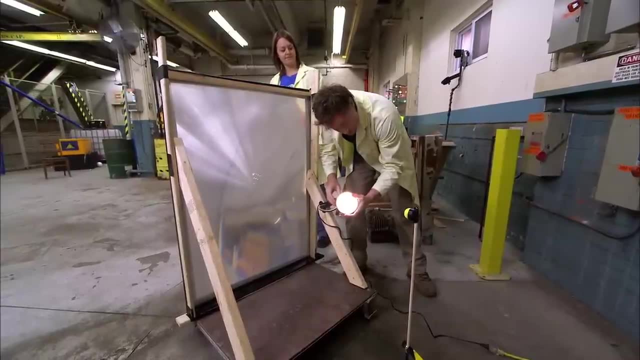 Sounds great. All right, I set the lens in front of the ball, which Ann has turned, so I can't see what's on it. I add a light. I'm going to shine it on the ball so that it's a little bit better illuminated. 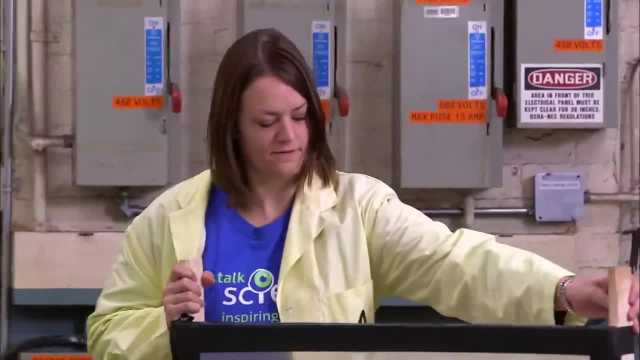 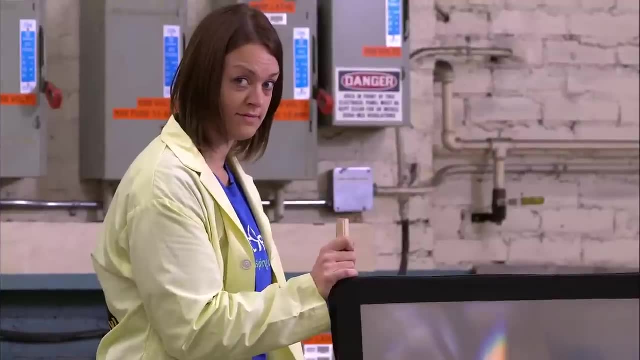 And then sit in the chair and ask Ann to move it. so it's aligned All right. so bring it to your left. Yeah, keep going, keep going, All right, Keep going. Right about there. Try bringing it closer to the ball. 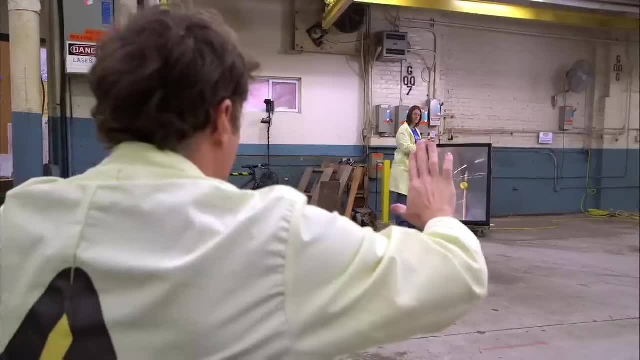 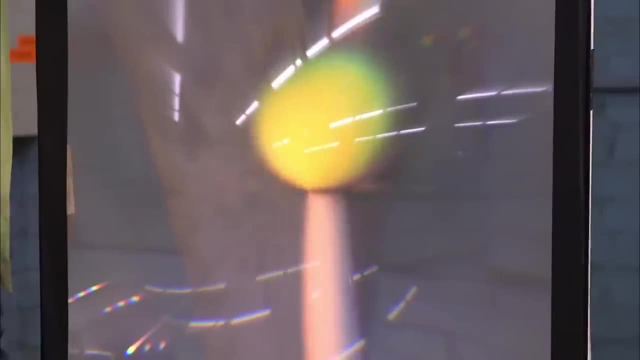 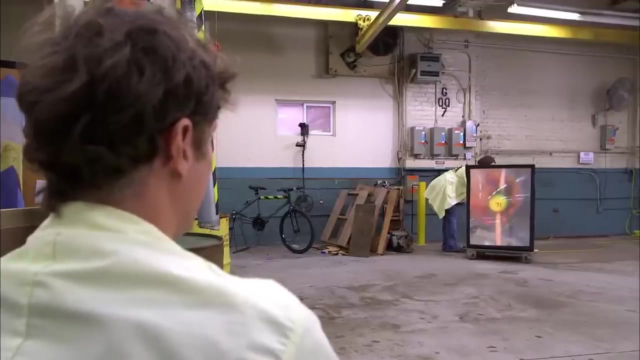 Okay, wait, That makes it smaller. Try going, bring the lens away from the ball. Ooh, Wait, Try a little bit further. Ooh, You're ready for me to spin the ball around? Yep, Okay, It says 71.. 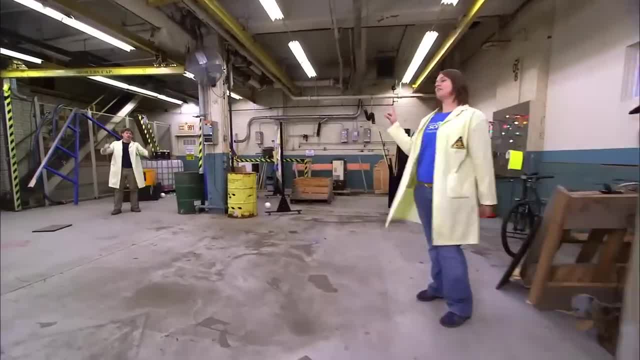 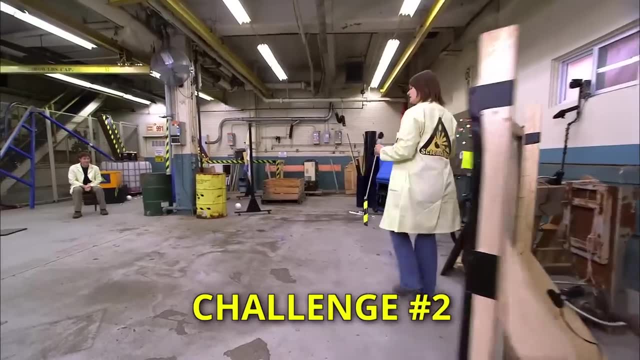 Nicely done, Easy Solved. Wait, wait, wait, What? That was just the warm-up. Oh yeah, Yep, You ready for challenge number two? Challenge number two: I've got another ball. Okay, There's something else written on it. 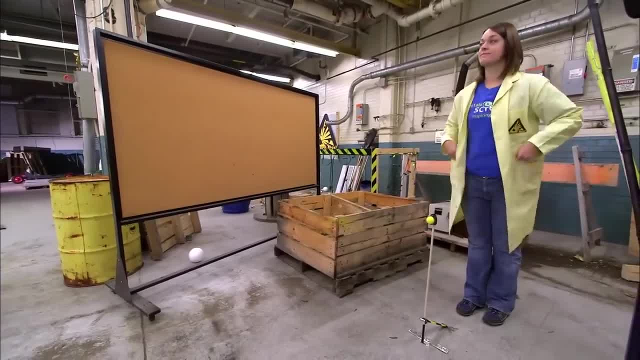 Wait, Are you coming back? Nope, Huh, But I can't even see you from here. Like, how am I? Huh, You're going to have to manipulate the light. I have to see around a corner. I have to see around a corner. 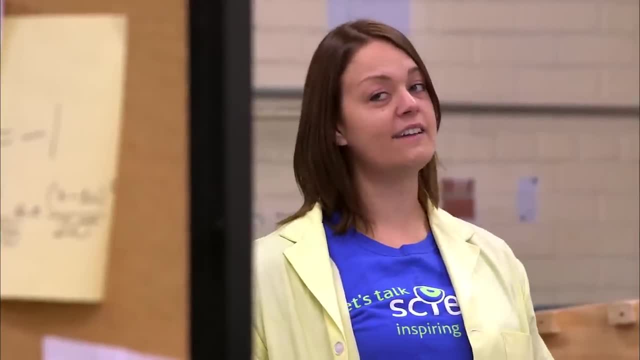 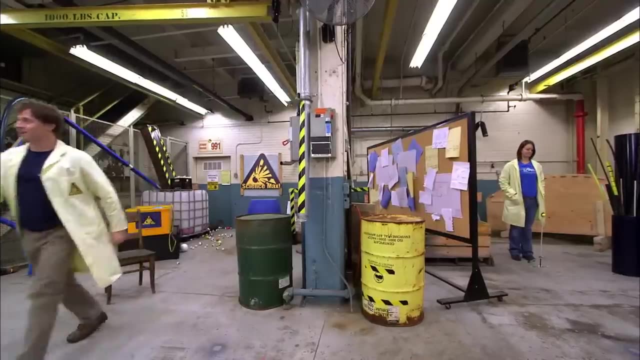 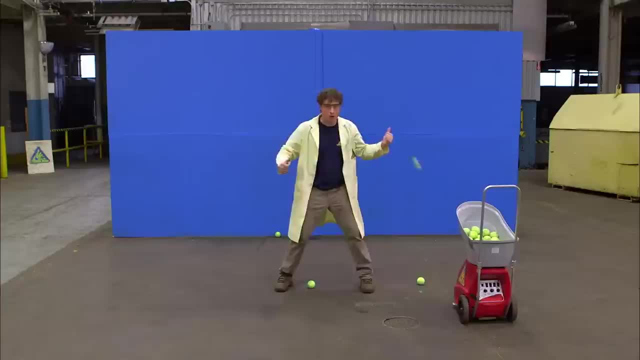 So you remember the tennis balls in the wall, right, Right, Okay, So the tennis balls are photons, What light is made out of? And the wall is a mirror. Now, right now, the photons are hitting the mirror and bouncing directly back. but what? 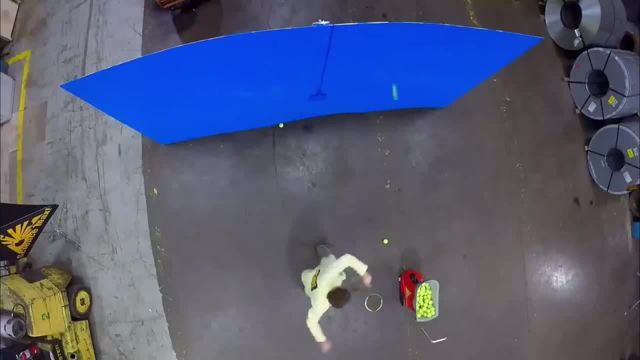 happens if they come in at an angle like this. Aha, Those photons are reflecting off the mirror and going that way, which means that the photo is reflected to the mirror at an angle of the ball, So I can get some picture of the ball. 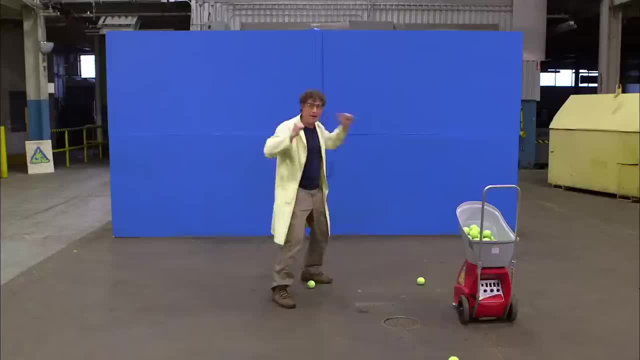 I can get some picture of the ball. All right, I think I got it. So while we wait, let's go to the wall. Let's see what the ball does. Yeah, Let's see what it's like. Huh. 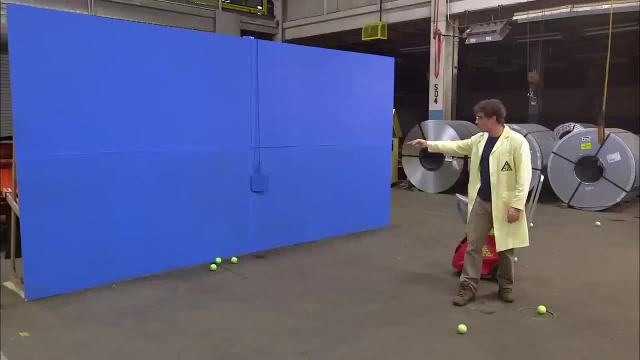 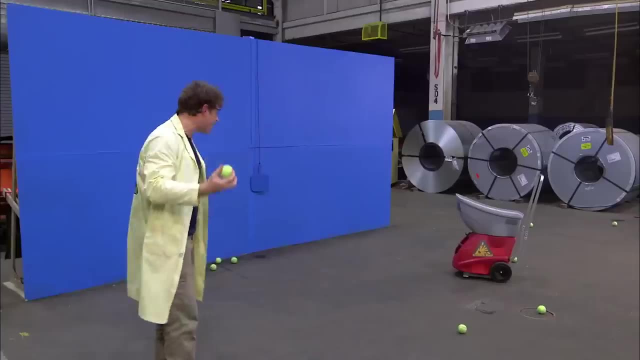 Oh, Aha, those photons are reflecting off the mirror and going that way, which means if I want to see what's emitting those photons, I can see it from here. The same thing happens when you look in a mirror. Okay, mirror. 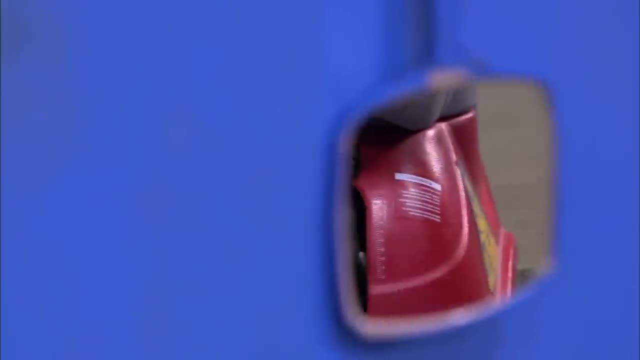 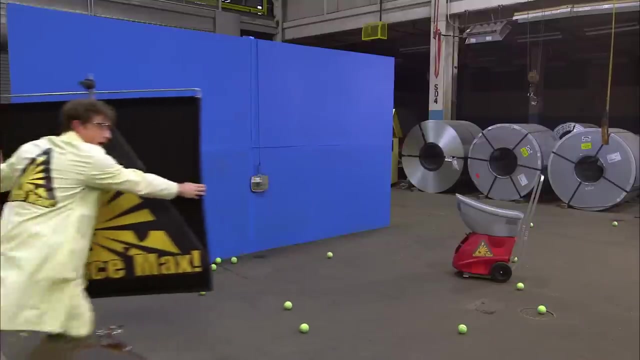 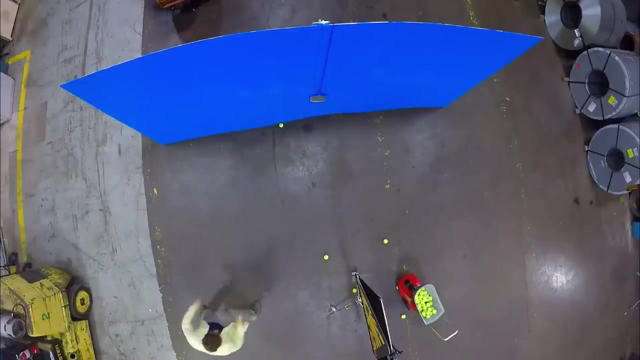 The mirror reflects the photons. over here I can see the tennis ball launcher in the mirror, which means if there was a barrier well between me and the tennis ball launcher, I can still use a mirror and the photons would reflect off the mirror. 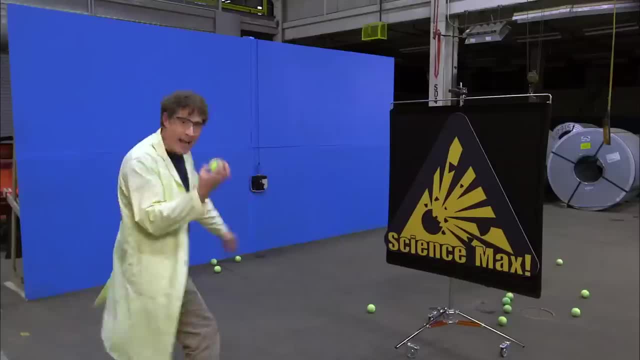 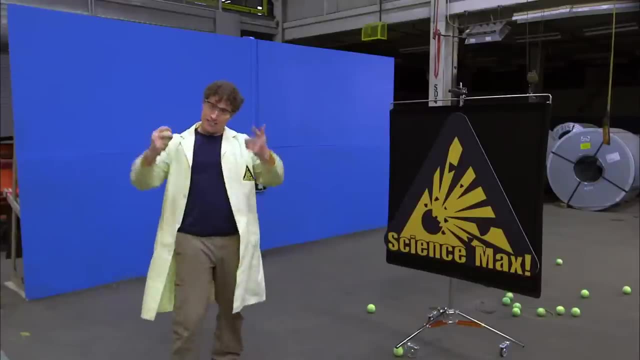 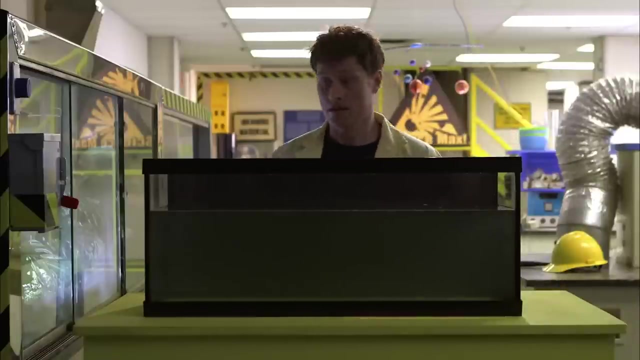 and it comes straight to me, which is how you can use a mirror to see around a corner. In fact, periscopes work the same way. Let's make a periscope right now. See, hey, it's dark in here. 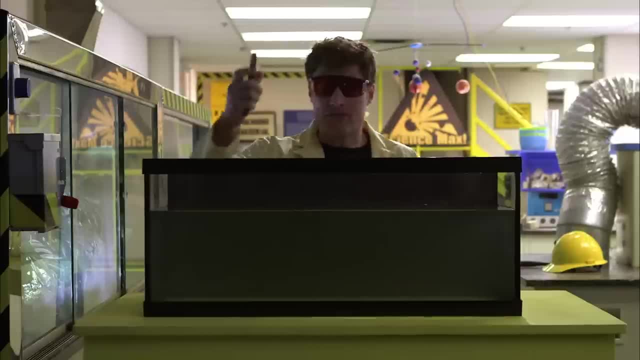 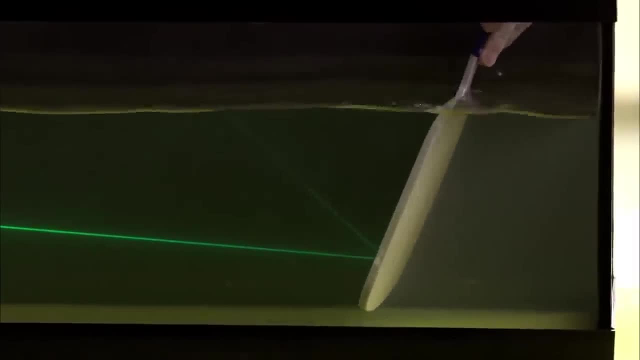 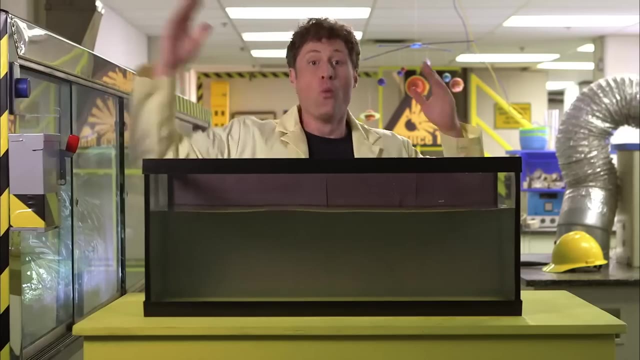 Oh right, because I'm going to show you my laser. So the light from my laser bounces off this mirror in a straight line Ha-ha reflection. We can use the power of reflection to make the light go where we want it to. 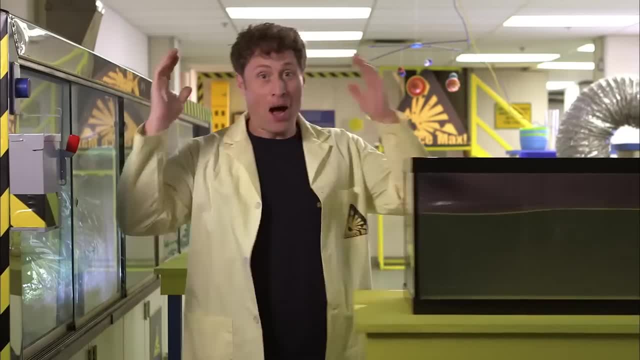 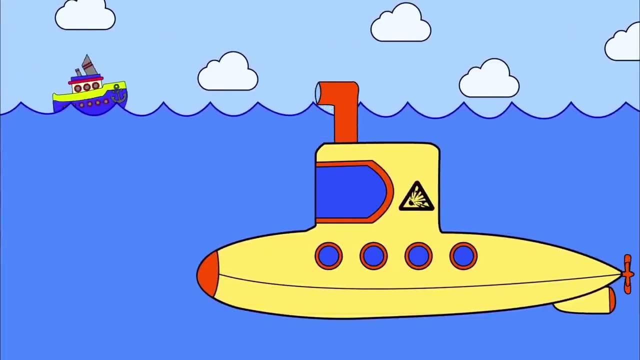 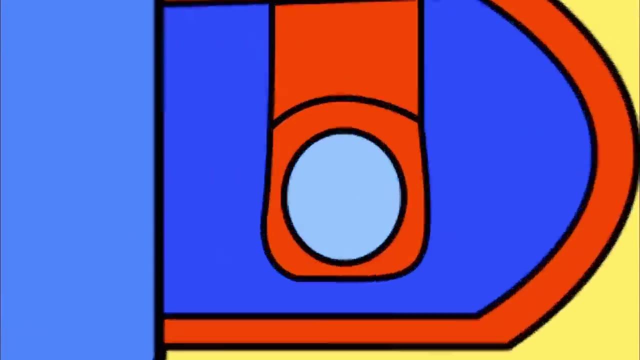 We're gonna. we're gonna build a periscope. Submarines use periscopes because it's hard to see when you're underwater. A submarine will extend a periscope up above the water. The image up here gets transmitted down here, so someone looking through the periscope. 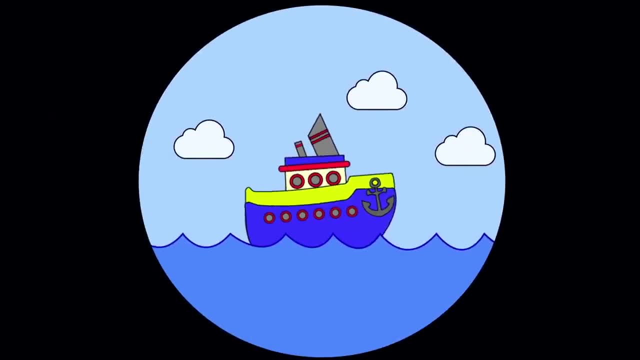 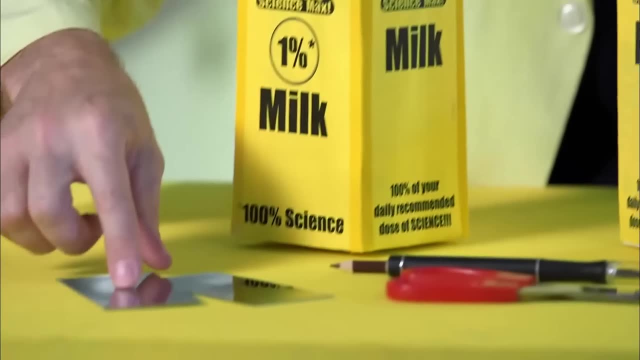 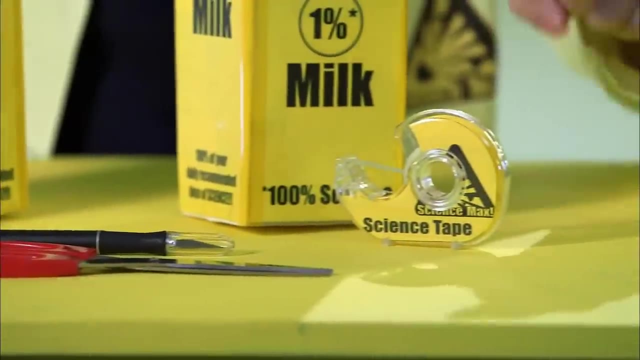 underwater can see what's going on up on the surface. And here's what you need to build it: Two cartons of milk, two small hand mirrors, scissors or a craft knife, a pencil and science tape which is the same as regular tape. 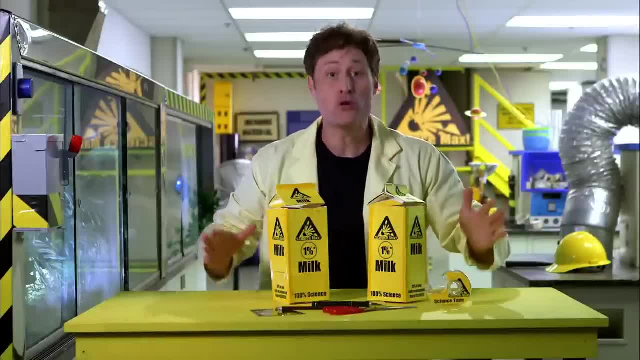 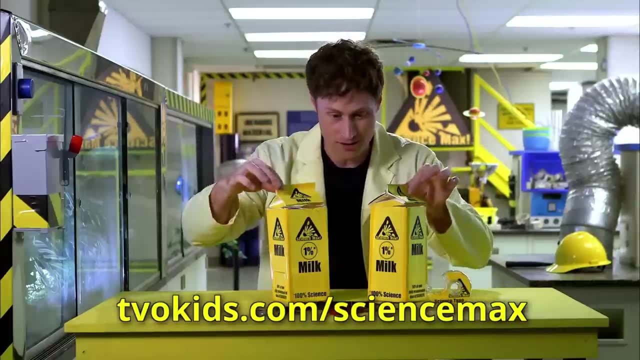 except you use it for science. And remember, if I go too fast, you can always find these instructions on our website. Step one: cut the top off, The top's off your milk cartons. Take your mirror and trace out a rectangle. 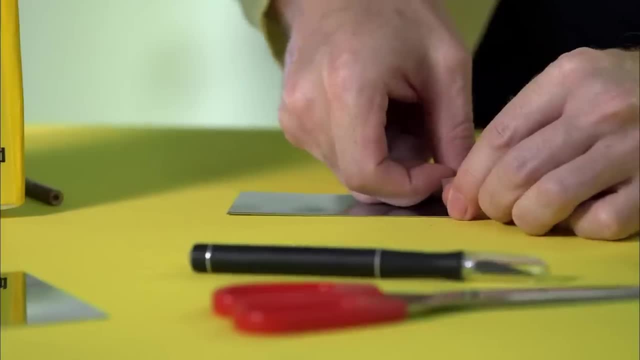 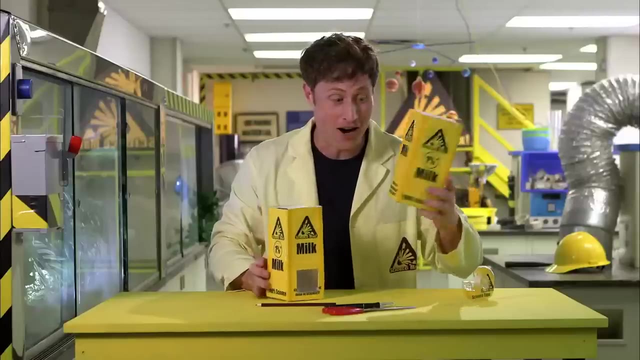 as wide as the mirror, then cut it out. Put some science tape on your mirror and stick it in the carton at an angle. Then put a piece of tape on the inside. Then get the other milk carton and do the same thing. 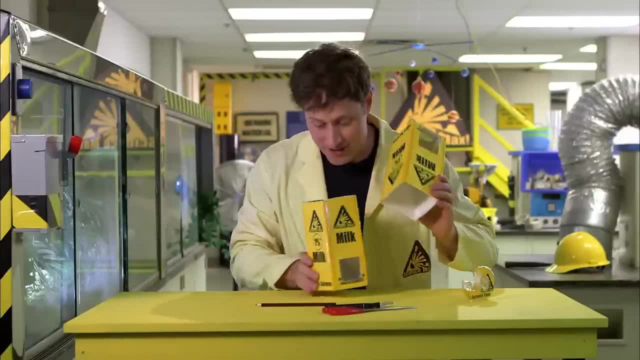 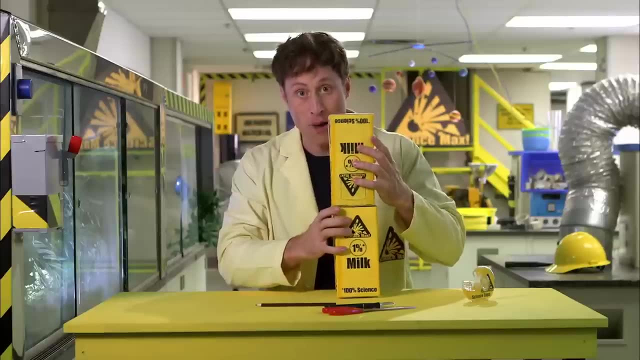 Put a mirror on the inside and then stack the milk cartons together, But don't stack them with the holes on the same side. Make sure you stack them with the holes on opposite sides. And here it is. Here is what's going on inside. 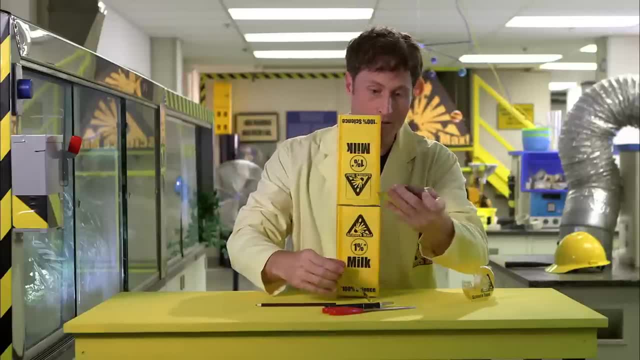 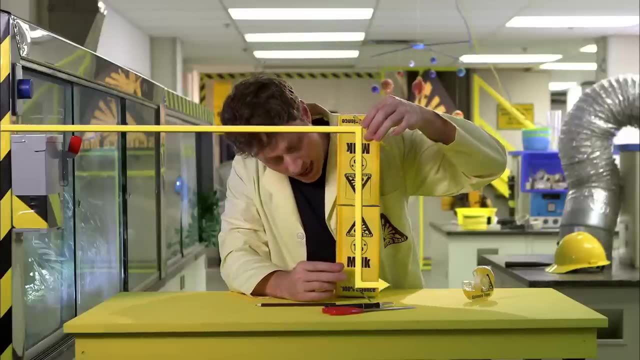 You've got your two mirrors, and one is angled like that and the other one is angled like this Light, from what you're looking at, comes in, hits that first mirror, goes down to that second mirror and goes to your eye. 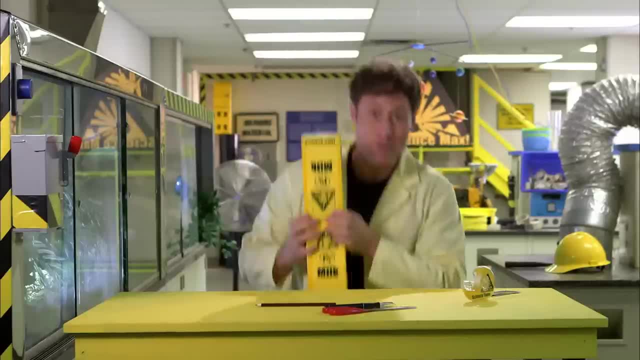 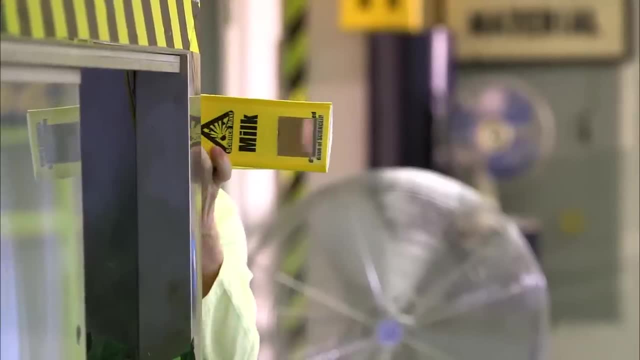 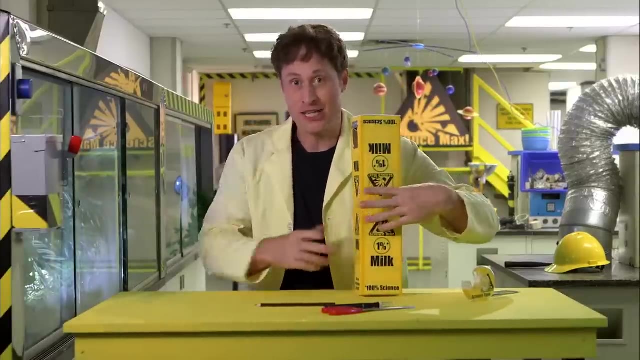 You can use it to spy on people from below the table- Beep, Ha, ha, ha, ha ha- Or from around corners, Beep, Beep. So there you go, Your very own periscope using light reflection. 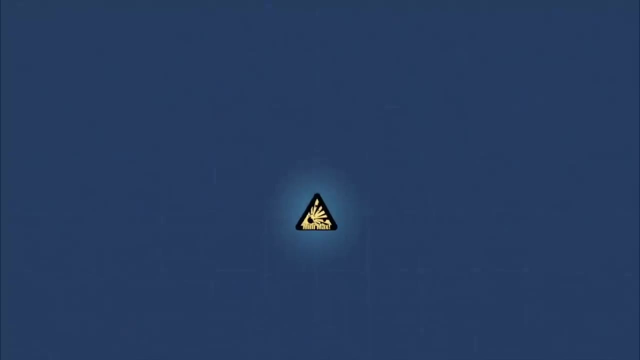 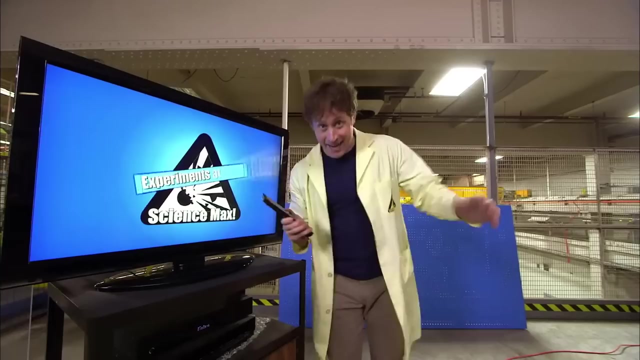 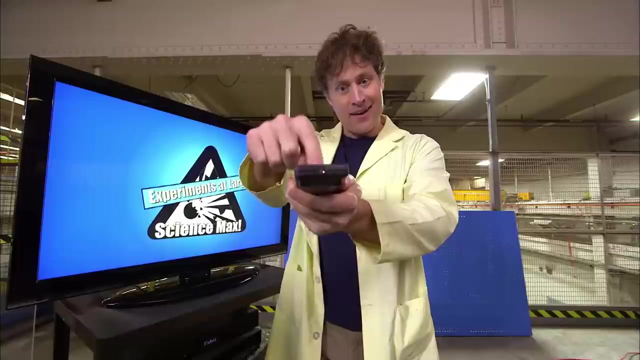 Did you know that your TV remote can be a flashlight? It's true, If you have the kind of TV remote with a little bulb on the end of it, then when you press the buttons, the bulb lights up. Yeah, I know what you're thinking. 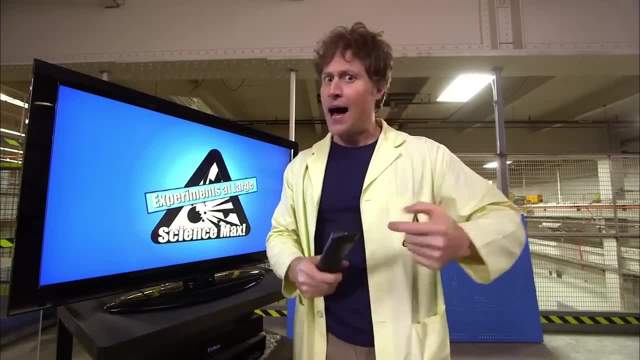 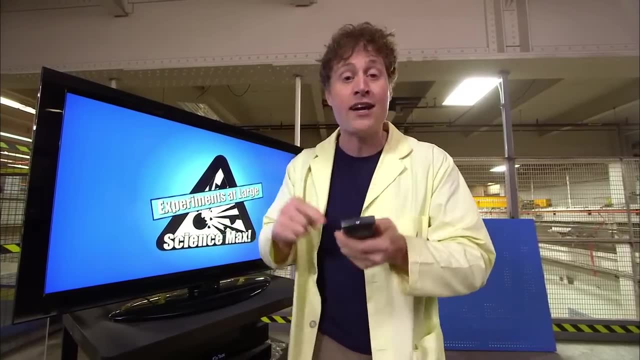 You're thinking, Phil, wait a minute. The bulb did not light up and I've never seen the bulb on my TV remote light up when I press the buttons. Well, that's because your TV remote works on infrared, which is a kind of light you can't see. 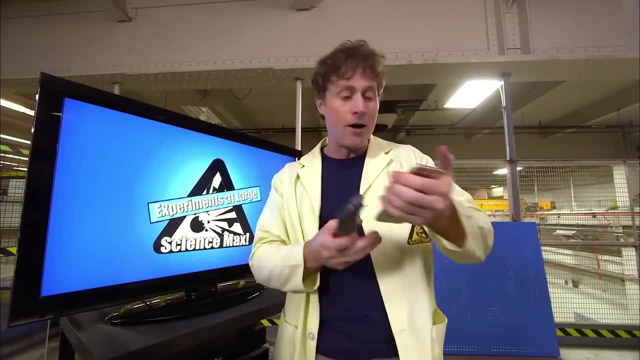 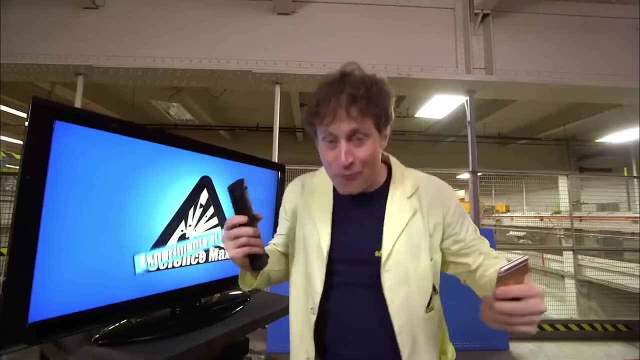 But you might be able to see it with a camera. If you have a digital camera or a camera on your phone, ah, now you can see. See. It lights up And because infrared light works the same way as visible light. 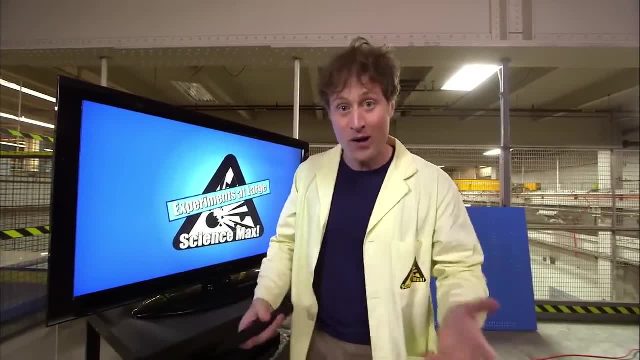 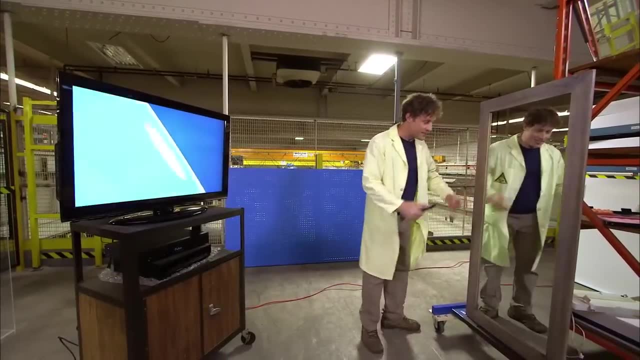 in that it will bounce off a mirror. here's an experiment you can do at home: Bounce the light off your TV remote, off a mirror, and turn on and off your television. Check this out. You get a mirror set it up just right. 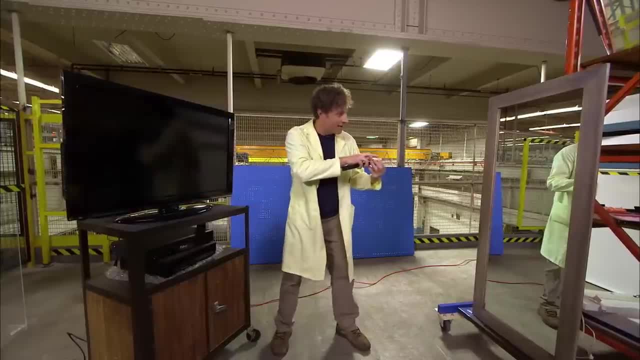 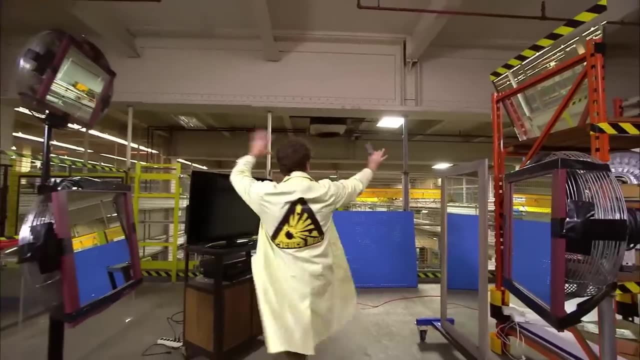 and then aim the remote at the mirror and it turns off the television. Pretty cool, right, But now let's max it out. I've got a complex series of mirrors set up here and I'm going to bounce the light from the remote. 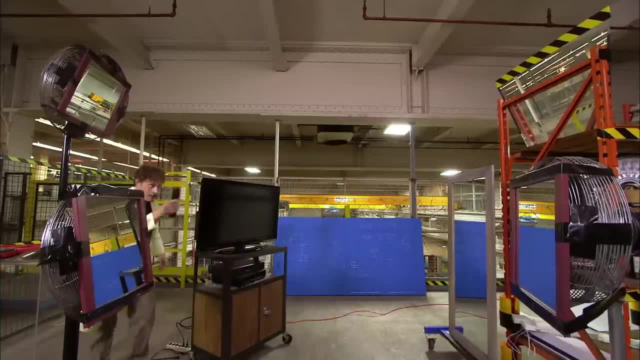 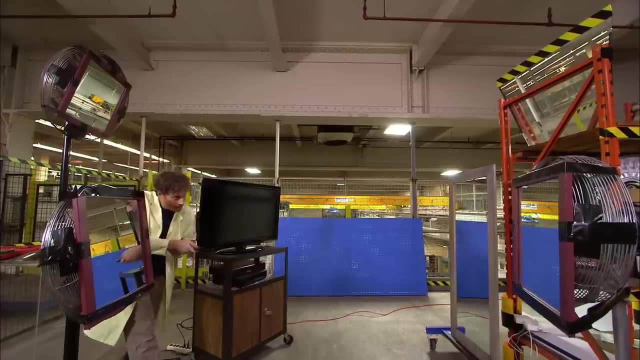 all over the room. And here's what that pattern looks like: The light from the remote hits this mirror, which reflects to this mirror, which reflects to this mirror, and then this mirror, and then this mirror, and then, finally, to the television. 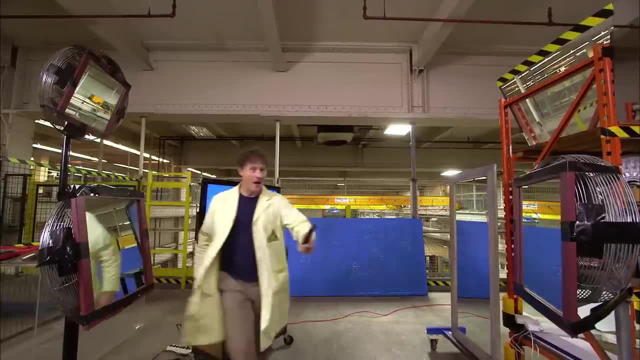 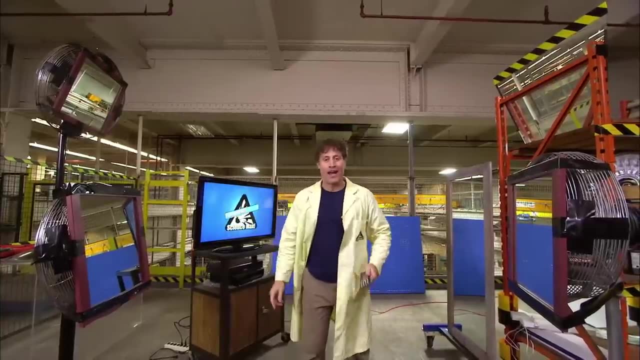 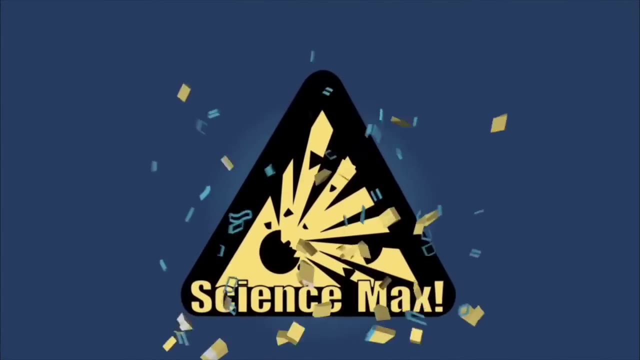 Isn't that cool. There you go, Maxed out, remote light bouncing infrared flashlight- I've got to come up with a better name, But still it's pretty cool. All right, Turn off the television, Leave the room. I solved Anne's first light challenge. 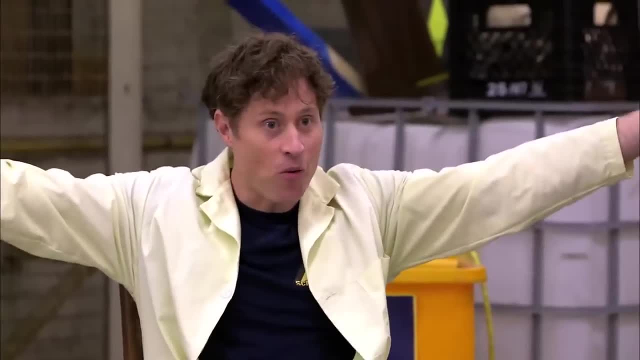 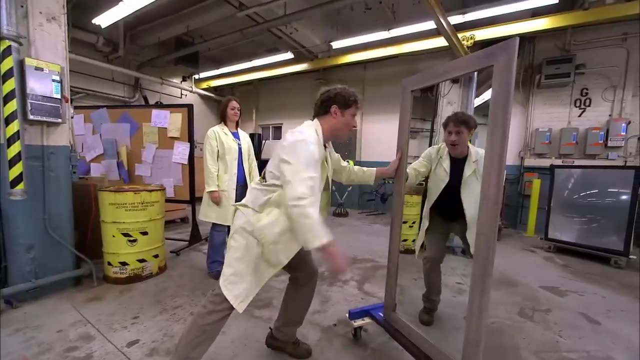 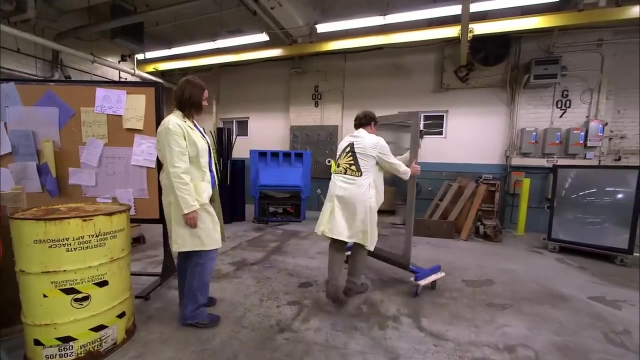 seeing something far away with a lens. It says 71. But now she's moved the ball around a corner and now I have the solution: Mirror. A mirror will let me see around the corner, Clever, OK. So all I got to do is put the mirror in a position. 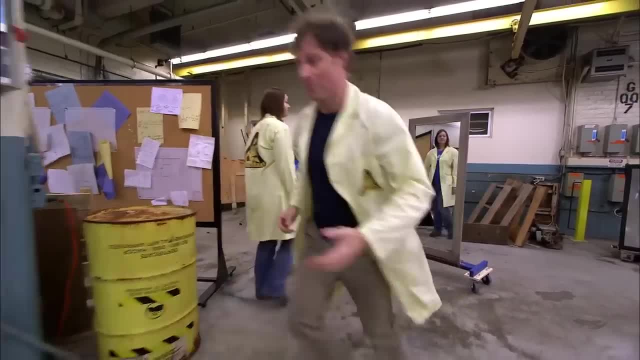 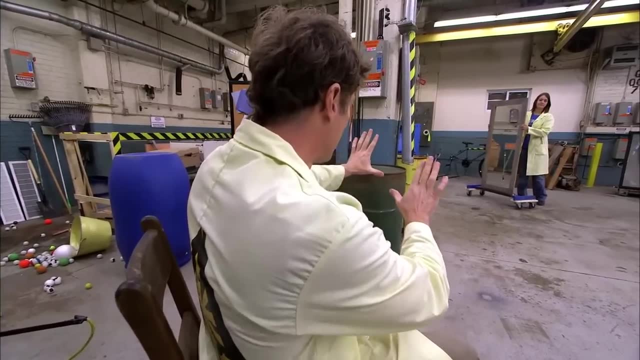 sort of like that, I guess, And then I'm going to sit in the chair. If you could help me adjust that mirror. Keep going that way, Keep going, Keep going. Yeah, stop, Nice, OK, Go ahead and flip the ball around. 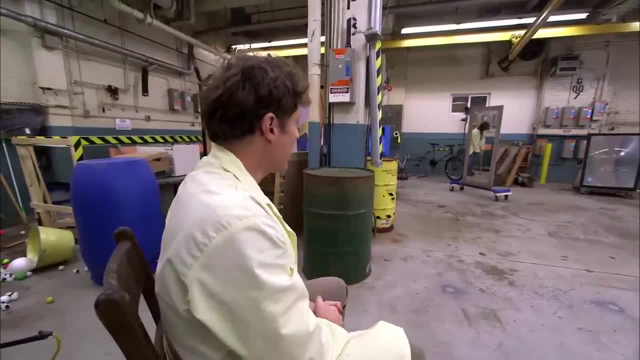 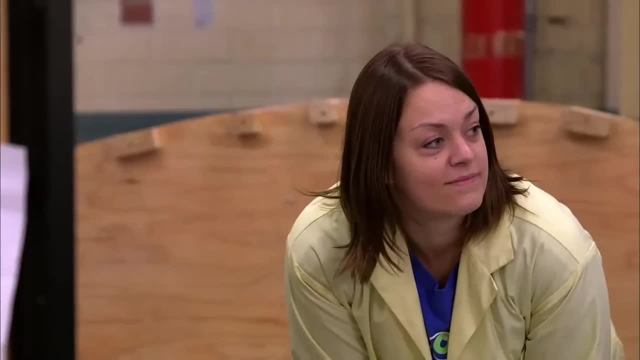 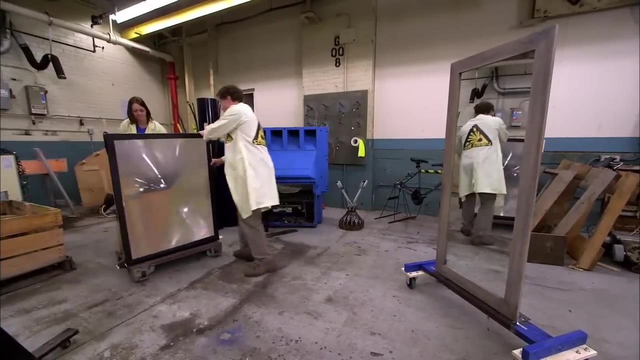 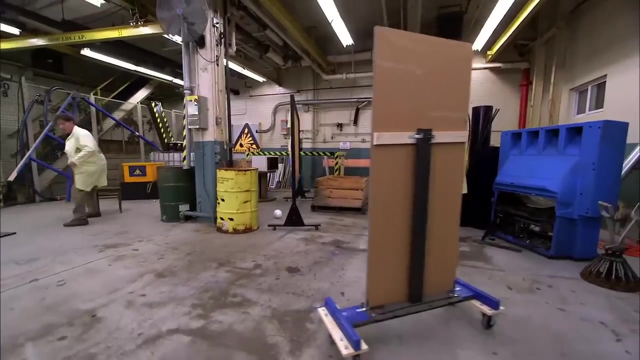 OK, Flip it around The lens. I need the lens, So we'll use a mirror and the lens to Good. Yeah, Yeah, OK, I'm going to sit in the chair. Here in the chair It is backwards. 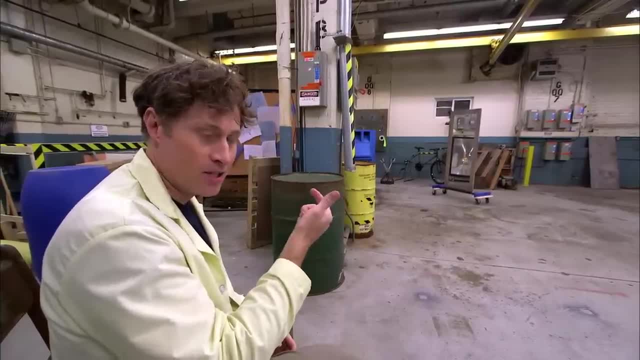 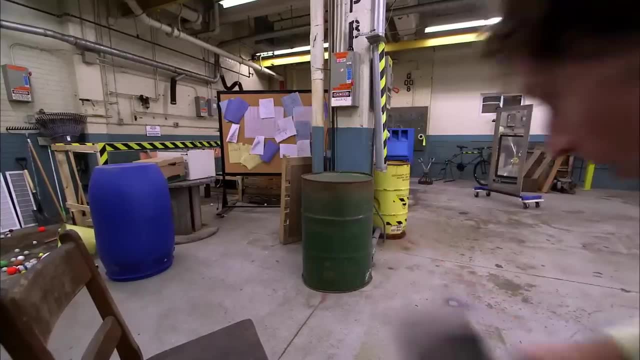 Oh yeah, A mirror inverts the image, doesn't it? Mm-hmm, That's OK. That's OK, I can solve this. All I need Whoa Other mirror is all I need to solve this problem. 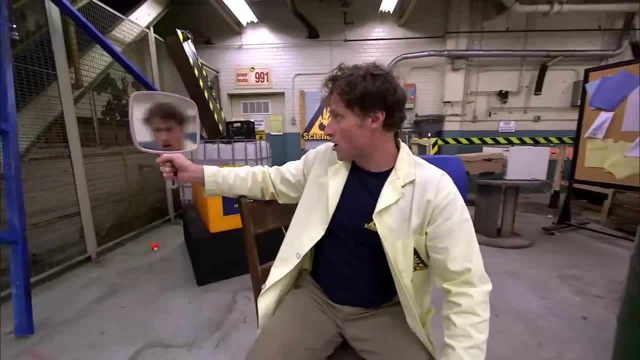 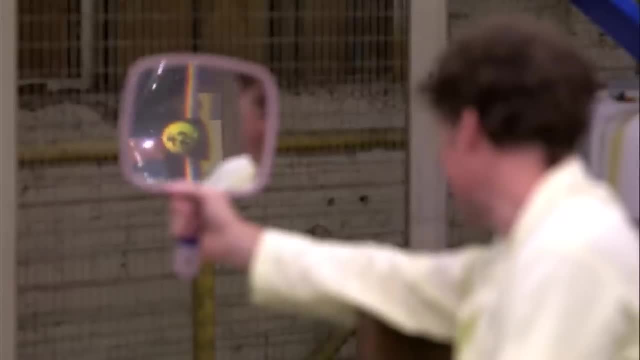 So if I take this mirror and I put it here, Let's see, There it is, It says 42.. Nicely done, Ha ha, ha, ha ha. Nicely done, I am ready for anything. What do you got planned? 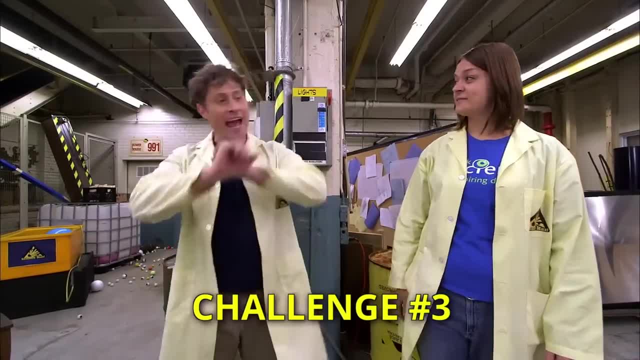 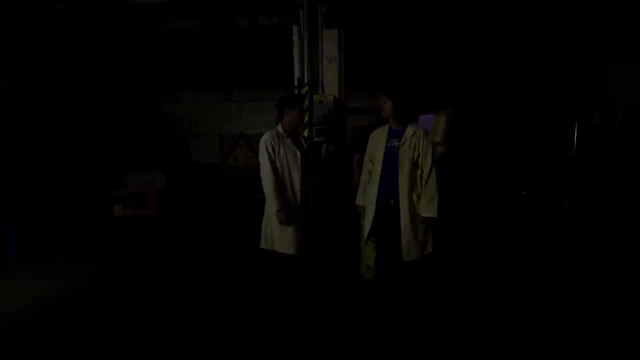 I'm ready for the hardest challenge. Are you sure you're ready for this? Totally, I am Challenge number three. Challenge number three starts now. What? Wait, wait, wait, wait, wait, No, no, This is a light challenge. 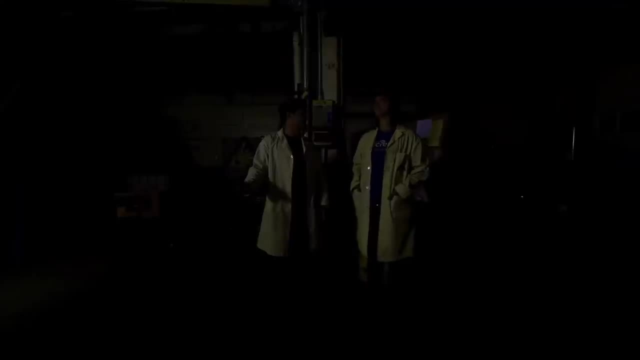 How am I supposed to do a light challenge if it's dark? You have to get creative, But it's dark, OK, No problem, I will think of something. I will be back, OK. OK, Careful, Whoa. 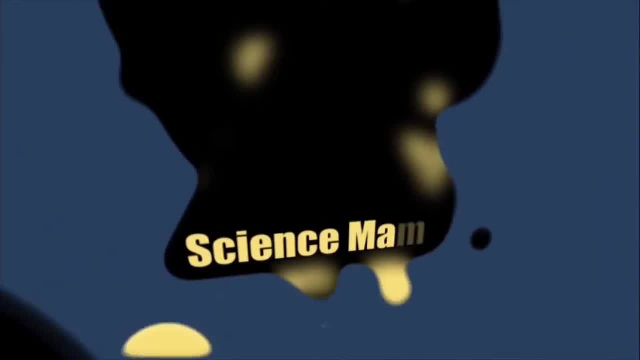 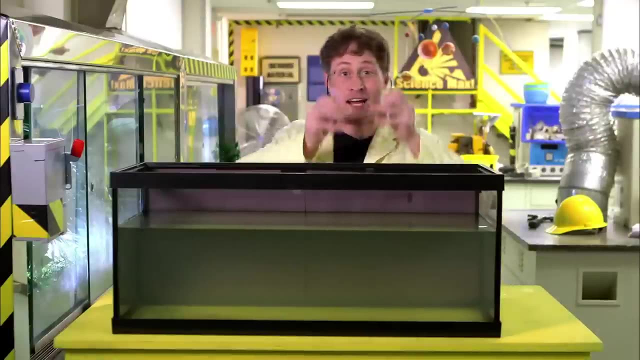 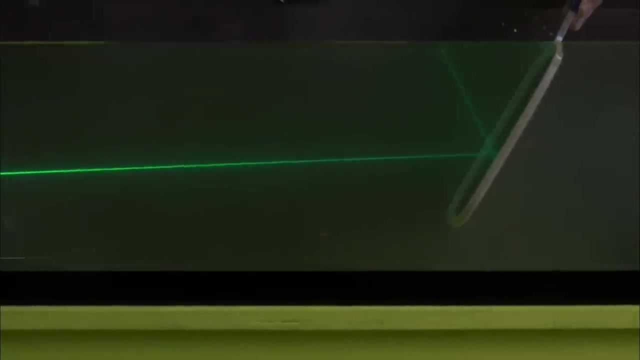 I'll be waiting, Whoa Careful. So you already know about reflection, right? That's when the beam of light, say from my laser, reflects off this mirror and bounces in a straight line. But check this out, If I don't use the mirror and I shine the laser. 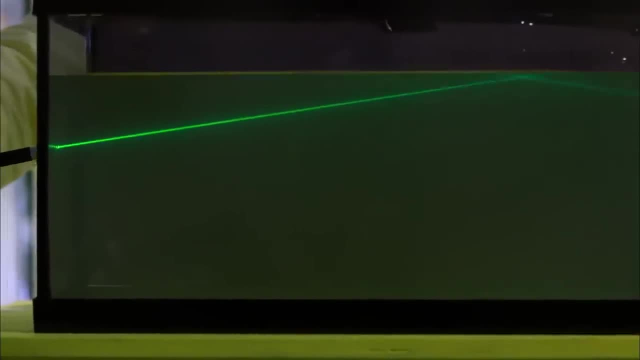 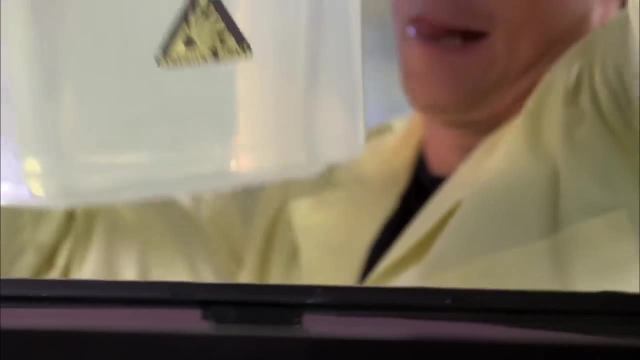 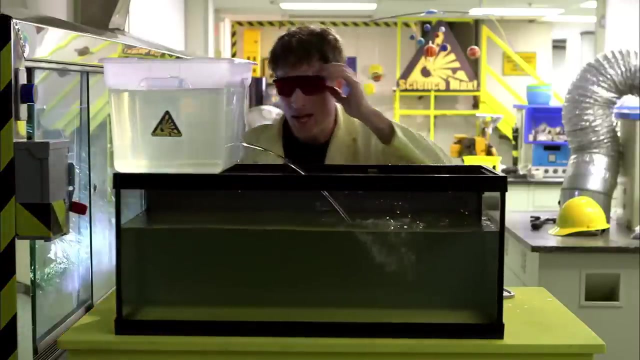 against the underside of the water. it also reflects, just like a mirror. This is called internal reflection. If I have a stream of water and I put my laser beam into the stream, you could see that the laser bounces around inside the stream of water. 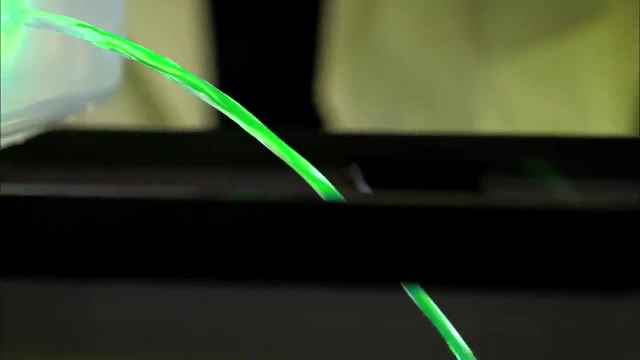 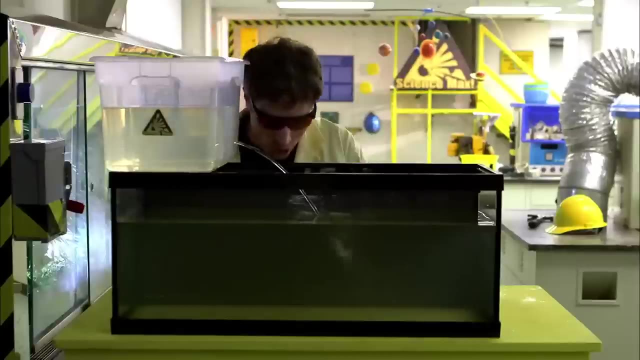 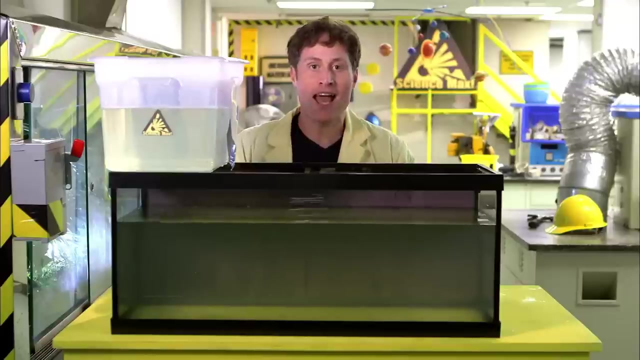 It's being internally reflected And the laser isn't going straight anymore. It's following the stream of water down where the water goes: Internal reflection. Now I know what you're thinking. You're thinking, Phil. how does this affect me in my everyday life? 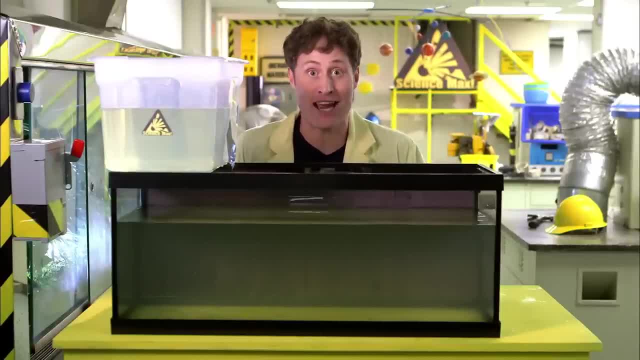 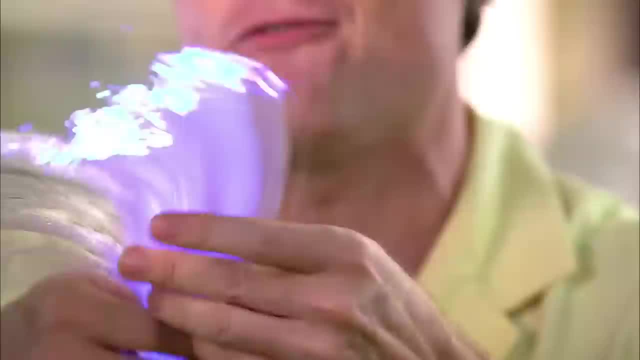 Internal reflection. Who cares? Well, I can tell you why you should care in two words: Fiber optic wires. Three words: Fiber optic wires. You see, fiber optics carry information all over the planet: The internet, maybe even your television. 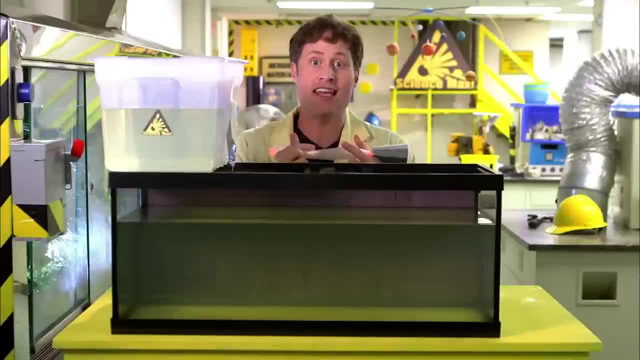 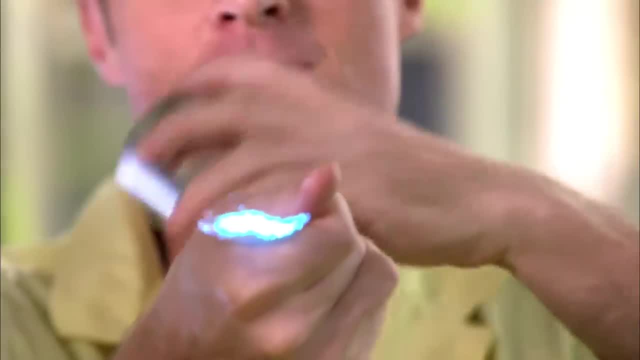 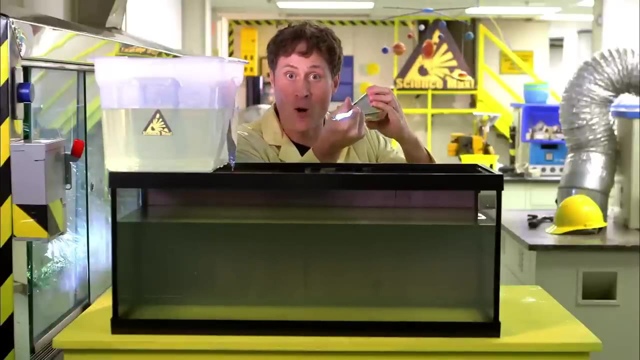 travels through fiber optic wires. The good thing is, because of internal reflection, you can bend fiber optic wires any which way, around corners, and the beams of light continue to go straight down inside the wires and get out the other end, making it go where you want it to go. 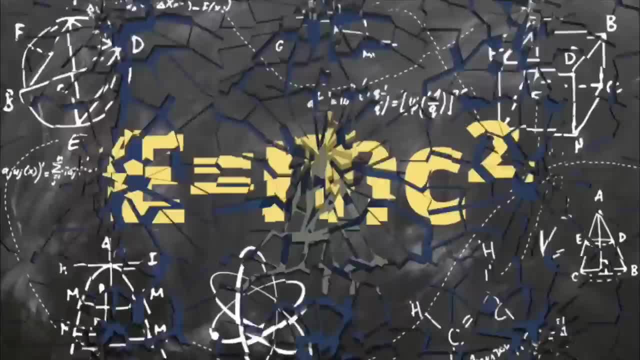 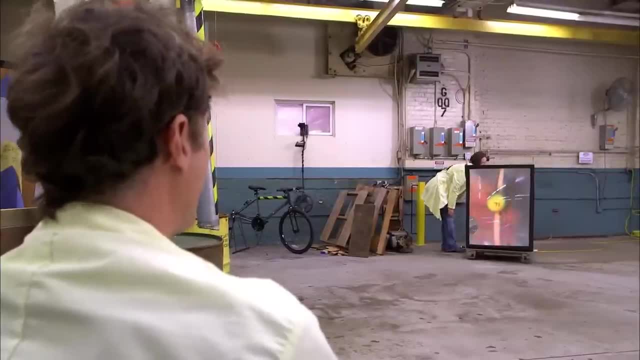 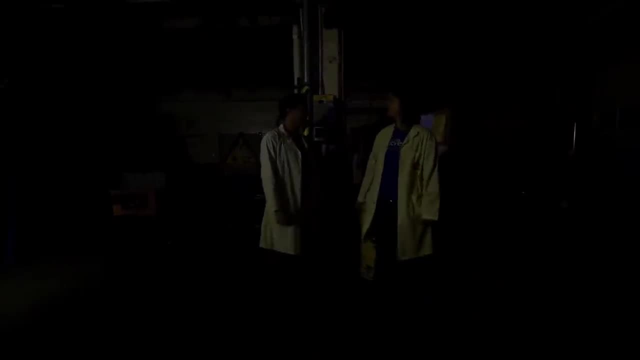 Internal reflection Science. Back to our light challenge. I've seen something small from far away, seen around corners, but now Ann has turned off the lights. But I have a solution, Ann, Ann, Careful. Okay, Sorry, I forgot how dark it was in here. 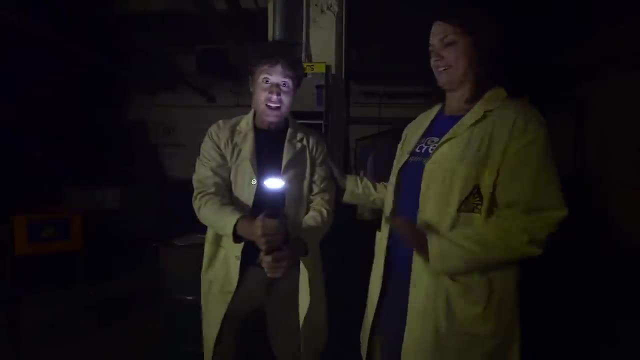 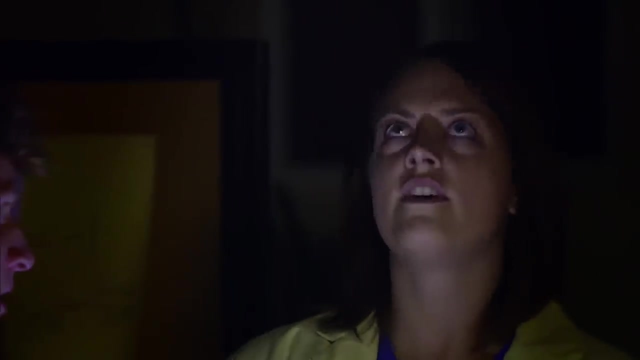 Okay, I figured it out. Okay, I have a flashlight. That's all I need to do. No, no, no, Hold on, Hold on What. There's one more rule. I didn't tell you What's the rule. 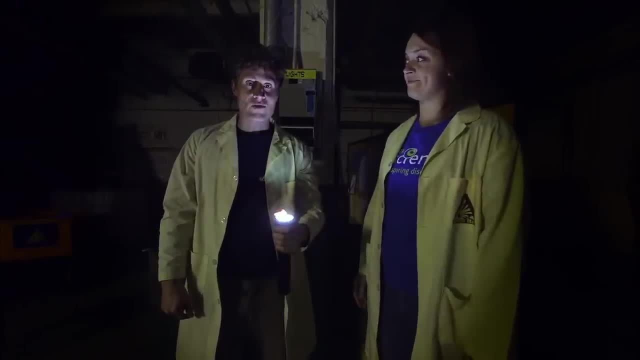 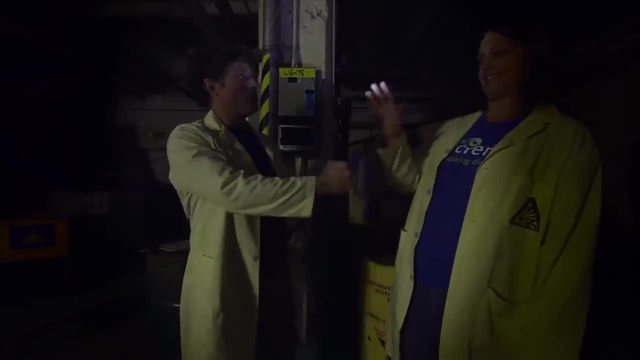 You can't use visible light. How in the world am I going to do this if I can't use visible light? It's a challenge. Uh, wait a minute. Wait a minute. Okay, here I'll hold my flashlight for a second. 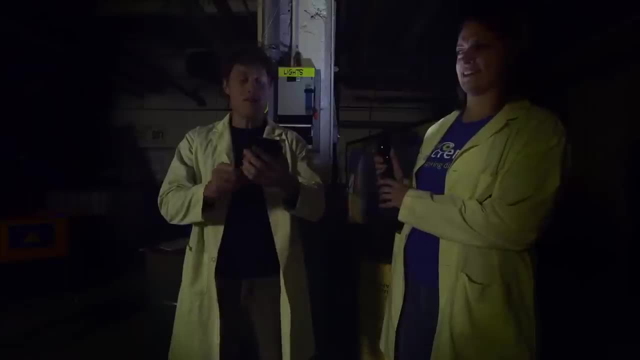 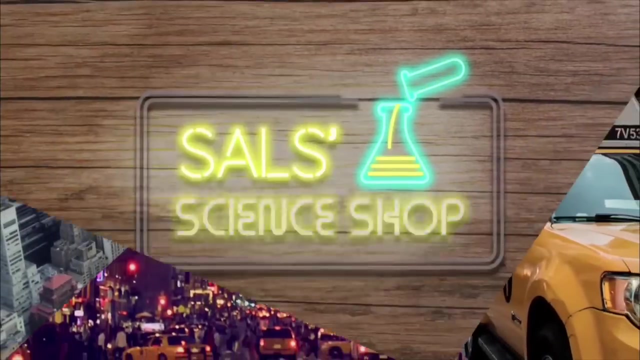 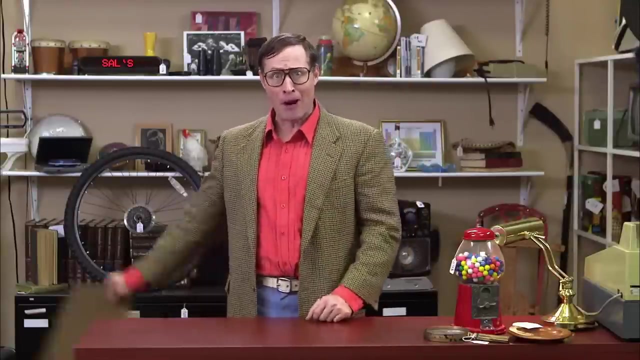 I'm going to make a phone call. Okay, I think I know what to do. I'll be back. I'll be back, Okay, Oh, careful, Oh, Oh, hey, good to see you. Speaking of seeing things, let's talk about the rainbow. 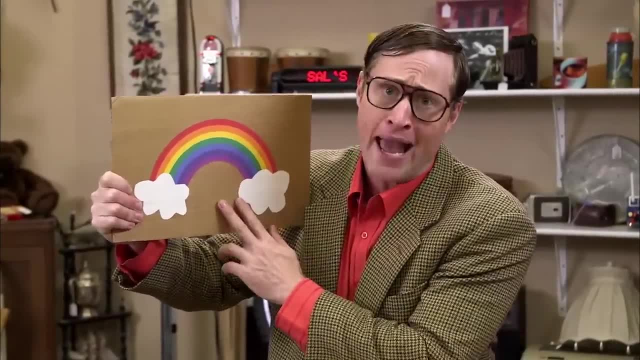 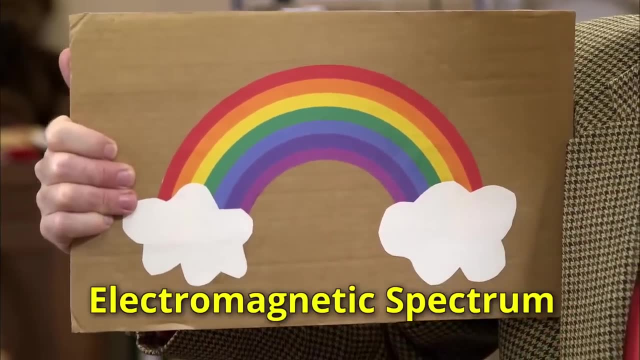 All the colors of the spectrum organized in a beautiful pattern. But what are the different colors? I mean, what makes them different? Well, it all has to do with the electromagnetic spectrum. This is visible light, All the colors of the rainbow. 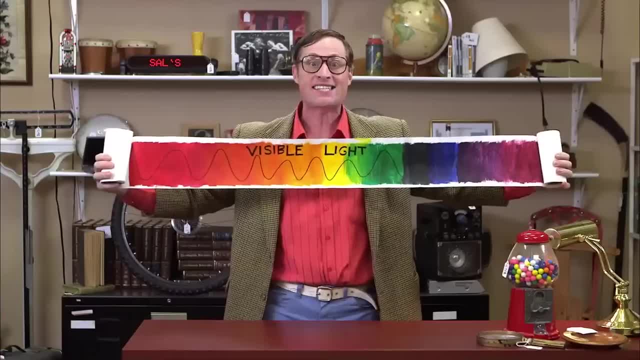 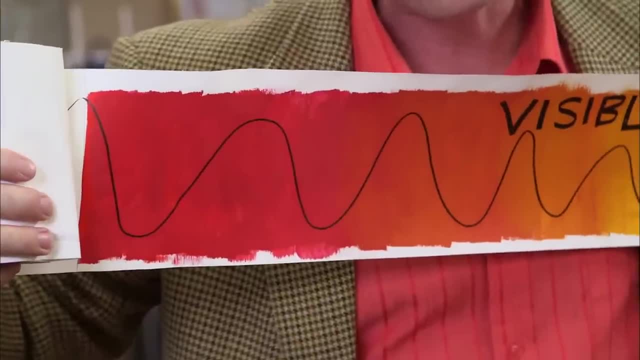 And take a look at that little black line that goes up and down there. That's the frequency of the light. Light is a wave. You see, the wavelength is a little wider out here on the red side and it's a little closer together here on the violet side. That's because every color of light has a different length of wave or wavelength, And that is what makes them different. It makes them different when we look at them. But if you think that's all there is to the electromagnetic spectrum, then you're mistaken. 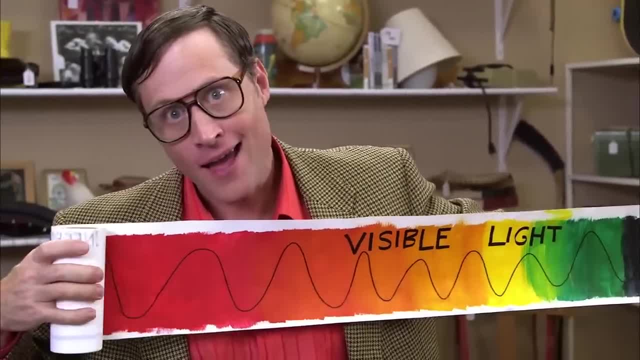 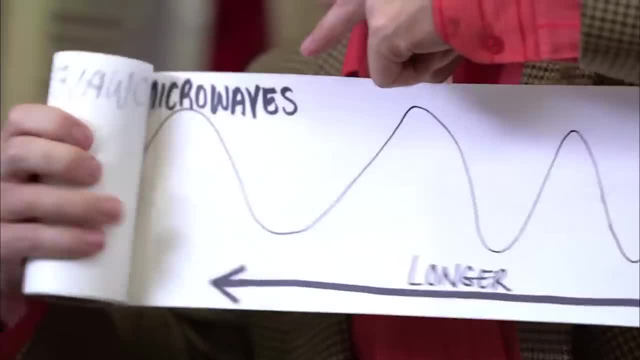 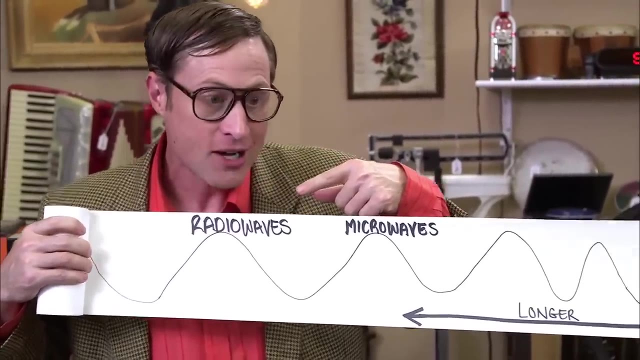 So what happens over here on the red side? Does it keep going? Yeah, it does. What Look? we got infrared here and then we got microwaves. These are the same kind of waves you use in your oven. And then we got radio waves, which are the same kind of waves you use in your radio. 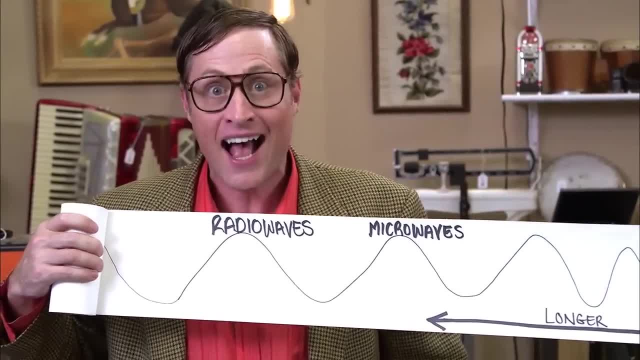 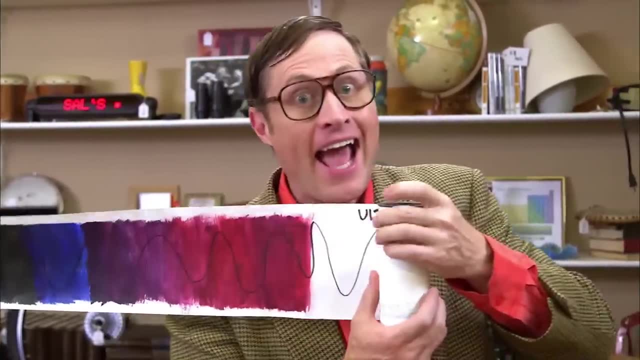 They're all part of the same thing as visible light. Huh, Let's take a look at the other end. Remember these short wavelengths over here beside violet Well, does that keep going? Yeah, If they keep getting shorter, you get ultraviolet and then X-rays. 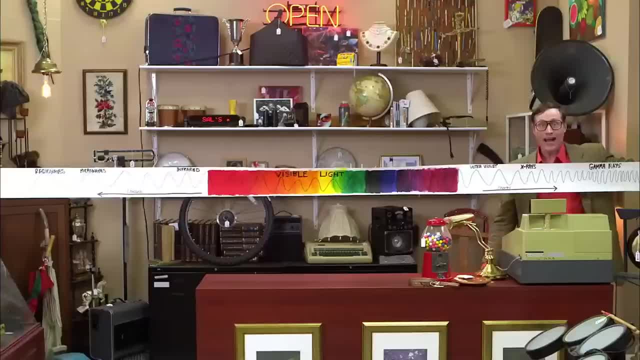 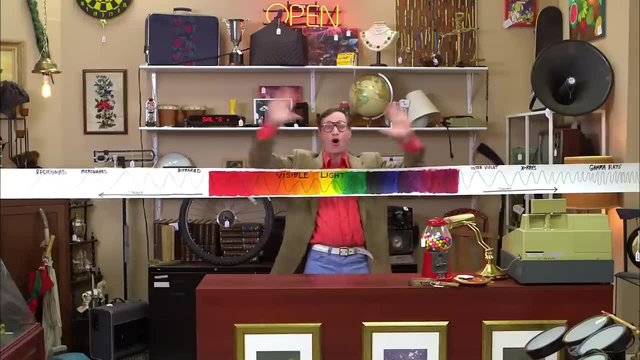 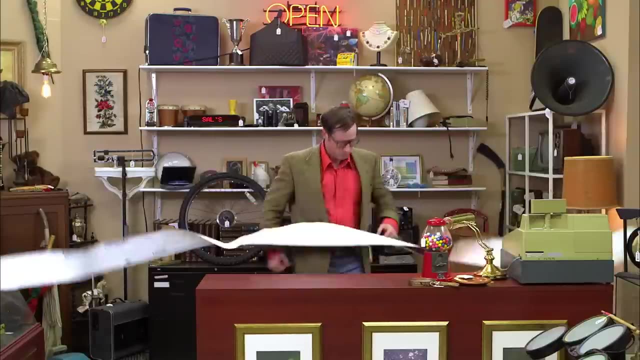 and then gamma rays- Huh, Pretty amazing. And look, it's all connected, From radio waves to gamma rays, to visible light. in between it's all frequencies of electromagnetic radiation. How is this staying up? So everything outside of the visible spectrum is invisible, right? 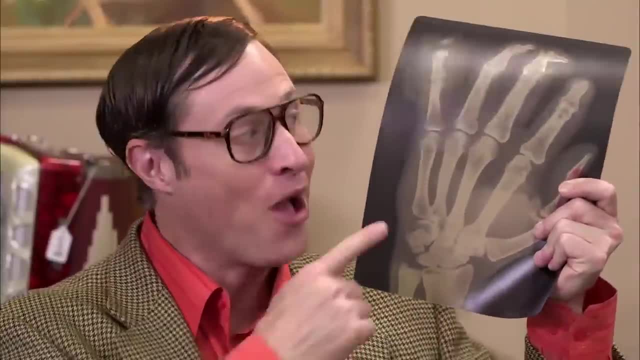 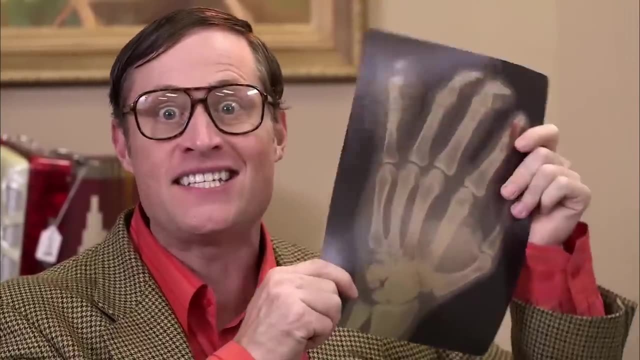 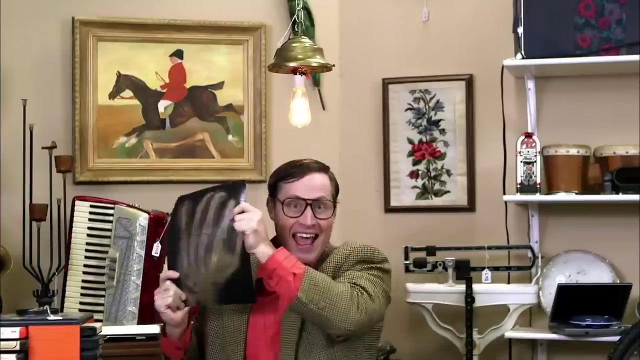 Wrong. Ha-ha, Bam, Huh, That is an X-ray, a picture we can take using this part of the spectrum. We can use special cameras to see outside of the visible spectrum. Huh, Huh, Right Yeah. 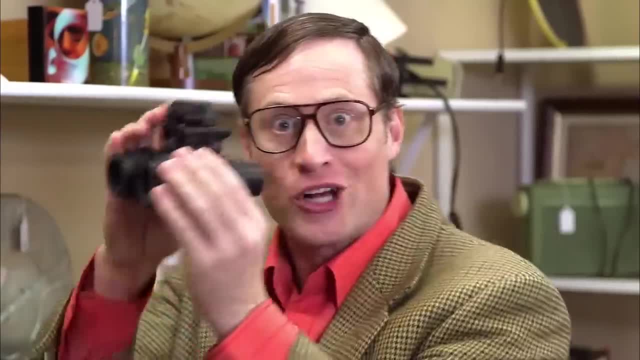 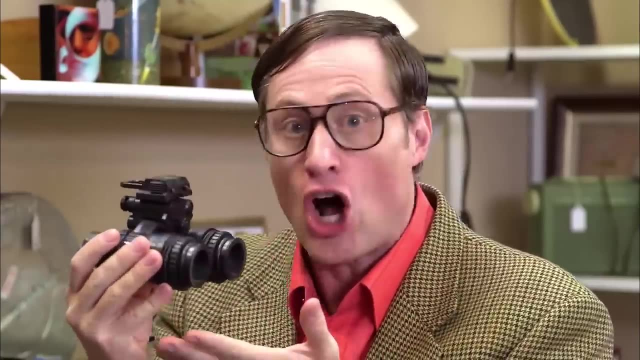 Okay, you got it. Huh, And look at these. These are night vision goggles. They help you see in the dark. They use part of the spectrum called infrared. For those of you keeping score, that's this part of the spectrum right here. 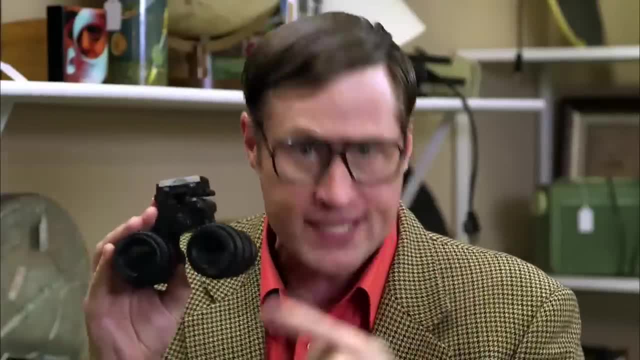 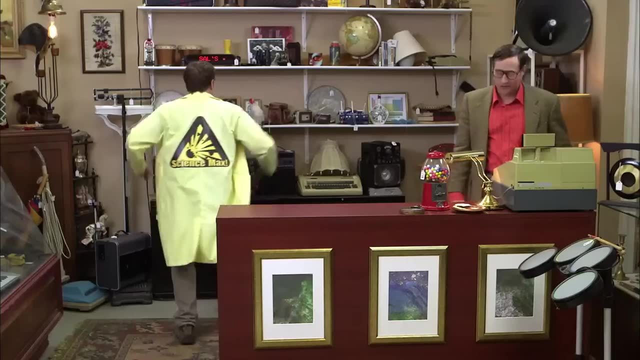 Pretty neat, right? I would sell you these, but they're already spoken for. Oh, here he comes now. Hey Sal, Hey, how you doing. You got those goggles I ordered. Yeah, go ahead, Help yourself. Thanks for putting them aside. 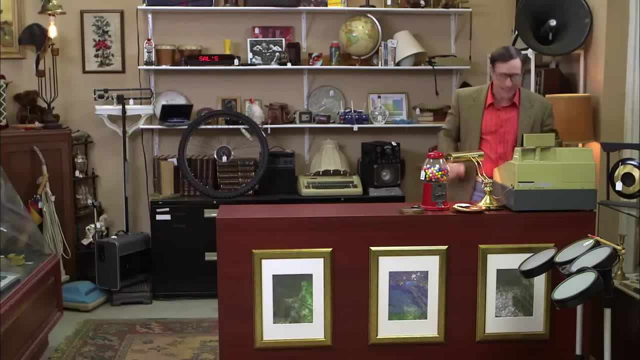 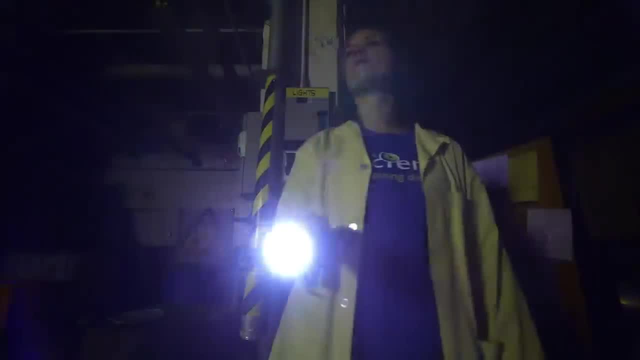 Can I put them on my tab? Yeah, no problem. All right, thanks, Sal. Okay, see you later. Nice kid, He's always in a rush though, Phil, Is that you? Yeah, Do you need the flashlight? 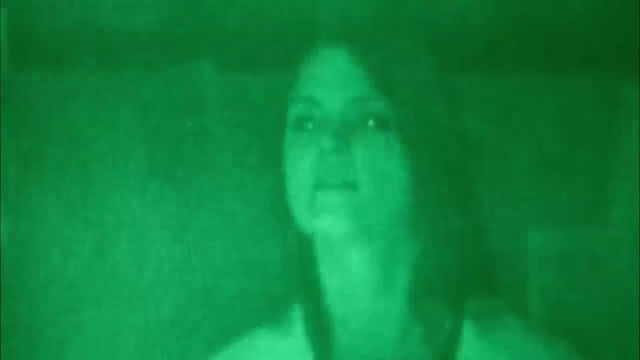 I don't Turn it off, I can totally make my way over to you. Oh, I can hear you. Yeah, I'm right here. Oh, right here, Hi, Because I have night vision goggles. Ooh, check it out. 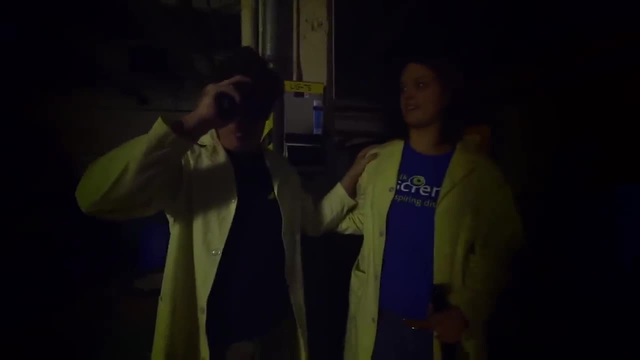 Oh cool, Pretty cool, right, That's awesome. So here's the spectrum again, and here's visible light. My night vision goggles use infrared- this part of the spectrum here- with wavelengths just like this one. Oh cool. 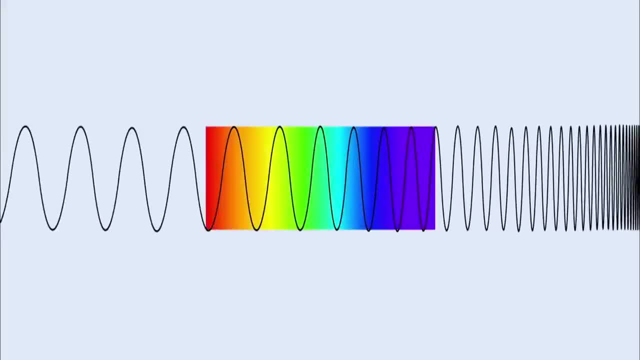 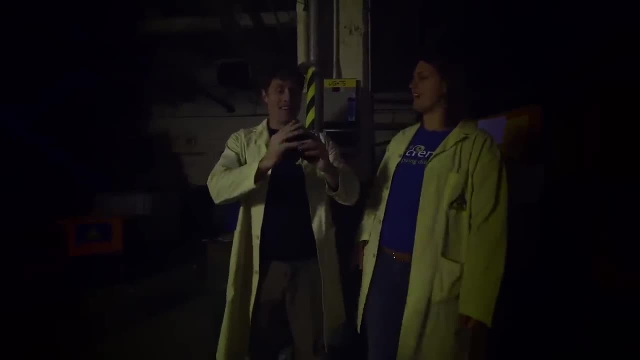 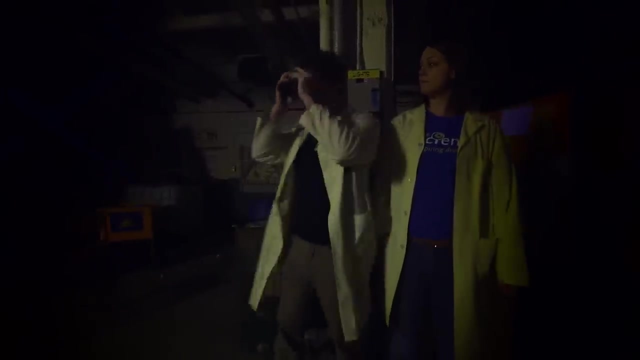 Outside of the visible light spectrum. All right, I would say that's allowed No visible light, and I will see the next ball. Have you got it set up? I set it up while you were out, Okay, good, I'm going to sit in the chair and see if I can see it. 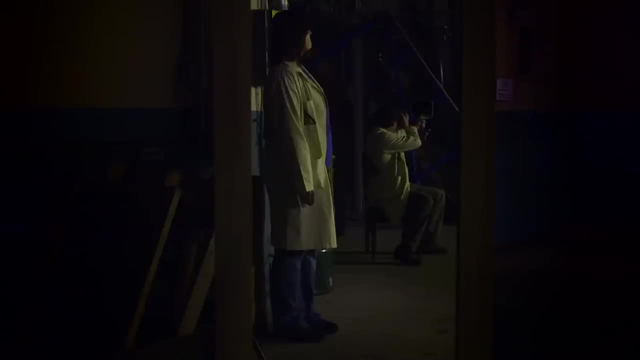 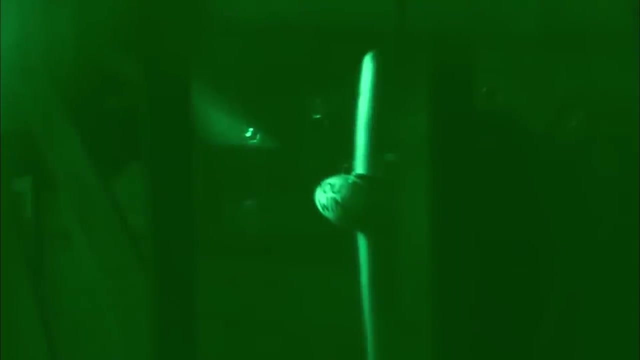 Okay, Here we go. Mm-hmm, Oh, wow, I can totally see everything. Can you tell me what the ball says? It says it says you win. Nicely done. So let's recap: This challenge is the same as the last one. 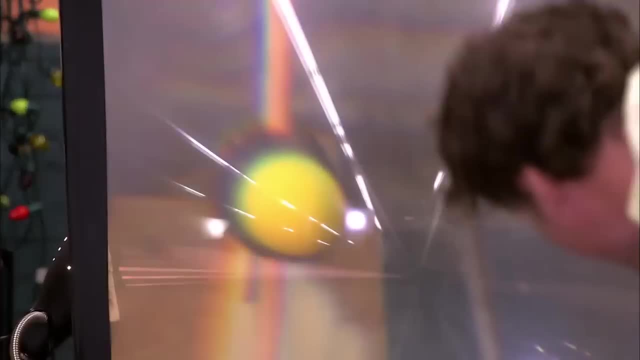 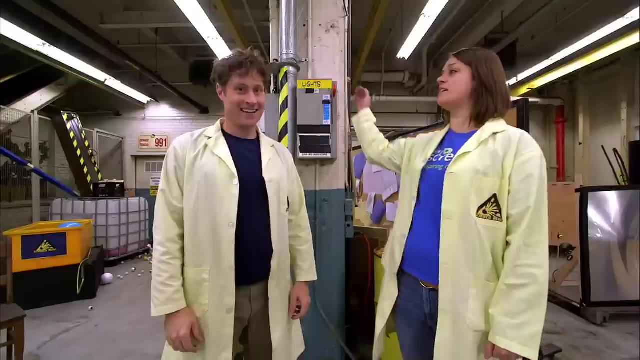 challenge. The light from the ball was magnified by the lens, sent around a corner by reflecting it off a mirror and flipped back around by using another mirror, But this time it's dark, so using infrared light thanks to my night vision. 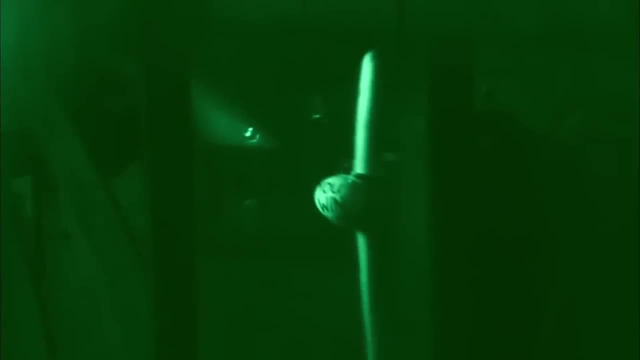 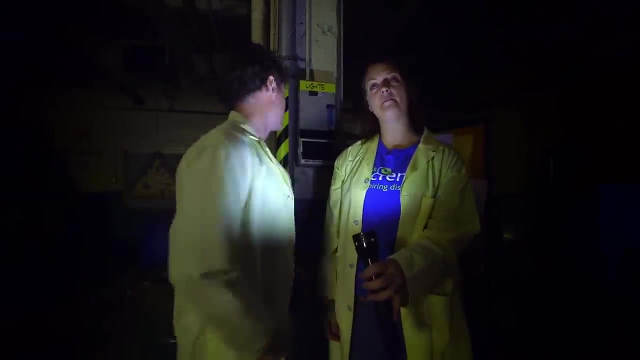 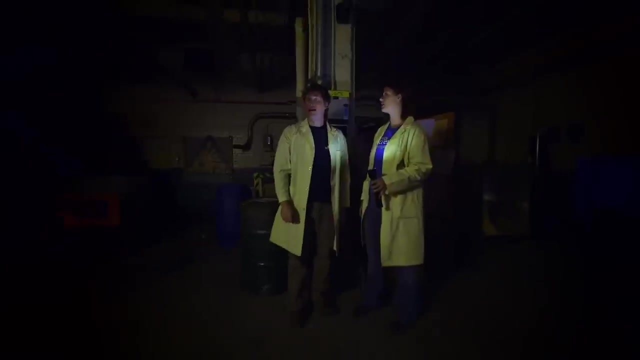 goggles, I was able to see the ball and win the game. The light manipulation challenge is done. Science Max: experiments at large Time to turn the lights back on. Yep, absolutely, Huh, What did you do back there? Um, I guess we blew a fuse or something. 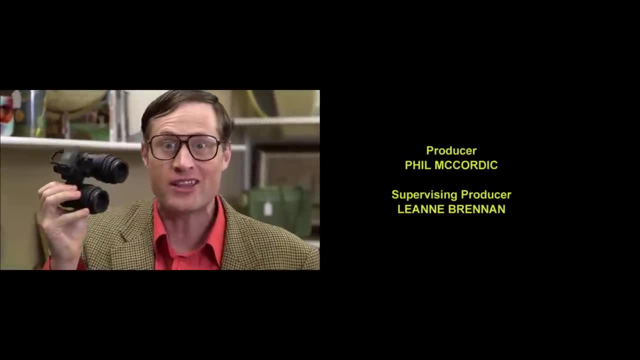 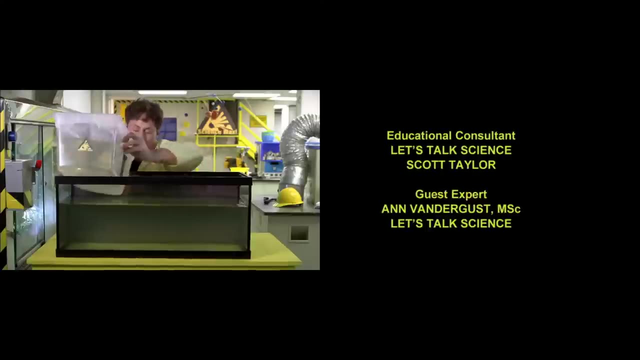 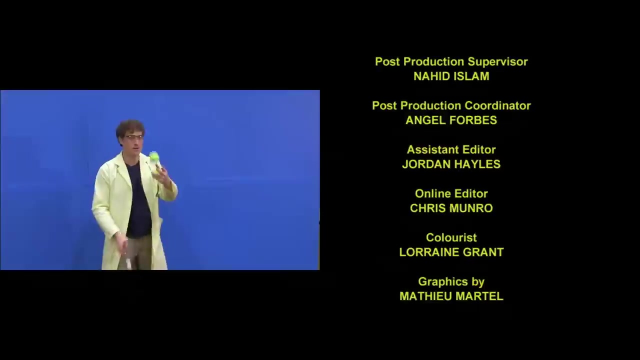 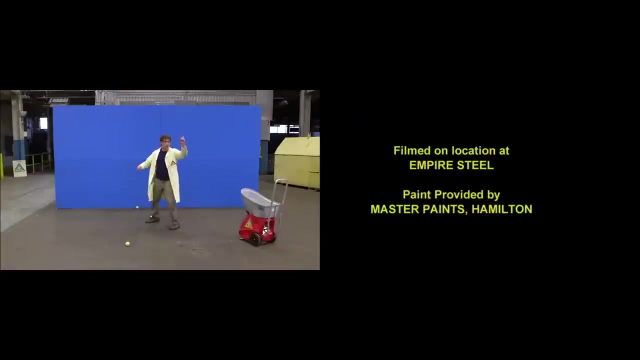 Uh-oh, These are night vision goggles. They use some of the v- the v- they use some things that I cannot pronounce. Have this container of water, Whoa, And I make it stream, But instead of going straight back, they're going. 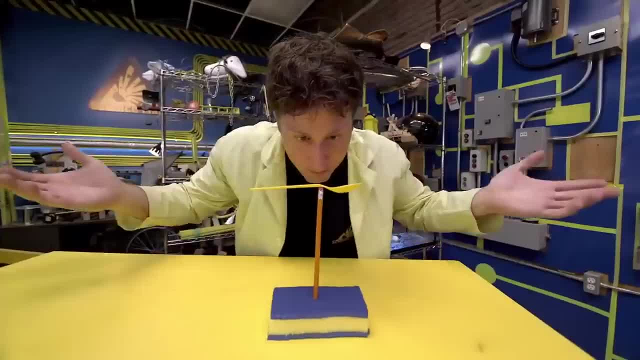 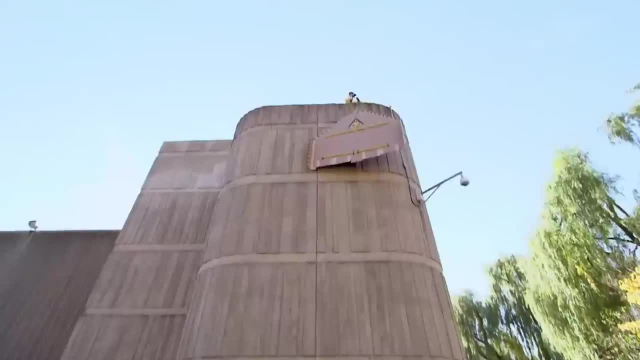 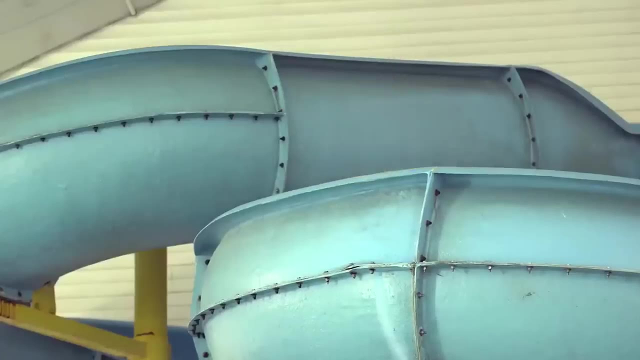 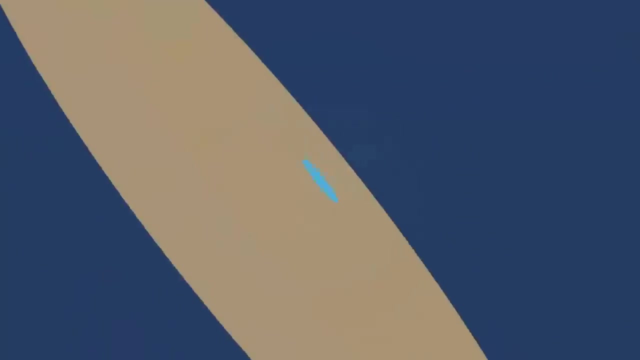 Have you ever done a science experiment and wondered what it'd be like if you did it big? I have. Yeah, My name is Phil and I take your life, Take your everyday science experiments and do them big. This is Science Max: Experiments at Large, Science Max. 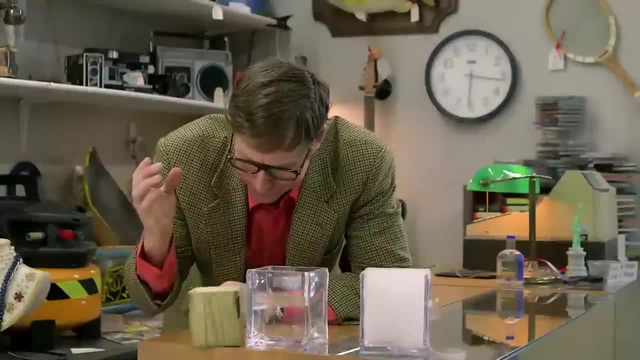 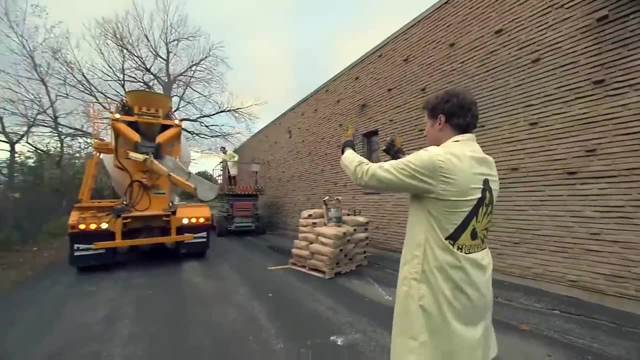 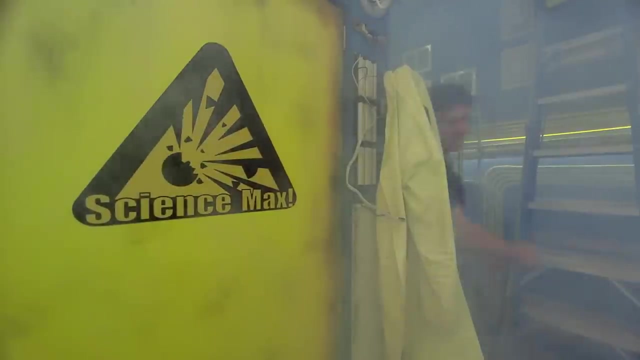 This episode of Science Max is a messy one. We're looking at solids, liquids and gases and things in between, like cornstarch mud Today on Science Max: Experiments at Large. Behold the power of states of matter. Greetings, Science Maximites. 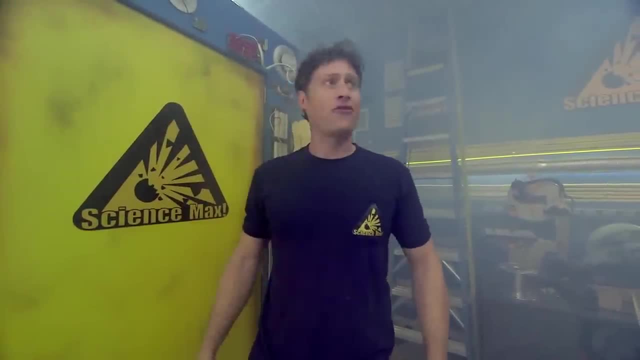 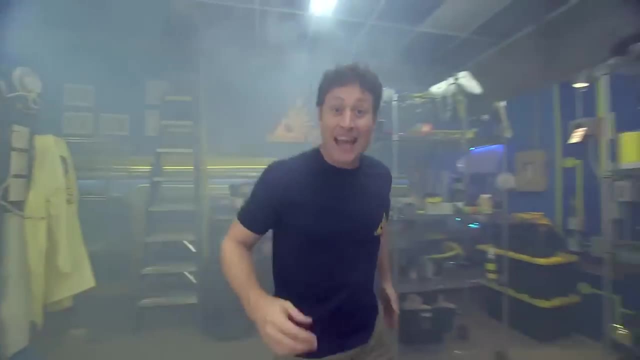 I'm Phil McCordick. I think I overdid it with the fog machine. This is Science Max, Experiments at Large. Can you even see me? Let's go over here. Today we're talking about states of matter. Now there are three main states of matter. Solid like this table. 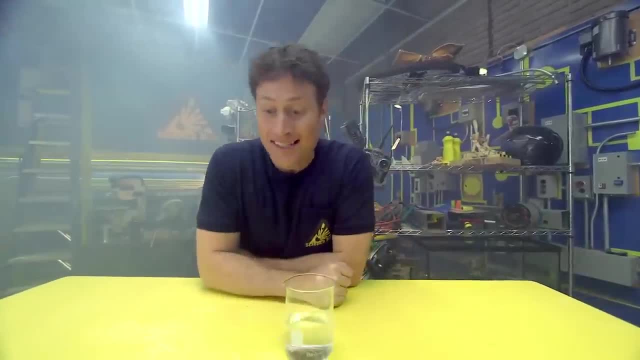 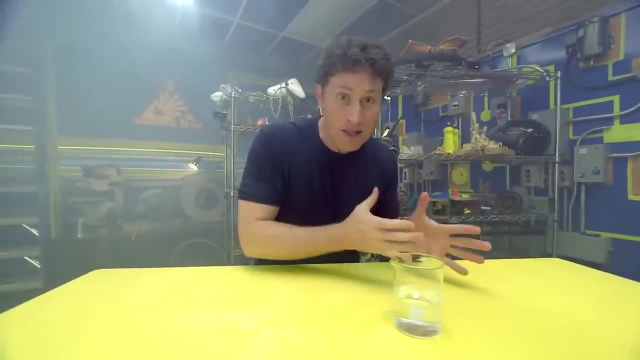 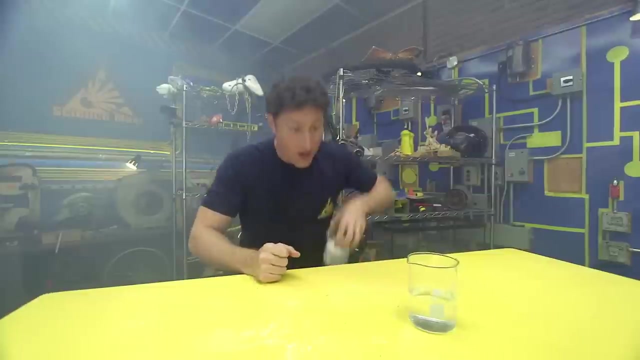 Liquid like the water in this beaker And gas. Yes, Thank you, And we're also going to be looking at the things that kind of go in between, Things that are sometimes solid, sometimes liquid, like cornstarch, Like cornstarch mud, which is very easy to make: All you need is water and cornstarch. 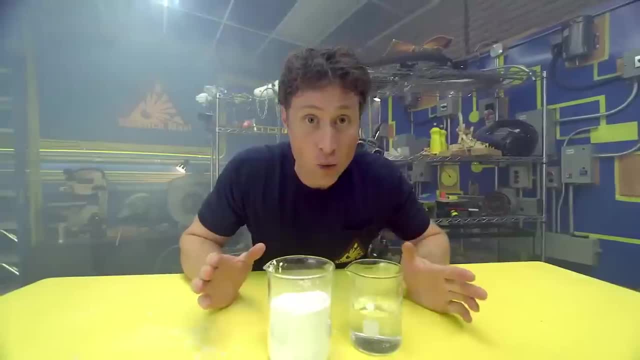 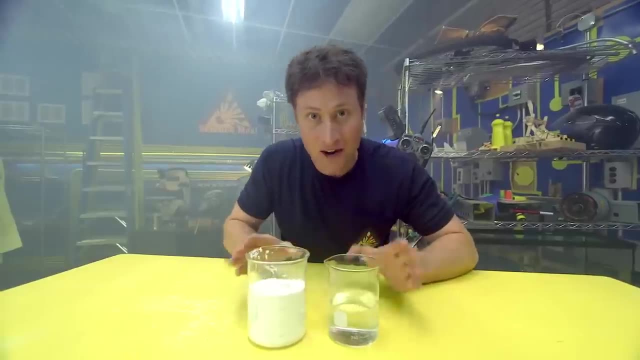 which you can get at the grocery store. Mix it up however much you want. Just remember two parts cornstarch to one part water. Twice as much of this than you have of that Very easy. Mix it up and you get cornstarch mud which sort of seems like a liquid unless you hit it. 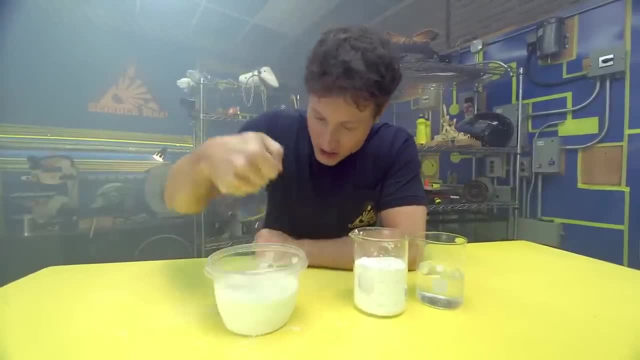 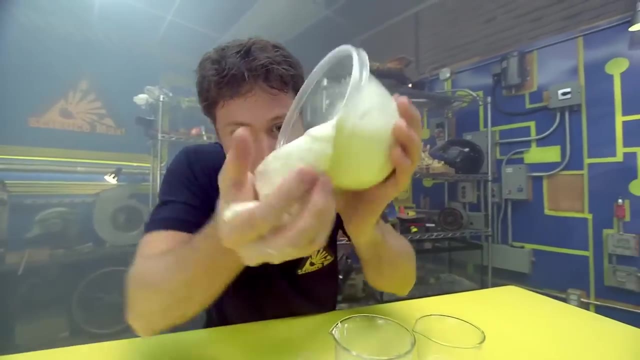 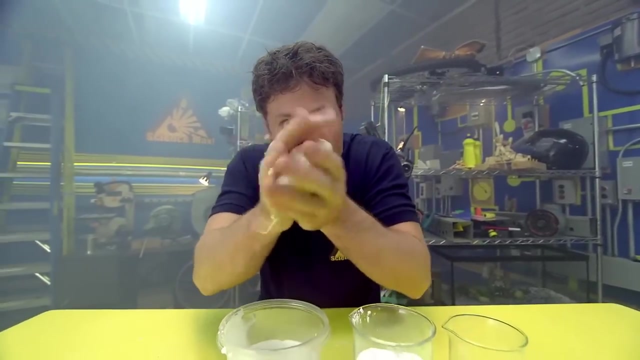 And then it becomes solid. But if I pour it It's a liquid. Even if I hold it in my hand and I hit it really fast, it turns into a ball, And it will stay in a ball as long as I keep hitting it or squeezing it. 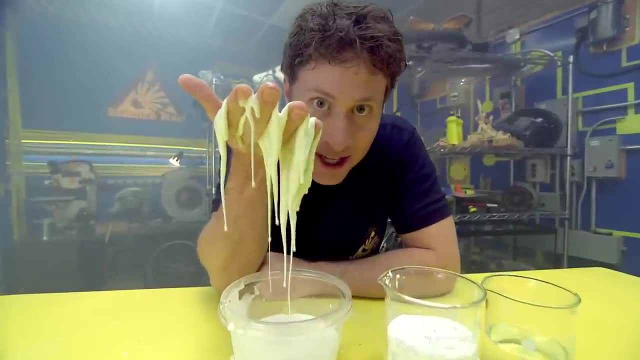 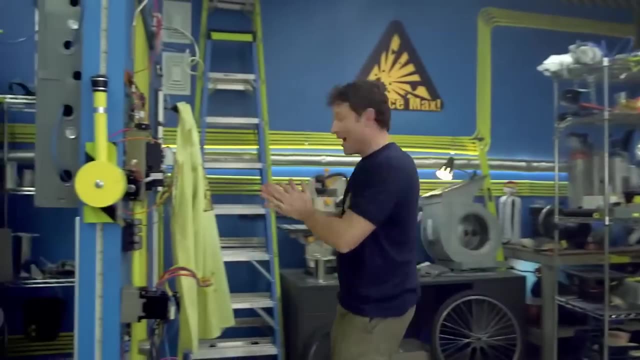 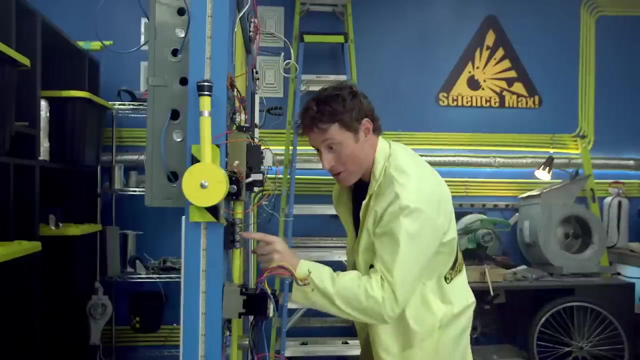 But as soon as I stop, it turns into a liquid again. Now we're going to max this out. We'll go through the portal and learn more about solids, liquids and gases. Right, That's why I'm going to the Center for Skills Development and Training. 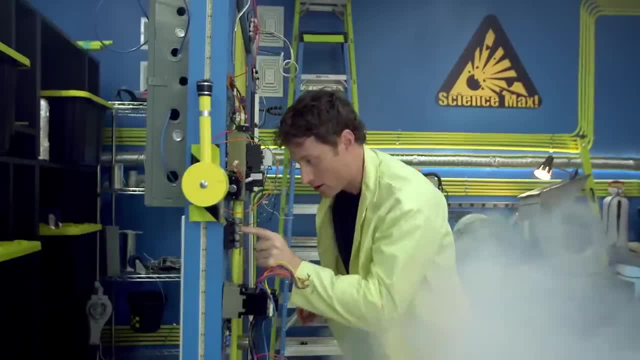 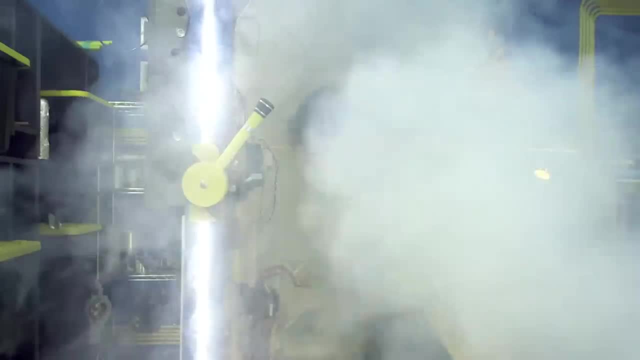 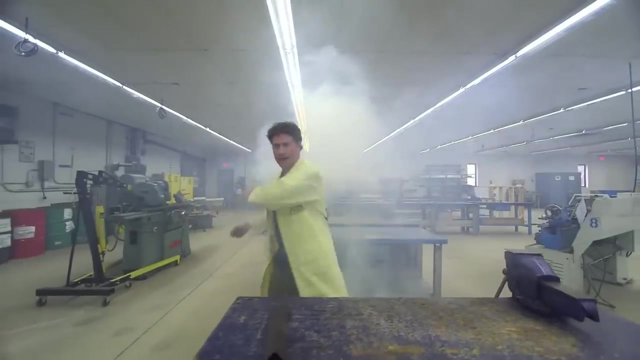 Oh, no, wait, That's the code for the fog machine. Wait, Stop, Stop. It seems to be stuck. Oh, never mind. Never mind, I'll fix it later. Hey Judy, How are you? Hi Phil, How are you? 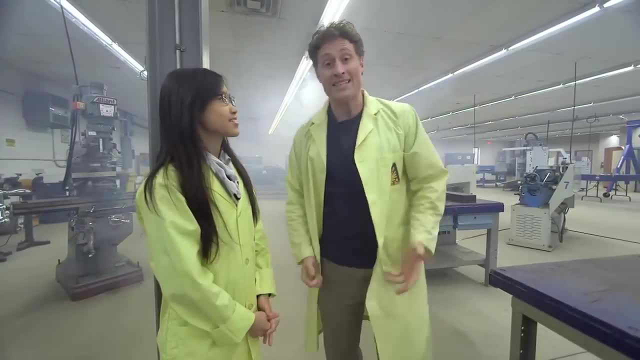 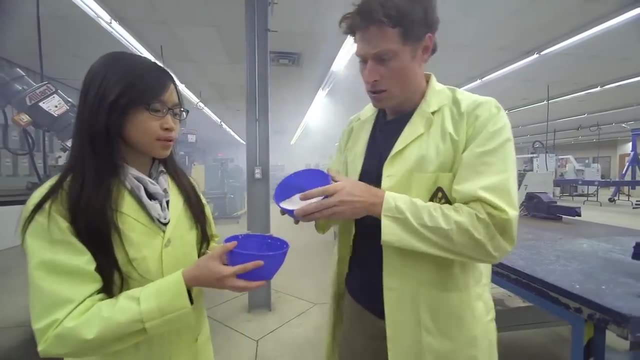 Good, Judy is going for her PhD in chemistry right. Yes, Fantastic, Because that means you can explain cornstarch mud to me. Now, is this a solid or is it a liquid? Well, it kind of has properties of both. 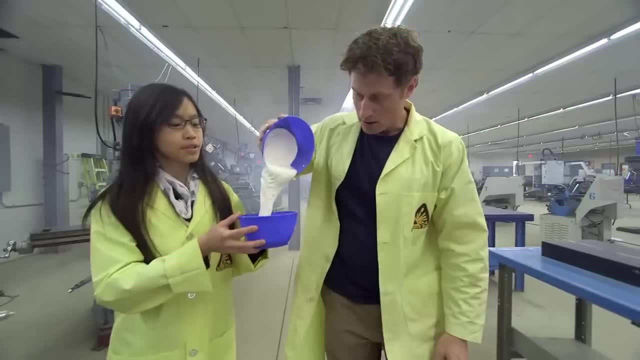 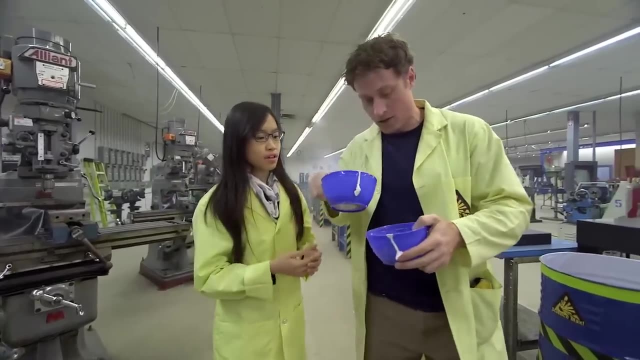 It's called a non-Newtonian fluid, So that makes it a liquid. A liquid, Well, I mean it pours like a liquid, But when you hit it it's a solid. So why does it turn solid when you hit it? 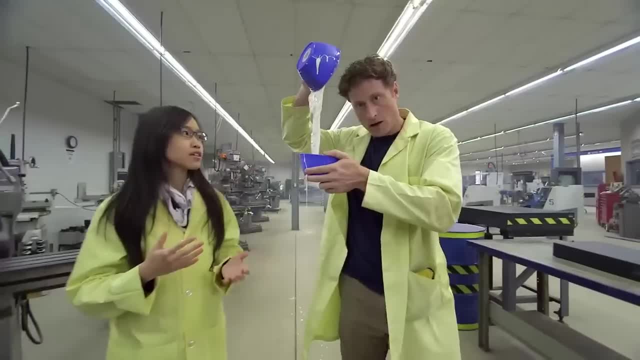 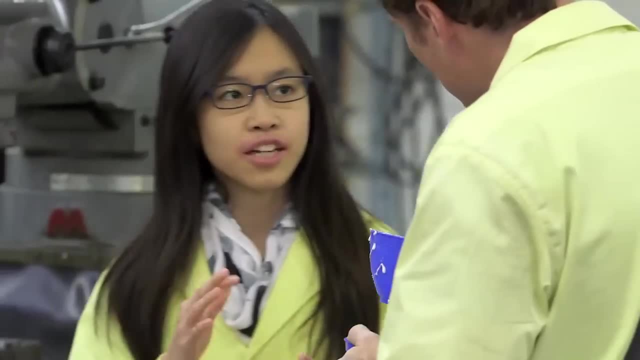 So when you're pouring it, the particles are still far apart, So they can't interact with each other, and so they stay a liquid. But when you're hitting it, you're jamming the particles together And they line up to become a solid. 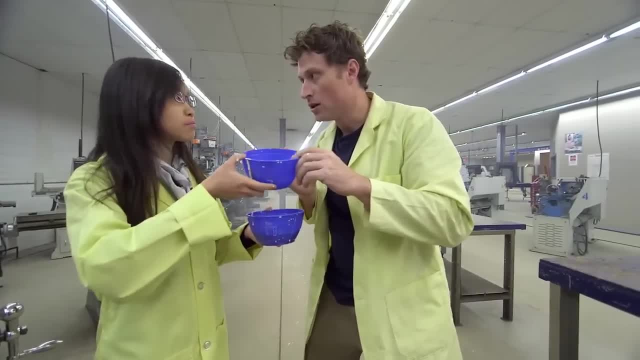 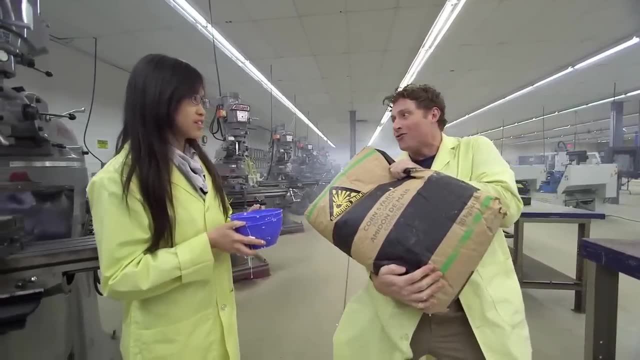 Now, does it still work the same way? if we have a lot more of it, It should. Great, Because I've got this 20-kilogram bag of cornstarch And I have 34 more of them. Wow, That's a lot. 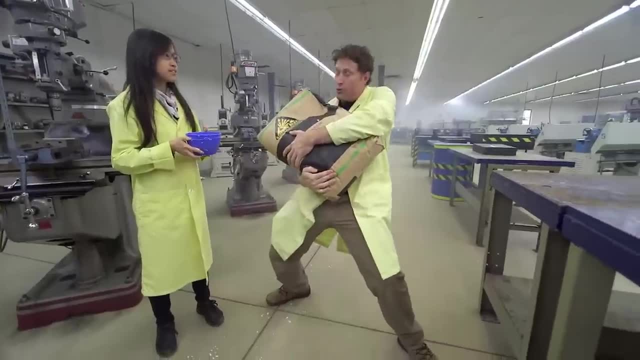 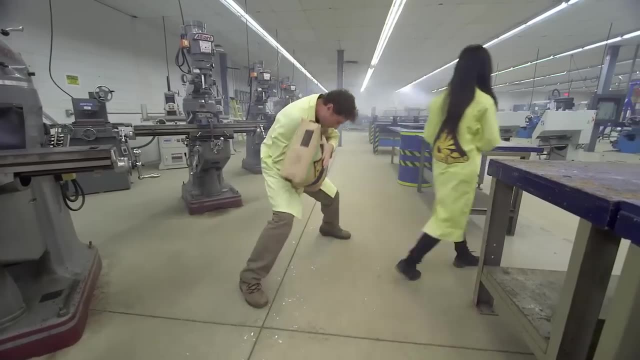 But I think you'll need a much bigger container, Much bigger container. Great, I got some wood over there. Why don't you go and I'll follow you. All right, I'll follow you, I'm coming, I'm coming. 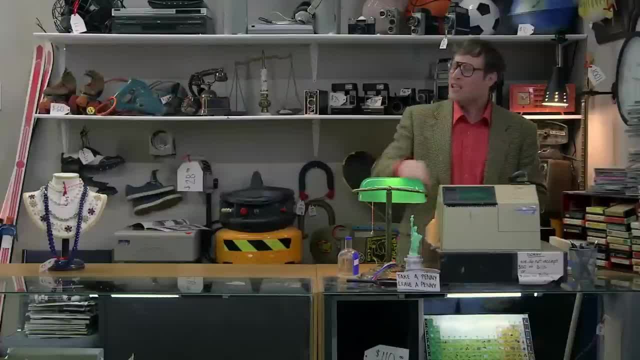 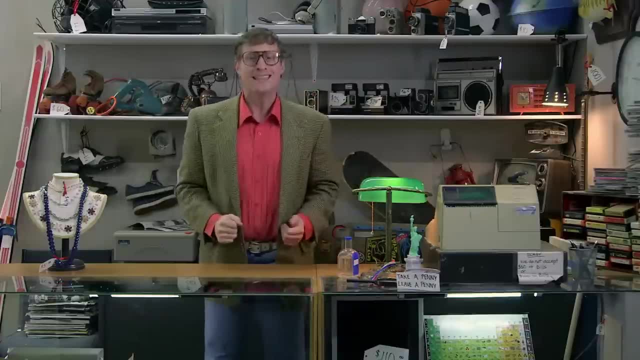 Yeah, Thanks, Ramona, And get me one of them fizzy drinks, Not too fizzy, Just sort of medium fizzy. Thanks a lot, Hello, Do you have trouble knowing what is a solid liquid or gas? Are you confused by jello? 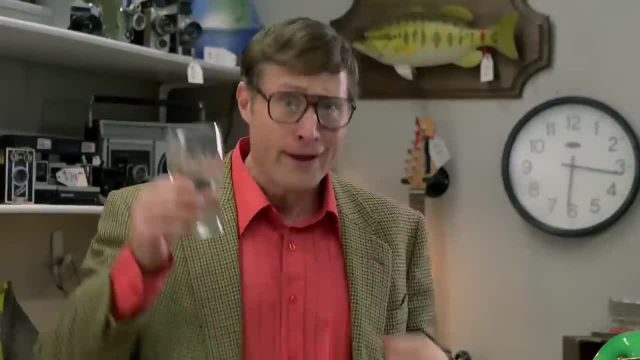 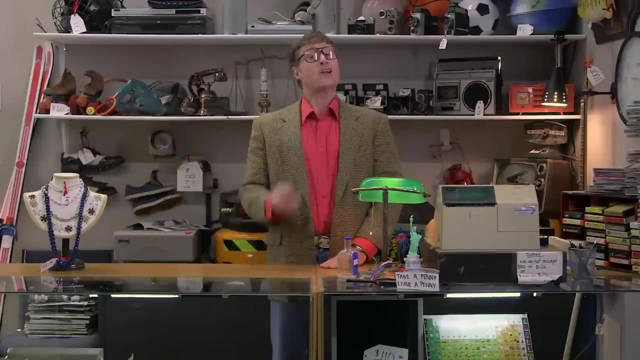 I mean, which is it? Is it a solid or is it a liquid? Water is a liquid, But what about when it's ice? Well, you've got to know your states of matter. There are three main states of matter: Solid, liquid and gas. 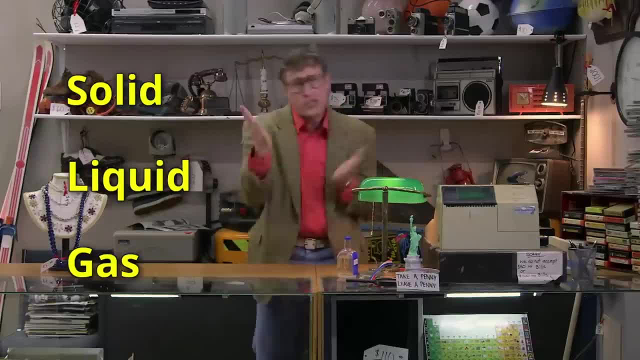 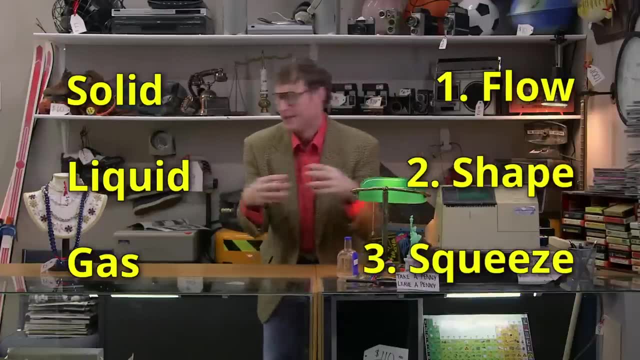 And there are three rules that you need to figure out. Which one of them is which. Does it flow? Does it fit the shape of its container And can you squeeze it? Rule number one: Does it flow Solid liquid gas? 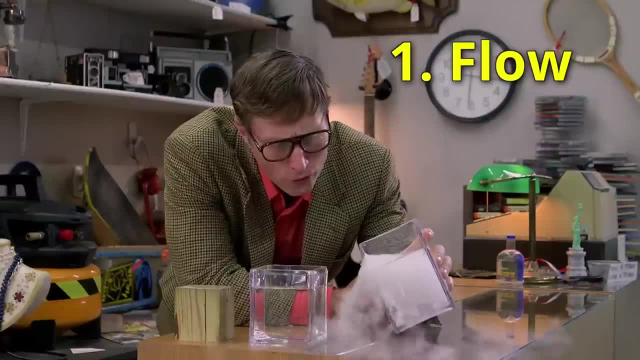 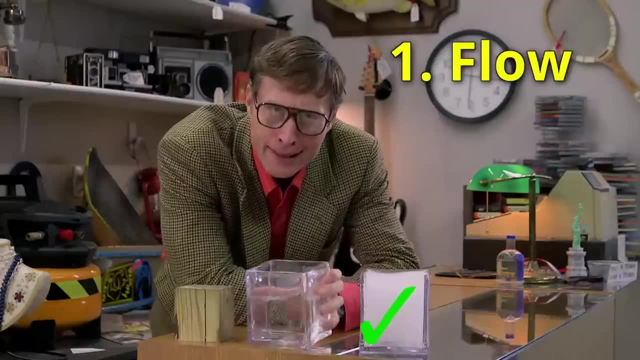 Here's a guess: Does it flow? Do the particles pour over each other and cascade down? Yeah, Yeah, they do. Does a liquid flow? Yeah, Yeah, it does. Does a solid Nope? Rule number two: What happens when you pour it in a container? 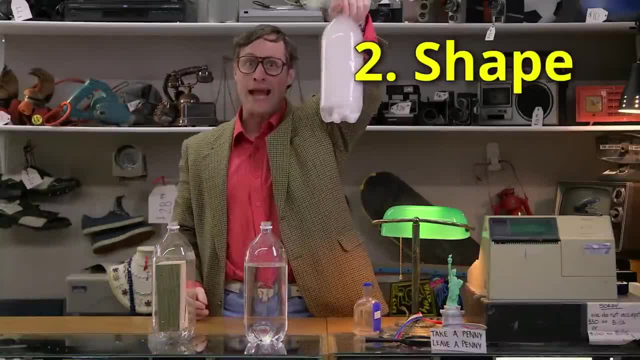 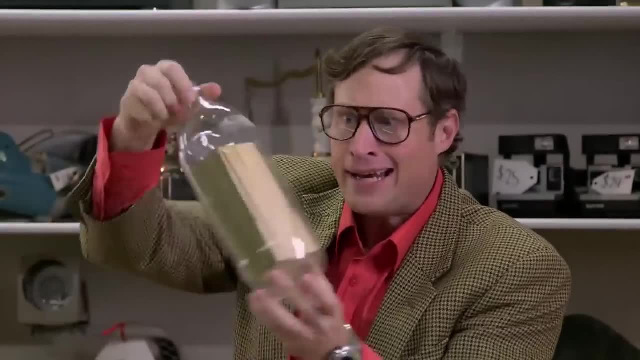 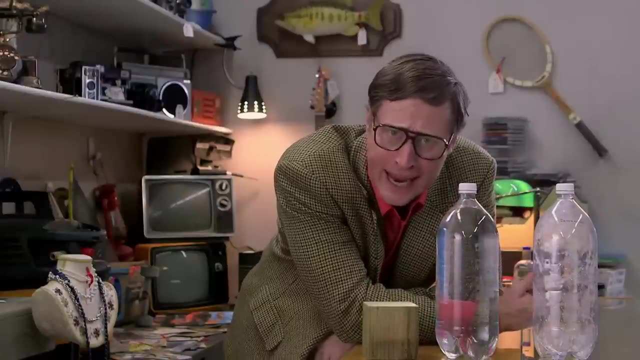 Does it take the shape of the container? Gases take the shape of the container. Liquids take the shape of the container. Solids do not take the shape of their container. No, I know what you're thinking. You're thinking I get the whole pouring and taking the shape of the container. 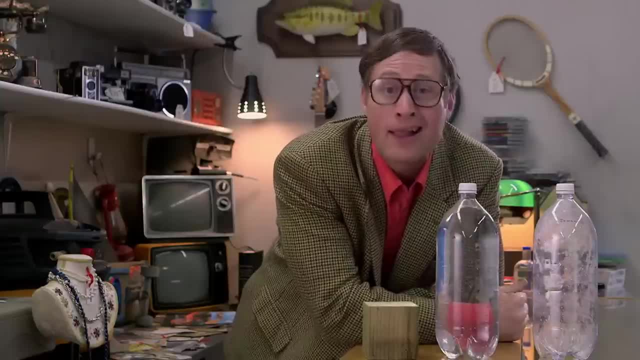 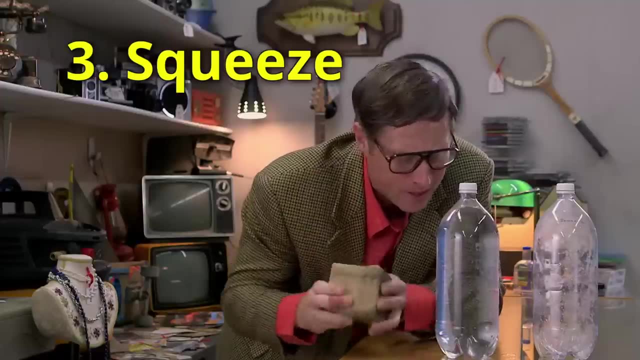 But come on Liquids and gases. they do both of those things. Well, it all comes down to rule number three: Can you squeeze it Now? solids, you can't really squeeze them. Liquids, you can't really squeeze them. 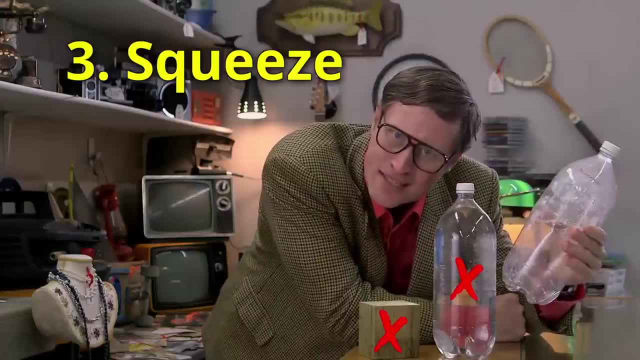 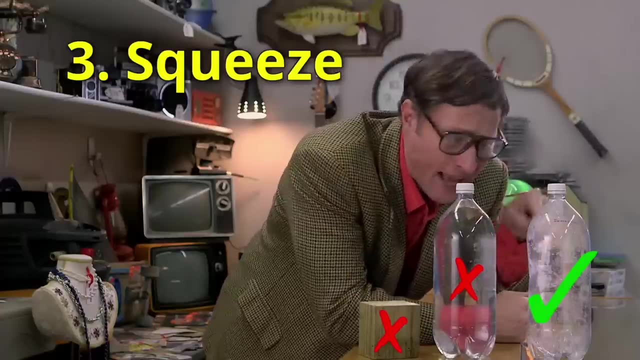 Gases, ha-ha bam, you can squeeze them. You see, gases compress Liquids and solids. they don't really compress very well. The other difference between gases and liquids is gases will take the shape and the volume of the container they're put in. 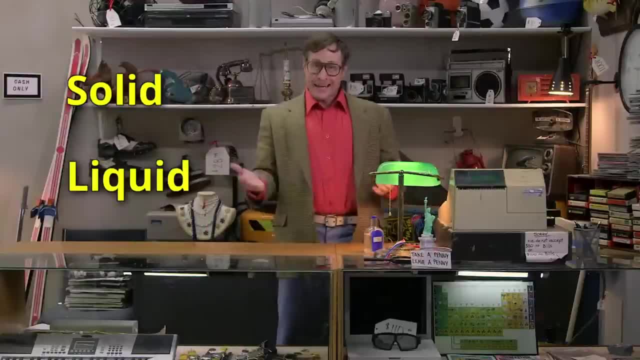 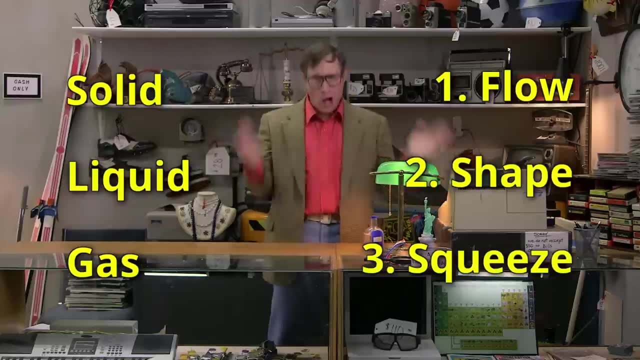 So solids don't do that. So there you go, Solid liquid gas And the rules. Does it flow, Does it take the shape of the container And can you squeeze it? Now you know your states of matter. That'll be $6.50.. 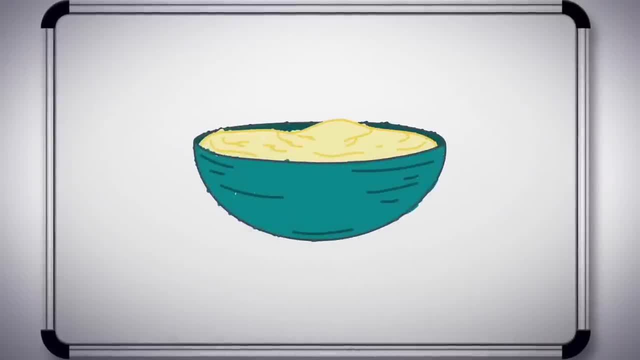 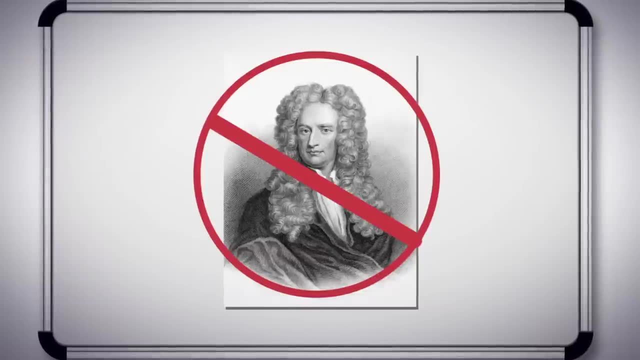 Cash only. So what is cornstarch mud and how does it work? Well, cornstarch mud is a non-Newtonian fluid, which means it behaves differently than you or Newton would expect. Here's cornstarch And here's water. 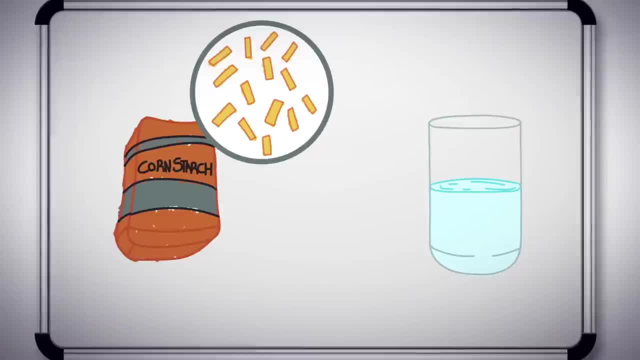 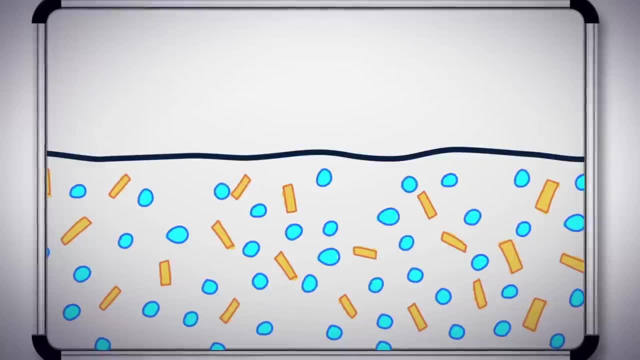 Cornstarch is made up of large blocky molecules like this. Water is made up of much smaller, rounder molecules like this: When you put them together, it looks something like this: It all has to do with how the molecules slide past each other. 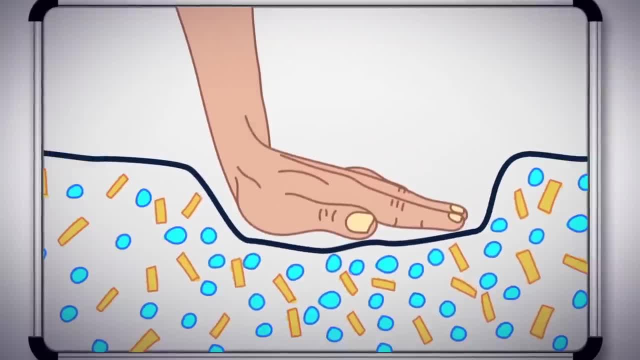 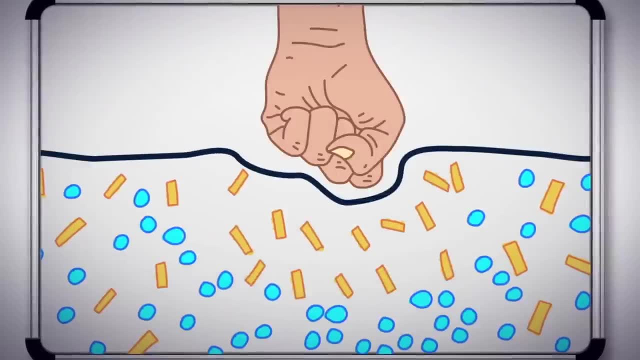 When you put light pressure or slow pressure on the mud, the water molecules and cornstarch molecules have time to shift out of the way. But when you put a sudden pressure on it, the water molecules squirt out of the way, but the cornstarch molecules don't have enough time. 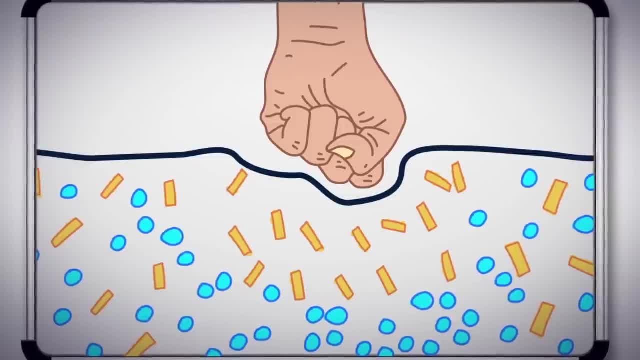 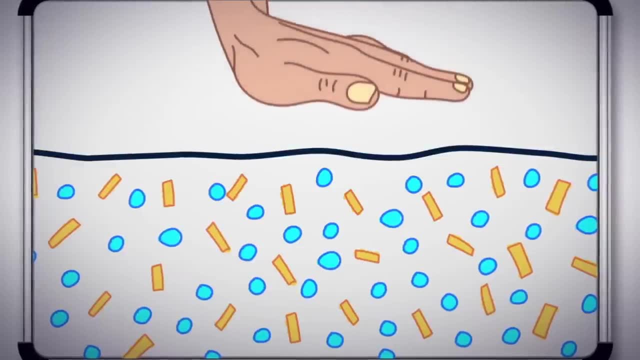 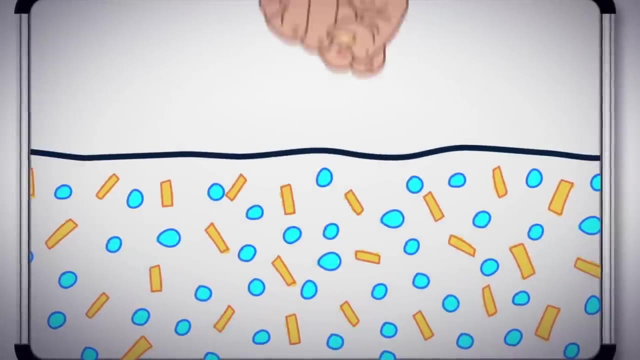 So you get a section that's nearly all cornstarch, which acts as a solid Cornstarch. mud is a shear, thickening fluid. Shear is talking about the force of things sliding around, In this case the molecules. So when the shear force is strong, 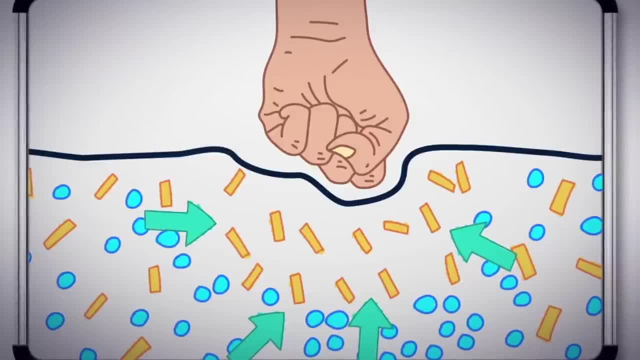 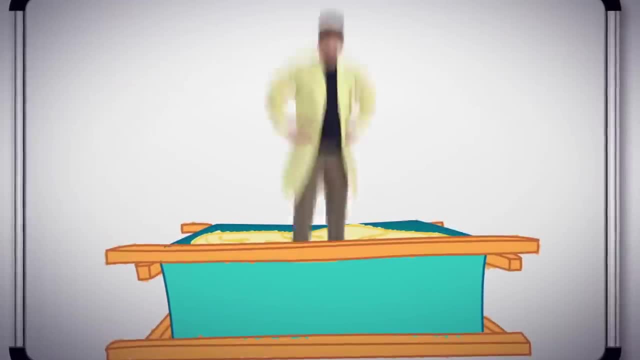 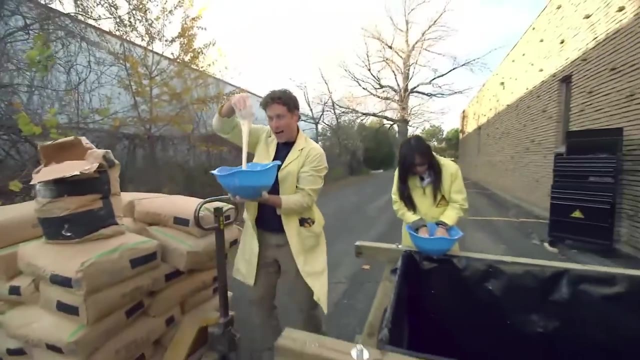 the fluid thickens, Shear thickening. So here's the plan. If Judy and I make enough cornstarch mud, could we run across it? Let's find out. Yeah, I think mine is just the right consistency. How's yours, Judy? 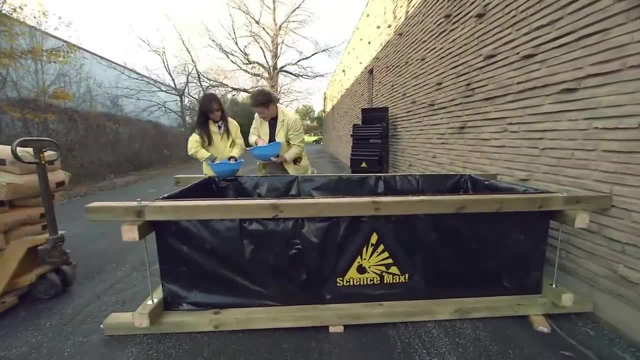 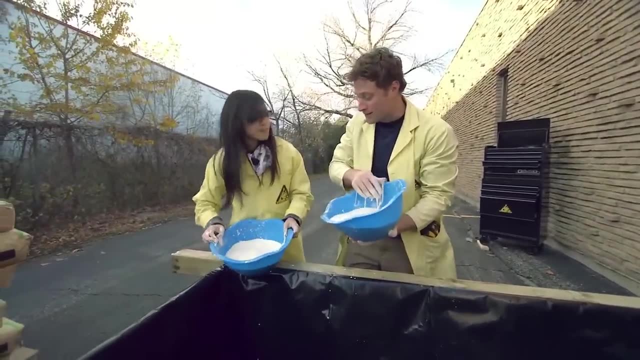 I think I'm ready too. This is much harder than I thought. Yeah, it's really hard to get it mixed at the very beginning, but mine is ready to go. Okay, here we go, first batch. You ready, Yep. 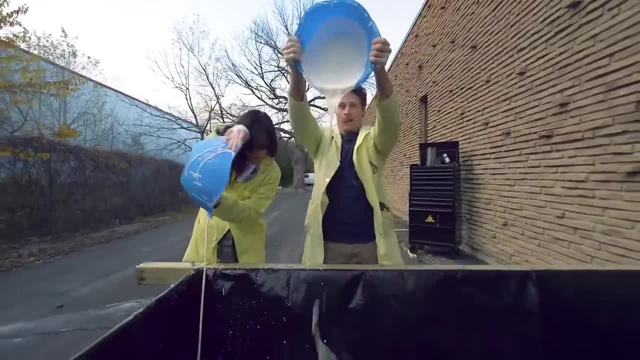 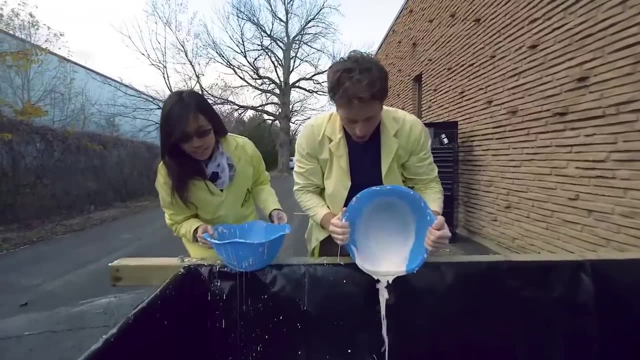 Dump it in Whoo, Whoo, Whoo. Hmm, I thought that would be more. I thought so too. It's really not filling this up very much, is it No? Huh, that's a lot of cornstarch. 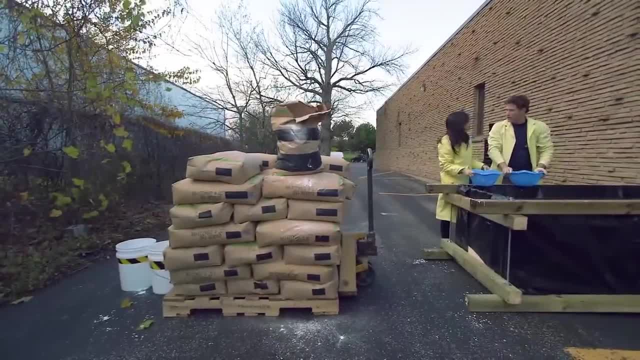 This is um, this is great, but I think we're gonna have to go a little faster than this. I think we need some sort of mixing device. Yeah, I mean, we don't have to do this by hand. We can get some sort of machine to help us. 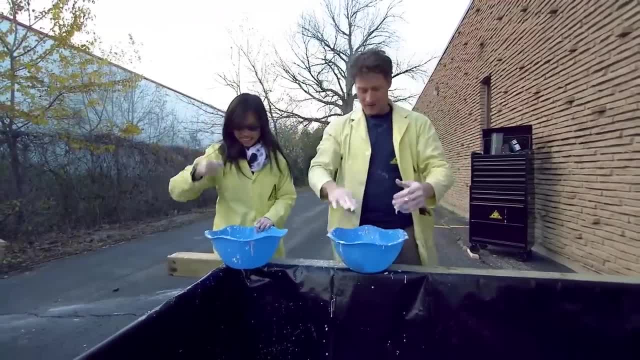 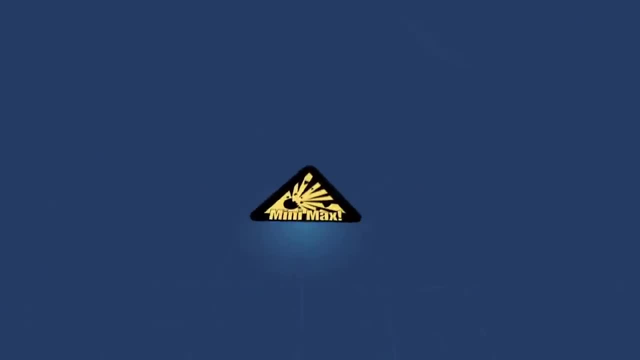 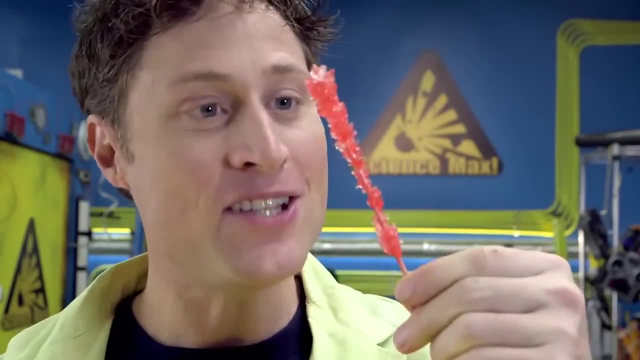 Yeah, Right on high five. Oh, We shouldn't high five when we have this stuff on our hands. Nope, Actually, it's really not very difficult. Mmm, this science is delicious. This is rock candy. It's basically crystallized sugar. 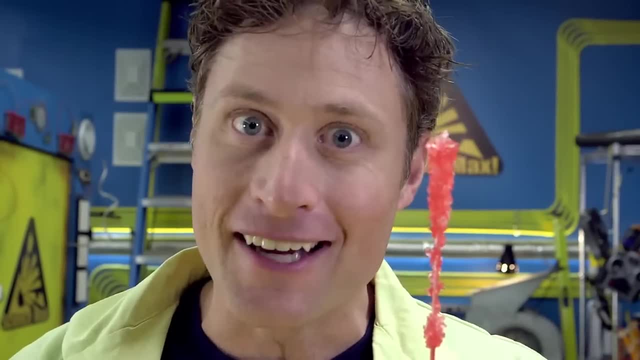 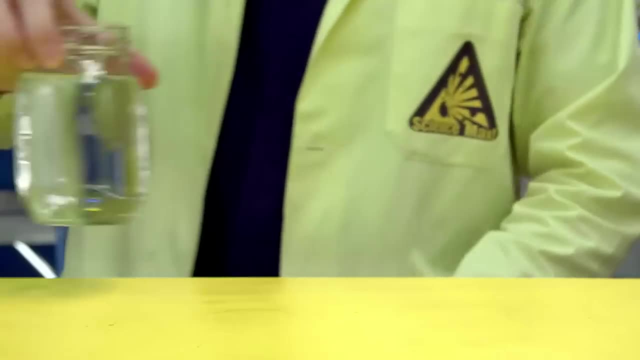 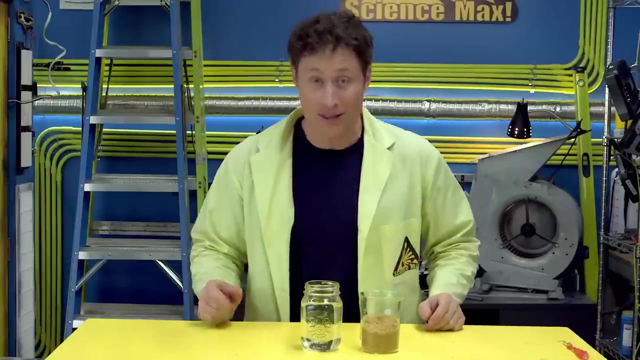 And you make it by turning a solid into a liquid and then back to a solid again. Here's how you can make it at home. You need a container that you're not gonna need for a while and some water, some sugar, brown or white- I like to use brown- and an adult. 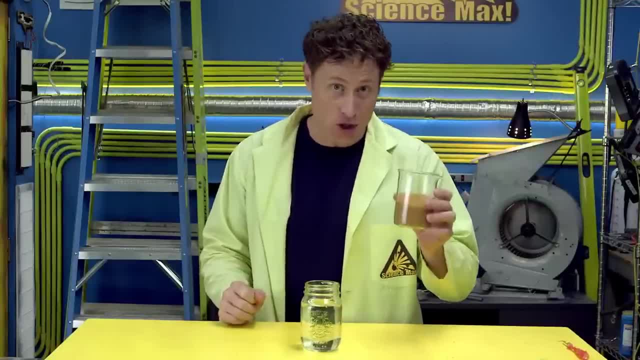 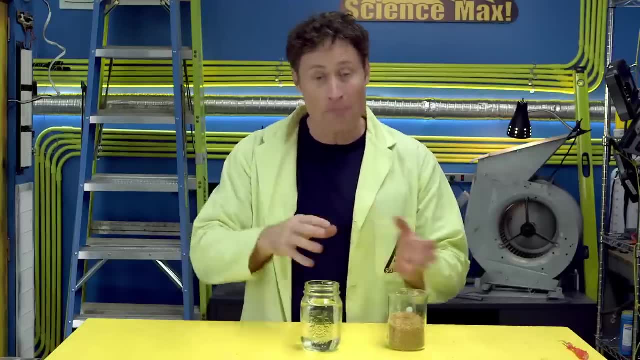 Here's why you need an adult. You want to dissolve three cups of sugar into every cup of water, and you can't do that unless you heat the water. So get an adult, a saucepan and heat the water up, pour the sugar in and keep stirring. 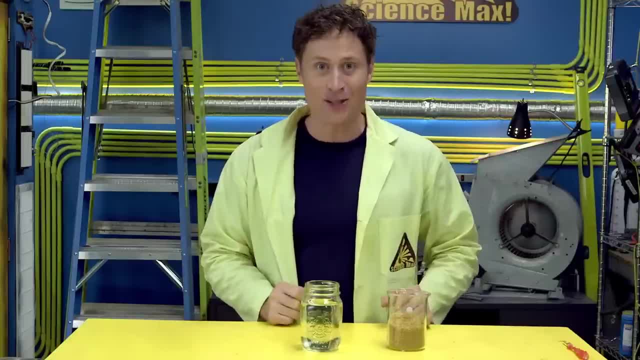 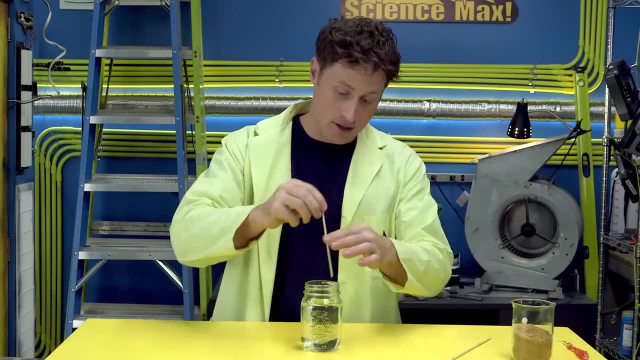 until it's all dissolved, Then pour it in your container and let it cool down. Then you'll need a shish kebab skewer, which is something you can get at the grocery store. Cut it down to the right size so it fits nicely into your container. 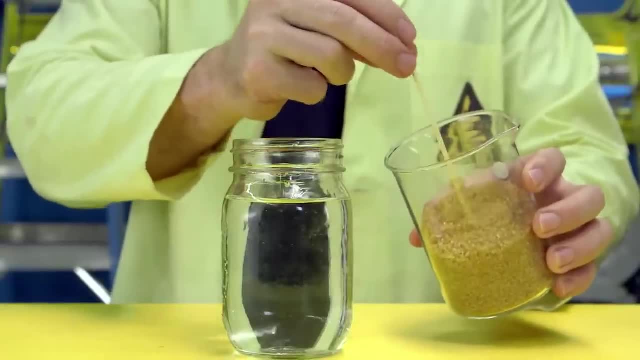 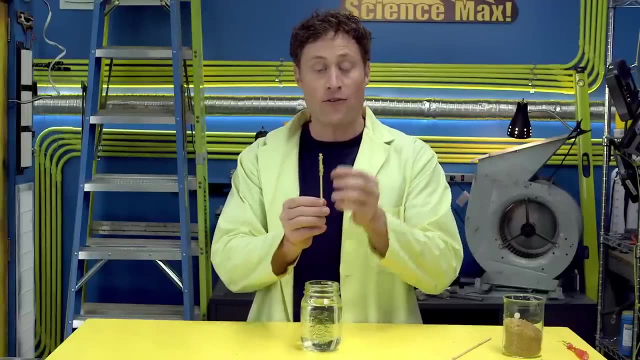 and then dunk it in your sugar and get some crystals coated around the stick. These are seed crystals and they get the whole process started. And now you have to wait for these to dry, otherwise they'll just fall off the stick when you put it in the water. 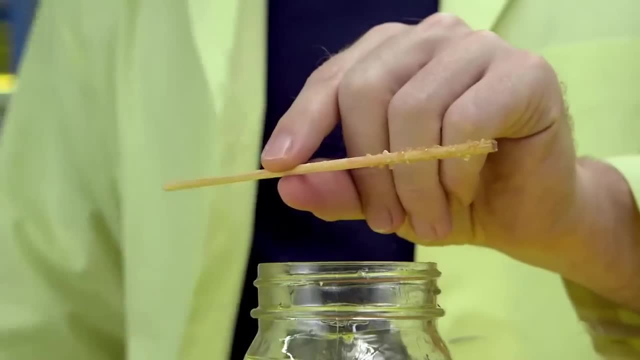 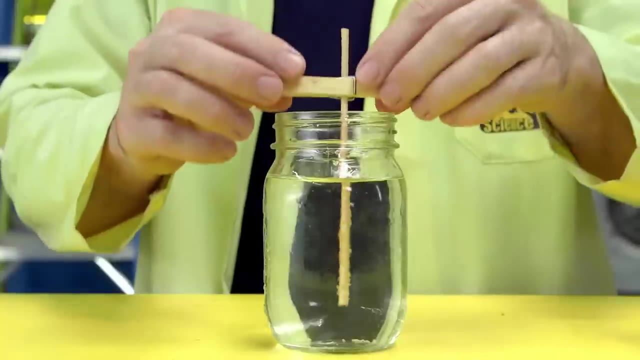 So I've got one here that has dried out. You'll also want something to keep it from falling in the top of the container, so I'm gonna use a clothespin, Put it in there and dunk it in the container like that. And now for the final step. 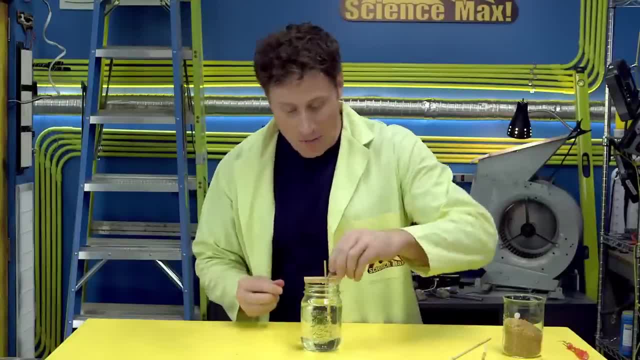 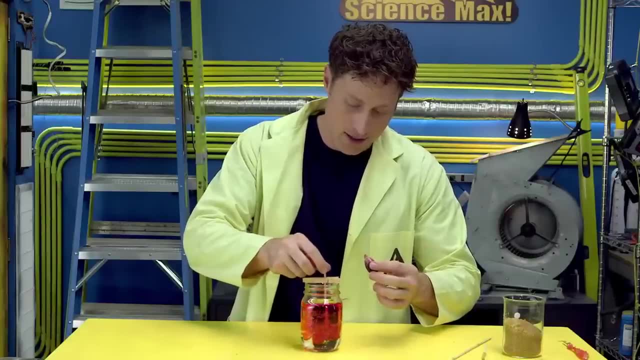 if you want, you can add food coloring. I like to use red because it reminds me of science, And I'm gonna use the stick to actually stir that up a little bit. There we go Now: the dissolved sugar crystals in the water. 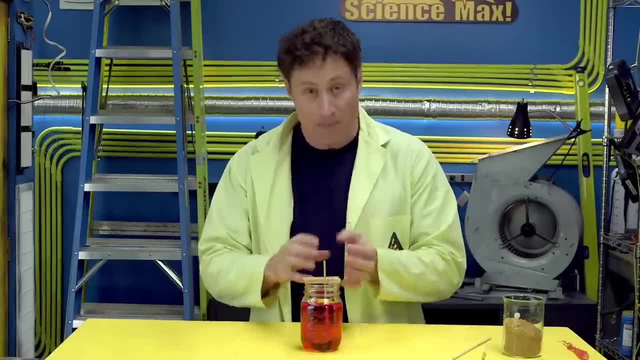 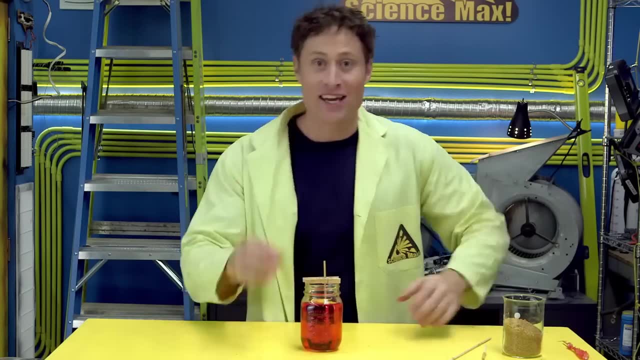 will slowly grow on the crystals that are already attached to the stick and it will eventually grow into a rock candy pop. But it takes about a week. No, I'm just kidding. I've already got one that's standing by. Here we go. 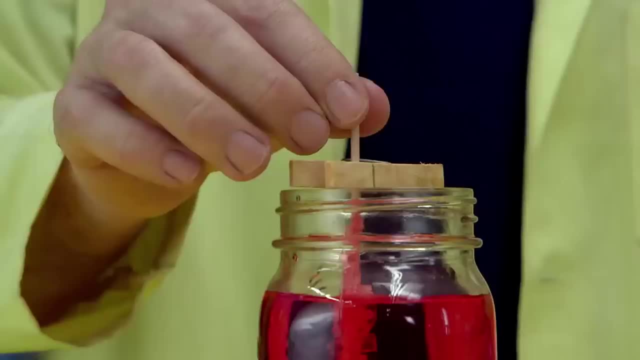 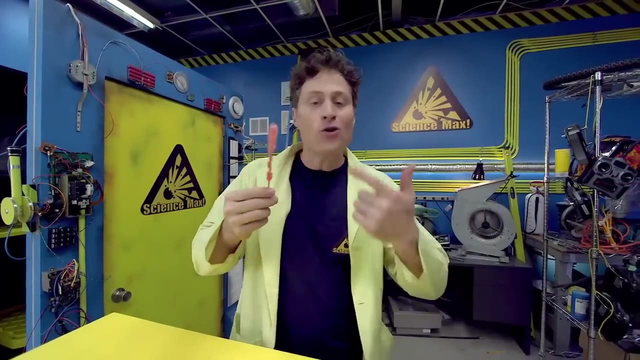 This one. This one has been growing for about seven days And there you go: Rock candy, Delicious science. Now, how can we make this any better? I mean, it's crystallized sugar. It doesn't get any more maxed out than that, does it? 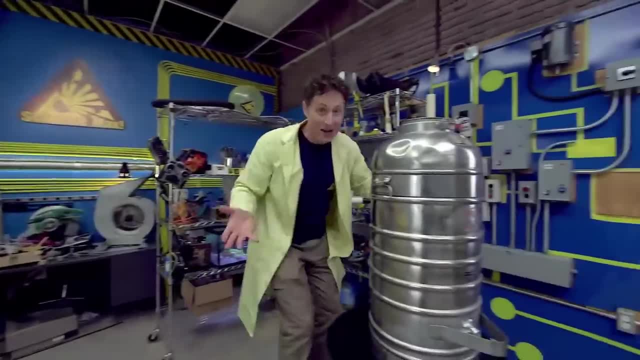 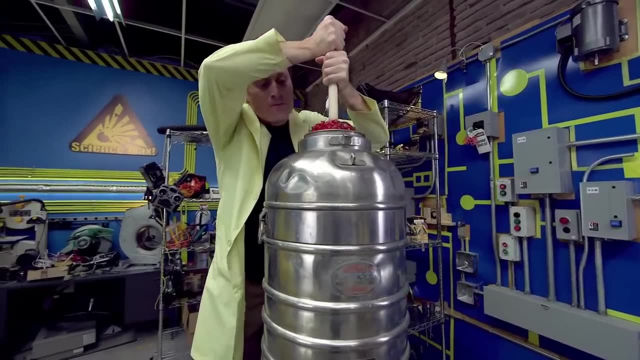 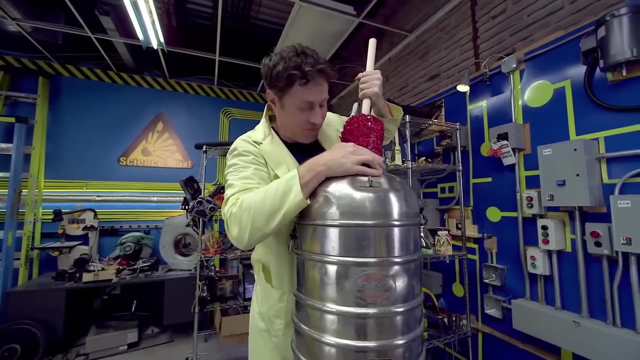 Yeah, it does. Come on, This is a giant container of sugar water and I've been brewing a massive rock candy crystal in it for a while, But it's sort of It's sort of getting a little bit too big to fit out the top of the container. 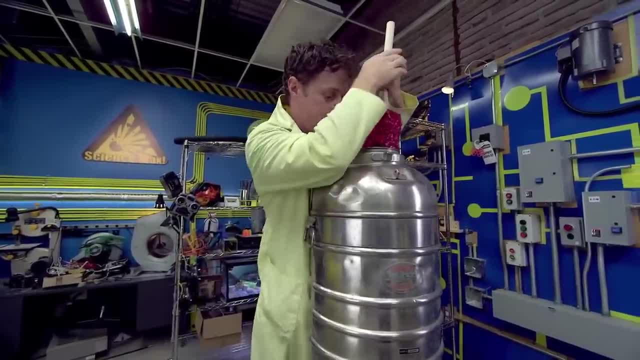 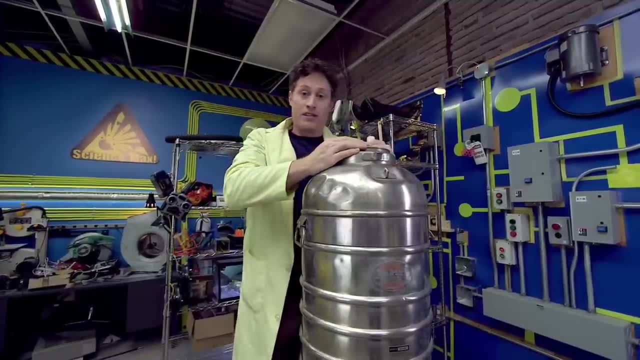 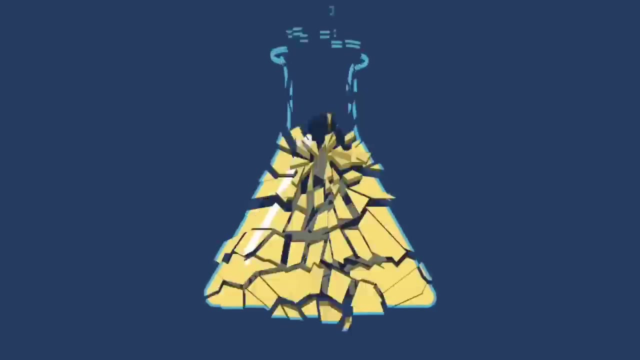 So you know what? I'm just going to put that back in there And chalk that one up to science, Because, well, eating a rock candy crystal that big would definitely not be good for my teeth. So yeah, So our big experiment is to take a whole lot of corn starch. 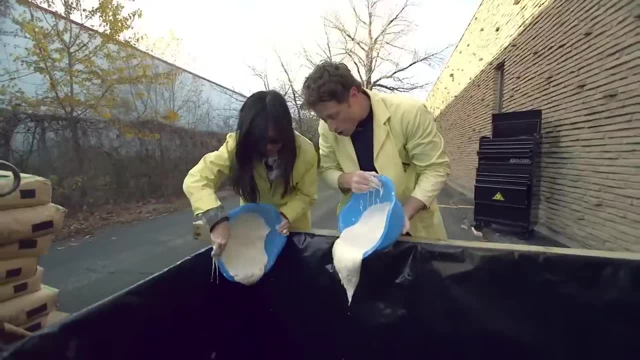 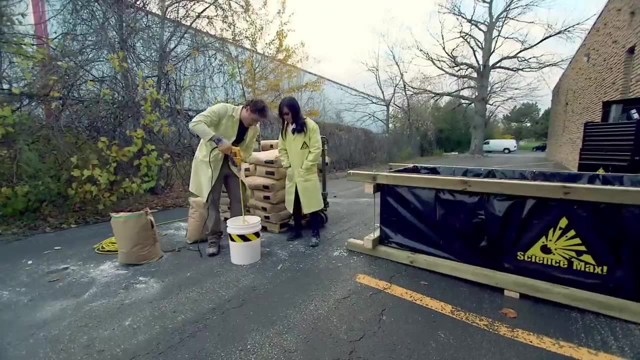 and fill a trough to see if we can run on it. But mixing it by hand was going to take forever, So Judy and I got a drill with a mixing attachment on the end. Whoa sorry, All right. so, Judy, I'm noticing a bit of a problem here. 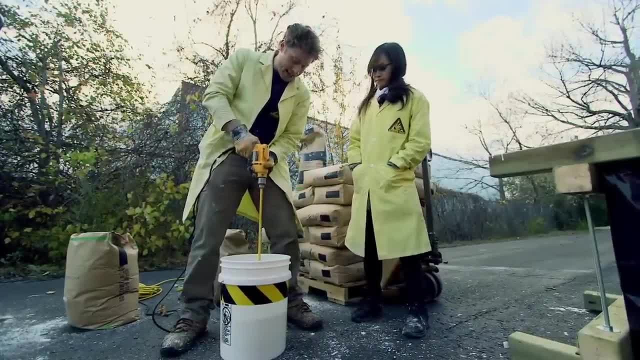 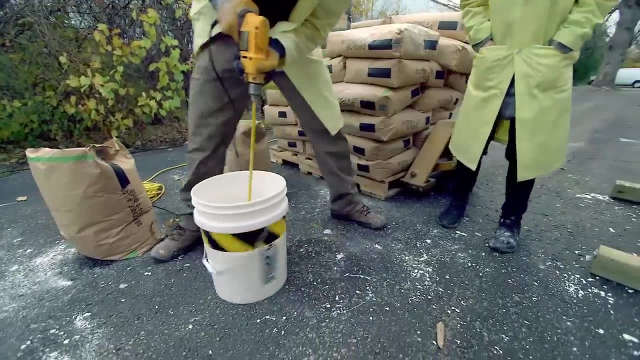 What is it? Well, if I mix at the top, everything's fine, But as soon as I get it a little bit deeper and then it gets really tough and the whole bucket starts to spin and the drill stops. Yeah, I think it's because the drill's. 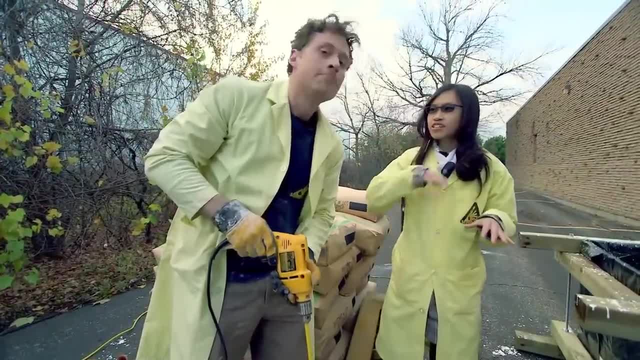 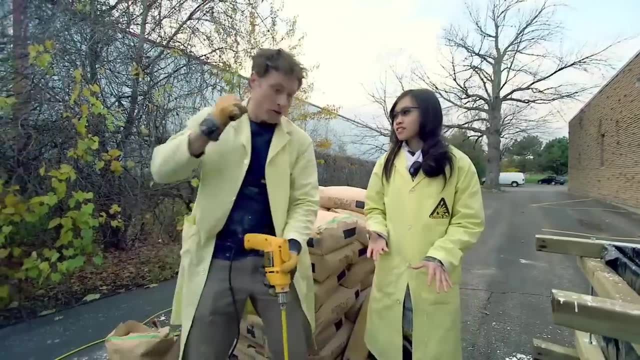 trying to mix it too fast. When we're mixing it by hand, it's slow and you can still let it stay a liquid, But now you're just making it a solid Right because it's a sheer thickening fluid. So if you hit it really quickly with something, 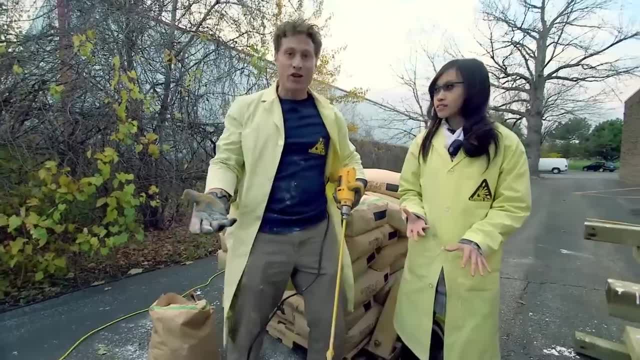 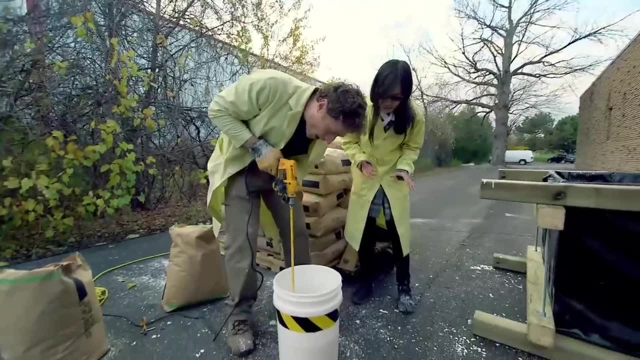 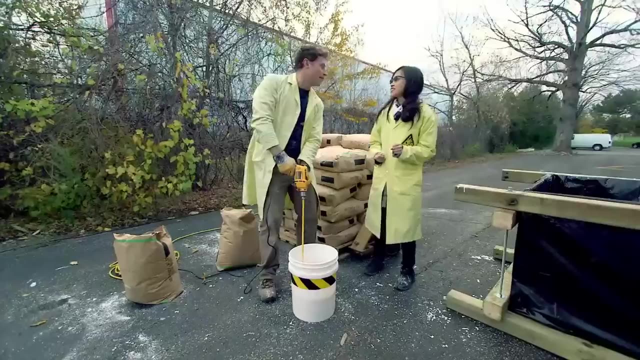 like the blades of this spinning really quickly in the thing, it'll suddenly turn into a solid and it'll be really hard to mix. So we go slow, Going slow, Going slow, Suddenly realizing that if we go slow we'll be here forever. 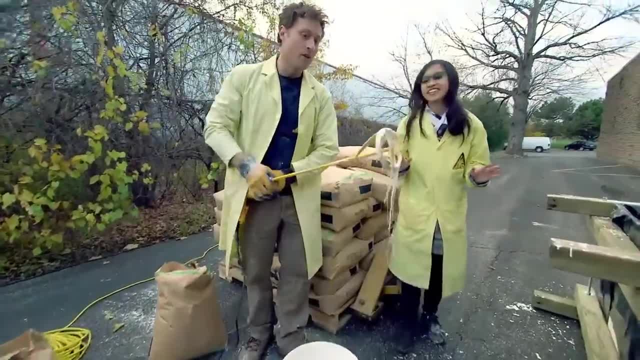 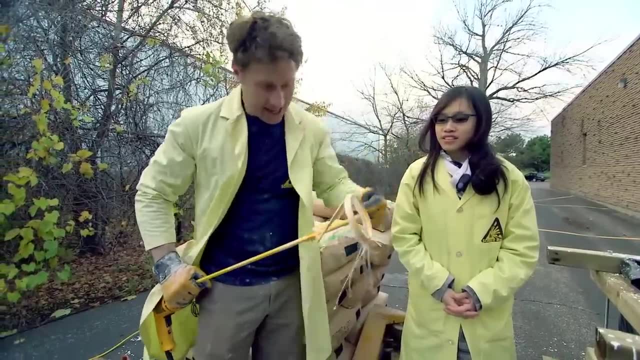 Yep, You know what I think we need. Oh, sorry, You know what I think we need. We need a different way to mix this Yep. We need a way to mix more of it and we need a way that it doesn't hit it with blades. 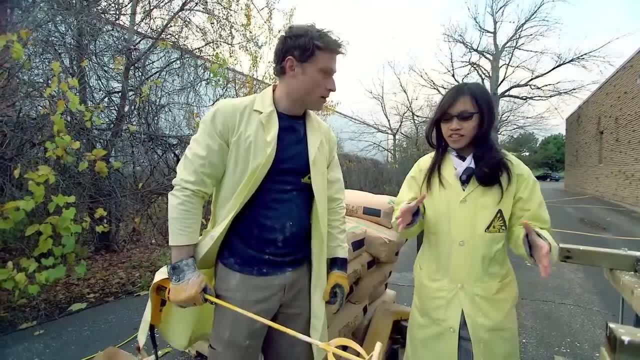 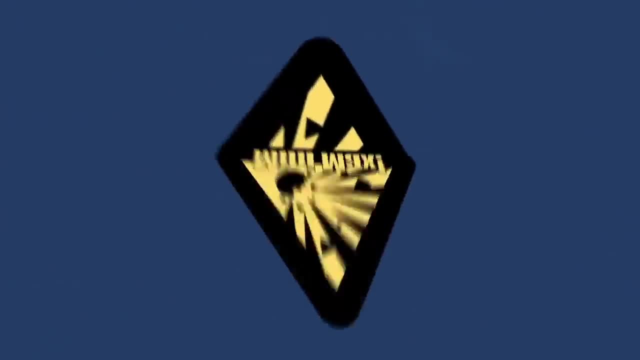 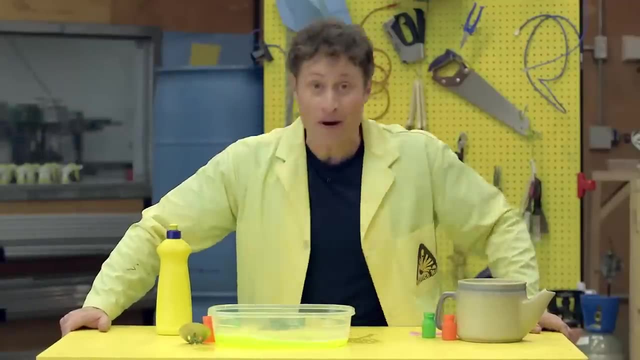 that suddenly go through it really quickly, Something that can mix on a large scale, but slowly. I have just the thing. Come with me, All right. The interesting thing about this is when you think about bubbles, is there a gas surrounded by a liquid? 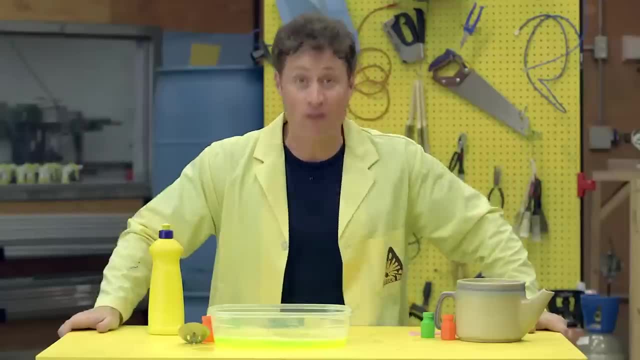 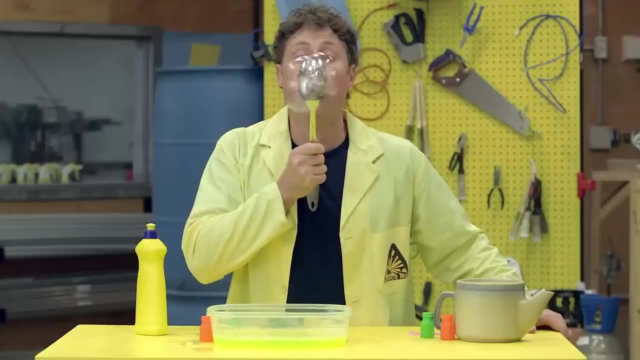 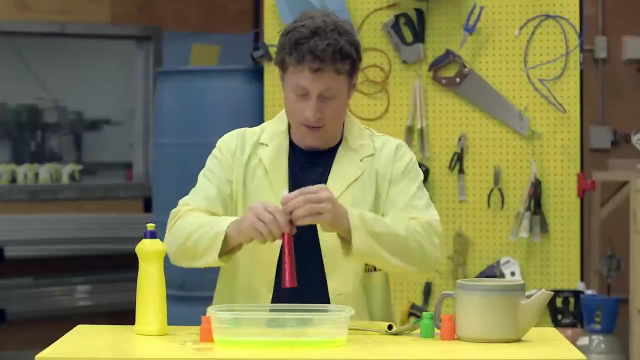 So get some dish soap and some water and then be science maximites and find things around the house that you can make bubbles out of. Just about anything that has holes will do Or mm-hmm, Or I like this one. 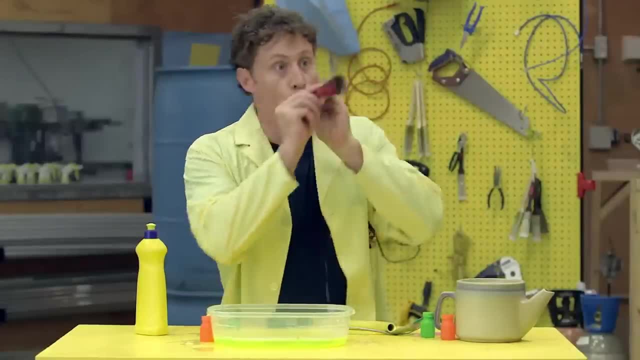 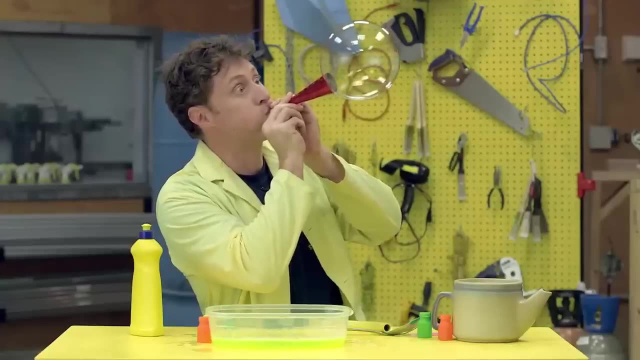 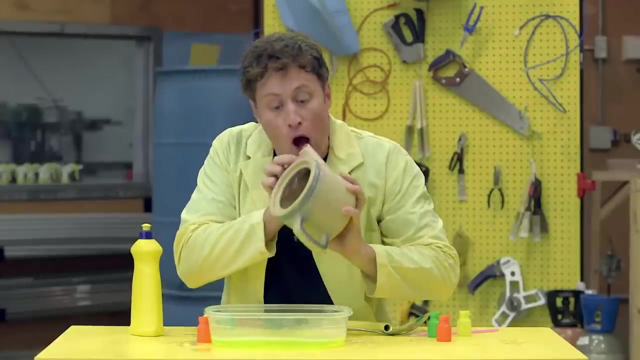 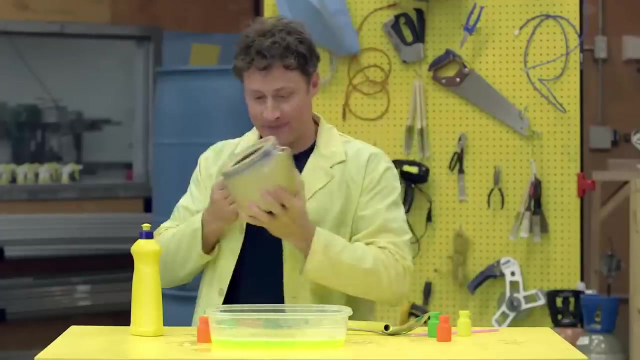 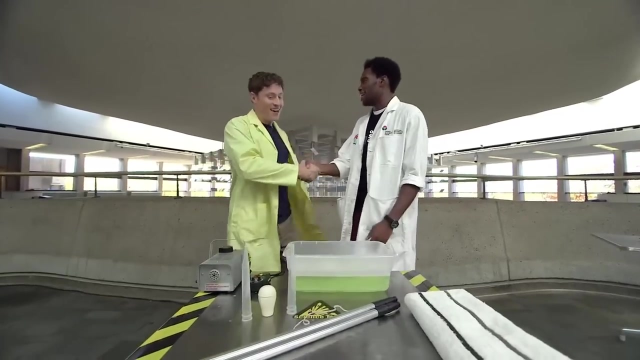 I call it the loud bubble. It makes bubbles. Or Now it's time to max it out. I'm here at the Ontario Science Centre And this is Anthony. Hey, Anthony, Hey, how's it going? Good, So you are amazing at bubbles. 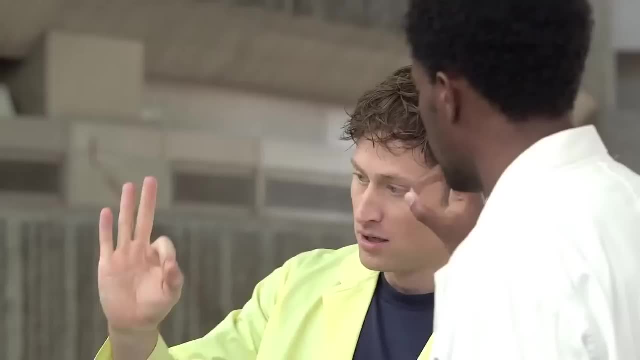 I am. I've been practicing for a while. You're gonna make an okey-dokey sign like this: You're gonna dip it right into our bubble solution. Come on, get right in there. right in there. Make sure you get it all up. That's a little too much. 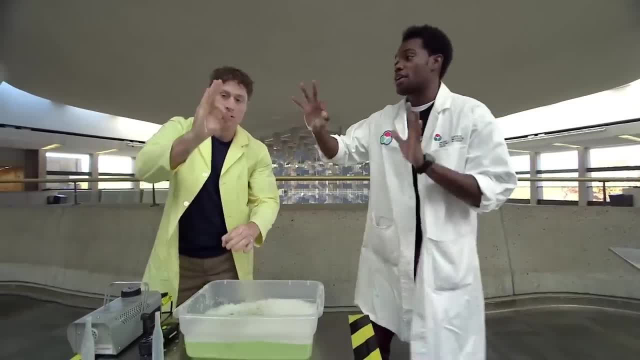 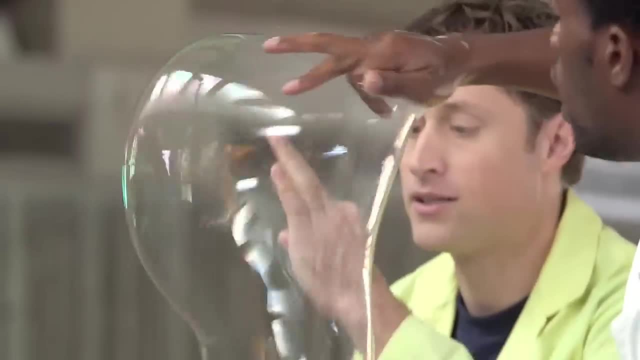 Well, I can make two, And then you're gonna keep that okey-dokey sign. You're gonna blow very gently Nice. I brought these two giant sticks here and I don't know if you noticed, but I've got a smoke machine here. 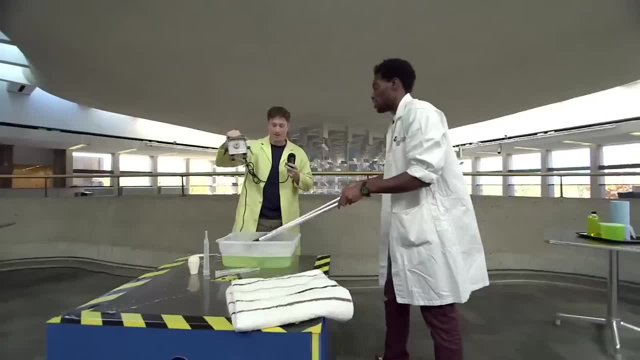 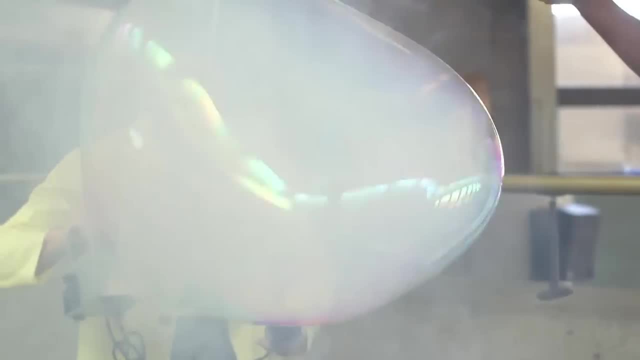 Right, So we'll turn that on And then if you press that green button there, it's gonna shoot some smoke and we're gonna try to catch that smoke in a giant bubble. You ready? Okay, I'm gonna try to. 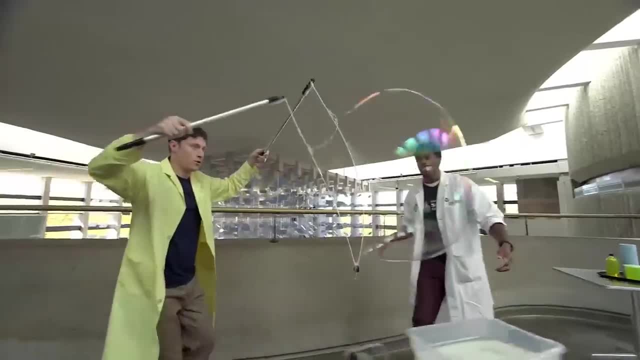 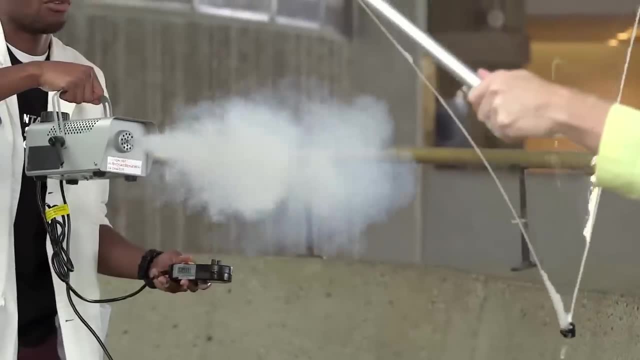 Oh, that was so close. Did you see that one? You give it a shot, Nice, Oh, check that out. That was amazing, That was huge. Try it again. Let's see if I can get the smoke machine Here we go, Go for it, go for it. 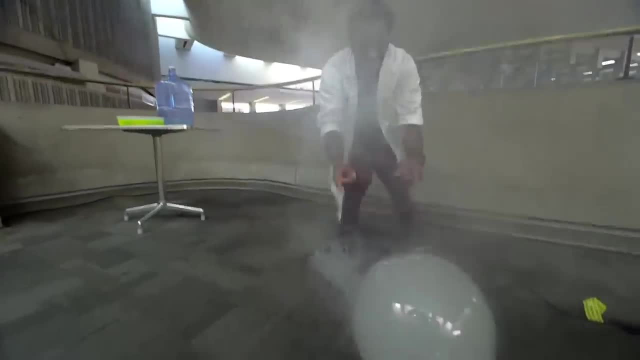 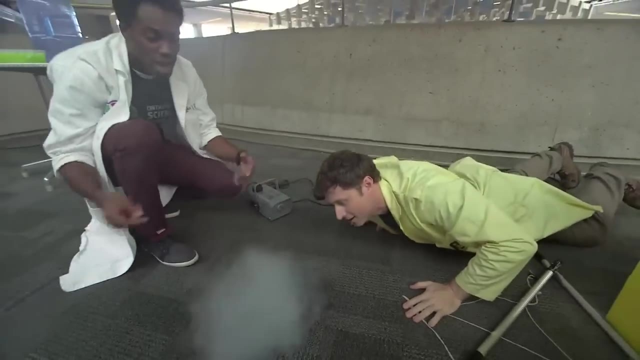 Push right towards. Oh, check that out, You did it. Look at that. Look at that smoke And it bounces on the floor. because the floor it doesn't have any oils on it. Isn't that amazing? That was great. 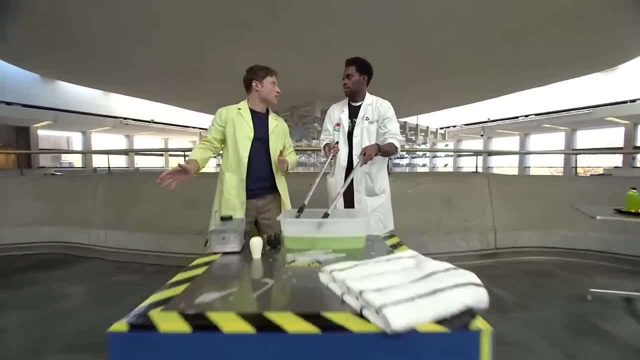 That was so cool. That was great. You know what I think we should do? What's that? Giant bubble tons of smoke Done. Okay, here we go, Let's do it, You ready? Giant bubble, tons of smoke Go. 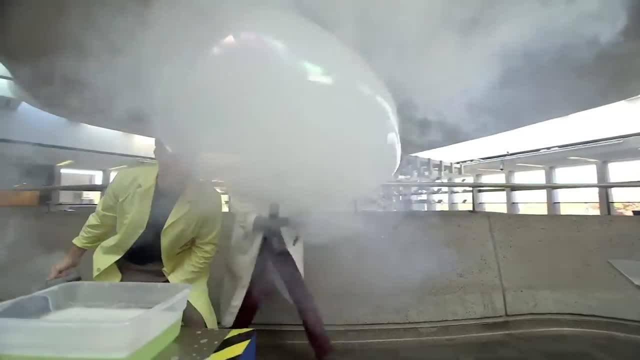 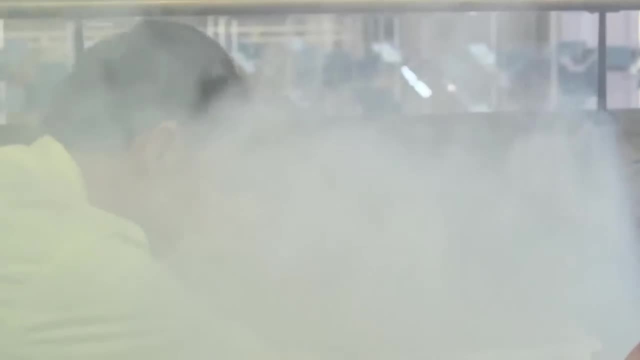 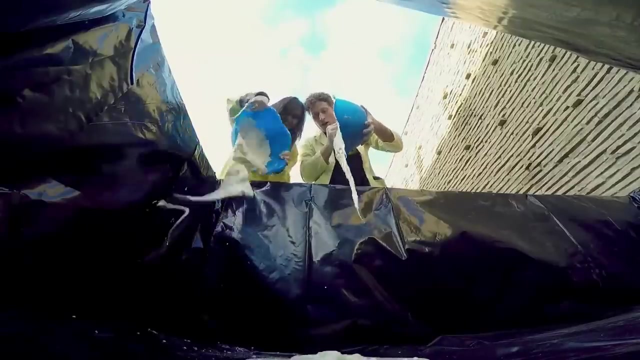 Awesome, Look at that. Look at that, That's crazy- Maxed out bubbles. Well, there you go: Giant, smoke-filled bubbles- Awesome. Yeah, Judy and I started mixing the cornstarch mud using a drill with a mixer attachment. 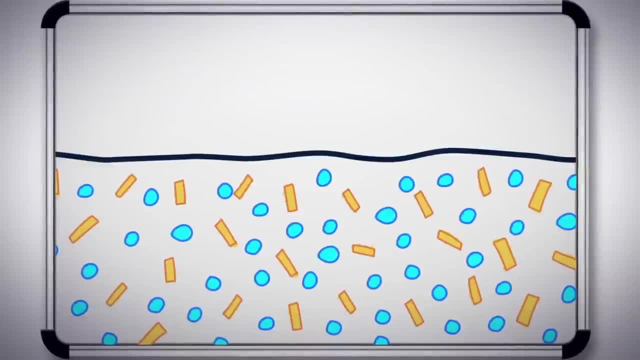 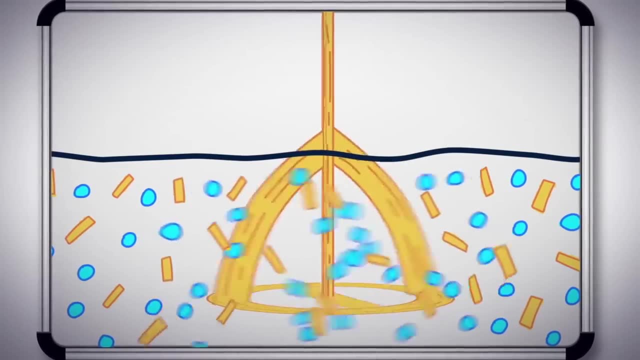 But it didn't work. We should have known better. Here's the mixer in our cornstarch mud. Usually a mixer works by going really fast and mixing everything together, But remember that cornstarch mud is a sheer thickening fluid. 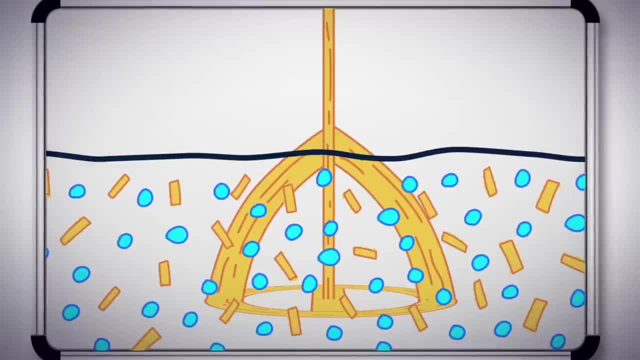 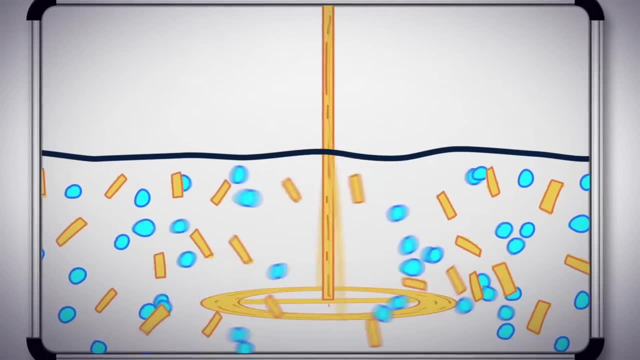 So when the blades of the mixer tried to go fast through the cornstarch mud, it did what it always does: Turn solid. The faster and harder you try to move it, the more solid it will become. This means the only way to mix it. 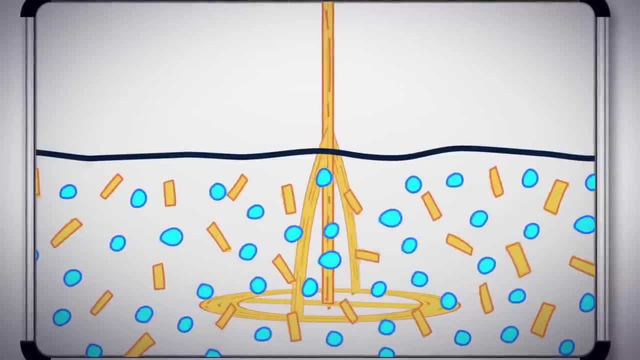 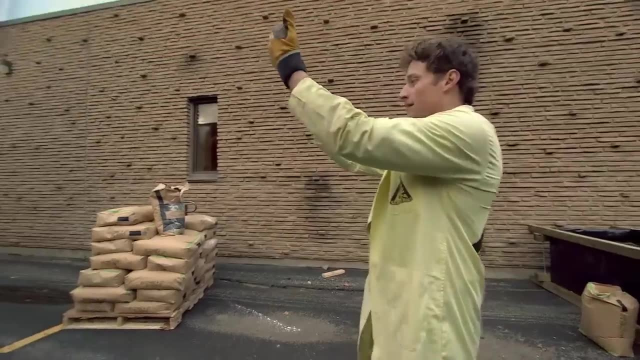 would be if we made the drill go very, very slow, Which wouldn't speed things up at all. So, with the drill and other lost cause, Judy and I need the biggest thing around that could mix stuff up. Come on back Good. 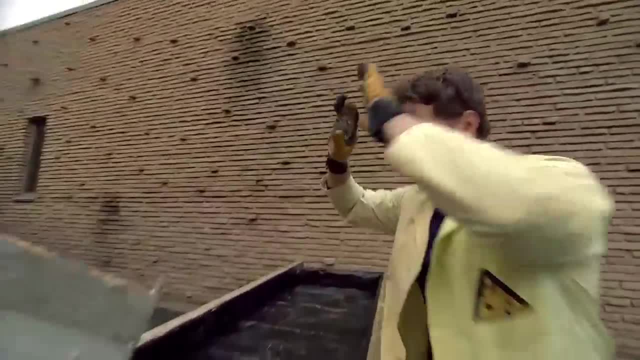 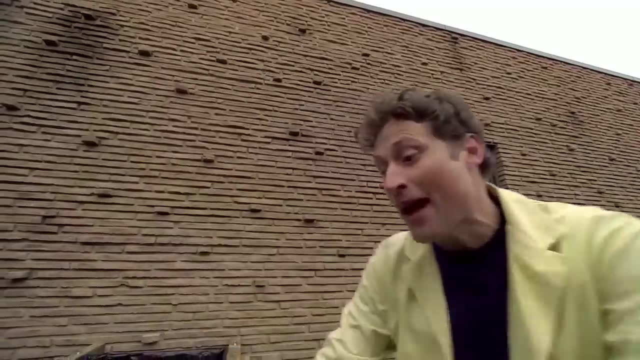 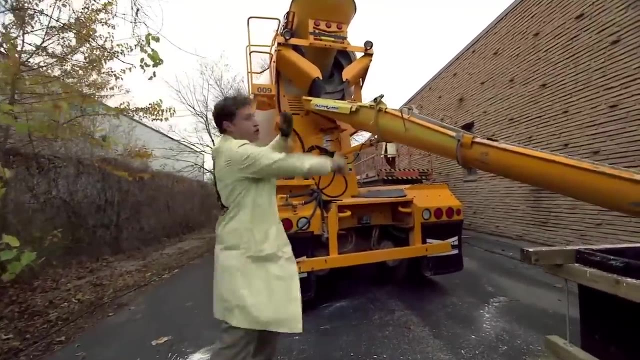 Little bit more. Perfect, A cement truck. A cement truck is the perfect thing to mix, because all we have to do is get all the cornstarch up in here and it'll mix it, and it doesn't move it too fast. It goes nice and slow. 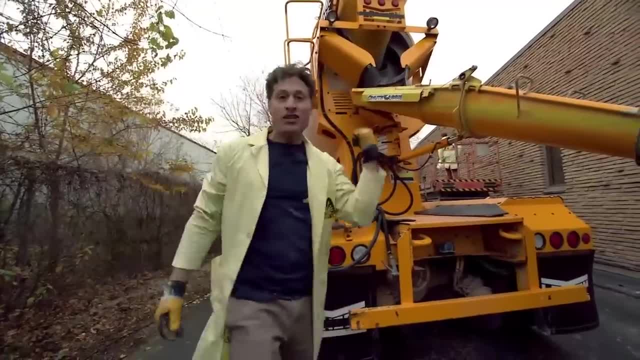 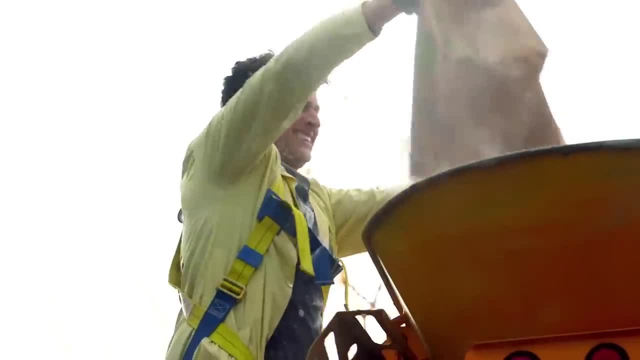 so hopefully a sheer thickening fluid will be fine. I'm gonna get Judy. She's driving the truck. Hey, Judy, that's perfect. The only problem is we needed to get all those bags of cornstarch into the hopper of the cement truck. 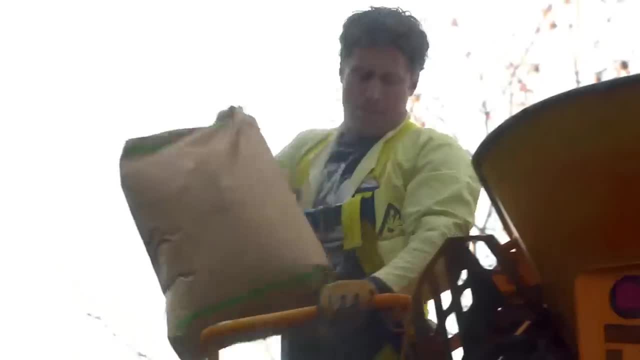 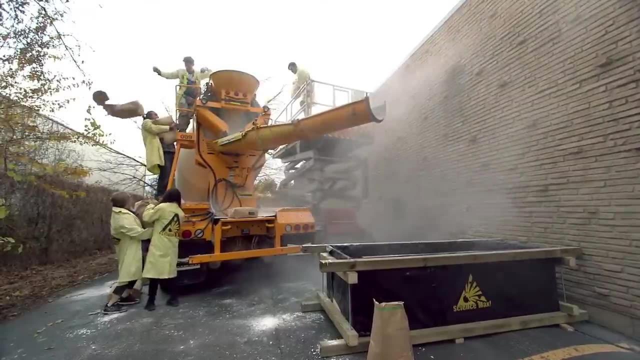 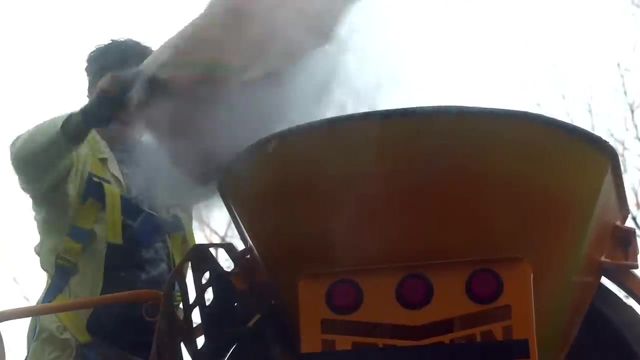 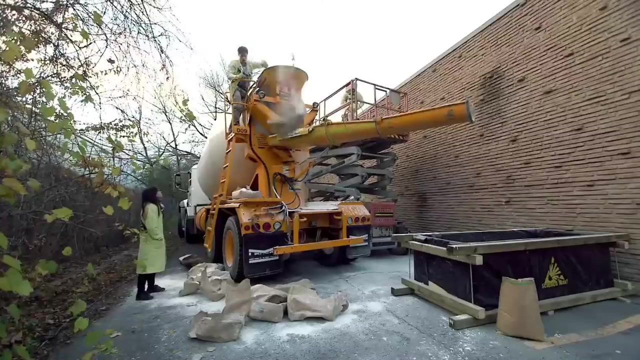 How could it be this messy? We needed to call the entire Science Max build team to help us out. This is possibly the messiest thing I've ever done- Awesome. Hey, Judy, you wanna lift up any bags? I'm okay. thanks, That's okay. 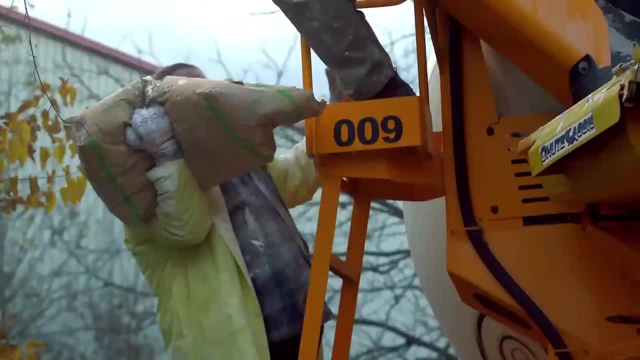 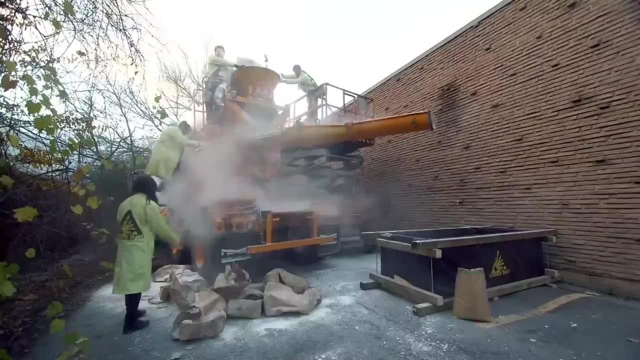 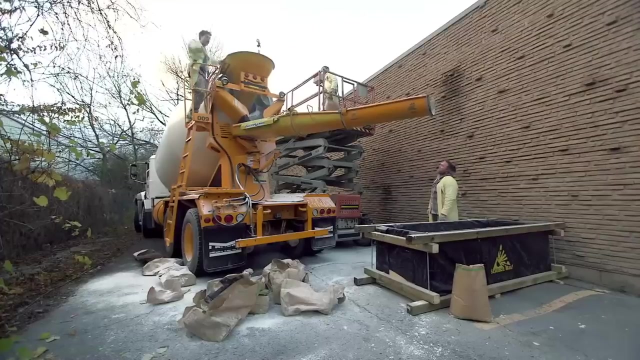 I'm having a lot of fun, so I can do them Cool. Oh no, Oh no, Oh no. I got most of it. I got most of it. Alright, I think we're done. I think that's enough bags. 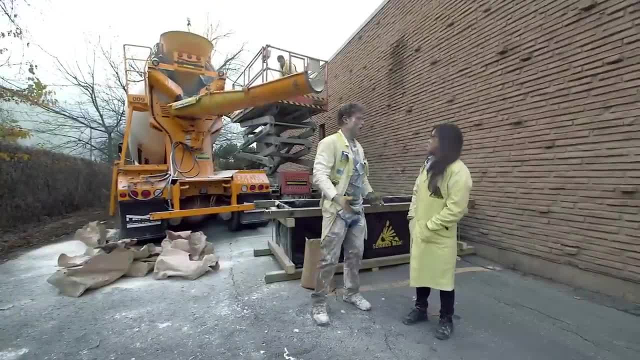 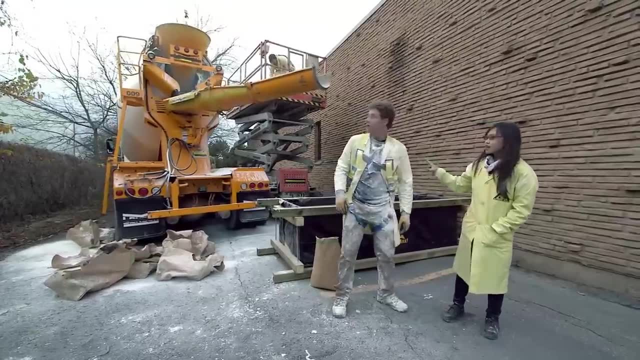 Let's start the mixing. So what do you think, Judy? Do you think it's gonna work? I think so, because you're mixing at a very large volume, but at a very low speed, And throughout the process it'll stay liquid until we're ready to run across it. 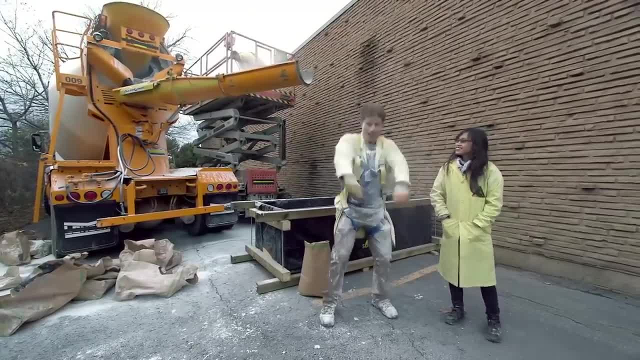 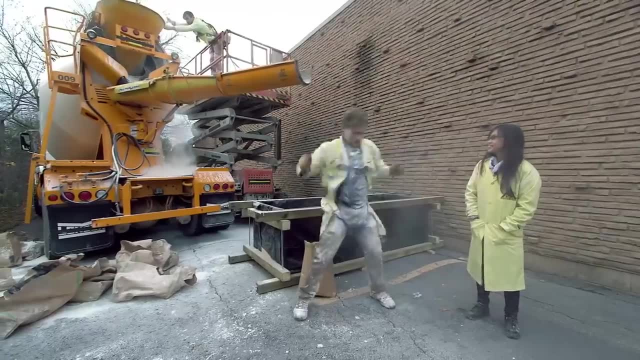 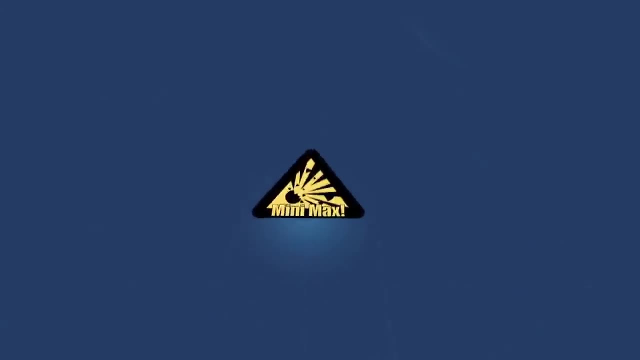 That sounds exactly like the kind of science I like to see. You know, what I really like is that every time I move, more cornstarch comes off. It's like. it's like I'm a human fog machine. Mini Max. This is liquid nitrogen. 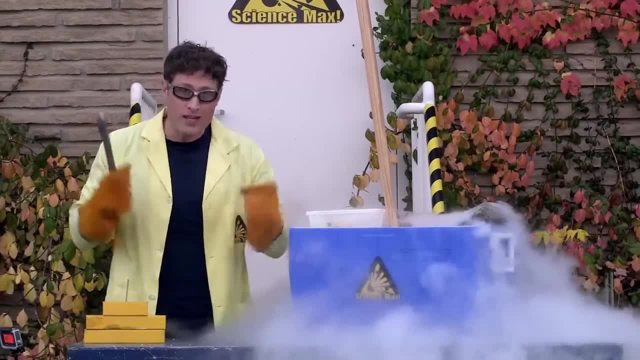 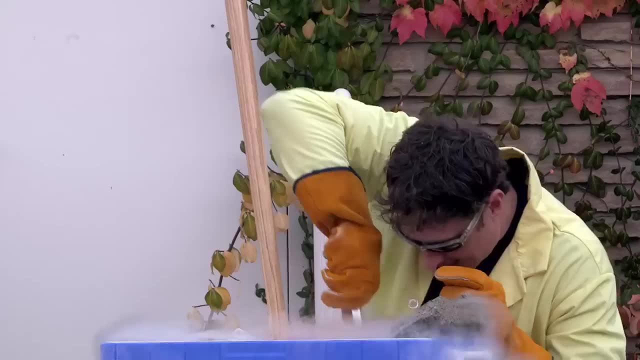 Nitrogen makes up most of the air we breathe, but if you get it really really cold it turns into a liquid. The fun thing is you can use it to make other things really really cold too, Like this banana. I have frozen this banana solid. 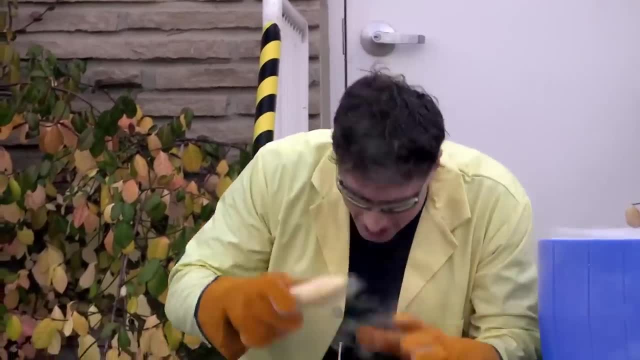 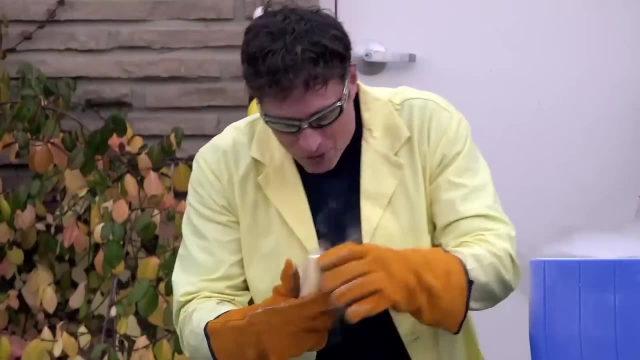 thanks to the liquid nitrogen, and normally a mushy banana would not be able to hammer in a nail. but whoa, because it's frozen, I can hammer this nail into this block of wood. So that got me wondering if I can turn a banana. 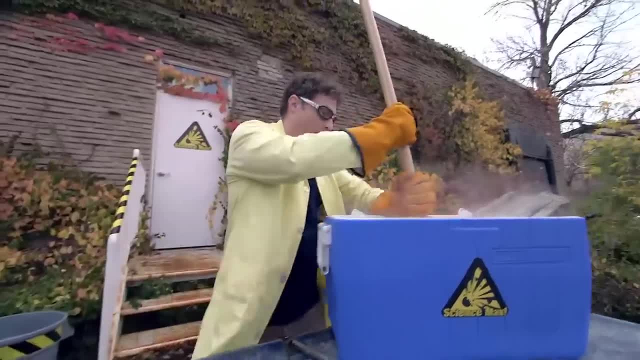 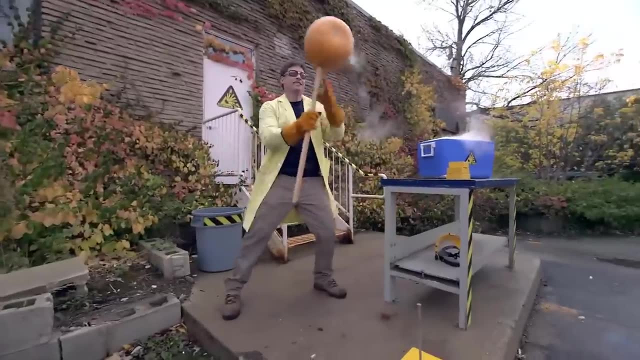 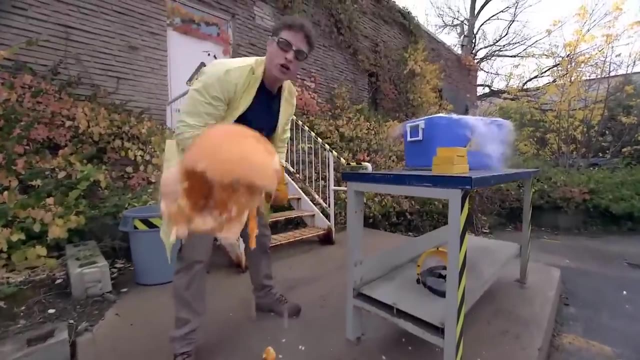 into a hammer using liquid nitrogen. could I turn a pumpkin into a sledgehammer? Let's find out. Pumpkin sledgehammer, take one. No, I think the answer is no. You cannot turn a pumpkin into a sledgehammer with liquid nitrogen. 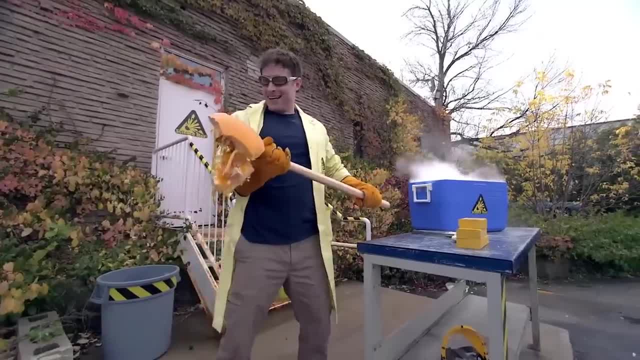 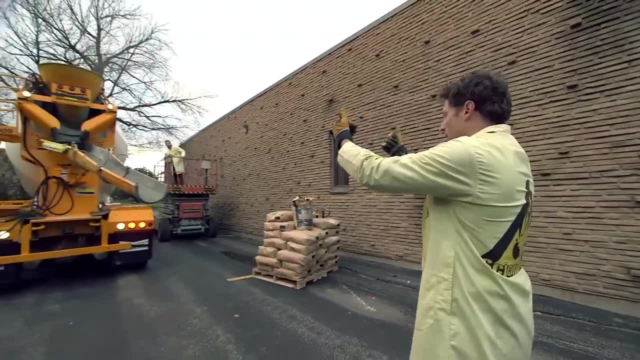 All you can do is make a really, really big mess. I'm going to have to clean this up, aren't I? Now we have a cement truck to help us do the mixing for our cornstarch mud After making a giant mess getting the cornstarch. 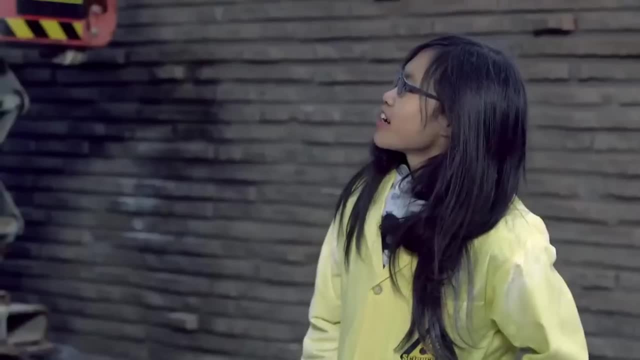 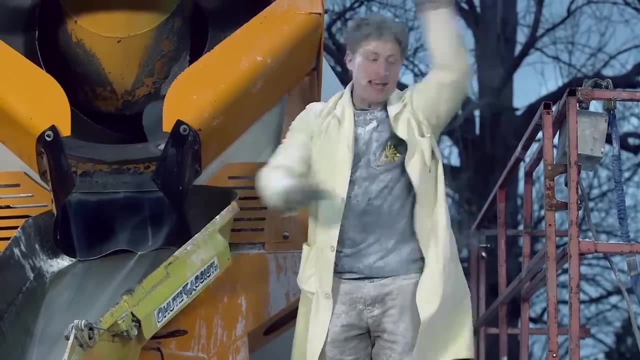 into the cement truck. it's time to see if it worked. Hey, Phil, how's it going? Yeah, it looks like it's mixing pretty well. I'm really glad we're not doing this by hand, Because it'd take a really 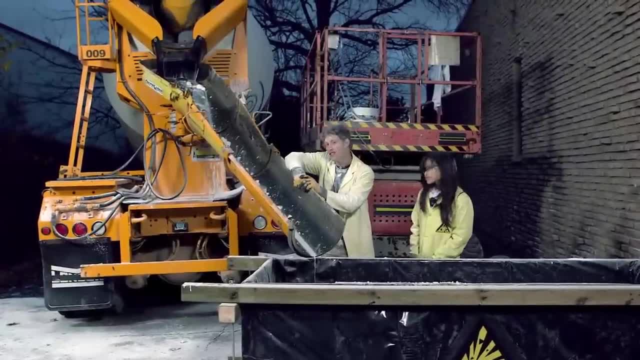 long time. We've almost got it at the right consistency, but it's taking some time. But it's getting a little dark out. Judy, I don't know, do you want to quit and go home? No, Of course not. That's not what. 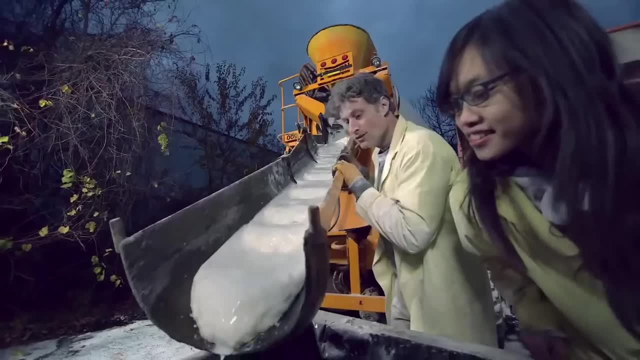 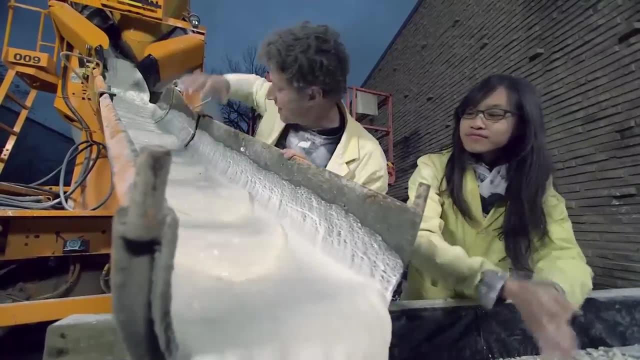 we do in science. Oh, here we go. Yeah, Awesome, Alright, let's see it. Let's see if it's. I like how it comes down in little steps And look it's still, it's working, just like it should. 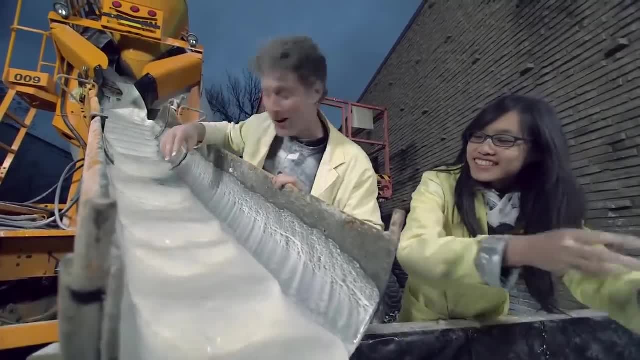 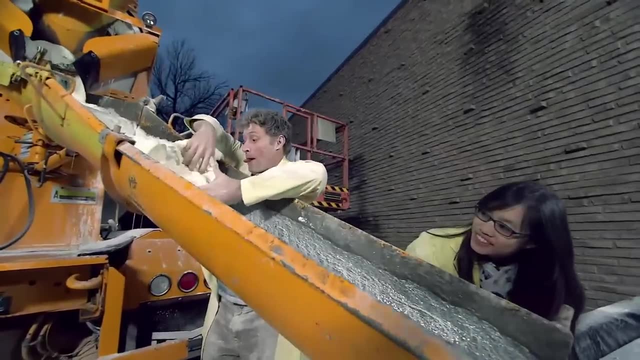 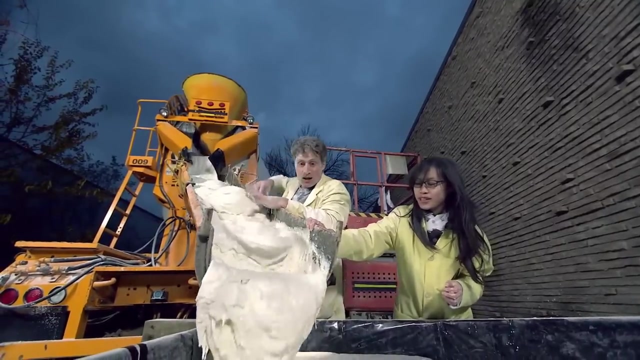 I hit it and it's solid, But you can see it's pouring like a liquid. Yeah, here comes a big wave, Here it comes, Wow, Wow, And it's totally filling up. Oh yeah, it's filling up really fast. 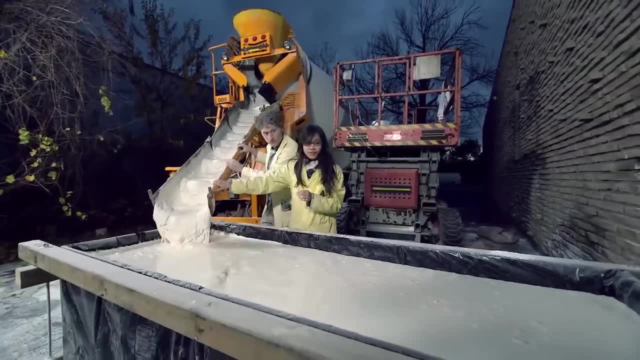 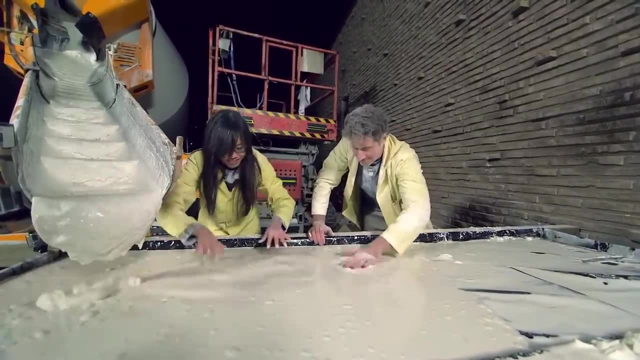 I think we should stop pouring very soon. Yep, we may not have a big enough bath. Yep, I'm liking it Good. Yep, I think it's time. It's not even done pouring, but I'm gonna try it. 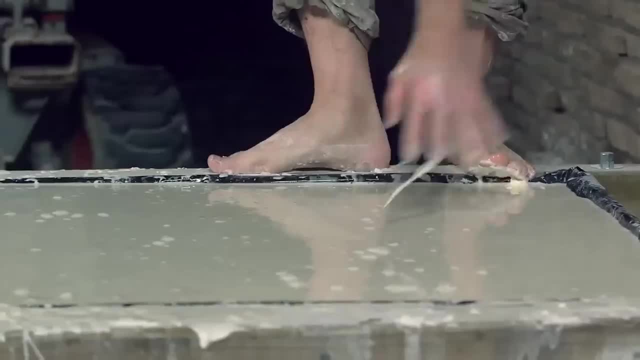 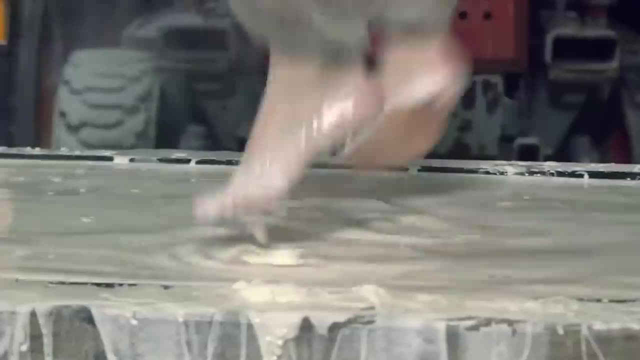 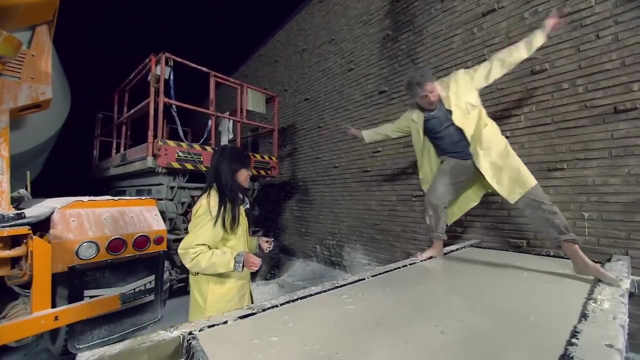 Okay, you ready? Whoa, Yeah, Oh, you did it. Whoa, You can't. You have to get back onto the sides before you stop moving, Or else it becomes a liquid. Alright, it's your turn. Okay, Here. 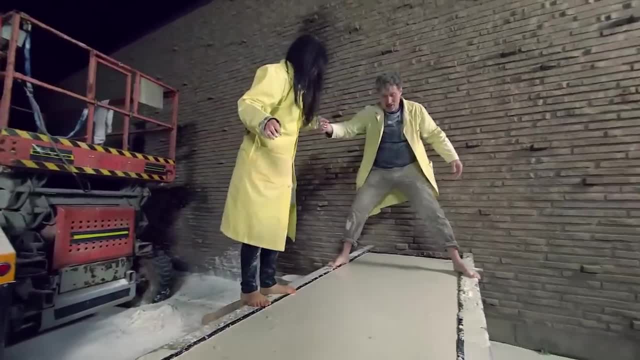 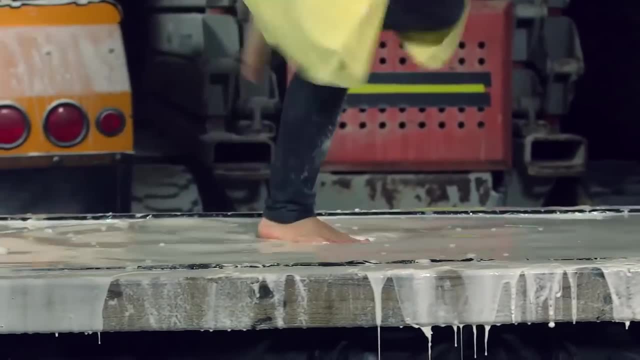 Go: Okay, ready. Okay, You gotta hit your feet really fast. Alright, Here go. Yeah, That actually works, Because cornstarch mud is a sheer thickening fluid. it means it stays a liquid until you hit it suddenly. 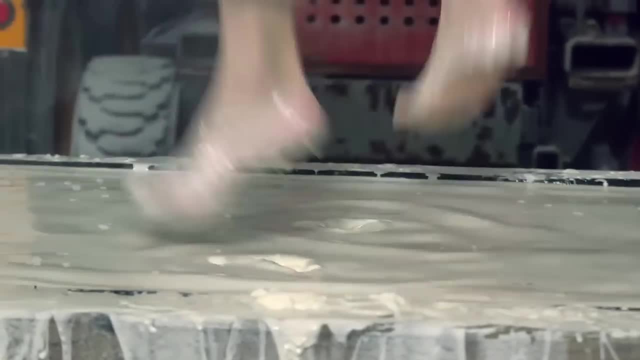 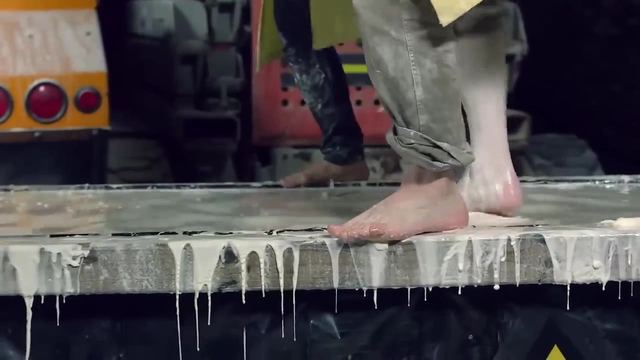 Like with your hands or, in this case, our feet, And then it turns to a solid. So as long as Judy and I keep slapping our feet down with enough force, we can walk on top of it. One more dance. Alright, let's do it. 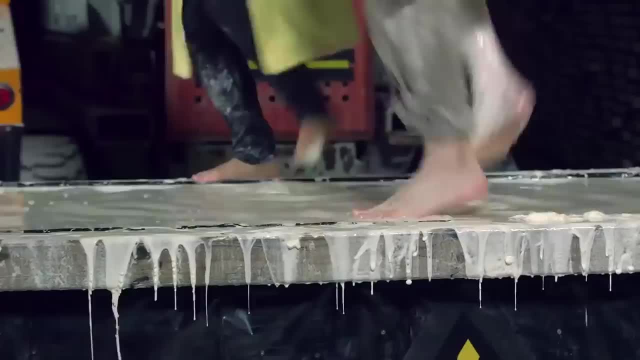 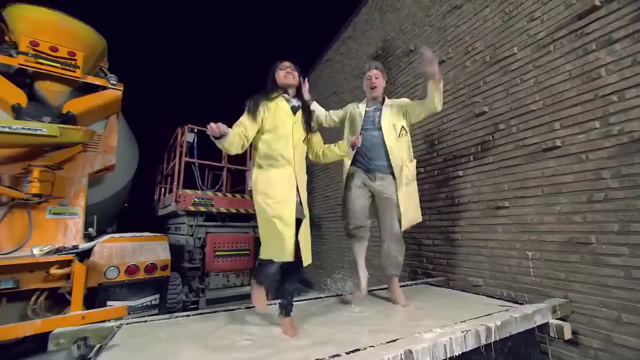 And tell you what we'll do. one more dance, Alright, let's do that. Okay, ready, Alright, Andgo, Alright, All right, There you go. Solid liquid gases. Thanks very much for joining us on Science, Max. 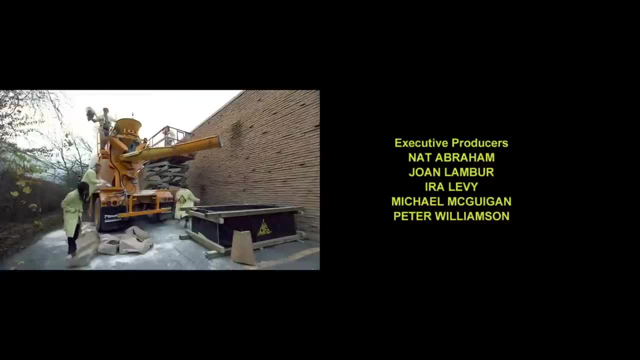 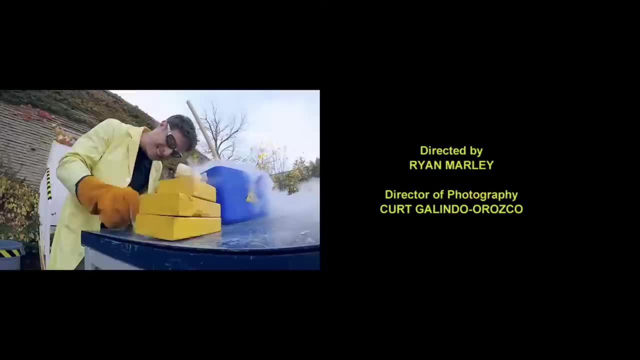 Experiments At Large. Whoo, Hey, Judy Catch. Ha, ha, ha ha. I have to be careful because the banana will shatter if I'm not careful. I think it's stuck on the bottom. I call this one the loud bubble. 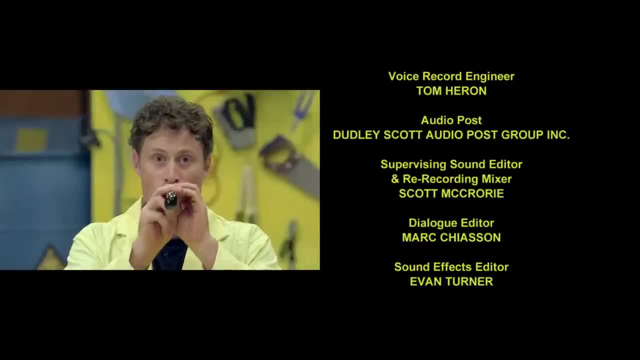 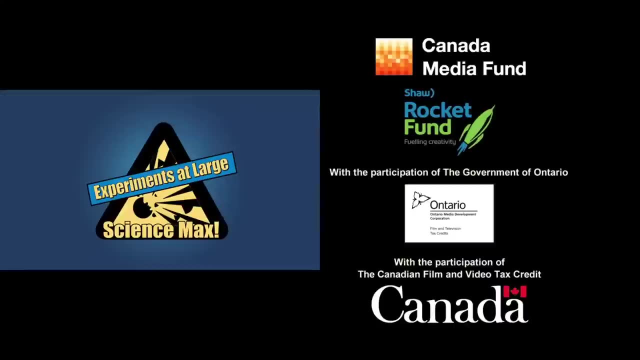 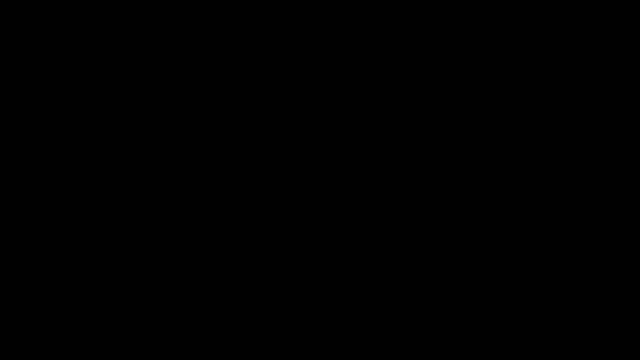 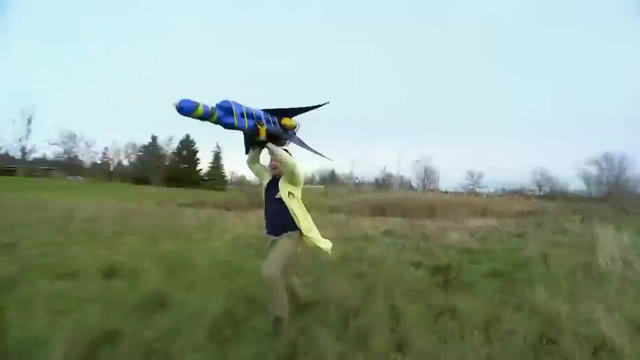 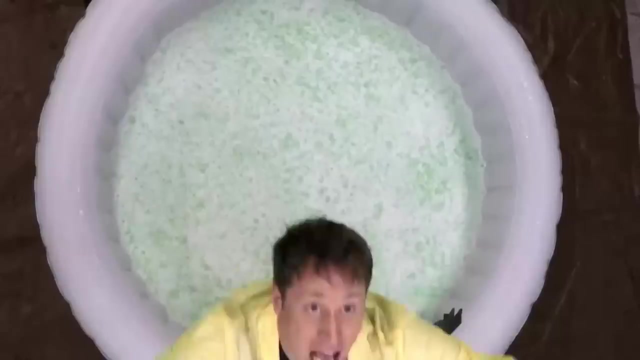 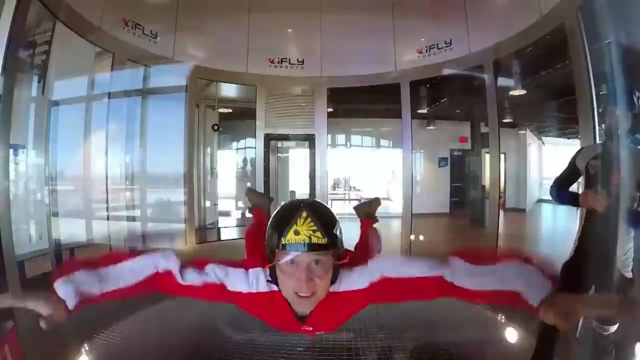 Oh well, Uh, I call this one the loud bubble. Ha C'mon. Judy Hane, Have you ever done a science experiment and wondered what it'd be like if you did it big? I have No. My name is Phil and I take your everyday science experiments and do them big. 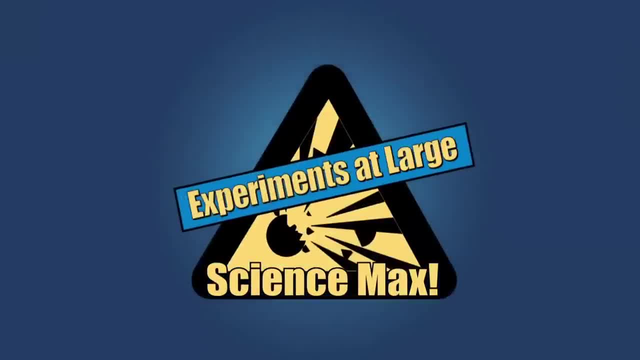 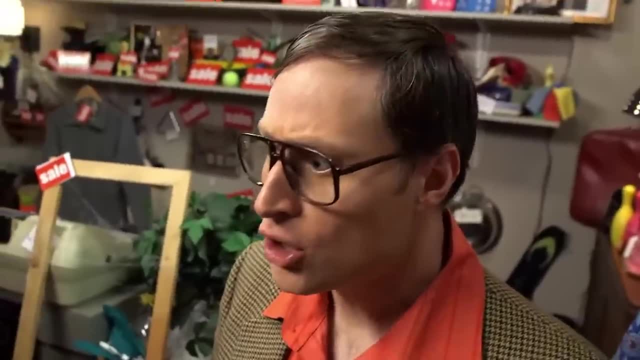 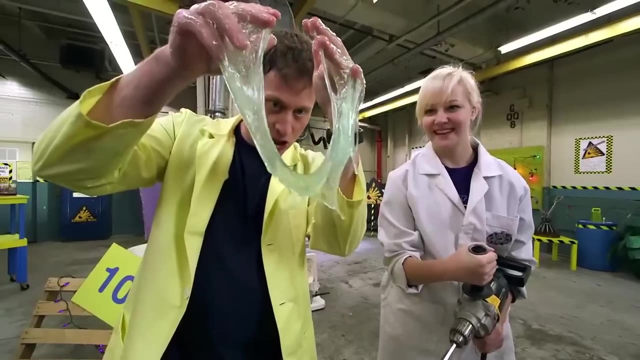 This is Science Facts, Experiments at large, Science Facts. Today we're looking at polymers, Polymers, polymers, polymers- Word has lost all meaning- Plastics, latex rubber and our favorite polymer slime. 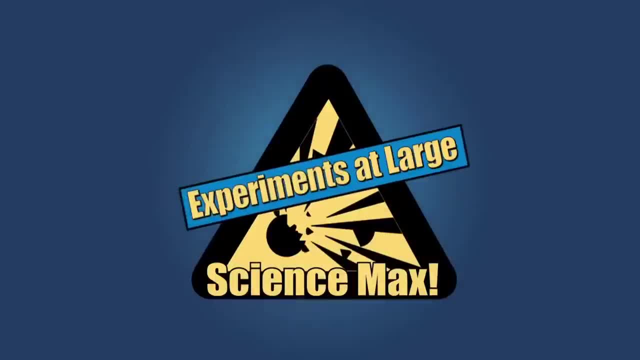 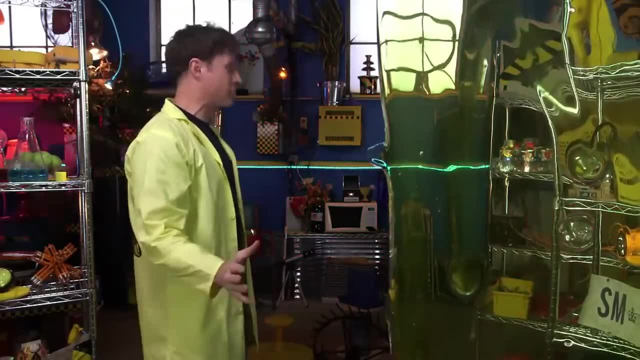 Oh yeah, All on this episode of Science. Max Experiments at Large. Greetings- Science Maximites. My name is Phil and I think I might have overdone it with the science. I mean, what's a better use of science than creating a whole bunch of slime? 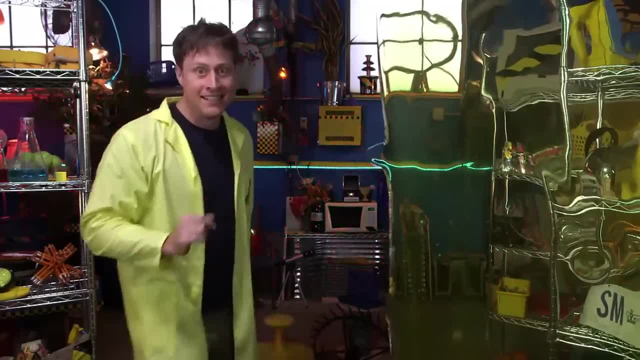 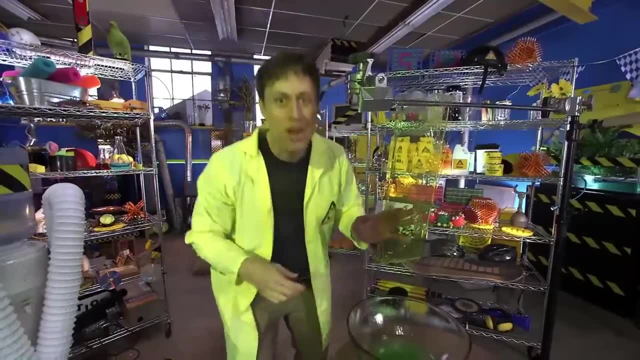 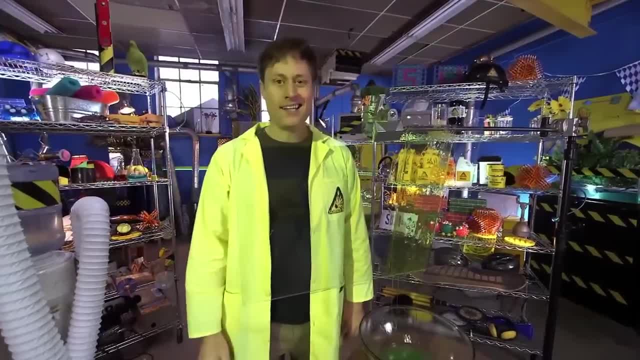 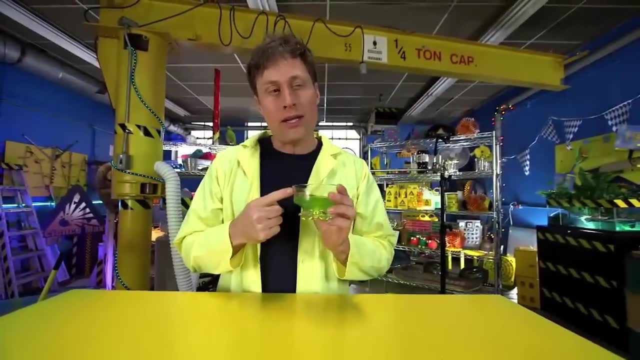 Ha, ha ha Ha. Yeah, it needs work. Anyway, today we're talking about polymers- Polymers like slime. But you see, polymers aren't really a substance, They're more how something is constructed, And there's all kinds of different polymers. 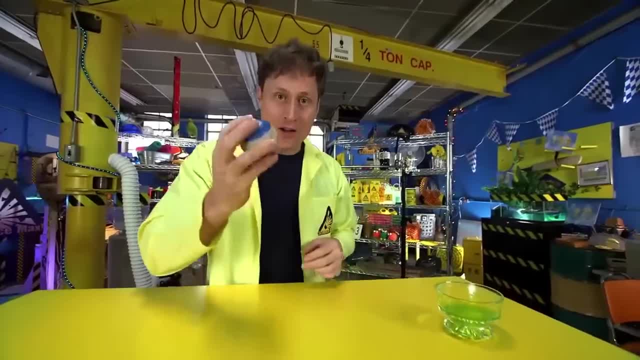 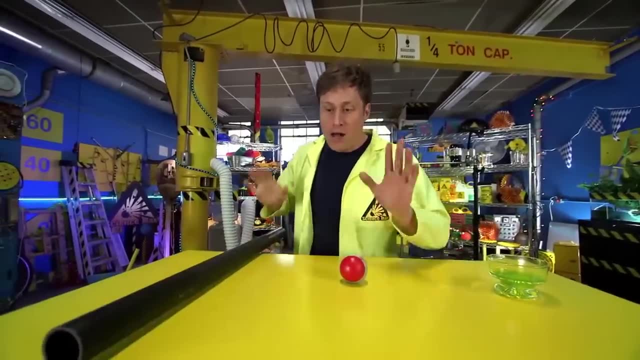 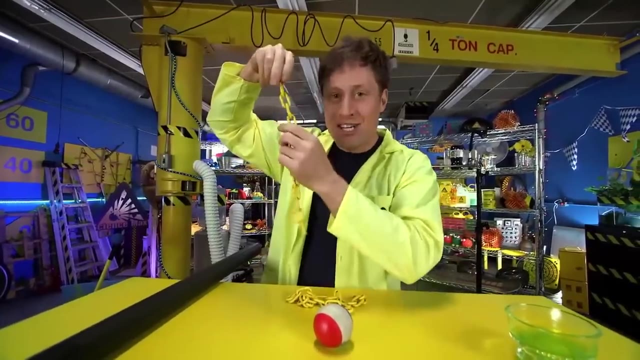 There's slime, obviously, and rubber polymers like well, like rubber, And there's also hard polymers like plastic. Now, polymers are all kind of constructed the same way, Like this: This is a chain. Yeah, So imagine this is a chain of molecules and all the molecules are the same. 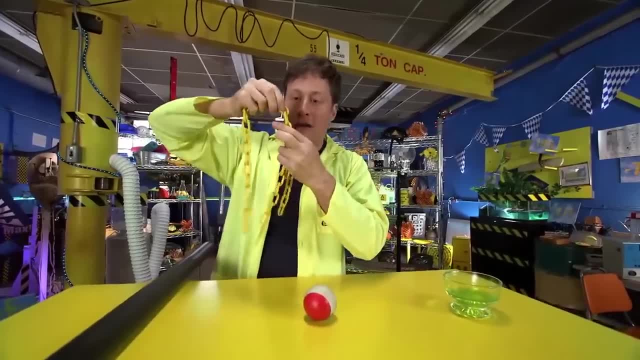 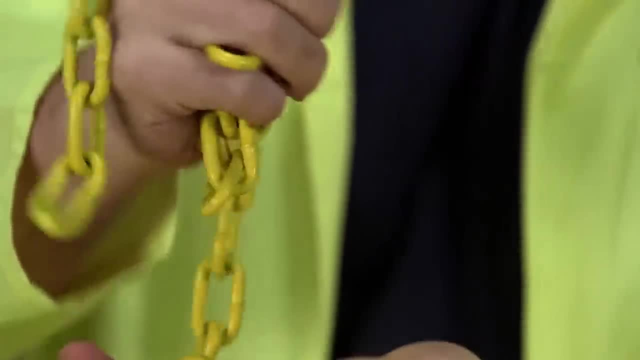 and they just repeat in a long line. Now, when you get a polymer like slime, all the chains are not connected, or very loosely connected, which means that they can flow over each other like a slime or sort of like a liquid and they behave like that. 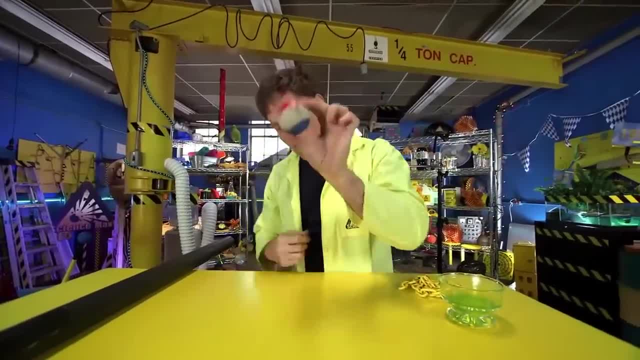 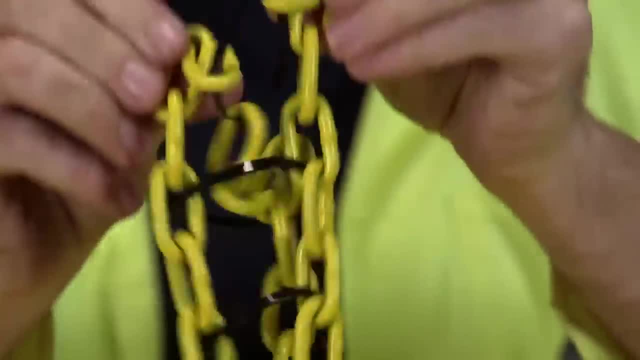 So that is slime, Right. But when you get to a rubber polymer you start to get little bonds in between the chains of polymers that work like this. You see, they still move around a little bit, but they can spread apart and they become flexible and bouncy. 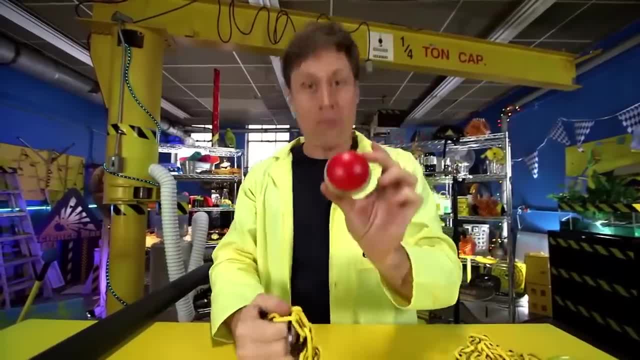 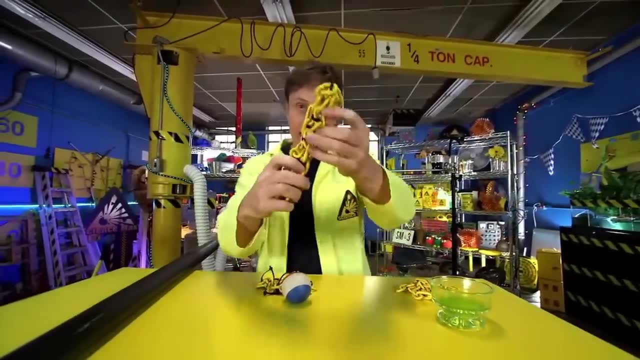 Yeah, I know, a chain doesn't really bounce, but rubber polymers do. Huh, Now, when it gets to a solid polymer like plastic, there's a lot more links and it's all kind of interconnected and it doesn't move at all. 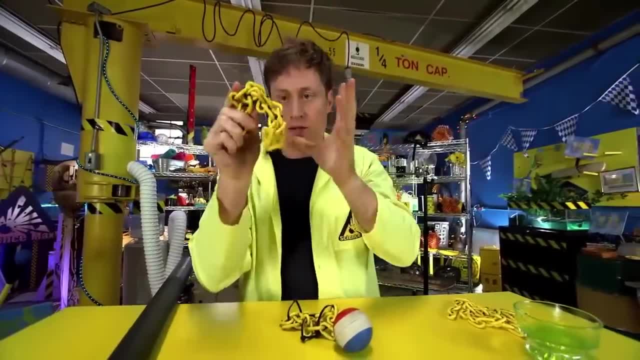 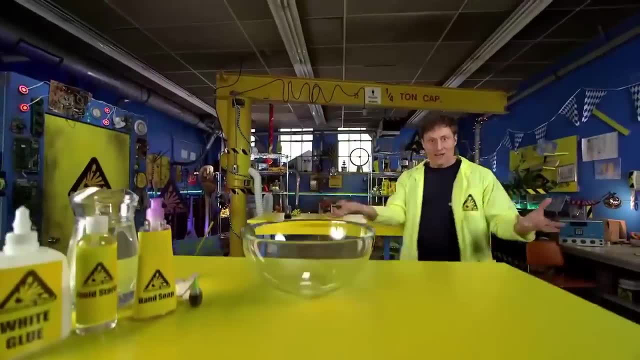 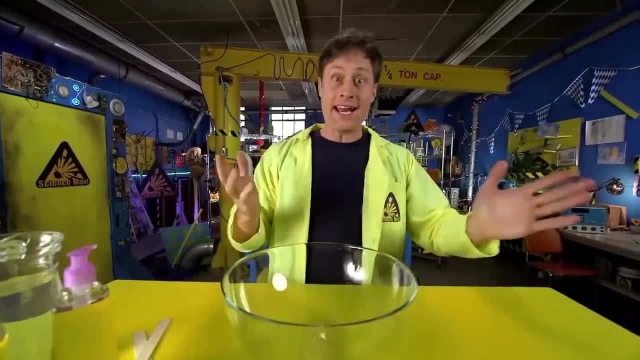 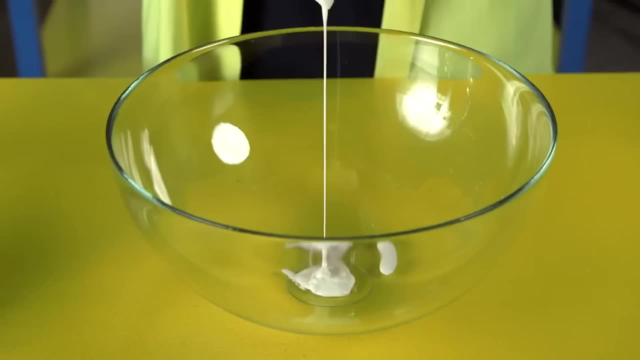 Yeah, too mad, not enough scientist. I'll keep working on it. Anyway, to make slime, take your white glue and pour in an amount. It really kind of depends on how much slime you want to make. Now you want to add about twice as much water as that. 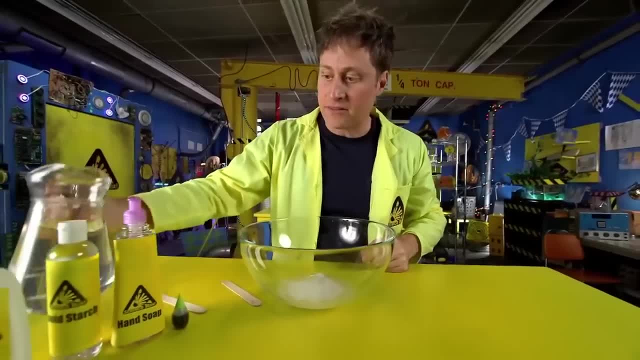 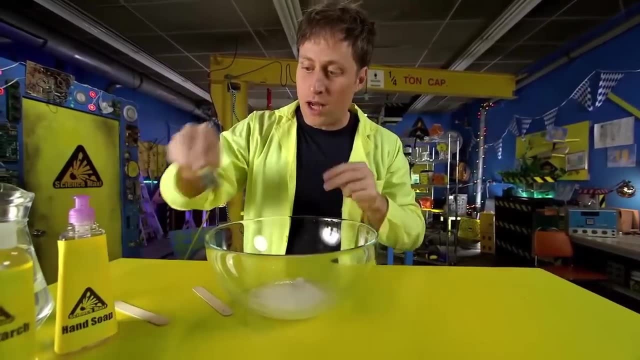 Uh Yeah, somewhere around there. Great, Now we want to put in just a little bit of soap, Mm-hmm, maybe there. That's good. And you want to put in your food coloring? I like green. Green seems like the right slime color to me. 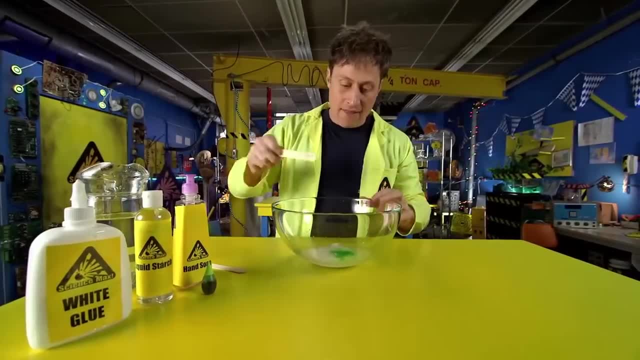 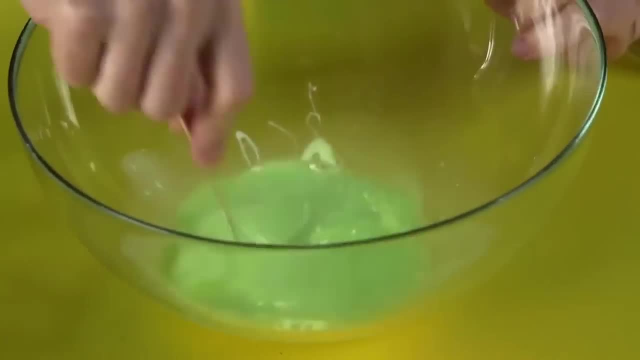 It's the right, appropriate mad scientist kind of slime. And then you want to start mixing that up until you get the right kind of consistency. That means make sure the glue and the water are equally mixed up. Good, And now we're ready to make it an actual slime. 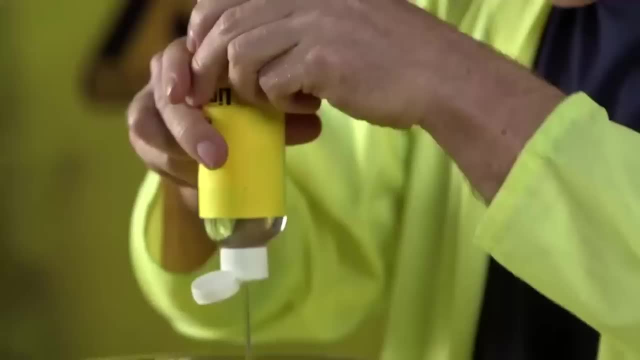 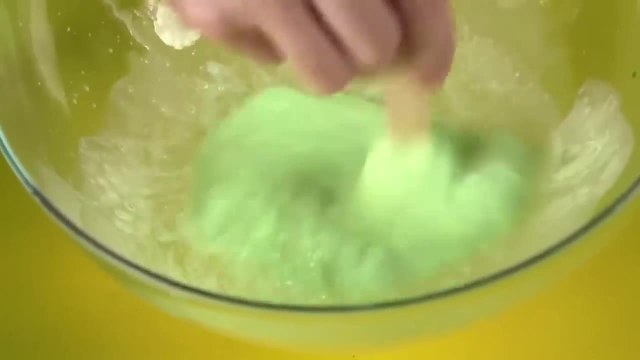 By bonding the polymers together, by adding liquid starch, Mm-hmm. very good, And you want to mix it up. When you add the liquid starch, it starts to bond the chains of molecules together, changing it from a liquid to a slime. 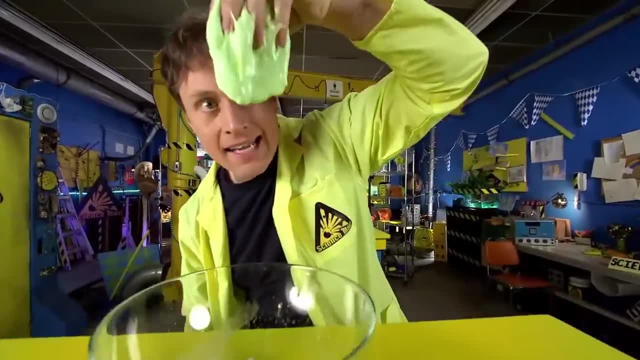 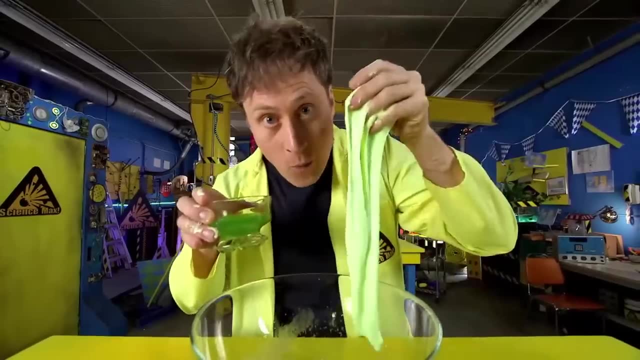 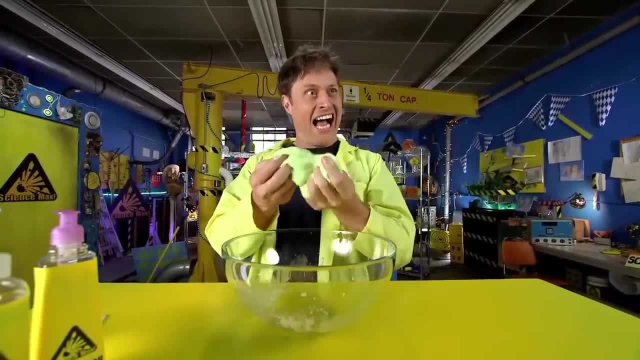 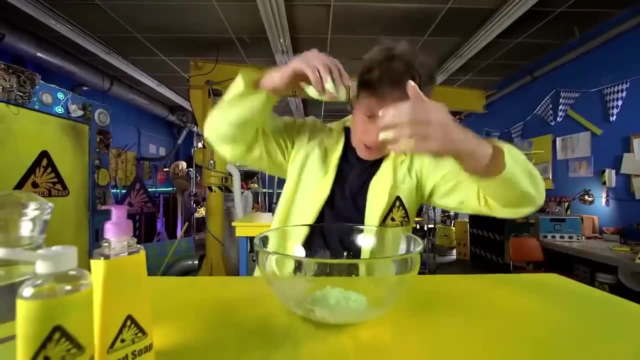 Mm-hmm, Mm-hmm, Mm-hmm. There you go, Slime To supervillain. Yeah, okay, Well, anyway, we All right. Now all you need is an expert to help me max it out. 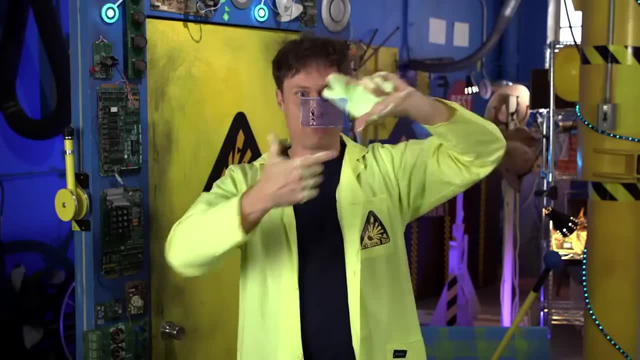 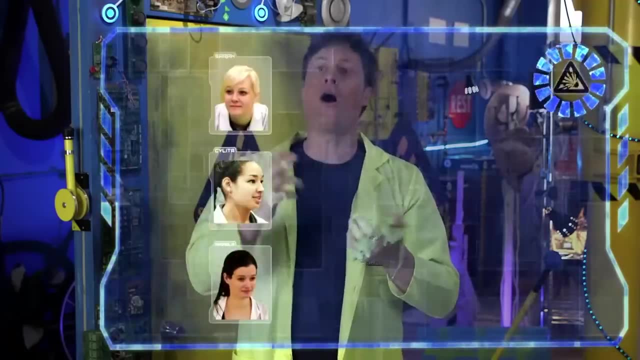 Of course, my interface is hand gesture based, so I don't know if the slime. Oh hey, there we go, Great, So you gotta Uh-huh. Oh, of course, Sarah from Mad Science, Mad Science, They are really nice. 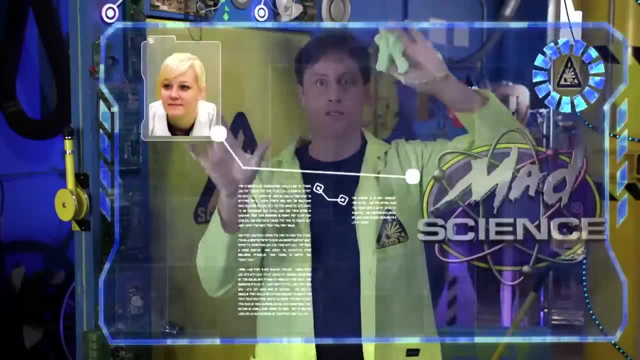 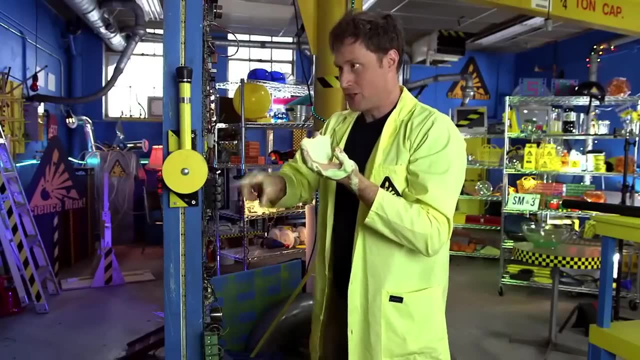 Mad Science know they're slime. This is great. Yeah, I got it Close, close, close. There we go. All right, I'm not sure if bringing it through the portal is such a good idea, but at least I'll have it on the other side. 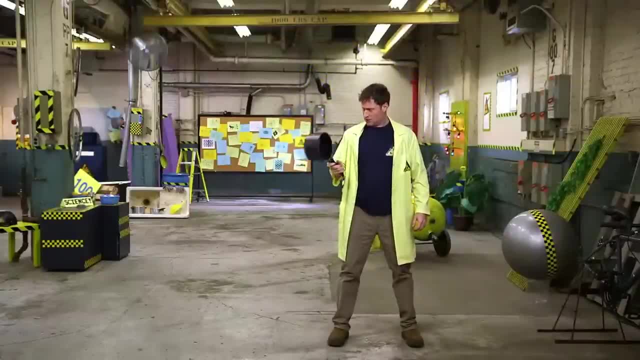 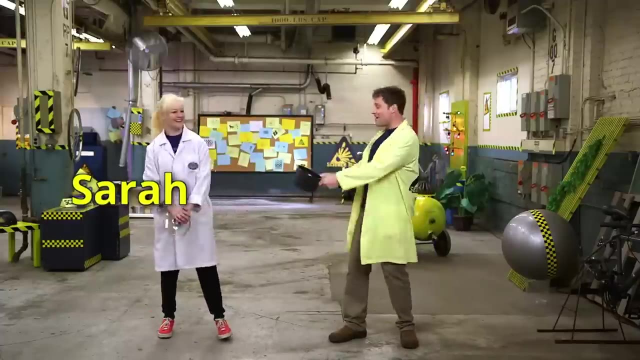 I have a pot. Why do I have a pot? I didn't have a pot when I went through the portal. Is someone somewhere missing a pot? or did it just create this pot out of nothing? Huh, Hey, Sarah, Hey hi. How are you doing? Good Sarah from Mad Science, you're gonna help me make some slime. 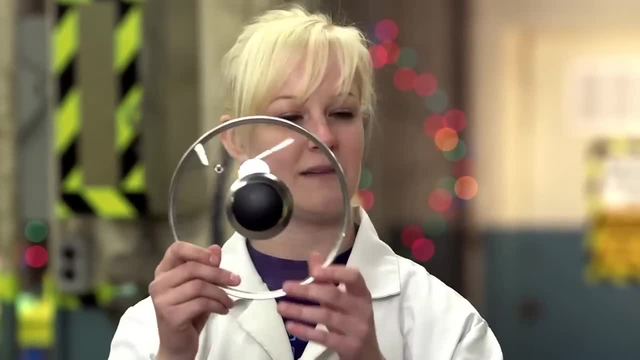 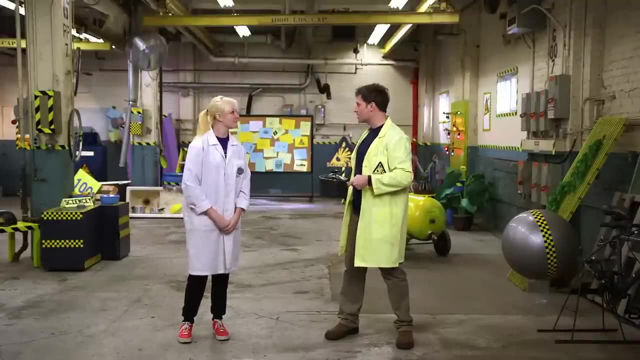 Yes, I actually brought some. Oh, this isn't slime, This is a pot lid. Hey, Oh Well, at least we have a set. Doesn't answer any questions, though, and I guess we're gonna have to make some more slime. Definitely, What kind of slime do you? 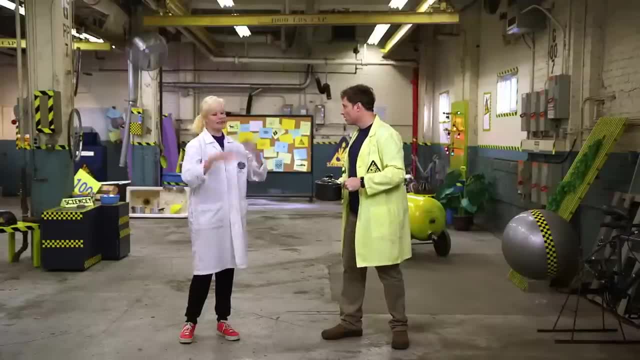 want to make. What do you mean? what kind? Is there more than one kind? Oh yeah, There are tons of different kinds of slime with lots of different ingredients and recipes. Oh, I only know the one. Can you show me all the others, Of course? 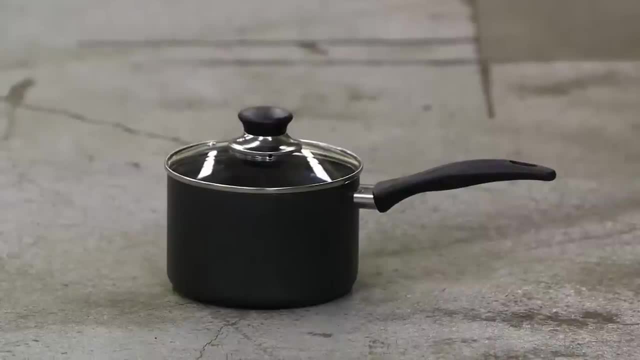 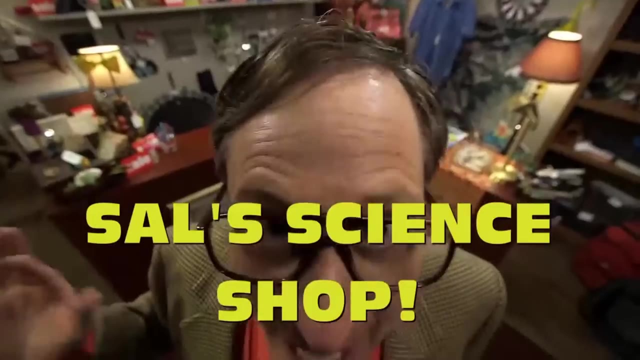 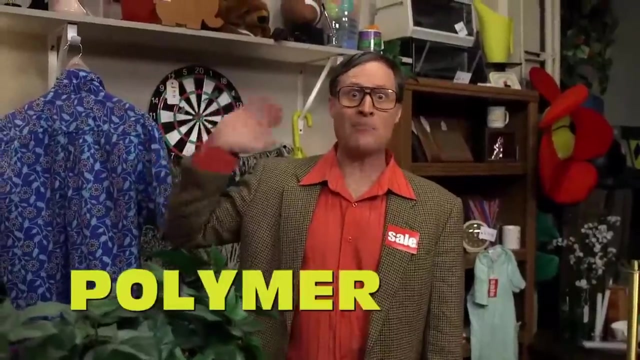 Let's go make some right now. Okay, great, Awesome. Come on down to Sal's Science Shop and see me sell while you shop for science. This week, only Sal's one-of-a-kind- once a year- polymer sales- Fifty to seventy-five percent off anything made of polymers- Rubber, That's a polymer. 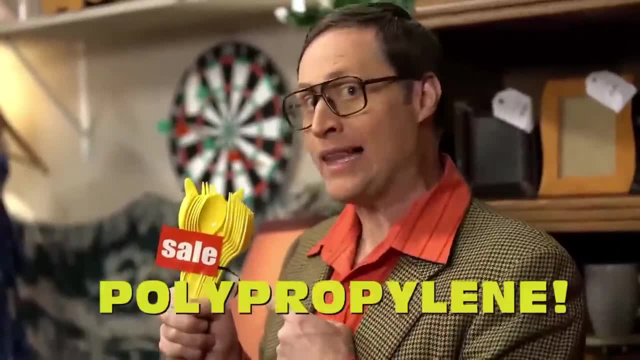 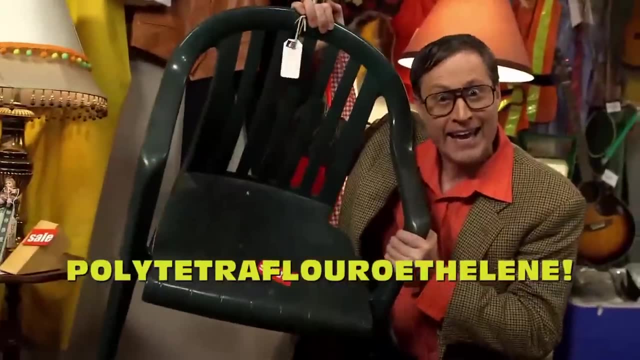 Polystyrene. When you're eating your next meal, I recommend some polypropylene. Low-density polyethylene. High-density polyethylene. You want some poly fingers? Polytetrafluoroethylene. We got it. We've even got polychlorotrifluoroethylene. 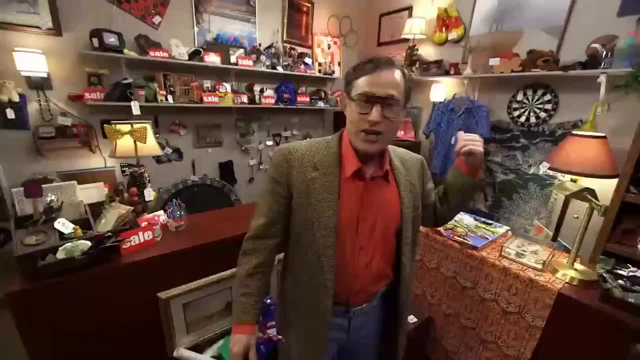 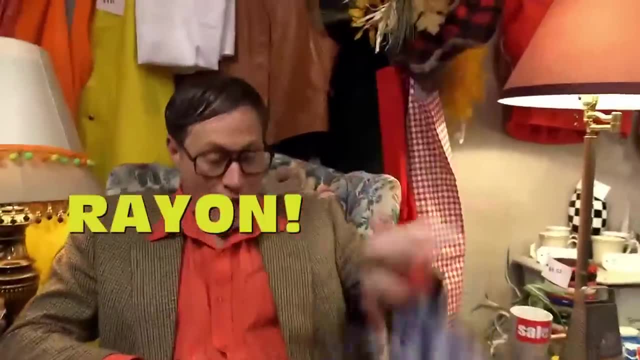 Do they even know how good a deal this is? Cause you're not gonna find. you're not gonna find that kind of deal just like every day. But hold the phone. polymers aren't just plastics: Rayon, nylon, teflon, you name the lawn. 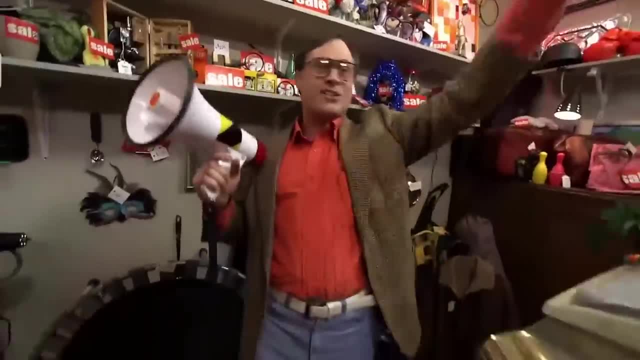 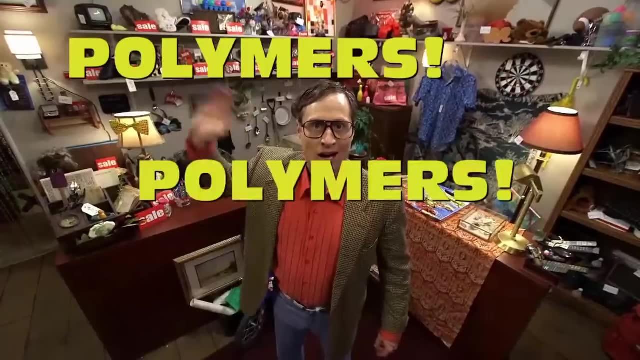 we got it on sale. What do we want? Polymers? When do we want them? Anytime, during normal business hours: Wool, Silk, Cotton, Polymers, polymers, polymers, Polymers, polymers, polymers. 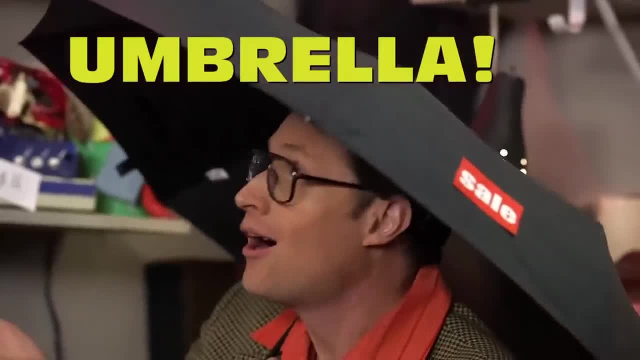 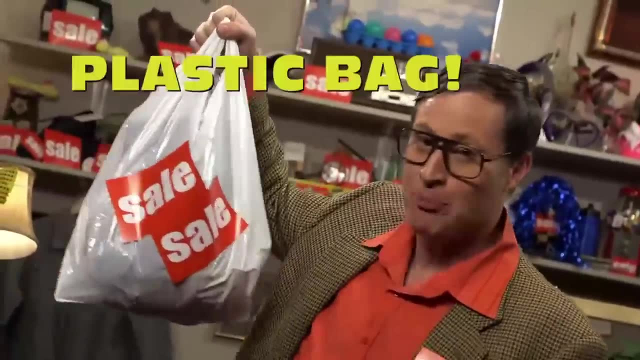 Word has lost all meaning. Glue, Paint, Umbrella fabric, Oh yeah, Carpet. You bet that's on sale, Roberta, I'm running out of sale signs. Buy it and I'll put it in a plastic bag also made of polymers. 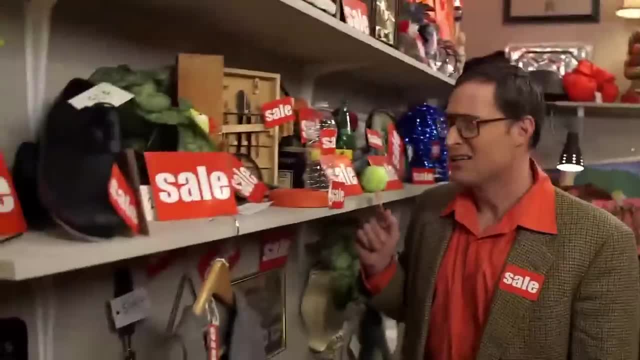 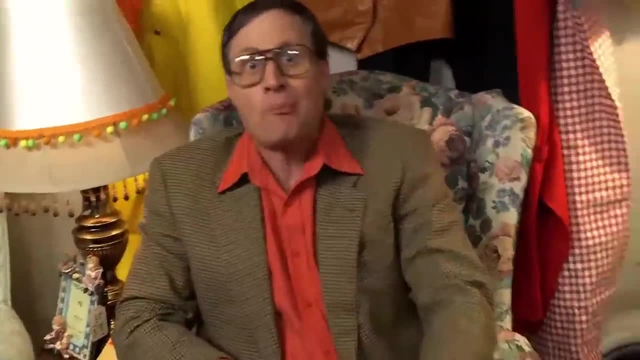 Seriously, Roberta, we can't have a sale on everything. No, hey, hey, even you, even me. the proteins in our bodies, even our DNA, all polymers, Haha. so come on down to Sal's Science Shop. 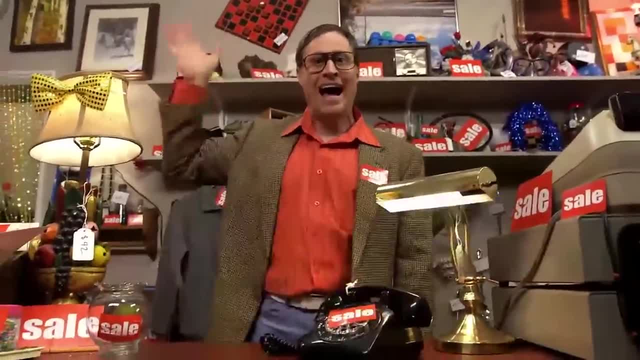 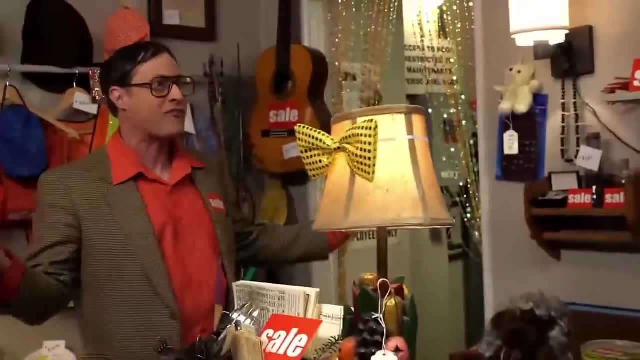 and get a great deal on your polymers for a limited time. I mean, it'd have to be a limited time, right, Roberta Cause? I mean I can't discount everything in the store to 75% off. how am I gonna make any money? 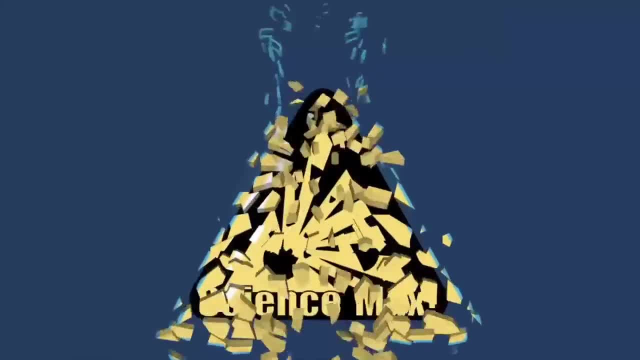 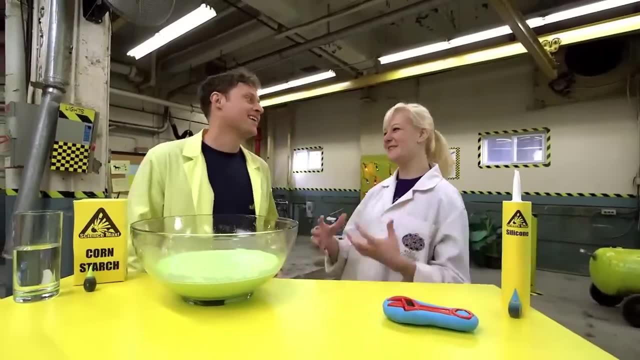 I mean, are we still rolling 100 different kinds of slime? Yes, it's gonna be so much fun, but we're not gonna make 100 today. Yeah, I know, we're just gonna do our top favorites. Yeah, it's gonna be super great. 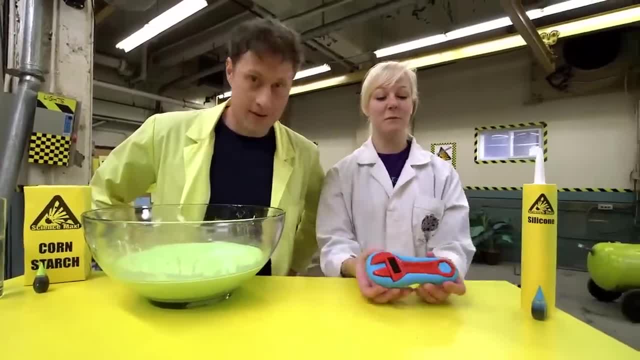 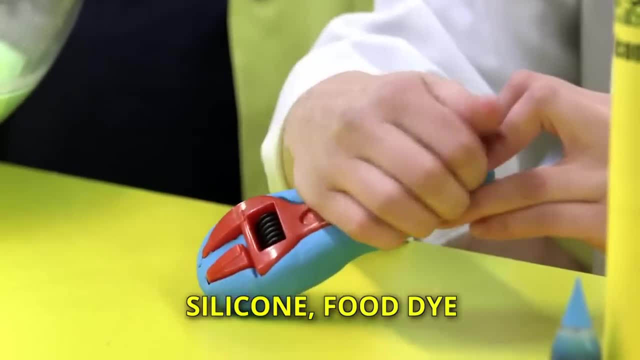 Alright, what are we starting with? So our first slime we're starting with today is some really cool molding slime. Now, this slime, actually, if you leave it out overnight it'll harden and you can make an imprint of whatever you like. 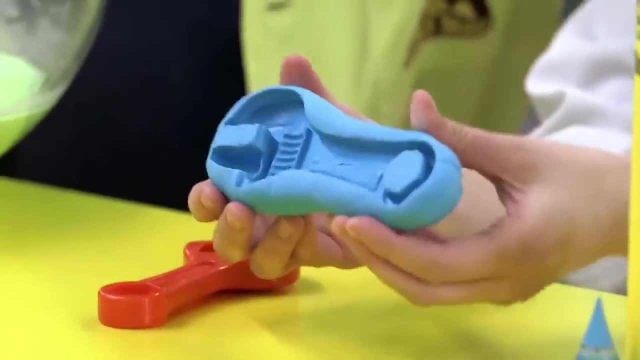 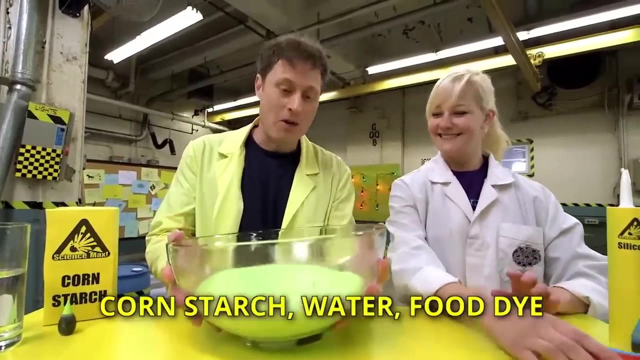 So here we made an imprint of our little tool there, So we're gonna look at a little bit more liquidy slime, starting with this one over here which I believe you already know about. This is cornstarch mud, Exactly. 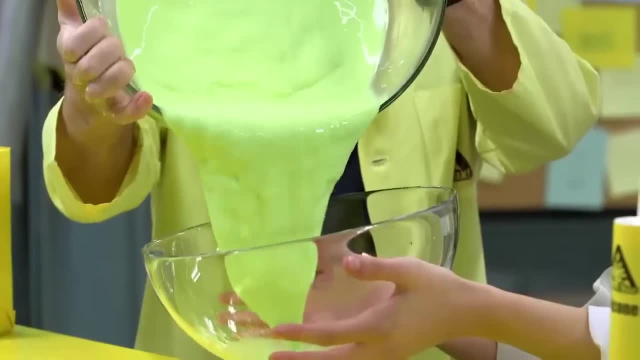 Can you hold? this Sounds good. I'm gonna hold this and we're gonna try pouring it. Whoa, Whoa, It's like it's like a liquid, but then if you do it fast, it's like a solid. 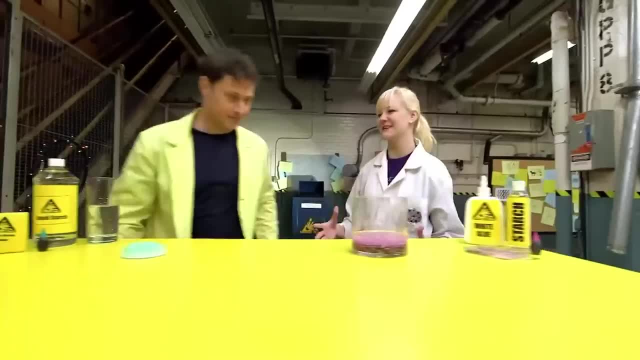 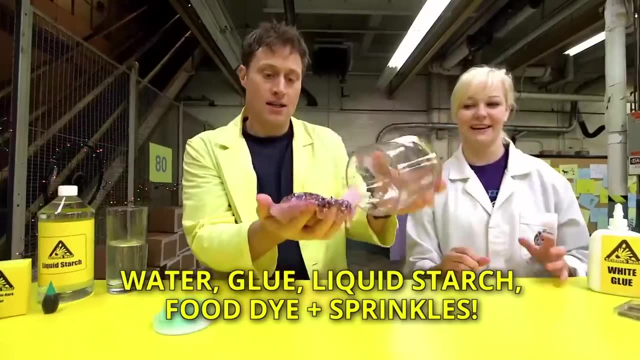 Alright, what's next? Over here we have some other really awesome types of slime. So right over here we have some crunchy slime- Crunchy slime- Exactly. Why is it crunchy? Now, it's crunchy because we've actually added. 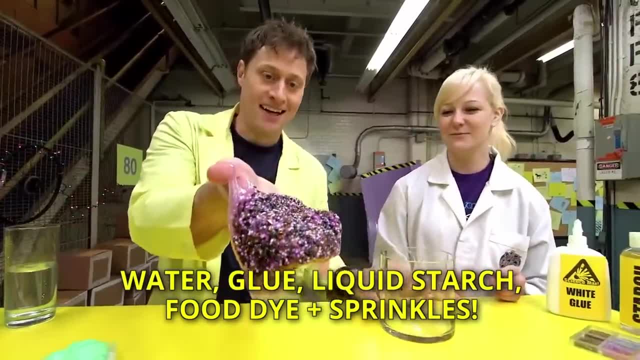 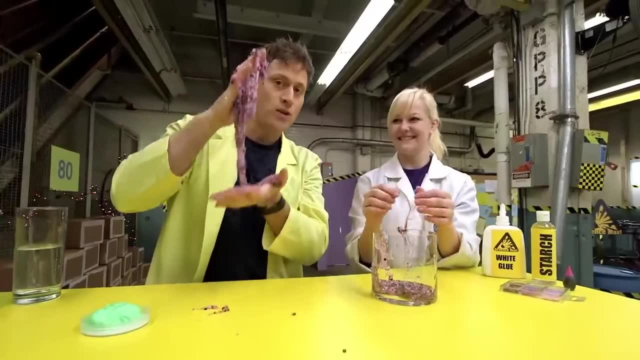 a few beads inside of it to make it crunchy. This is some really cool, awesome slime Here. you take half And you can feel the beads as you get to stretch it out. It's so cool. This is why this one is a little harder to clean. 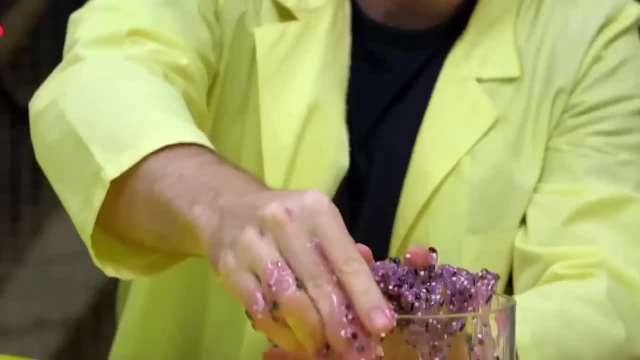 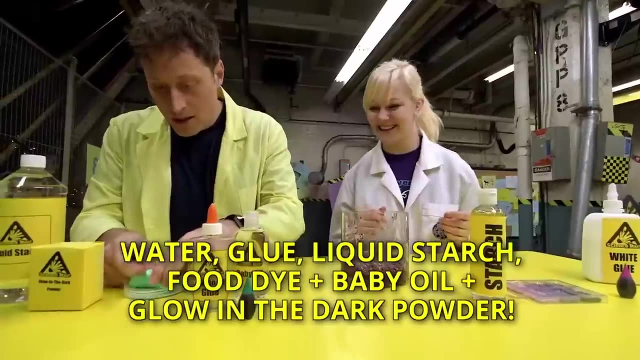 Exactly. Oh, I'll just do that, Alright. so what's next? So next we have some really cool glow-in-the-dark slime. Glow-in-the-dark slime- Yeah, It's so awesome. Ooh, Look at how much it glows. 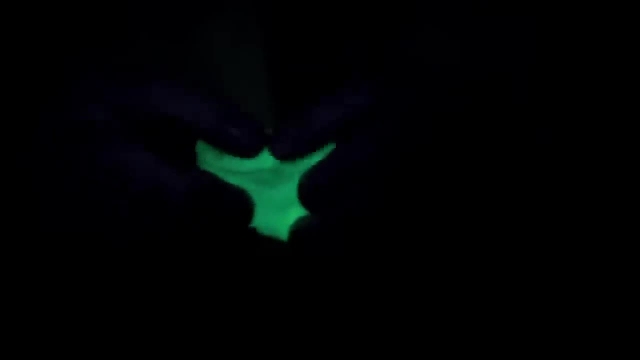 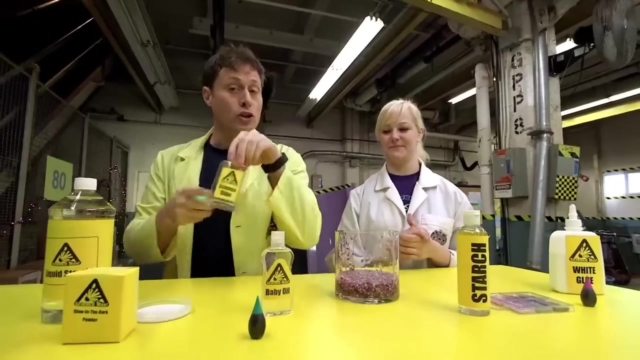 That glows a lot, That's super glowy slime. So to do the different kinds of slime, we need the polymer, Yes, And then the thing that sticks the polymers together, Exactly So: the glue is the polymer, Glue is the polymer. 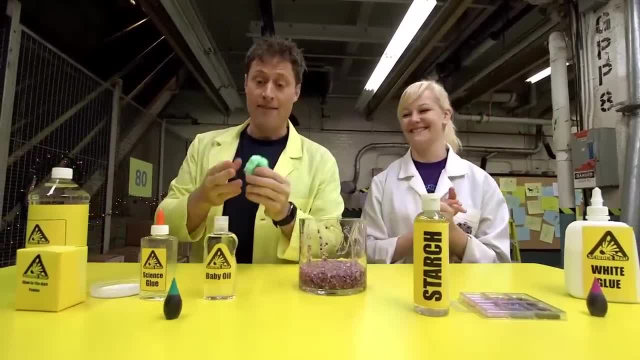 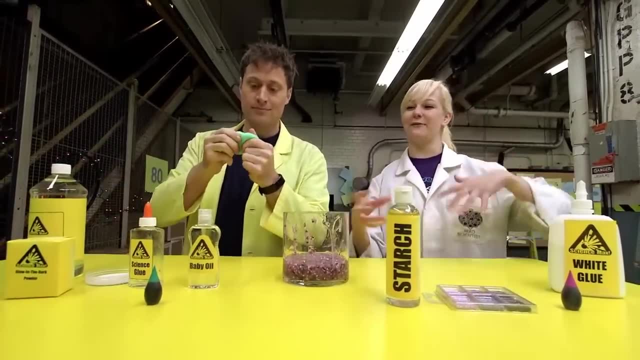 And the starch is the thing that bonds it. Yes, Uh-huh, Very cool. And then you put the thing in that makes it the kind of slime. Yes, Right before you add the bonding component, because if we keep adding stuff after it's. 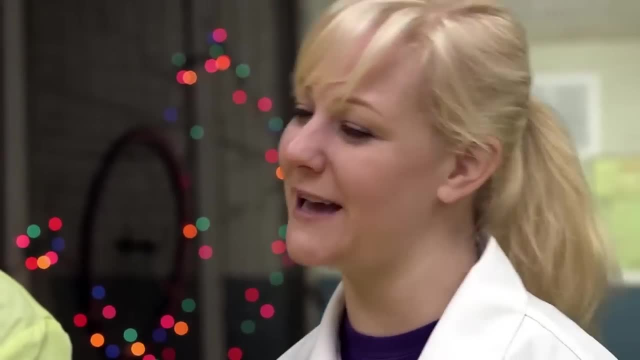 already made it unfortunately won't be able to take it, So we add our powder before we add our starch. in this situation, Should we go on to the next thing? Yeah, Let's move on to the next. slime, More slime, Little Max. 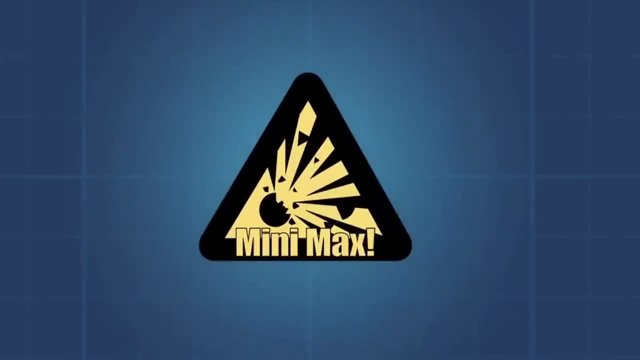 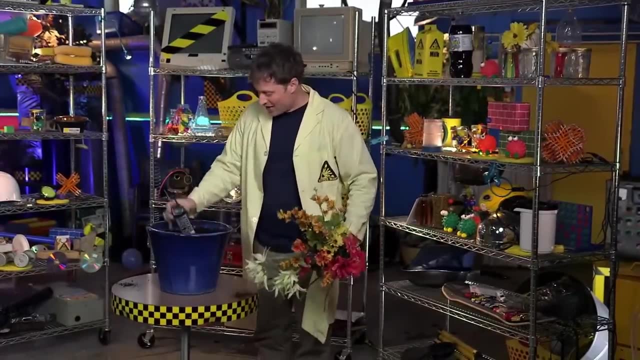 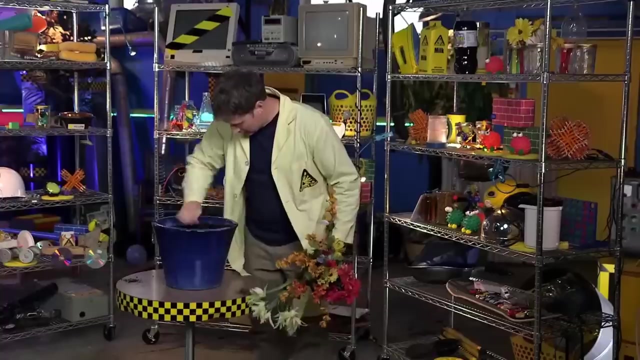 Plastic is great and plastic is everywhere. But the problem with plastic is it isn't very biodegradable. It doesn't break down in the environment. Huh, I'm still on hold. Oh well, There you go Back for another couple years, I guess. 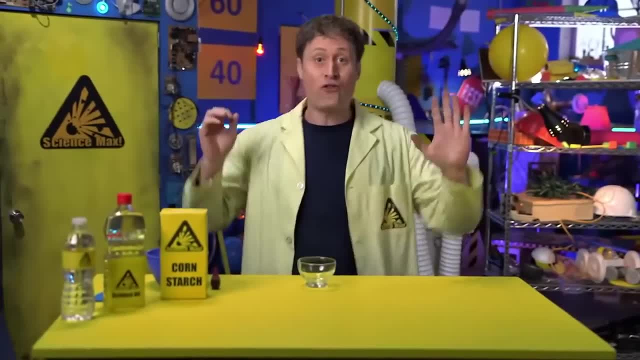 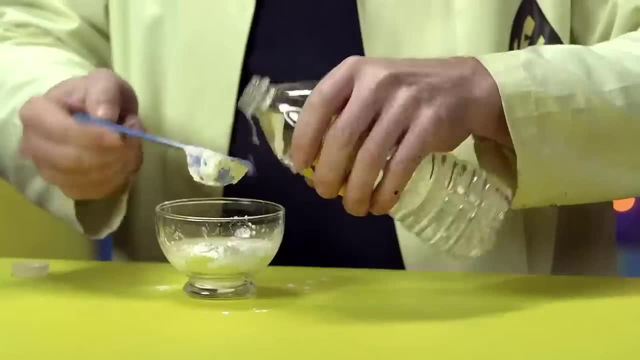 But here's a way that you can make bioplastic. It's fully biodegradable because it's made of natural materials. The recipe is easy: Two parts cornstarch, three parts water, A few drops of cooking oil and some food coloring to make it whatever color you want. 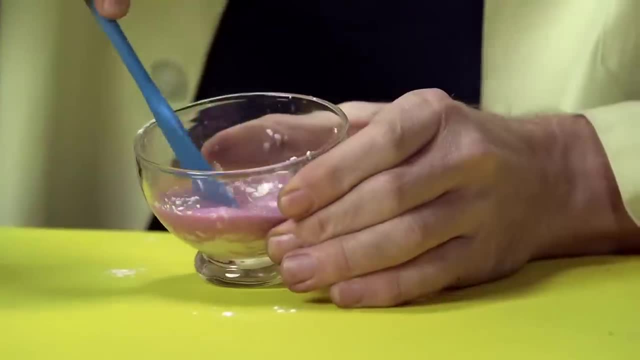 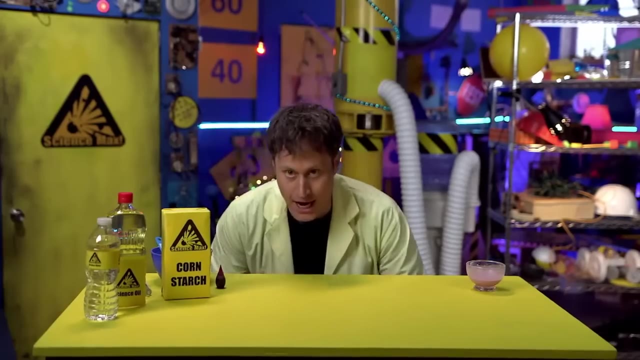 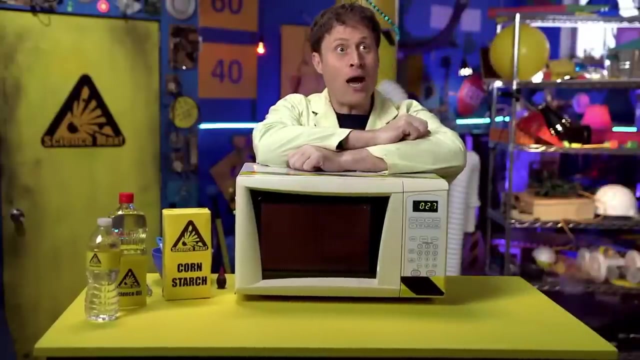 Purple Science, purple. Mix it up and it turns into a paste. Now what you'll need are two things: One an adult and two a microwave. Put it in for 30 seconds. Clock wipe. There we go. 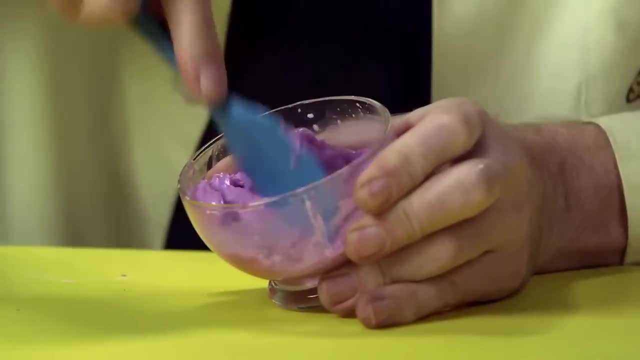 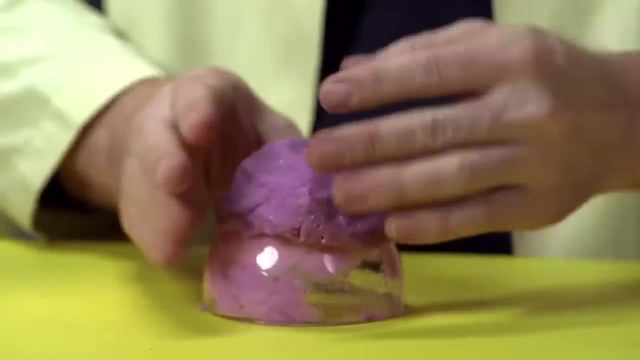 Then take it out and mix it some more until it cools down. Then you can pull it out and use your hands to sculpt it into a shape or take the shape of something else. Once you put it all the way around, you can turn it into a little flower pot. 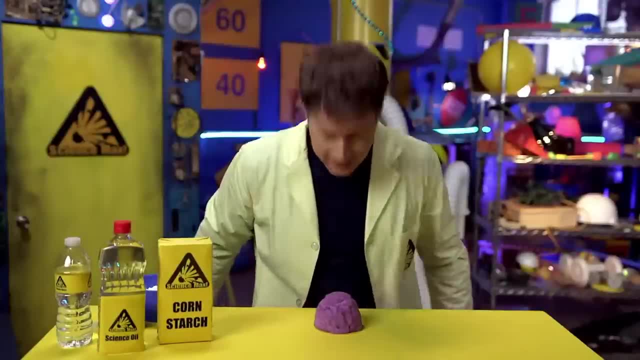 Once you've sculpted it, you need to wait for it to dry, which will take about a day. Clock wipe After waiting a day. What It's been a day? Oh, You have something made out of bioplastic. Like this little flower pot you can use to grow a small plant And then, when it grows big enough, you can take this biodegradable flower pot and plant it right outside in the dirt, and this pot will biodegrade and turn back into dirt. 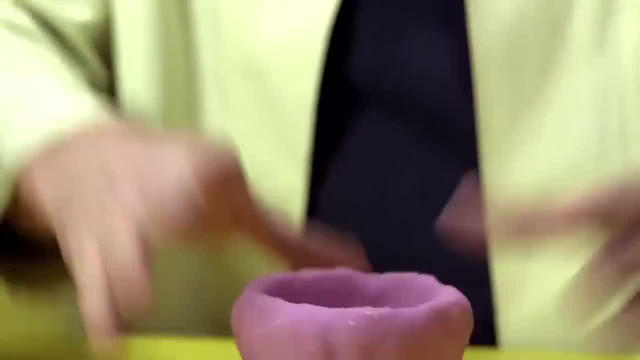 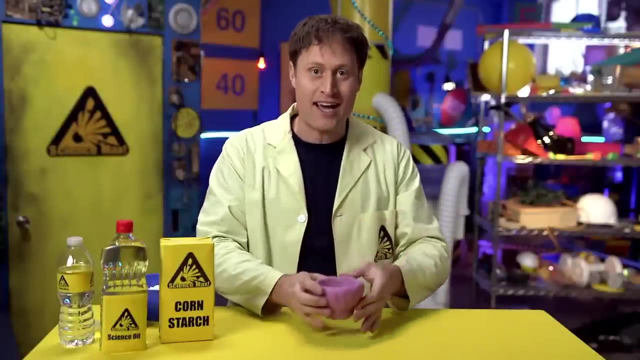 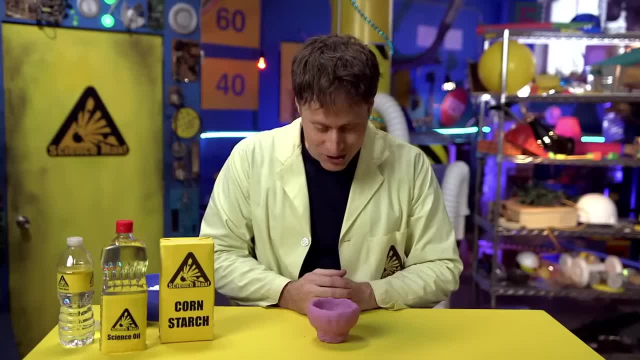 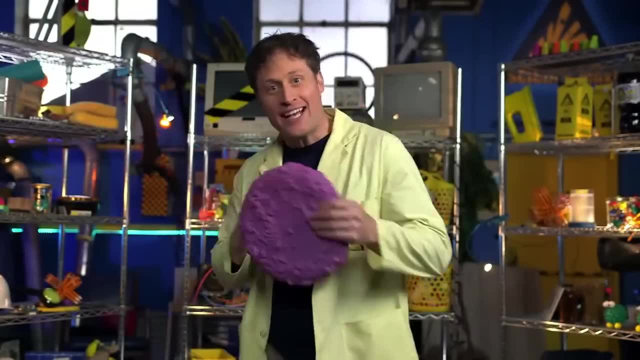 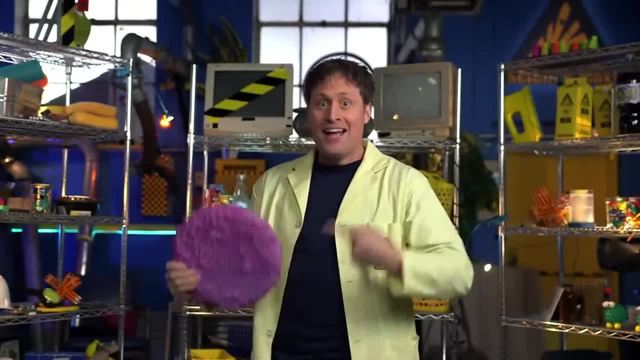 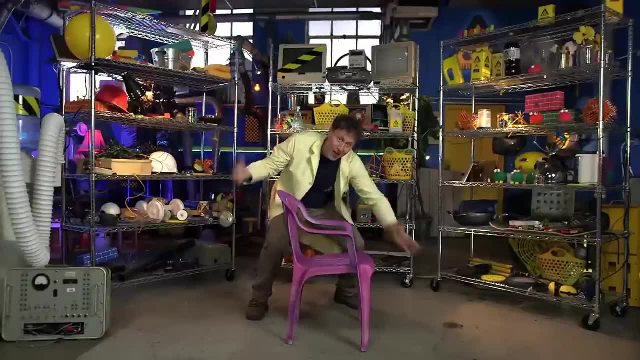 So you throw it around in the park, But if you lose it it turns back into dirt. Ha ha, What? Not enough, Okay, Clock wipe Biodegradable lawn chair, Use it for one season and then return it to the Earth afterwards. 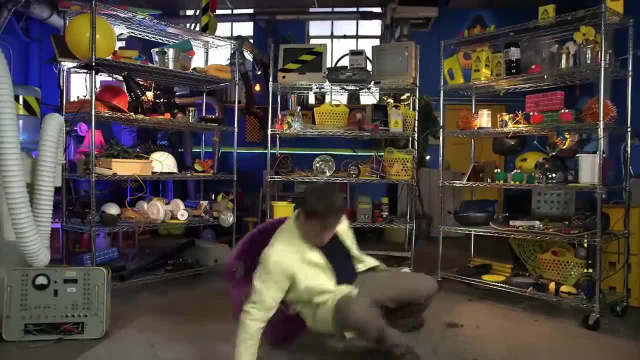 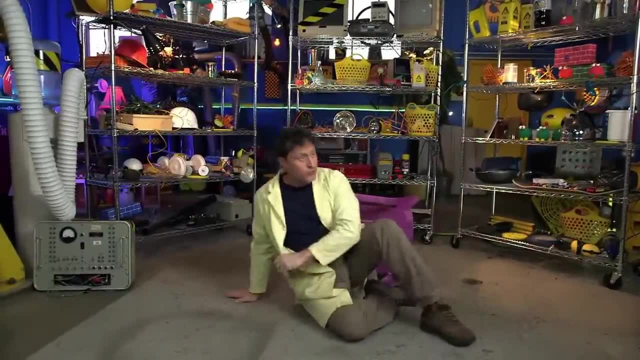 I think this is one of my best Science, Macs I Okay bioplastic lawn chair not as strong as regular lawn chair. We've learned that lesson now, so that's good to know. I mean, how would I have known if I hadn't tried it? 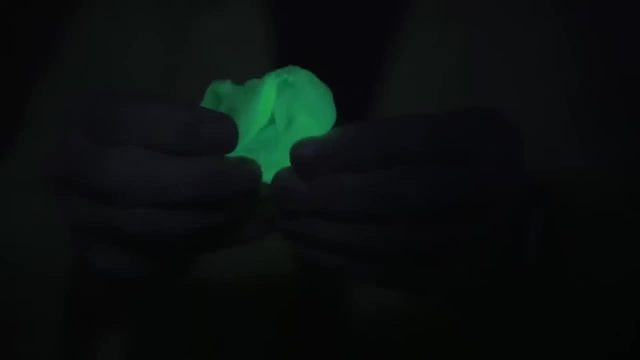 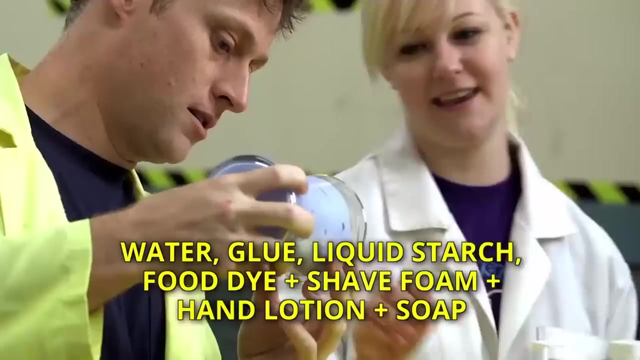 Sarah and I are looking at different recipes for slime. All right, what do we got here? Over here we have some amazing foamy slime which has so so many ingredients in it. Here, watch what happens when we start pulling it out. 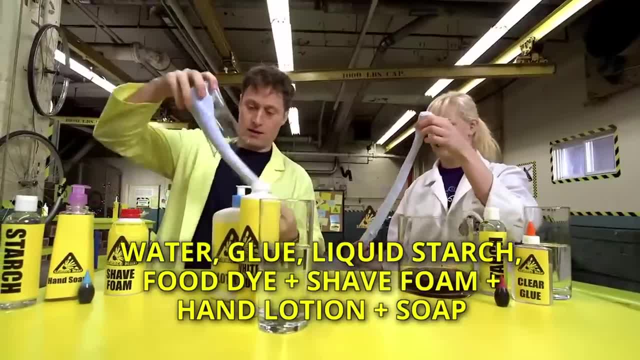 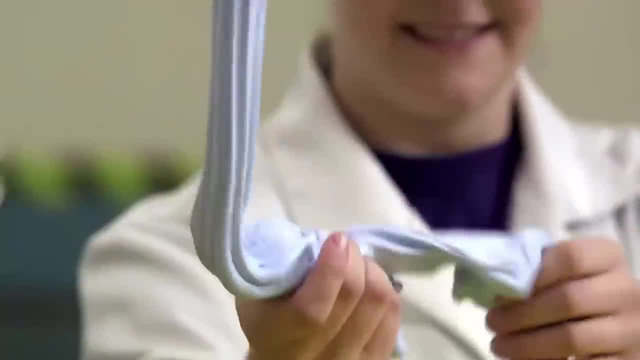 Ooh, wow. So it's like super stretchy and super fluffy. Yeah, that's great. Okay, now you gotta hold yours, You gotta hold this end. Then you take, and then take some more, and then we take that and then yeah. 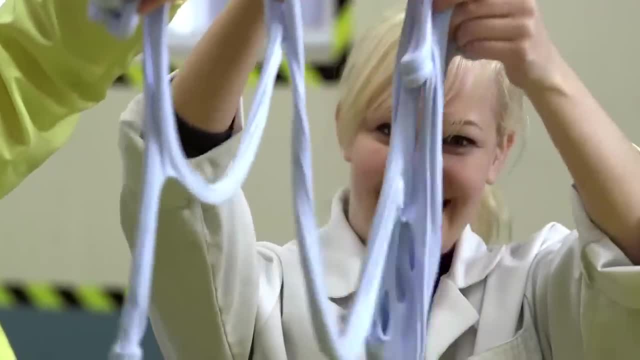 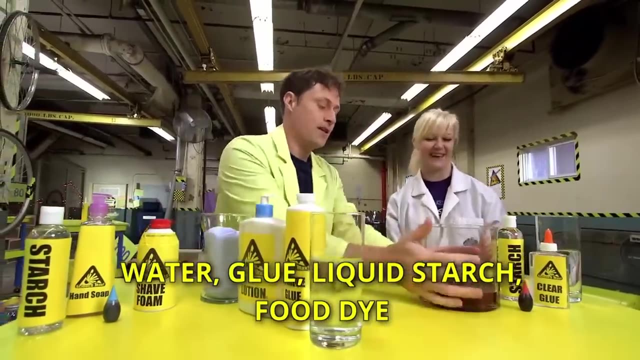 It gets thinner and thinner and it becomes more and more lines of foamy slime. Yeah, and the last kind of slime we made today is some classic flubber slime. Ooh, It's so much fun. Now, why do you think it's called flubber slime? 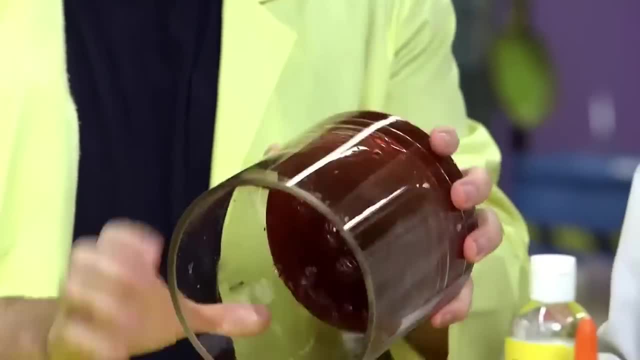 Because it's. is it really a slime? It is a slime, Yeah, It's super fun and it's super stretchy. Oh, okay, I get it. Look. look at that and it's sort of like like a little bit like gelatin. 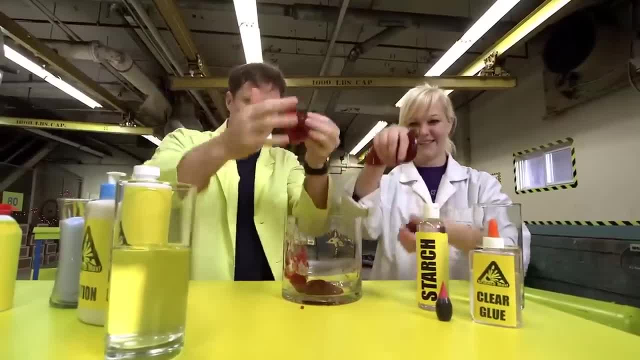 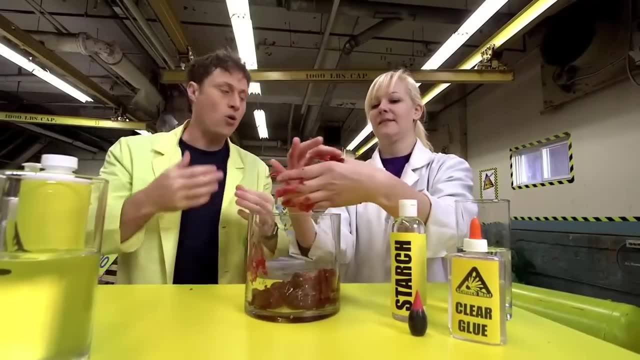 It is almost like gelatin: Here you can have some, There you go. Whoa, Oh, oh, oh. All right. so, Sarah, now what we need to decide is how we're gonna max it out, Right? 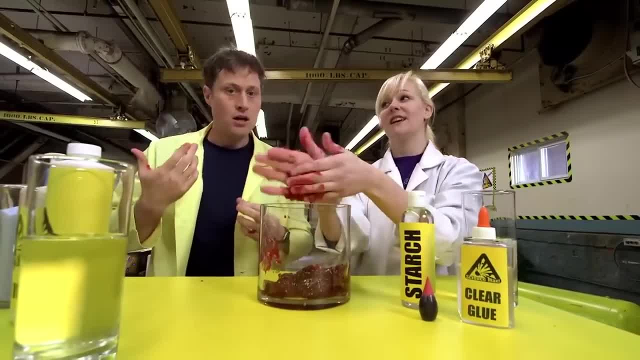 Like: should we just get a lot of slime? That sounds like a really good idea, but we are gonna need something to put it in, cuz we can't just have slime all over the floor. Okay, you're right, So we'll get. we'll get some sort of container thing. 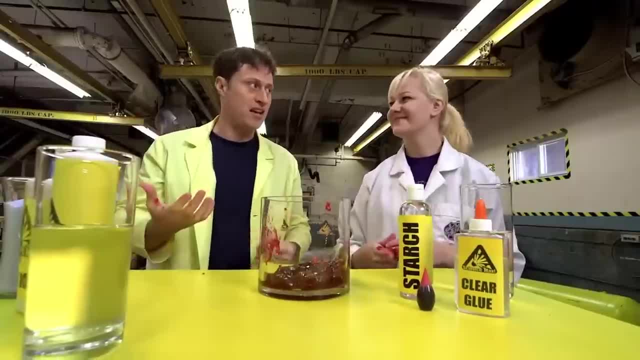 Yeah, And we'll see how much, how much slime we can make, and then we'll just play with it and see what happens. Sounds good, And we will experiment, cuz it's science. Yeah, Okay, high, high five. 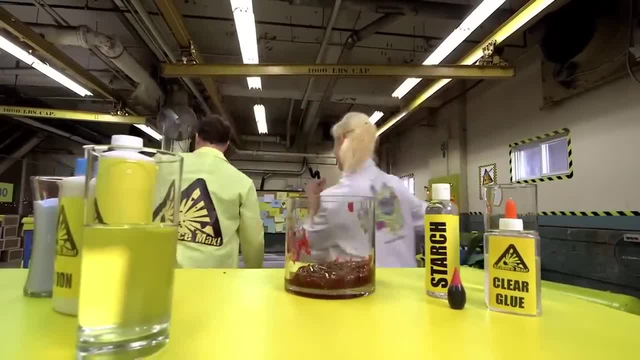 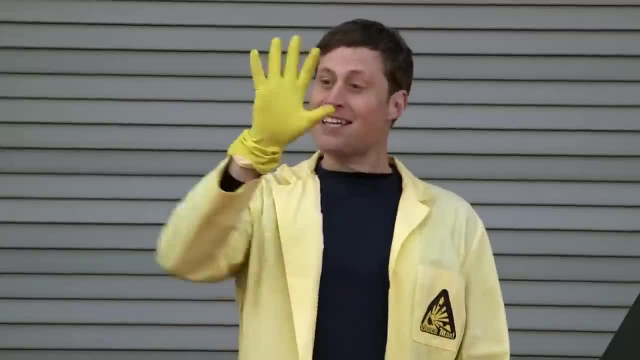 Careful high five so we don't splatter. Okay, good, Okay, let's go. This is like: This is a rubber glove. Well, actually it's a latex glove. What's the difference? I will get to that in a second. 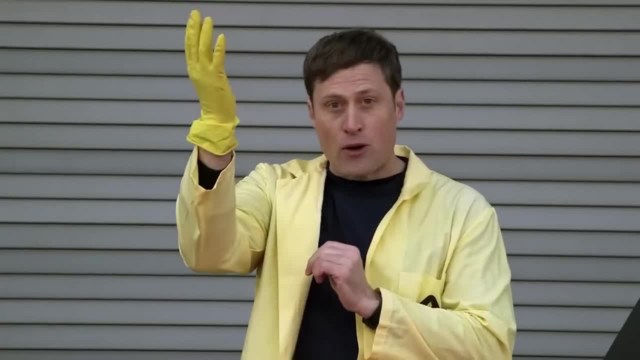 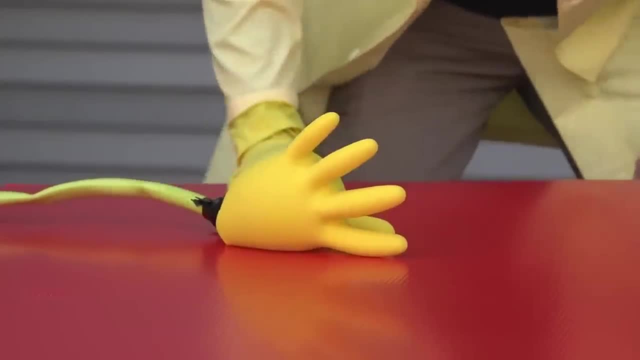 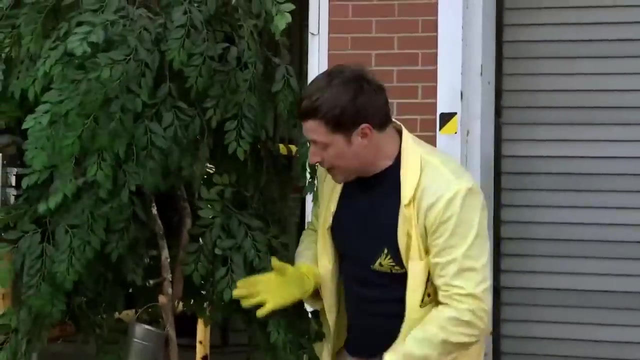 But I'm sure you can agree, it's super stretchy. How stretchy. Let's try it. Let's fill a rubber glove with water and see how big it gets. So difference between latex and rubber: Well, it all comes from a rubber tree. 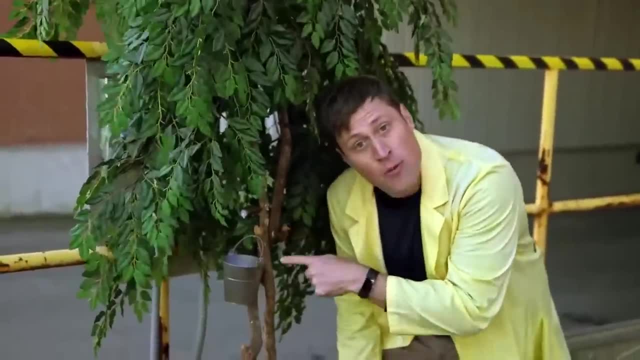 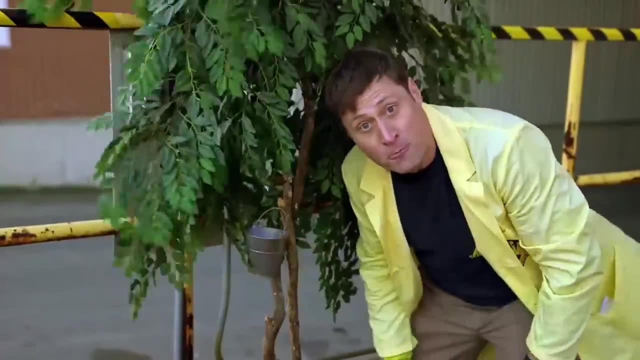 Well, actually it's a fake tree. It's just to show you how it works. The sap of the rubber tree is collected just like this: There's a spigot and then the sap goes out and it's collected. It's the same way that the sap for maple syrup is collected. 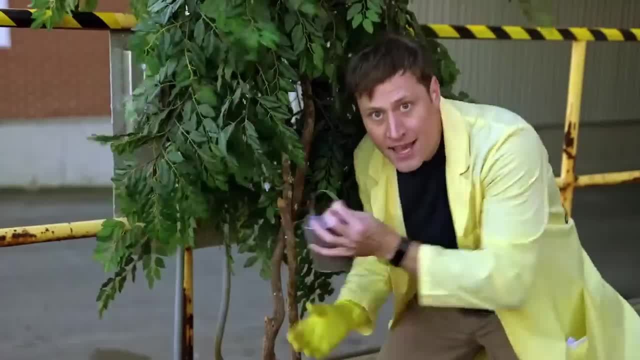 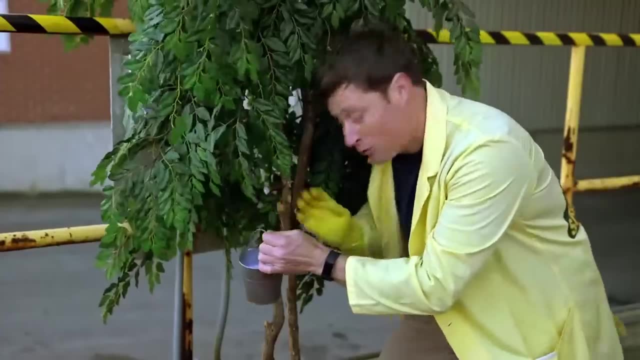 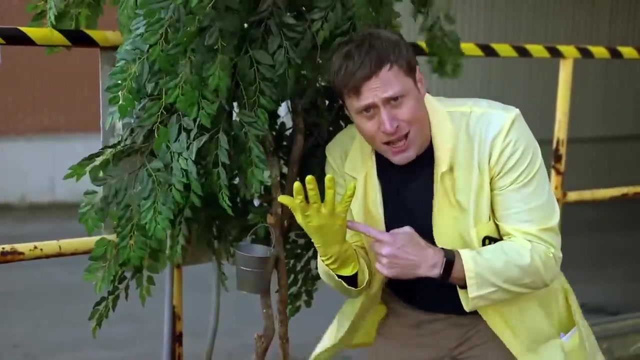 And this? this is natural, Natural latex. If it's dried out, it becomes natural rubber. Latex generally means the liquid form and rubber means the solid form. But wait then, why is this a latex glove? The glove is not liquid. 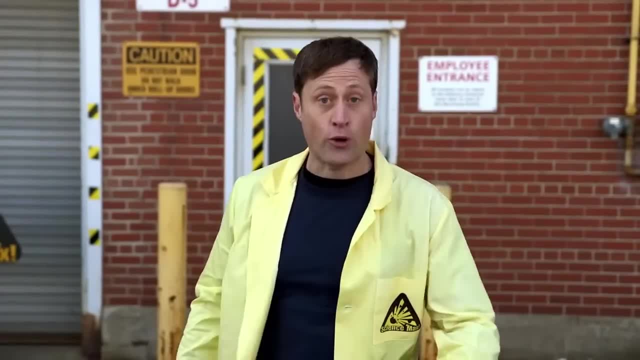 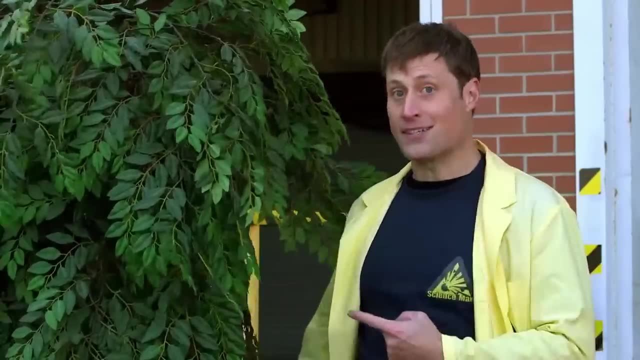 What's the deal? Well, generally latex means water-based or liquid, like latex paint, But it could also mean synthetic latex, That's latex that's man-made and doesn't come from a rubber tree. So we call rubber gloves rubber gloves because they're 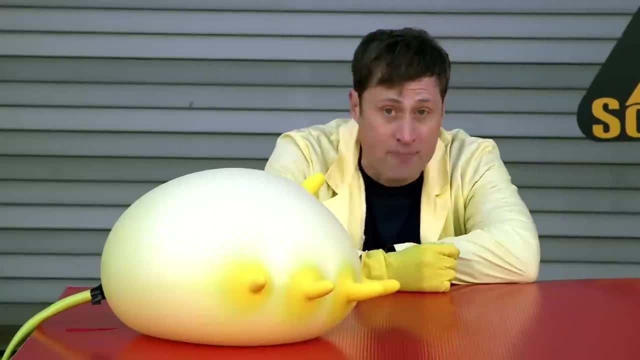 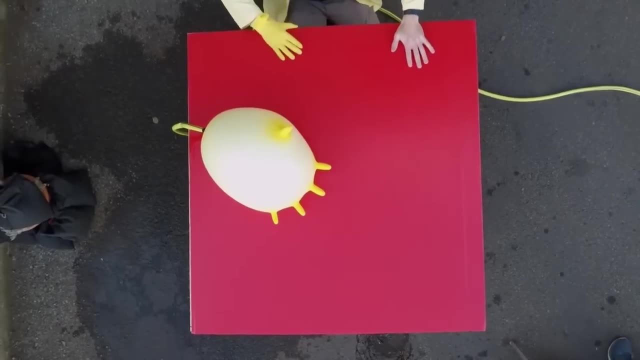 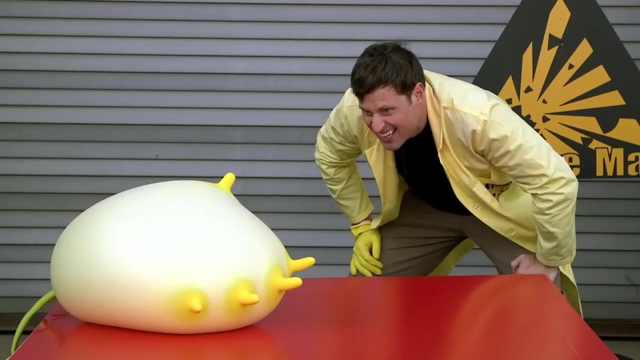 because they used to come from rubber trees, But now they're usually made out of man-made latex. But either way they're super stretchy. I wonder how big this is going to get. Science, Sarah and I are maxing out Polymer Slime. 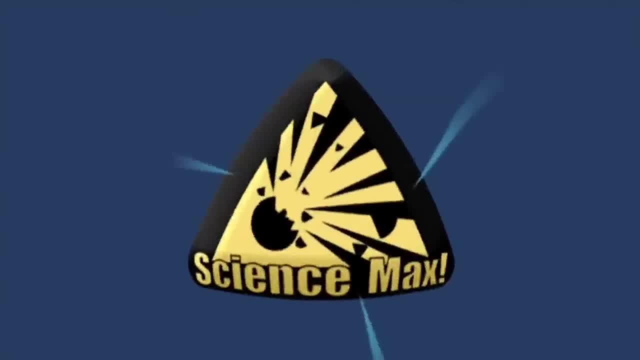 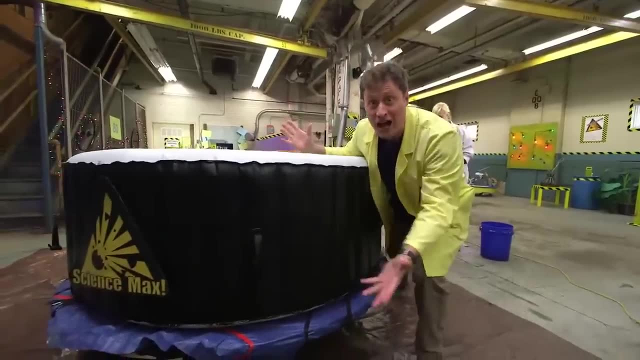 That's what we're going to do. Science, Science. How Maxed out tub of slime? Whoa, Okay. so how do you feel Is it? are we mixed up enough? First, we mix up a bunch of slime in a garbage bin. 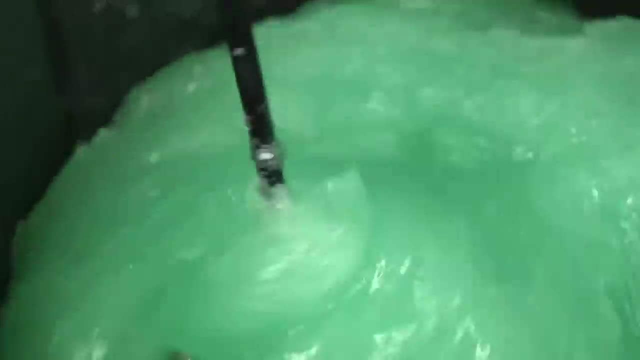 So with the polymer chemistry, the polymer is generally a liquid, right Yep, And the bonding agent makes it stick together. So the more we use, the more of a solid we get. Exactly, yes, So we want to split it and make it sort of halfway between a liquid and a solid. 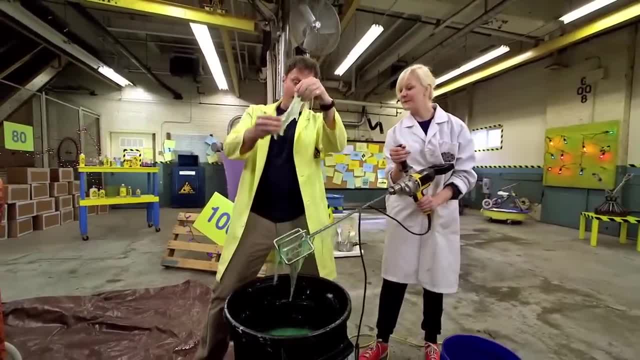 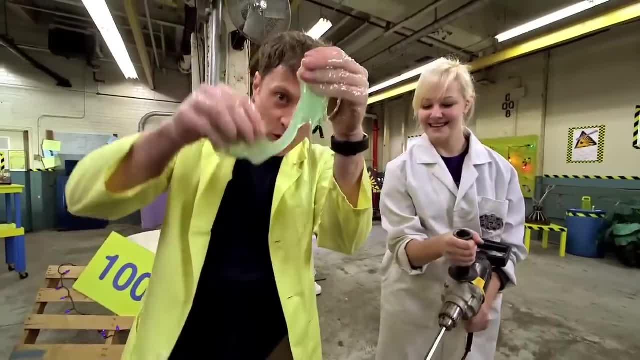 Let's take a look. Let's take a look, Let's take a look. All right, Then we dump it in. Oh gross, Whoa. It turns out we needed more slime. Um, I don't think that's going to be enough. 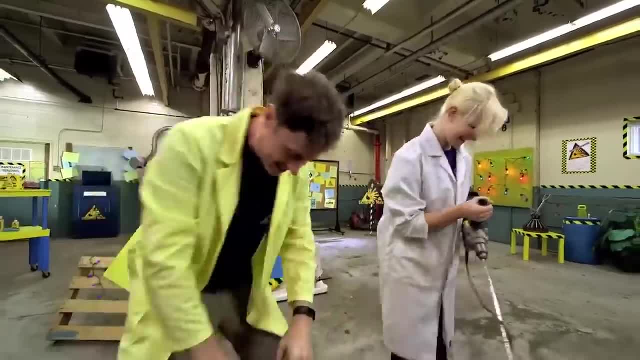 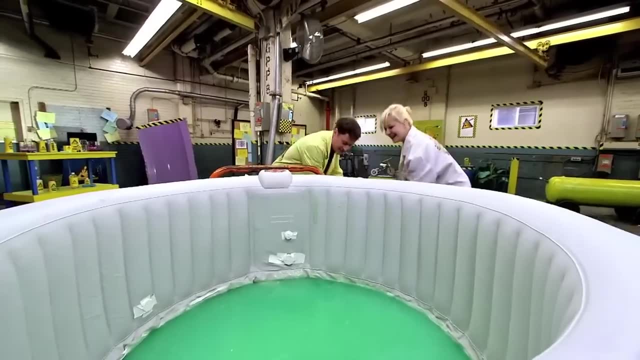 I think we may need some more slime. Yeah, How much more do you think we need? So we added 11 more. Oh, Whoa, Whoa, Whoa, Whoa, Whoa, Whoa, Whoa. 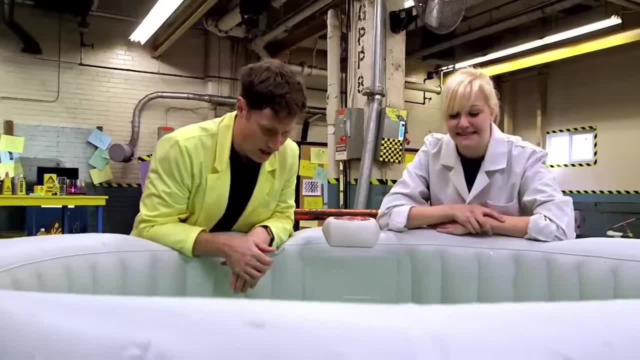 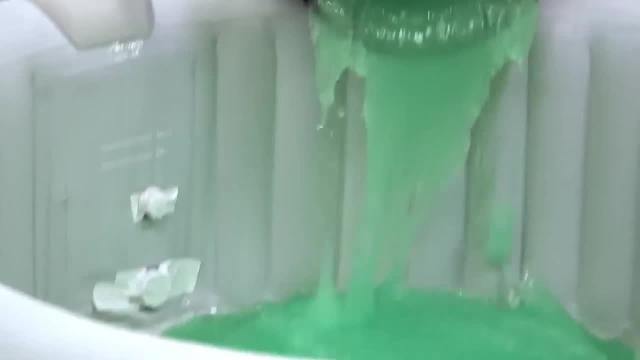 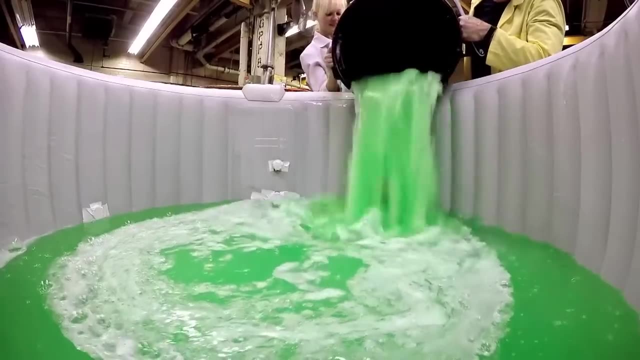 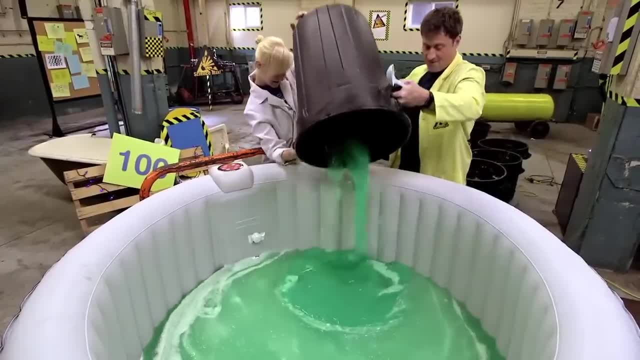 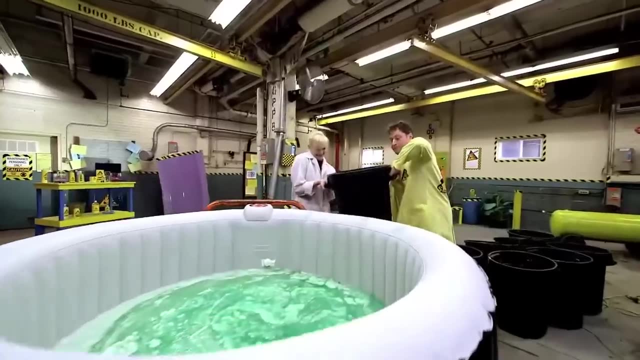 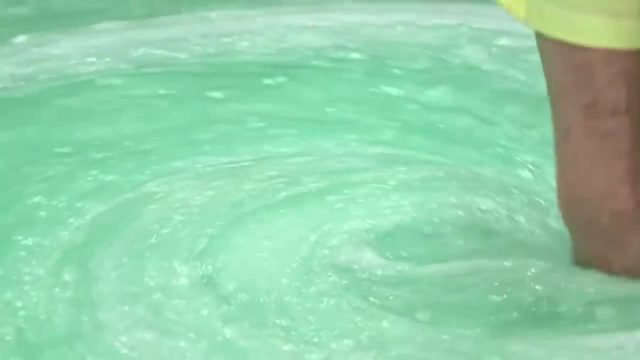 Ah, delicious, Ah, Very good, Yeah, Oh, Last one, Last one, Oh yeah. Then we experimented. Oh, Oh yeah, We have a giant, giant tub of slime. Ha, ha, ha, ha, ha ha. 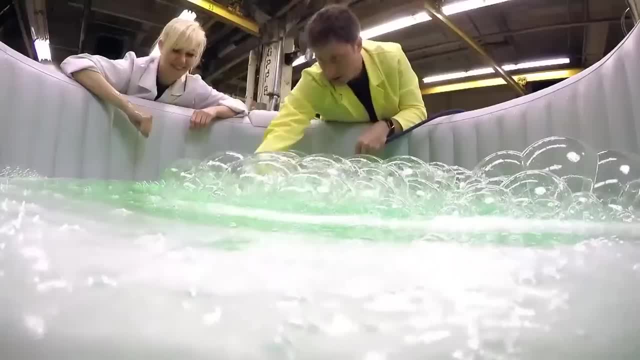 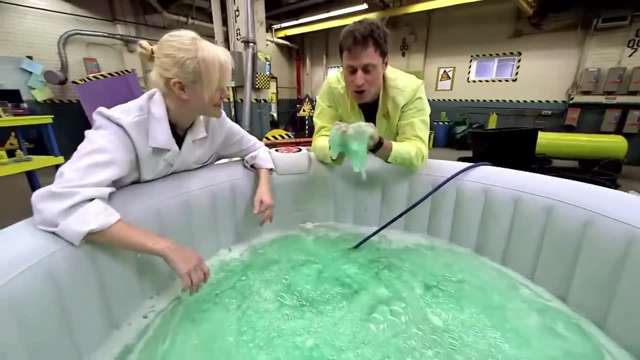 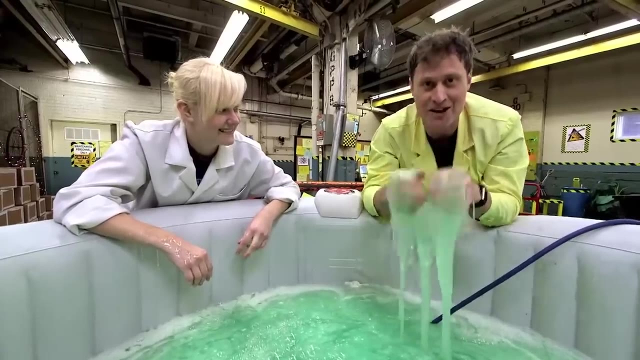 Because the slime is stretchy, it created amazing bubbles. So do you think I could blow a bubble with the slime? Well, maybe not you, but definitely the air compressor. No either. No, I'd have to just put it on my face. 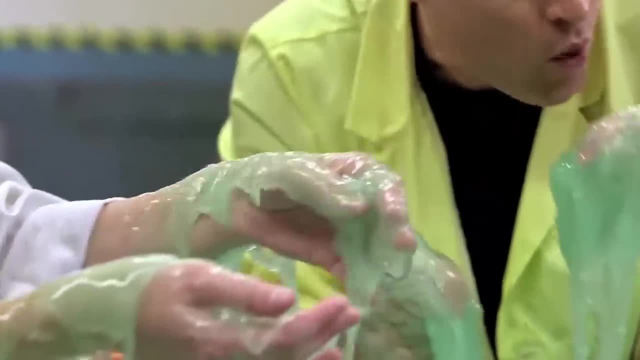 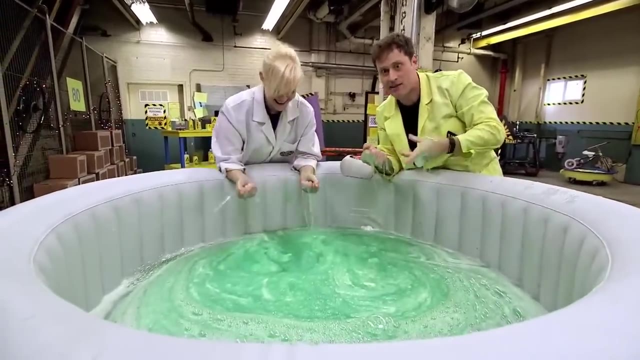 I think I've already got it on my face. Then there was only one thing left to do: We get in the slime. Can we do that? We can totally do that. This is Science, Max, That's so exciting: Going swimming in slime. 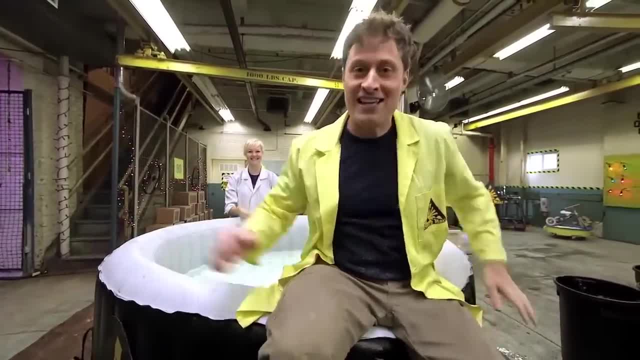 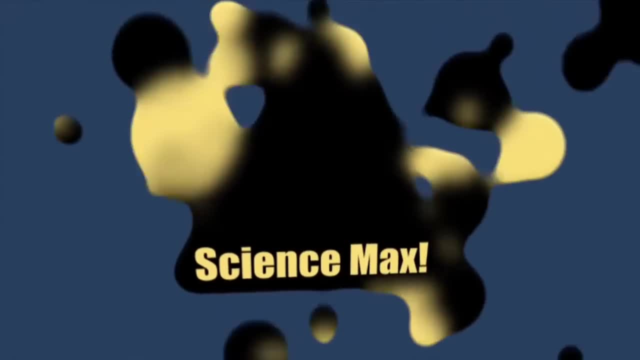 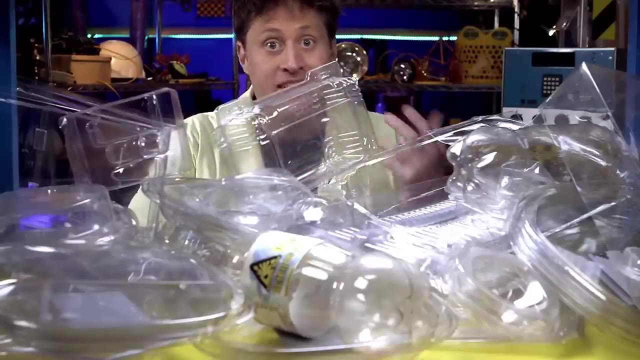 Who's going first? You are, I am obviously All right. this is how Science Max does. polymers, Three, two, one. Plastic is everywhere, but what can we do with it, aside from recycle it? Well, we can reuse it to make cool plastic charms. 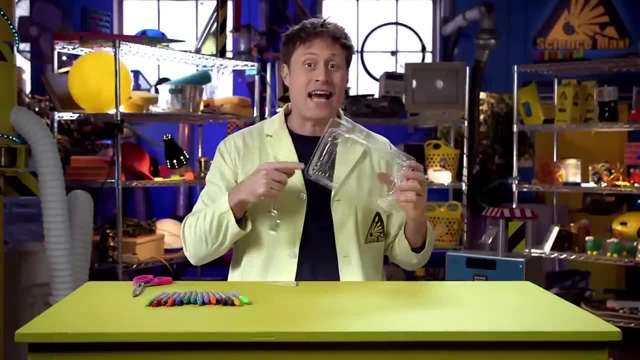 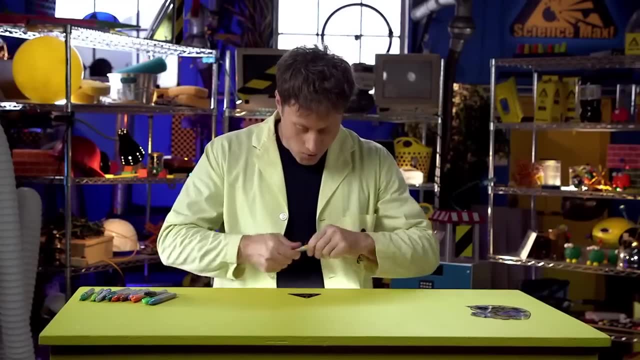 But you're going to need the right kind of plastic And you need polystyrene. Just look for the little number six inside the recycle symbol. Cut out some plastic and decorate it however you want. There we go. Ha-ha, check it out. 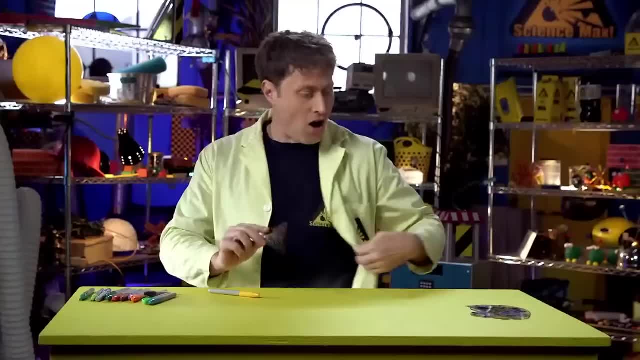 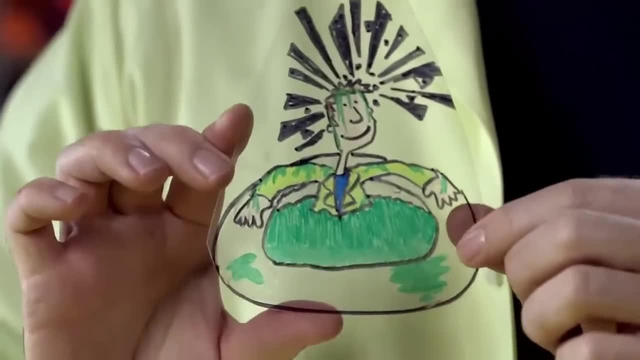 The Science Max logo Also. I've made a couple other things. I've got a chemical symbol, an atom and this is me in some slime. Then get an adult to help you put it in the oven or Toaster oven. 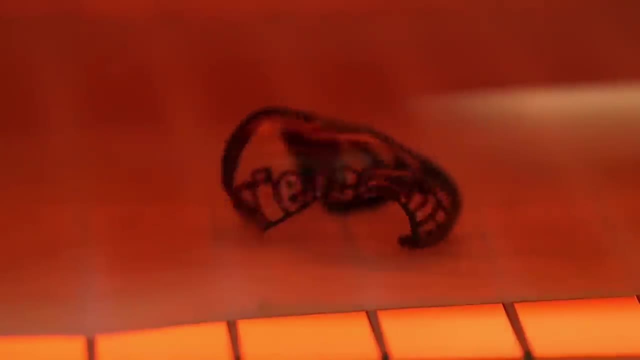 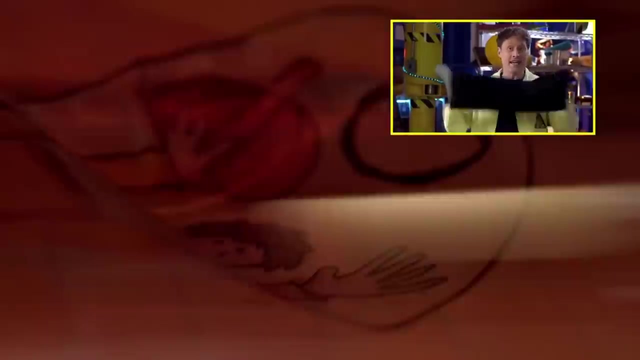 At 350 degrees It only takes a few seconds for the plastic to shrink to one third its size. The reason why this happens is when plastic is manufactured, it's heated and stretched out and then cooled and it sort of freezes in that stretched out shape. 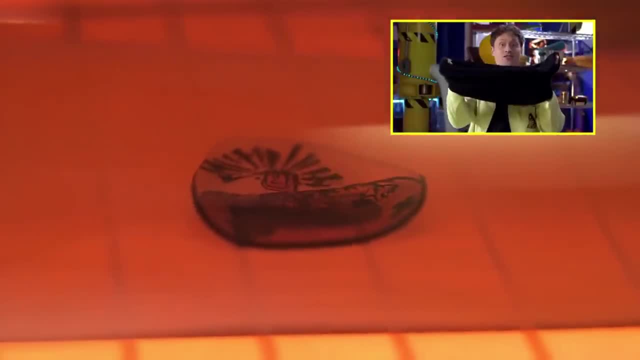 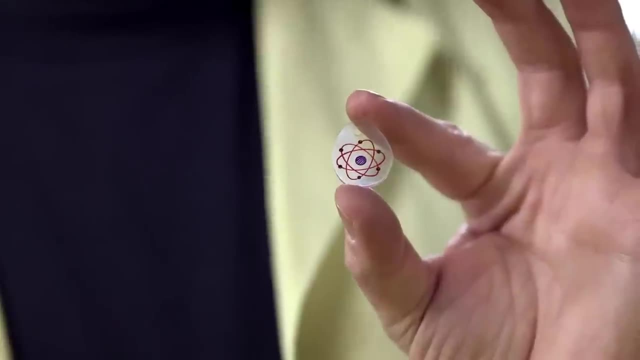 And when you reheat it it shrinks back down to the unstretched shape. Get your adult to take it out and wait for it to cool and you'll have yourself some small plastic designs you can use for keychains, bracelets, name tags, bookmarks, whatever you want. 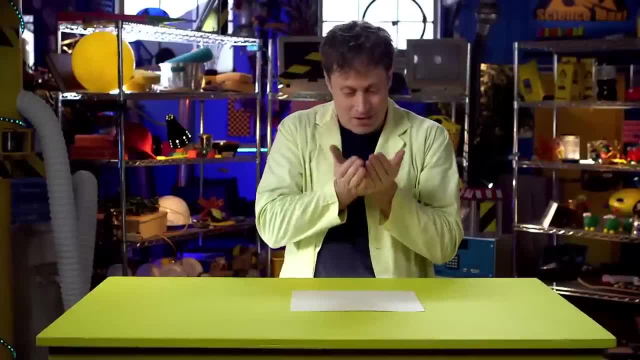 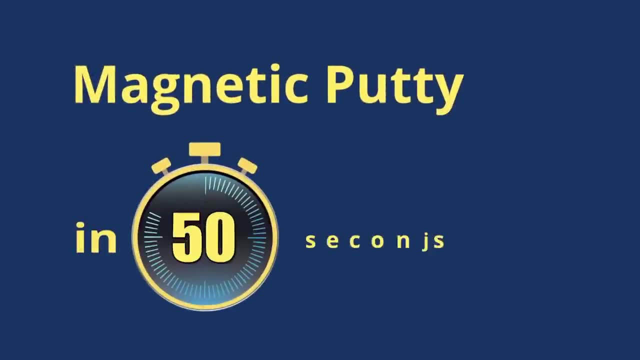 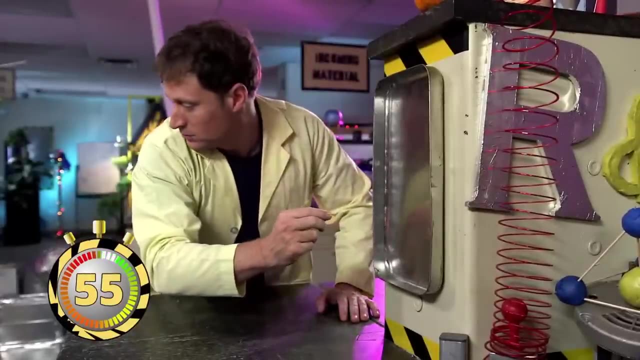 All using the power of polymers. Awesome, I'm going to make all of those. What was that again? Keychain Ornament, Magnet Um, Magnetic putty in 60 seconds. This is magnetic putty, Take it. 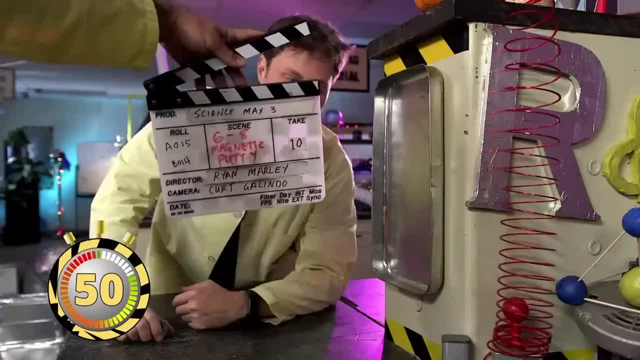 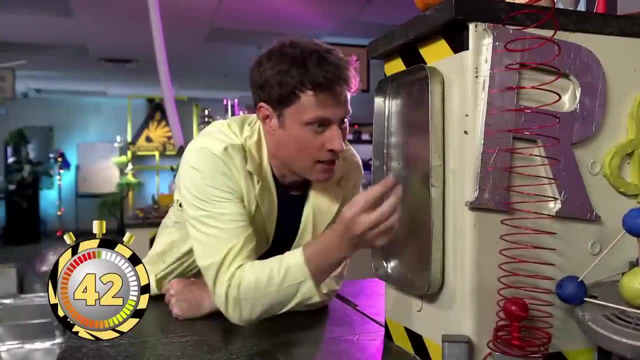 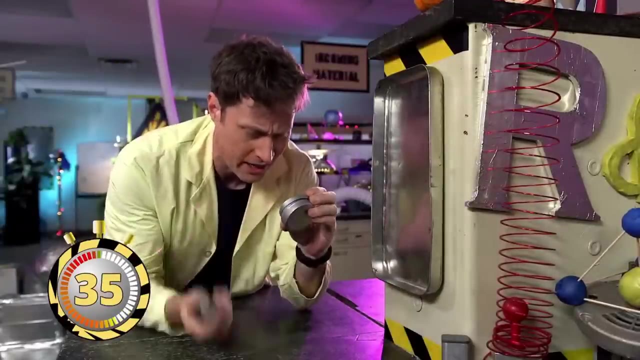 This is magnetic putty Ten. take. This is magnetic putty Twenty-six. This is magnetic putty 2,635.. This is man. this is magnetic putty. I can't count this high. This is magnetic putty. 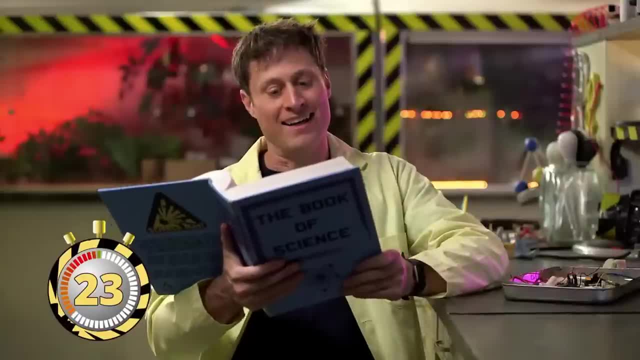 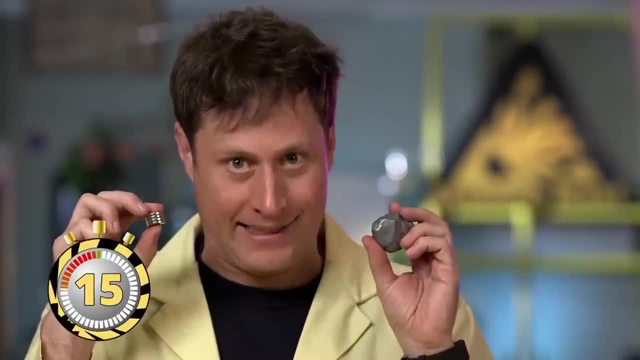 Ha, Magnetic. Oh, it's not a magnet, It's attracted to magnets. Oh, that makes more sense. This is magnetic putty and this is a magnet. The putty is made of polymers, which means it can flow over itself. 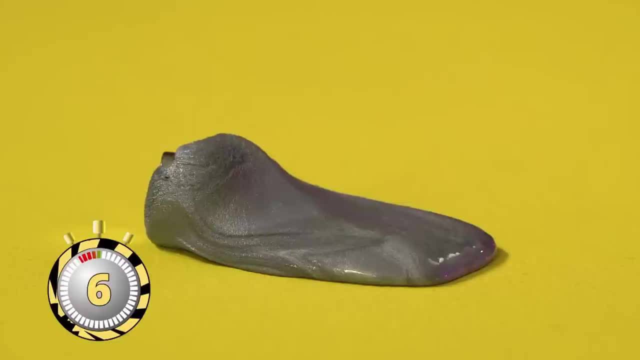 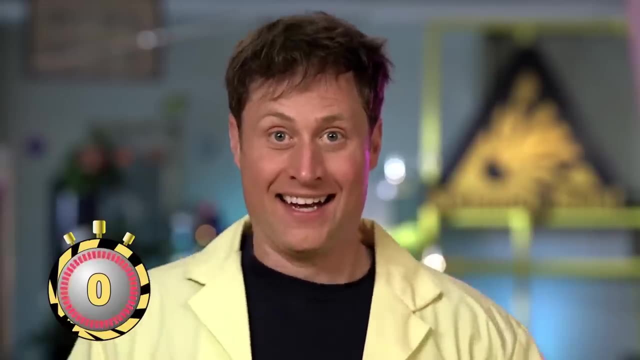 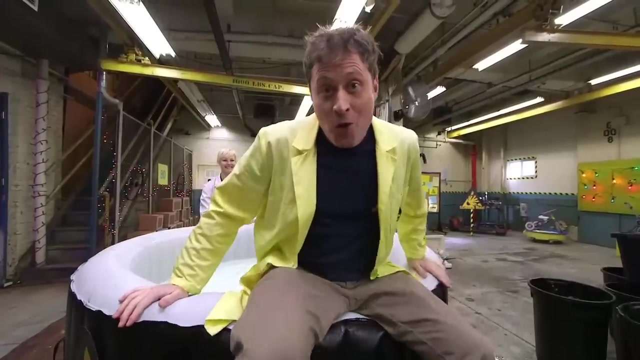 It also has lots of iron filings in it, which is why it's attracted to magnets. This is what happens over several minutes And there you go: Magnetic putty. Okay, So where were we? Oh yeah, 3,, 2,, 1, yeah. 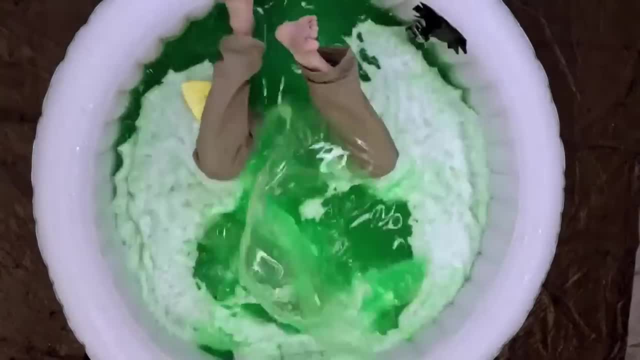 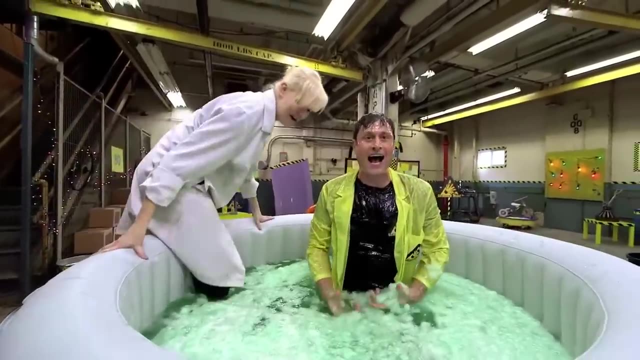 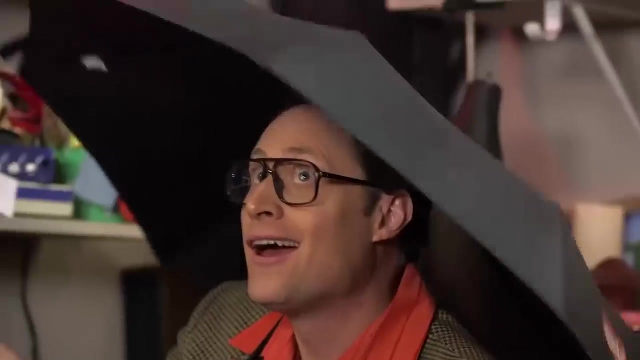 And remember, don't try this at home Slime: Sarah and I enjoyed our maxed-out tub of slime. So let's recap: Slime is made of polymers. Polymers come in a lot of different forms. It's all about long chains of molecules. 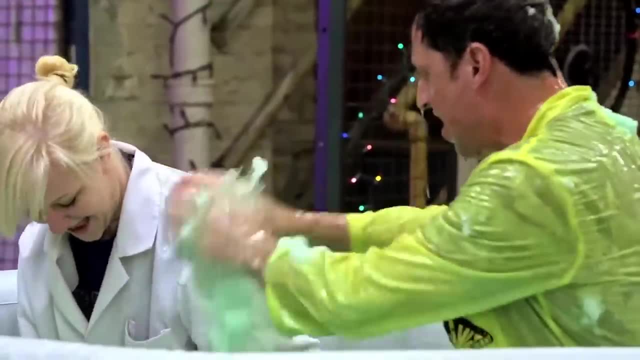 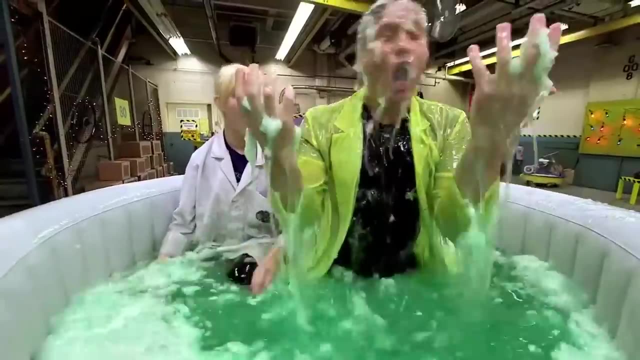 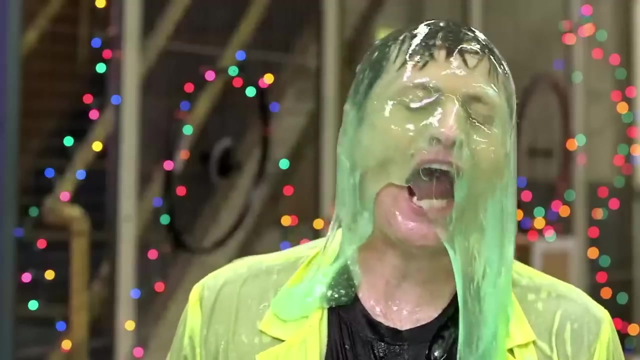 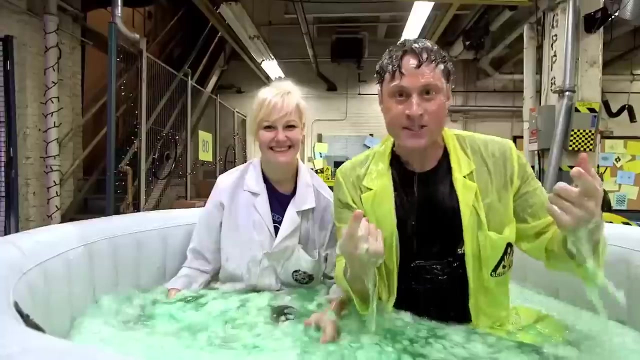 And none are more fun to swim in than slime. Do I have slime here? Yeah, definitely. Slime here. Slime. Well, there you go. Science match Experiments at large Polymers- Slime- Yeah, High fives. 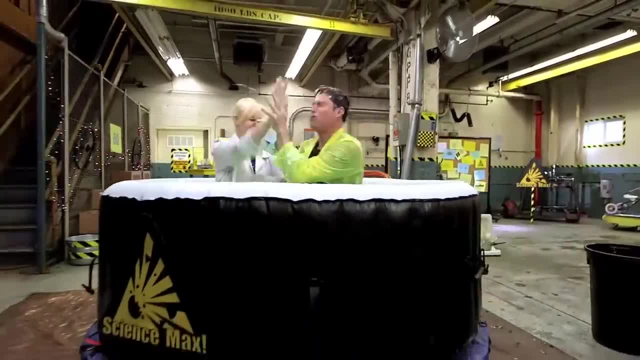 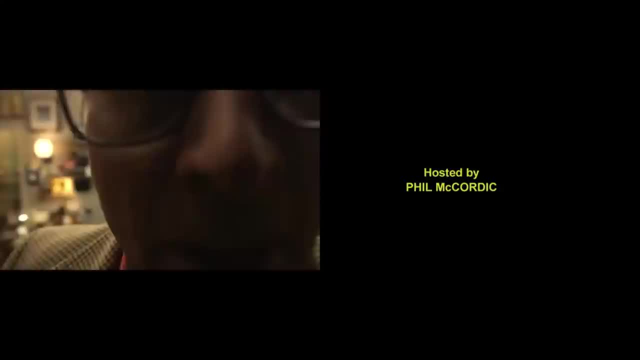 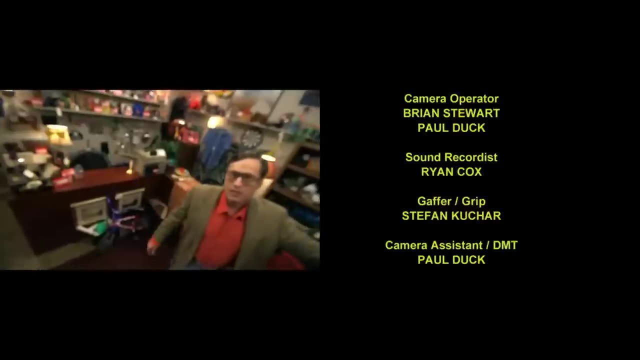 Yeah, Slimey, high five, Take three, Do it. Yeah, Do you see it? Is it still close? Am I too close to the camera? Biodegradable frisbee. Am I looking at this camera Or is it this one? Is it this one? 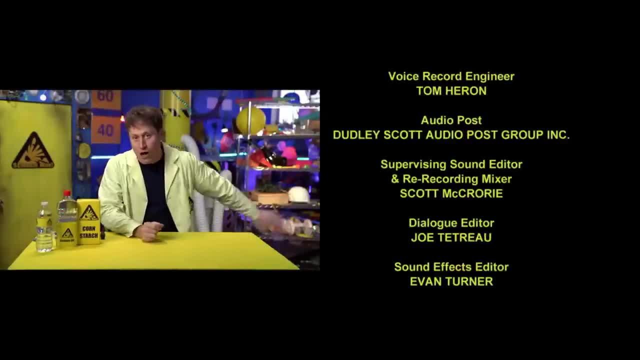 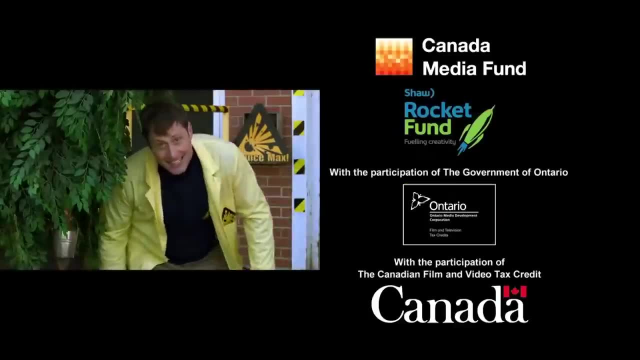 First, you need that bowl. I told James to go and watch, Forgot to ask him back for that. But hold the phone. Nylons, Nylons, That's latex, that is man. Ugh, Ugh, Science. 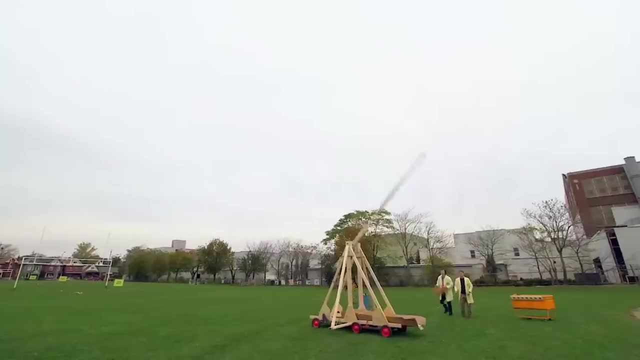 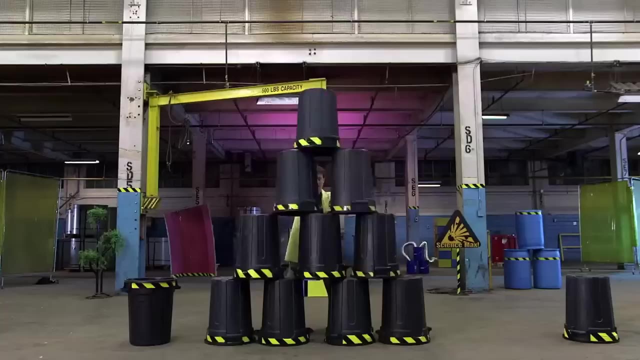 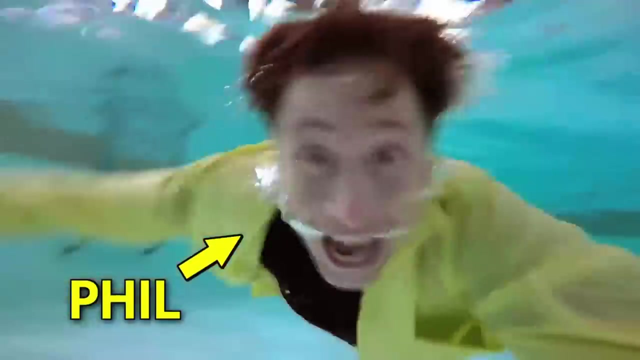 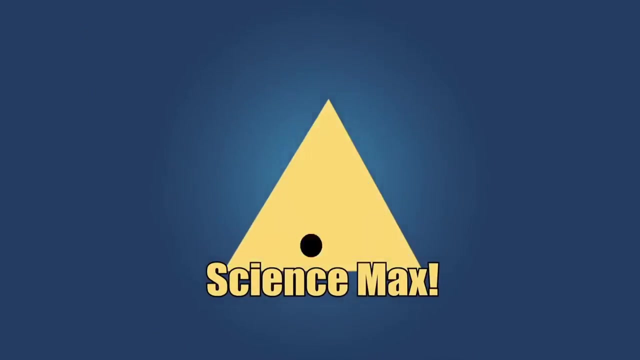 Have you ever done a science experiment and wondered what it'd be like if you did it big? I have, My name is Phil, and I take your everyday science experiments and do them big. This is Science Facts. Experiments at Large- Science Facts. 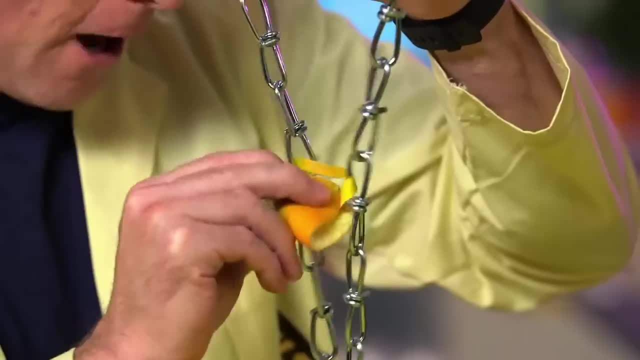 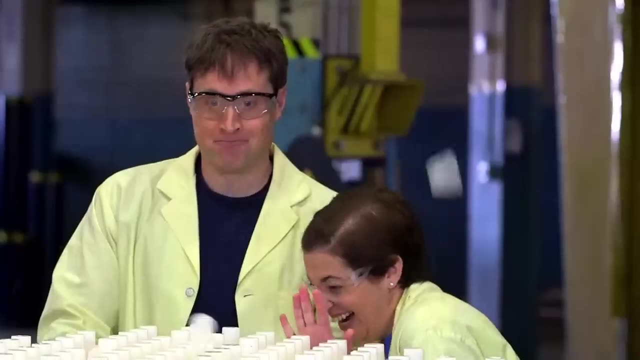 This episode is all about chemical reactions. Om nom, nom nom, Om nom nom, Om nom, nom, nom, Om nom nom. Delicious Reactions to make things fly, to make things glow, to make things pop and to make things fly. 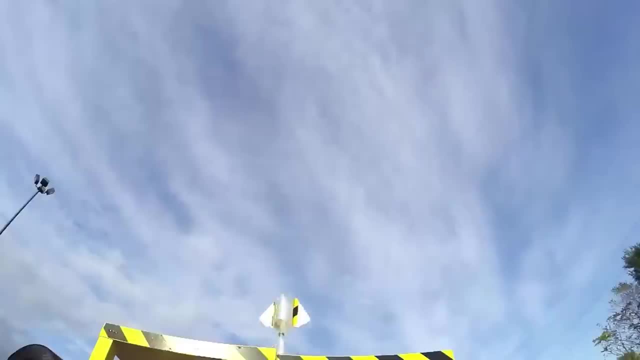 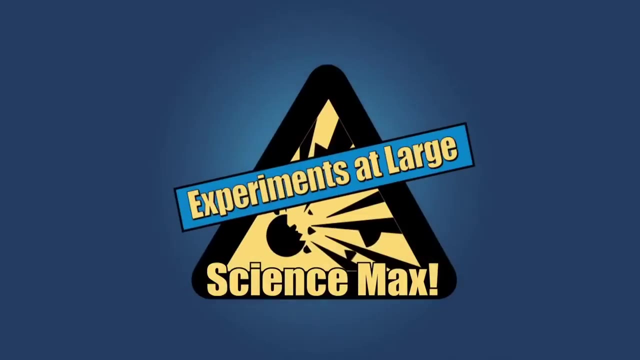 Hahaha, That worked. Wait, did I mention the flying? I'm sure I did, but I'm mentioning it again because it's awesome. All on this episode of Science: Max Experiments at Large. Okay, Science Maximites. 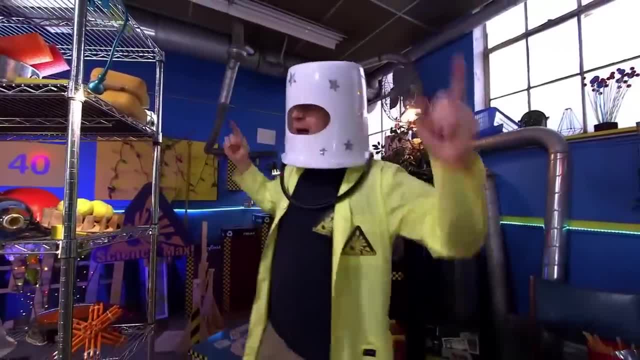 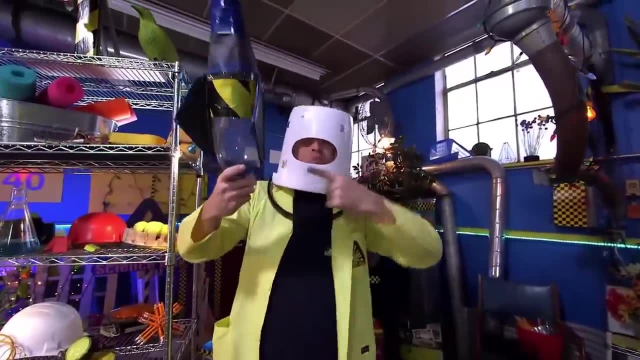 prepare to hurtle through the cosmos. I am Captain Phil, and today we're going to be building rockets on Science Max. Now, we've built rockets before like this one powered by air pressure, And this one stomp rockets. 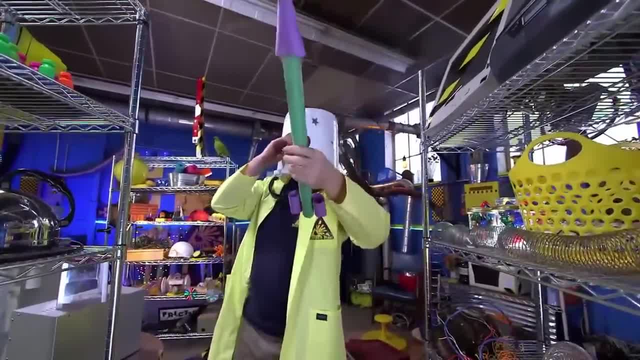 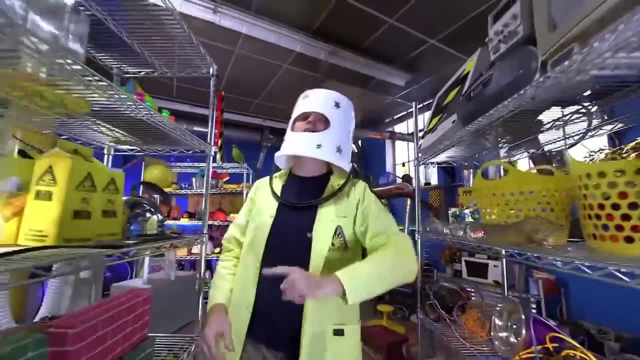 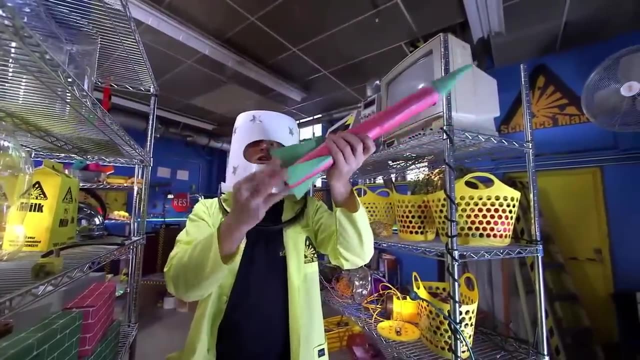 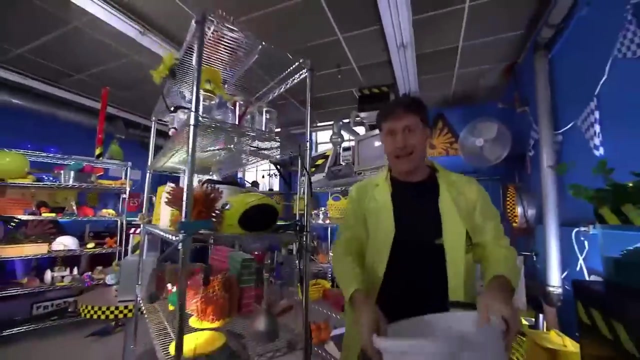 which were also technically powered by air pressure: Air pressure rocket. But today Science Maximites. we are going to be building rockets powered by chemistry- Chemical-powered rockets- away. Okay, I promise it'll be more exciting than that, Because today Science Maximites. 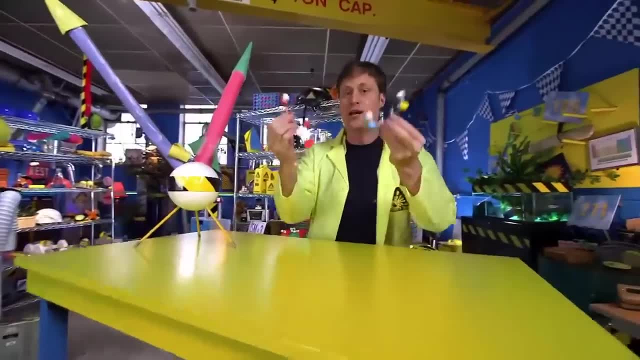 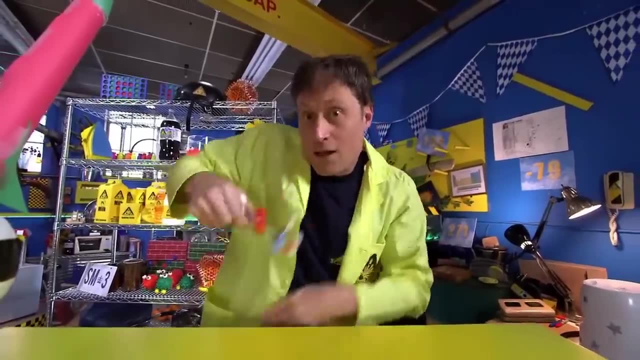 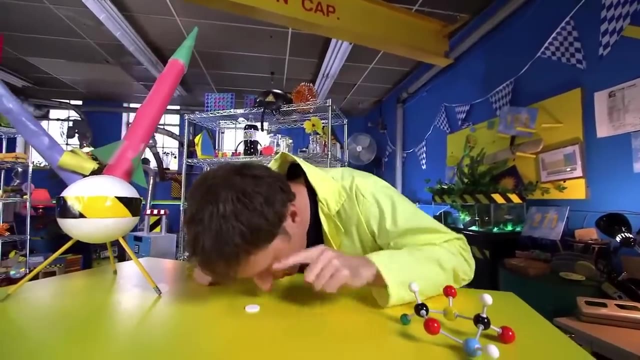 we are going to be looking at chemistry. Chemistry is when two molecules combine to make another molecule, Like magic Woo. So let's take a look at what will be powering our chemical rocket. This- It's an antacid tablet. When you put an antacid tablet in water, 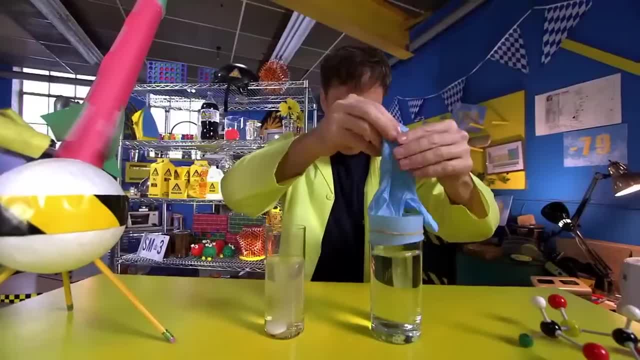 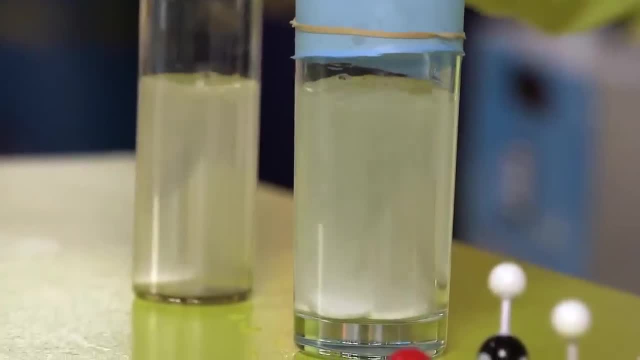 it makes little bubbles of carbon dioxide gas. This happens because of a reaction between two kinds of molecules called acids and bases, Like vinegar and baking soda, but all contained in a small package that won't start working until you put it in water. 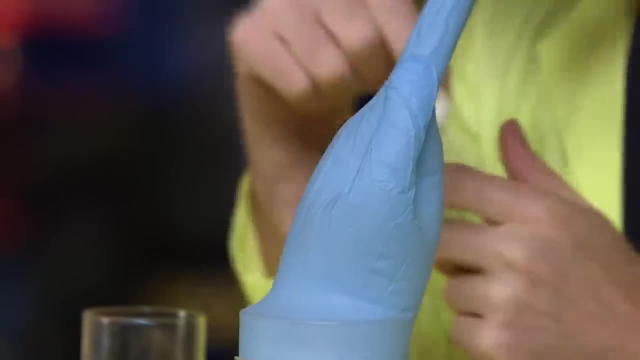 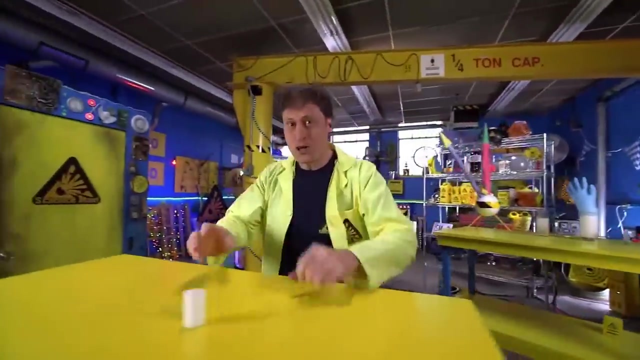 If we contain the reaction, the carbon dioxide gas builds up and creates pressure. High five for science. All right, so let's look at our chemical-powered rocket. What you need is one of these. This is a. This is a film canister. 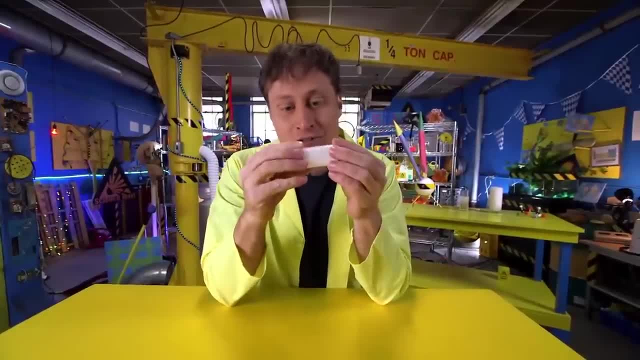 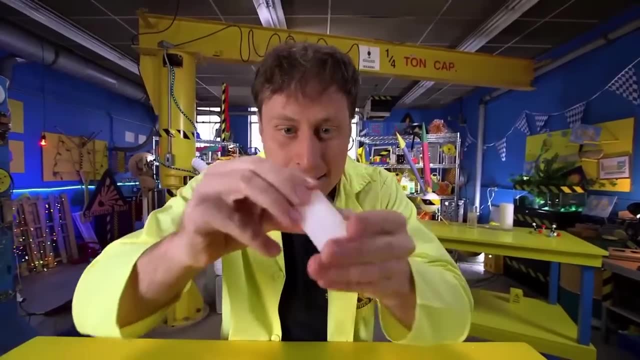 And ask your parents what that actually means, because they're not used for holding film anymore. You can get these at craft stores, though, to hold paint or little things, but really all you need is a plastic container with a good lid that snaps on nice and tight. 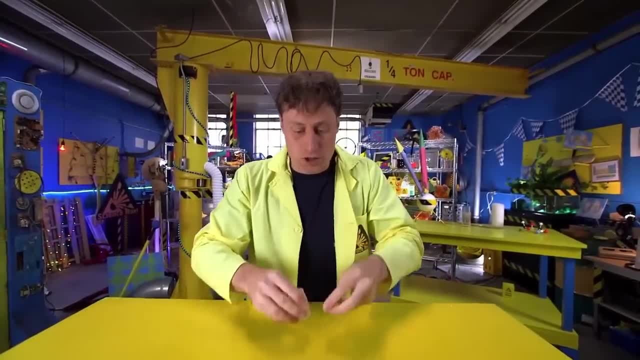 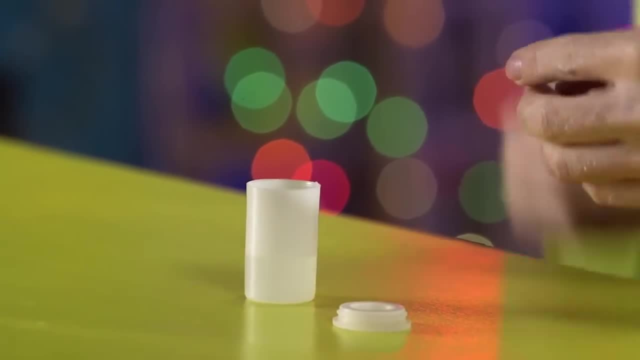 and keeps the air in. And then, of course, what you need are your antacid tablets and a little bit of water. So pour in some water and then put in your antacid tablet and snap the lid on, flip it over and wait for the carbon dioxide gas to build up. 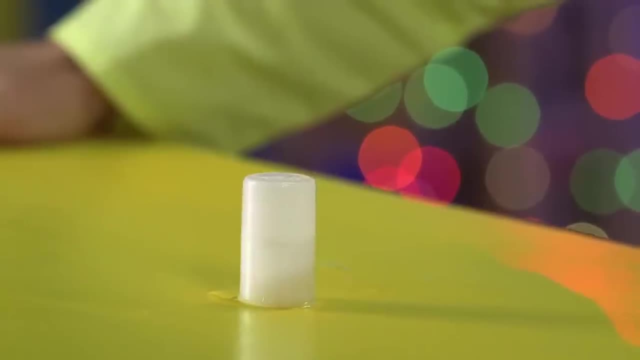 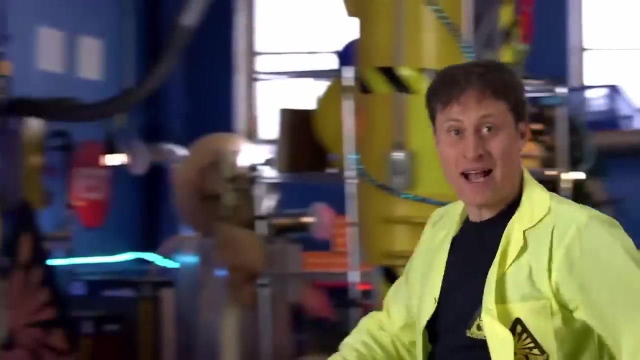 which will build up pressure which will launch your rocket. Ha-ha. So there you go, a chemical-powered rocket. Come on, let's max it out. So first I need an expert to help me, Um. 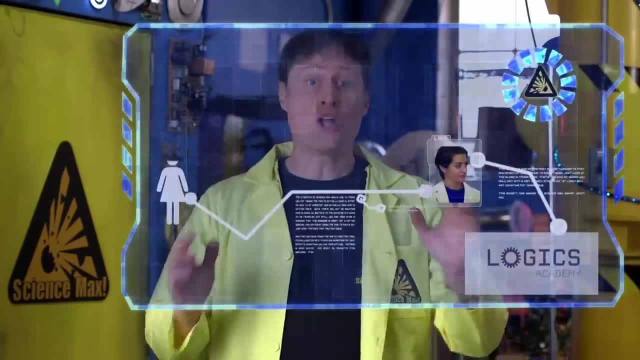 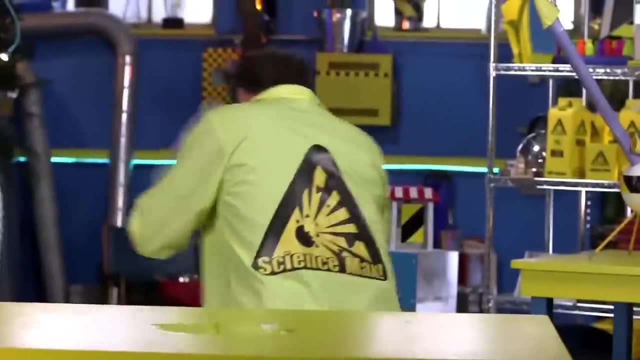 Oh, Lisa from Logix Academy, Of course Logix Academy. people have helped me launch all the rockets on Science Max. This is gonna be great. Ooh, I'm gonna get my helmet first. Okay, let's put. Let's launch some rockets. 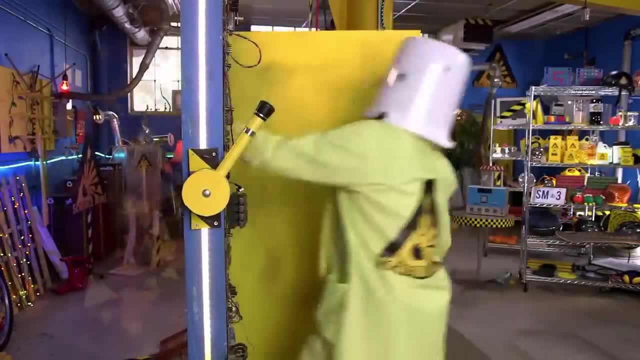 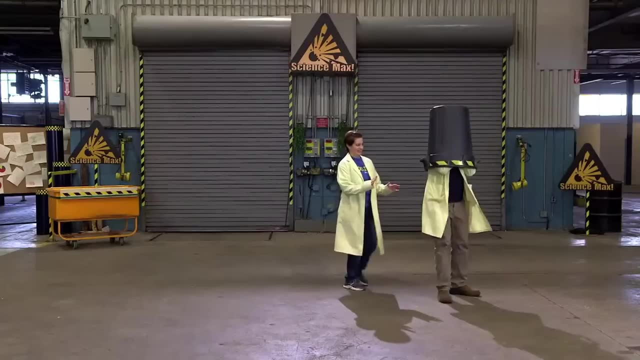 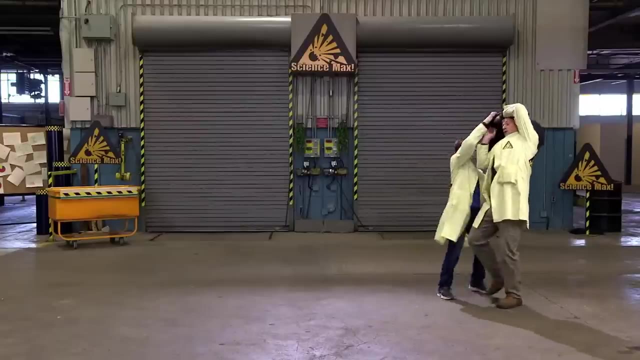 Let's go. Whoa wow, it's really dark in this room. I can't see anything. Bill L-Lisa, Bill Lisa, What? Bill Ugh? Oh, Oh, Oh. Where did this come from? 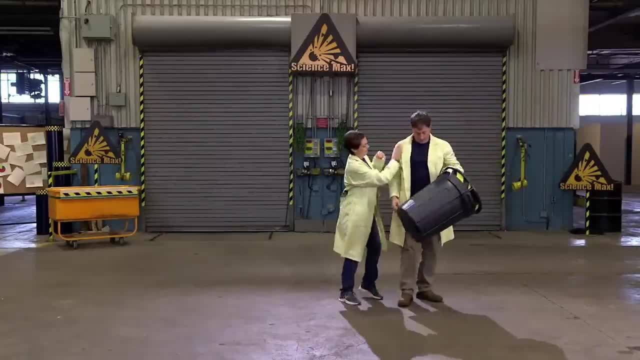 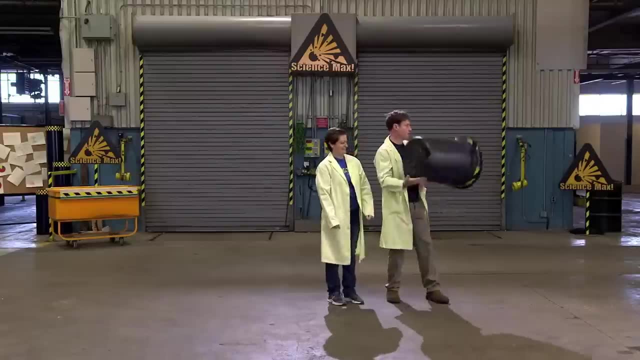 I guess the portal's malfunctioning. Hey Lisa, Hi From Logix Academy. great to have you here, Great to be here. Just put this over there: We are here to max out the energy of the rocket. So what's your mission? 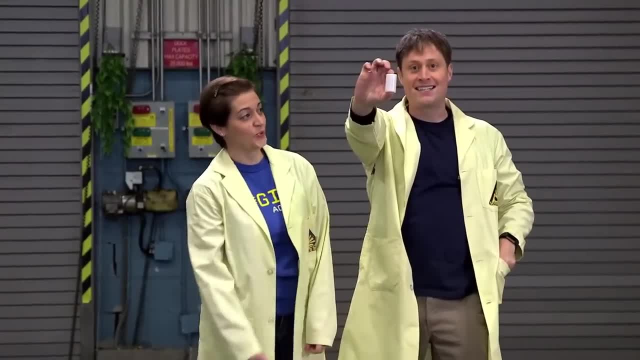 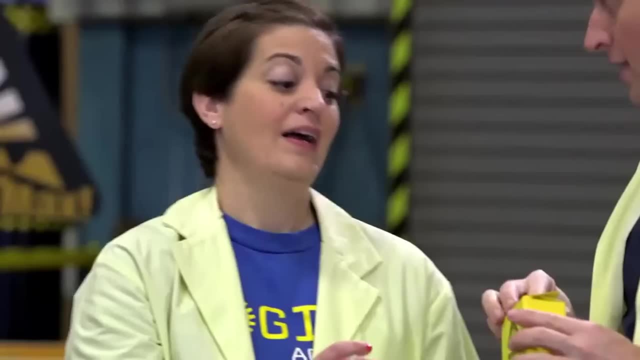 to max out the chemistry rocket: Ooh, what is that? It's just a small plastic container, But when we put an amacid tablet in there and some water, Ah, we get a chemical reaction. We get a chemical reaction, and so that's what creates the pressure. 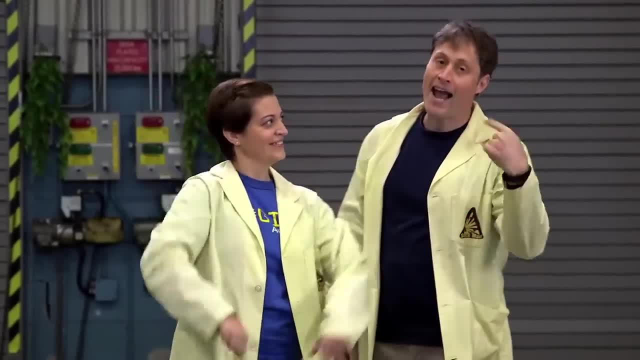 and then that pops the lid off and we get a little rocket Kaboom. But now we're going to max it out, Get a bigger container and more. Ooh wait, What? How about if we launch a whole bunch of them? 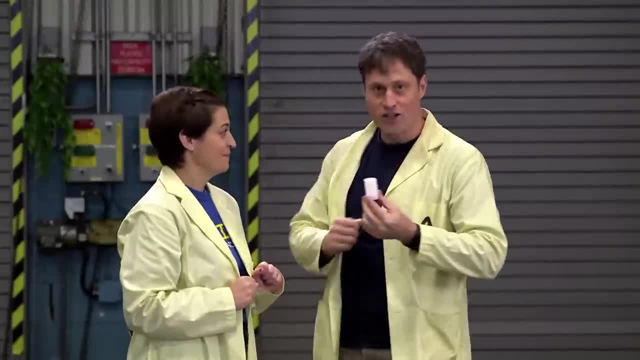 Ooh, so we just get a lot of the small one and we launch them all at the same time, Exactly, Okay, great, So we just need a whole bunch of these and a whole bunch of Yeah, and a whole bunch of science antacid. 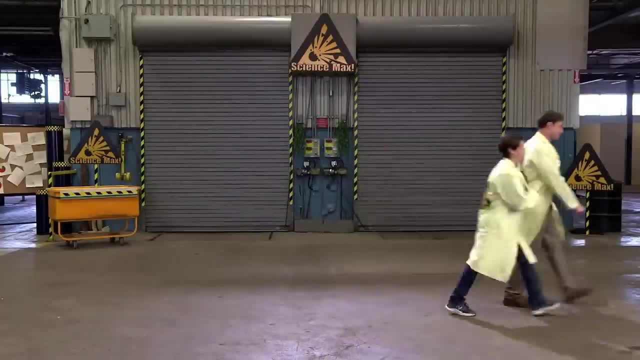 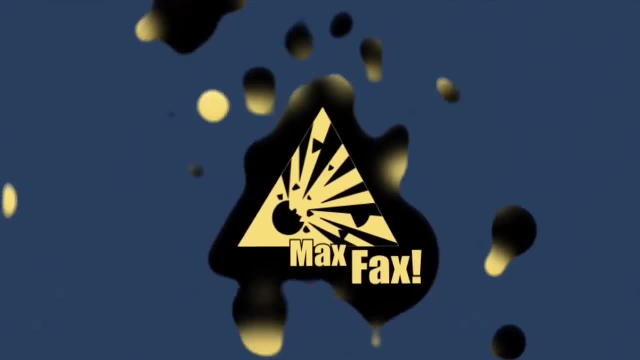 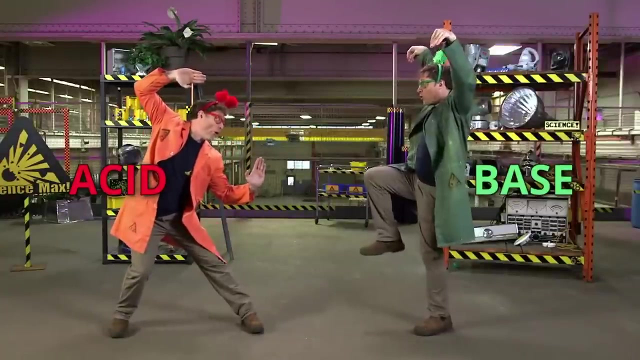 Yeah, well, that's okay, I get them both in bulk. Come on, let's go put it together. I'm an acid and I'm a base and we are enemies. Well, we're not really enemies. Yeah, that's true. 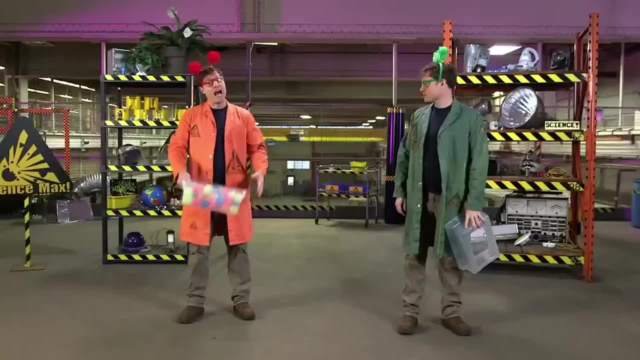 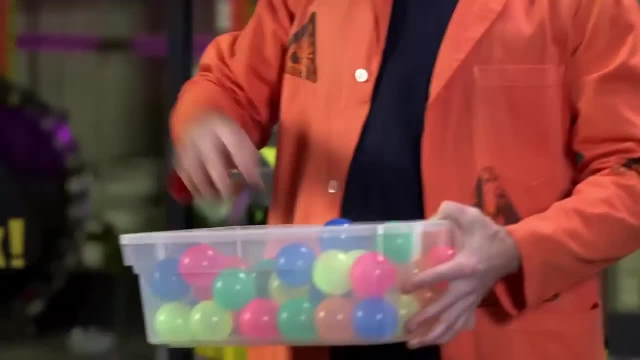 It's all about how we react chemically. You see, As an acid, I really want to give protons away Protons. Who needs your protons? Get your protons here. Protons- I got more than I want. 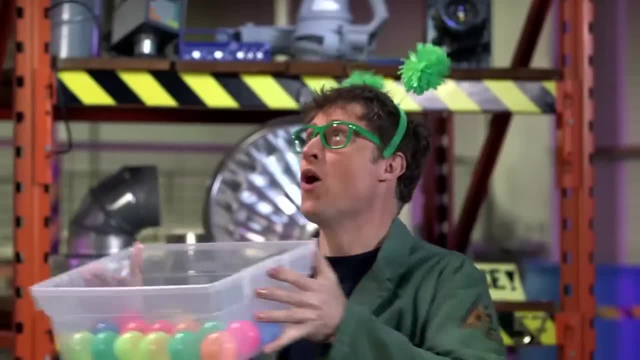 I don't need them anymore. And bases: we need protons. We'll do anything to get them. Protons: are you giving protons away? I'll take some. I'll take some protons. You'd think that when you get these two together, 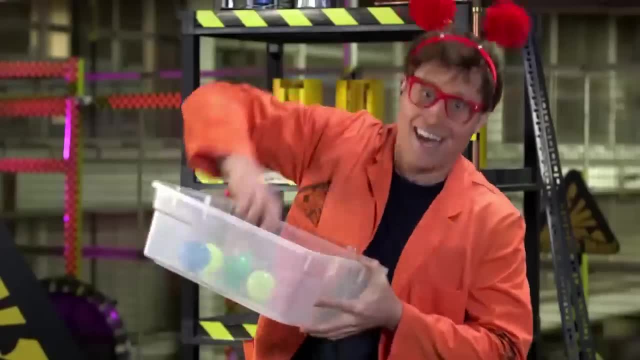 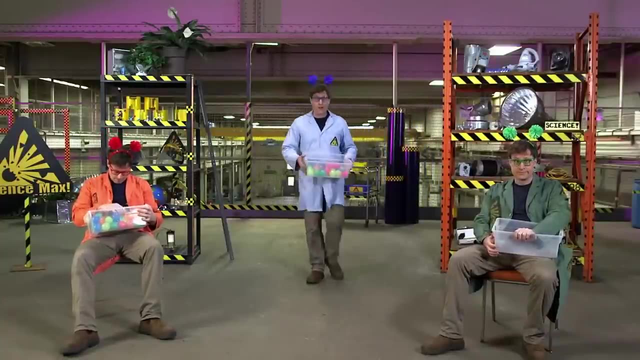 you'd have some pretty great chemistry, But the truth is, when they're together, they often don't react. Whoa, That is until water gets involved. Once you have water, acids and bases react. Here, take some protons. 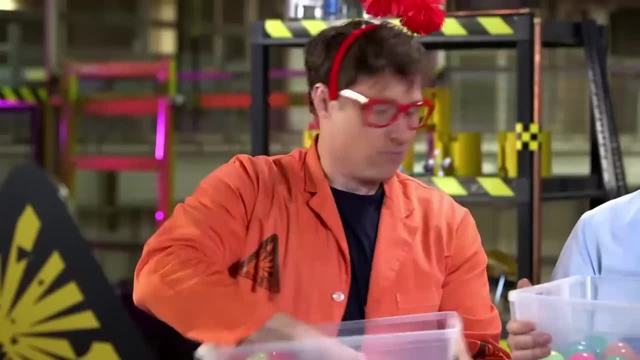 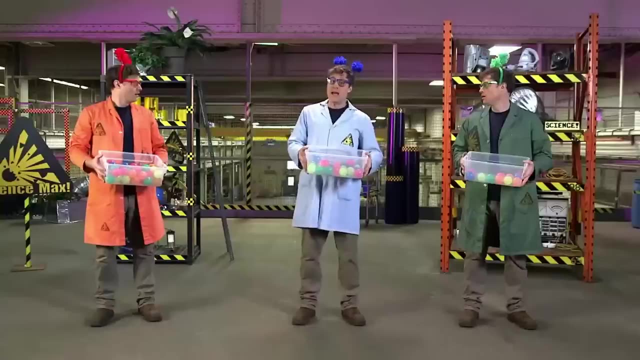 All your bases belong to us. Take some protons. I don't need them More. I want more. I want more protons. Water is a solvent allowing the chemical reactions to take place, Depending on the strength of the acids and bases. 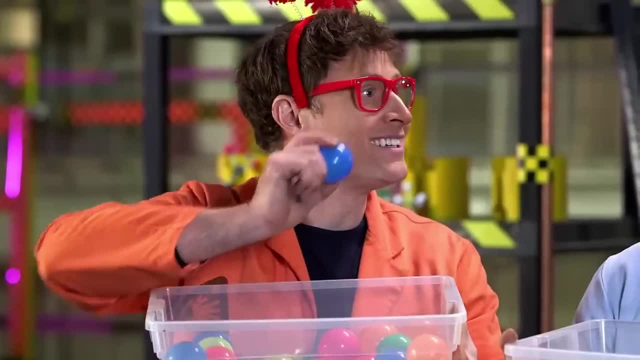 that reaction can be mild. Would you like a proton? Oh no, really, I couldn't Please, please take it. Oh well, thank you, That's very generous. Have another? No, perhaps, maybe I will. 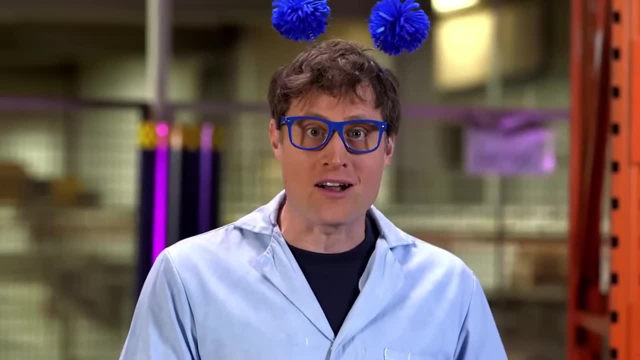 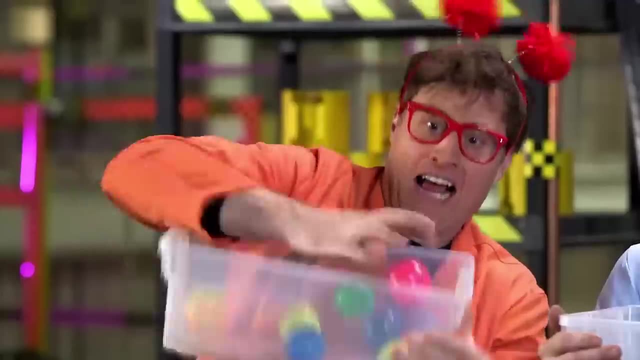 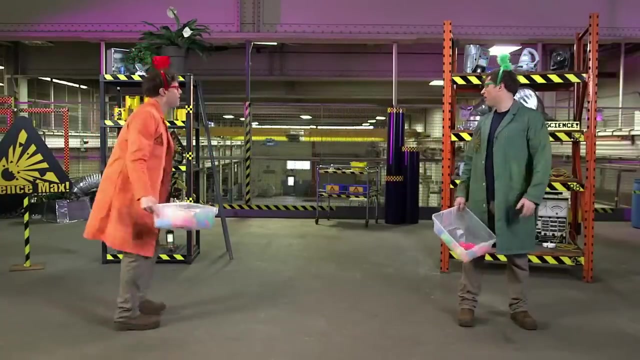 Here's one, Maybe just one. But if the acids and bases are strong, the chemical reaction can be really extreme. This is what's going on in the antacid tablet And why, without water, nothing happens. Oh, water, Water. 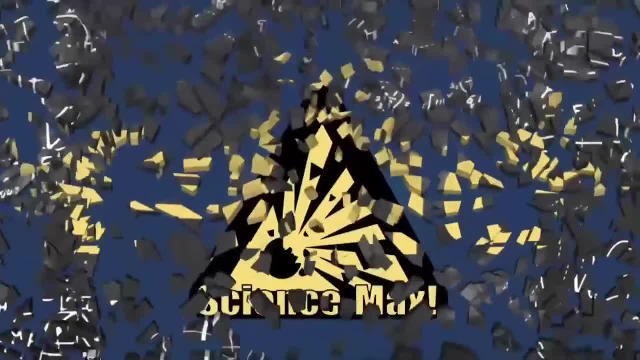 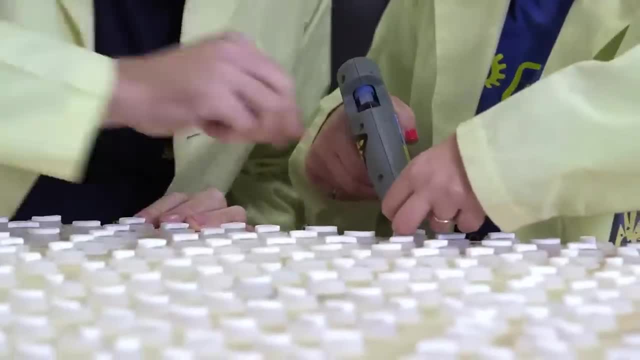 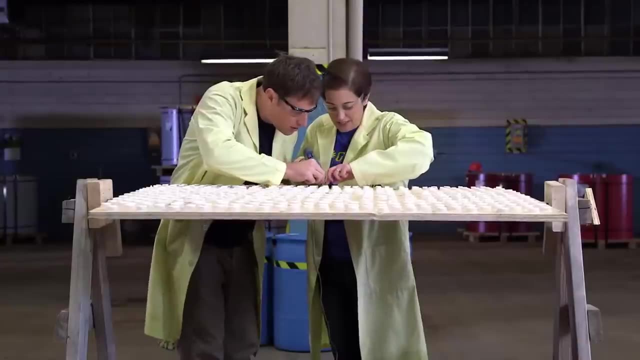 Come on, What'd you do? And that's the last one. Lisa and I are maxing out our chemical-powered rocket, not by making it bigger, but by making more of them. How many more? 400 caps all glued down. 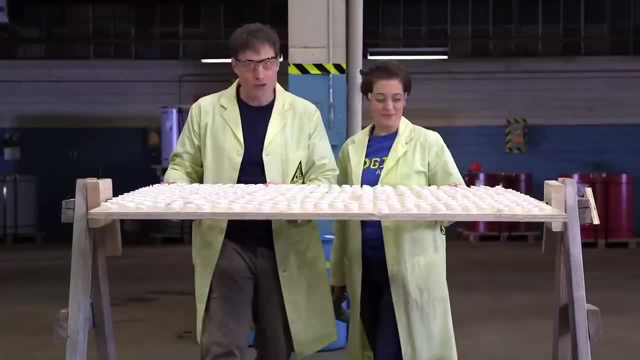 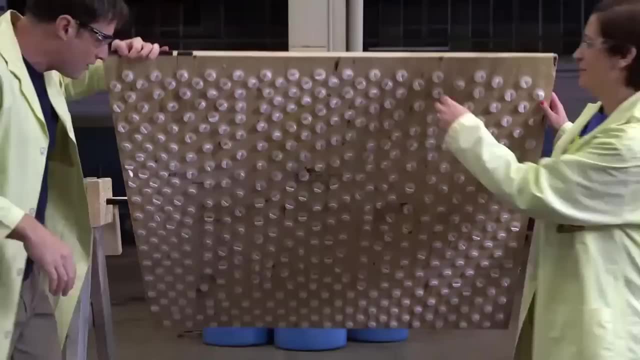 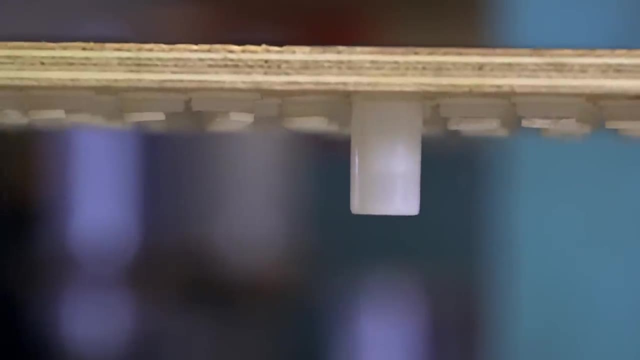 400 antacid tablets, or part of all, glued down. and they're glued on this fancy-pantsy spinning surface. So we rotate this part upside down, We fill each container with a little water and snap it on underneath. This way, the antacid tablet and the water don't mix. 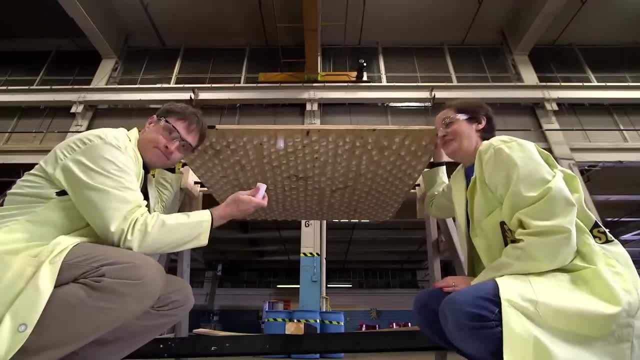 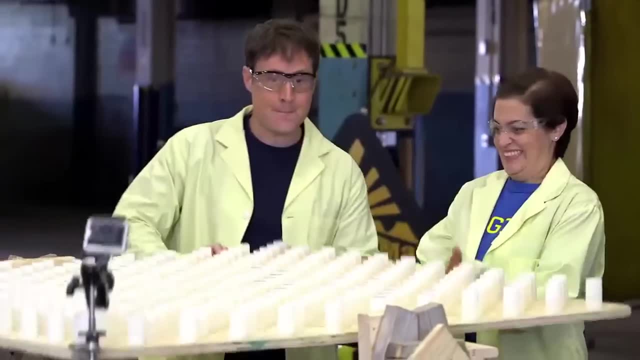 until we flip it back over. It also allows us time to snap it on and put them all on. Okay, ready, Ready, All right, 400 containers, Here we go, Let's do it. Whoa, Once we flip the board back over. 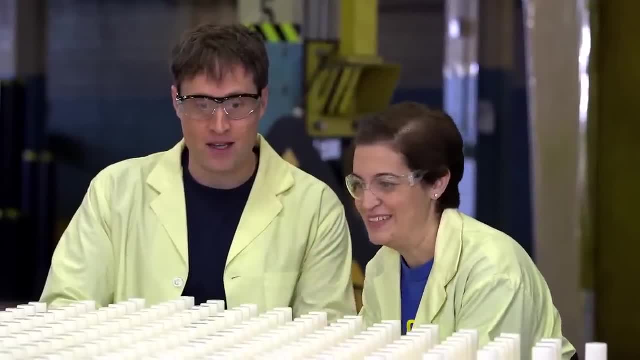 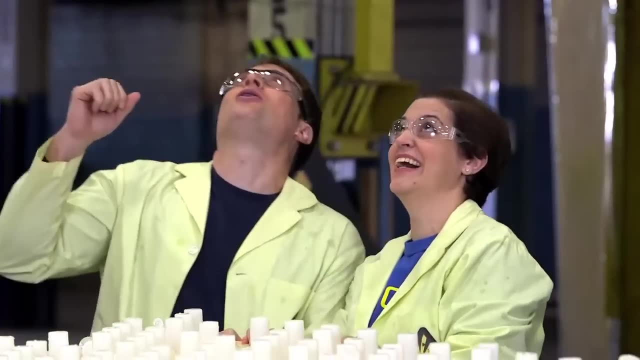 the reaction started taking place, building up carbon dioxide gas and increasing the pressure until Oh, Whoa, Oh Whoa, Oh yeah, Oh yeah, Oh my goodness. Ah, Good job Lisa, Good job Lisa. 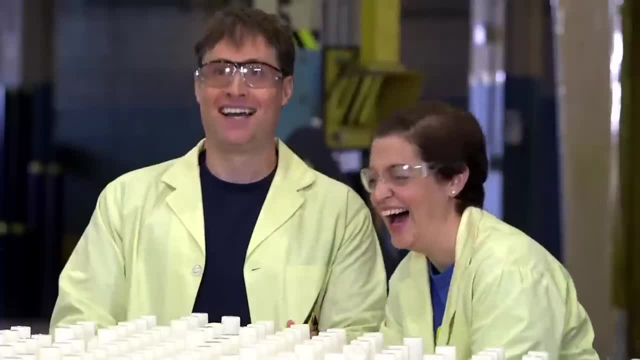 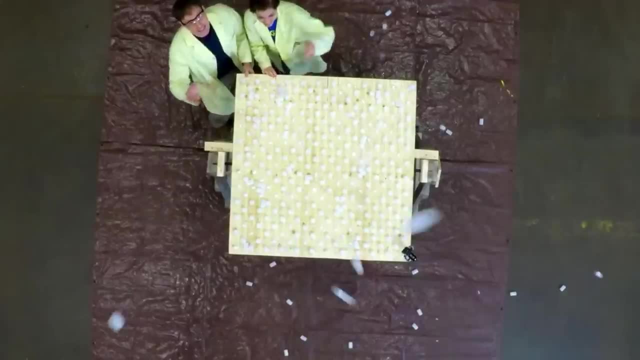 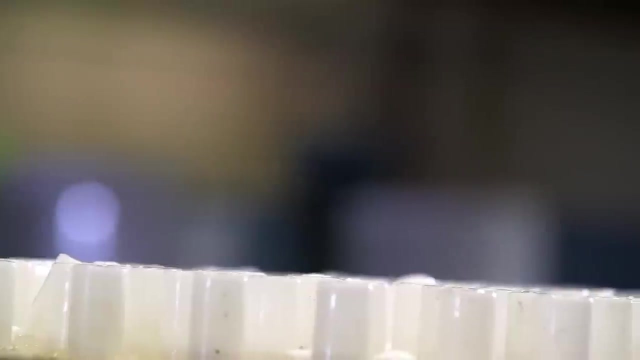 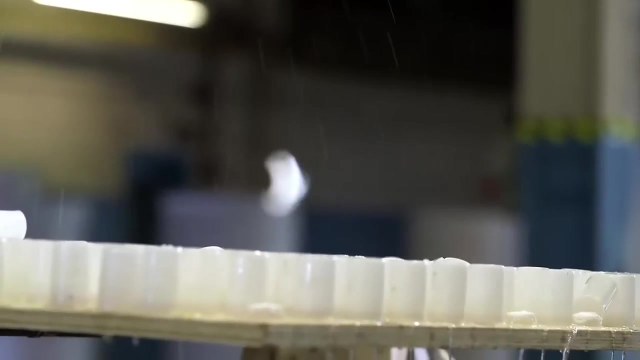 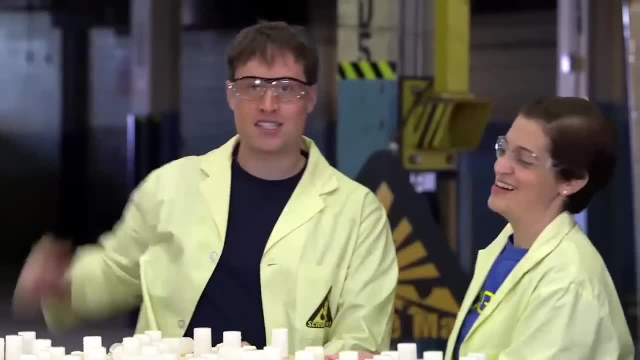 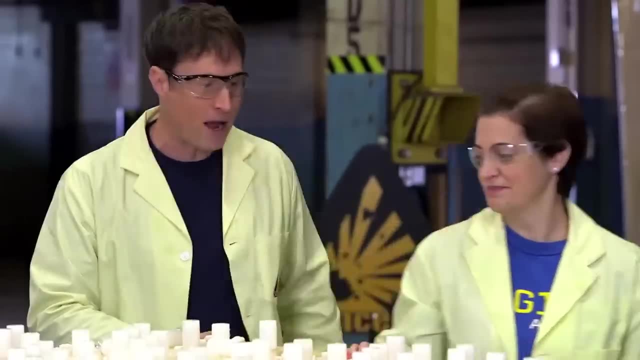 Wow, Okay, so high fives on that. Yep, That worked spectacularly. That was awesome. So we've done this. Let's go bigger. Let's go bigger, OK. So let's go, and we'll clean this up afterwards. 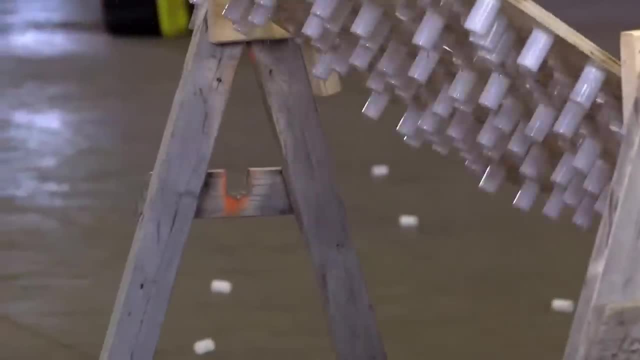 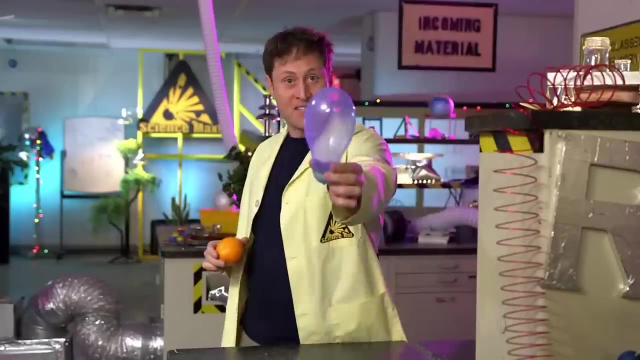 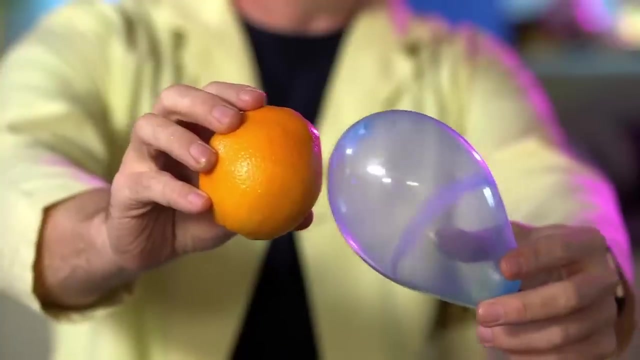 OK, Let's do it. OK, let it go. Whoa, Whoo, Whoa. This is a balloon and this is an orange. When you put them together, a chemical reaction happens. I had you going there for a minute, didn't I? 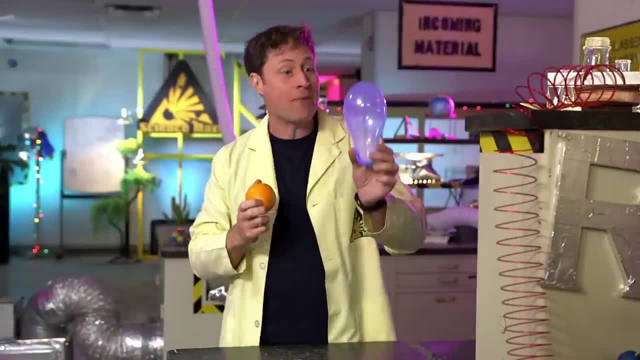 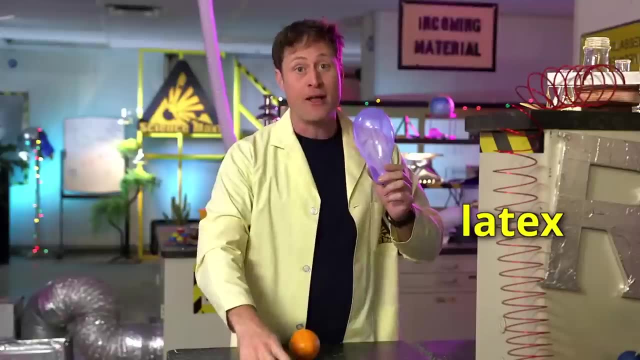 No, No, All right. Well, you can actually do a chemical reaction between a balloon and an orange. You see, balloons are made of latex, which is a kind of polymer that's very, very stretchy, And orange peels contain a chemical called limonene. 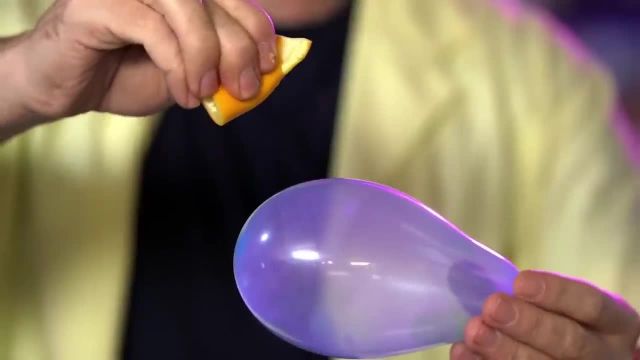 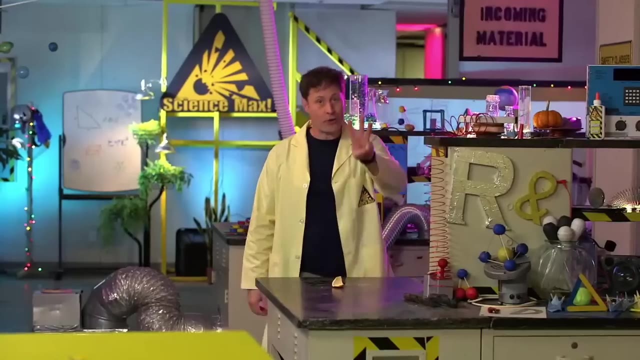 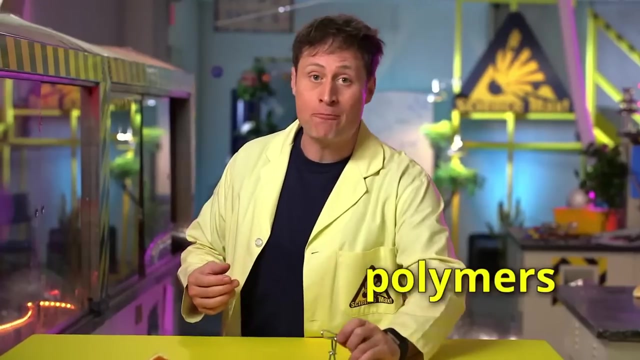 Limonene breaks down latex. So we have three questions. The first is: why does this happen? Well, like I said, it's all chemistry. You see, balloons are made of polymers, chains of molecules held together by chemical bonds. 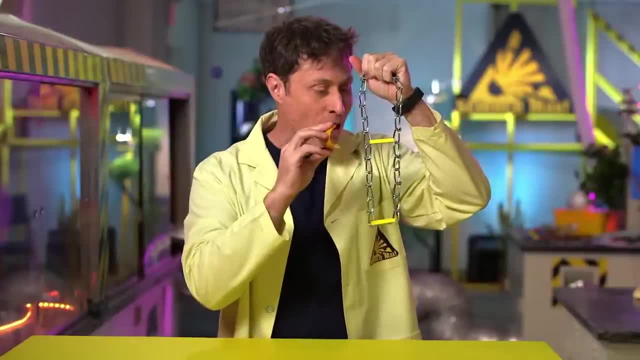 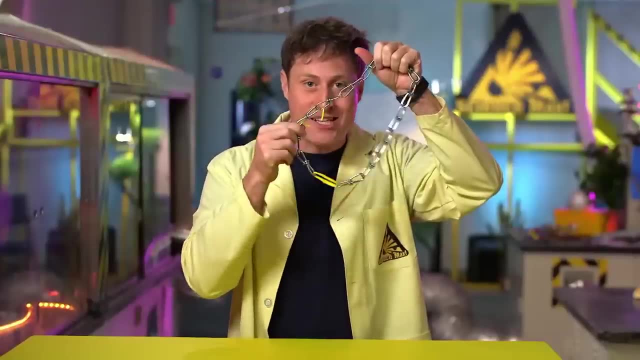 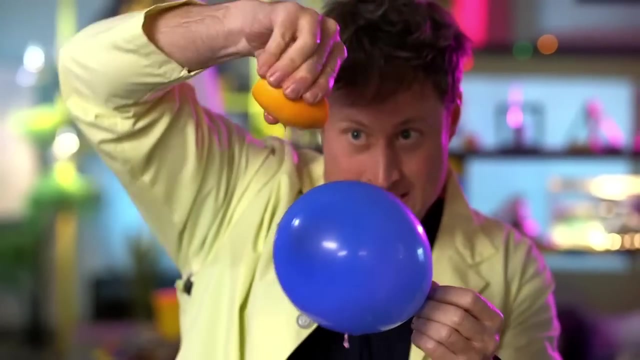 A limonene molecule attacks those bonds- Om nom nom nom, Om nom nom, Om nom nom nom, Om nom nom, Delicious- And breaks it. That separates the polymers and that pops the balloon. But remember, it only works with natural latex. 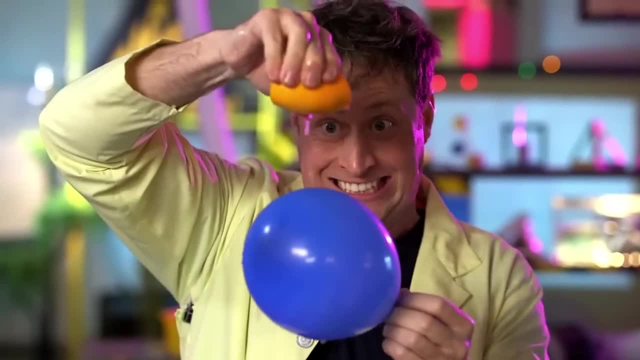 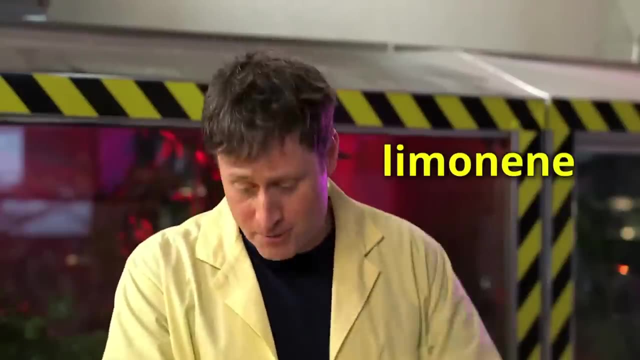 So make sure you're using natural latex balloons. Second question: Why do they call it limonene when it's in orange peels? I mean, yes, it's in lime peels And lemon peels, But the chemical itself smells like oranges. 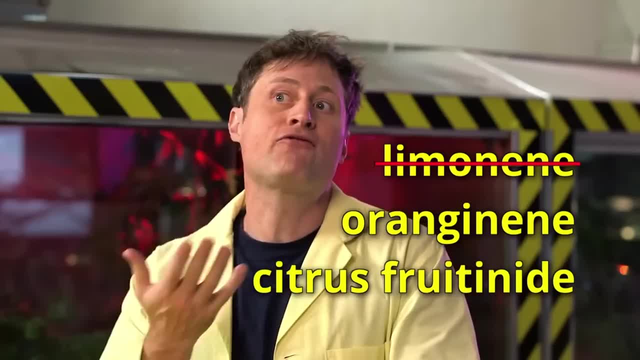 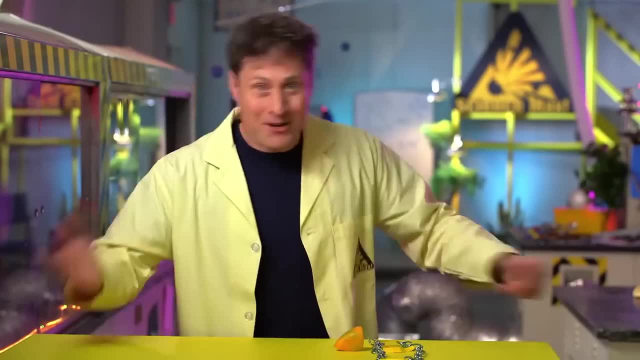 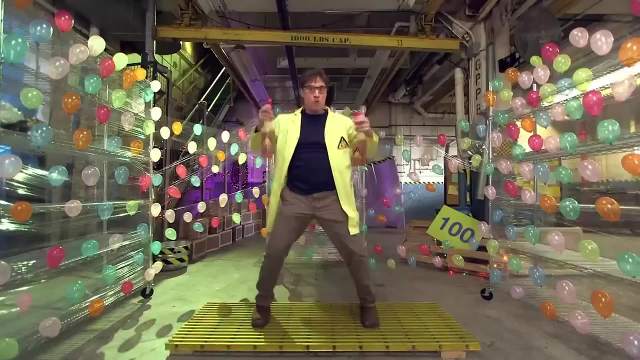 They should call it orangenine Or citrus frutenide Oranyway. Third question: Should we max it out? Of course we should Come on. 200 balloons versus two bottles of limonene Ready Go. 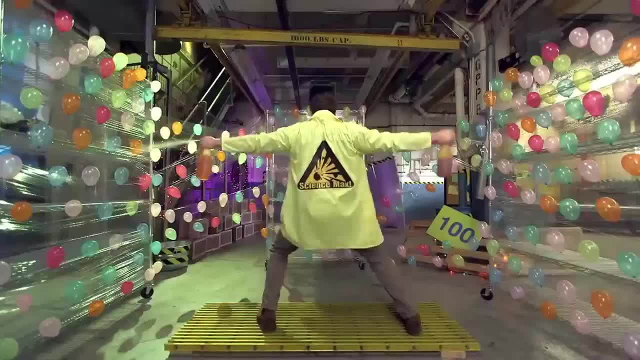 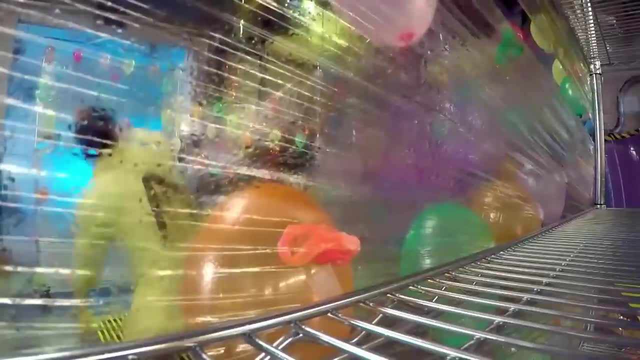 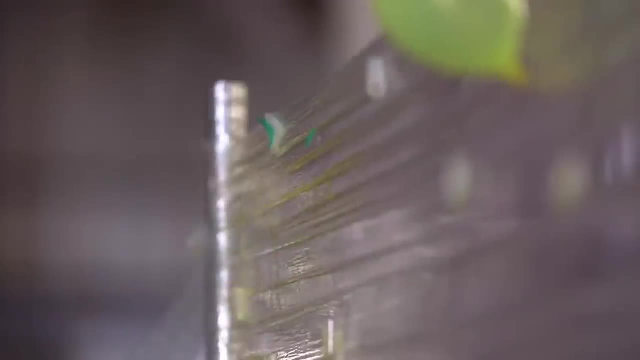 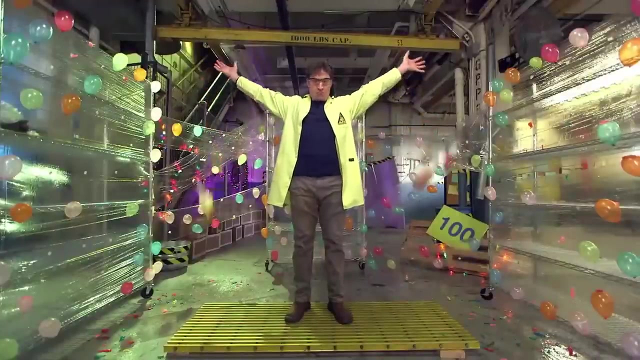 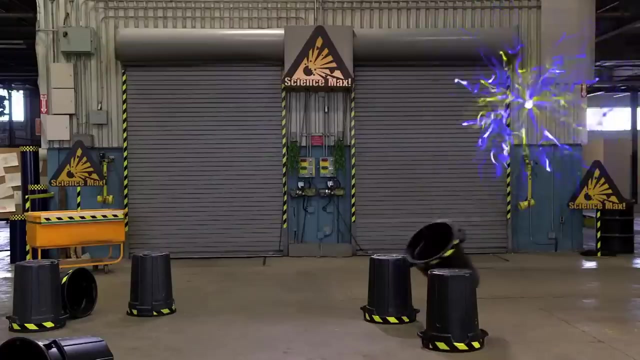 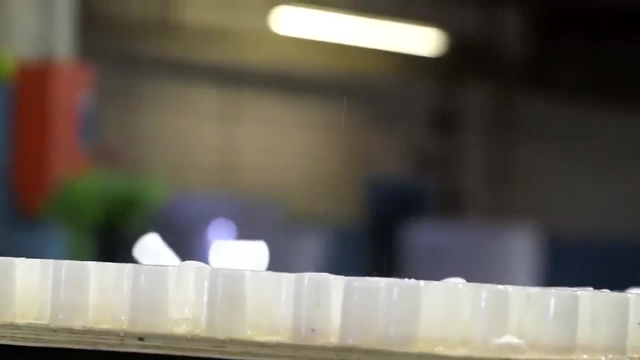 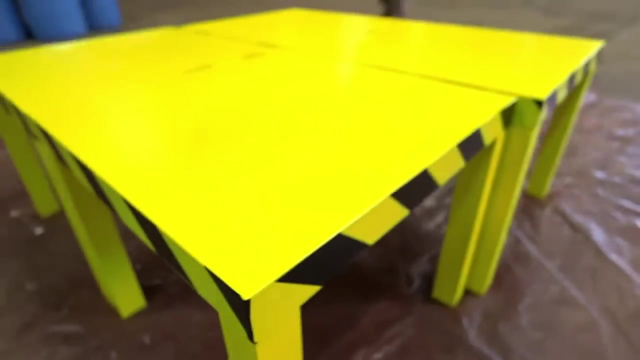 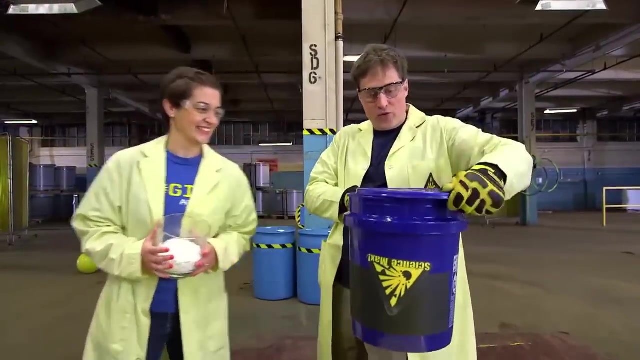 Science. Our first attempt to max out our chemical rocket was 400 plastic containers. Oh yeah, That worked well, but now it's time to make the container larger. Whoa Giant, maxed out chemistry rocket canister. I have a big plastic container with a groovy lid that sits there on airtight, which is great. 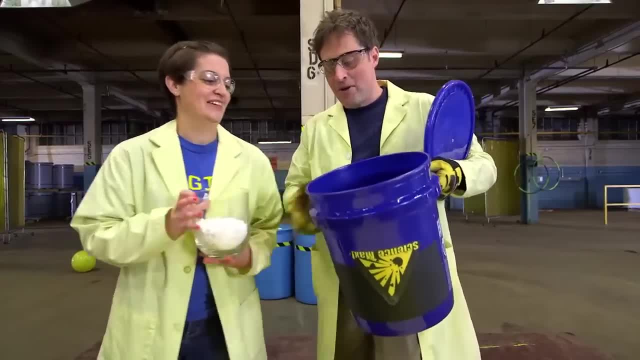 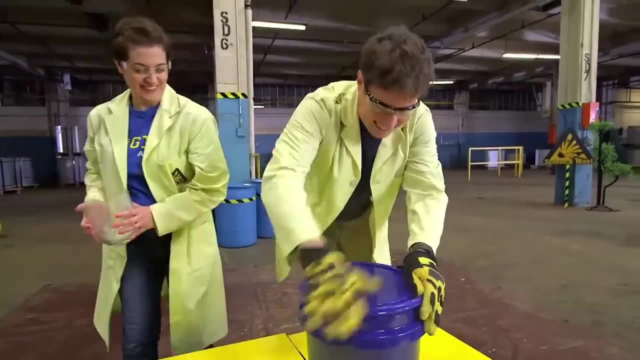 And I have a giant jar of antacid. How many was it? Like 60 antacid tablets or something At least. This works exactly the same as our smaller containers. We dump the antacid in, seal the lid airtight, then flip it over. 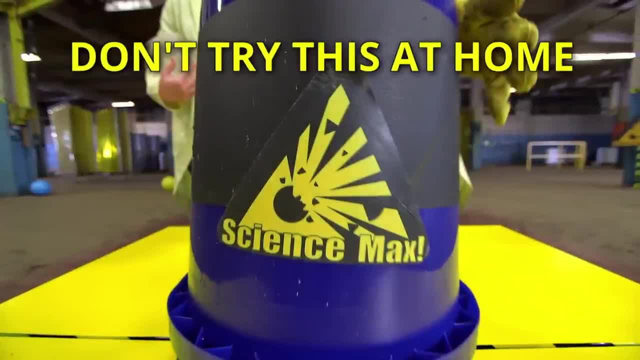 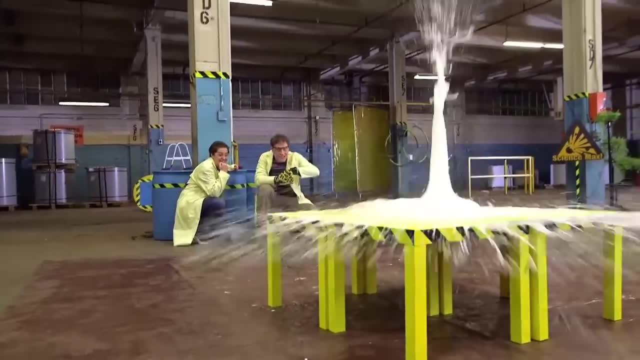 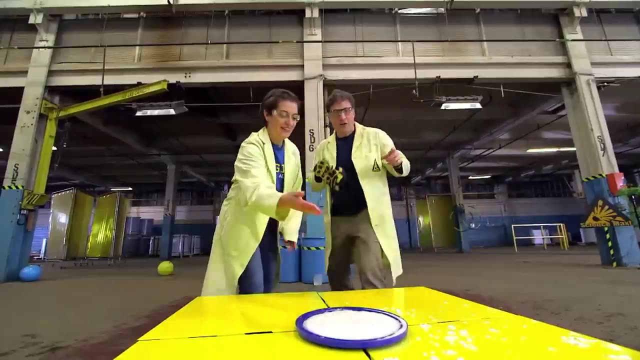 And now would be a good time to mention not to try this at home. Okay, Oh, it's not gonna take long. Oh my God, Oh, Oh, Oh, Oh, Oh, Oh, Oh. All right, So that was the canister version. 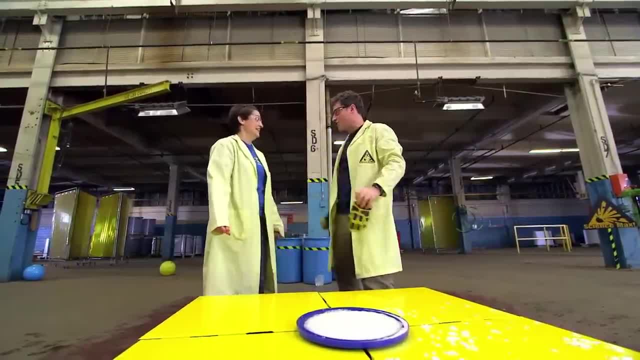 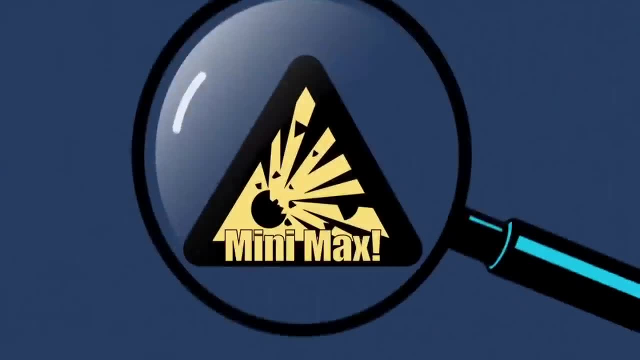 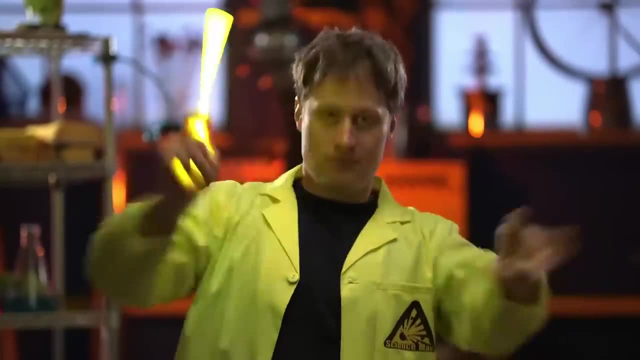 Now we need the popper, Now we need the pop bottle version, the rocket version. Yes, Okay, Let's go make that, Let's do it, Okay. Mini Max, This is a light stick. It creates light using a chemical reaction. 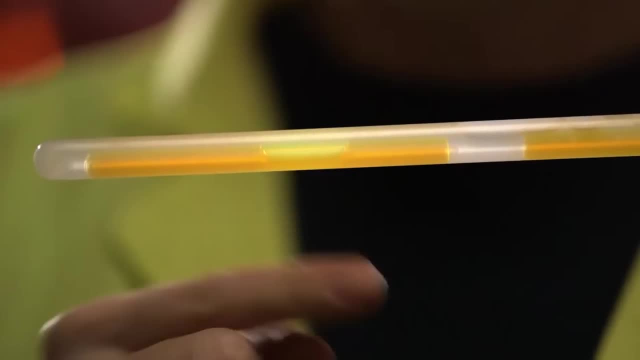 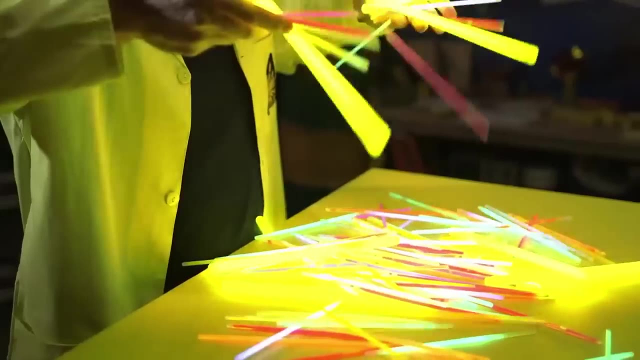 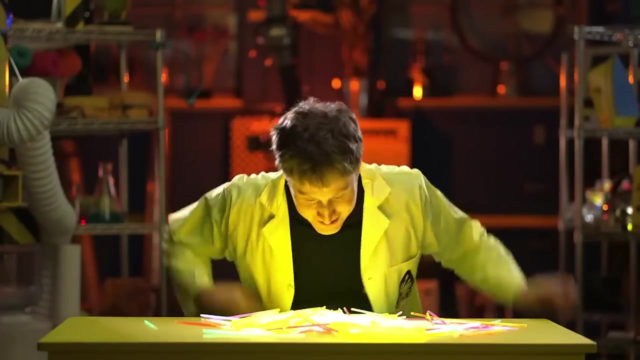 There's a liquid chemical inside and also a glass container that holds another chemical. When you bend the light stick, you break open the container and the two chemicals mix, creating light. There you go: Light sticks, Chemical reaction And yes, of course we're gonna max it out. 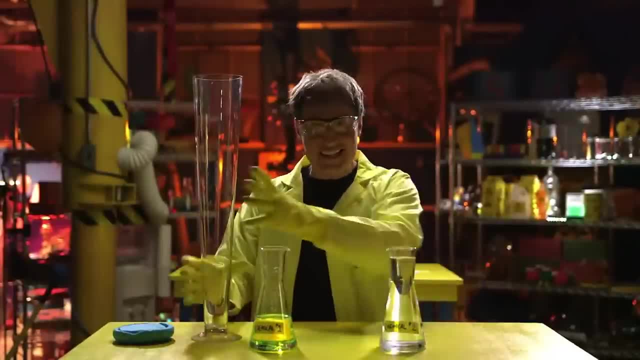 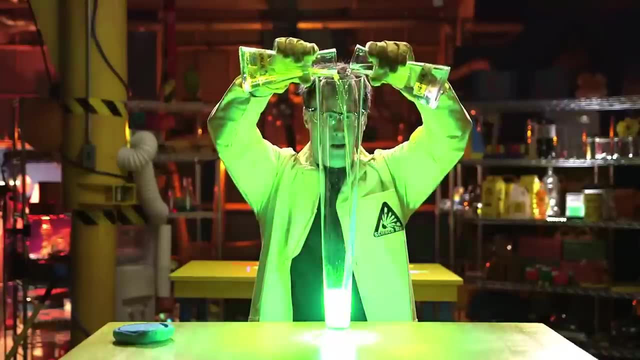 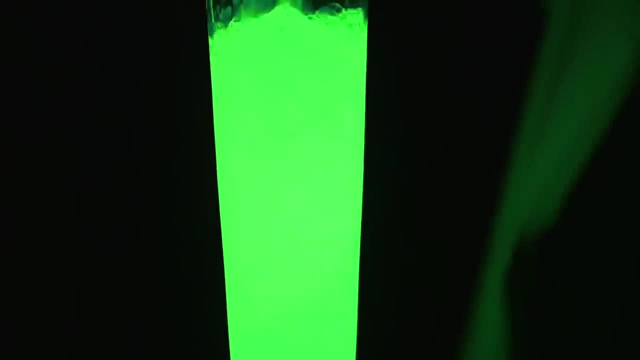 This is a whole bunch of the two chemicals and a light stick. Let's max it out. So how does a chemical reaction produce light? Well, a lot of chemical reactions produce energy. You might think of a chemical reaction producing heat. Well, heat is a kind of energy. 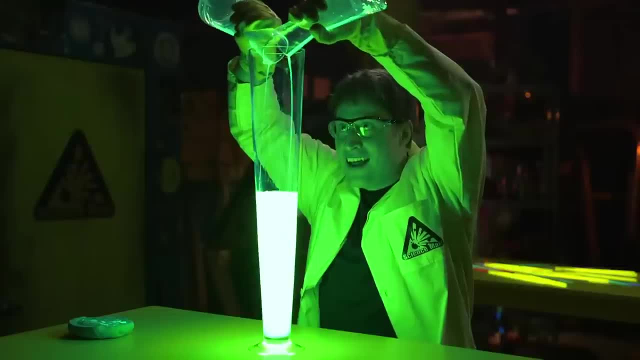 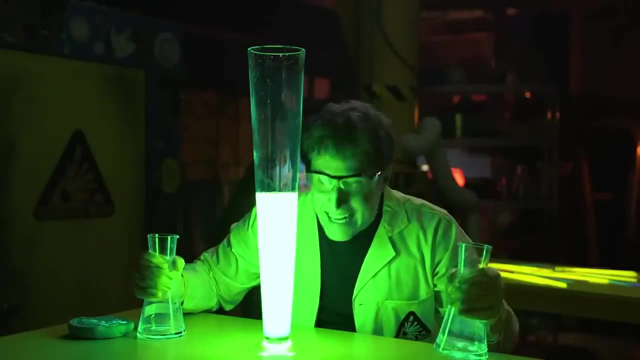 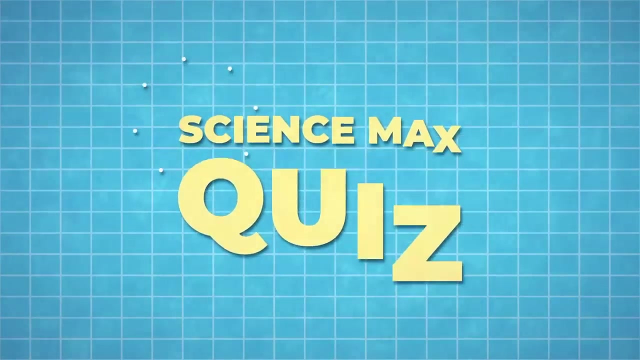 This chemical reaction produces energy. This chemical reaction also produces energy, just energy in the form of light. It's just a different kind of energy. Whoa maxed out light stick. And now for a Science Max quiz: Chemical change or not? 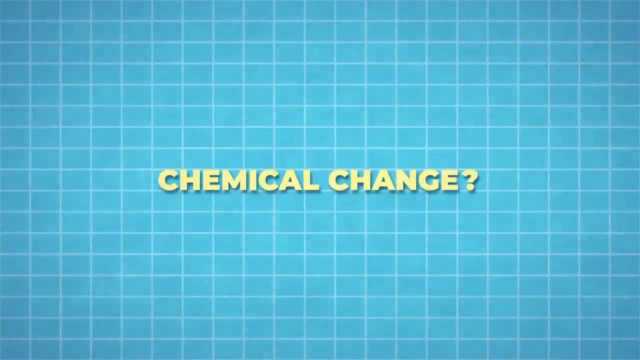 What's a chemical change? Well, let's demonstrate. Look at this: It's a happy little molecule of iron, And here's another molecule of oxygen. If they were to have a chemical change, they would react and form different molecules. Look, it's a molecule of rust. 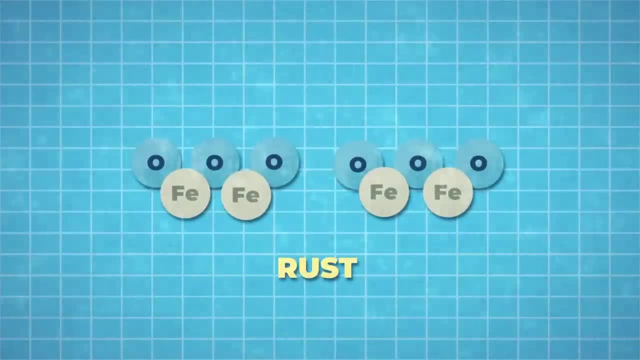 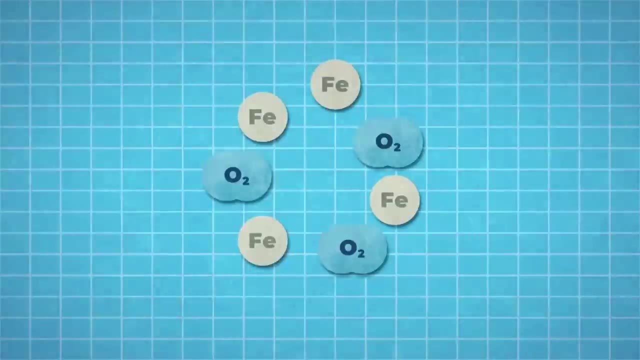 Rust is a different chemical than either iron or oxygen. It's a chemical change. Now, if these molecules mixed and did not change, then it's not a chemical change, It's a physical change. Sometimes it's hard to tell if it's a chemical change just by looking, but asking what kind? 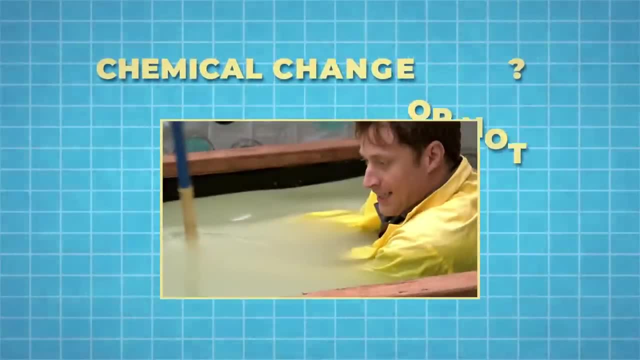 of change it is leads to good science. So let's look at some examples: Vinegar and baking soda: Is it a chemical change? Yes, Vinegar and baking soda react to form different chemicals: Sodium acetate, that's the white stuff that's left over, and carbon dioxide, which makes 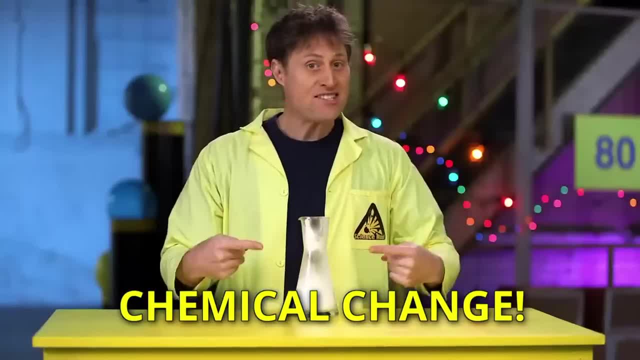 the bubbles. How about a nucleation fountain with diet cola and mints? Ha ha, A lot of people think that's a chemical change, but it's not. The mints cause carbonation, the bubbles to escape faster, But in the end you still have cola and mints. no new chemicals. 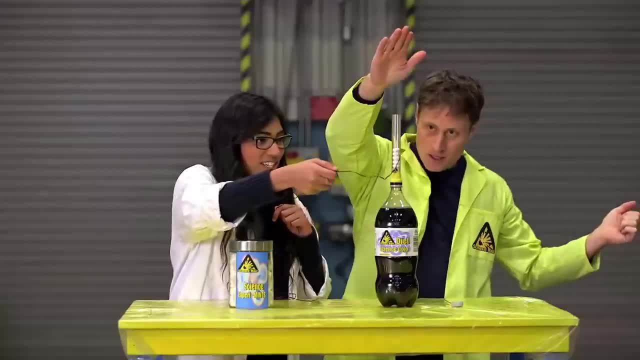 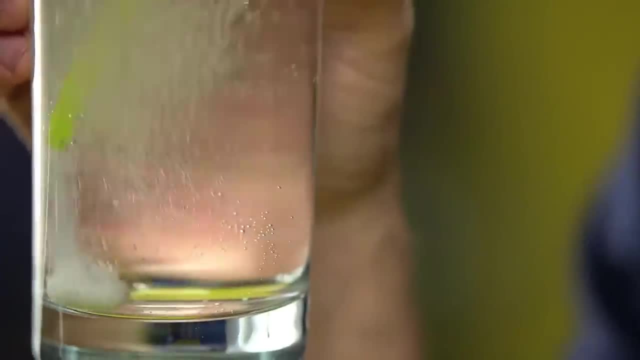 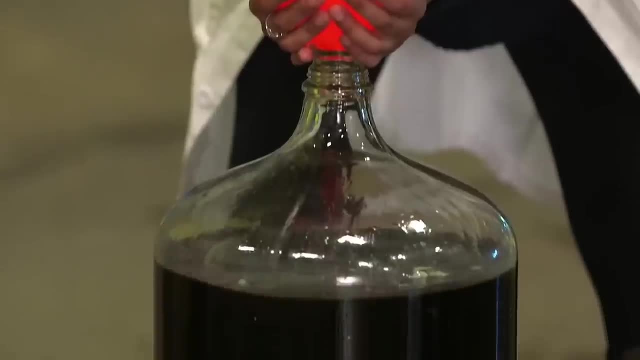 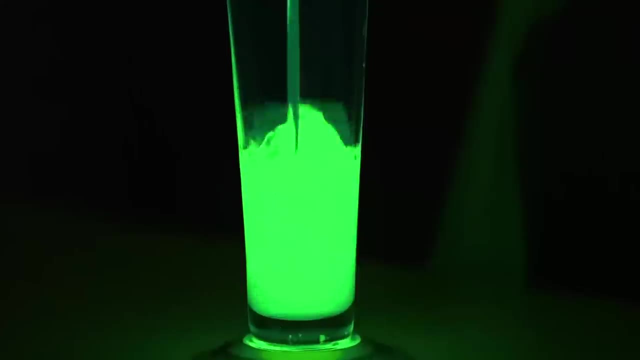 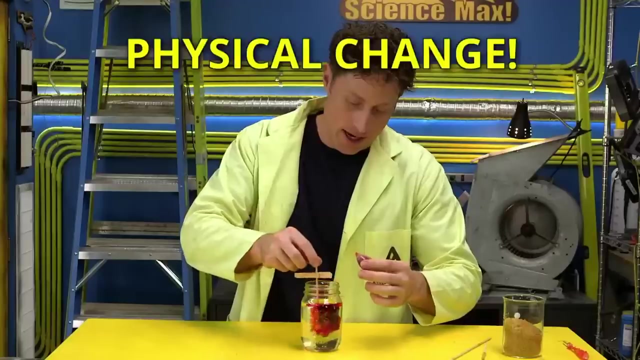 Glow stick chemicals. Well, producing light or heat is usually a sign of a chemical change. How about mixing sugar and water to make a sugar pop? That's a physical change. You start with sugar and water, you mix them and when you have a sugar pop, what chemicals? 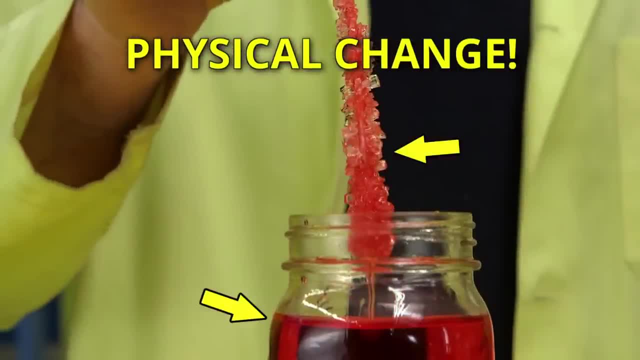 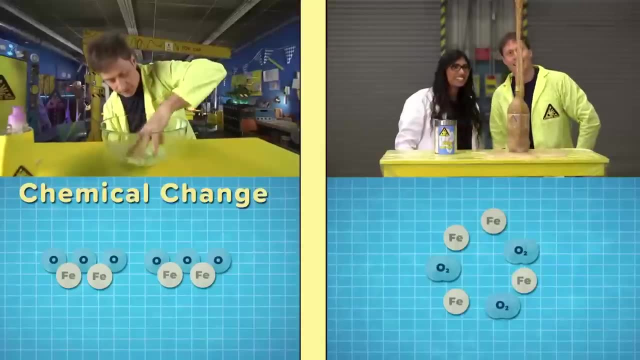 are you left with? Well, sugar and water. so no chemical change. It can be hard to tell sometimes, but whenever two things mix, think to yourself if it's a chemical change or a physical change. and now you know it's either one or the other. 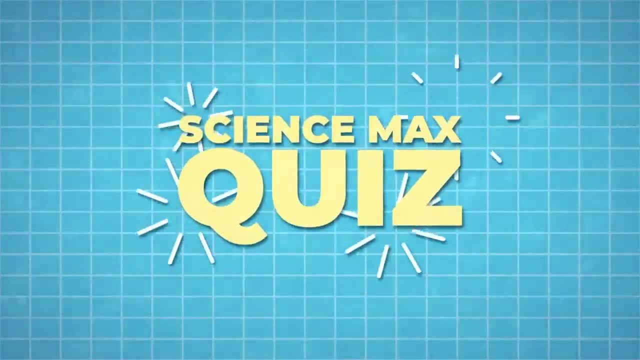 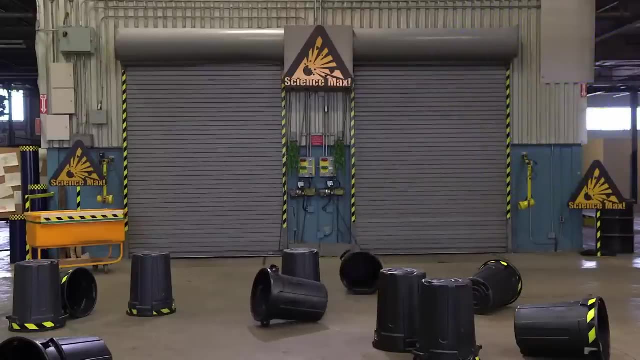 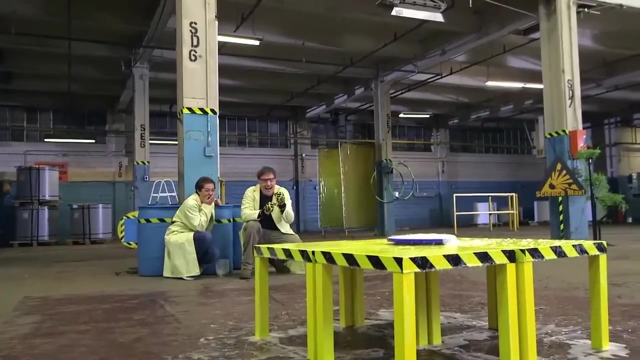 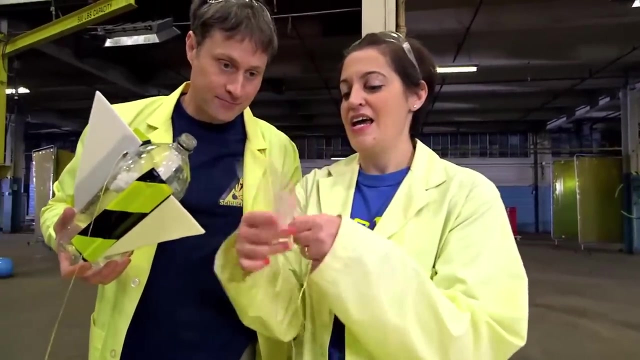 and that's the first step to good science. Thanks for playing our Science Max quiz. Our maxed out rocket worked great Now to make it look more like a rocket, So we have a mesh bag here to put the antacid in Right. 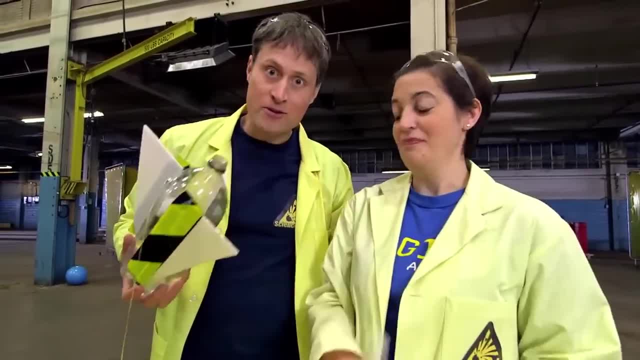 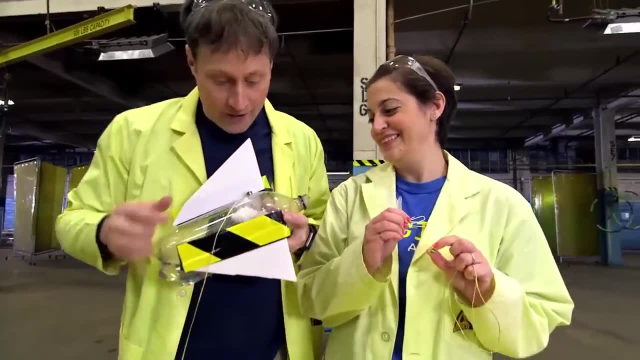 And we have some paper clips attached to it. And what are the paper clips for? Well, Phil, we have a magnet, Ah, And so the magnet sticks to the paper clip, And so that's what we have here. You see, the bag is full of the antacid tablets which. 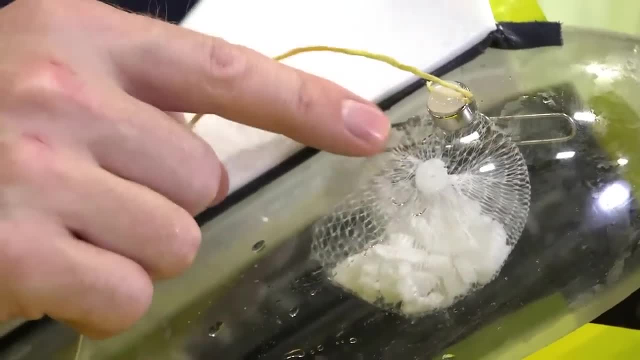 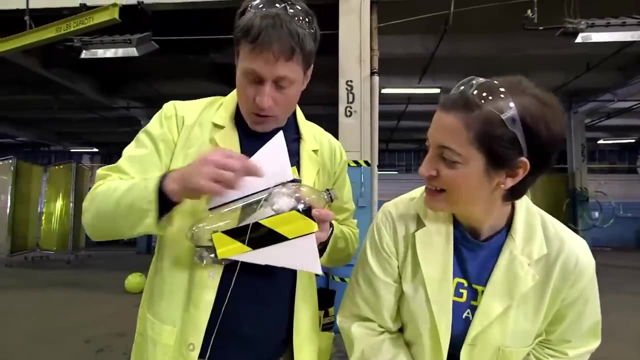 we put through the mouth of the bottle, and the magnet is holding the paper clips on the other side of the plastic so we can sort of move it along, So we can start With the bag over here where the water's down there. 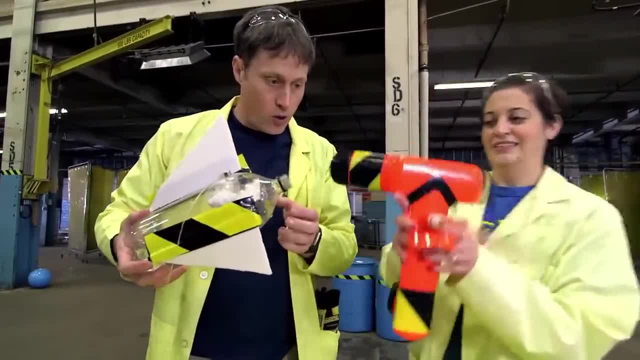 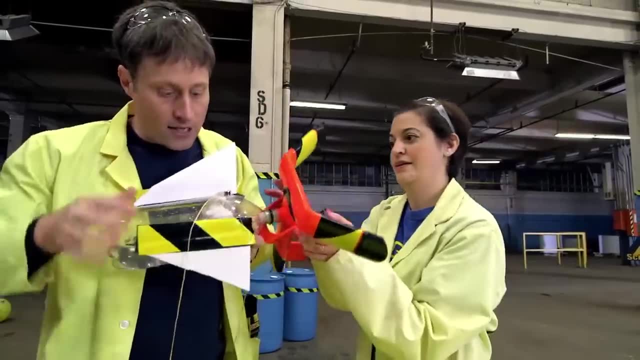 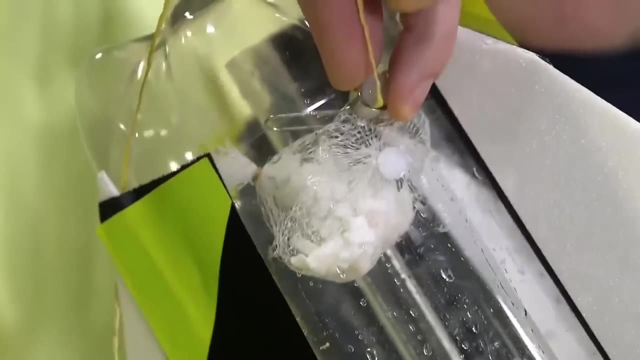 But now we attach the launcher, like. so. All this effort is to keep the reaction from happening until the bottle's on the launcher and we're ready to go. And then, as we pull the bottle over, we bring the bag up this side, And there the water and the antacid have never touched. 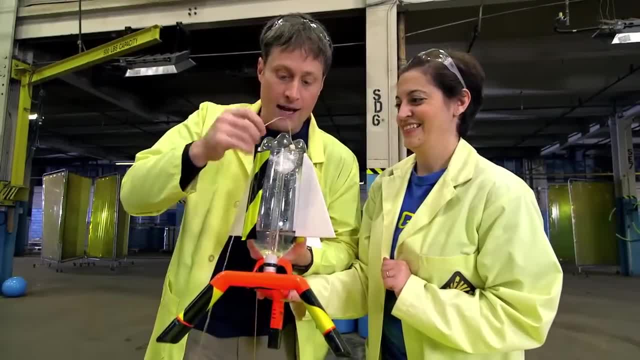 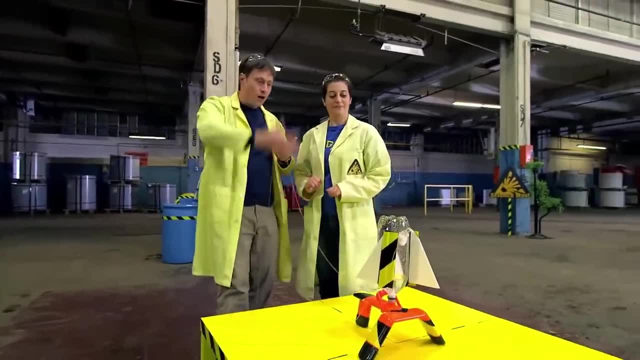 No reaction. All you need to do now is just we pull this magnet away and the bag will fall into the water, And then we will have the launcher down here And we pull the release and the rocket will go. We add some weight to the launcher. 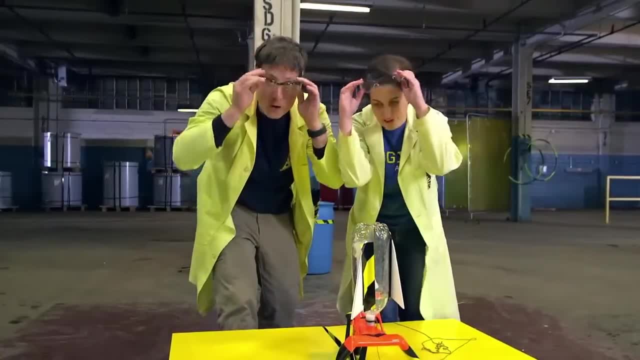 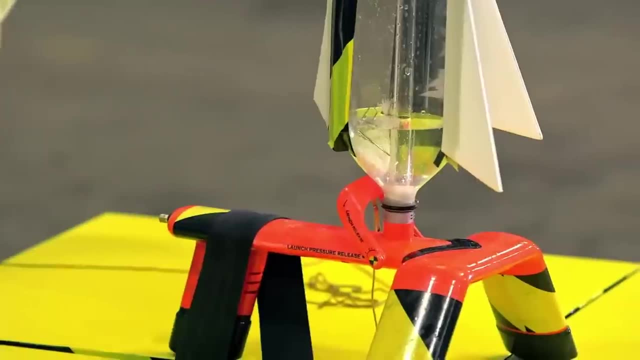 to help keep it in place. OK, right, wait, Glasses, Safety first. OK, ready. And then we pull the string with the magnet That drops the bag of antacid tablets in the water and starts the chemical reaction, Because we have a latch holding the bottle down. 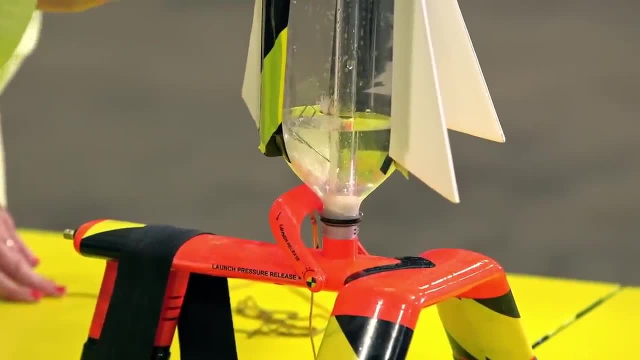 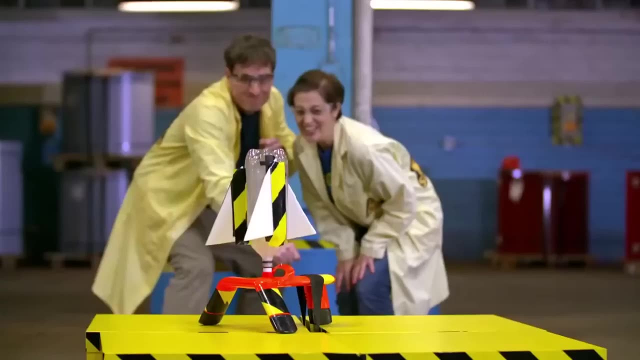 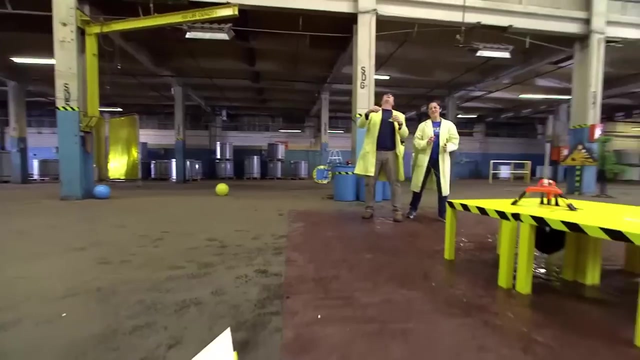 we can wait until the chemical reaction happens fully And there's a lot of gas pressure in the rocket before Three, two, one run Woo. Oh, that worked. Yeah, I hit the ceiling. I think we need to do this outside. 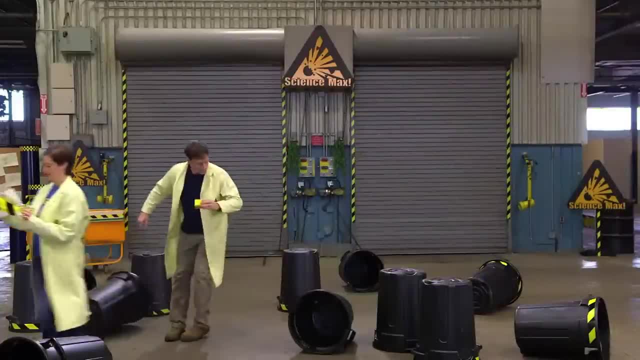 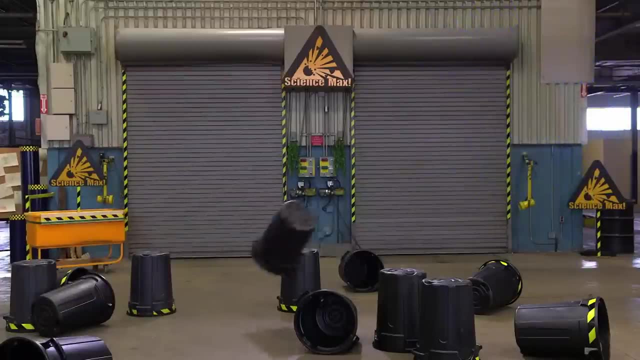 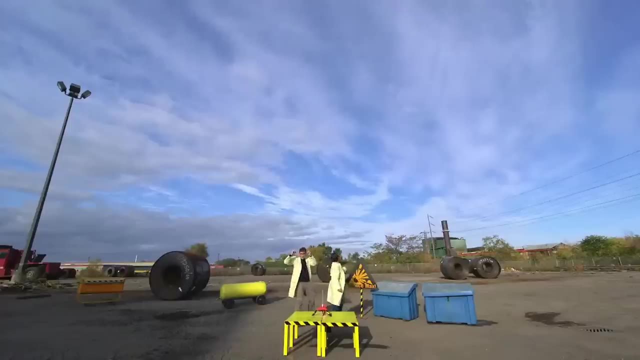 Yeah, I think we definitely have to do it outside. All right, totally great, Weird. Anyway, I was saying we should put three or four of them. Three, two, one, go, Woo Woo. There it is, Oh my gosh. 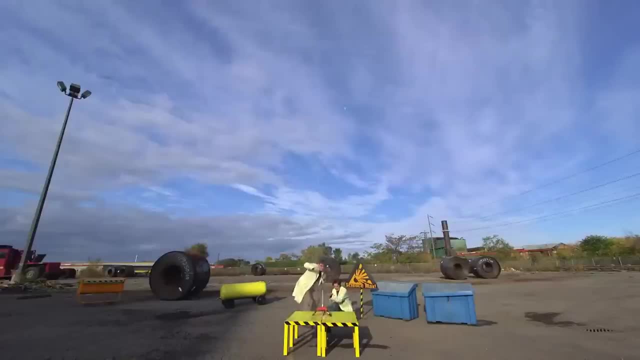 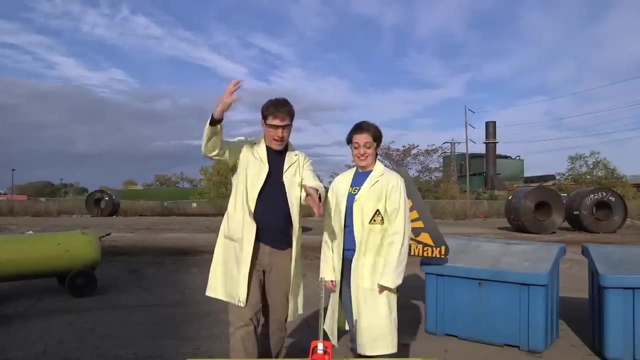 Yeah, We tried it outside and it worked great. The only thing left was to max it out even more. So larger chamber, Yep, more antacid, More antacid, more air, more water, Absolutely Bigger rocket. OK, so you know what? 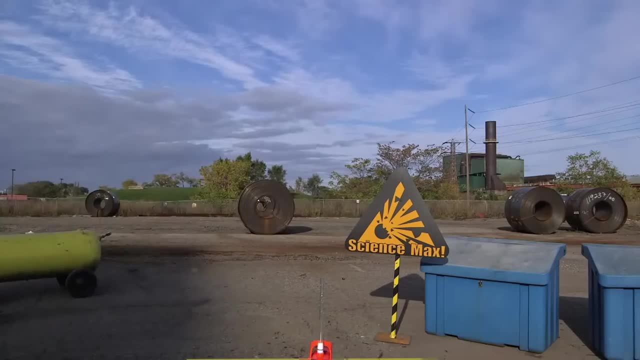 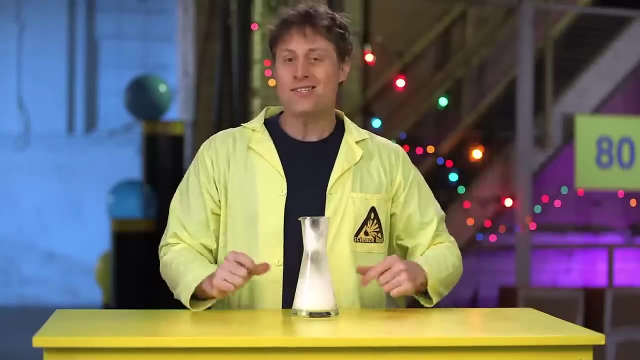 I know how to splice two bottles together. We can increase the size of the chamber. All right, This is sodium acetate. How do you get sodium acetate? How do you get sodium acetate? How do you get sodium acetate? 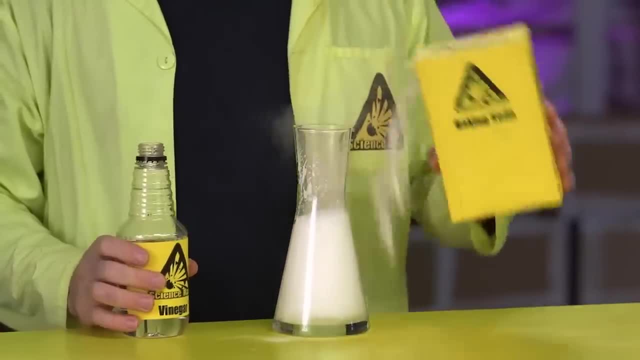 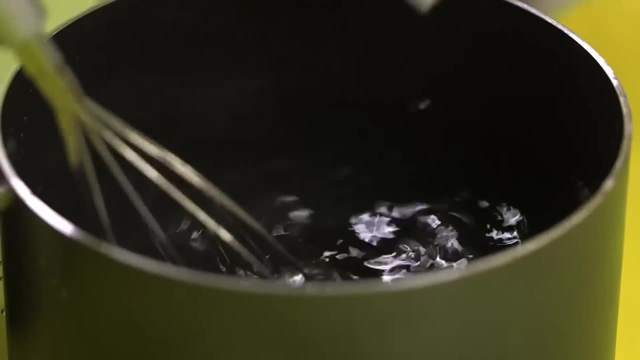 Well, when you do a vinegar and baking soda reaction, what you have left once the reaction is finished is sodium acetate. It's a crystal and you can do something fun with it. that may seem familiar. You make a supersaturated solution of sodium acetate. 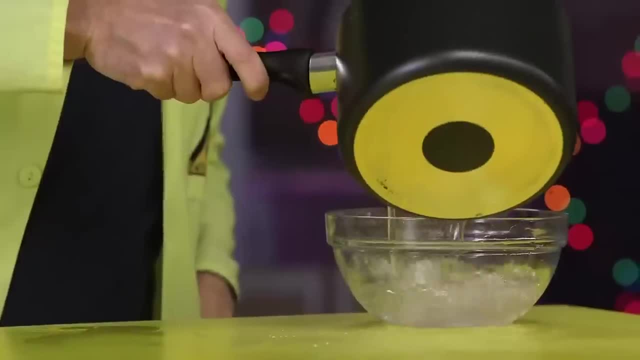 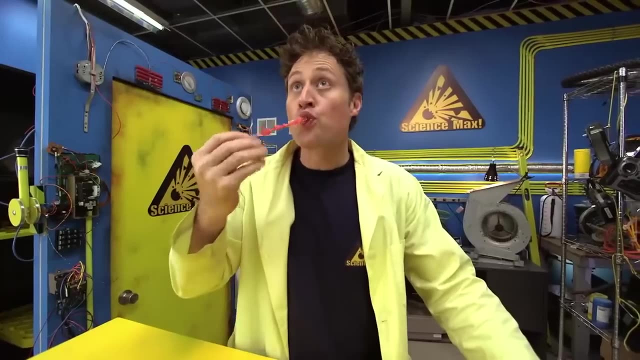 by heating water and dissolving as much as you can, And then, when it cools, you can get the crystals to reform. Now, if you did this with sugar, you could make a sugar pop, which we've done before. If you do it with salt, you could make a salt pop. 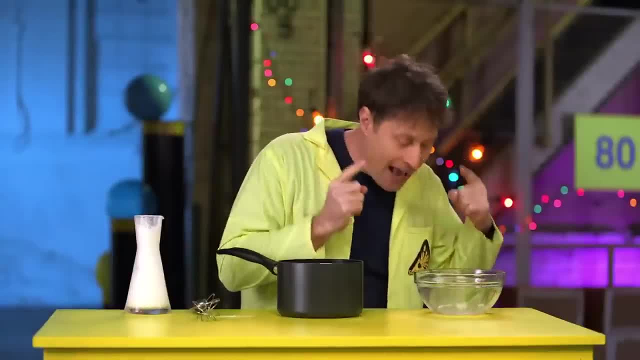 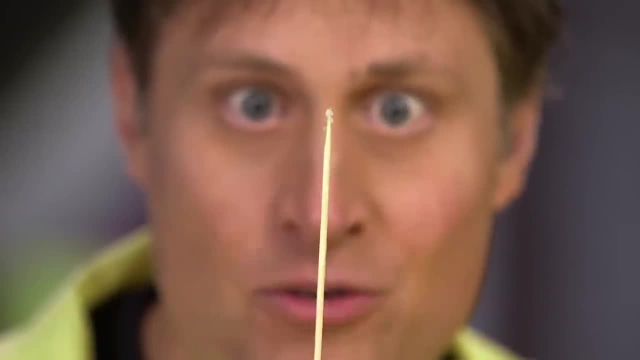 Which is less appealing. And if you do it with sodium acetate, you can do this Just like with the sugar pop. all it needs is a seed crystal to get the crystals to reform, But unlike sugar, which takes a few days. 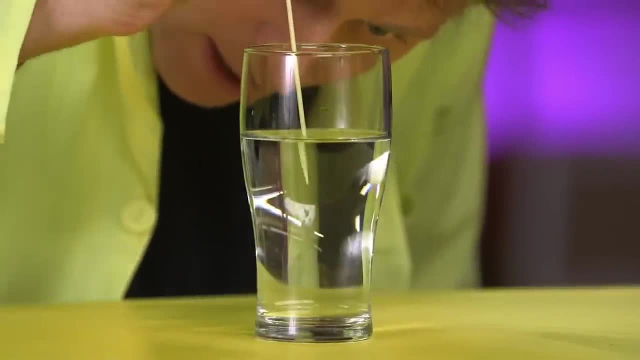 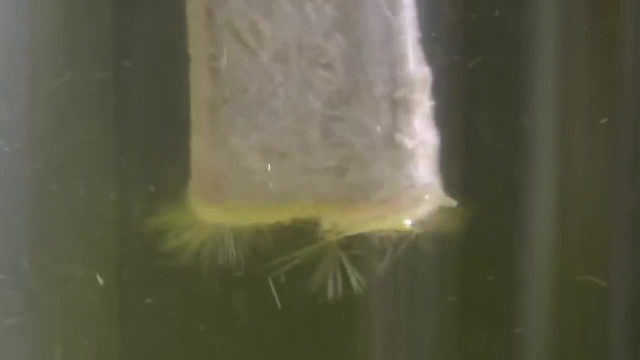 sodium acetate recrystallizes right before your eyes. Because we heated the water, it allowed more crystals to dissolve in it, Ooh- But then it cooled down afterward. There's more crystals sitting around in this water than there should be at this temperature. 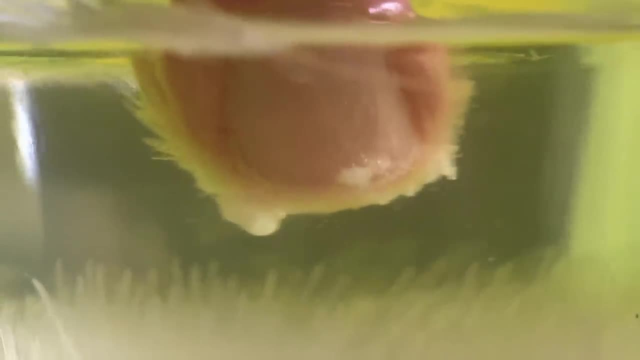 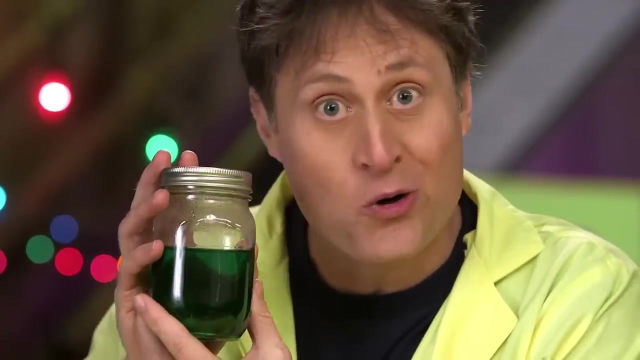 They want to turn back into crystals, and all they need is something to start them going. I've colored this one green because I don't know science. Maybe it'll look cool. A tiny crystal on the end of the stick is all we need to start the reaction happening. 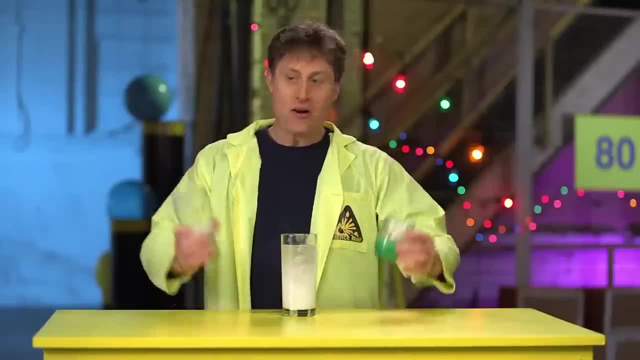 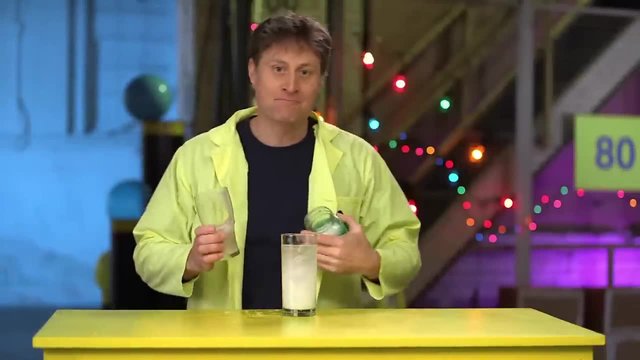 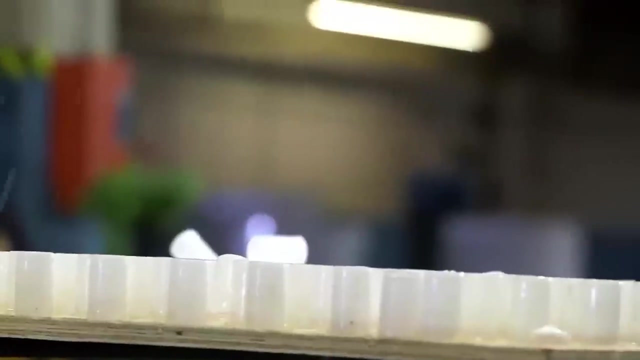 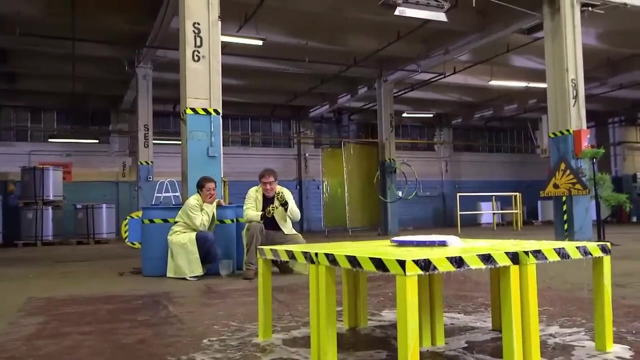 Whoa, Wow, And there you go, Sodium acetate. Hmm, That one wasn't done yet We've gone from small containers, Oh yeah, To a large container. Whoo, Whoo, Whoo, Ha, ha, ha ha. 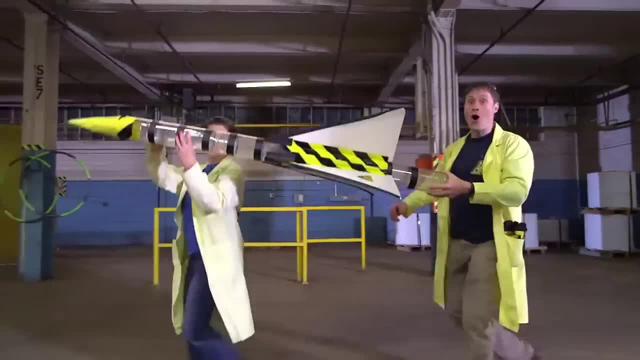 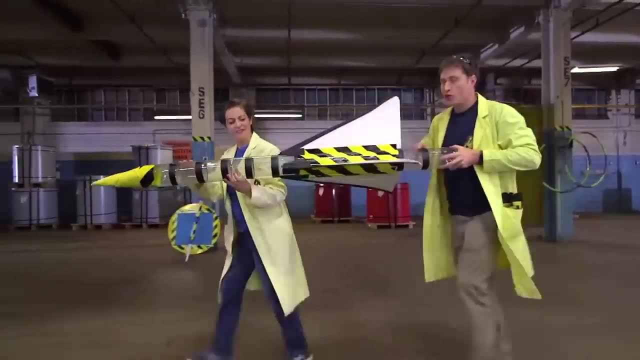 To a rocket Whoo Whoo. Yeah, Ha, ha, ha ha. So what's next? Super maxed out rocket Whoo. 12 two-liter bottles all spliced together to give us a very large chamber to build up pressure with. 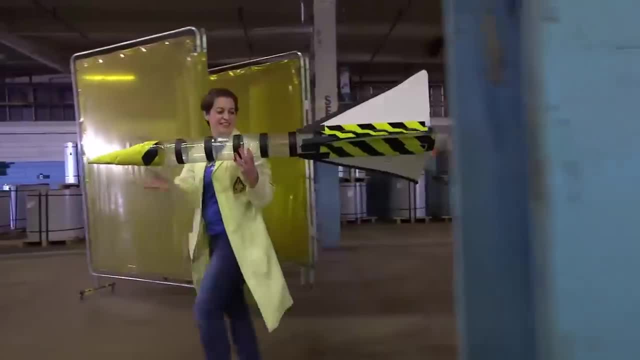 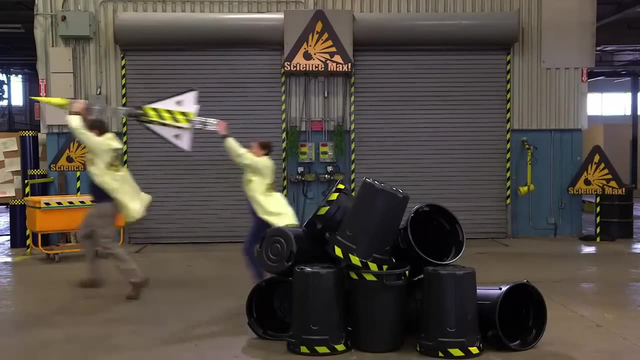 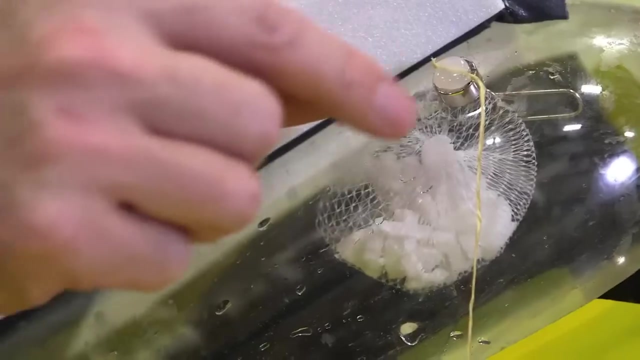 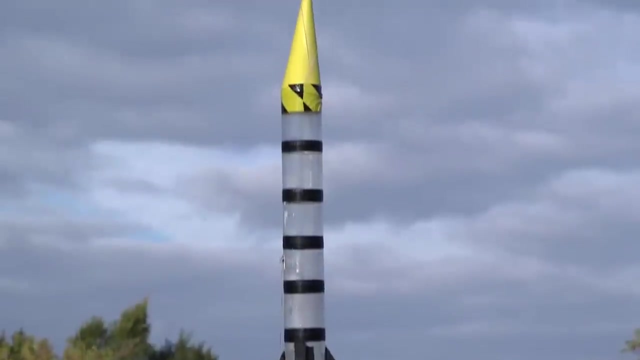 So the chamber is all the same. so it's all one big hollow tube tube, and now we're gonna fire it off. let's go. Lisa and I follow the same procedure as before. we use a bag of antacid tablets held up inside the rocket with a magnet and once it's sealed on the launcher, we pull it off. 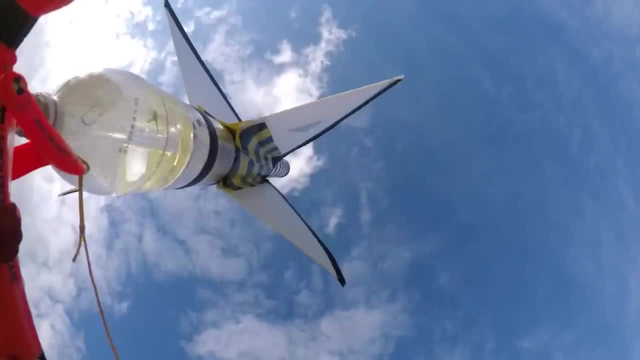 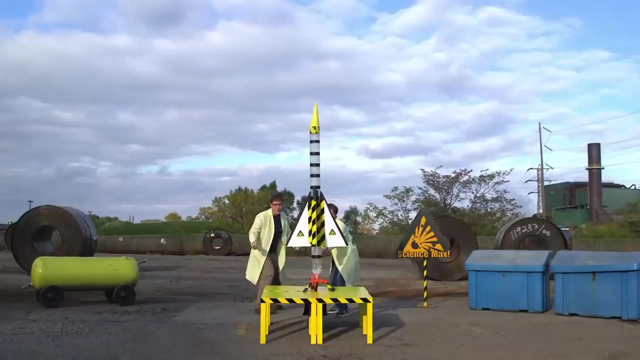 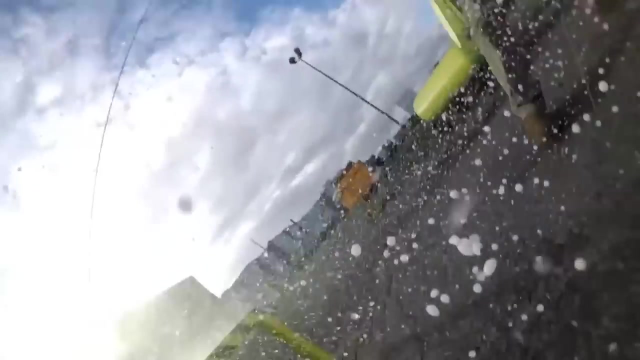 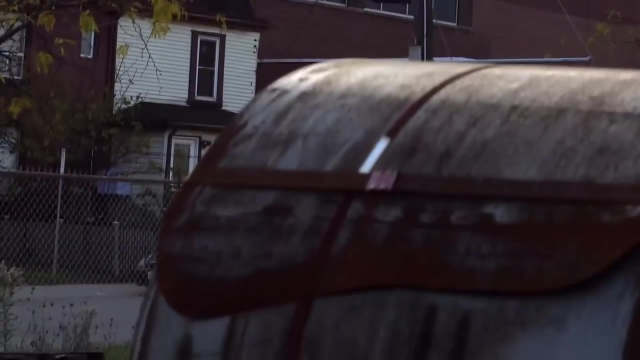 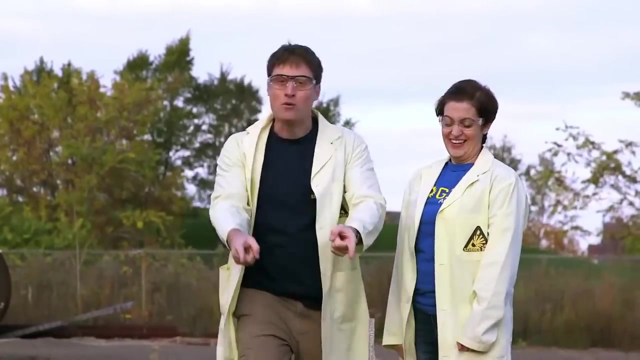 let the antacid mix with the water, let the chemical reaction happen for a while to produce enough gas pressure, and then we fire it. okay, here we go. three ever shot a rocket on science max. amazing, well done, chemical reaction rocket. thank you very much for joining us on science magic. 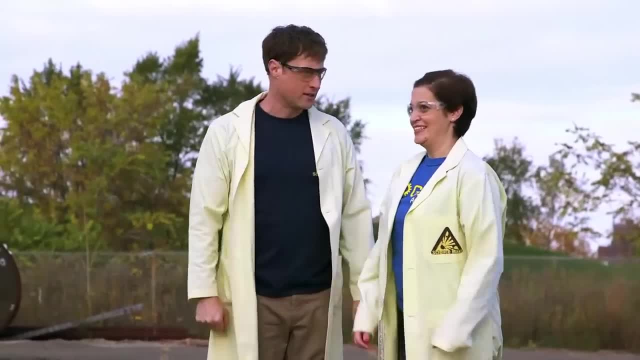 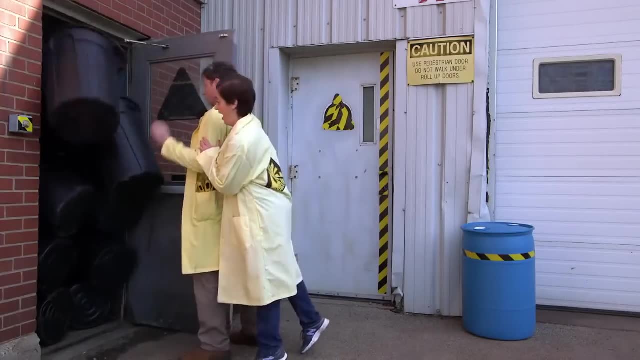 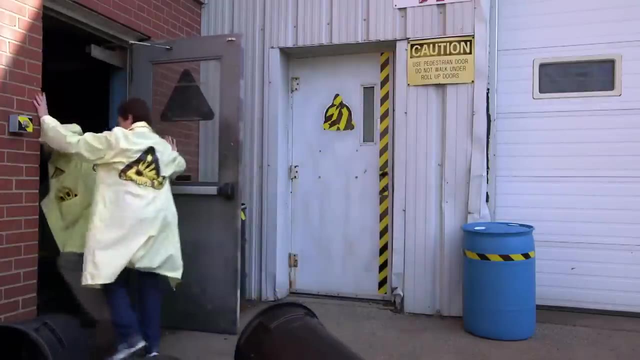 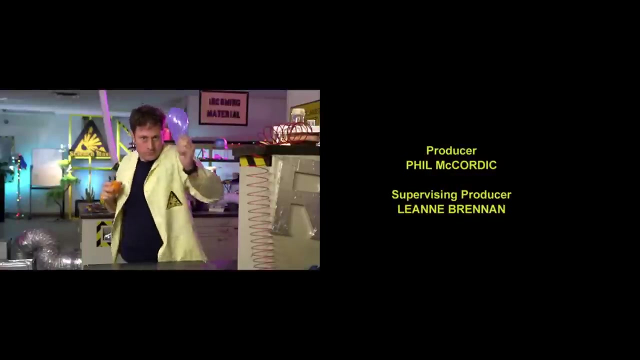 at large, we should build another rocket, because that one is probably broken. that's done, okay, let's go do it all right? so this time, I think what we should need to do is nothing but garbage cans in there. we're gonna turn the portal up. science antacid- the perfect antacid for all of your science needs. 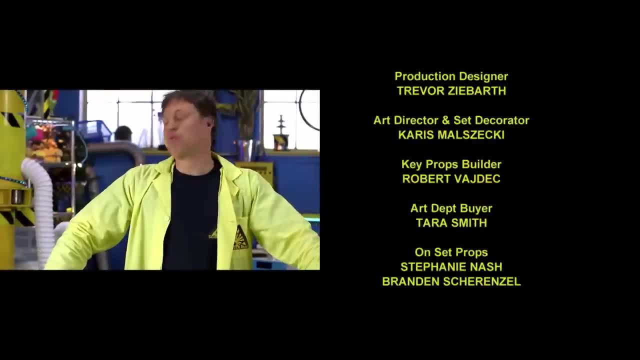 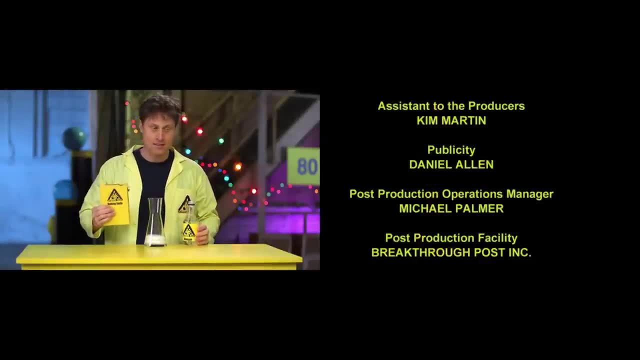 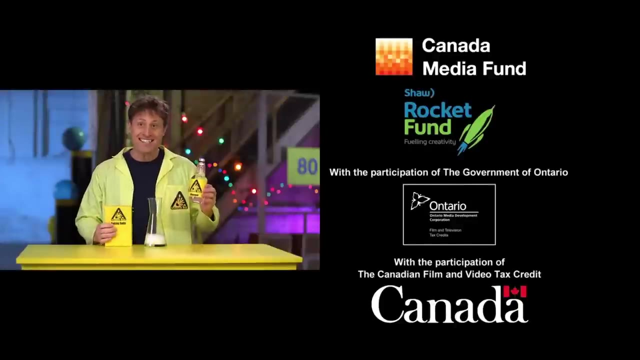 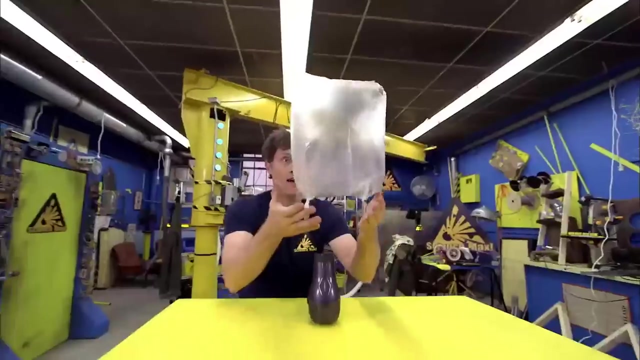 so let's launch some chem. let's launch see, vinegar is a base and baking soda is an acid. vinegar is an acid and baking soda is a base. science guy: have you ever done a science experiment and wondered what did it be like if you did it big? I have. 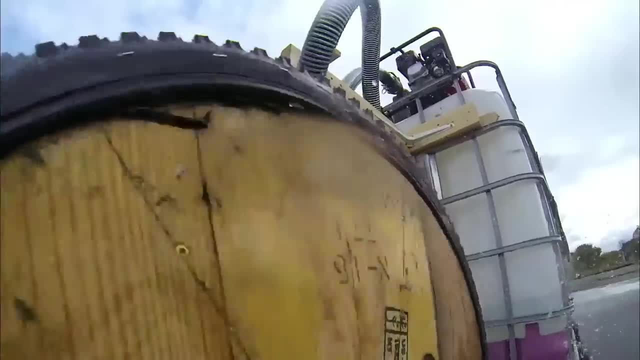 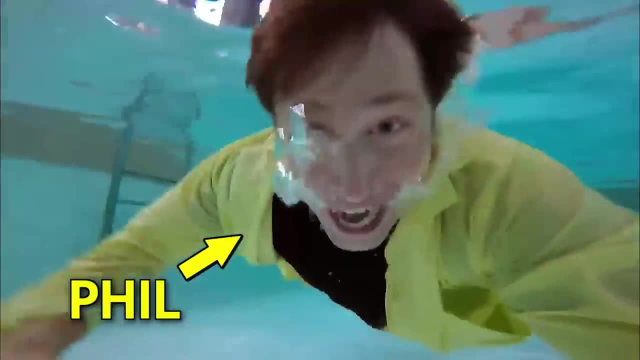 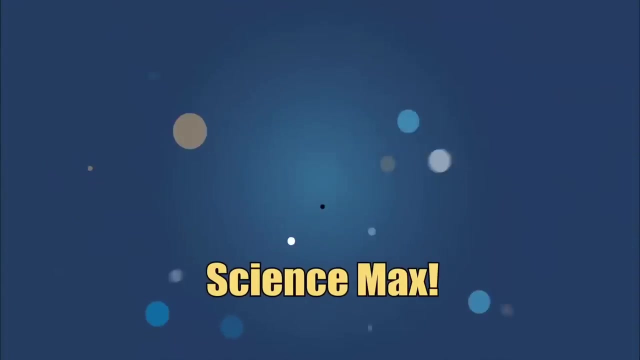 size isn't over the question. my name is Phil and I take your everyday science experiments and do them big. this is science max: experiments at large. on this episode of science Max, I'm on a. this episode of science Max, I'm on a quest to harness the power of lightning. 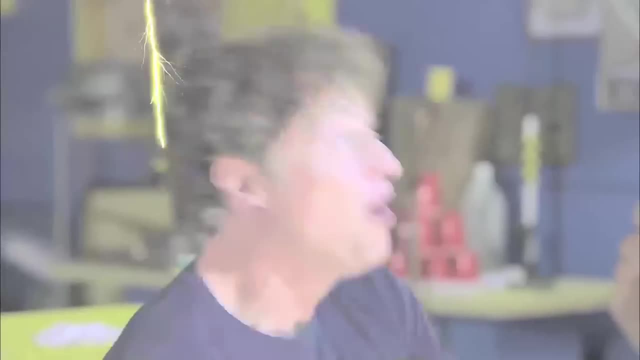 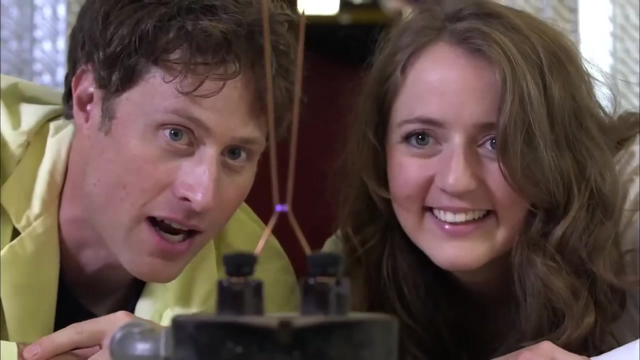 quest to harness the power of lightning. it's balloon-sticking, hoop-like. on a quest to harness the power of lightning, it's balloon-sticking hoop-like. it's balloon-sticking hoop-like. The balloon-sticking hoop-levitating hair-raising power is all thanks to static electricity. 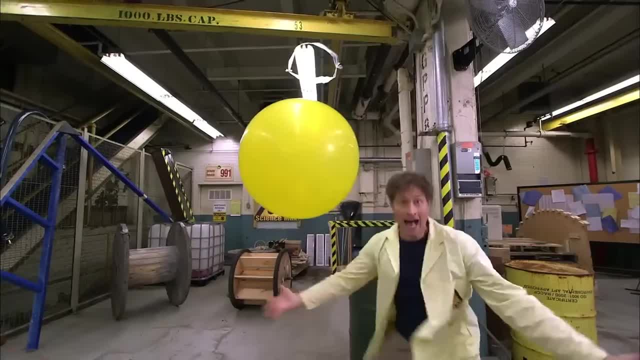 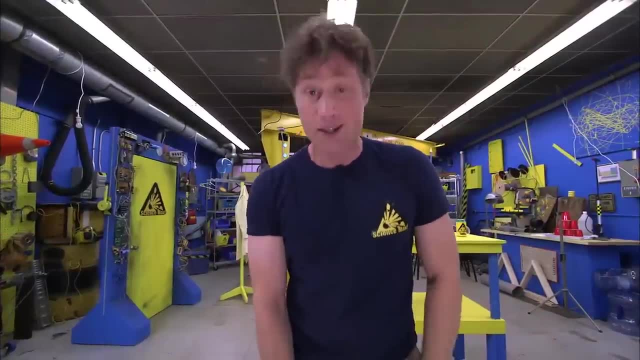 Hold on to your grounding rods. there's electricity in the air. All on this episode of Science Max Experiments at Large. Greetings Science Maximites. welcome to Science Max Experiments at Large. My name is Phil and today, on Science Max, we're going to be harnessing the awesome power. 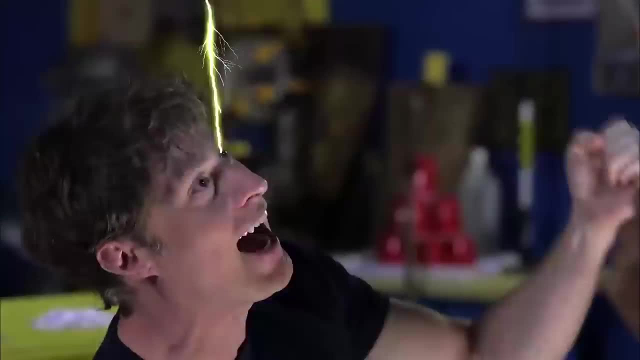 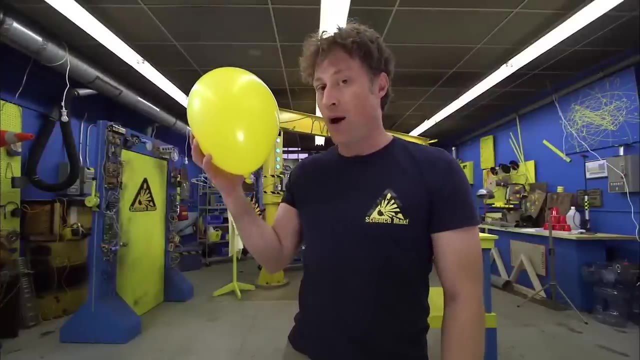 of lightning. Wahahaha, Wahahaha. How are we harnessing the power of lightning, you ask, With this balloon? I know what you're thinking. You're thinking, Phil, what's similar between a balloon and lightning? Well, nothing right now. 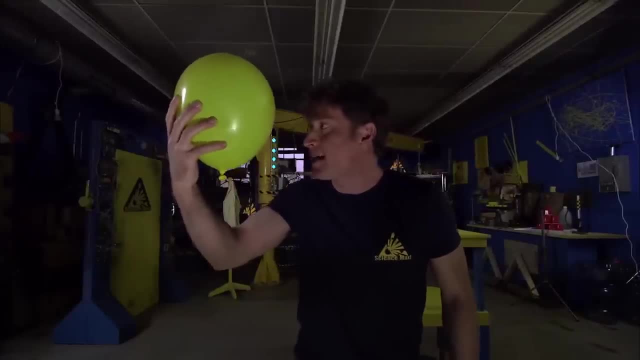 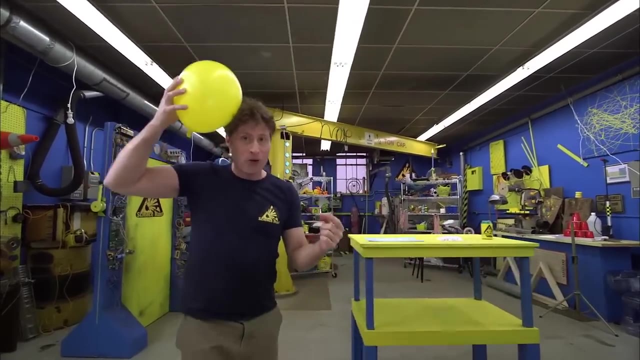 But behold as I use the power of static electricity and rub the balloon on my head, because basically that's how it starts. You see, when I rub this balloon on my head, it's stealing electrons from me, creating a positive charge in my hair. 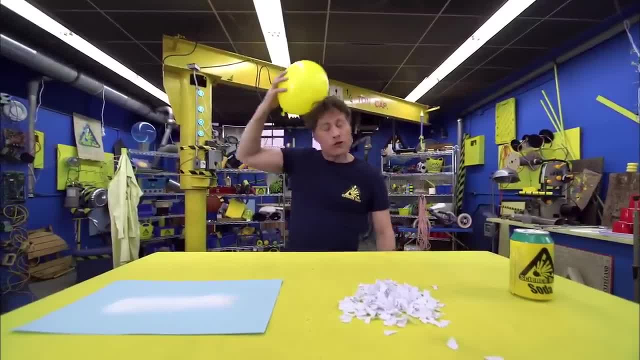 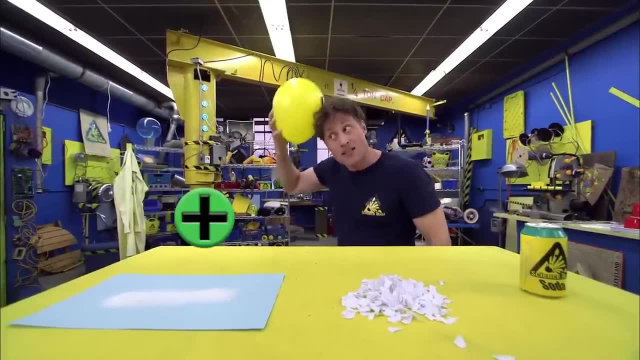 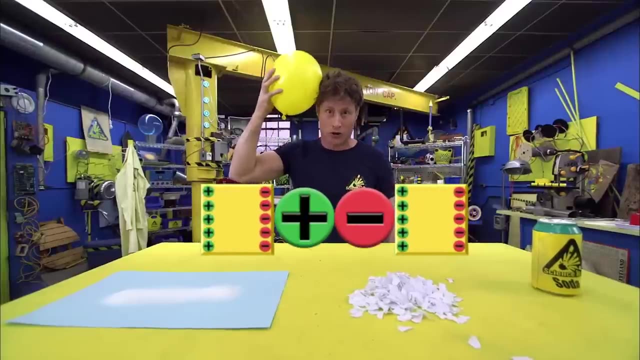 And a negative charge in the balloon. And the interesting thing is you know that things with opposite charges attract each other. right, Something that has a positive charge will attract negative things, and vice versa. But anything with a charge will attract anything with a neutral charge. 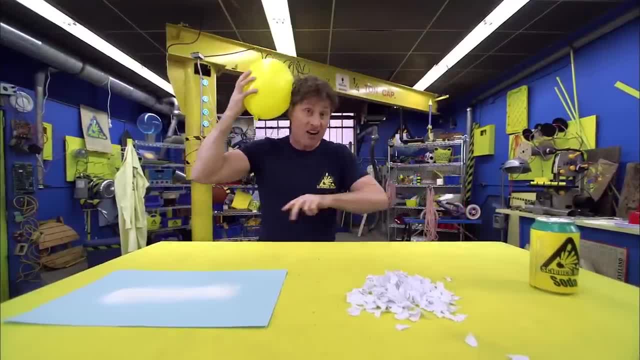 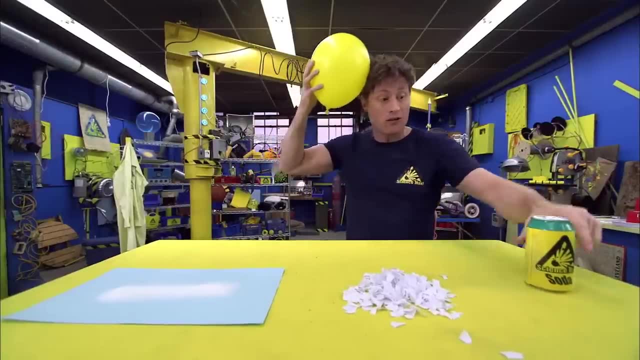 See all these things on the table. They all have a neutral charge, which means they've got equal amounts of positive and negative. Right now, this balloon is building up a big negative charge, which means it will be attracted to all of these things. 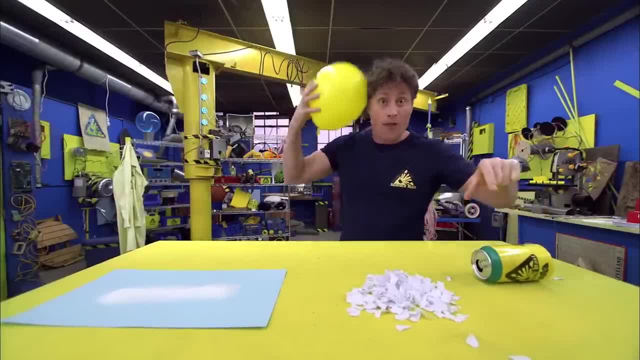 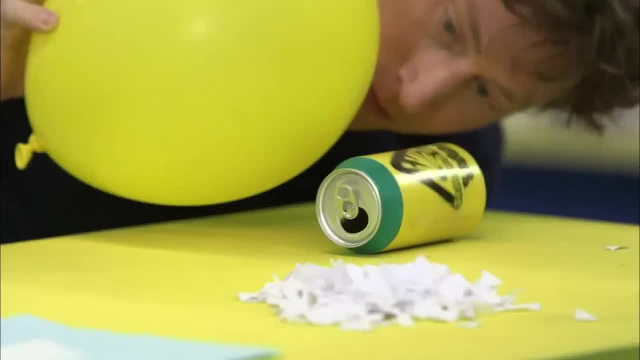 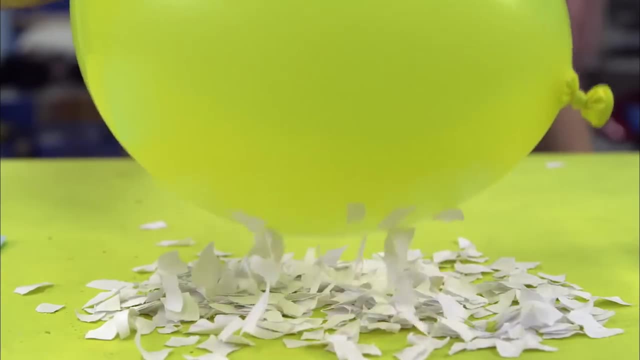 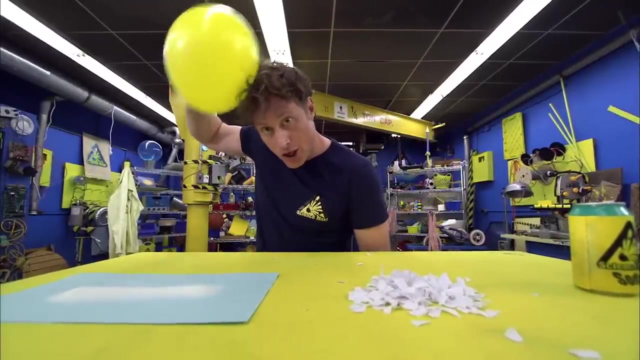 This can of Science Max Soda. it has a neutral charge. The balloon has a negative charge, which means the can will be attracted to the balloon. And this paper is neutrally charged, which means the paper will be attracted to the balloon. And if you hold the negatively charged balloon next to neutrally charged sugar, ha ha sugar. 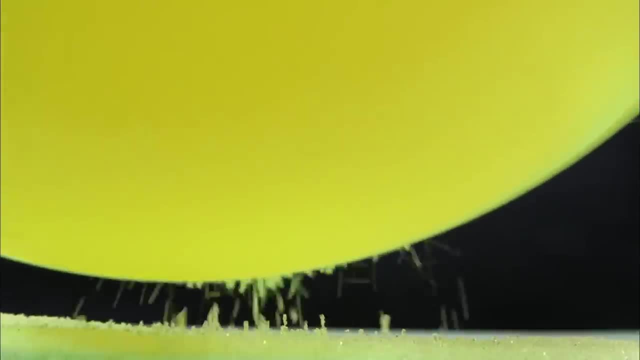 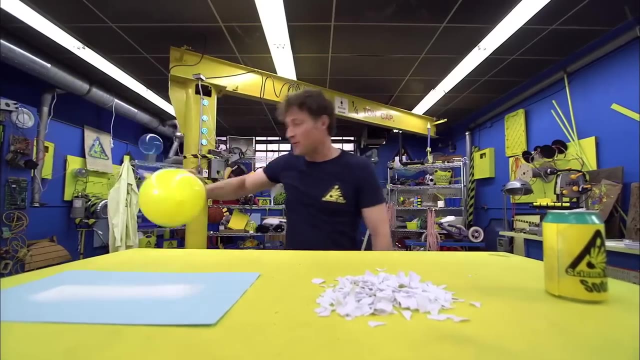 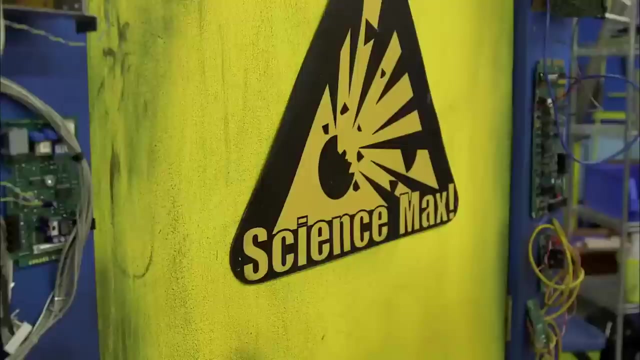 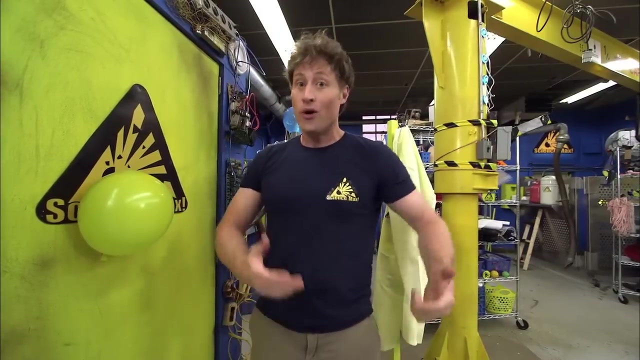 storm And you probably wait. I don't want to get sugar in my hair and you probably know this trick: If you rub a balloon on your head, you can stick it on the wall. ha ha. But what does any of this have to do with lightning? 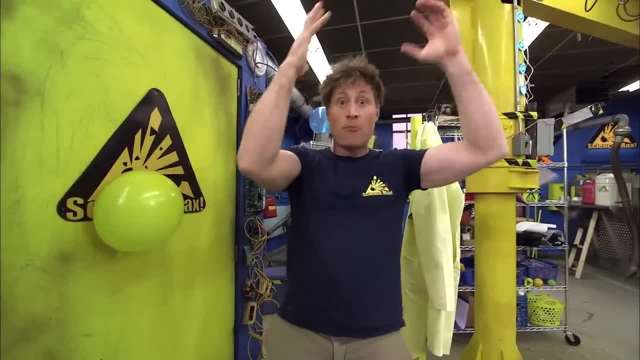 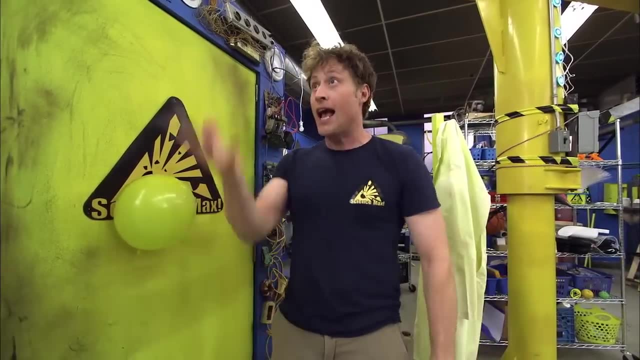 Well, the same thing is going on with a lightning bolt. The clouds become negatively charged and that negative charge wants to equalize itself with the ground, Which is neutrally charged, And that lightning bolt is the electricity jumping from one place to another. 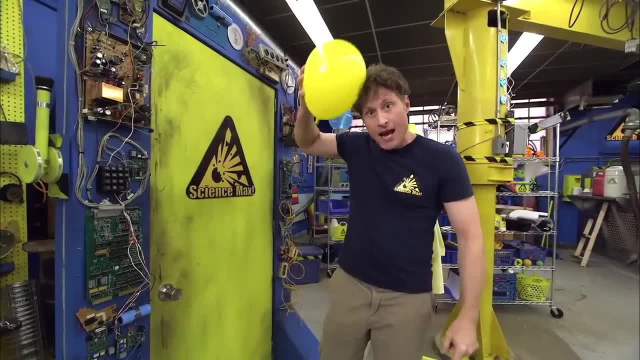 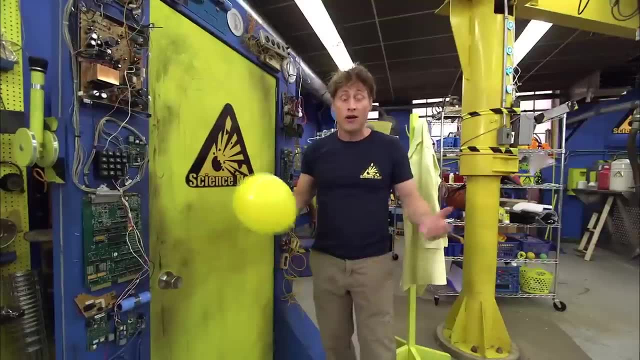 And you can see this yourself. If you rub a balloon on your head and you put it next to something metal, like a doorknob, there'll be a spark. But here's another thing you can do if you don't have a balloon, which I guess I don't. 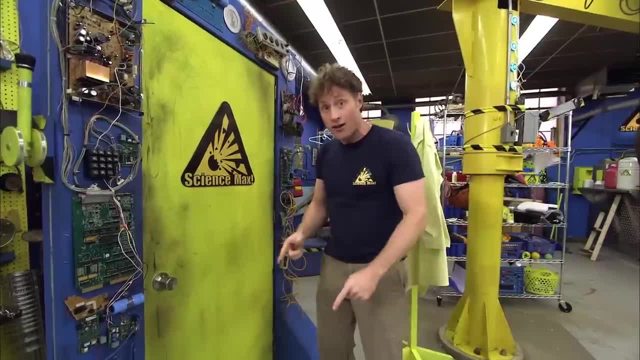 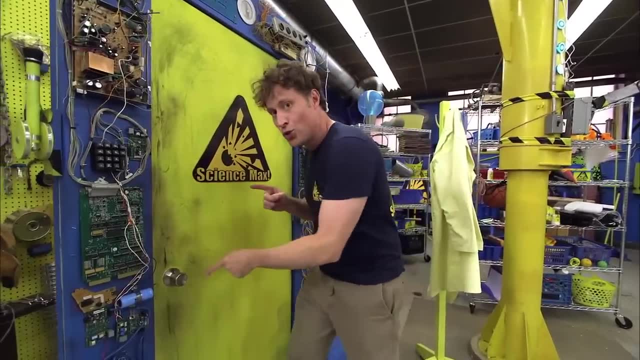 anymore. Rub your feet if you're wearing socks on a carpet and then turn out all the lights and touch a doorknob, You might be able to see a spark jump from your finger to the door. That's lightning. 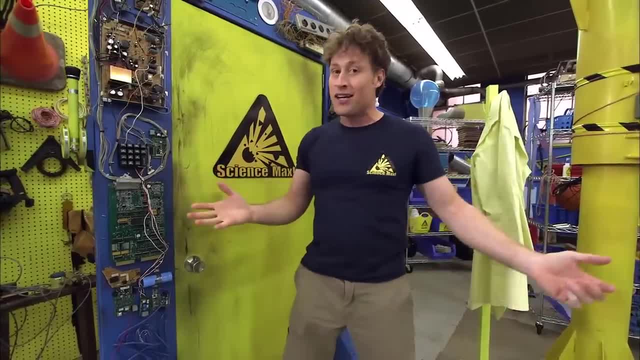 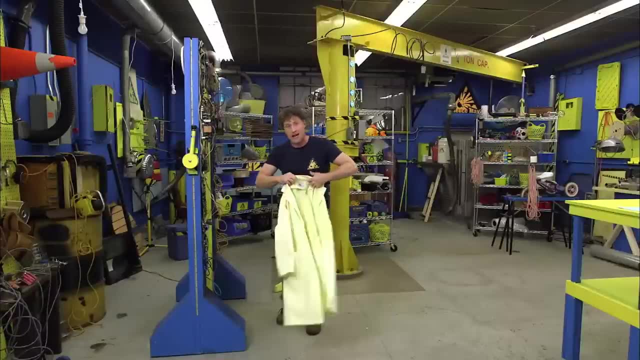 In a very, very small form. So that's what we want to do today. on Science: Max Experiments at Large, Max out lightning, I think I'm gonna go to the Ontario Science Centre and ask Heather her advice. She really knows her stuff. 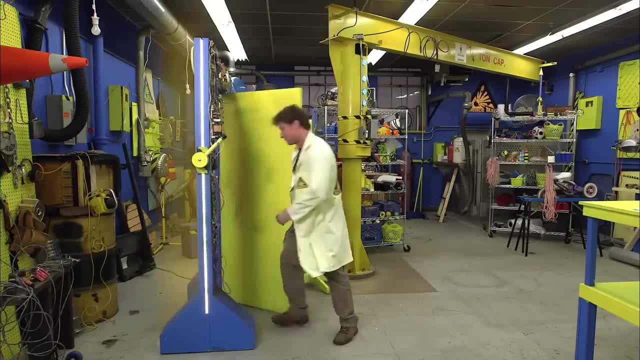 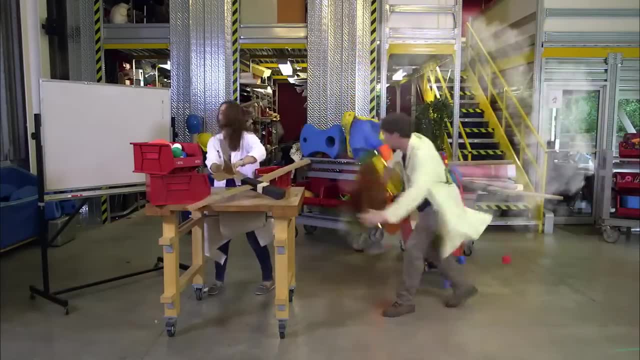 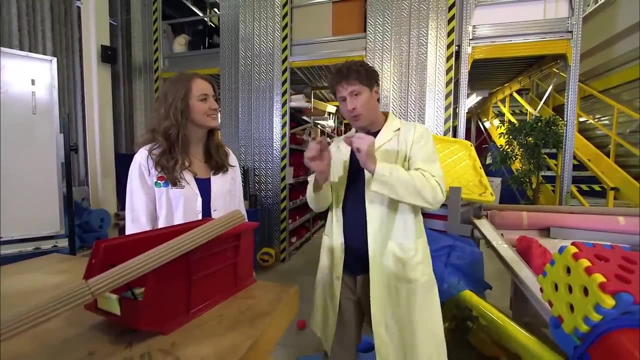 I'm gonna go see if she's busy right now. Come on, Will you got the portal fixed though? eh Well, it's not exactly fixed. It's still got a couple bugs that I'm ironing out, but I stopped coming in 10 feet above. 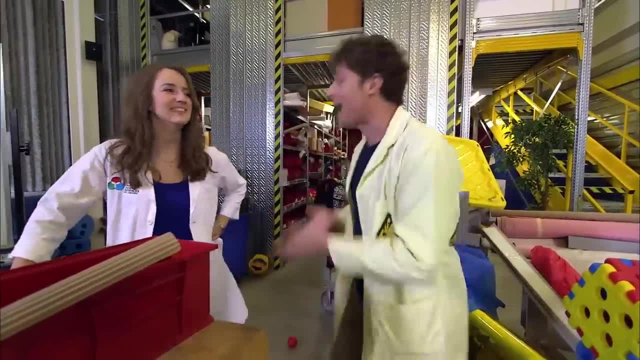 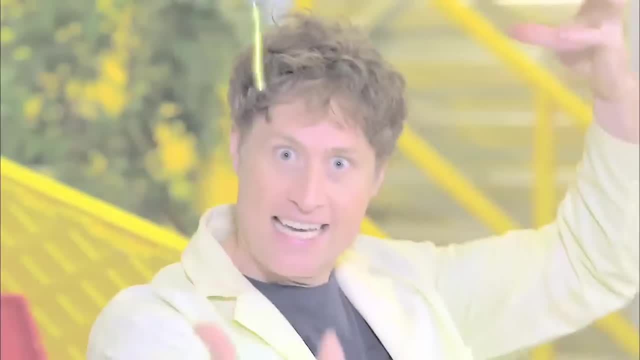 the floor. Hey, So that's a step in the right direction. Anyway, Heather, I've come here because I want to ask your advice on something. Yeah, for sure, Awesome. So what I am doing is creating lightning. So this is where I'm at right now. 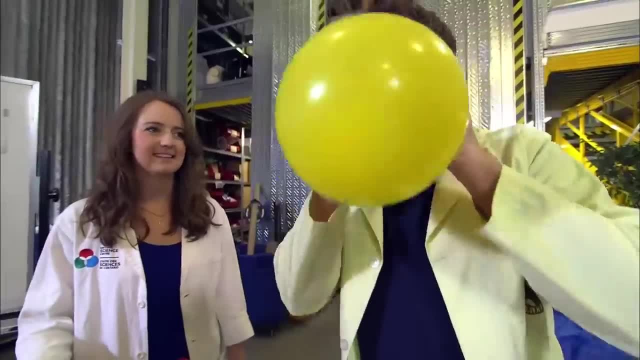 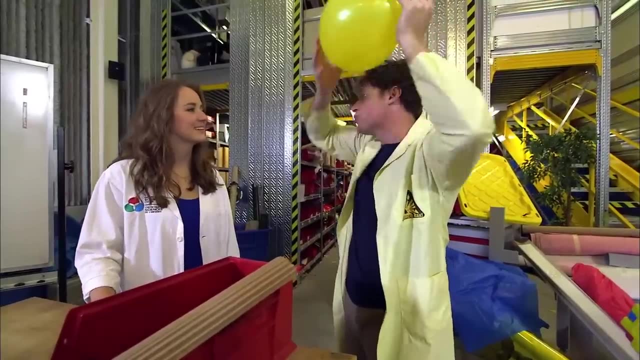 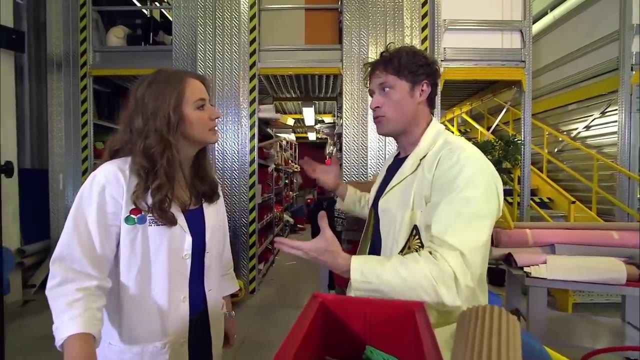 So this is a balloon. I blow up the balloon And then I rub it on my head And it creates a static charge, right, Right, yeah, Just like in the lightning bolt between the clouds and the ground. So I was wondering if you could help me. maybe max that out. 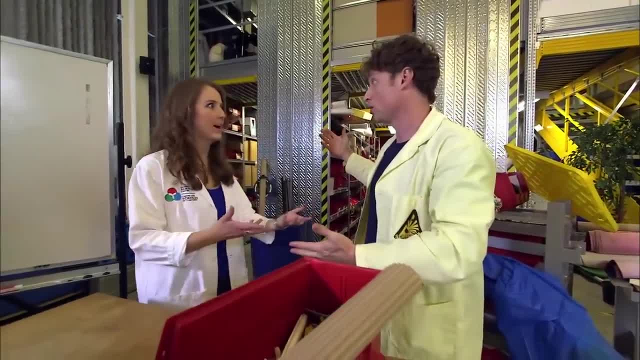 And I thought the perfect place to start would be a larger balloon. Ooh, right on, Actually. yeah, I like this. Yeah, I've got a big balloon. If you just give me a second, Sure, All right, catch. 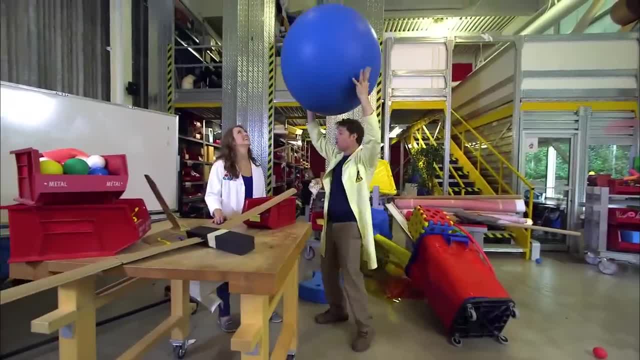 OK, All right, giant balloon. So what I figured is I'll just start rubbing it on my head, OK, And then we could maybe stick it to the wall or something. Yeah, I think instead of a wall we can even try on this whiteboard here. 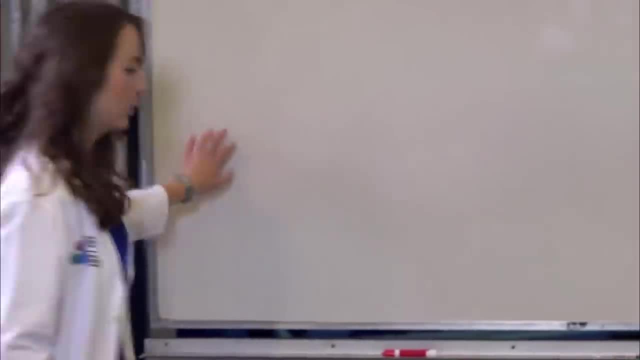 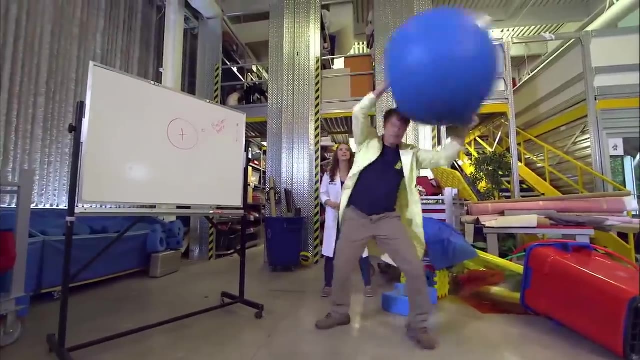 Oh, OK, great, Keep rubbing. I'm rubbing. All right, ready? Yeah, Let's give it a try. Here we go, And So that didn't exactly work, Right? yeah, Both of us rubbing our heads on the balloon. 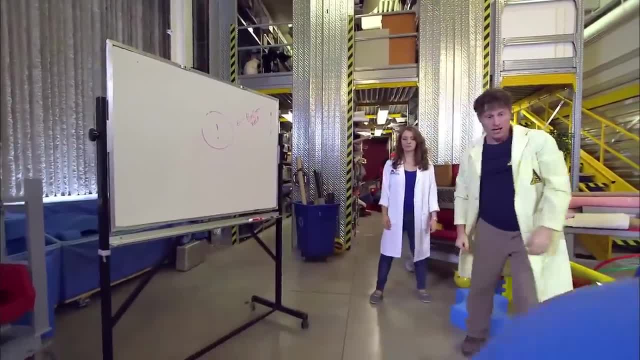 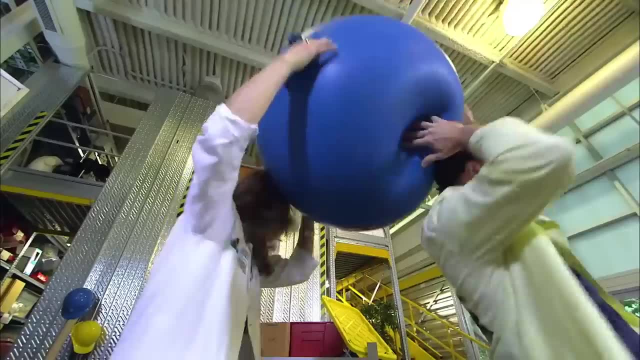 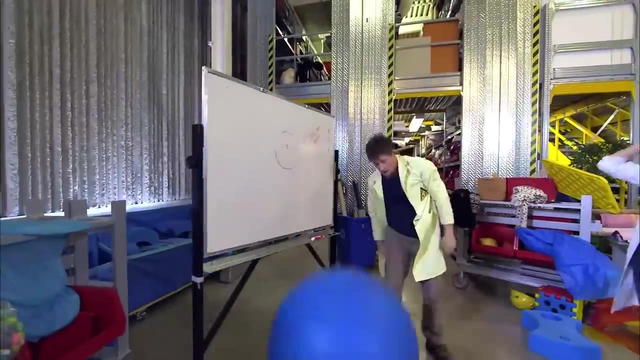 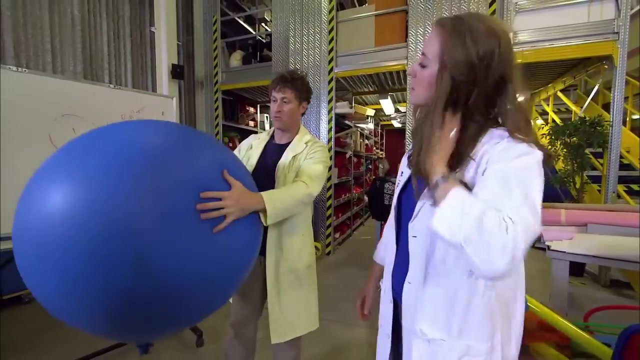 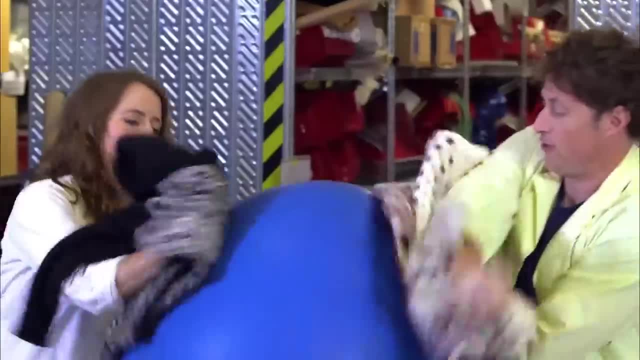 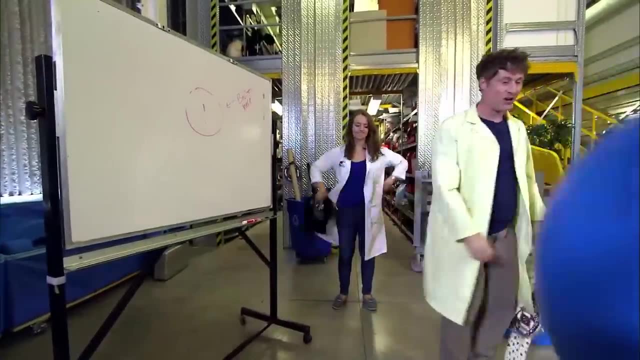 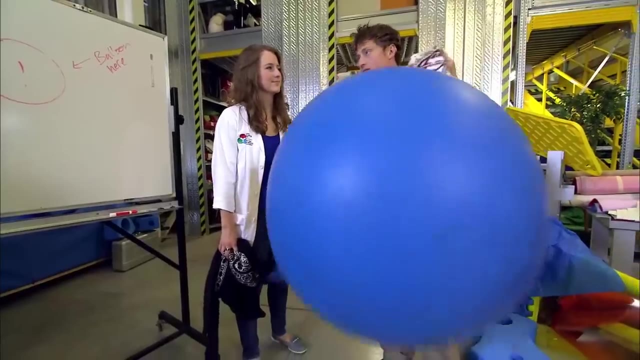 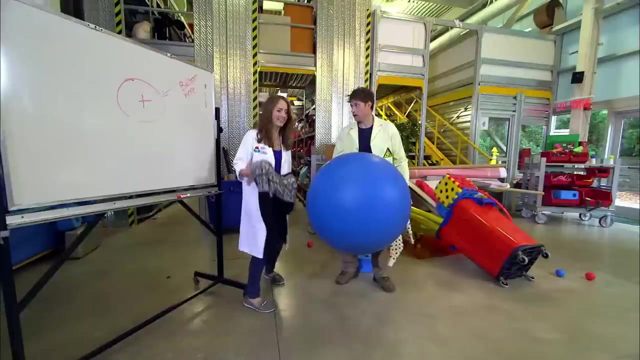 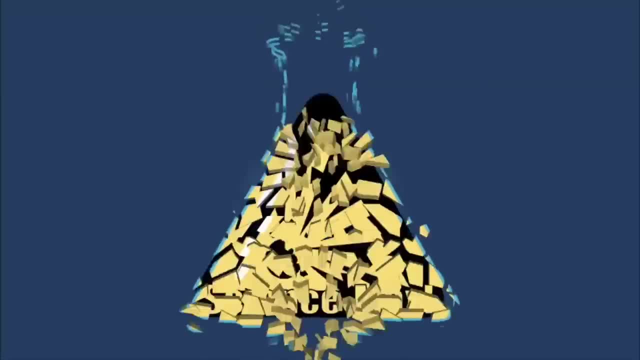 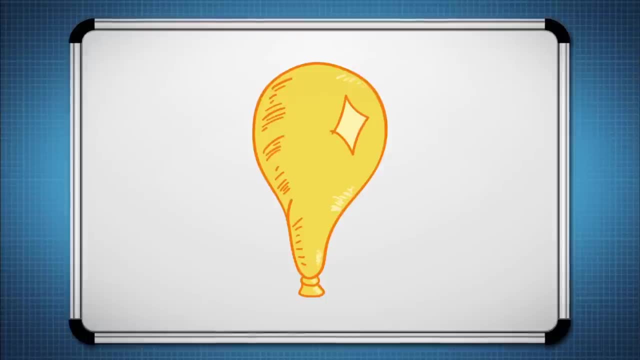 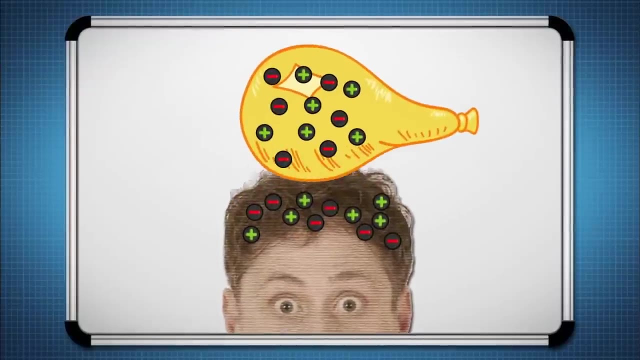 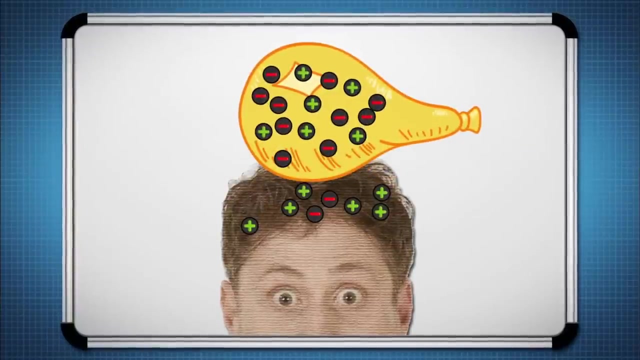 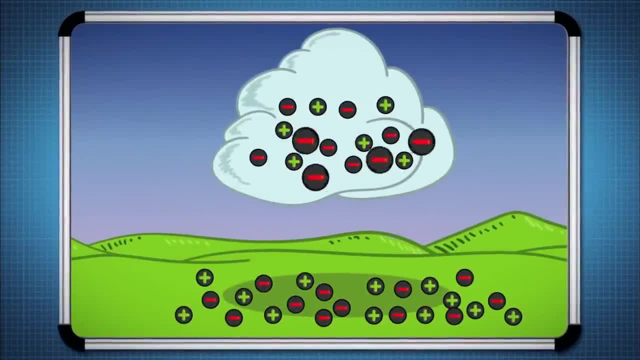 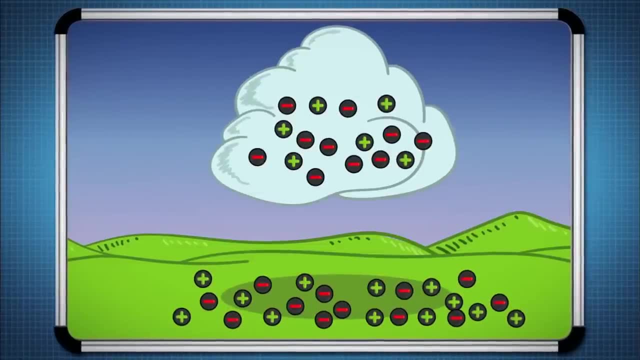 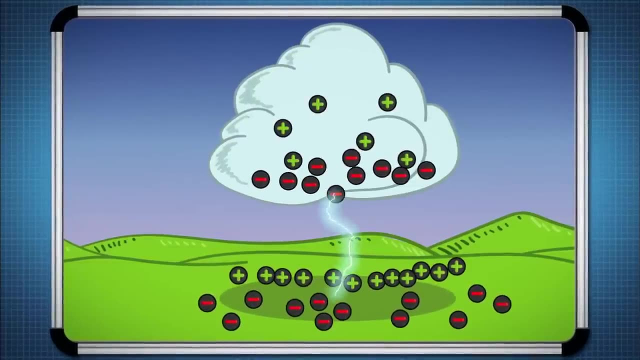 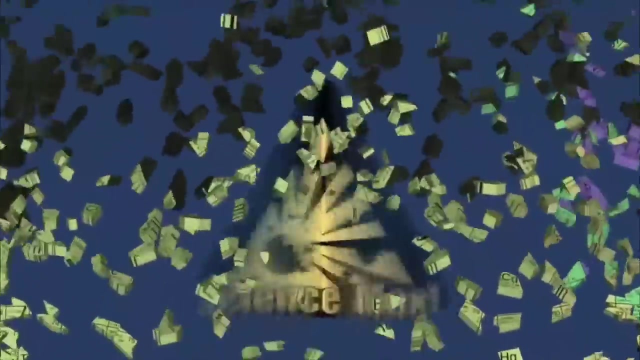 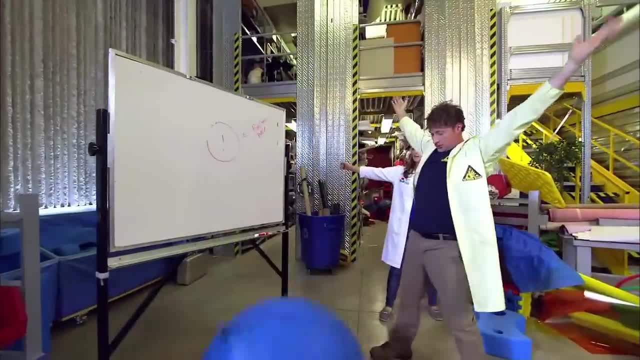 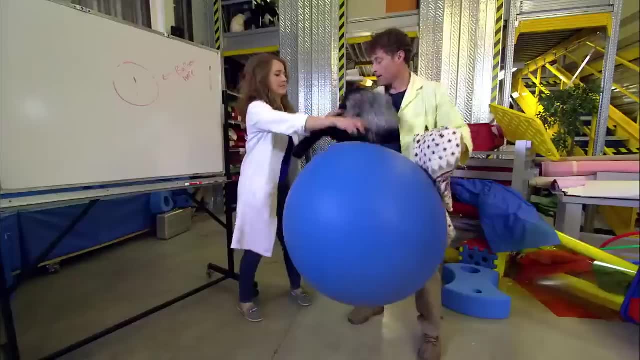 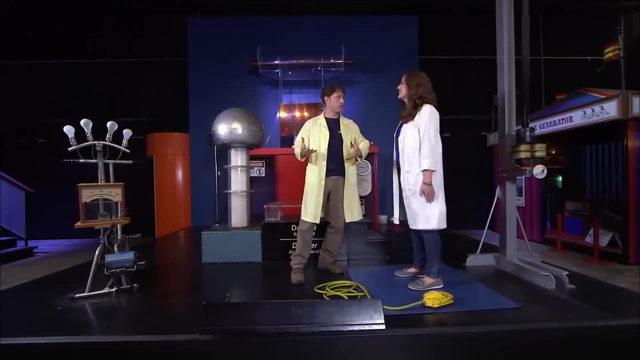 but a big heavy balloon just doesn't hold the same charge. That didn't exactly work, But we're only interested in maxing out the static charge and Heather knows just what to use. Wow, So this is the Ontario Science Centre electricity show. 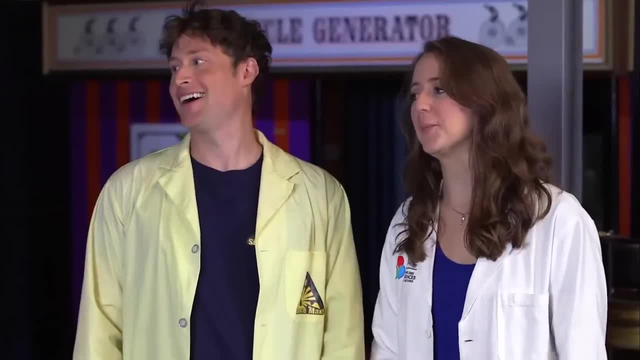 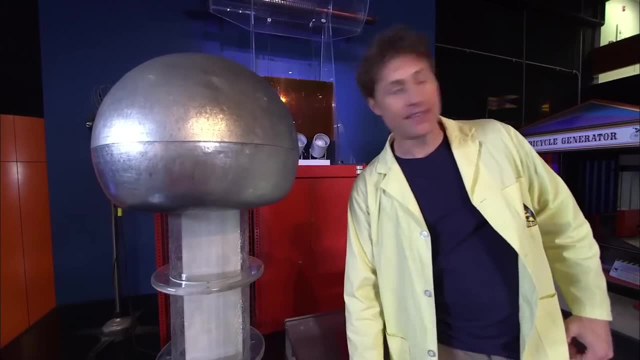 Yes, Okay. so where's the electricity part? The one we're going to be playing with is right there. So the giant mushroom- Yeah well, it does look like a mushroom. We're going to make some sort of electricity salad. 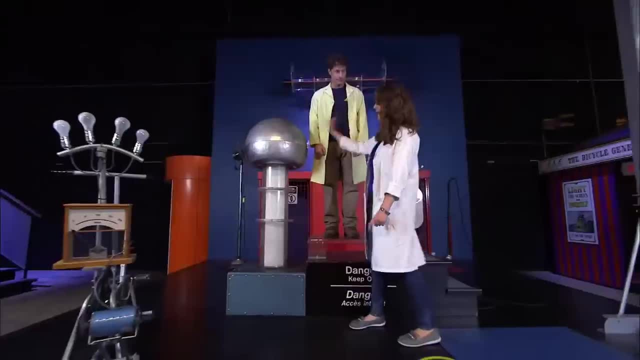 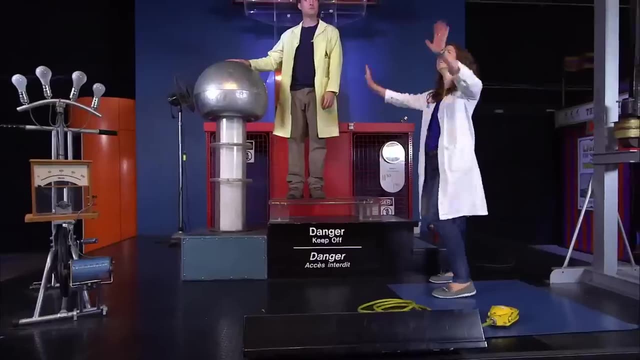 All right, head on up onto that platform right there And I need you to put one hand on that silver ball. Yes, So the way it works, Nothing is happening. Patience, Okay, Once I turn it on when I engage it. 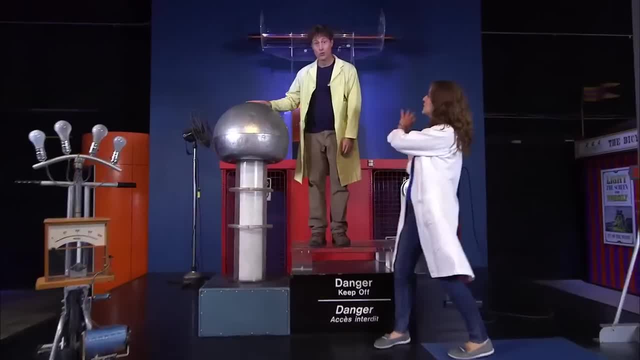 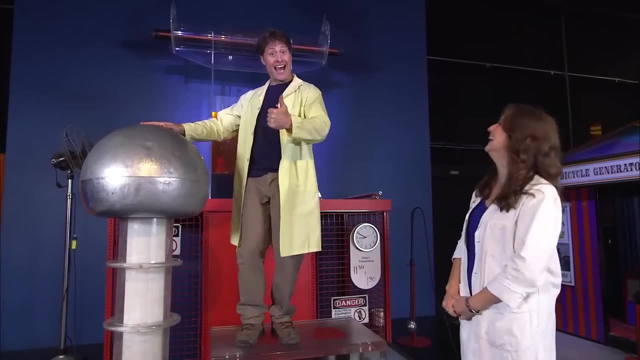 this is going to steal your negative charge, So it's going to steal your electrons. So if it steals electrons, you're going to be pumped. I'm positively charged, So it'll make me more positive, Even more positive, Yay. 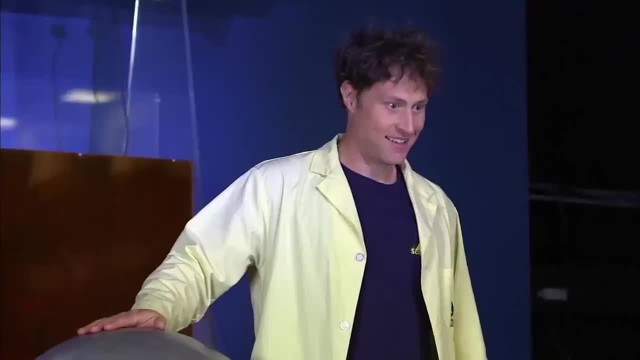 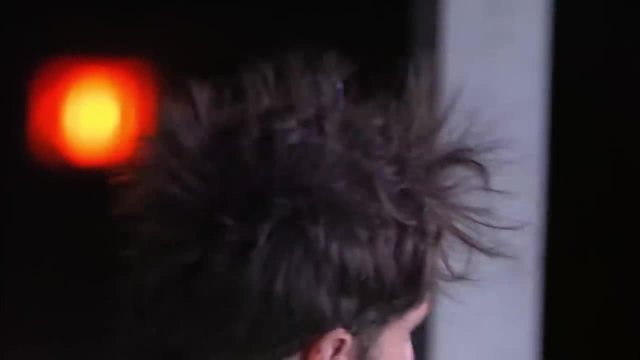 Woo-hoo, I am positive. Here we go, Woo, Ha-ha-ha-ha-ha. This machine is called a Van de Graaff generator and it pulls the negative charge away from the person touching it. Ha-ha-ha-ha-ha-ha. 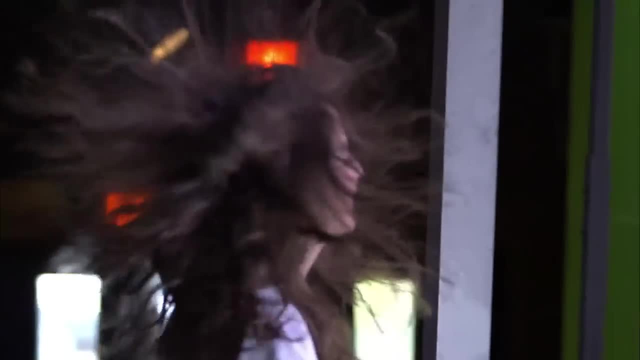 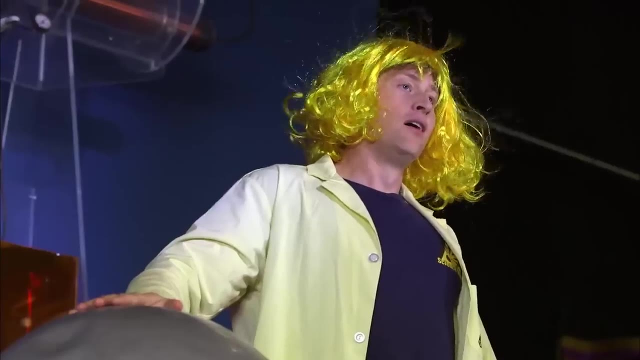 That is great. Instead of having equal amounts of positive and negative charges, you become positively charged. Woo-hoo, Science hair, Yeah, Like when you try to put two positive ends of magnets next to each other, each hair on your head starts to repel the others. 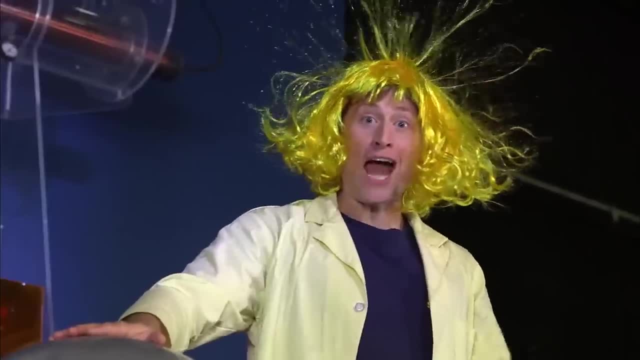 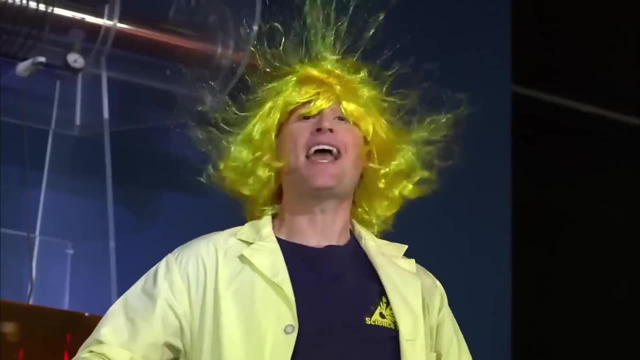 and be repelled from your head. Science hair Dude. So your hair stands up. Ah, yes, Woo-hoo, I can't see anything. So this is more of a machine to generate hair standing up, but it doesn't make lightning. 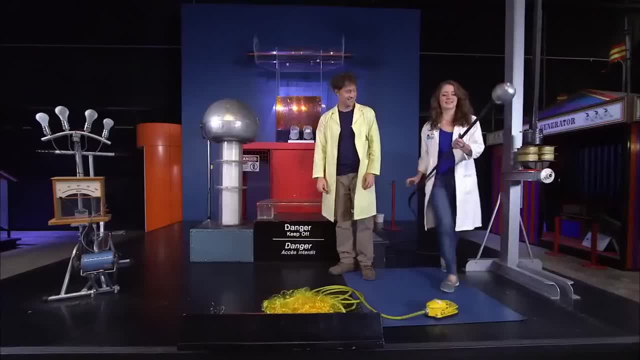 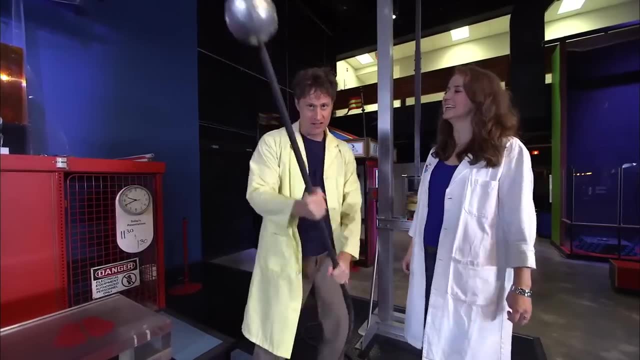 Oh well, actually I have a demonstration in my back pocket. This is going to help us, Okay, To create lightning. This is our grounding rod, It is my scepter of science, And so we're going to use this to continuously provide that negative charge. 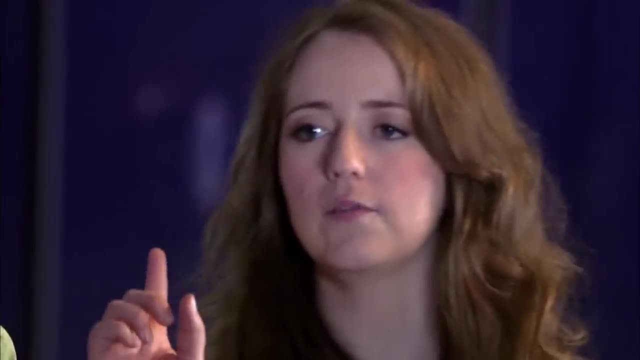 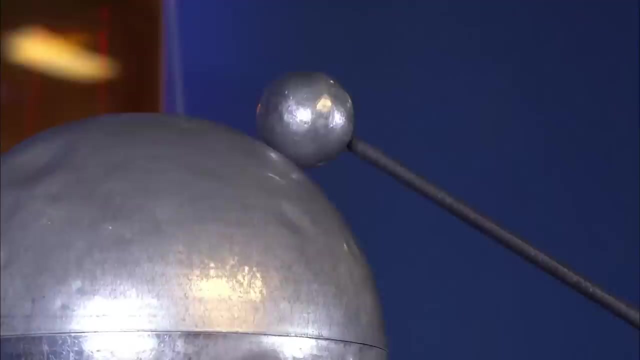 That's why it's plugged in. That's why it's plugged into the ground. yeah, Okay, Okay. so then, if you touch it to that metal ball, Got it Not too exciting, right? So pull away and let's see what happens. 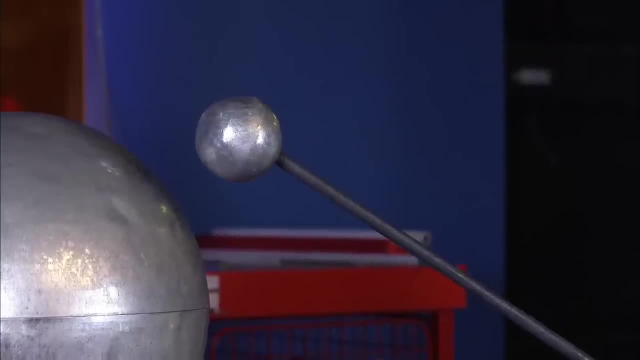 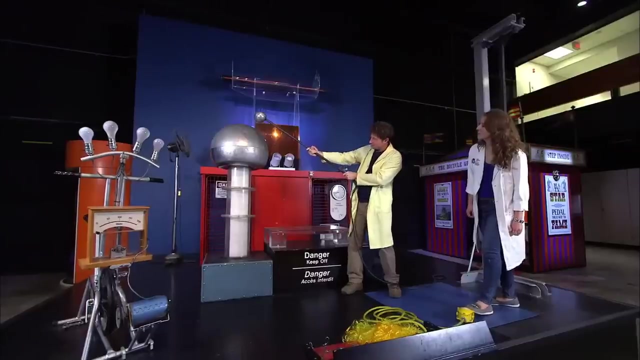 Whoa, Ha-ha-ha-ha. This is what I'm talking about. Very good, The Van de Graaff creates a positive charge, The rod has a neutral charge. When the difference becomes big enough, the charge jumps the gap. 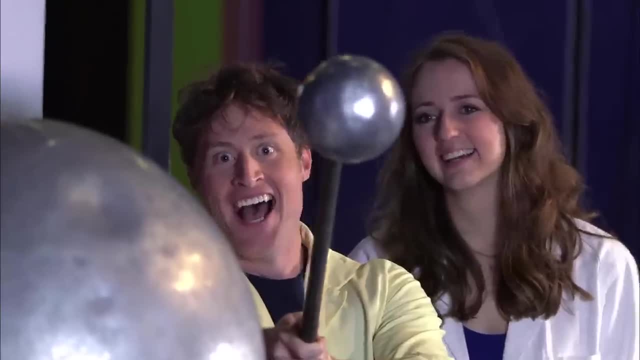 Behold, I have the power of lightning. Ha-ha-ha-ha, Ha-ha-ha-ha, Ha-ha-ha-ha, Ha-ha-ha-ha. So it's the difference between the positive and the negative. 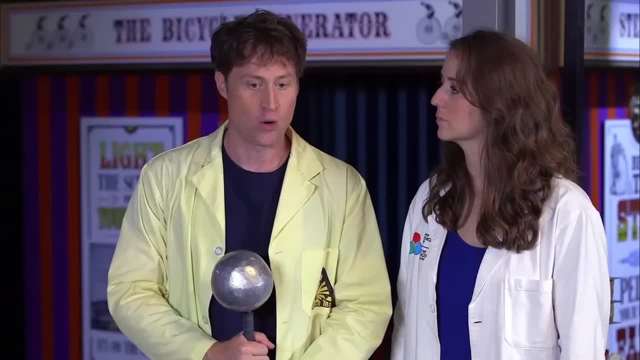 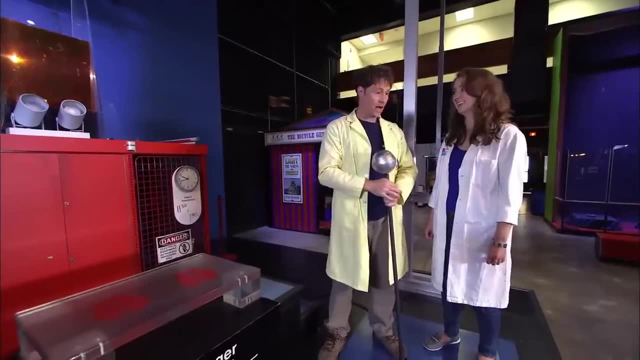 is what we want when we want to make a lightning bolt. Yes, So is there something we can use to make that happen? Large difference of charge: Yeah, I think I have just the thing. Oh yeah, Yeah, you want to check it out. 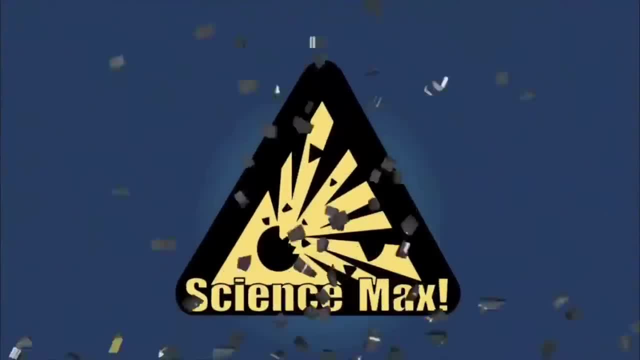 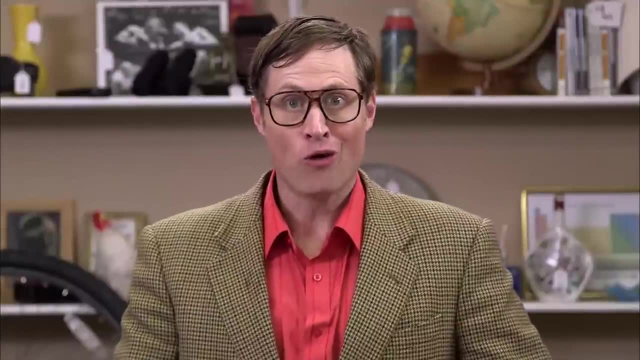 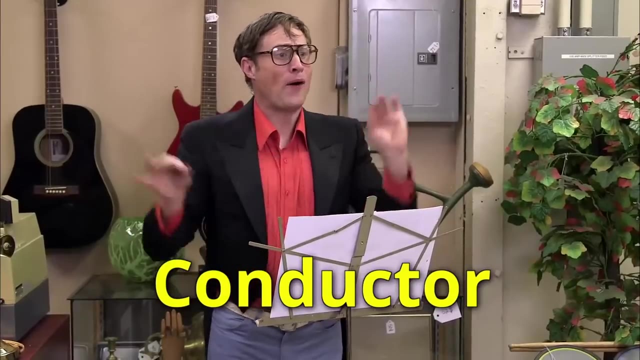 Absolutely. All right, let's do it. Okay, let's go. So you would like to move electricity from here to there? Well, what you need, my friend, is a conductor. All right, a little more arpeggio this time. 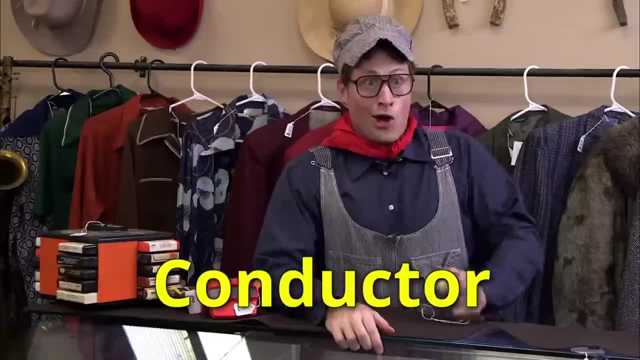 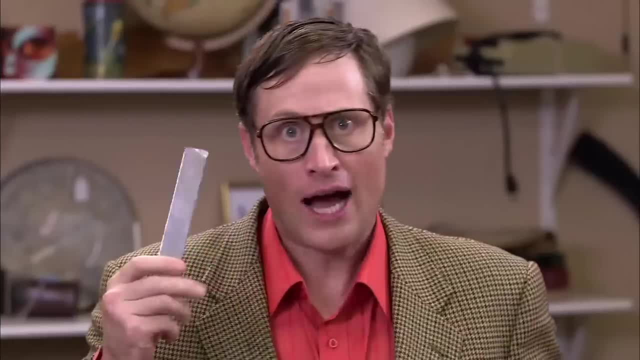 No, not that kind of conductor All aboard. No, not that kind of conductor either. This kind of conductor. I know what you're thinking. You're thinking, hey, this is a piece of metal. Well, that's right. 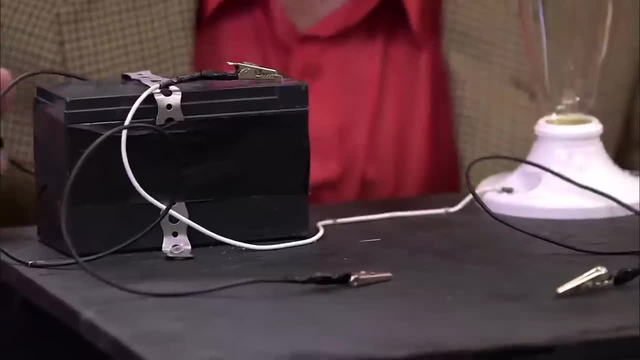 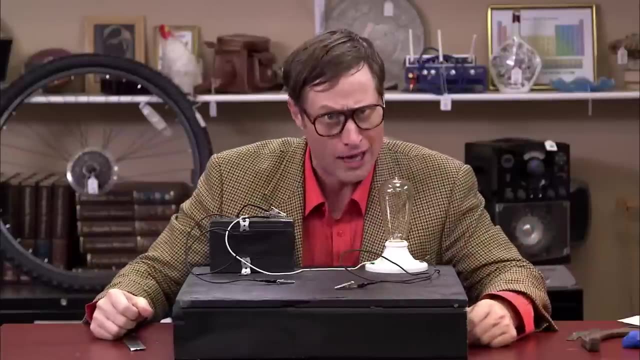 That's because you're smart. This is a circuit. Electricity flows from this battery along the wires and into the light bulb. But, Sal, you cleverly observed, the light bulb is not lit. This is true. That is because we have a gap in the circuit. 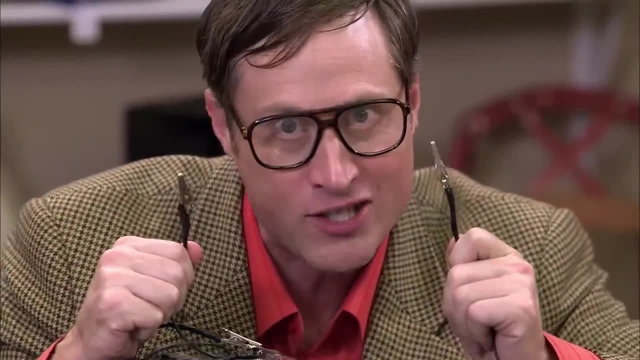 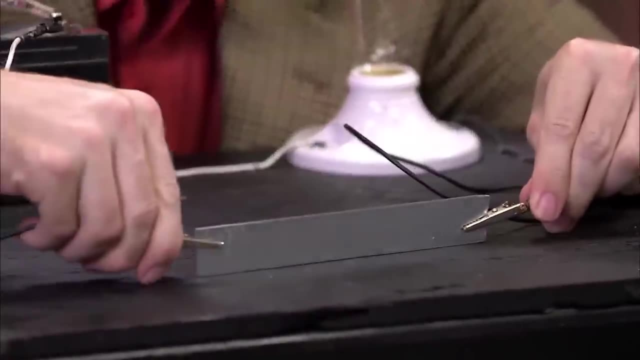 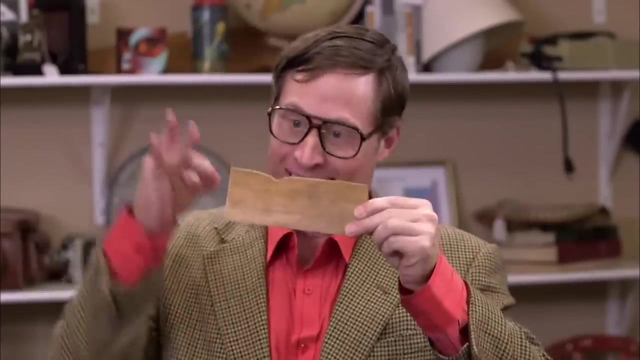 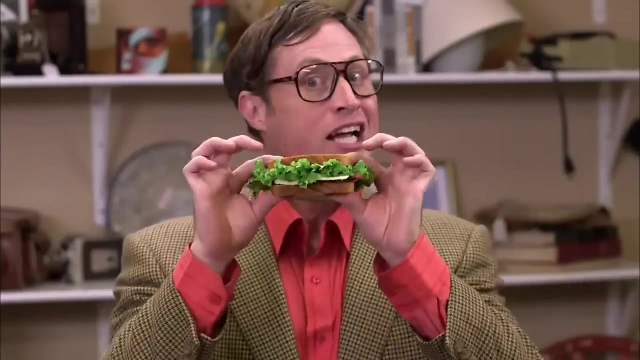 And air is not a good conductor of electricity, Is metal a good conductor of electricity? Let us find out. Metal is a good conductor of electricity. What about wood? Nope. What about this horseshoe Is a good conductor. Will this sandwich conduct electricity? 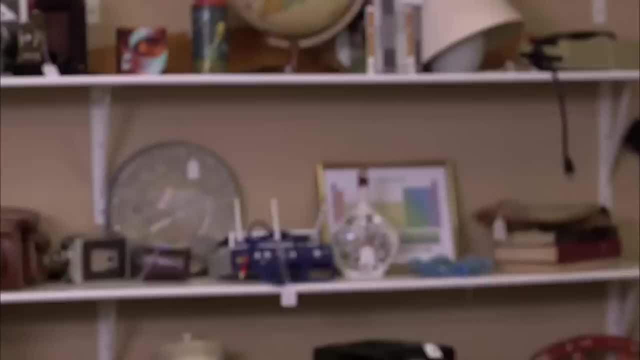 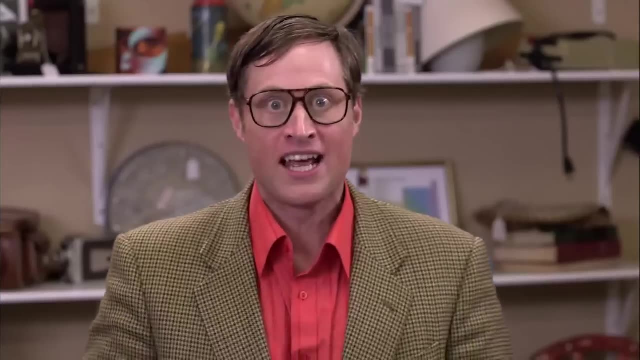 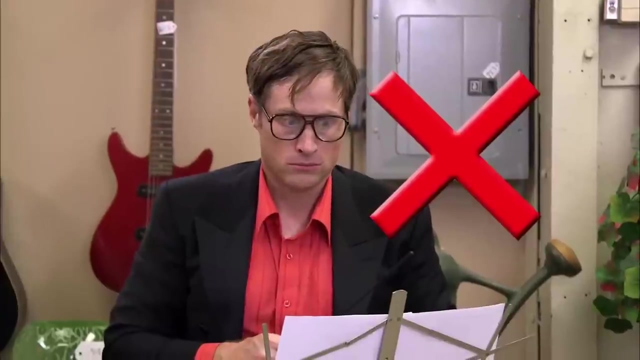 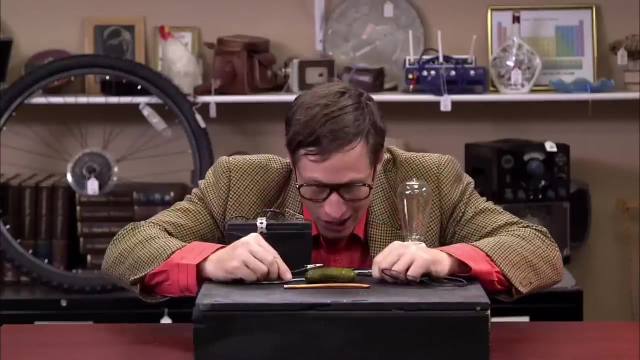 Nope, No. What about this plastic fish? Nope. What about this pickle? Nope, Nope, No. Pickle is not a good conductor. That's why we make electrical wires out of copper and not pickles, you know, in case. 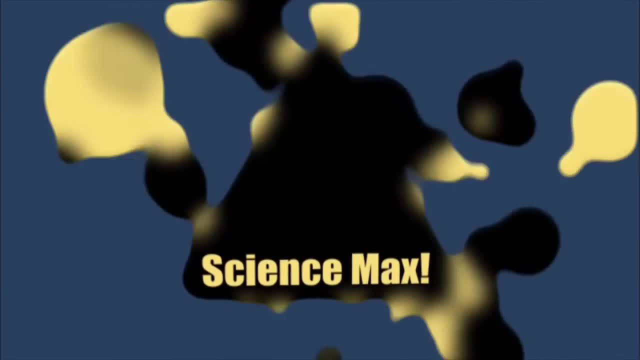 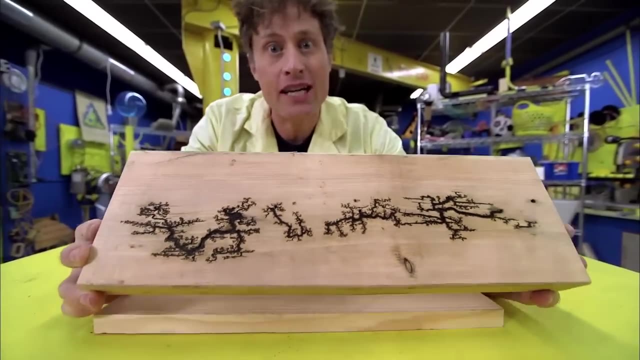 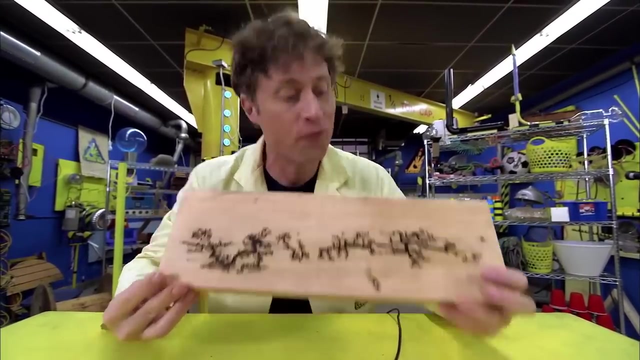 you were wondering, Lightning bolts make interesting patterns. That's because the electricity is searching for a way to get from one side to the other. But it's hard to see the patterns of lightning bolts because they happen so fast. Fortunately, using the power of science, we can observe these patterns for ourselves. 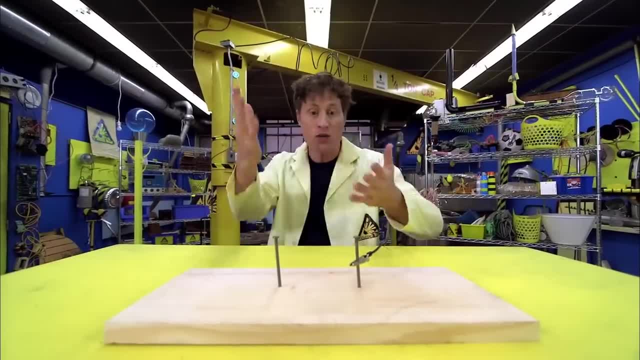 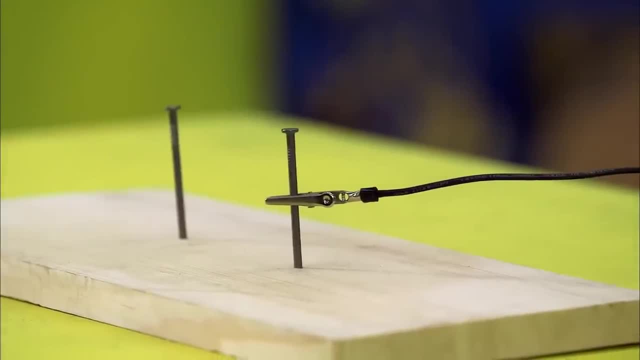 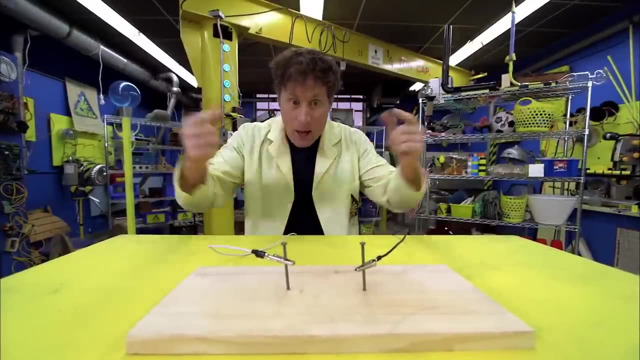 in a motion we can perceive, I'm going to use electricity to recreate a lightning bolt pattern. I've got two nails and a piece of wood here and I'm going to attach electrical leads to both nails. Now the electricity wants to go from that side to that side, but it can't. 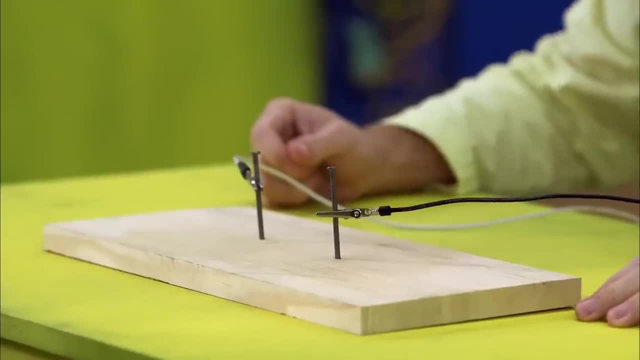 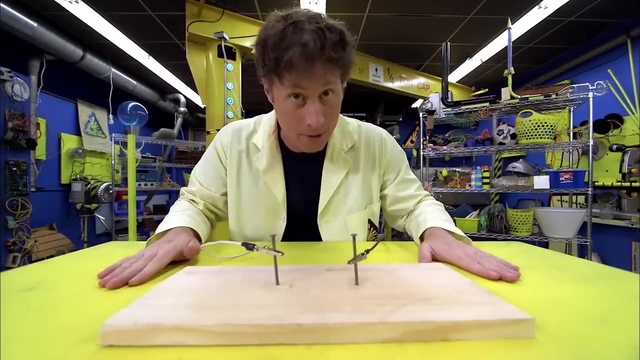 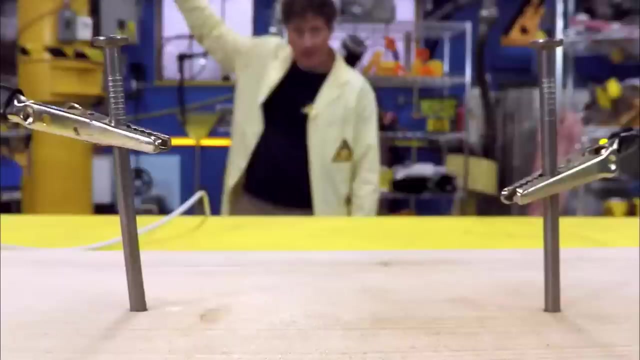 It has to go through the wood, and wood is not a very good conductor of electricity. Now, this is very dangerous. I need a special machine even to pull this off, so this is definitely not something you want to try at home. In fact, I'm going to stand way back here when I turn it on. 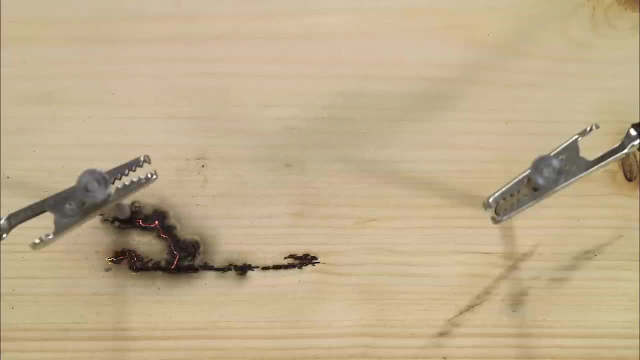 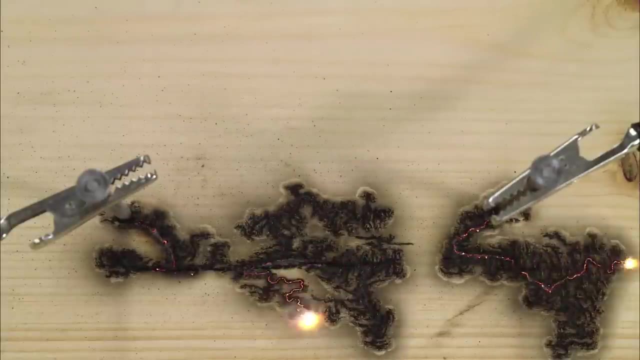 Like water, electricity tries to find the easiest route to get from one place to another, But sometimes that involves branching out until the right connection is made. Lightning bolts do the same thing when they branch out between the clouds and the ground. Finally, there's a spot where the branches don't connect. 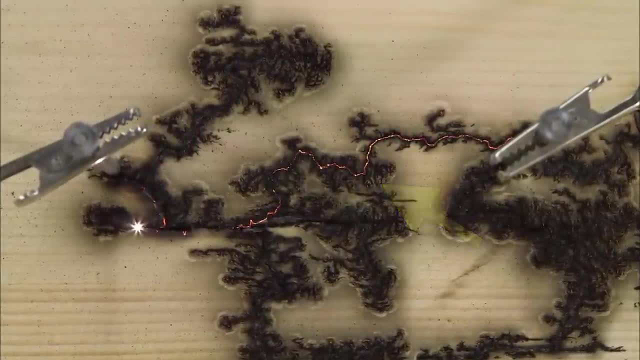 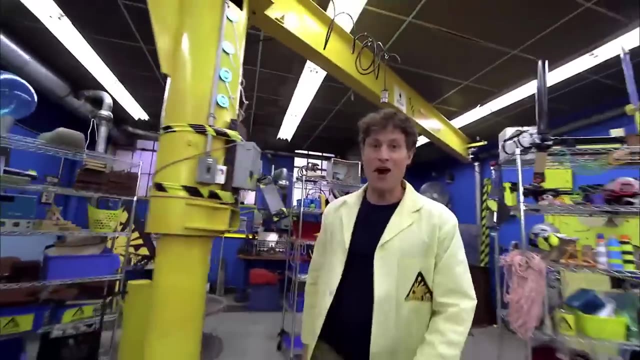 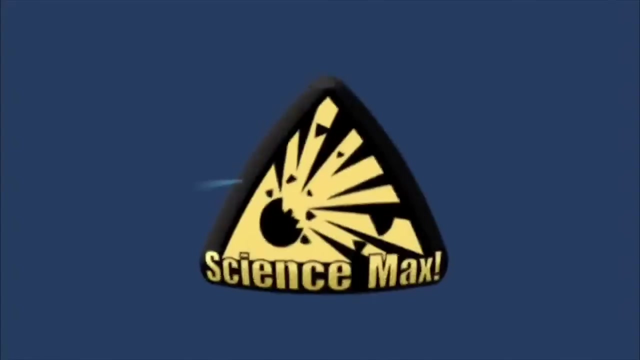 There's a spot where the branches don't connect. The branches meet and the circuit completes itself. Then the electricity follows this one path, ignoring all the others, And there you go. We just watched a lightning bolt happen in slow motion Science. 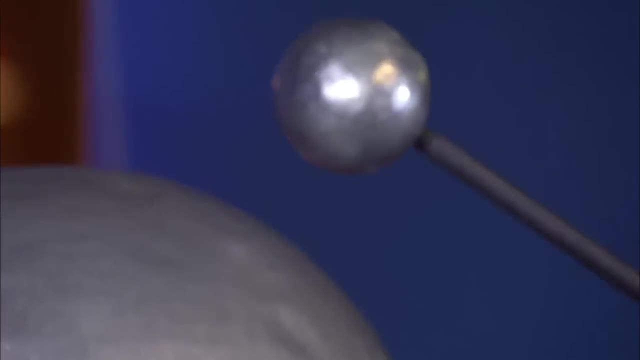 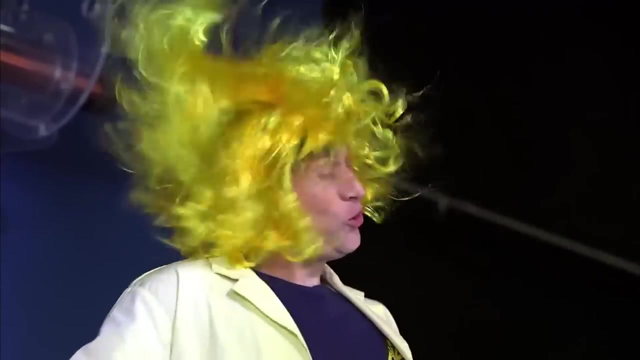 Back to our main experiment, where Heather and I are on a quest to use static electricity to recreate a lightning bolt. Our experiments with the Van de Graaff generator had some hair-raising results, But Heather has another experiment she wants to show me. This is Jacob's ladder. 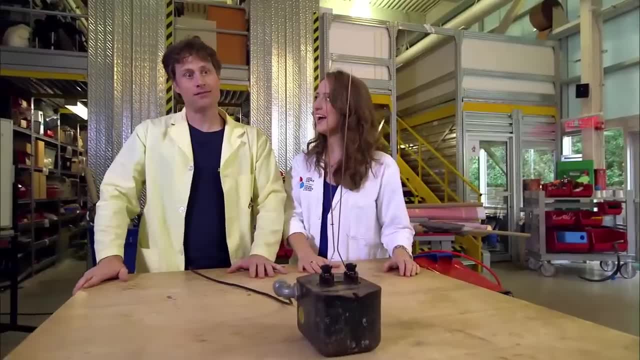 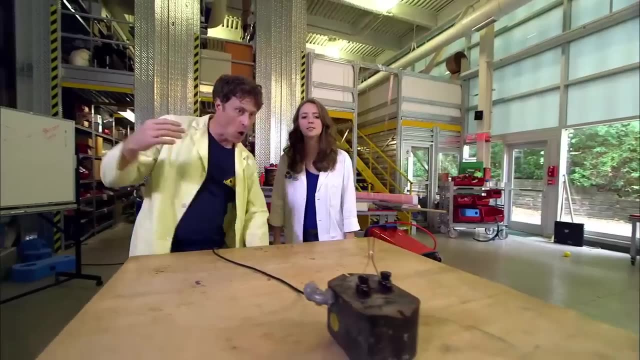 Oh, so this is another way to make. lightning, Yes, Lightning, Yes, Let's do it All right. How do we get it to go? All right, So we want to turn it on. Behold, Oh, turn it on. 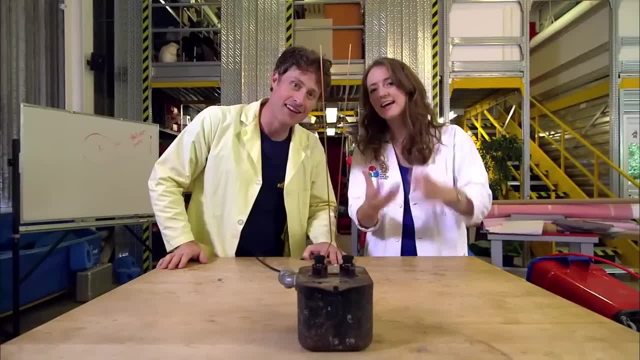 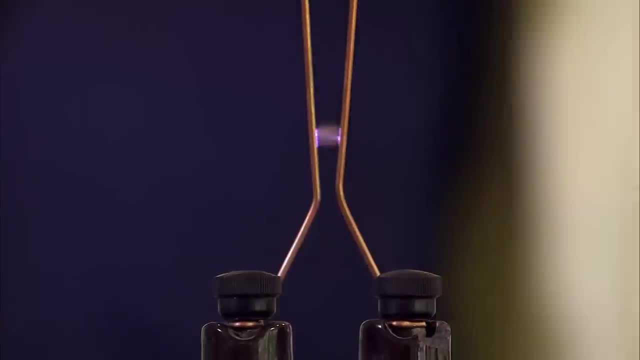 OK, Go, Oh, Look at that. You can actually see that light climbing up between the two copper wires. That's why you call it Jacob's ladder, because it's got the rungs of the ladder. Yeah, Between these two points there's a really great chance. 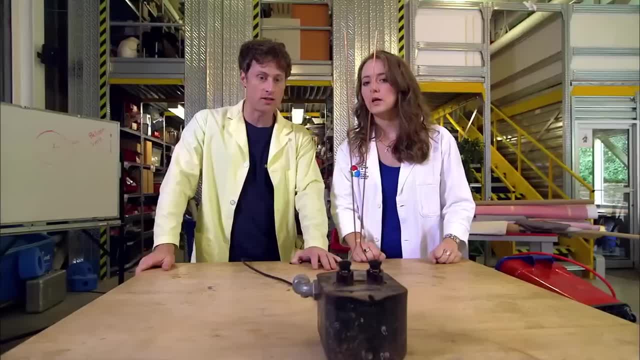 Oh, There's a really great charge difference, right, OK. So what's the difference? 10,000 volts, if you're looking at it. 10,000 volts, Yeah, And volts is how you measure the difference in charge. 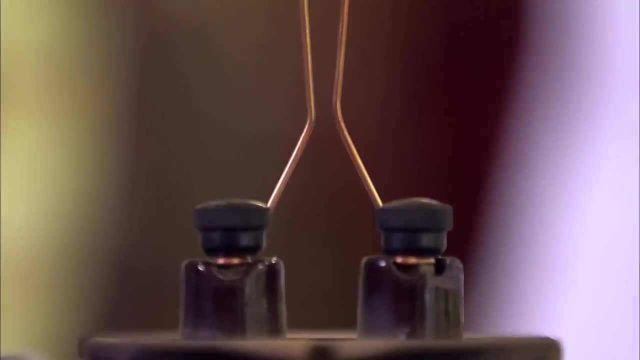 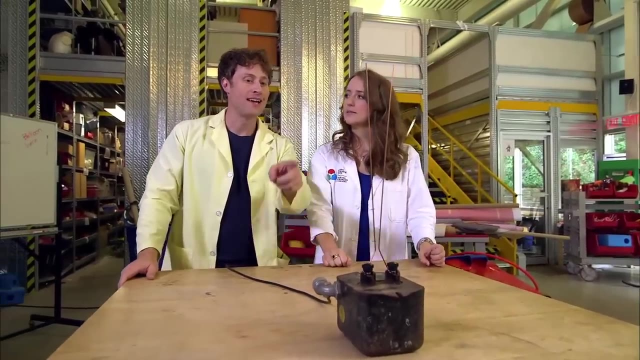 Exactly. Why does it go up? So it goes up because, rather than just staying at the closest point, it's because we're heating up the air. Oh, So, at a certain point, yeah, So hot air rises, Hot air rises. 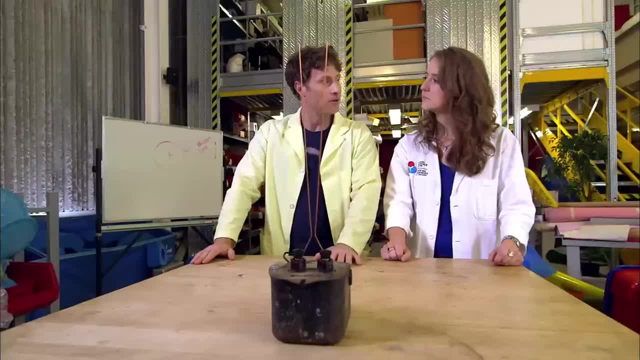 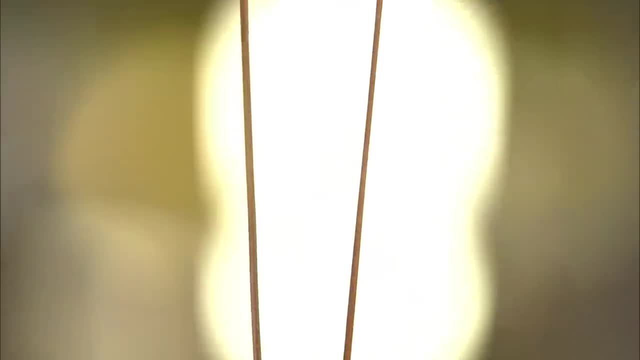 And it takes the electricity with it. So if we cooled the air it wouldn't go up, Wouldn't immediately go up, yeah, And there it goes, And it heats back up again. Yeah, That's neat. OK, So we have a Van de Graaff generator. 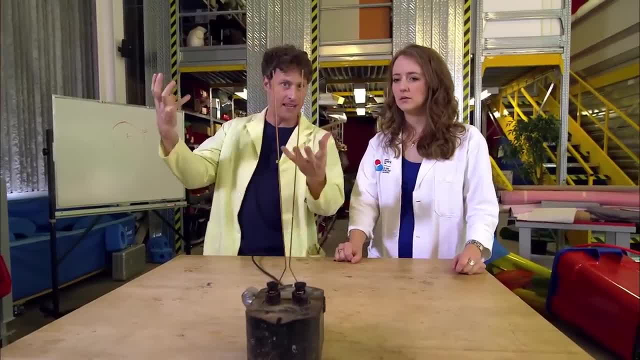 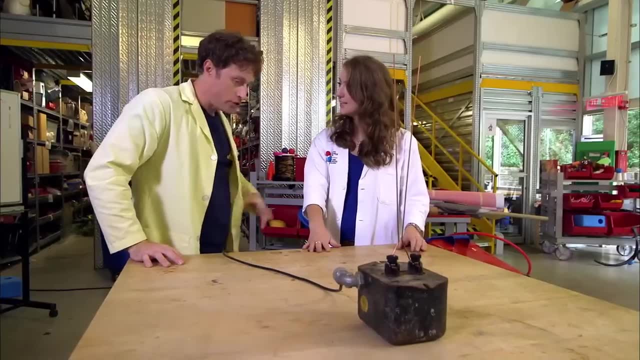 We've got a Jacob's ladder. Are there any other devices that make lightning like this? Oh yeah, There's other things, like the Tesla coil. Really hot, I have a Tesla coil. You have a Tesla coil, I do, I've got one at the lab. 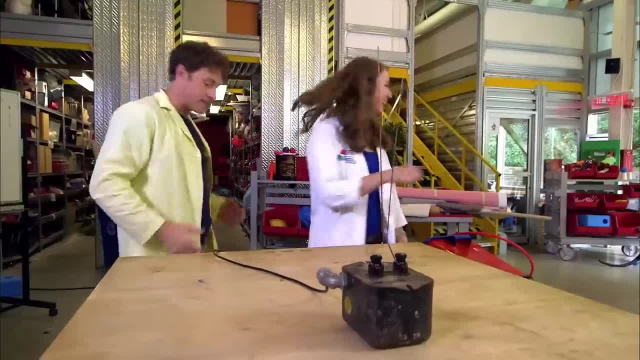 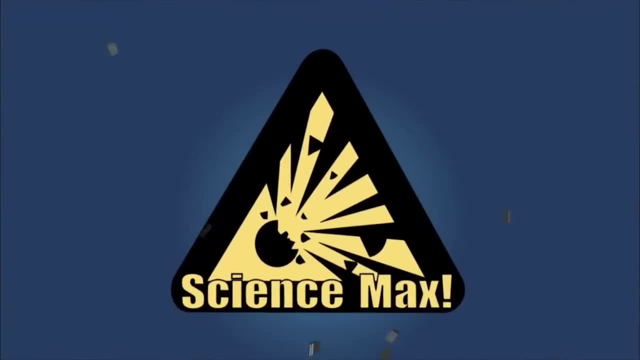 I've just never known how to hook it up. Oh, I can help with that. Yeah, Really, Yeah, OK, Let's do it. Great, Let's go back to the lab. All right, Let's do it. By now, you're probably an expert on what happens when you rub a balloon on your head. 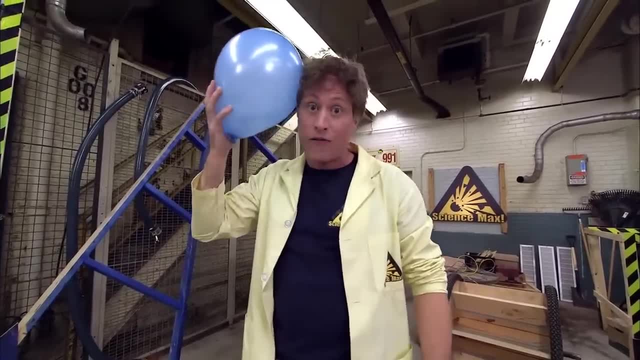 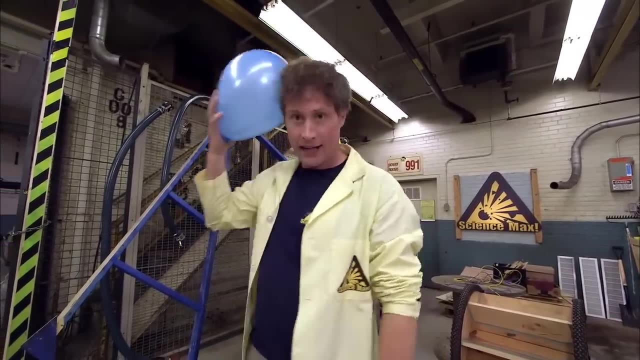 right, The balloon becomes negatively charged, which means it will attract anything of an opposite charge or anything positive or anything that is neutrally charged. like me, Look at the hairs on my arm when I bring the balloon close. Whoa, You see. 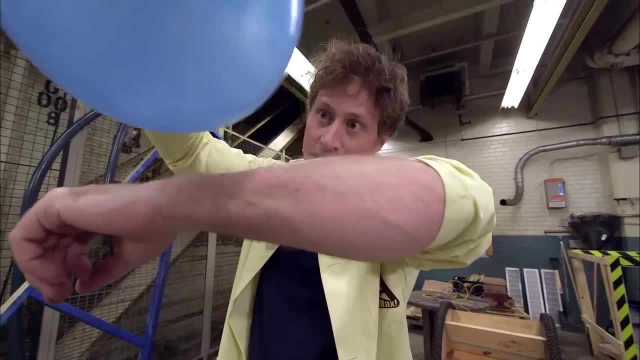 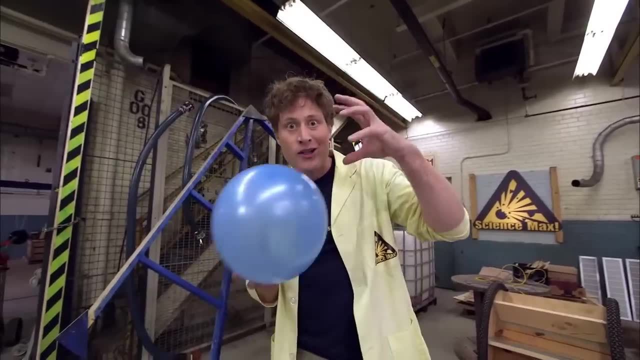 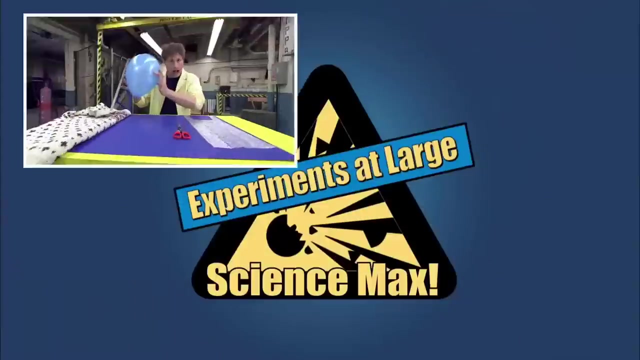 The neutral charge in my body is being attracted to the negative charge in the balloon. So if something is negatively charged, what happens If you bring something else negatively charged nearby? well, they'll repel each other. And here's an experiment you can do: to make something fly using static electricity. 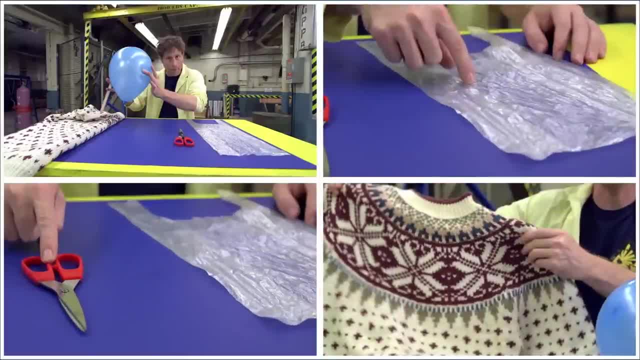 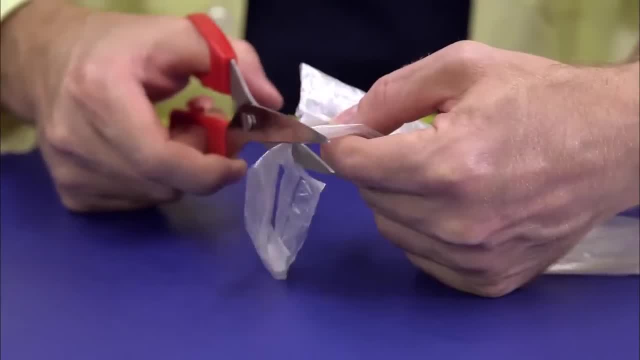 You'll need a balloon, a sweater, scissors and a plastic bag out of the thinnest plastic you can find. Fold the bag up and cut off the bottom. You don't want that part. Then cut another strip from the bag. 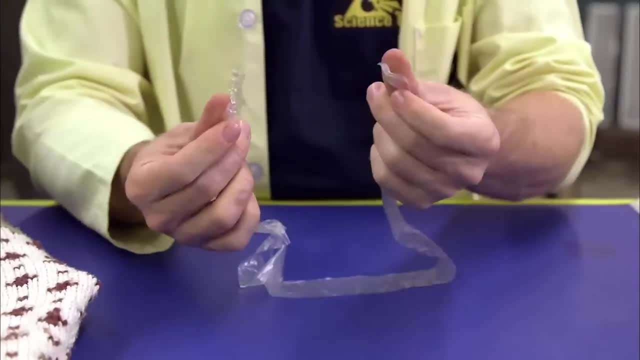 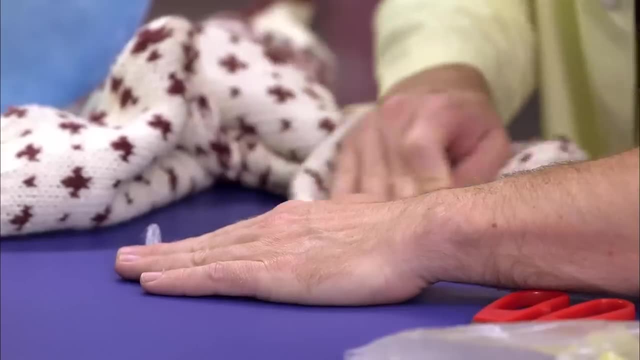 This will give you a hoop of plastic. I find it works better if you break it and tie it again. OK, Lie it flat and rub it with the sweater. This will give it a negative charge. You'll know you've got enough of a charge when it really wants to stick to the table. 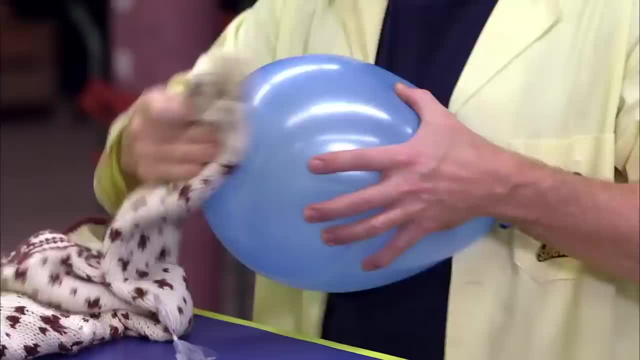 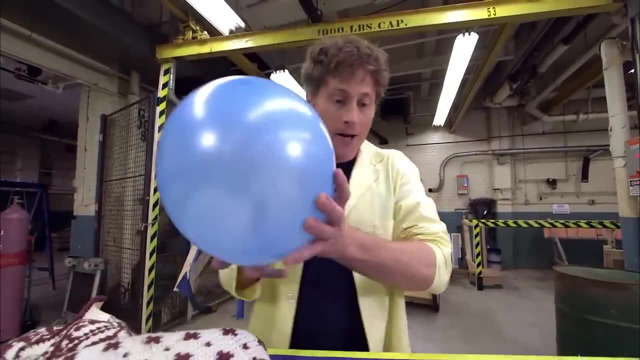 Then take your balloon and rub the sweater on the balloon to charge it up, Because both the balloon and the hoop have negative charges. they repel each other. Then put them together and it will repel And you can get the hoop to levitate. 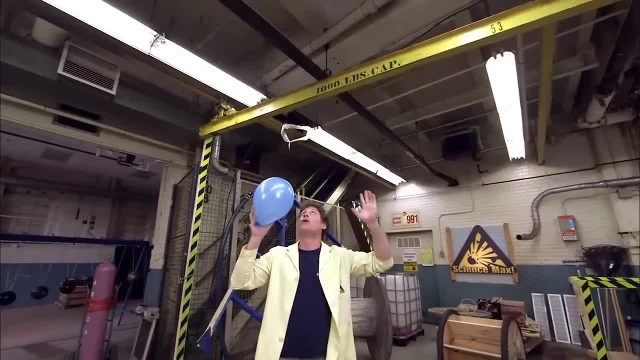 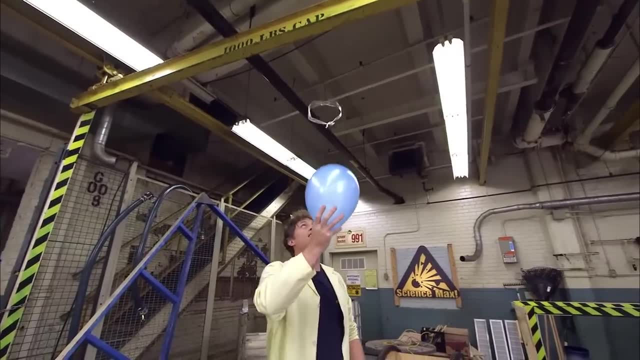 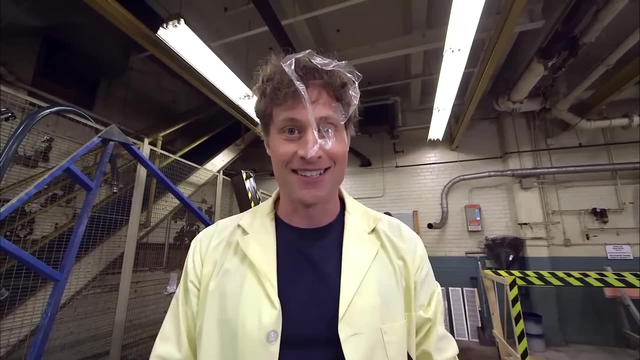 Ha ha, It floats. Here's a floating bag of static charge, But here's the thing You need: to keep it away from your body because if you get close, the bag will stick to you, because you're neutrally charged and the bag is negatively charged. 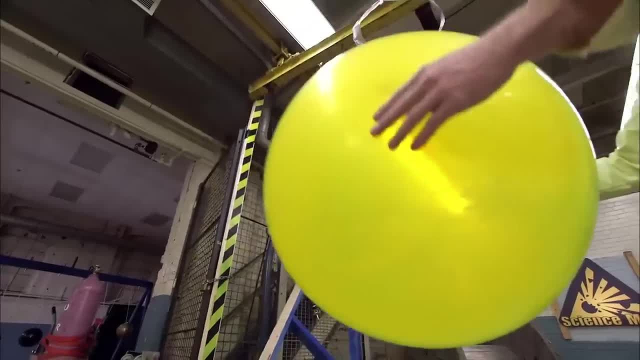 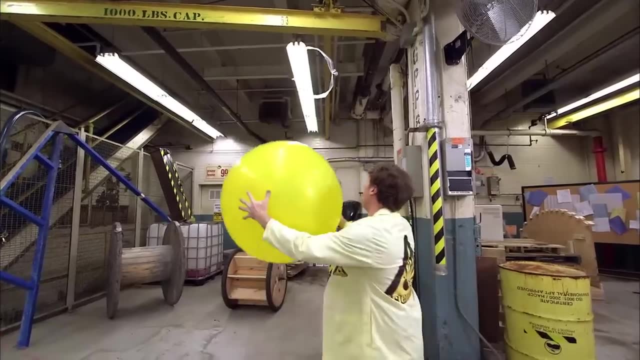 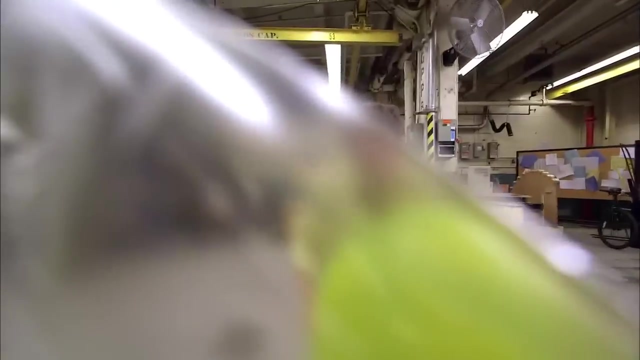 Pretty cool, right? Well, let's max it out. Maxed out, floating static ring. Ha ha, Yeah, Look out, Look out. Oh no, Oh, sorry about that. Uh, Oh well, It was, it was. 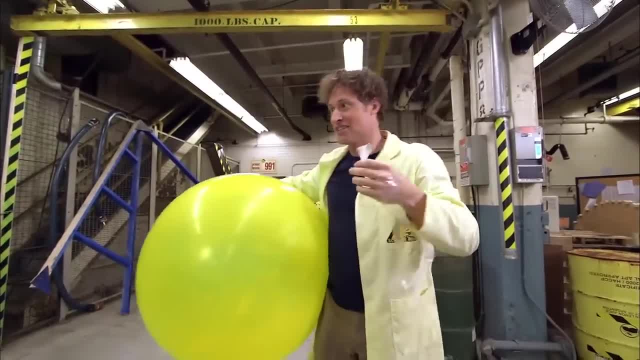 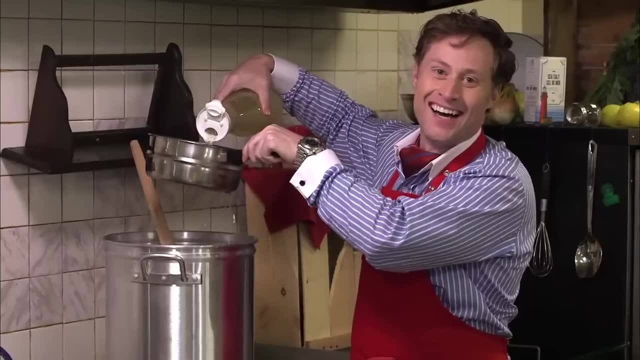 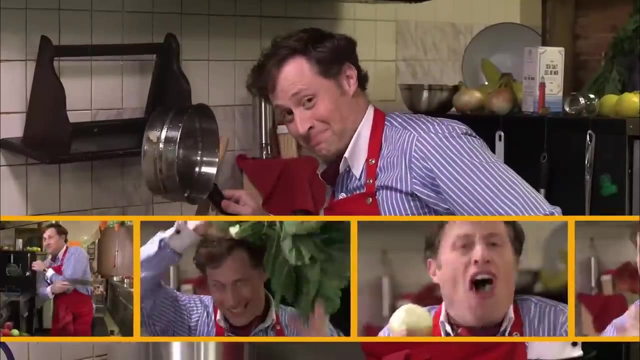 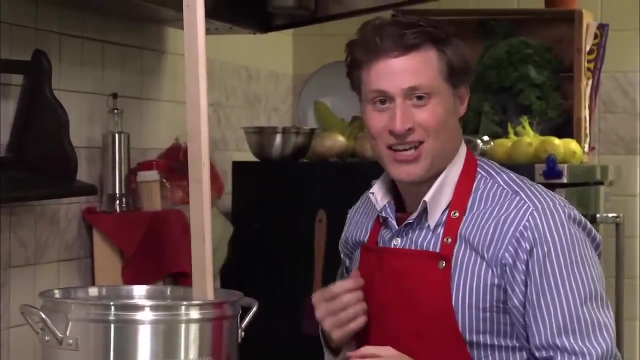 fun. while it lasted, I got to charge these up again. Being a chef is my absolute passion, And cooking up science recipes is my speciality. I'm Buster Beaker and this is Cooking With Science. Oh hello, I didn't see you there. 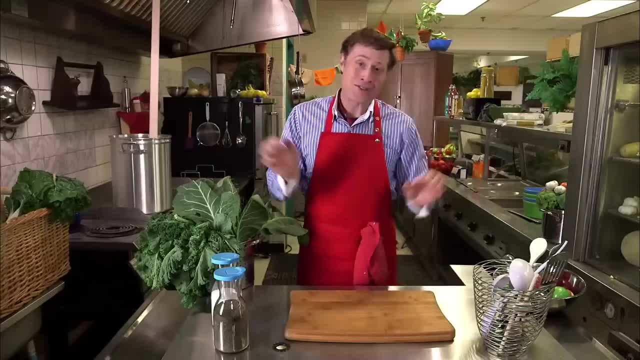 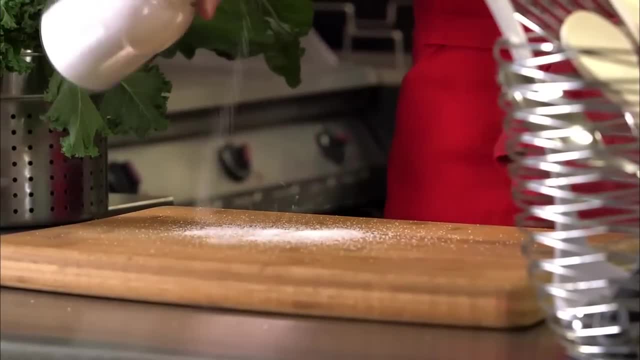 My name is Buster Beaker and welcome to Cooking With Science. Let's say, for example: I've spilled the salt, Oh no, Look at me. I've spilled the salt, Oh, there's salt all over the place. 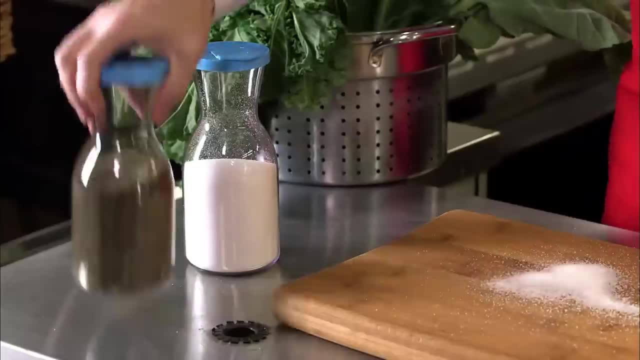 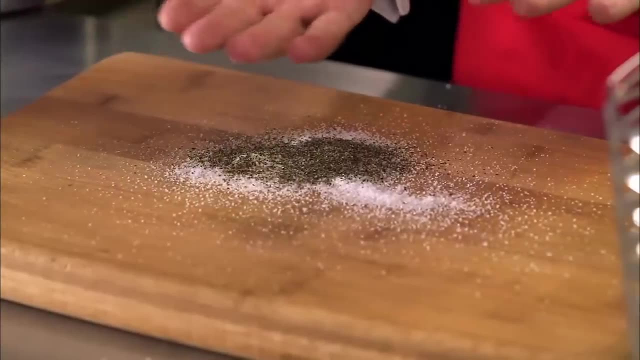 Not really a big deal, right, All you have to do is clean up the salt, put it back in the container. But oh no, I've also spilled pepper on the salt, But that's all right. Separate the But no, Oh dear. 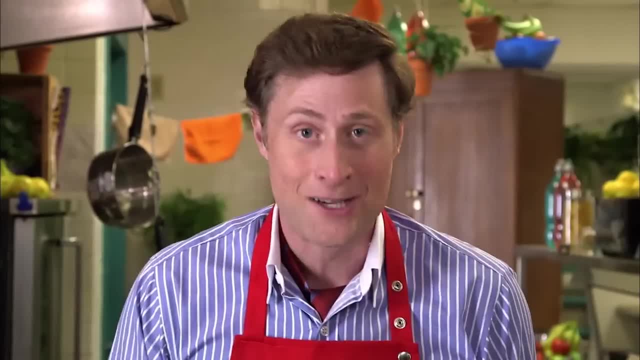 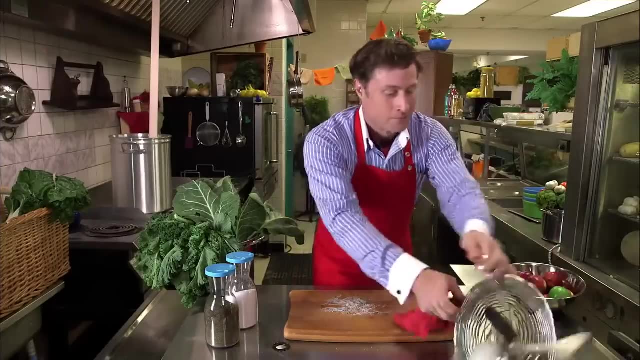 Look, the pepper and the salt are all mixed together. What do I do? Well, here's how you can save the day Using the power of science. All you need is a cloth and a plastic spoon Like Like this one here. 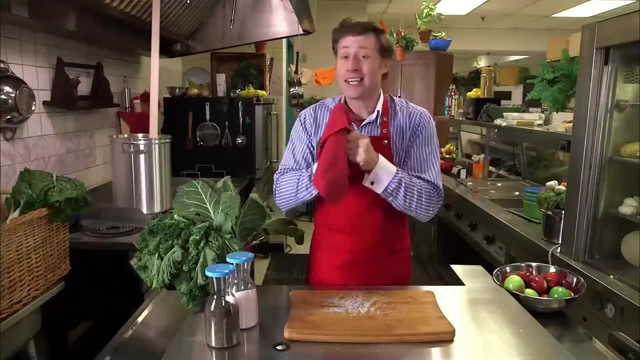 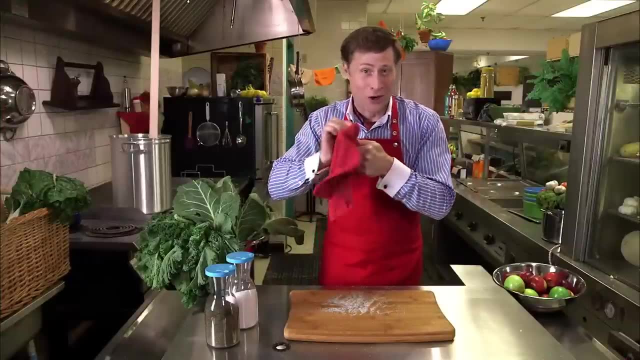 Just rub the plastic spoon on a cloth and you'll be charging it up with a negative charge of static electricity. If it's got a negative charge, it will attract anything that has a neutral charge, just like the salt and pepper. But I know what you're thinking. 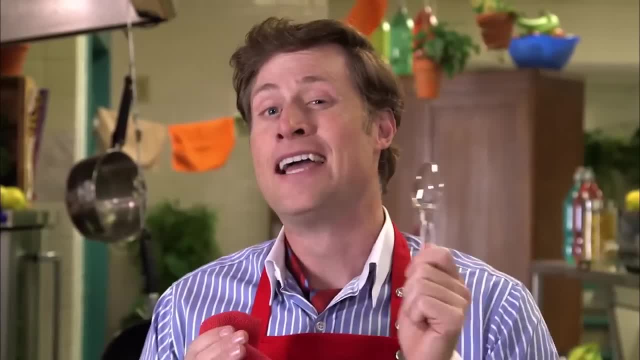 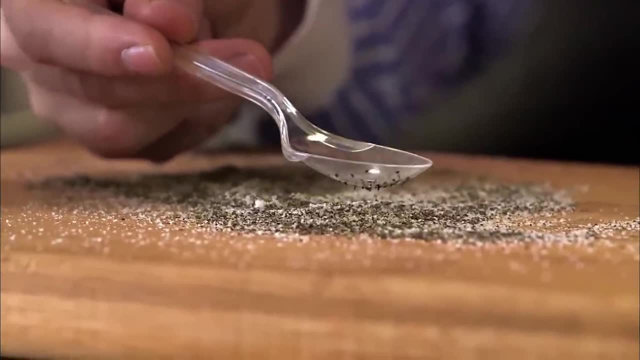 How will we separate them? Well, here's the answer, my friends. Pepper is lighter than salt. Observe: If you hold the spoon high enough, the pepper will be attracted and make the jump up to the bottom of the spoon, but not the salt. 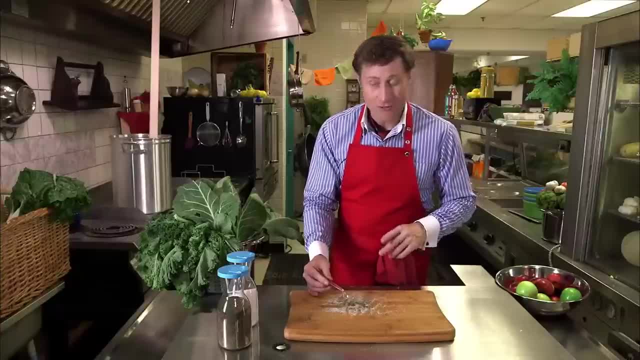 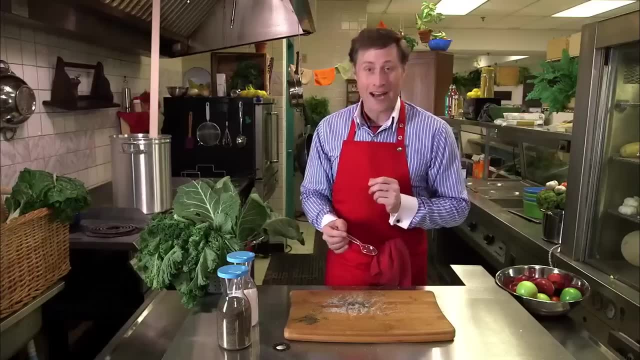 as long as you've got it high enough up, Because the salt is heavier, you'd have to bring the spoon closer, which we're not going to do, And if you tap it off to the side you'll make a nice little pile of pepper. 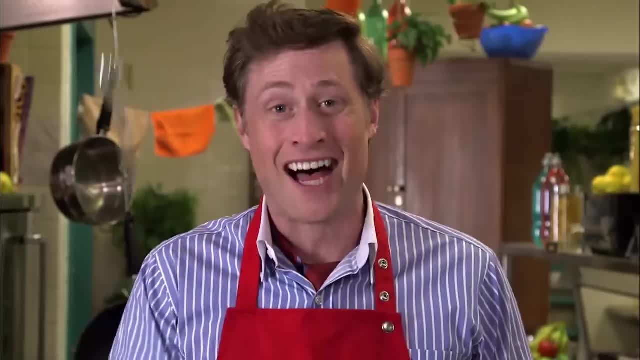 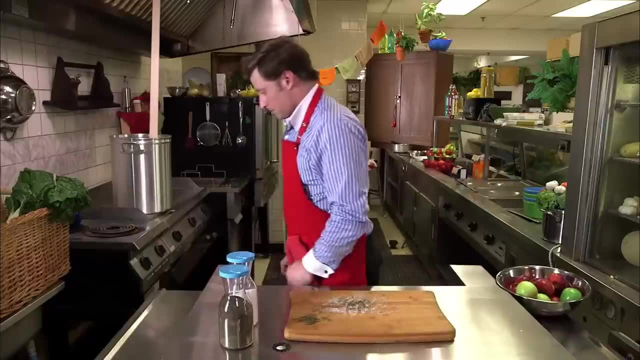 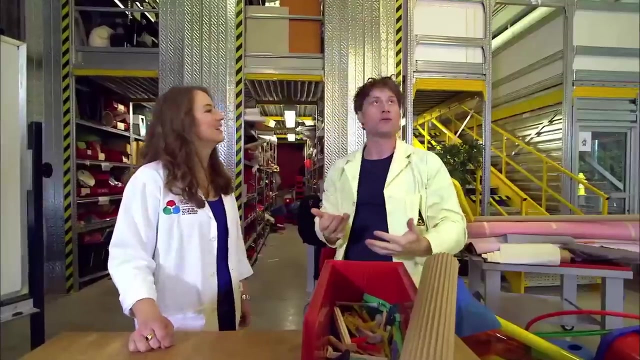 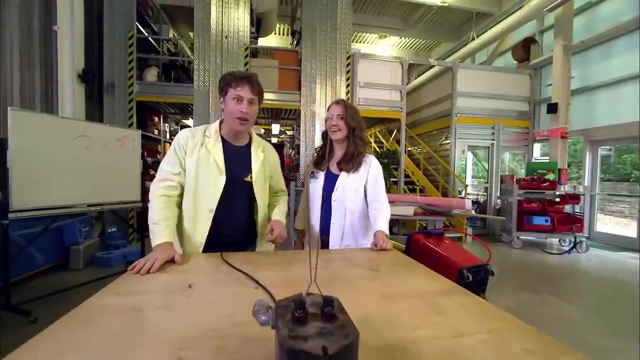 separating the pepper from salt using the power of science. Thanks for watching. Cooking with Science. I'm Buster Beacon Heather and I have been on a quest to recreate lightning using static electricity. We've gone from balloons to a Van de Graaff, to a Jacob's ladder. 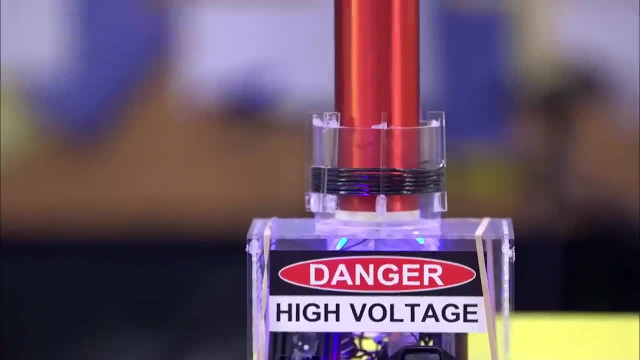 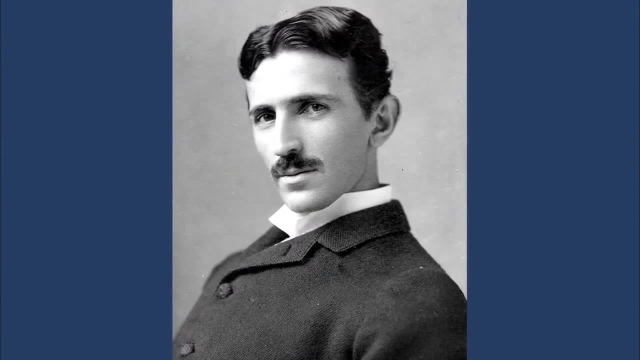 each more lightning-y than the last. Finally, Heather suggests we use a, A Tesla coil. Oh, is this named after Nikola Tesla? Yeah, he invented it. Oh, one of the founding fathers of electricity- right, I love Nikola Tesla. He's cool. 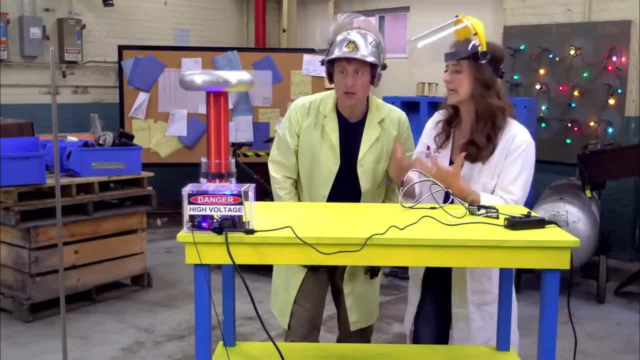 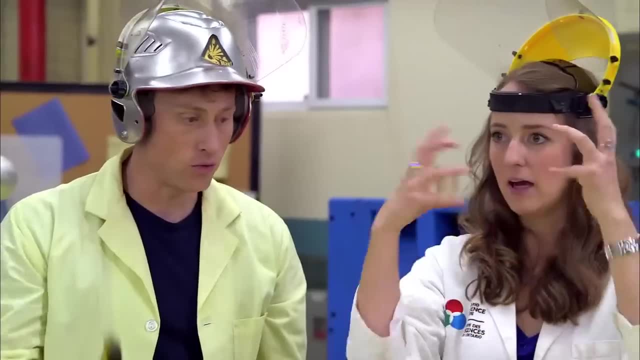 So how does it work? So the way this works is it is a step-up transformer, meaning we take a lower voltage and bring it up and ramp it up to a much higher voltage. Okay, so normal voltage is 120 volts. That's what we have: a normal plug-in socket. 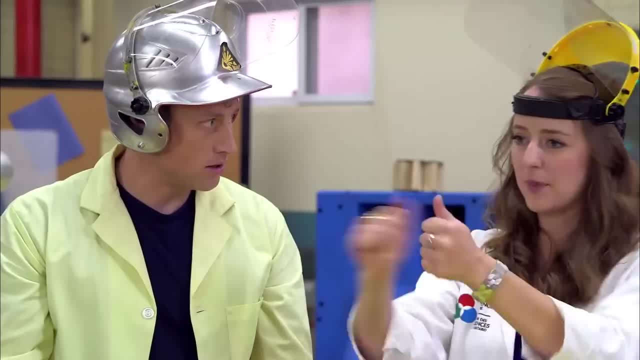 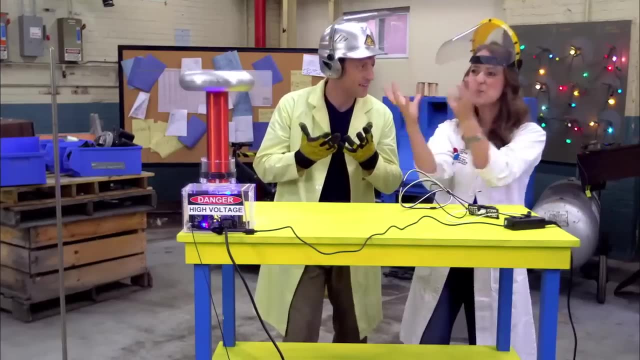 Typically, we're getting it out of: Yeah, exactly, And we're going to ramp that up to really high amounts, upwards of 25,000, maybe even 250,000.. Wow, Volts, That's a lot. And all that charge buildup. 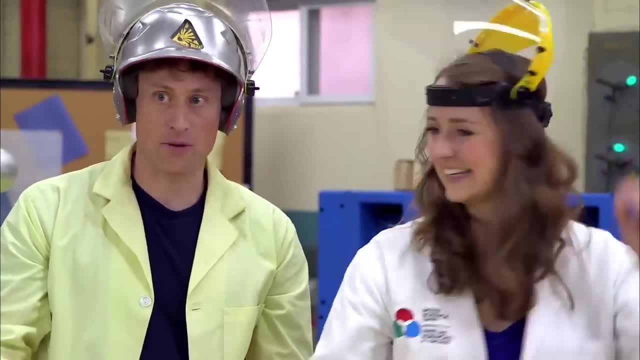 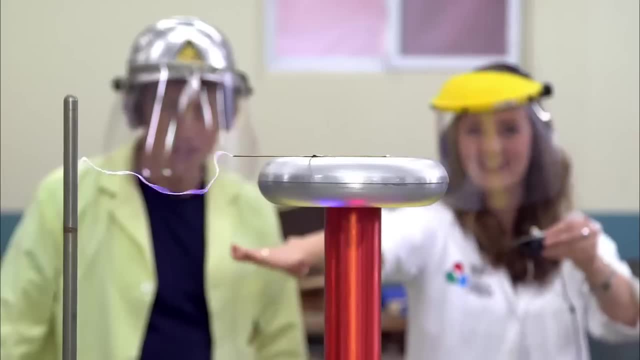 we're going to see something pretty amazing happen. Okay, Do you want to see it? Yes, We stand back there, right? Yep, Let's check it out. And Yeah, The Tesla coil builds up a charge which jumps through the air to this neutral rod. 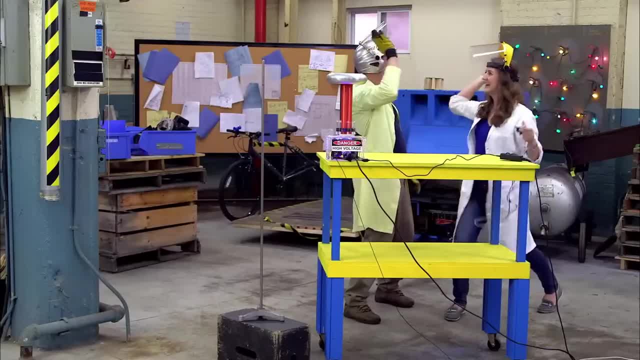 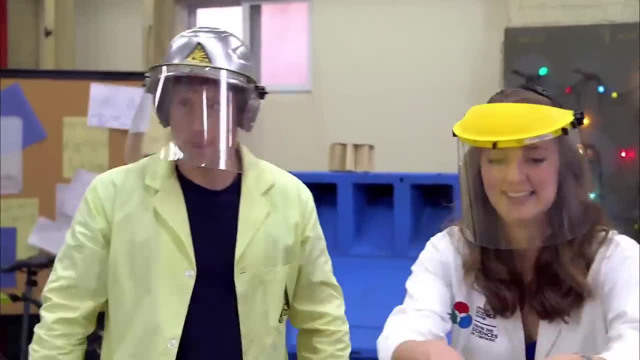 just like a lightning bolt. We made a lightning bolt That totally jumped a long way. That was impressive. That was a really good one. So can you control it? Yeah, It's coming, You want to see? All right, I'm going to lower my frequency. 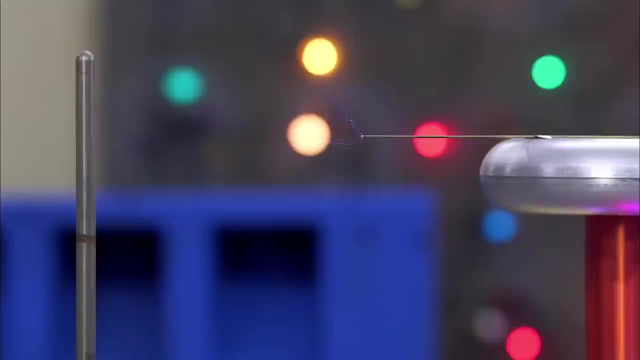 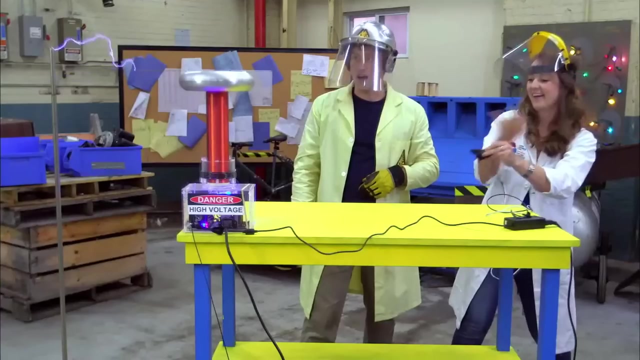 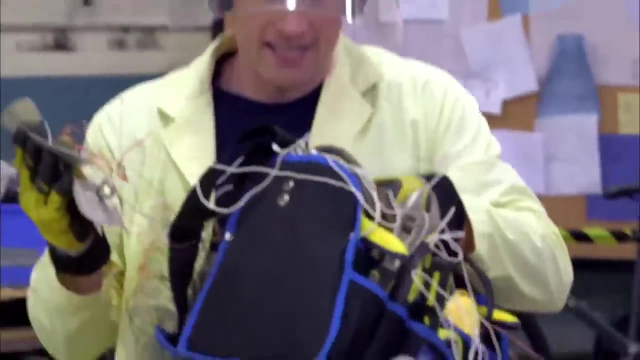 Okay, Let's see what happens. Oh, that's amazing. It's like a scattered lightning bolt. Oh, wait a minute, So you can play different notes. Play different notes. I need five minutes. Hold on, Okay, Okay. 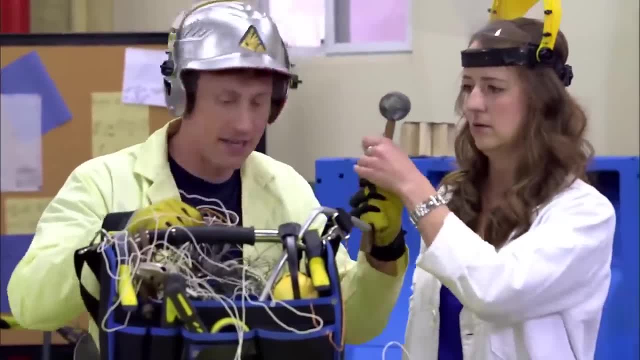 All I need is five minutes. You know what I was thinking. If you can make different, Hold that for a second. If you can make different frequencies, that means you can make different notes, right, Right, So Oh, I don't need that either. 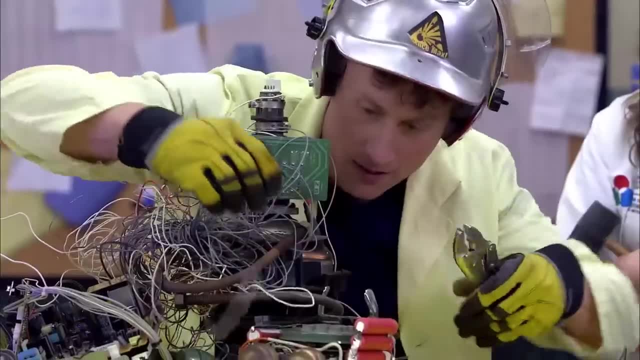 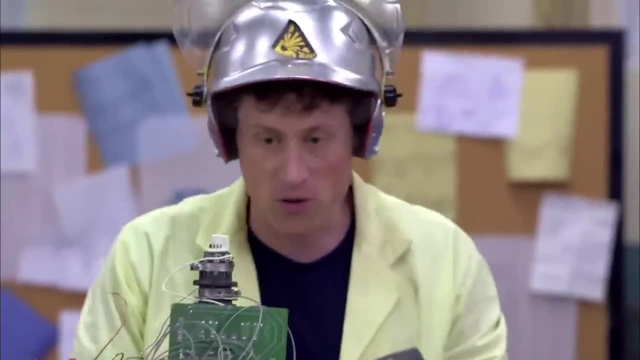 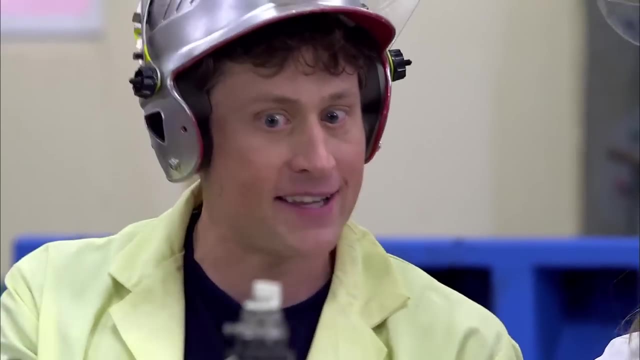 Hold on? Ah, That's not what I need. Okay, One more thing. Can I get that hammer? Yeah, Okay, Ready to go. So what is this? When you told me the Tesla coil could play different frequencies, I thought we could make different notes come out of the Tesla coil. 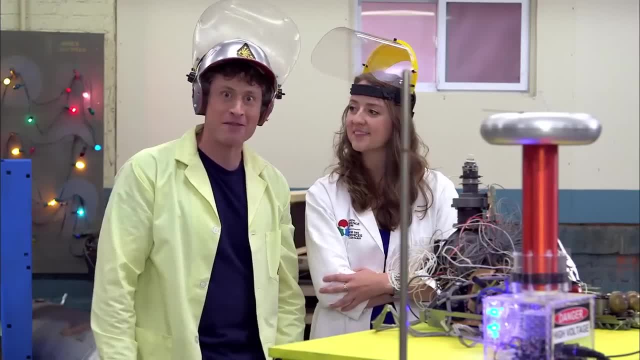 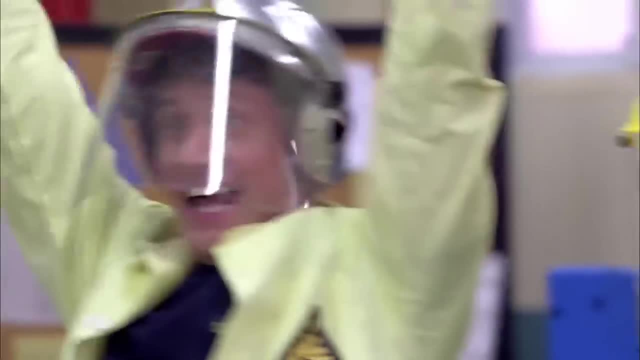 so I programmed it to play the notes of the Science Max theme song. What, Yeah, You want to hear? Yeah, Yeah, We did it, We did it. Yeah Yeah, Science Max: experiments at large Lightning bolts. We created lightning. 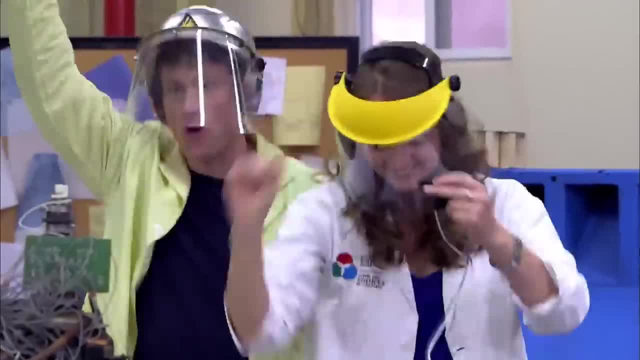 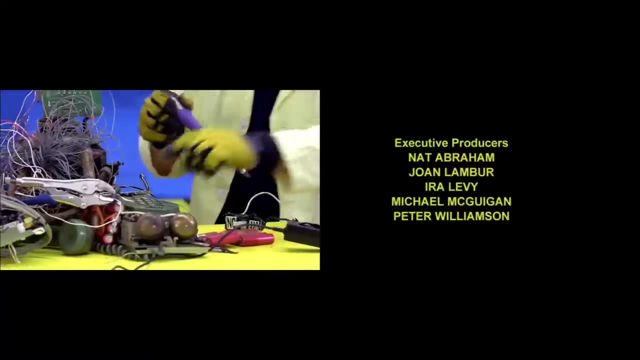 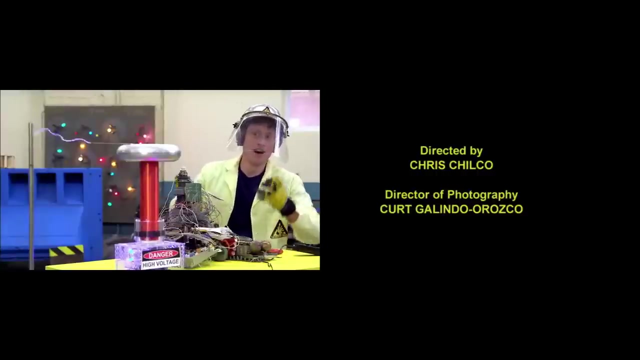 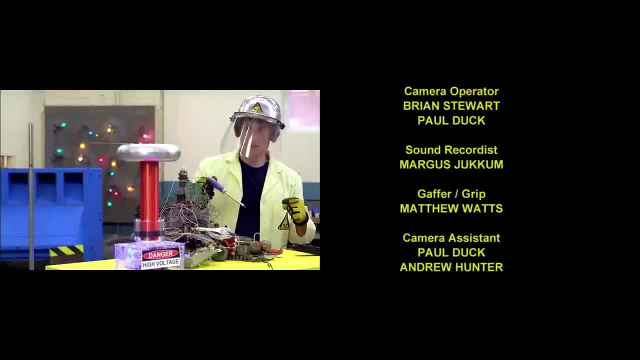 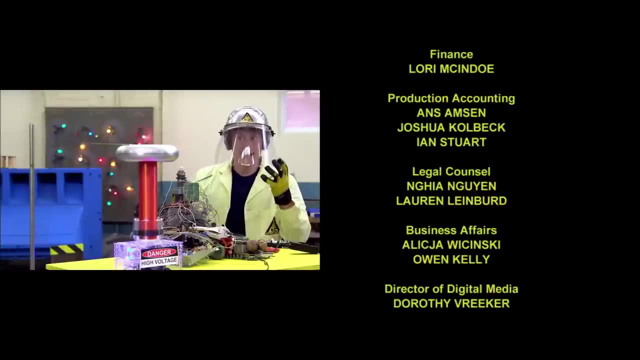 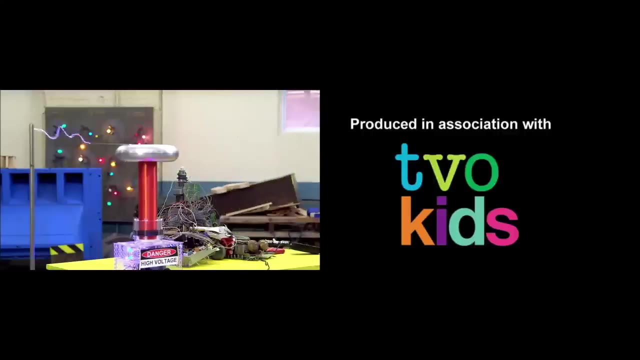 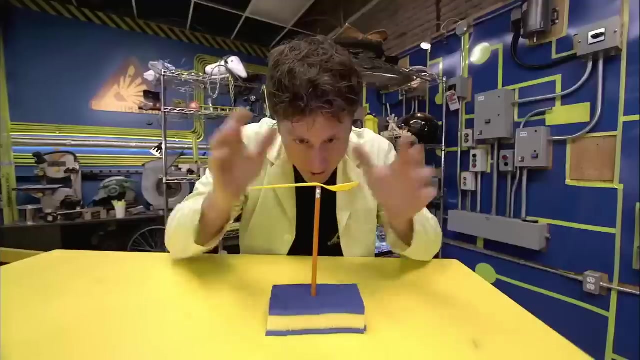 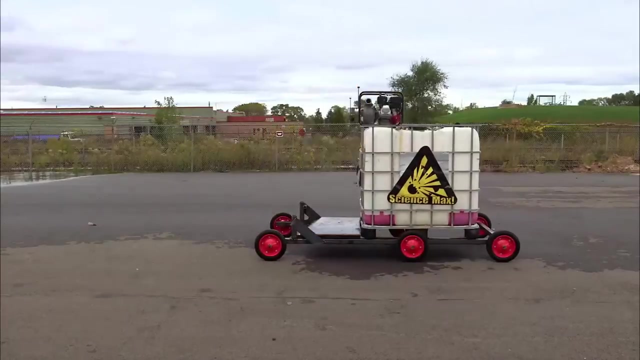 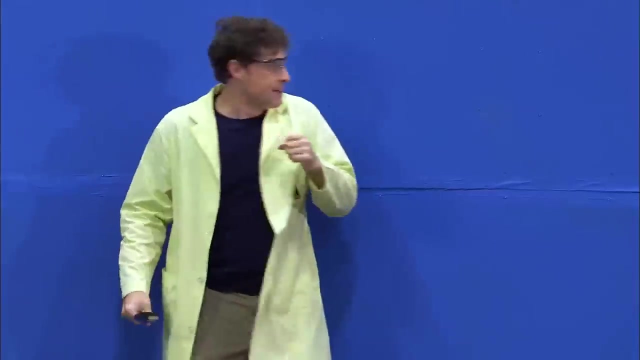 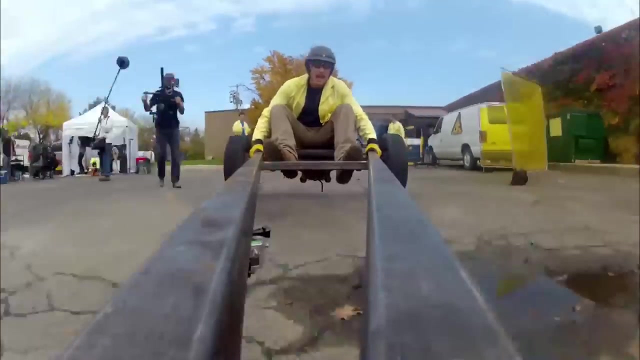 Uh, Uh, I give up. Have you ever done a science experiment and wondered what it would be like if you did it big? I have, My name is Phil and I take your everyday science experiments and do them big. This is Science Max: experiments at large. 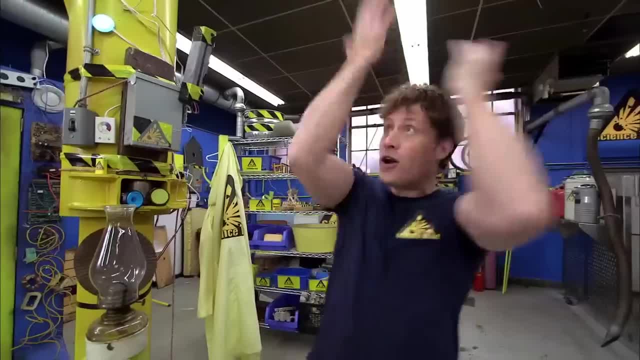 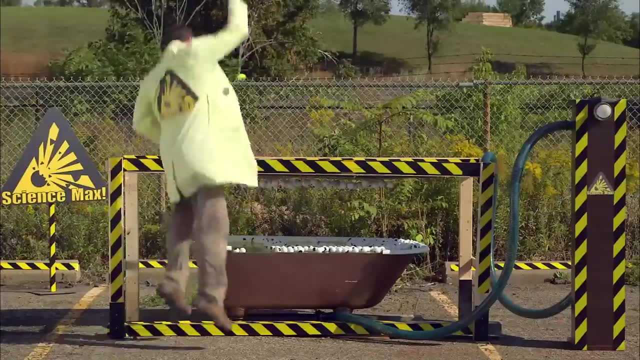 This episode of Science Max is all about generating electricity. Where do we get this electricity? The electricity that we use all the time? We try to generate as much as we can using human power, Plus solar energy, tidal energy, wind energy and more. 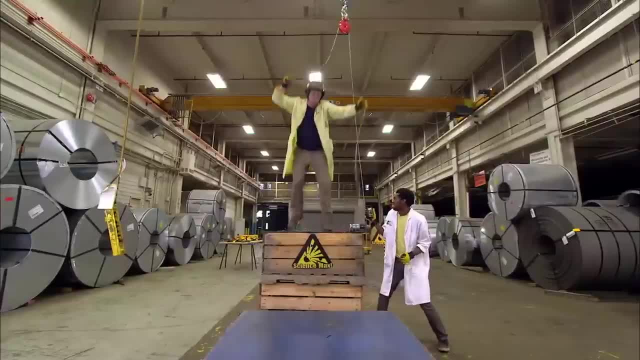 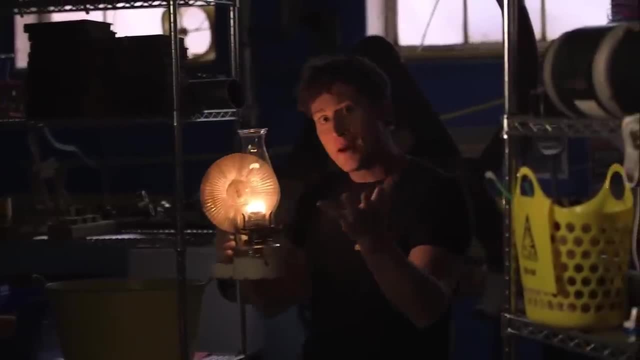 All you need to do is turn to generate All on this episode of Science: Max experiments at large Greetings, Science Maximites. Take a moment and imagine with me, if you will, a time when the only way to light your house was with candles or oil lamps. 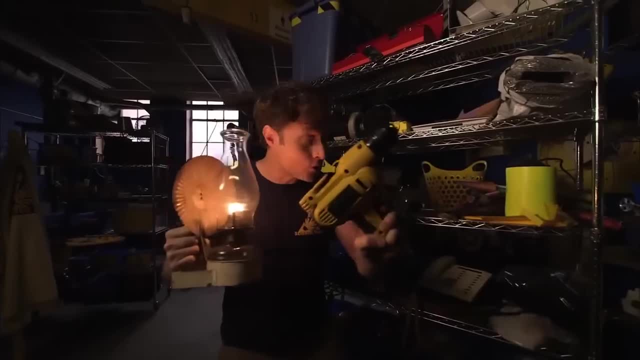 There was no electricity, That meant no power tools, no video games, no telephones and, worst of all, no electricity.